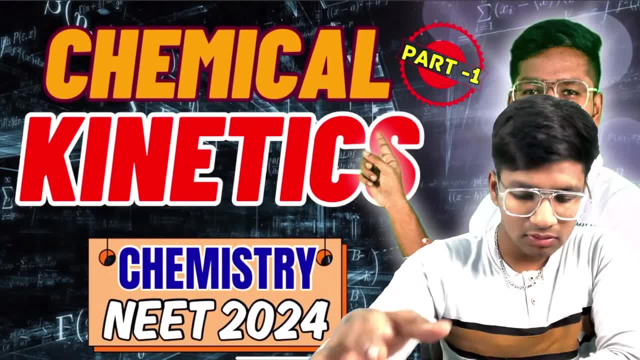 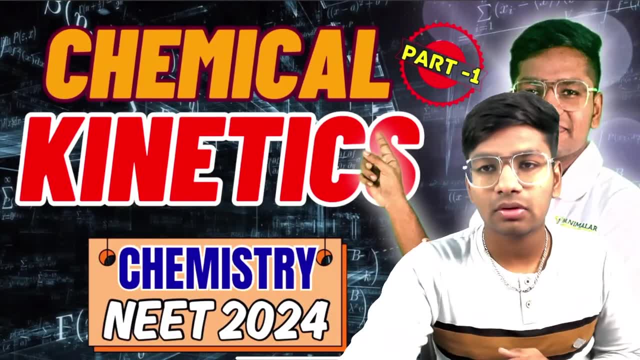 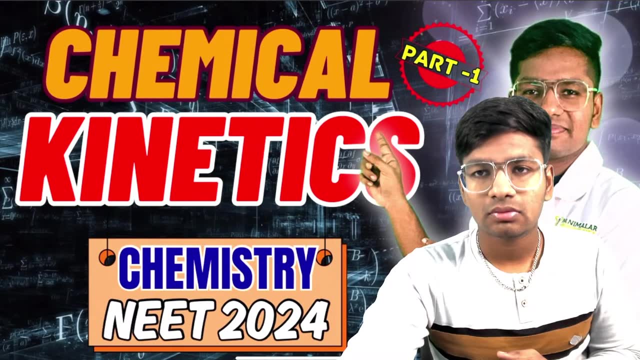 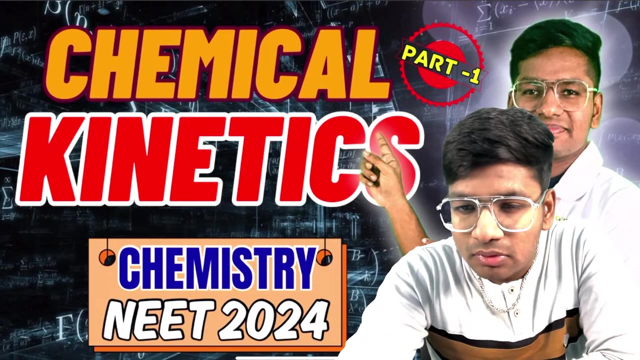 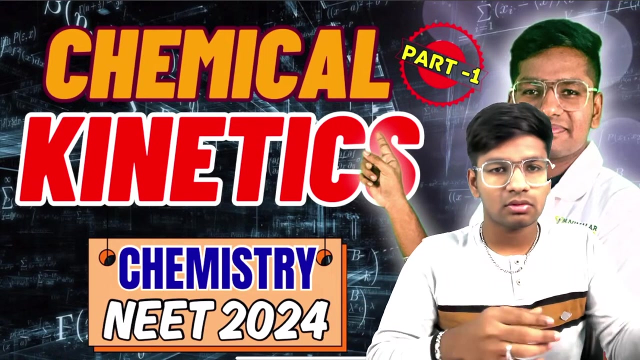 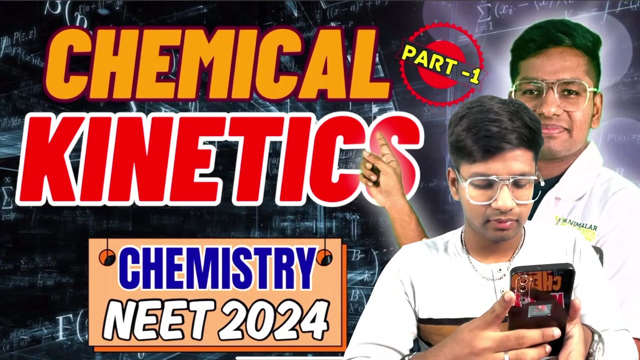 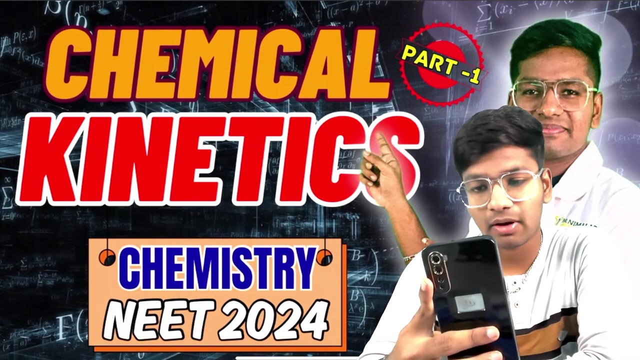 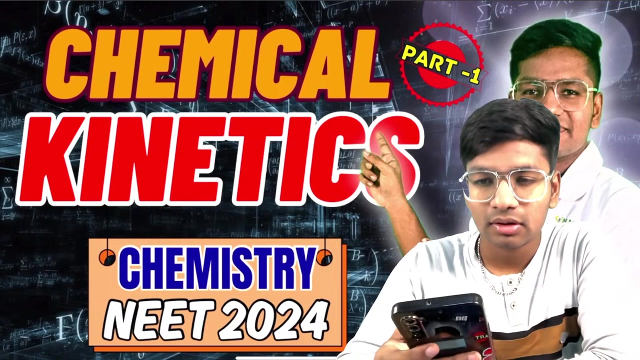 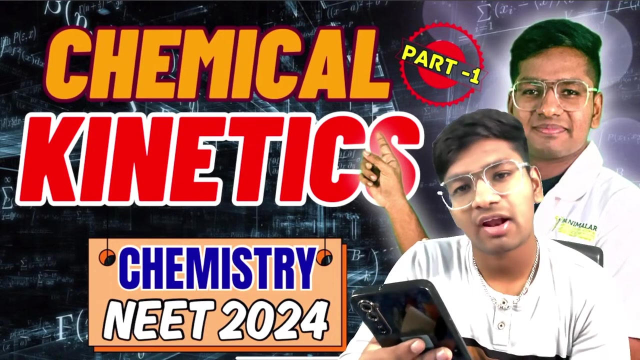 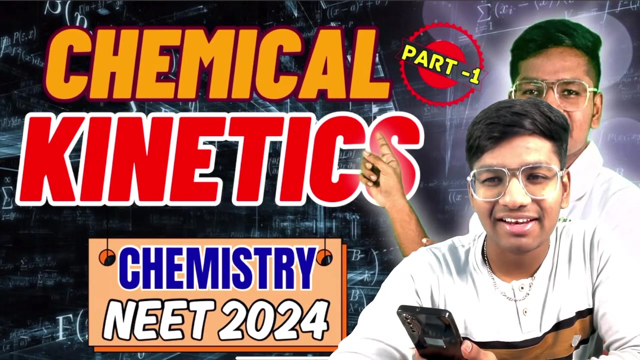 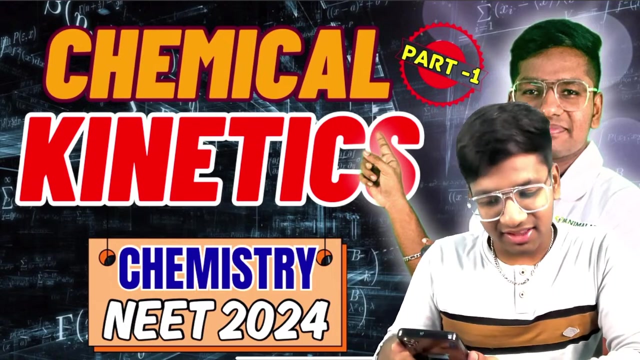 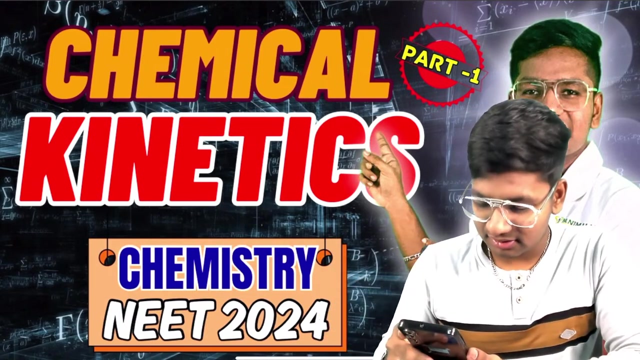 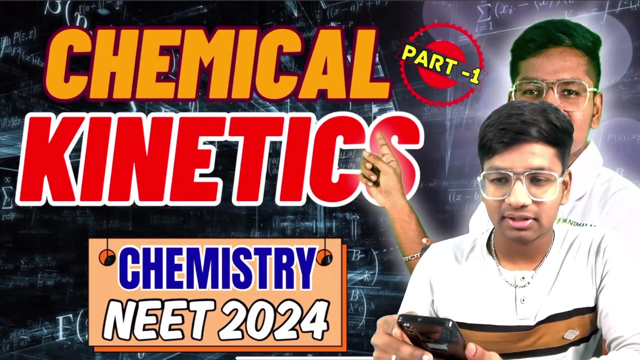 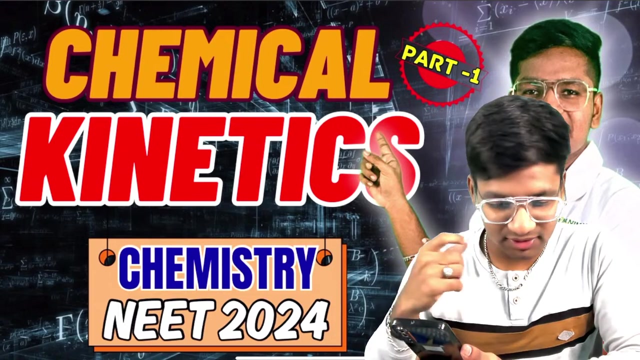 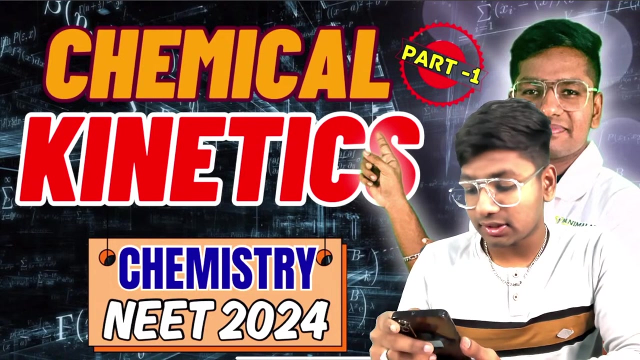 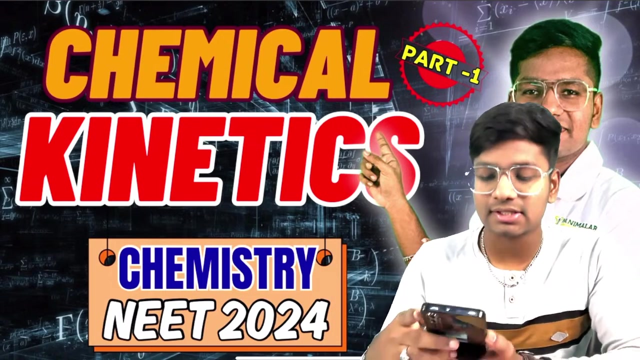 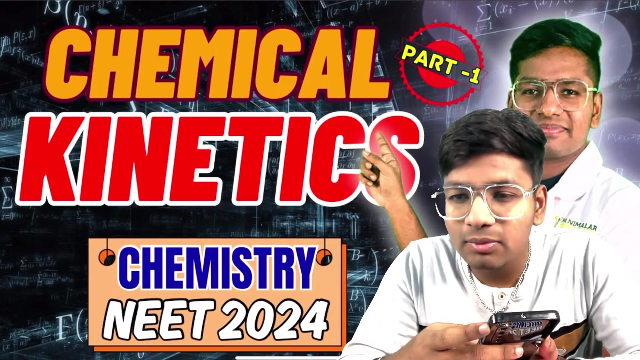 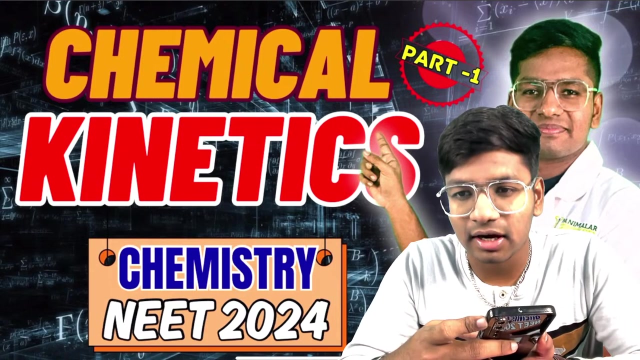 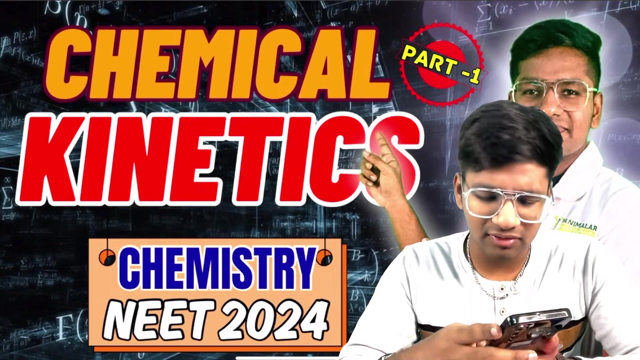 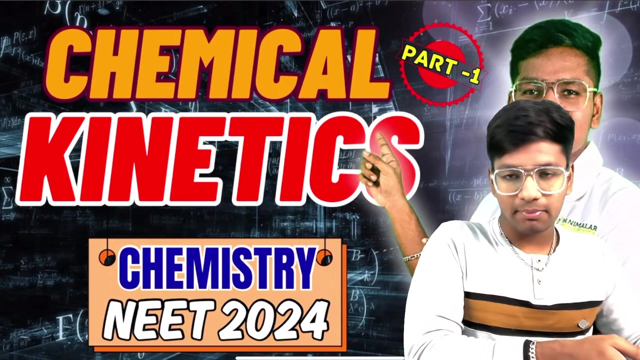 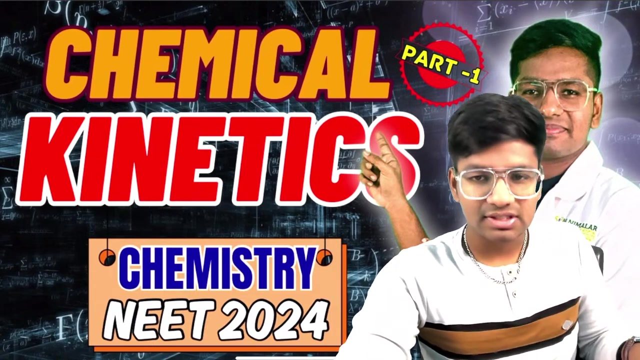 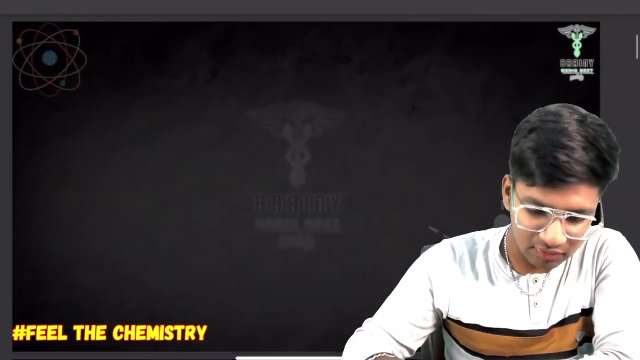 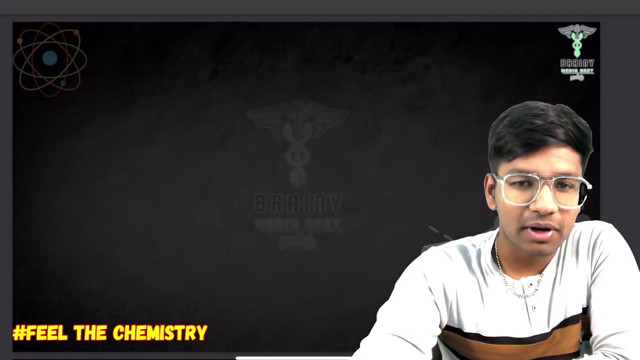 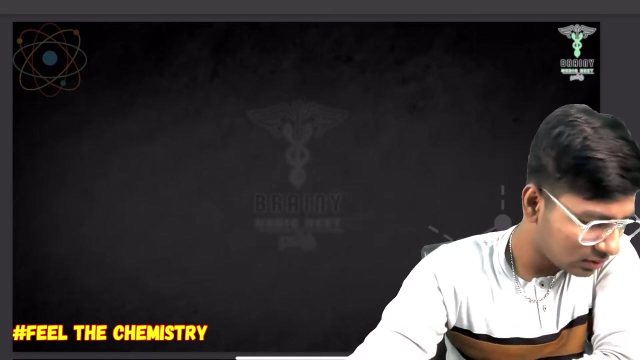 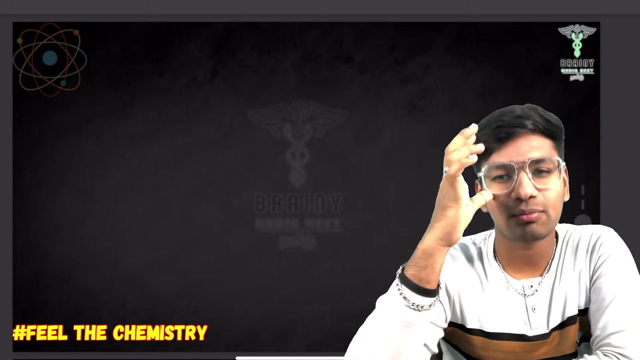 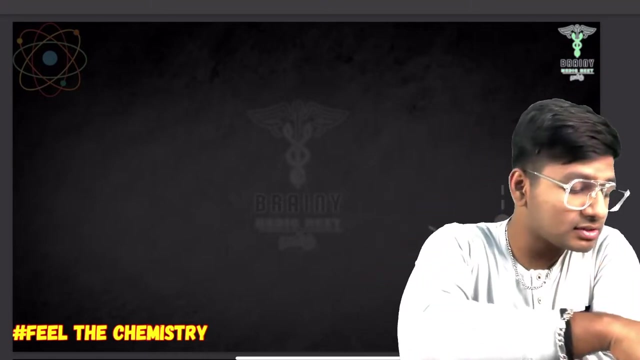 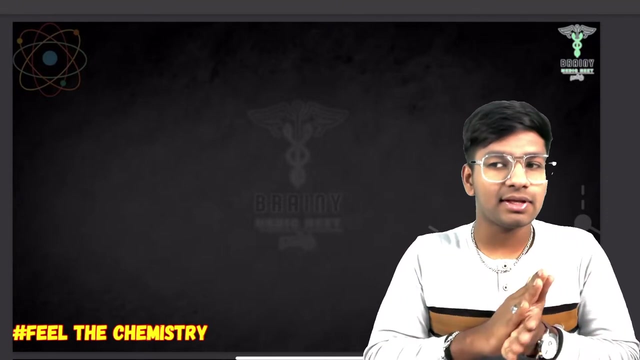 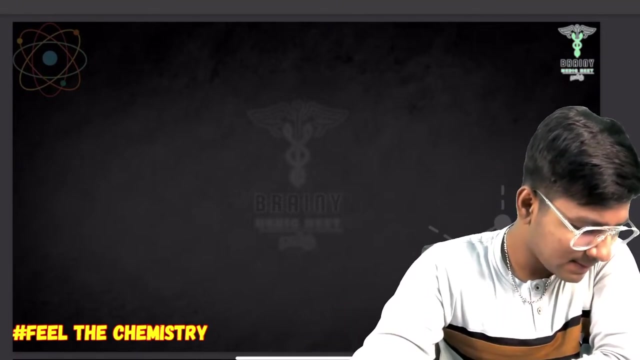 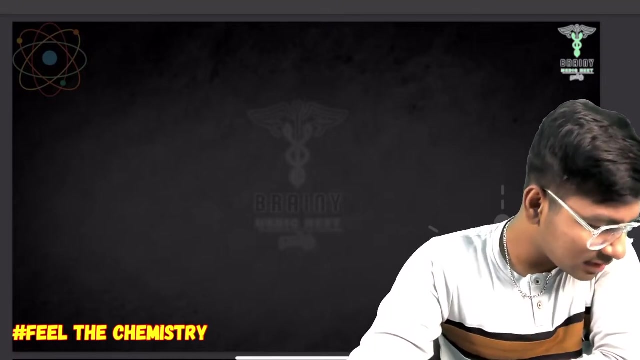 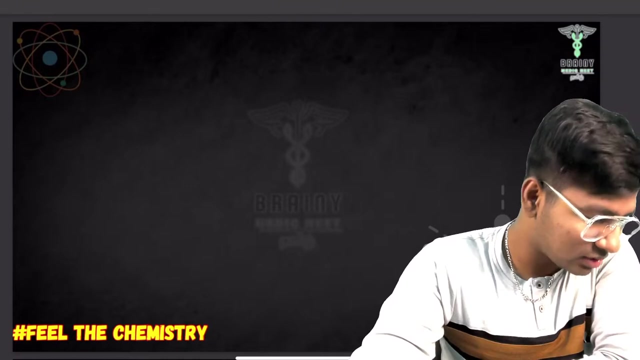 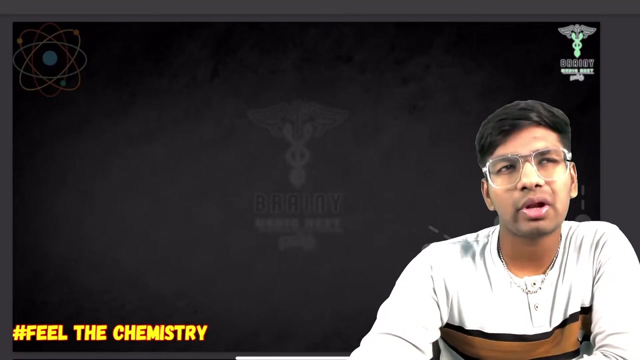 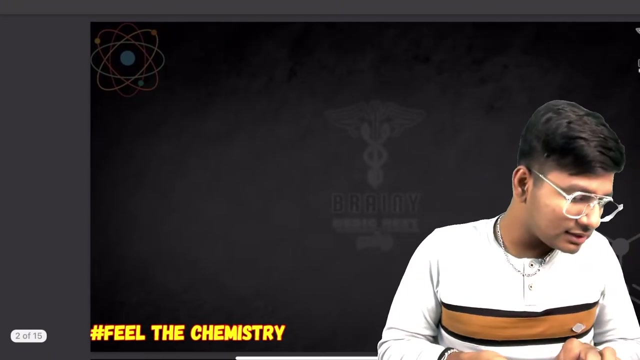 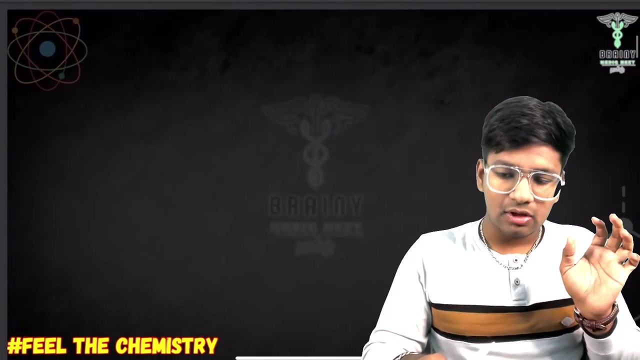 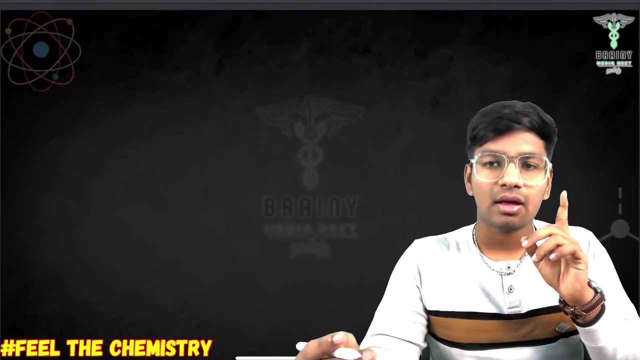 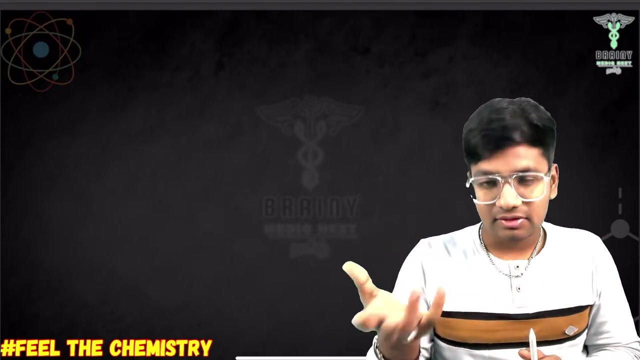 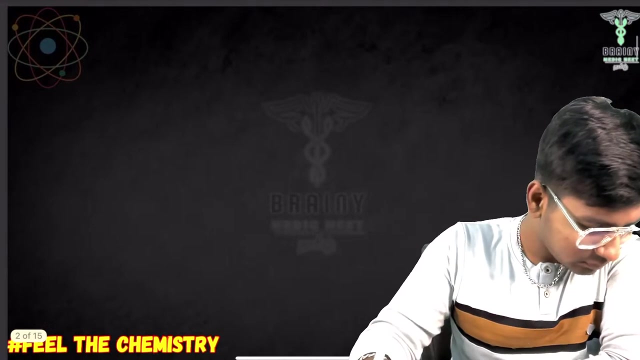 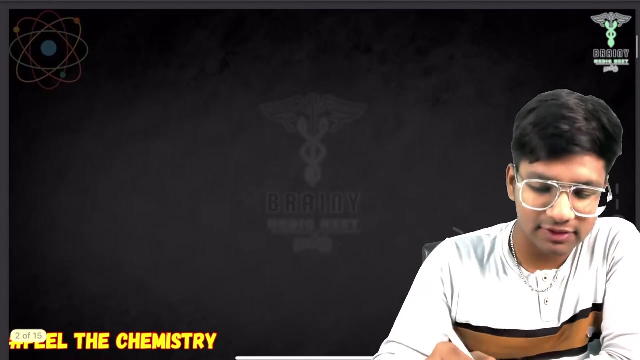 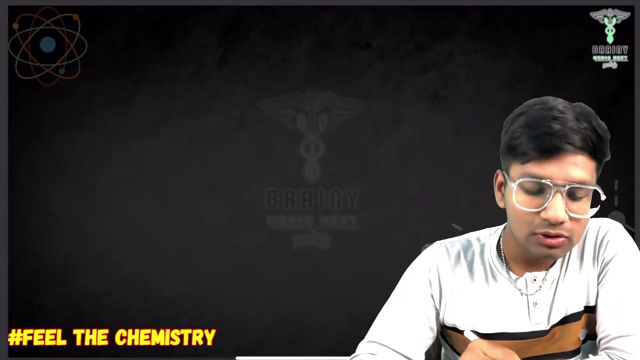 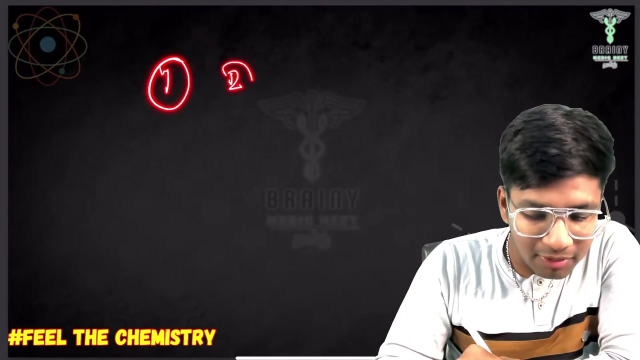 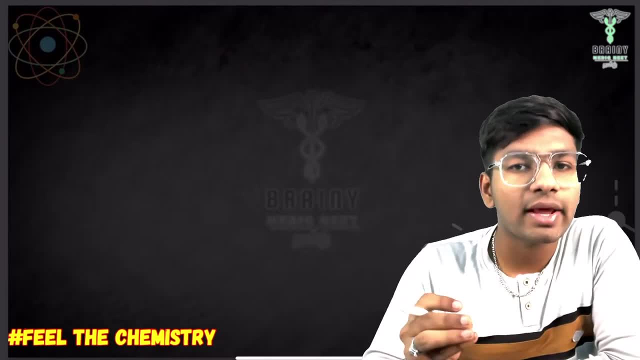 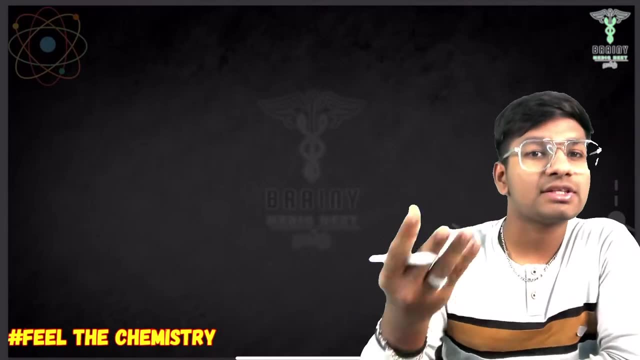 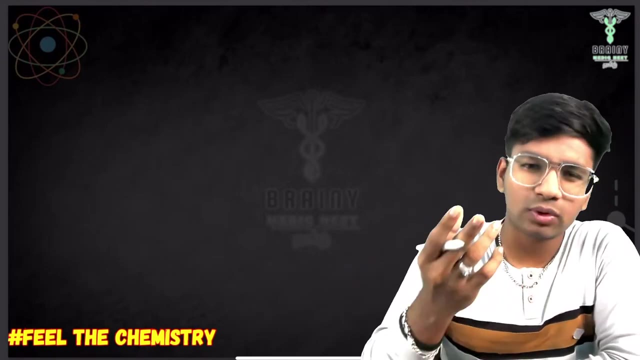 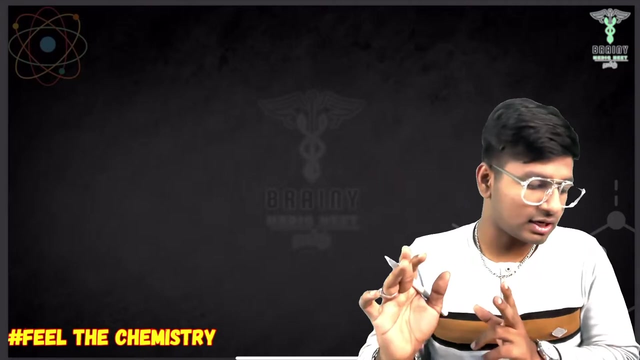 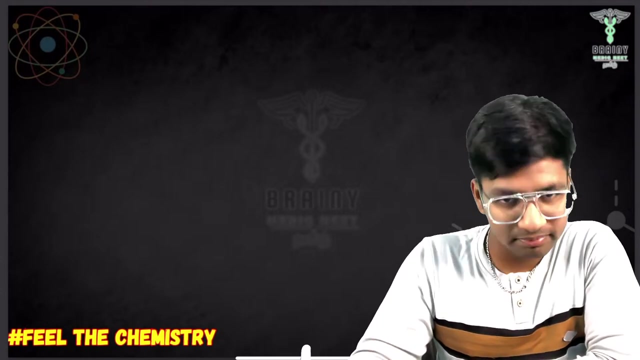 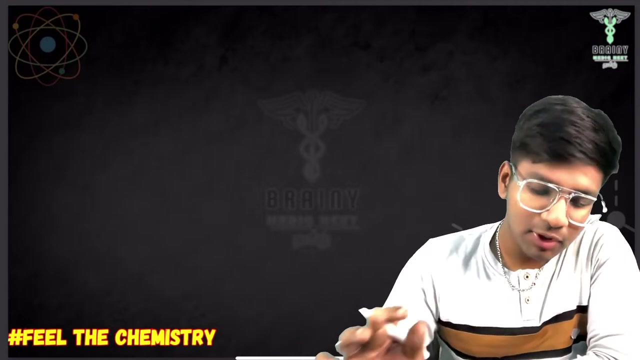 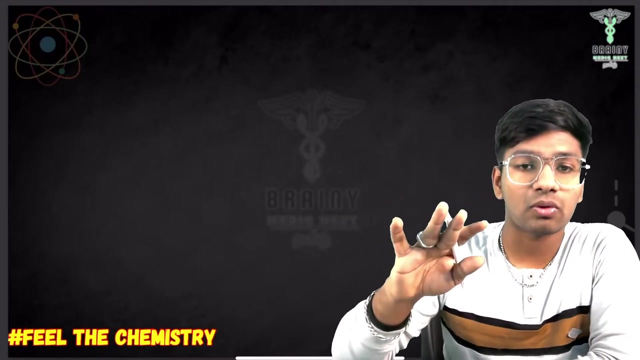 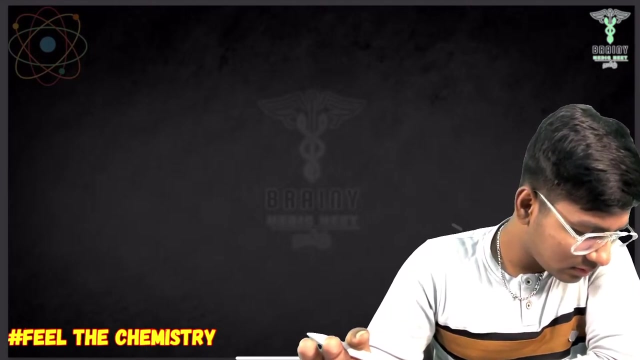 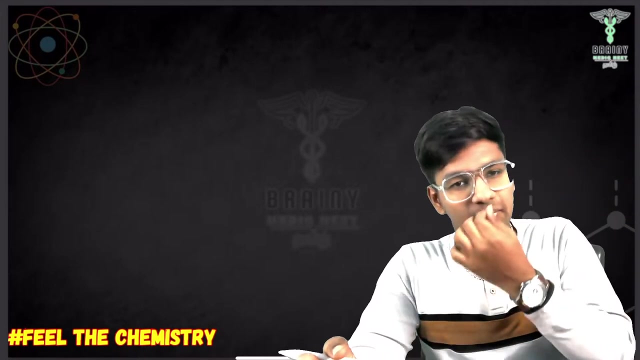 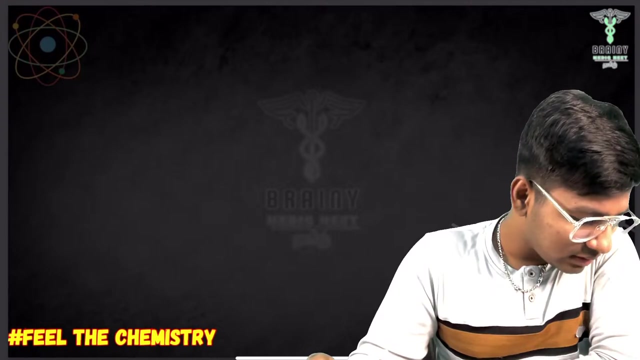 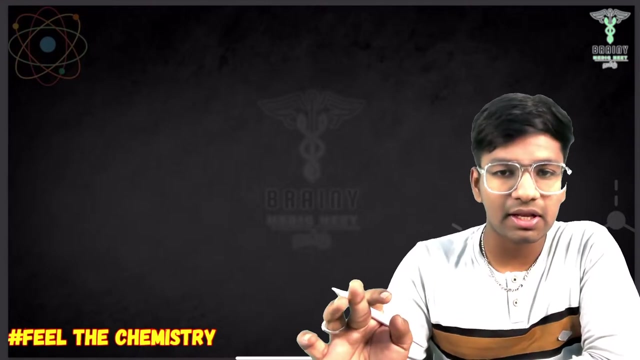 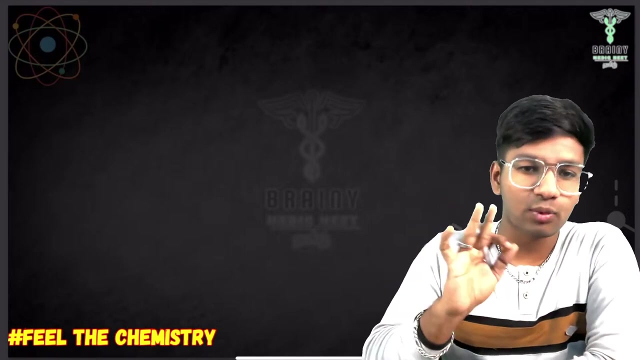 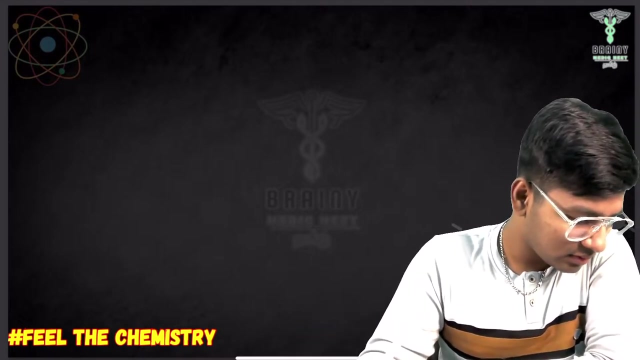 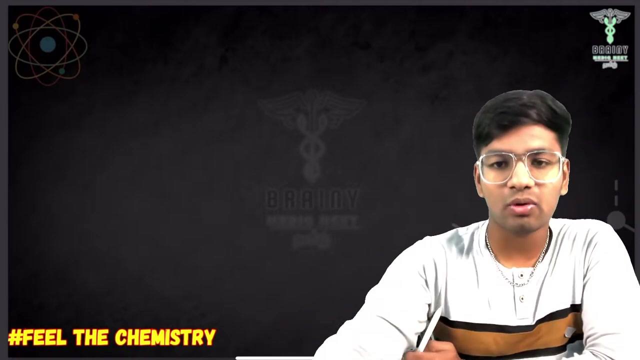 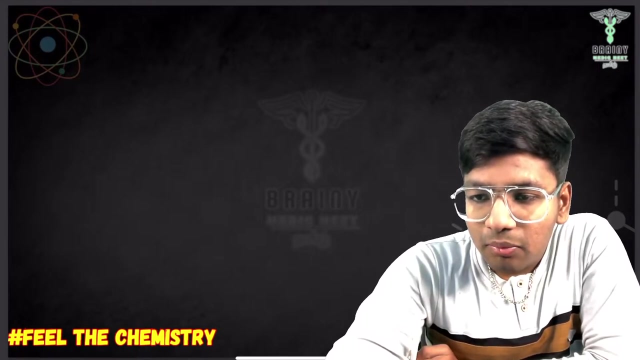 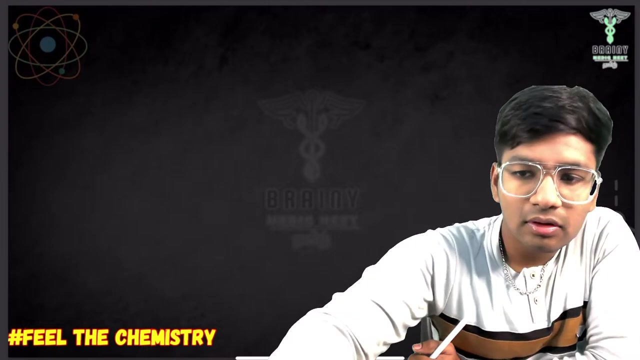 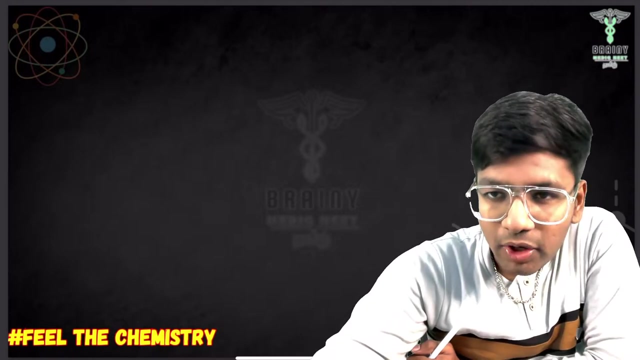 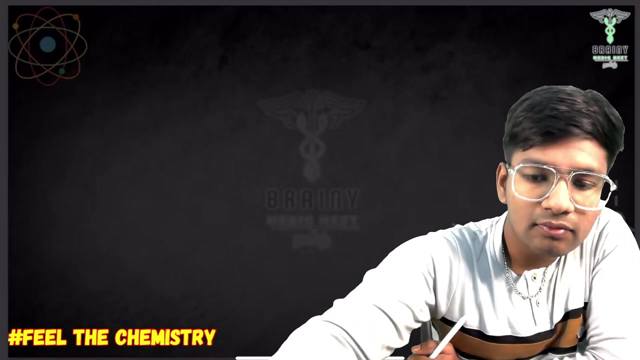 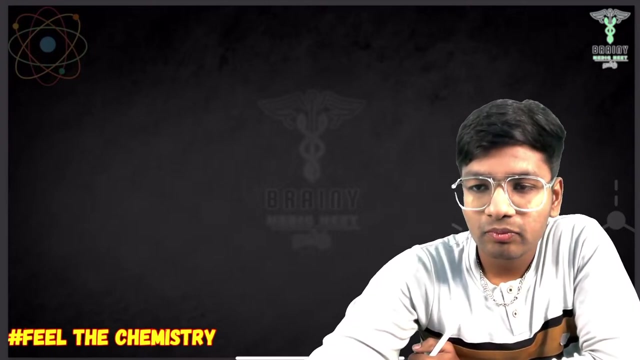 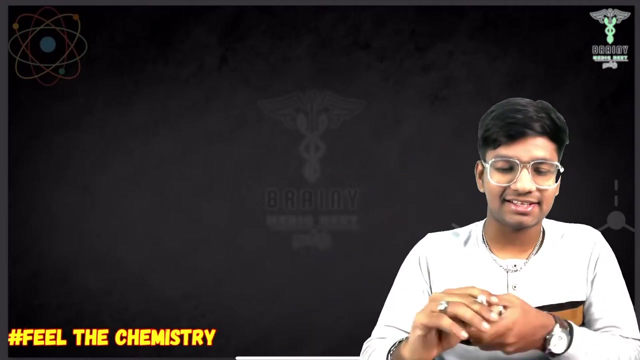 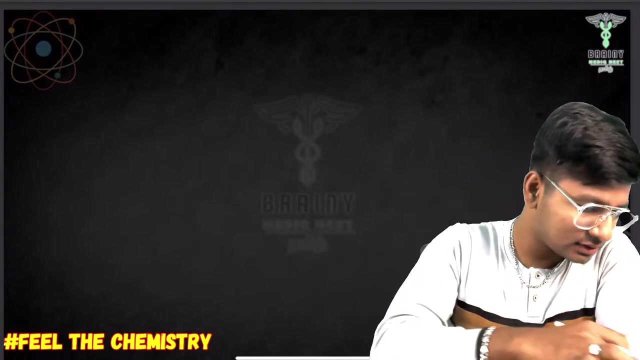 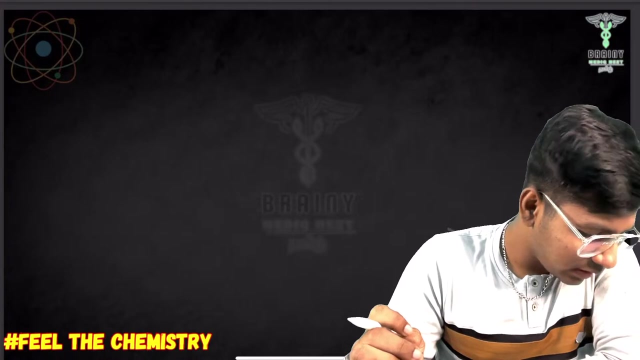 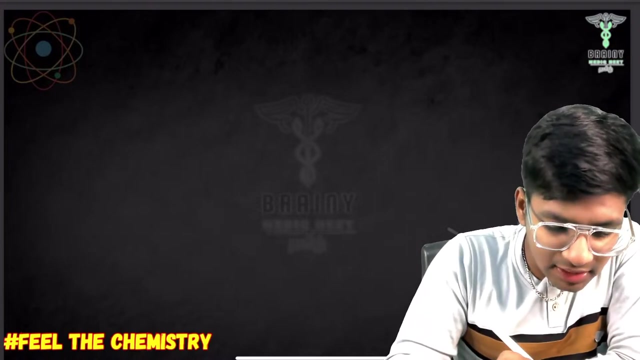 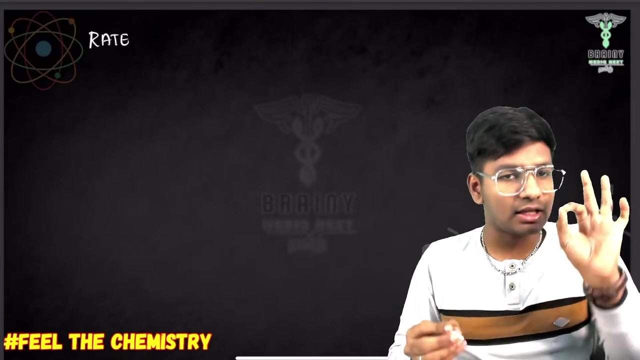 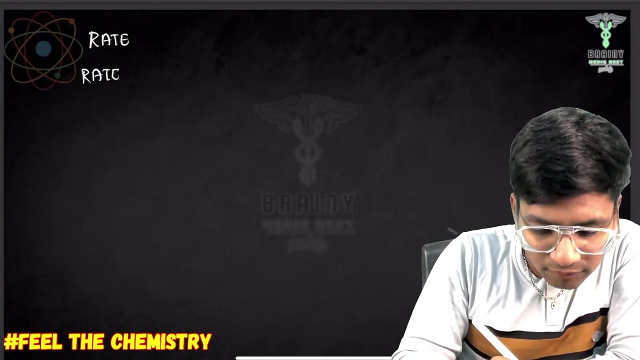 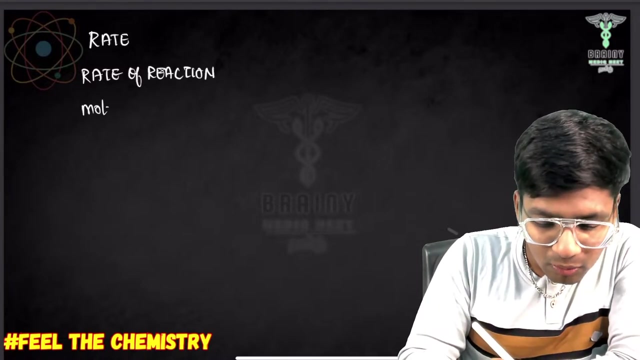 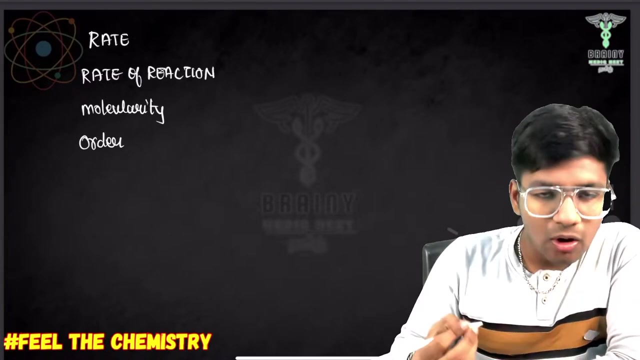 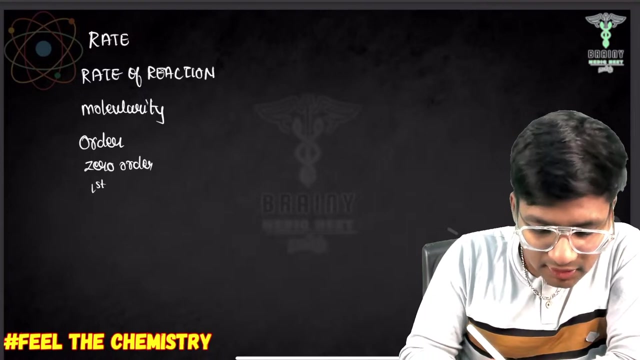 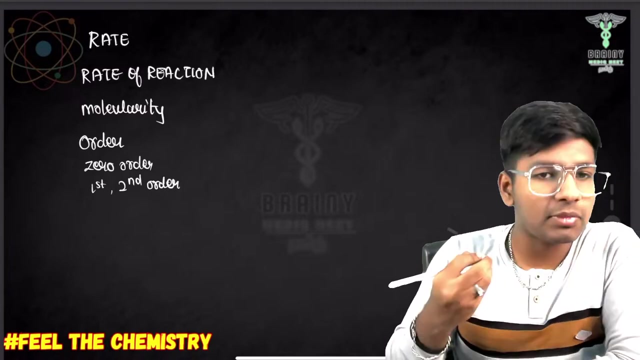 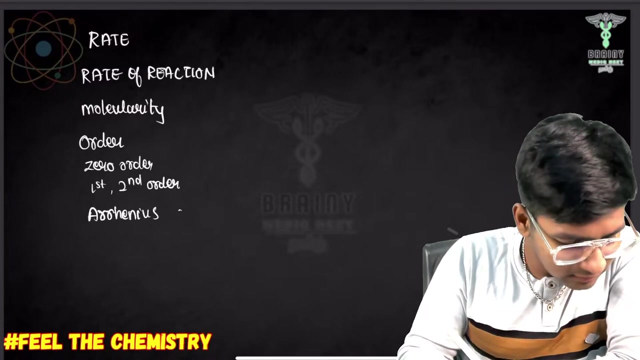 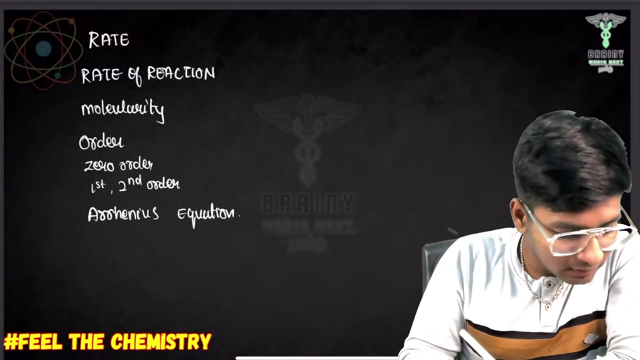 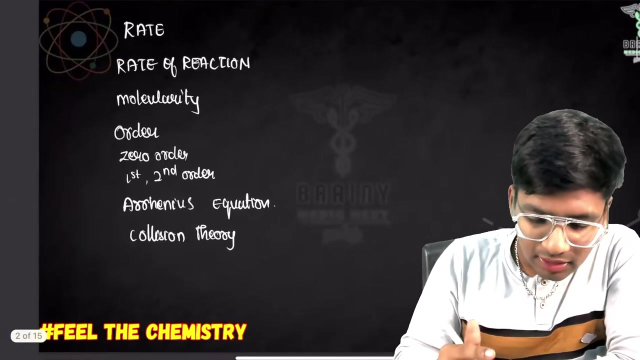 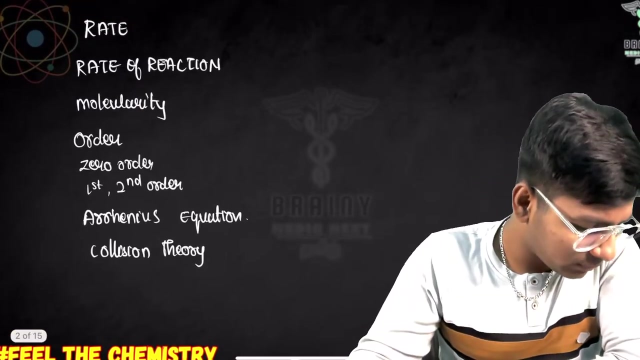 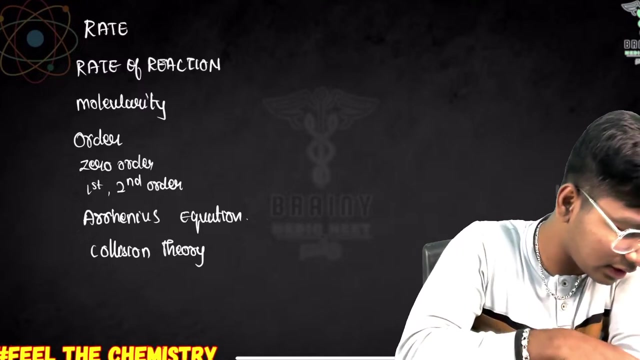 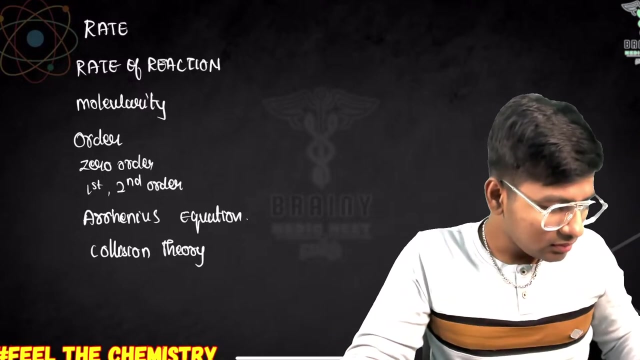 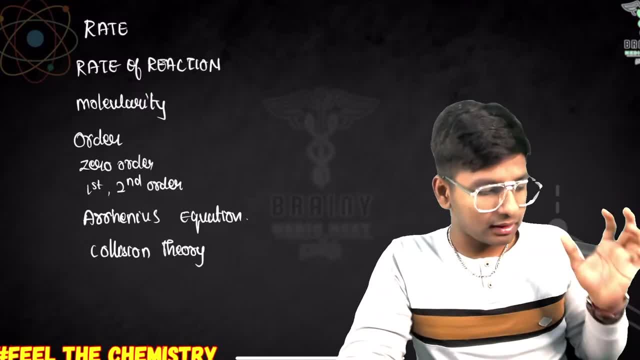 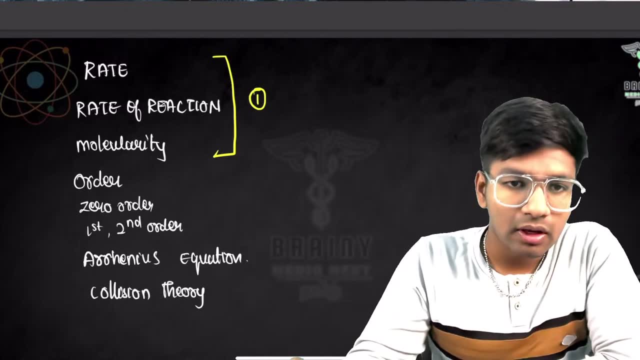 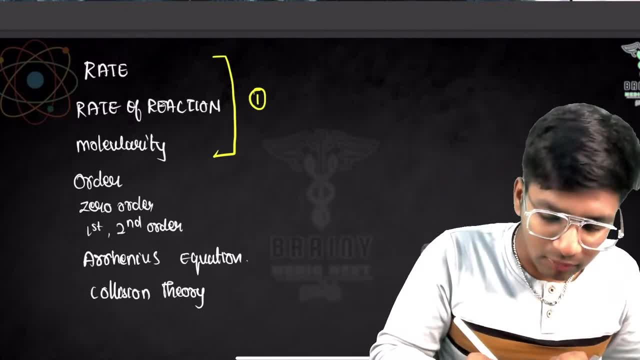 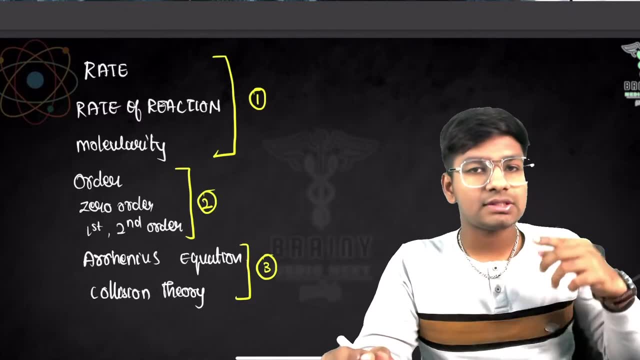 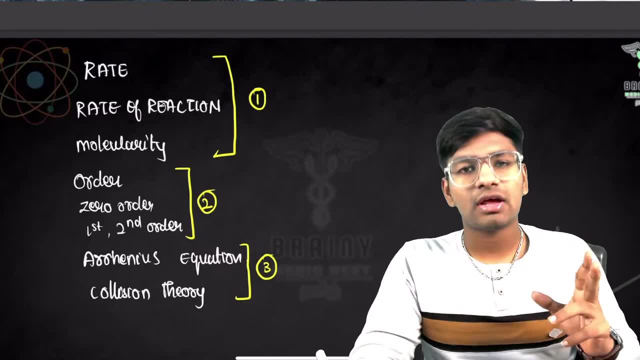 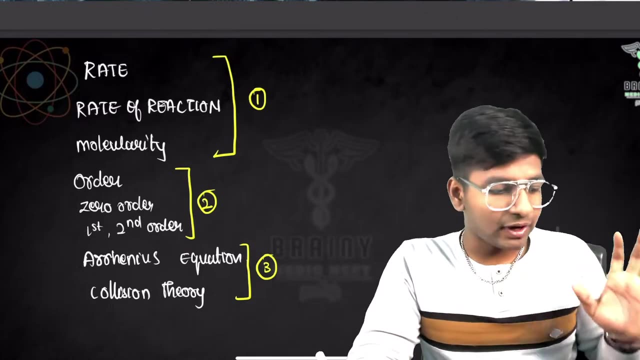 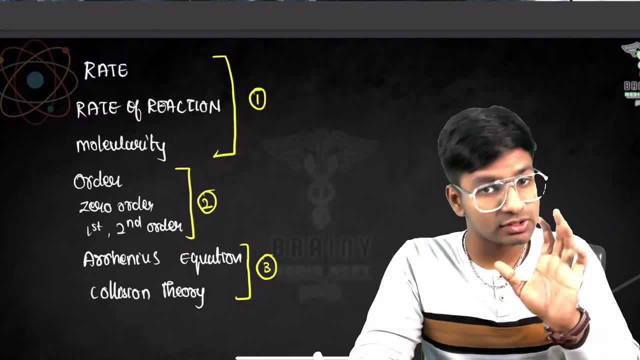 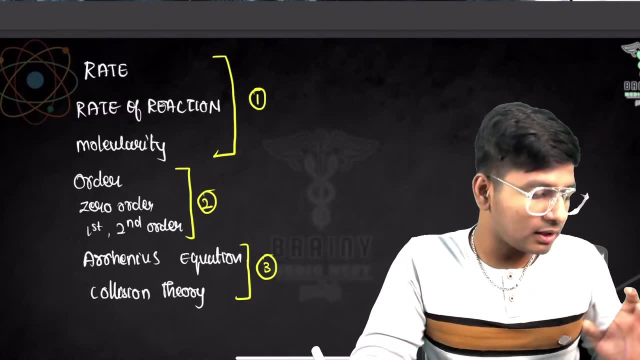 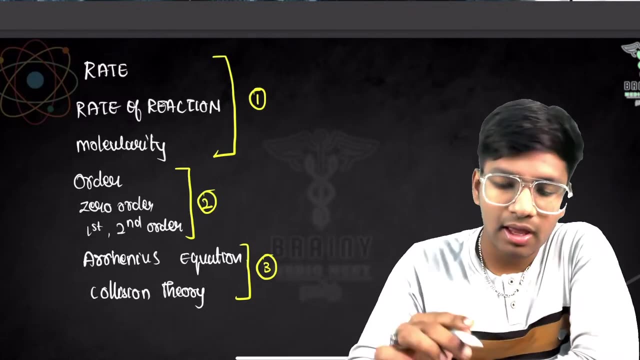 questions are shortage in shortage. 5 to 6 questions to ask in physical chemistry. if you are not a video player, increase the quality. it is in 144p. happy birthday, bro for me. ok. then 6 questions start in shortage. the questions are in the nature of the lessons, that is, thermodynamics. 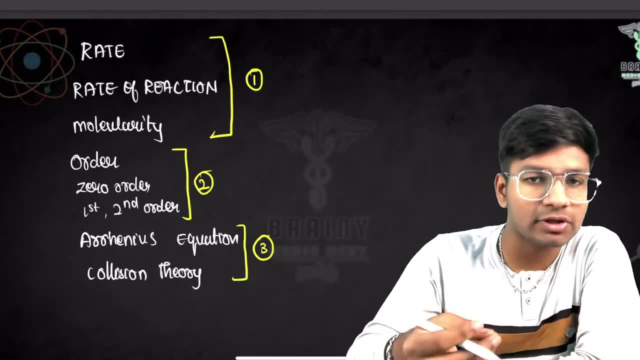 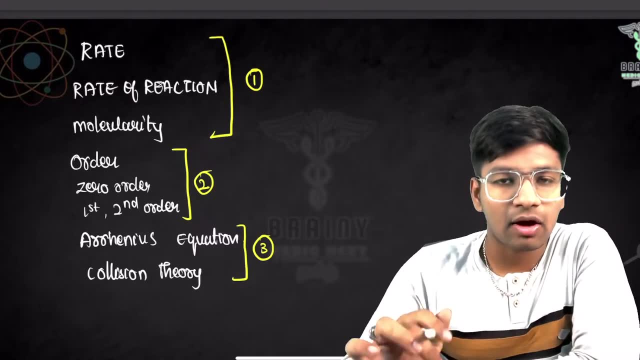 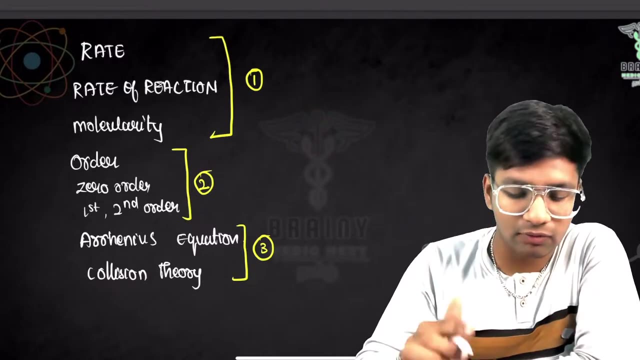 equilibrium. there is a chemical equilibrium, ionic equilibrium, atomic structure in the mother lessons the balance from the one. okay, okay in the mother lessons with our balance from our. so in the lesson there they regular awesome or so in the question, were regular awesome or so in the question. 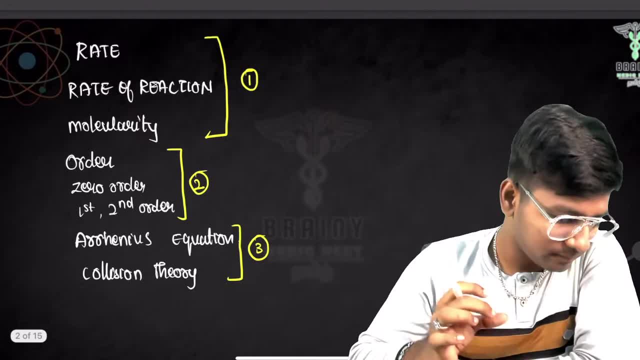 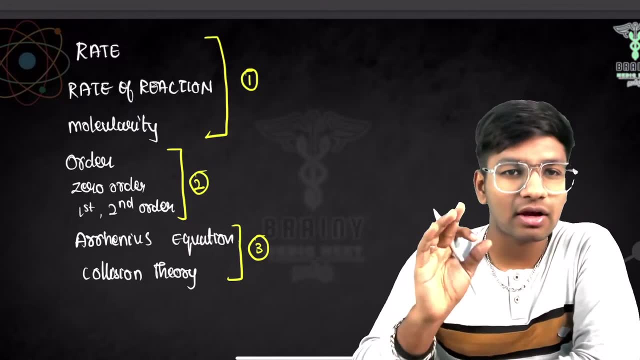 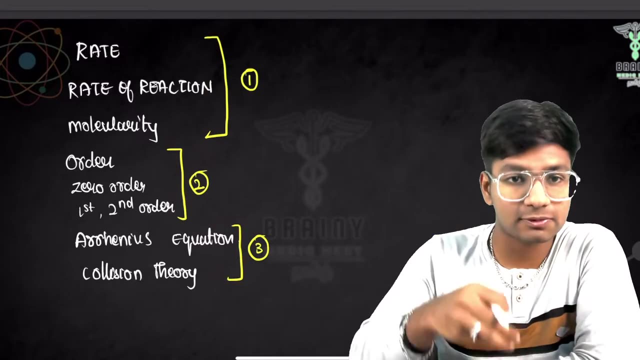 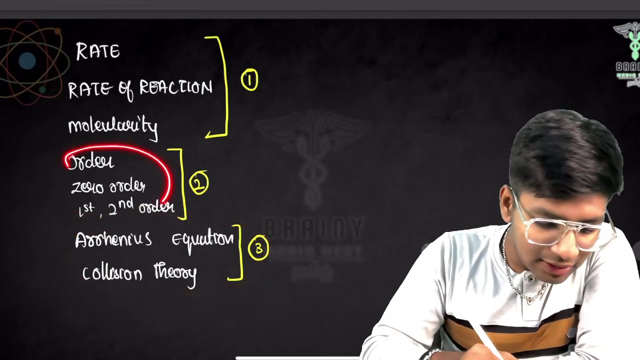 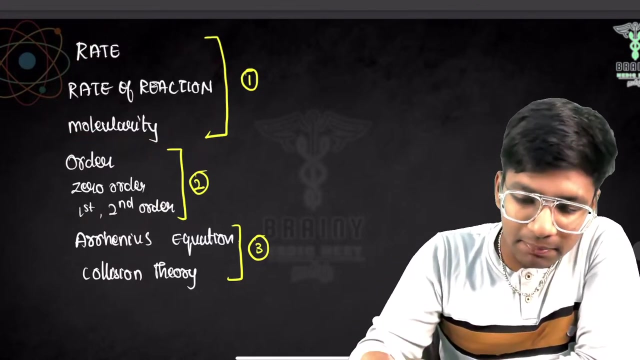 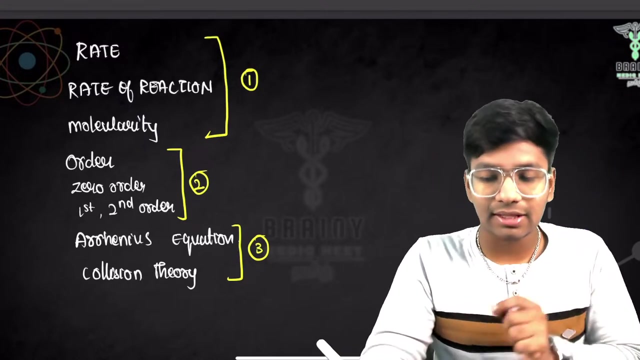 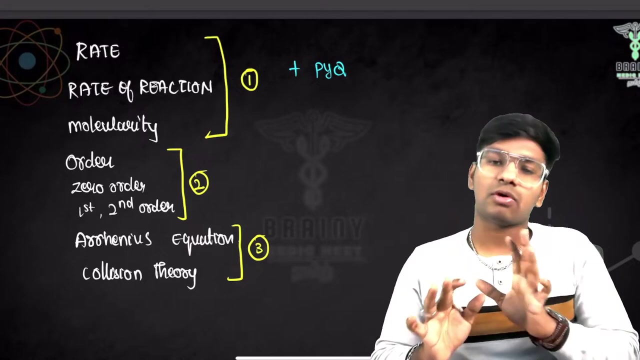 were wrong but in the air, you know question were at the kind of chances are the you know question analysis earlier the lesson I be not at the poor and so theного false you did. you know. see you called we morning also present In this lecture we are going to solve the previous questions and in future we are going to solve the questions. 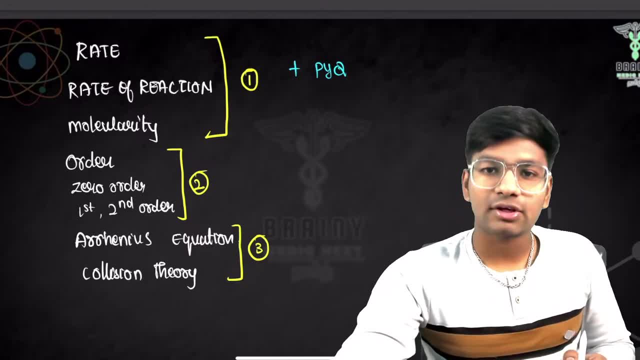 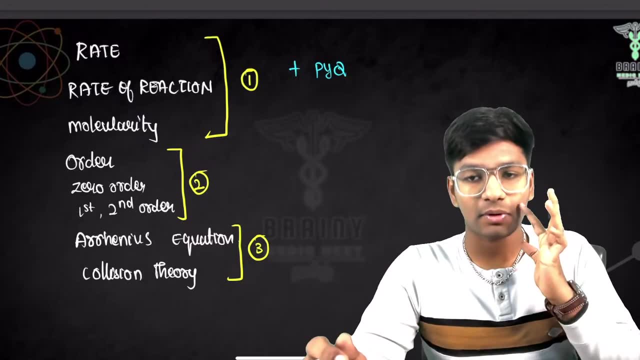 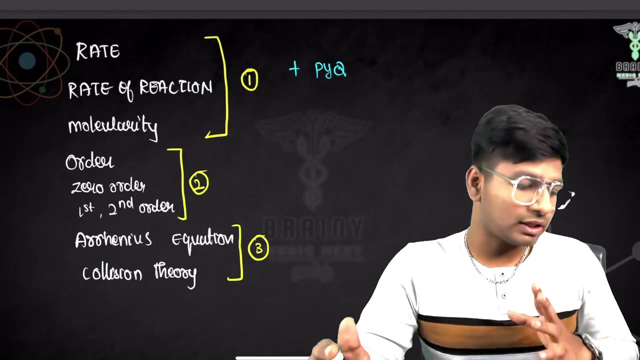 Shall we start? Did you understand what I said? In physical chemistry, there is a very less number of questions. Similarly, in chemical bonding, we are going to start the question series Concepts plus questions. Both will be revised. Ok, I will start a series like this. 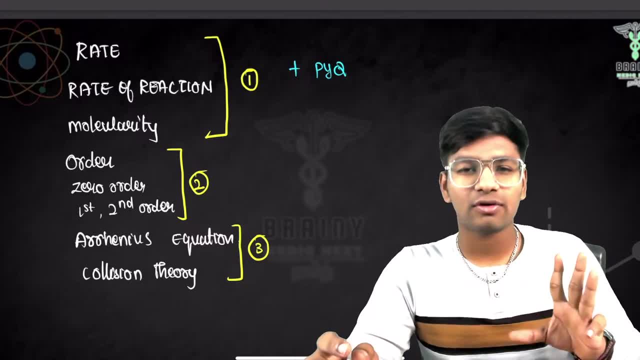 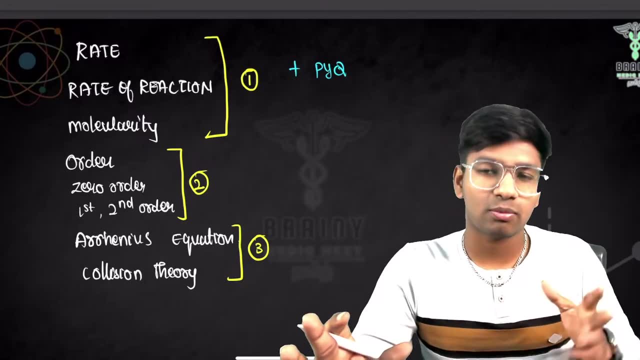 And 450 questions series 3k views are not yet available. We will see If I get 10k views in a week. I have a chance to increase it further In chemistry and biology. I will do what I say. 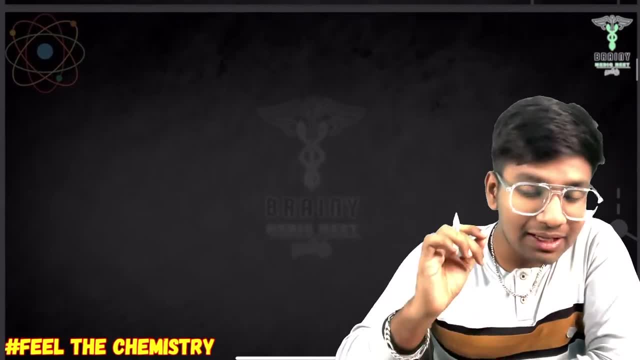 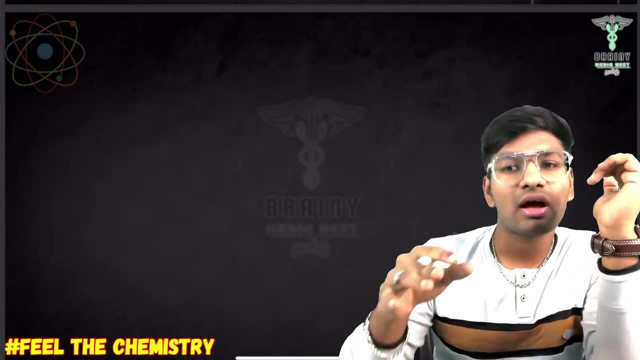 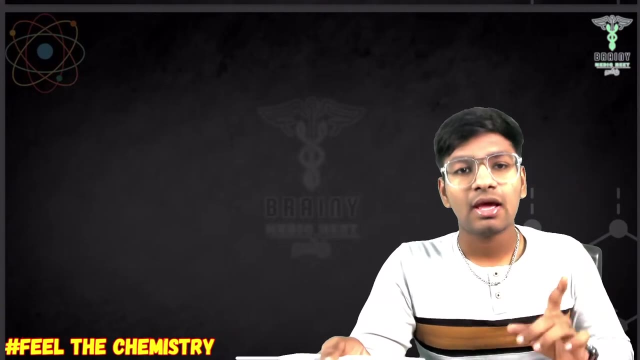 Ok, Fine, No problem. So in the lesson chemical kinetics Look at the word kinetics. Kinetics is a word, Kinetics is something Speed, Speed is kinetics. Ok, What is kinetics? Speed is kinetics. Read about speed. 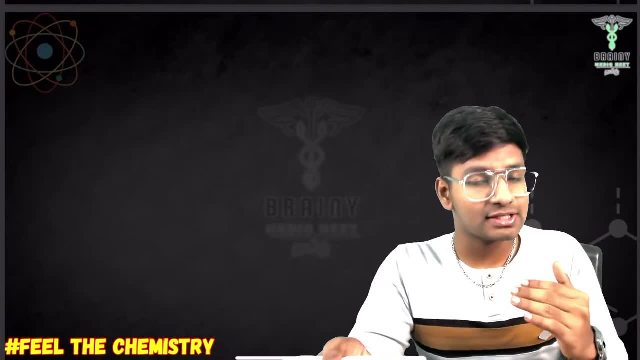 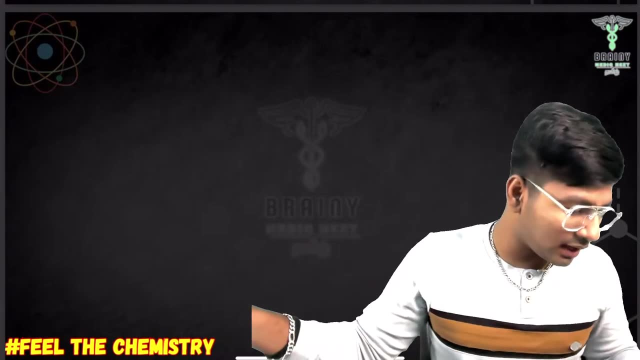 And how does a reaction proceed? A reaction is happening. For example, yesterday is valentine's day. Yesterday, many reactions have happened throughout Chennai. Many of you will be here. Ok, Many of you will be here. You would have done many reactions yesterday. 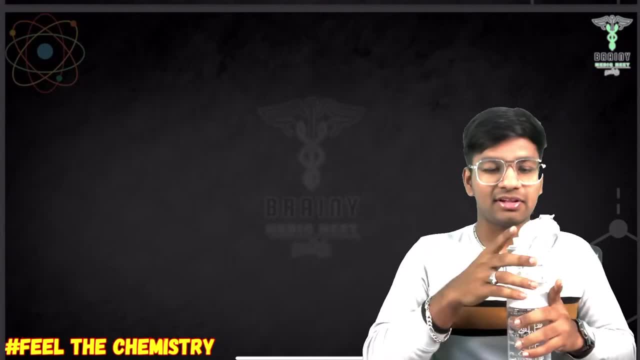 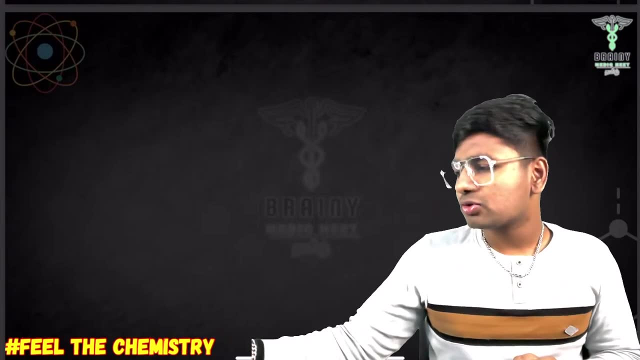 We don't know. If you were good, you would have been good, You would have been good, And you would have been good, You would have been good, Correct? So in this section, how will you measure reaction, How long you both were there? 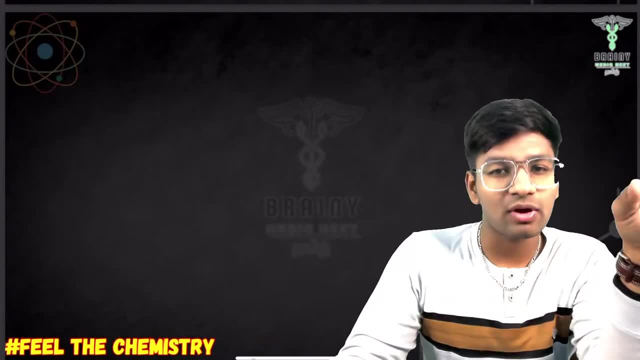 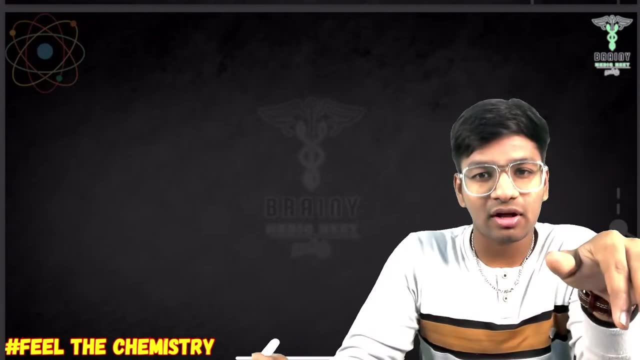 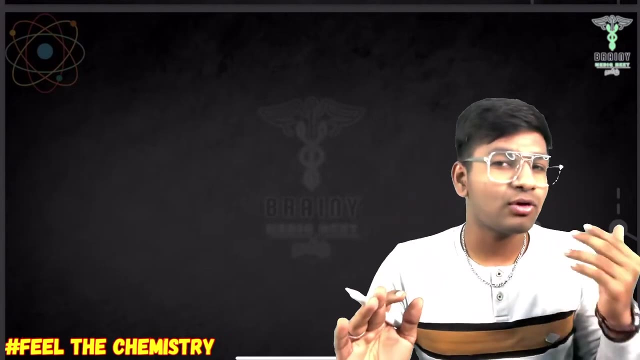 With that we will measure the reaction Correct. What reactions have happened inside? Did he buy Yairi milk or something else? Did he give the greeting card or something else? Ok, Number of giving number of taking divided by how much time he was there and how much time he was not there. 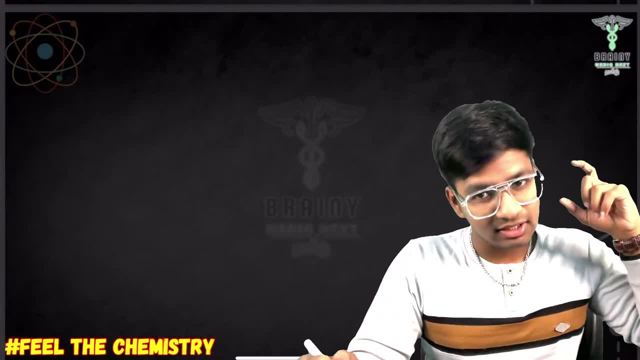 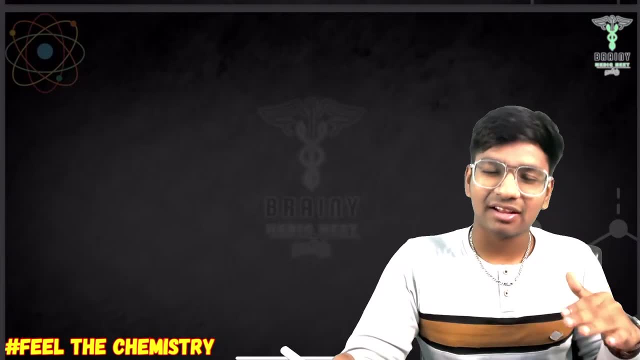 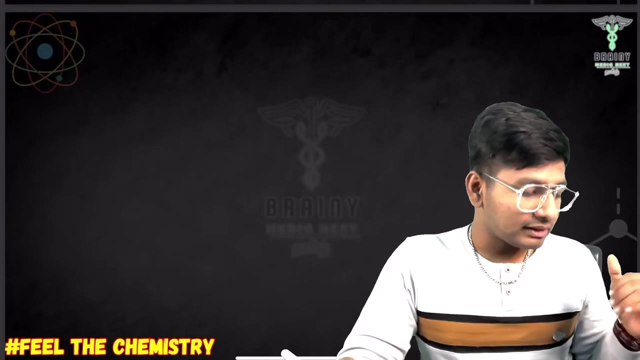 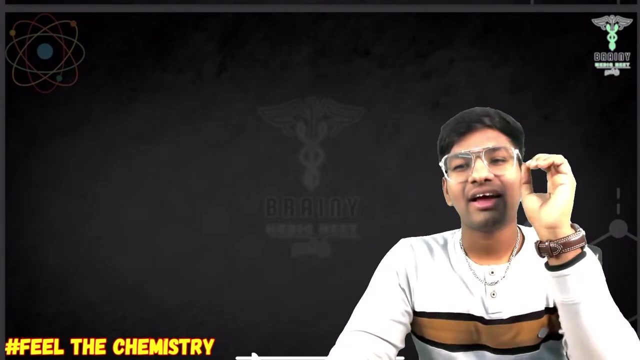 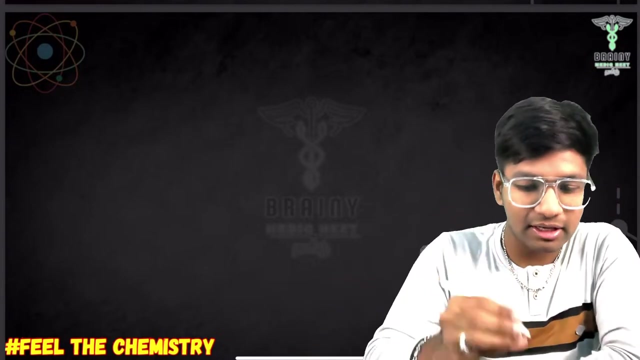 this is the reaction. if it was a fast reaction, if it was a slow reaction, if it was a strong person, he would have reacted fast. similarly, you are also in the same plane. if it was a slow, fast or moderate reaction, it would have proceeded. we are going to study types of reactions. 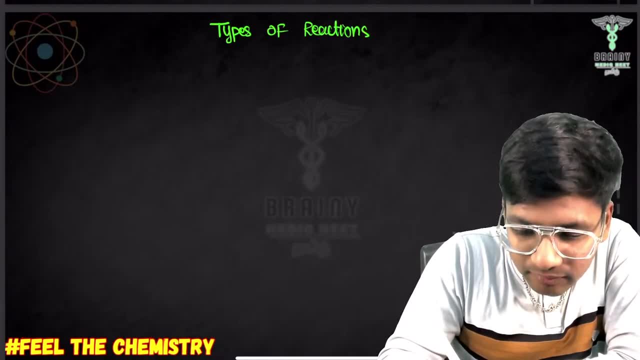 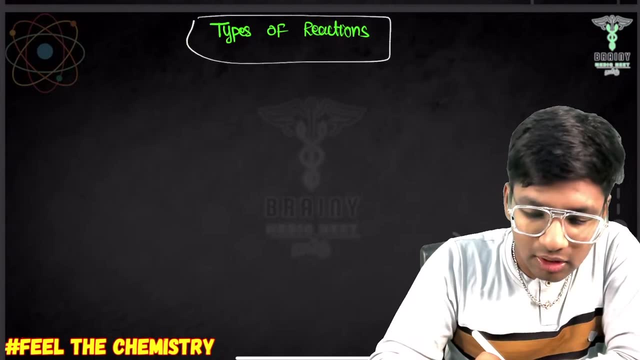 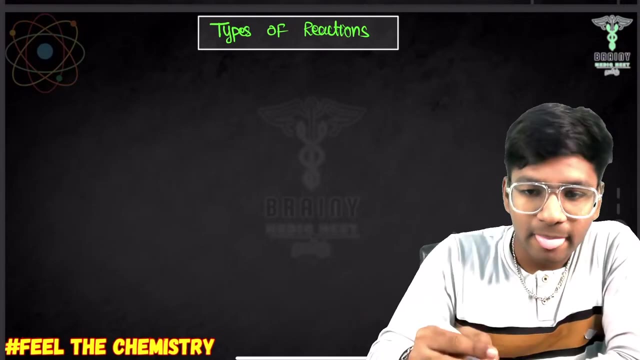 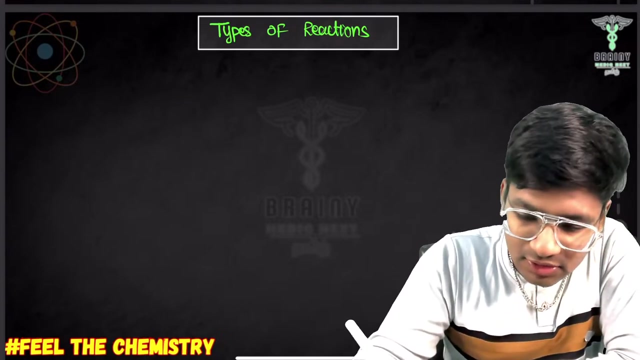 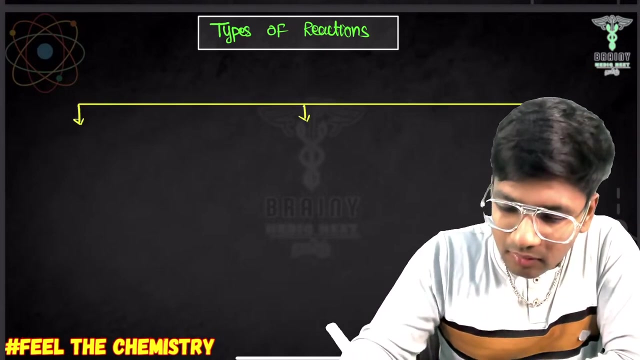 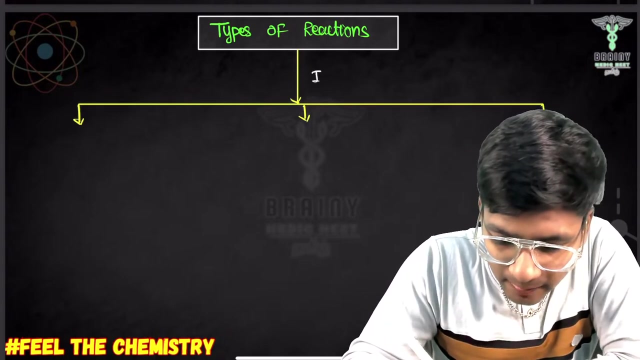 types of reactions. I think I have given a good example. you should not forget it. there are 3 types of reactions. there are 3 types of reactions which are based on. we have 3 types of reactions over here, based on the rate of the reaction in the basis of: 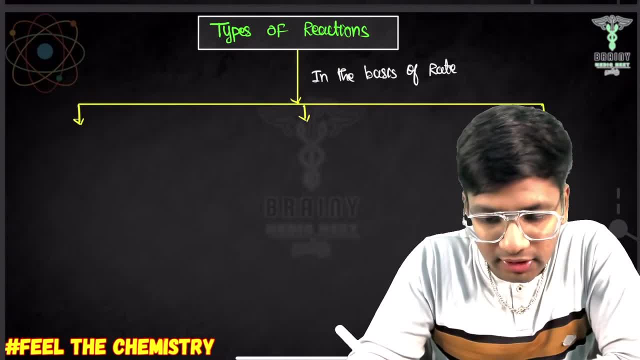 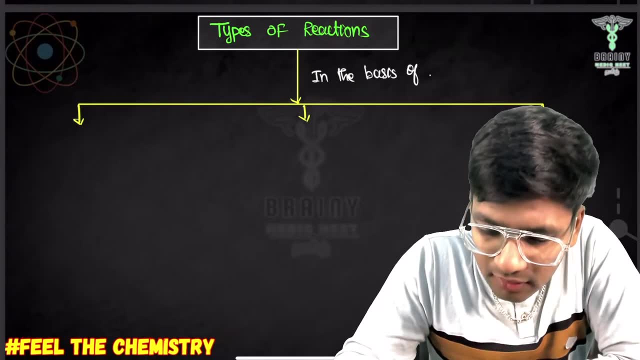 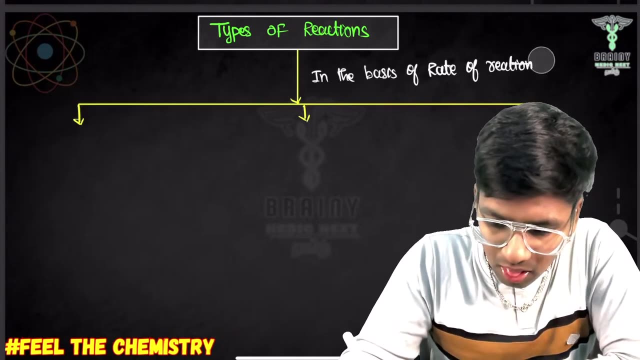 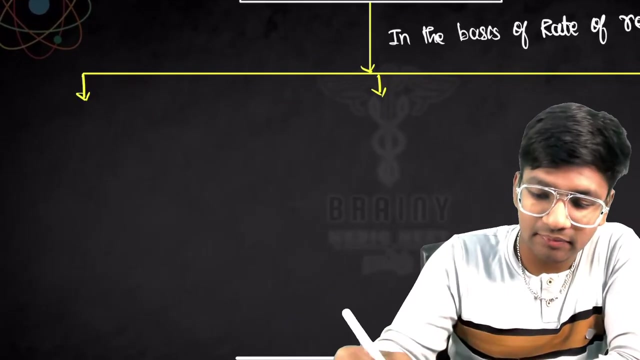 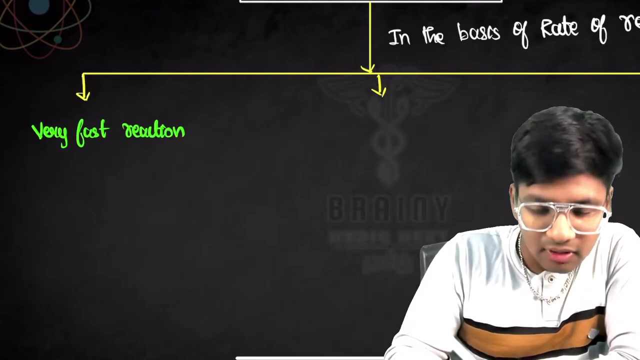 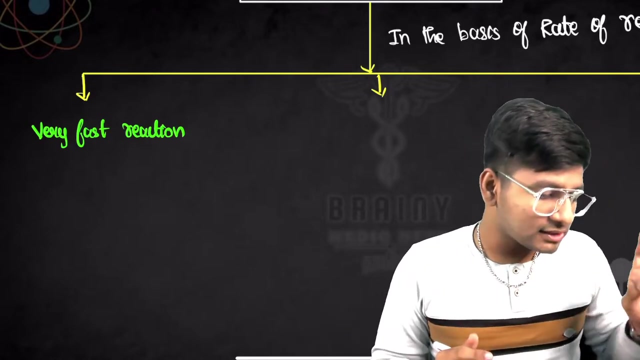 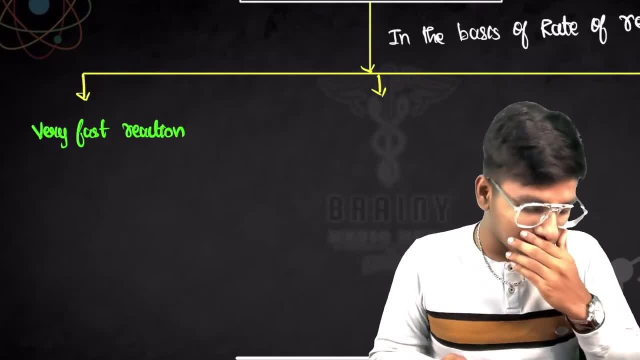 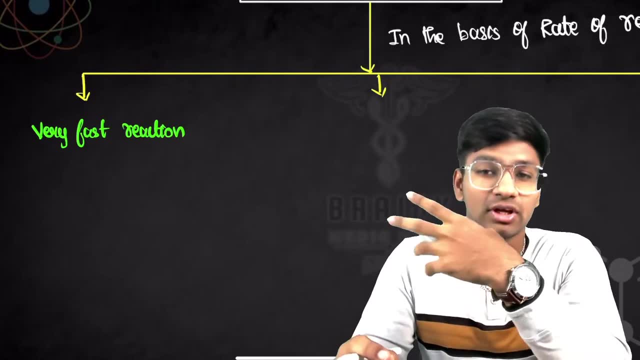 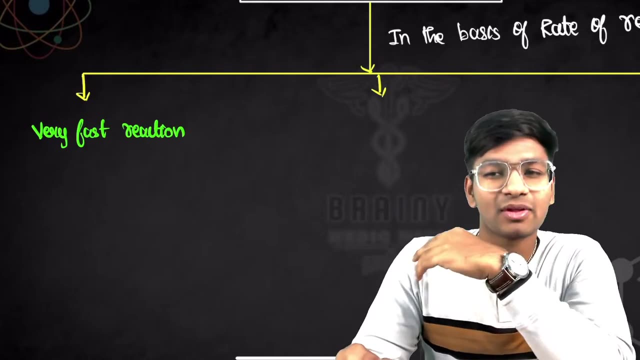 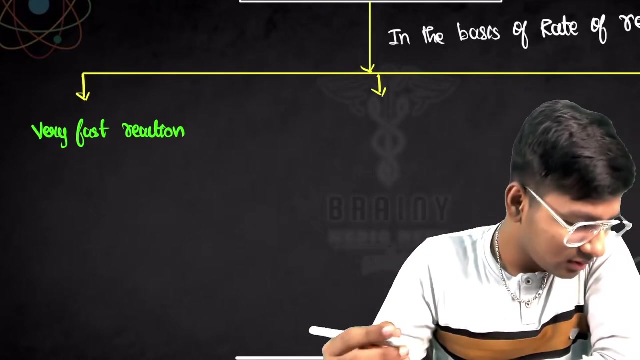 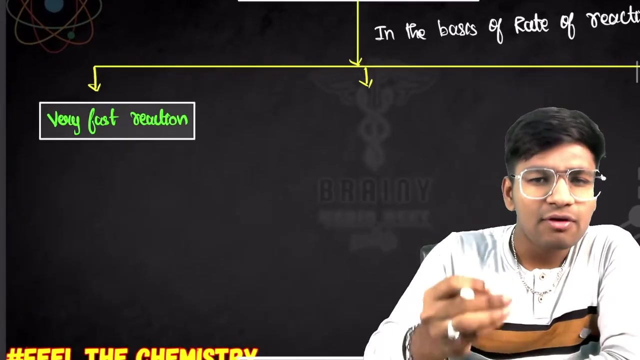 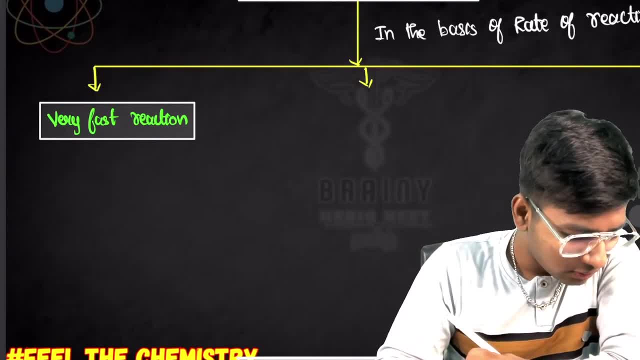 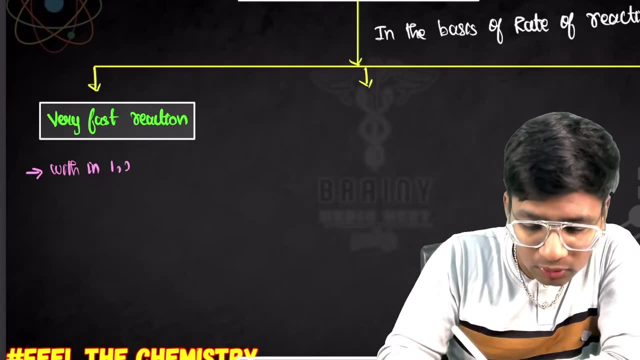 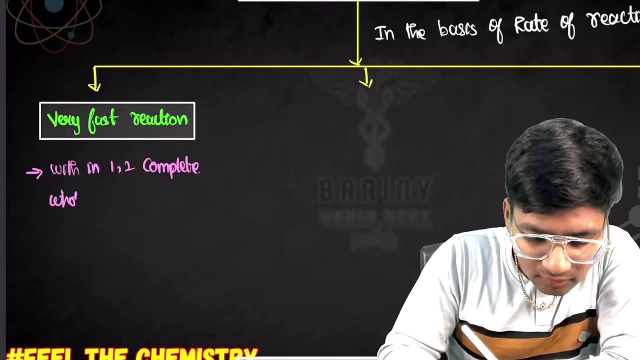 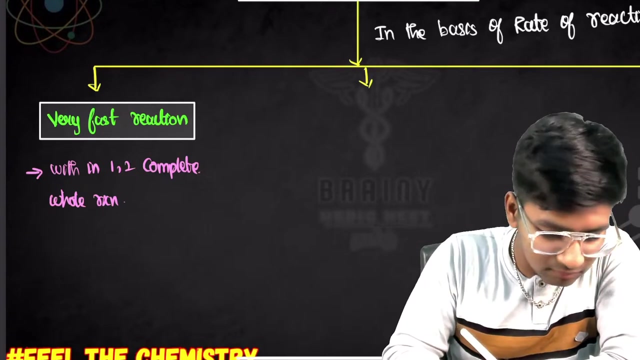 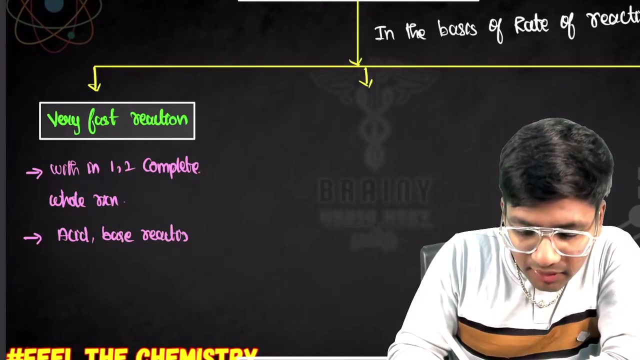 the whole reaction will end: waste of yellow. ok, within within 1 to 2 seconds. 1 to 2 seconds. the whole reaction will end. complete whole reaction. ok, most of the reactions- acid based reactions- will be like this: acid based, acid based, acid based reactions will be like this: 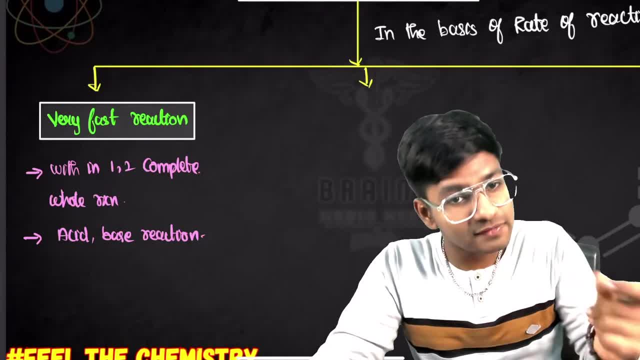 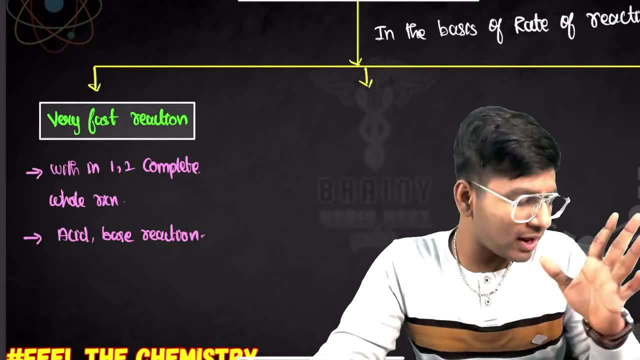 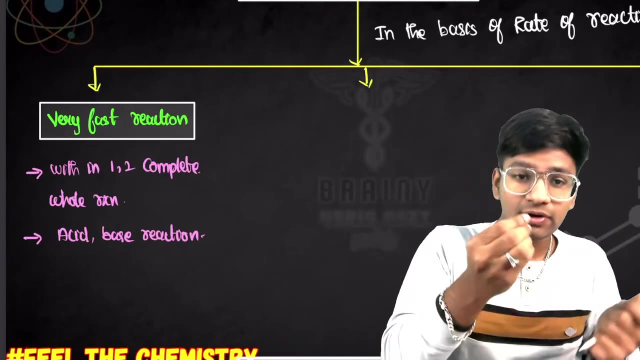 now, what i am asking is in fraction of seconds. in fraction of seconds, the whole reaction will end in fraction of seconds, in fraction of seconds. if the whole reaction will end, is it possible to measure in fraction of seconds? can we measure in a part? is it possible to measure? 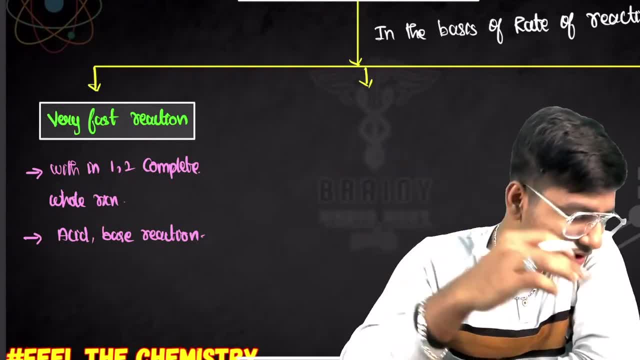 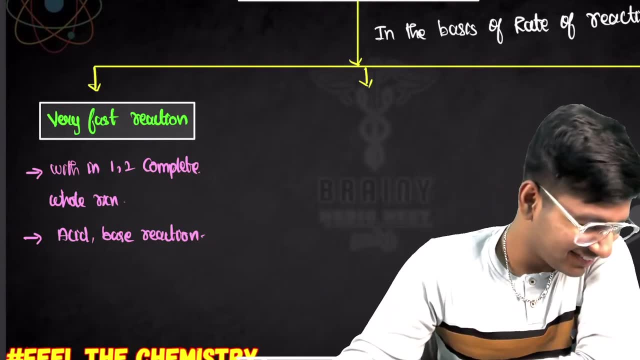 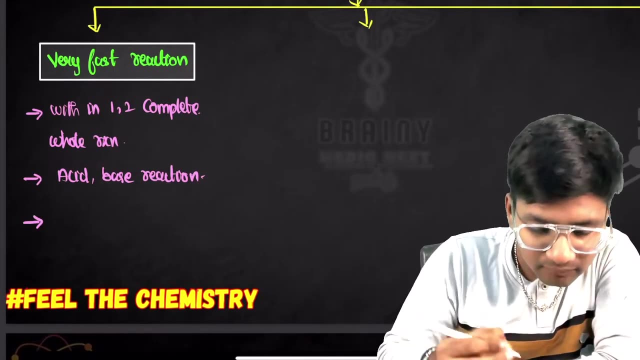 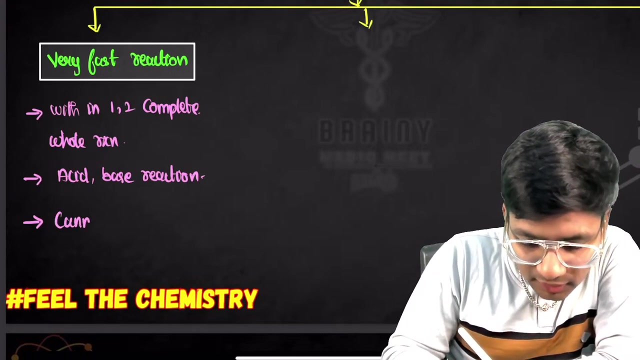 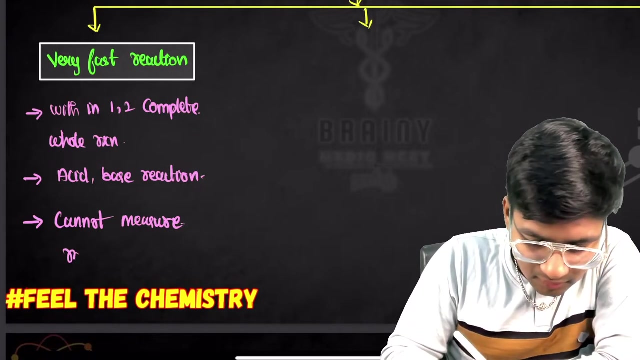 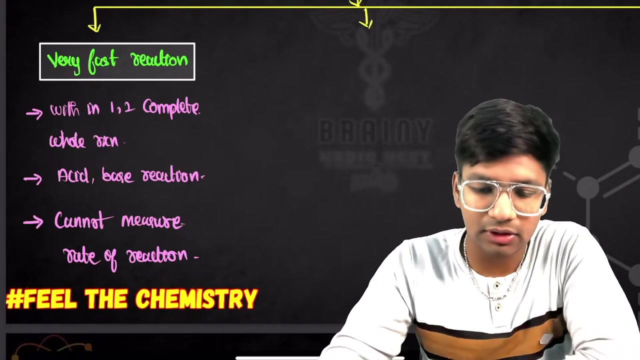 is it possible to measure, because rate of reaction is the measure of the reaction. cold since chocolate day because of more chocolate received- i don't know anyone chocolate, So you cant measure this type of reaction. you cannot measure rate of reaction. rate of reaction, you cannot measure the rate of reaction. 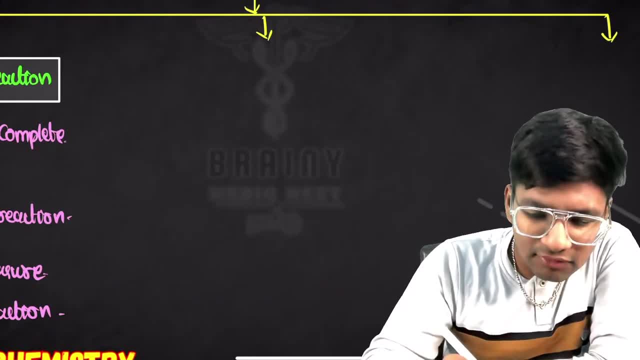 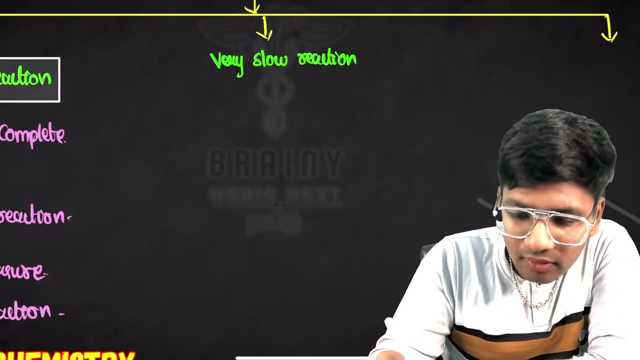 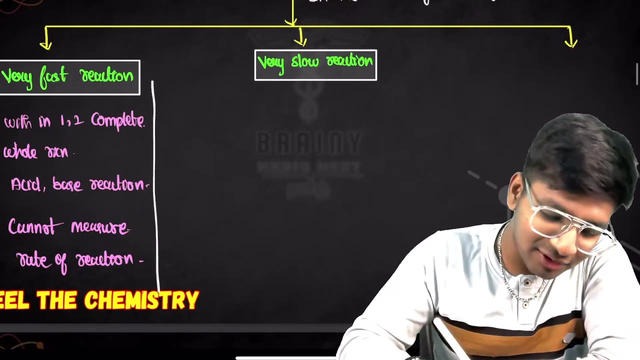 second very slow reaction in a day: very, very, very slow, very slow reaction. okay, very slow. I'm a start from now. on the fire, on the mood, upon a Thalia. they would either come on, drop or on the phone. on the solitaire day we tend to really come around so long okay. 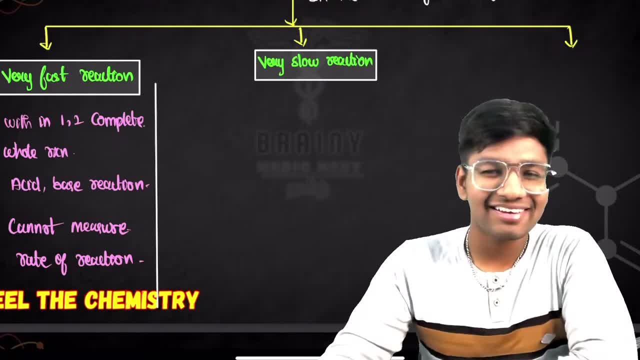 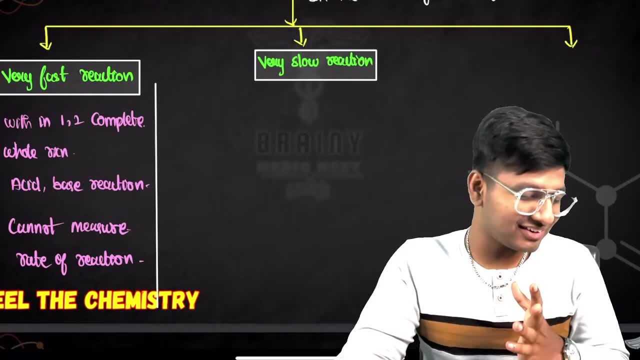 hey, I don't know why don't the camera be fun? Rai Widiwa, they would run a chocolate line under the camera. if you ponder a party pandanum in police alone- I know a lot of it a bit earlier- then you're part of a single meaning. 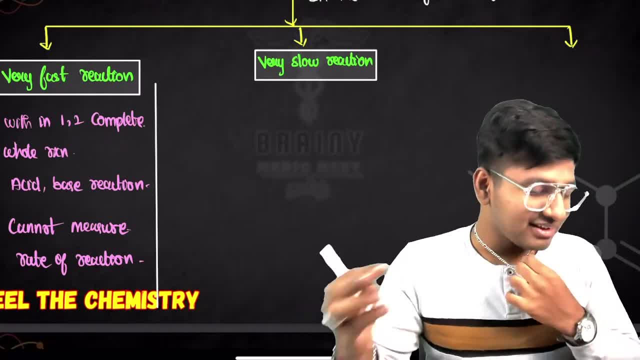 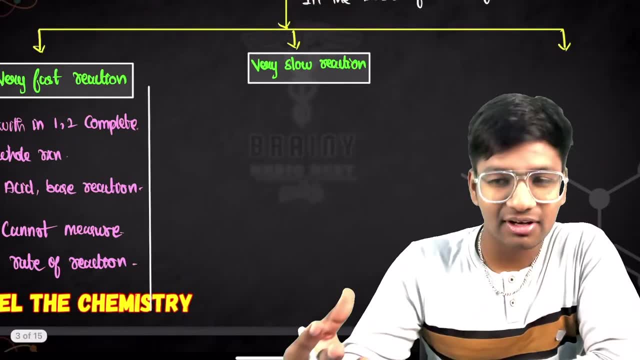 opposite of a game in the city, given three other. okay, what? yeah, any city. can you agree it? chocolate, are they not sitting? okay, so see how we're not. so long. you are part of a new vehicle and under our poor owner you are a very mistaken one. the TV to get a piece of diesel, you don't? 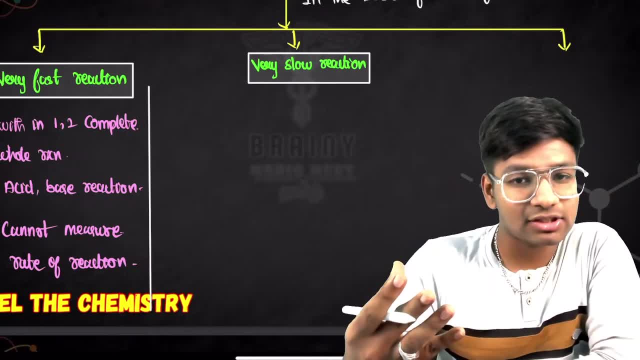 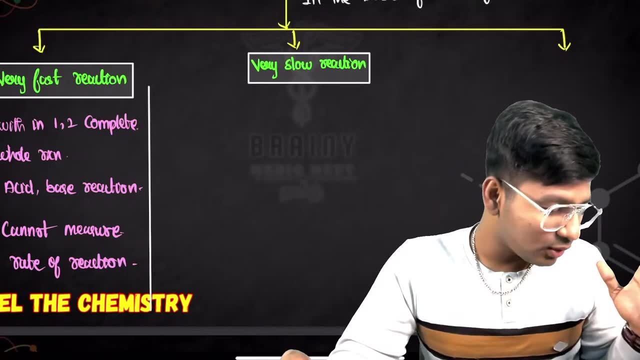 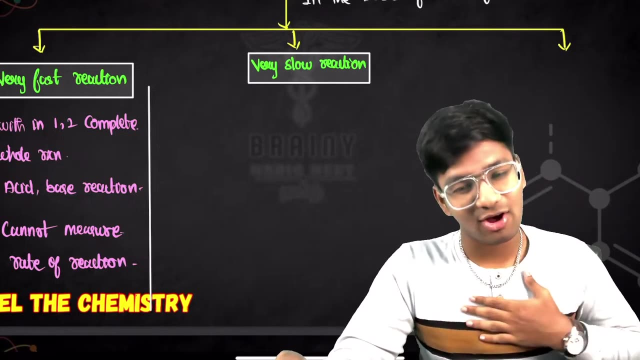 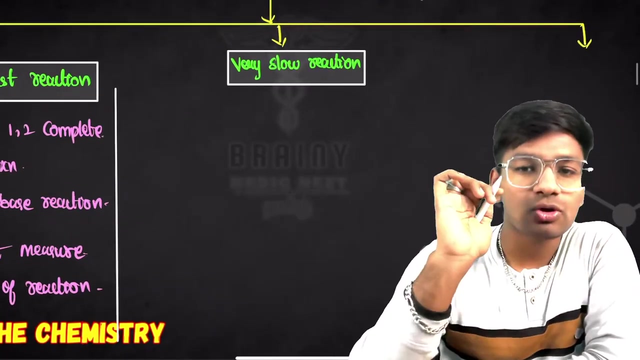 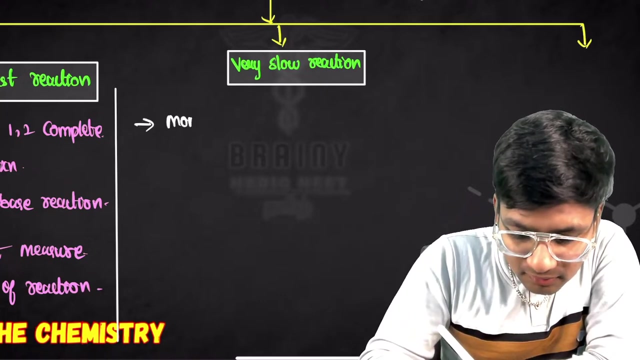 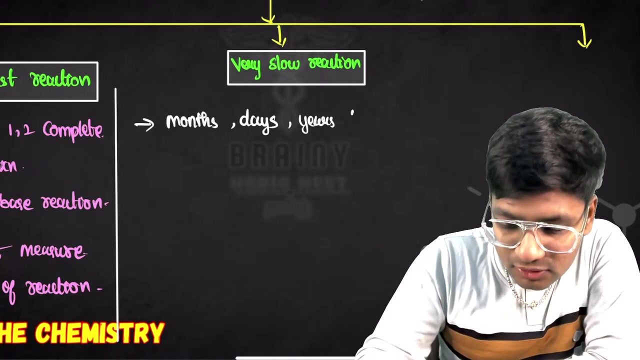 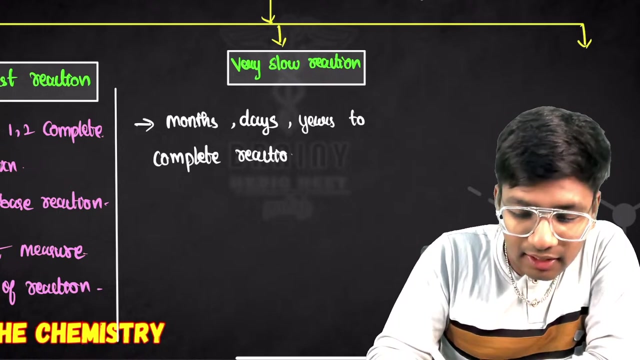 understand. okay, Wow, okay, okay. so very slow reaction in the reaction: months days, years sometimes, okay, sometimes months days. i'm a medical, so it's not a problem. so months days or years to complete months. months days or sometimes years, years to complete complete reaction. now I'm asking you a reaction. you don't know when it will end. you don't know when it will end. 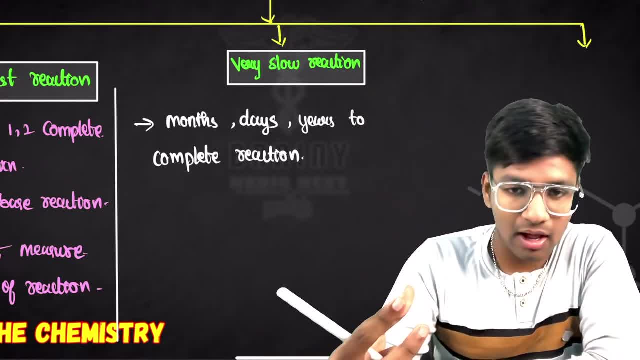 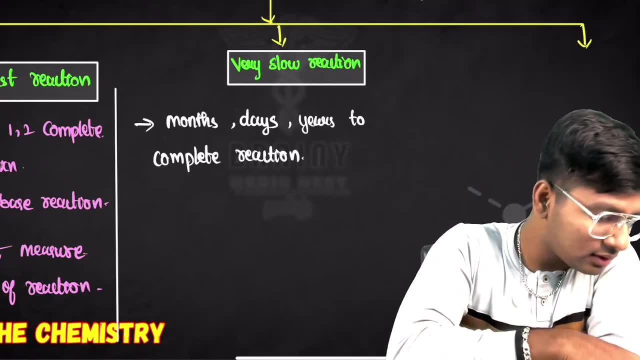 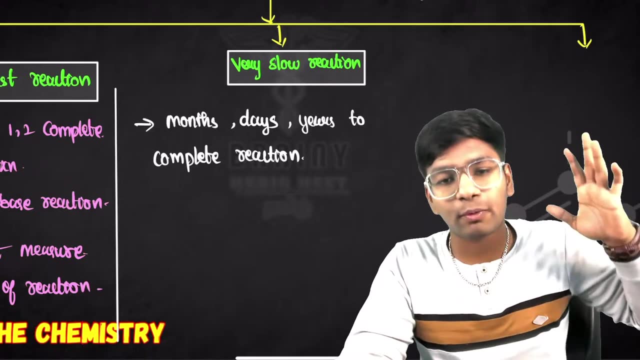 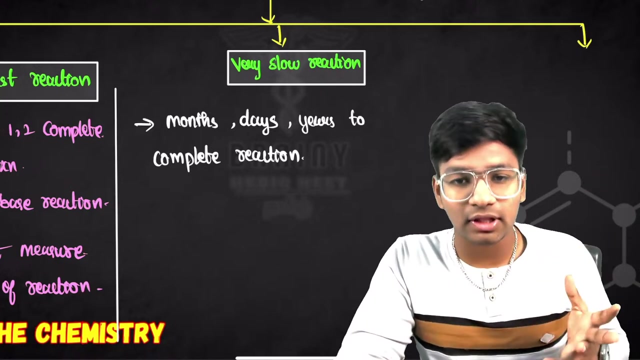 if you don't know the interval of time, you don't know the reaction that is, can you measure the rate? you don't know the time gaps, you don't know the time gap, the time that the reaction is going towards. you don't know if it will end it. we don't know if it will go to the end. 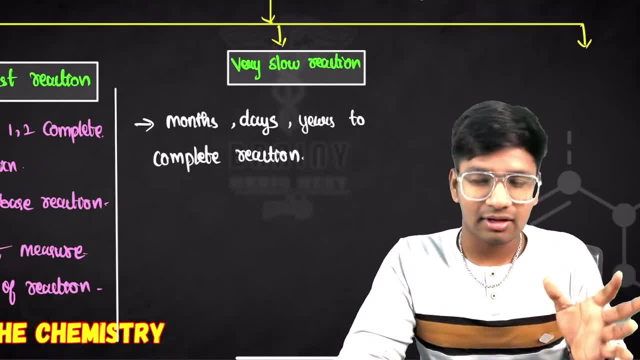 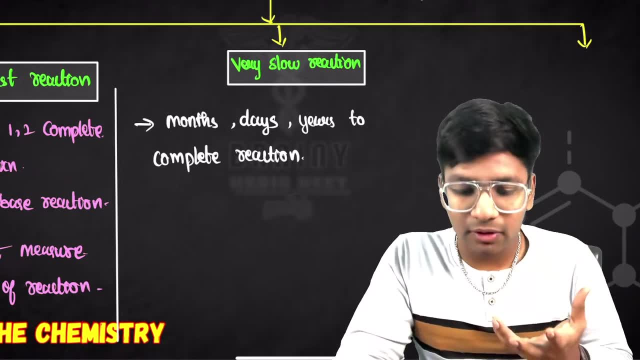 but you wait for months, days, years. first of all, many of you will wait for it, my true love. I don't need it, but this time, what I'm asking, can we measure it? No, we can't Correct, So we can't measure this either. 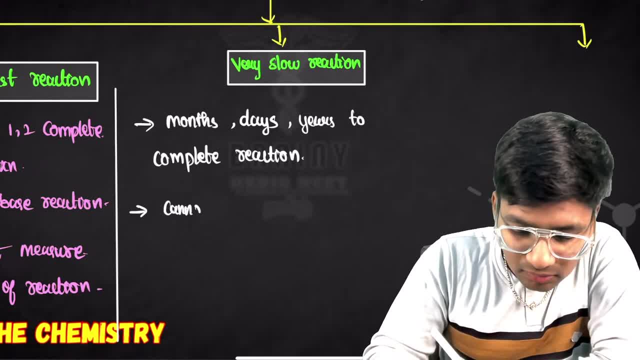 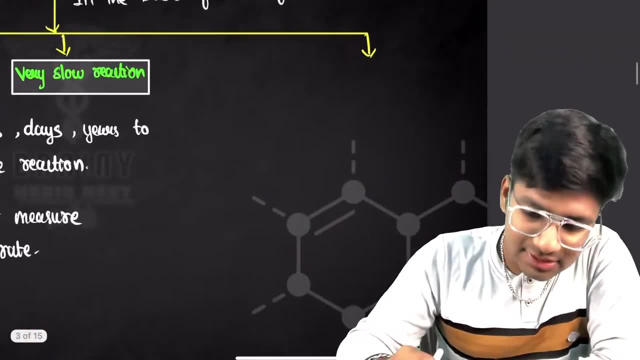 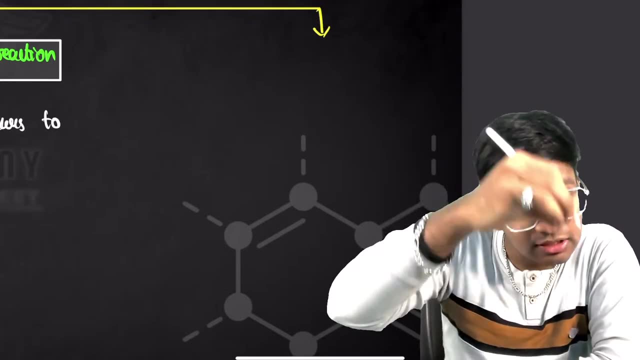 Does not measure, We cannot measure, Cannot measure, rate. Okay, our last reaction is slow or moderate. This is very slow and this is slow. Sorry, this is very slow and this is very fast and this is slow. There is a difference between both Slow or moderate. 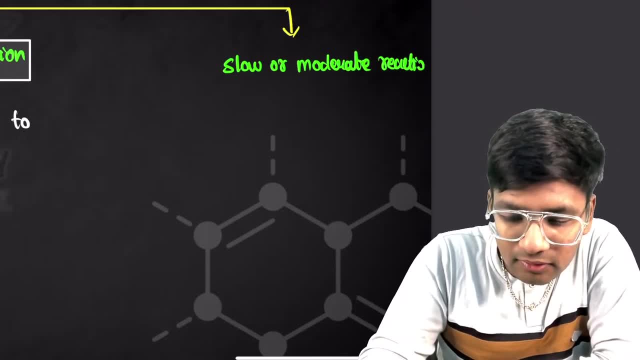 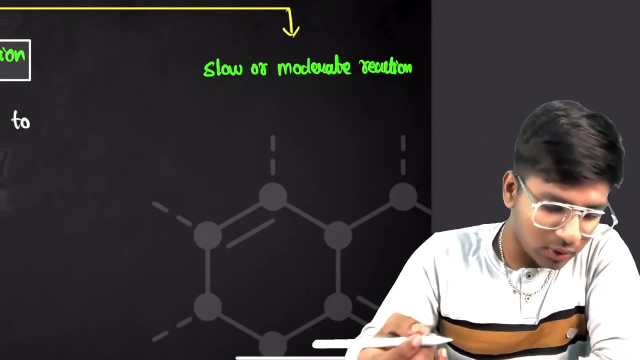 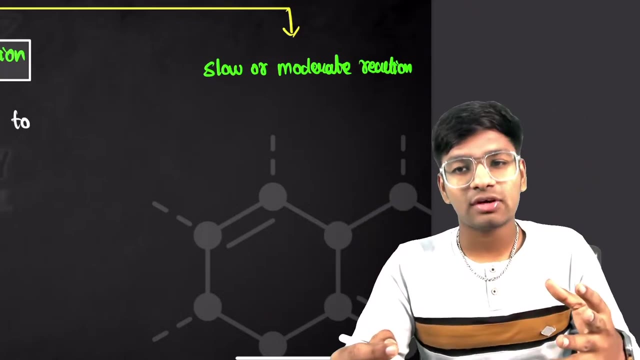 Moderate reaction. Okay, They would have already made a plan. This should be done and that should not be done. This should be done and that should not be done. If there is a short circuit in between, you cannot bring it here In this example. Let there be a short circuit or catalyst. 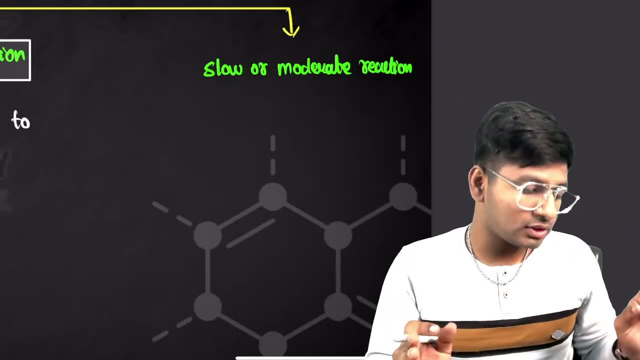 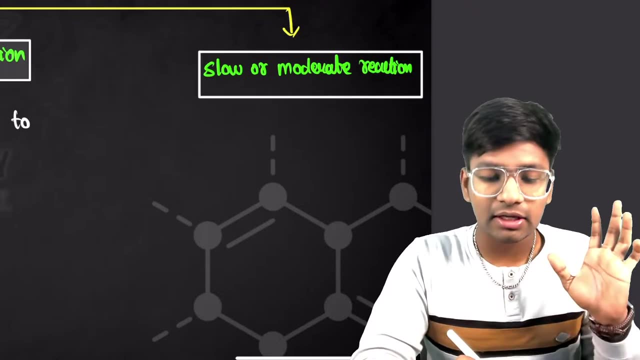 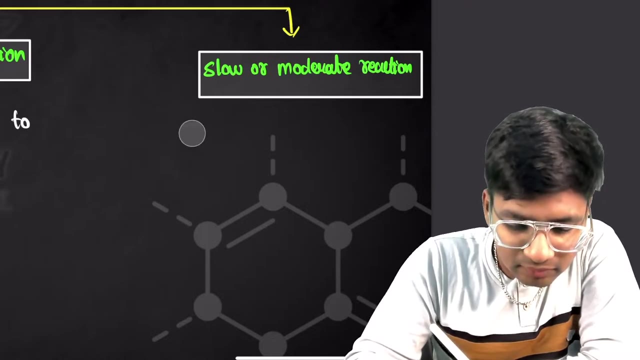 But there will be a plan already. Okay, The reaction will be like this and this will be like this. Okay, I don't know if there will be a short circuit or not, But this will be completed in minutes. This is within minutes and hours. 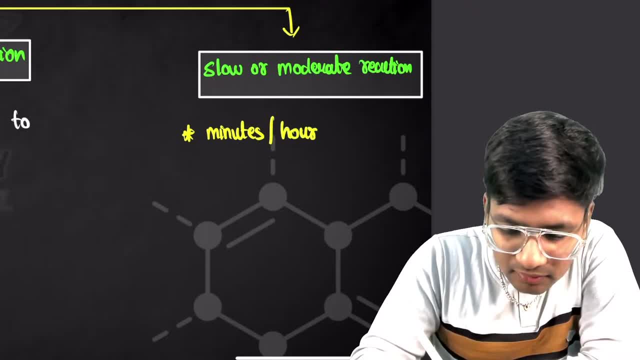 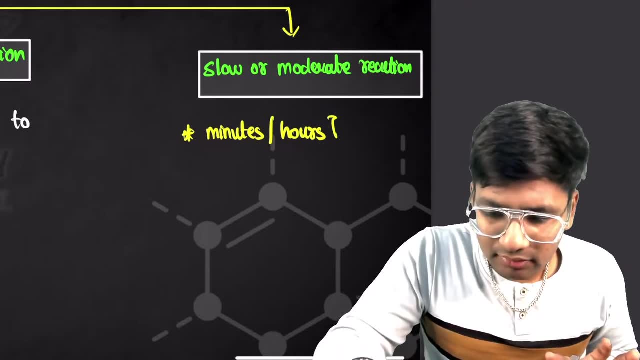 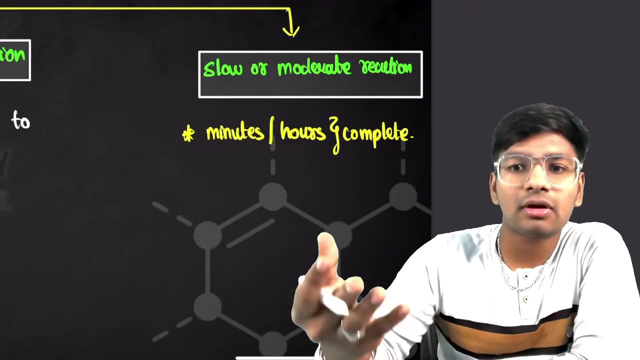 Minutes and hours. It will be completed in minutes and hours. Okay, Don't spend too much time in days and hours. It will be completed. It will be completed. Then what will happen? You'll know. your reaction will end in this much minutes And in this much minutes. your reaction will end in this much minutes. 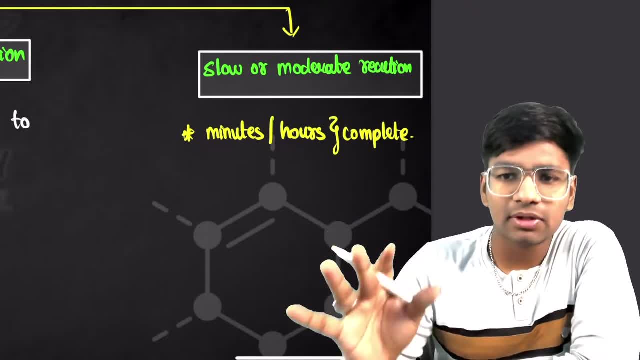 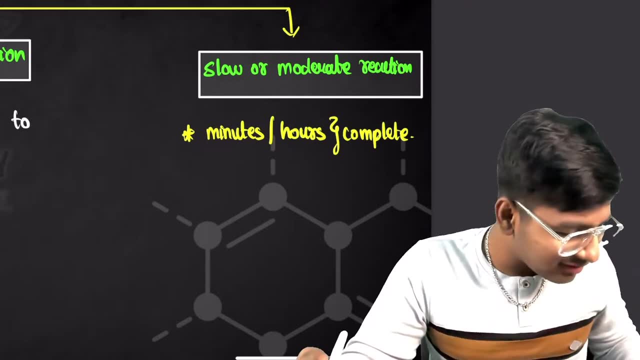 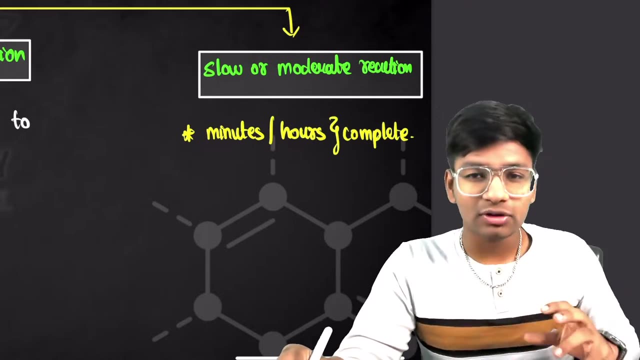 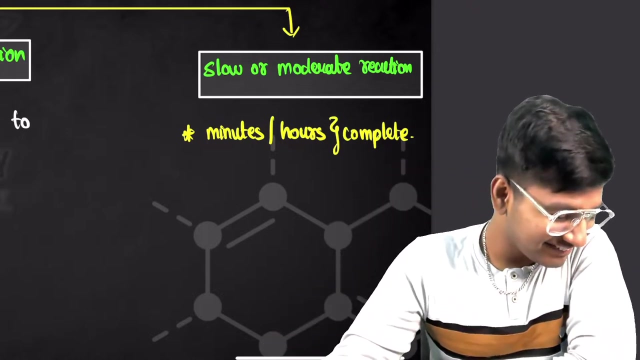 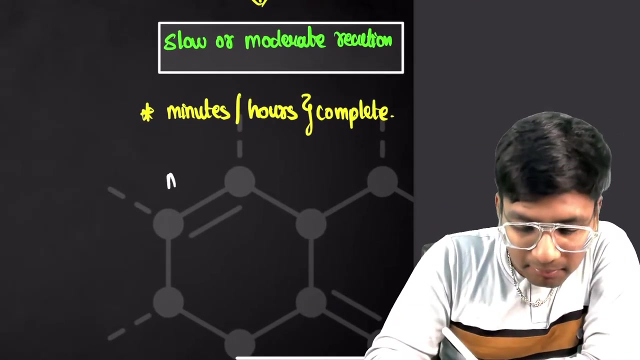 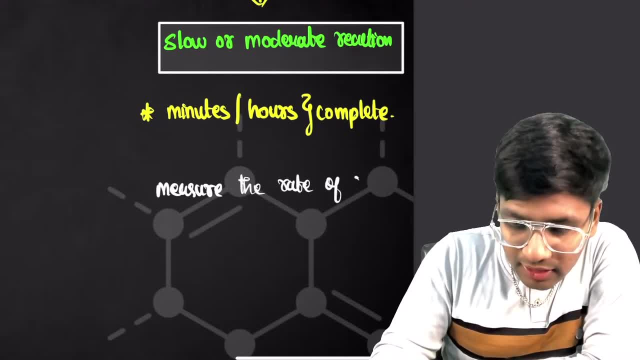 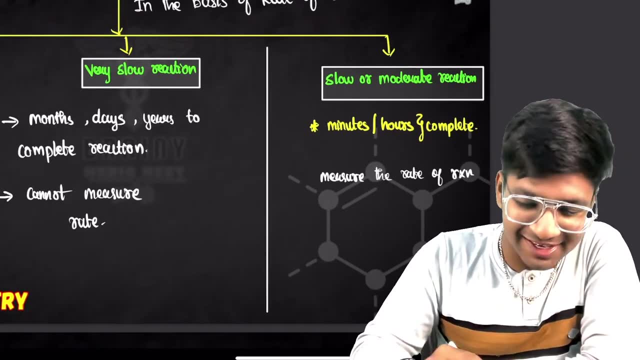 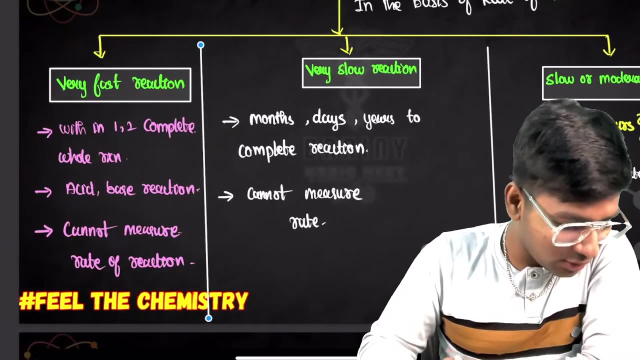 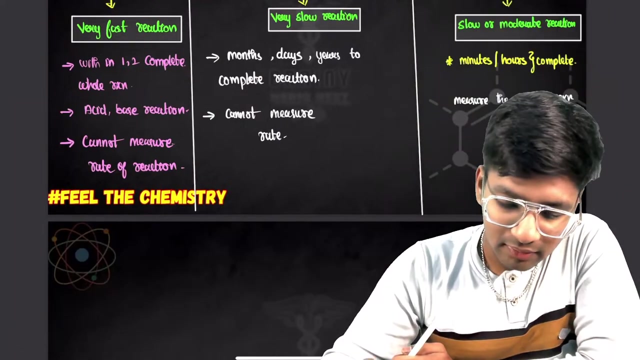 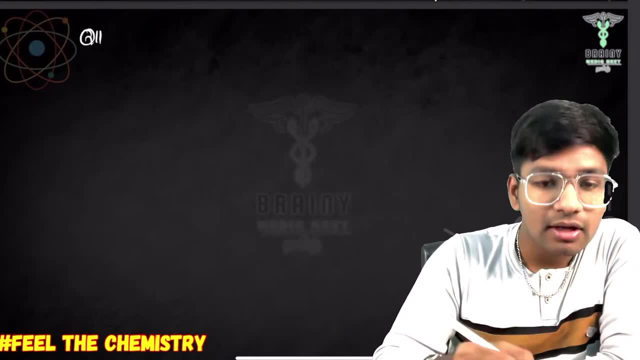 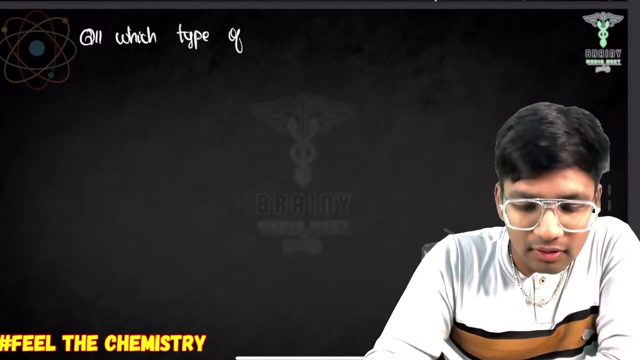 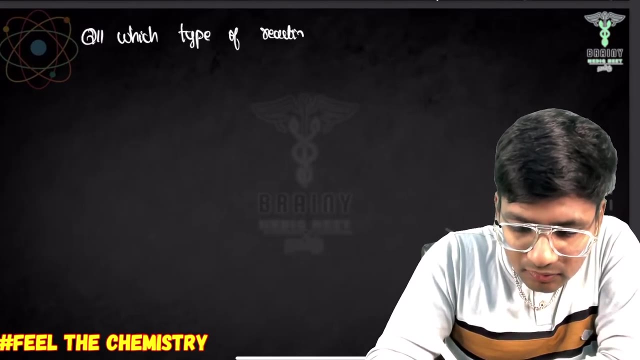 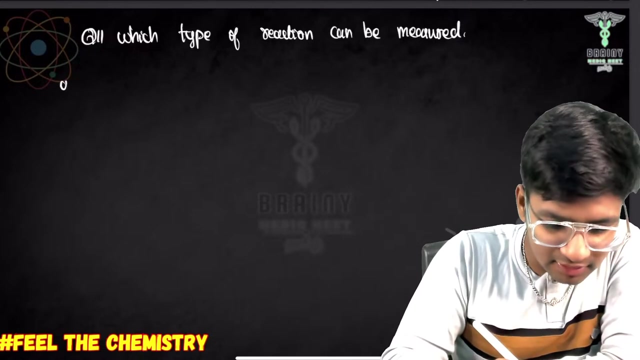 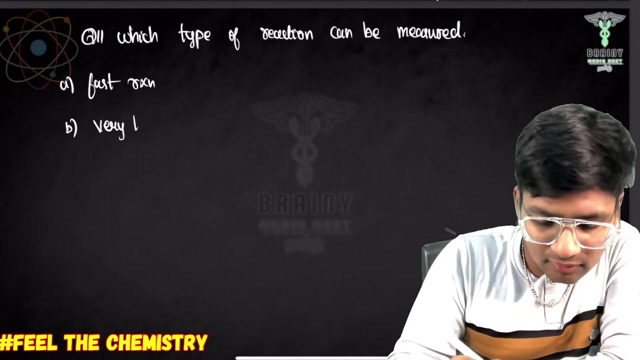 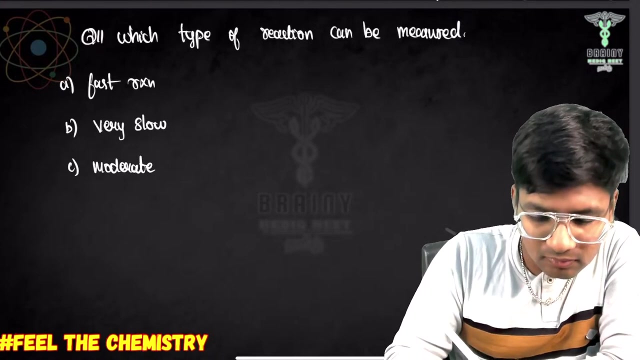 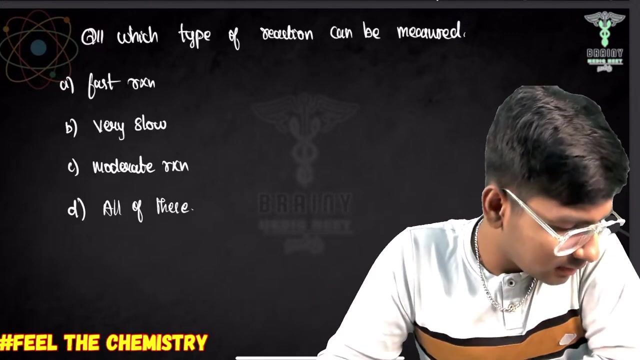 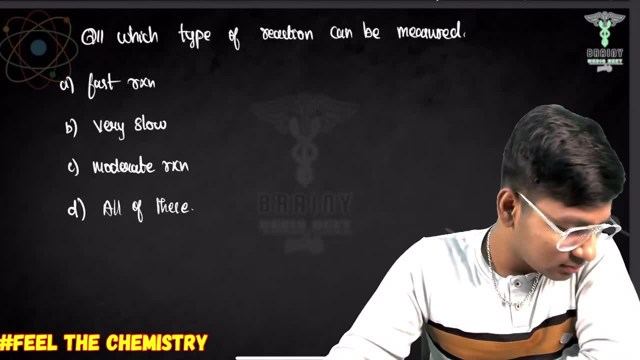 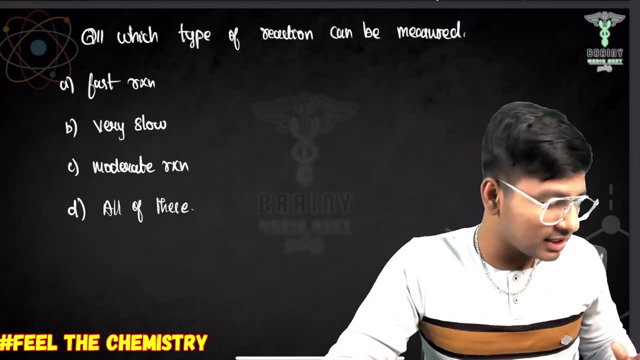 rate measure. ok, very easy question. if a sonata, which a pretty good through the question and I was in the answer, sorry for late, no problem. no problem, see. see is the correct answer. yeah, I need the ncr delay. you can and I am going to, not a. 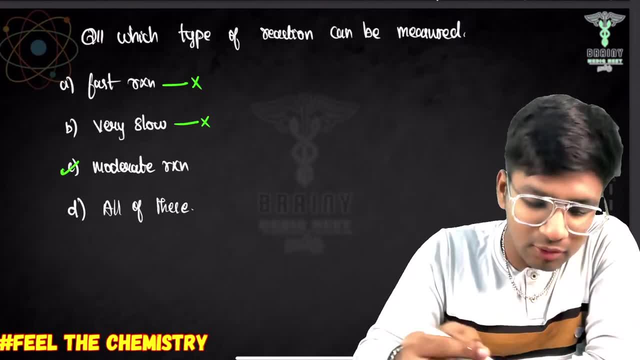 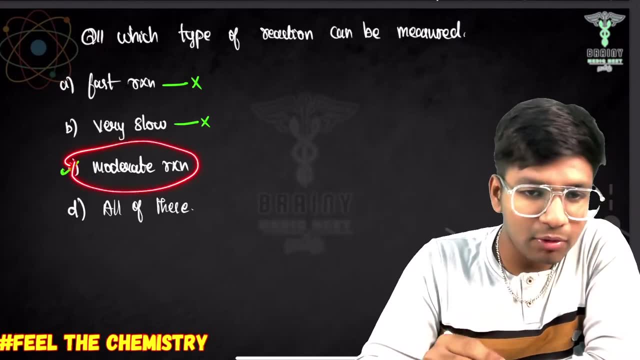 martin guy there, but not okay. so see either in the way when the one other measure panamera, you know measure panamera, you know measure panamera there. okay, so you can measure moderate type of reaction. all of this can be powered out of the editor and I may end up over on a rate to pop or rate to 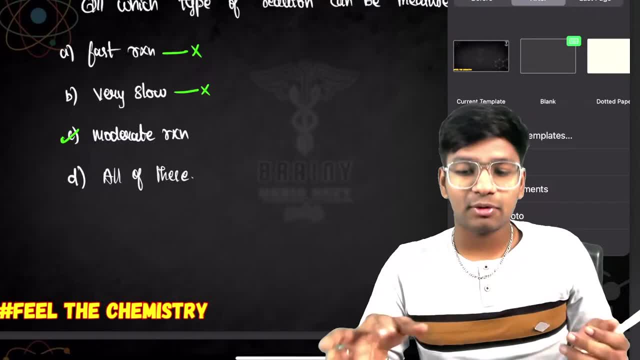 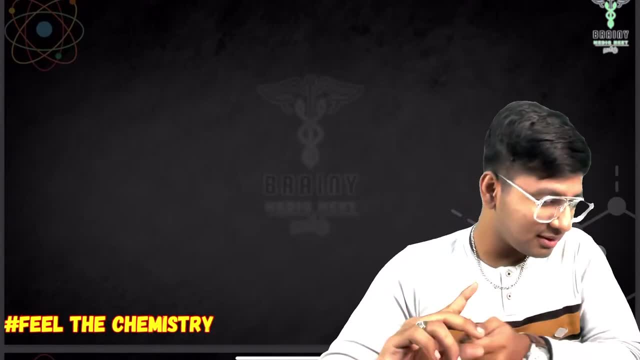 pop or not, a rate to pop, or I'm so Lala great, great night. now I've been so liberal or I've been sold, I think on the top. I did the pinion in your pro and I sold ran in the summer period on very, very, very a fan item. bro, bro, okay. 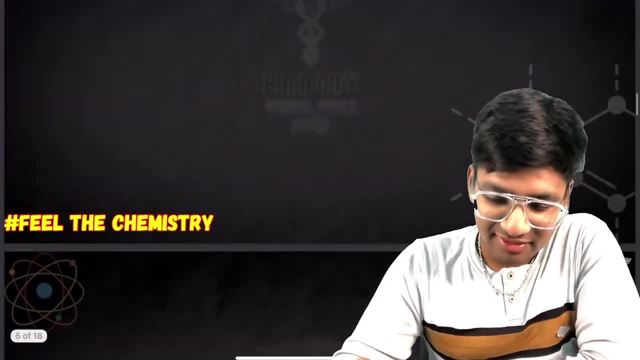 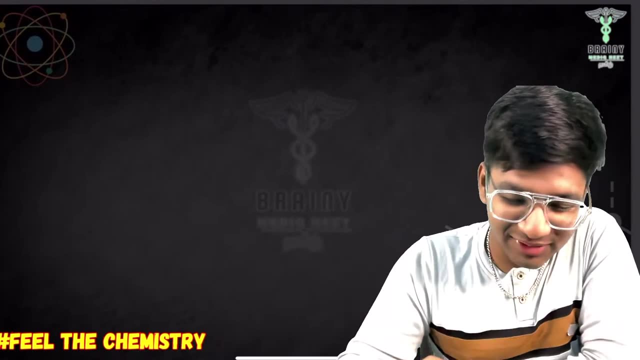 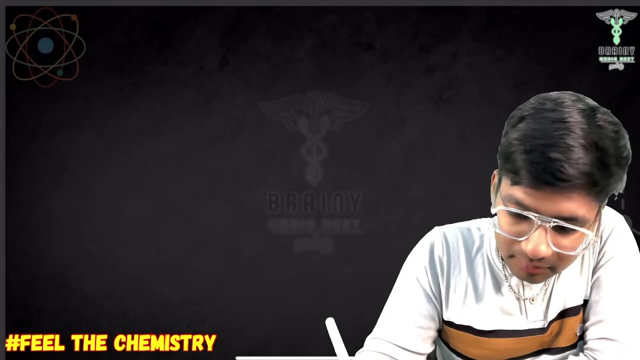 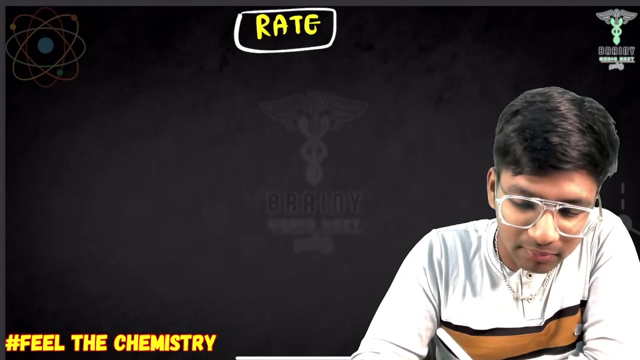 O'Shaughnessy Oriental Oriental. you know, Dr Nezha, my name is not based on the limit of the pathology, that the money I'd say. I think I said you wouldn't. ah, next to date, what is a date great? when I could get into a rate nine, our definition so liquid, or panga, correct ah? 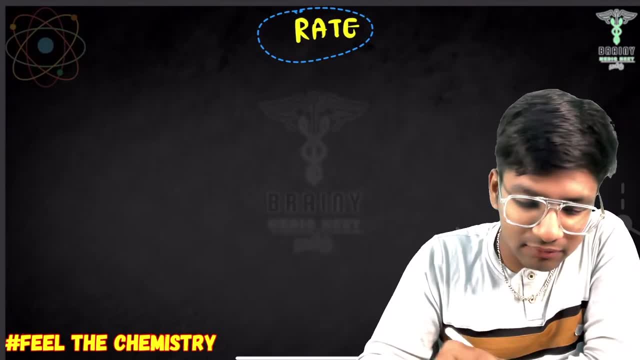 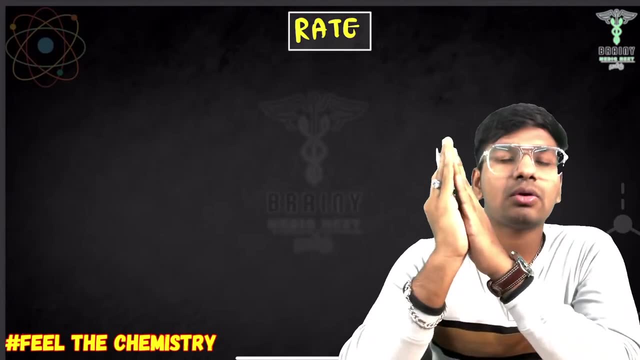 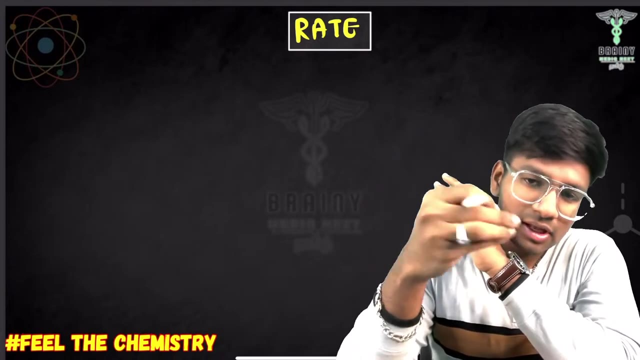 one of the things over eight, nine and our definition. something would definition, you know, a definition of the future, correct, ah, but trade or reaction or reaction, not a good enough to manage on that. ah, okay, what a reaction. not a calculation of the reaction and it pretty much. 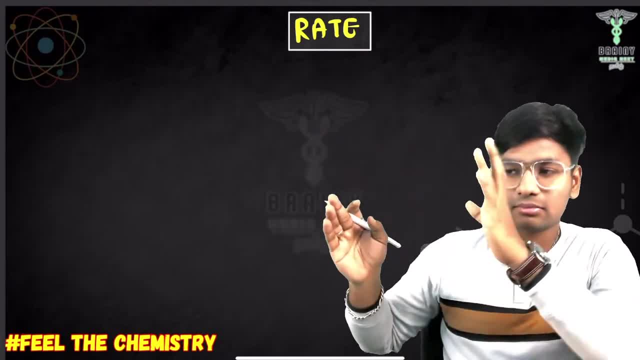 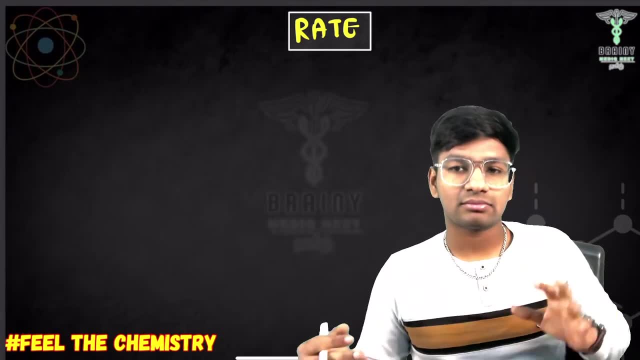 measure for na, my number number two. good to beat a inom bi-randal reaction or contactable. I've just put an item rhυ reaction, the reaction like a hem zen and measure like that and get me the reaction. I've been a measure from lake. well, if they don't, let me share on the. 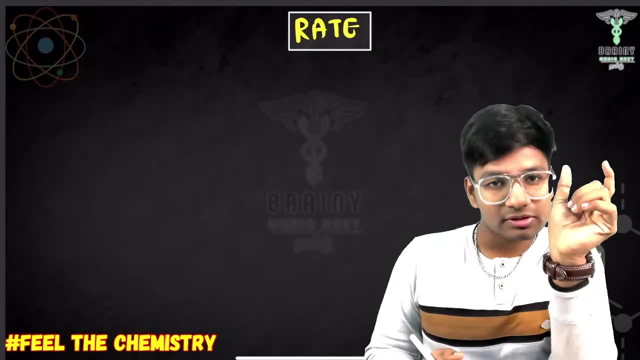 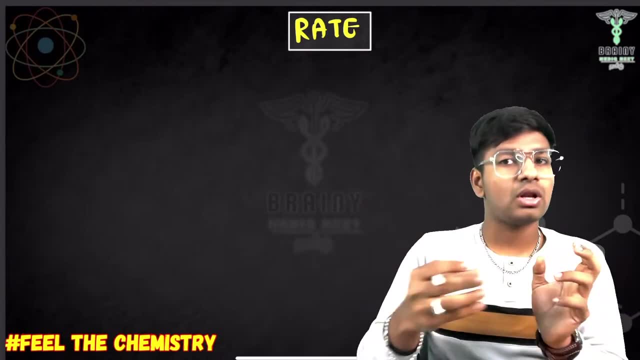 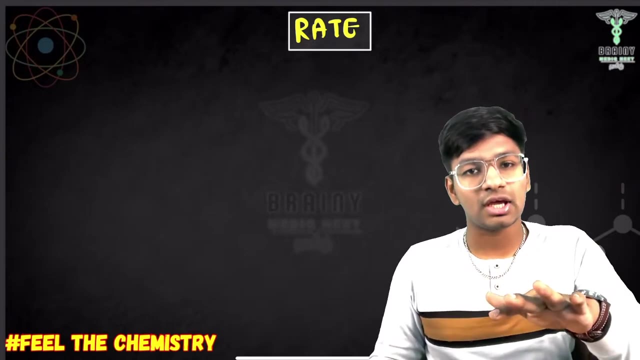 measure money with requested upon that for a reaction, la substance for concentration, or go on the concentration of agor interprets album here and I'm. it will decrease or increase. it will decrease. you should measure. that means how much concentration reduced or increased. ok, it decreased and increased. 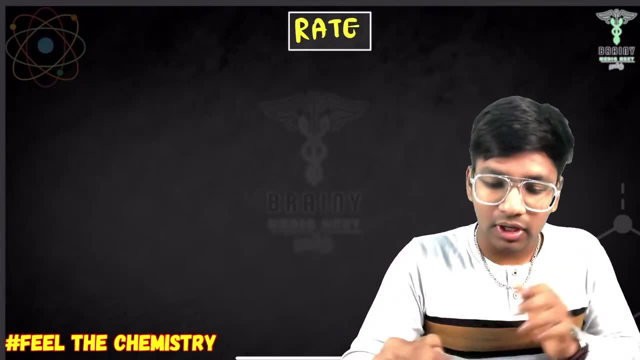 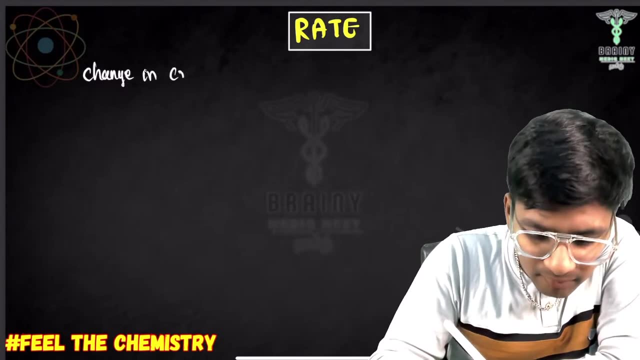 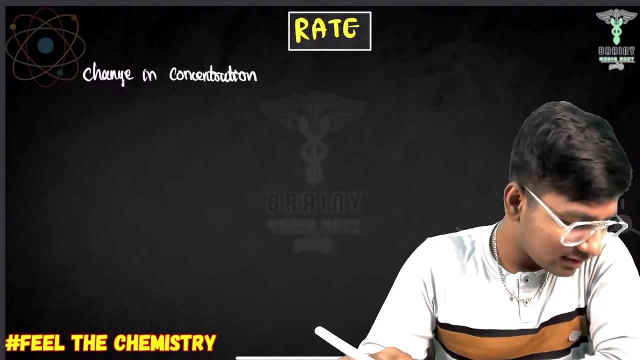 how much time it took. this the rate. ok, now take a definition: change in change in concentration. concentration, concentration- change in concentration. ok, What is my phone? What phone do you have? Wait, if I see all the questions, I will answer them at the end. 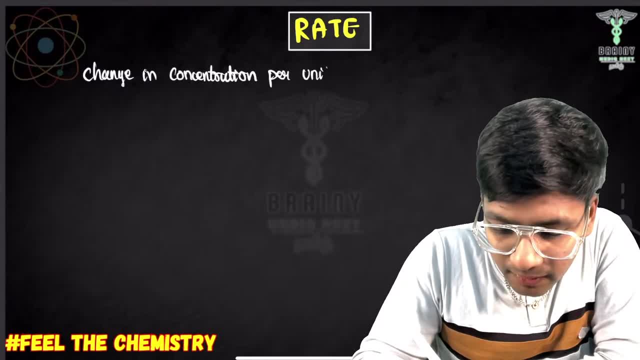 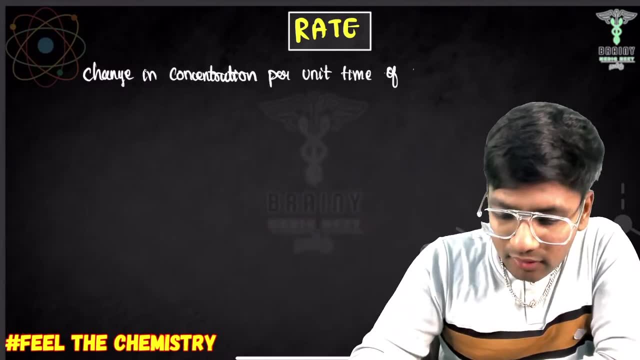 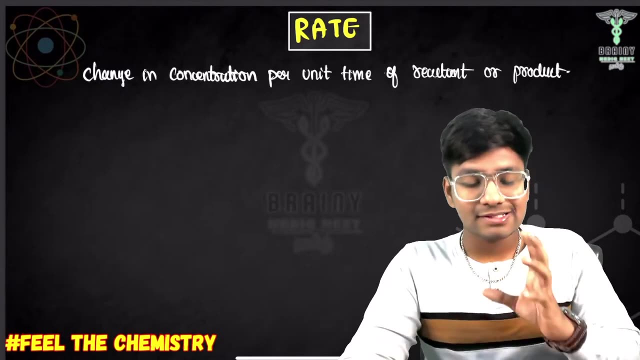 I will not answer now. Per unit time. Per unit time Time of reactant or product, Of reactant or product. Ok, Ok, I will ask another question: Is it possible for rate to be negative in India? Is it possible for rate to be negative or not? 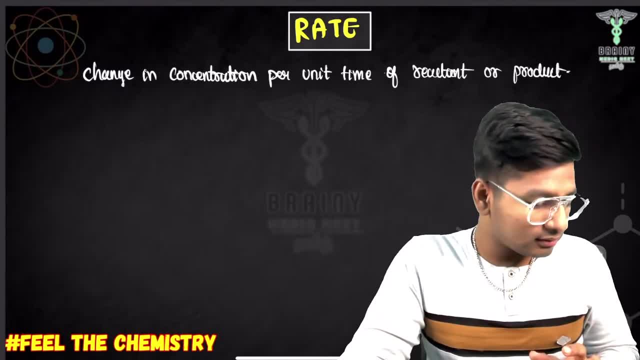 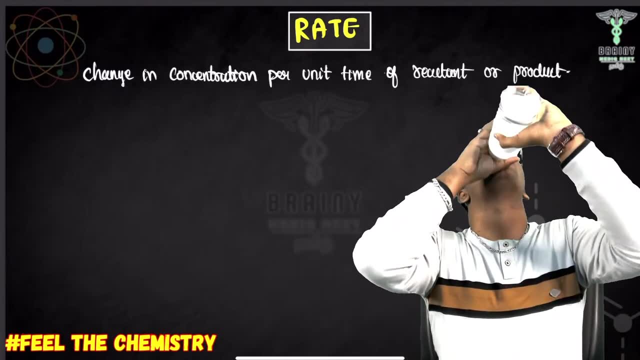 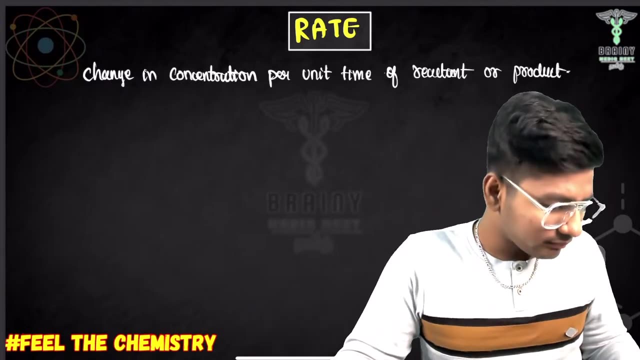 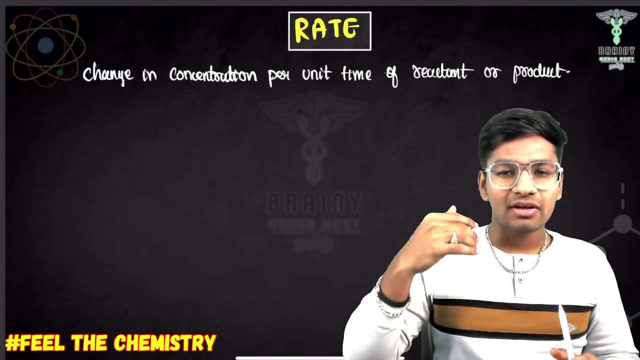 Next question: Is rate possible for rate to be negative or not? Just think and answer this question. Just think, For example, call your friend and say: Hello dude, where are you? I am going behind in minus 20 meter per second. 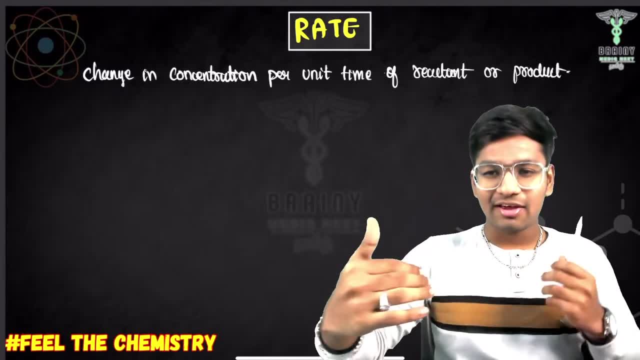 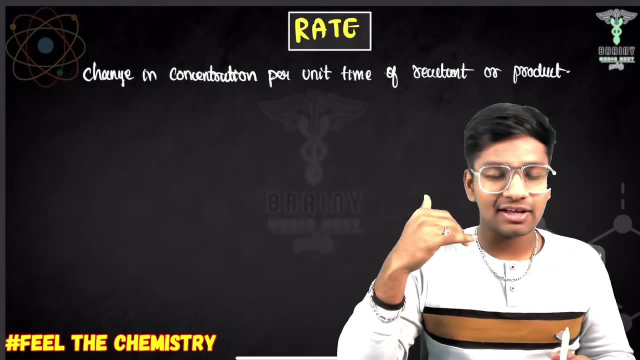 I am going behind in minus 20 meter per second. Can you say that I am going inside the house? Huh, Can you understand? Hello dude, where are you? Can you say that I am going inside the house in minus 20 meter per second? 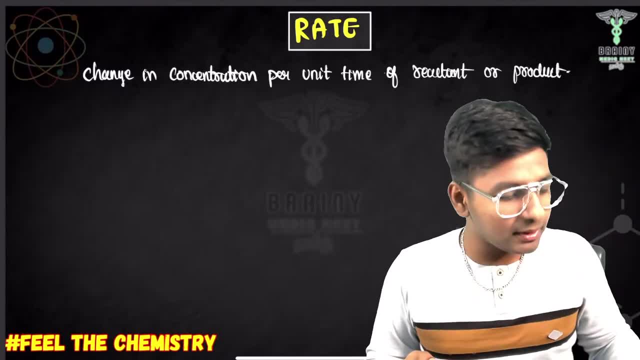 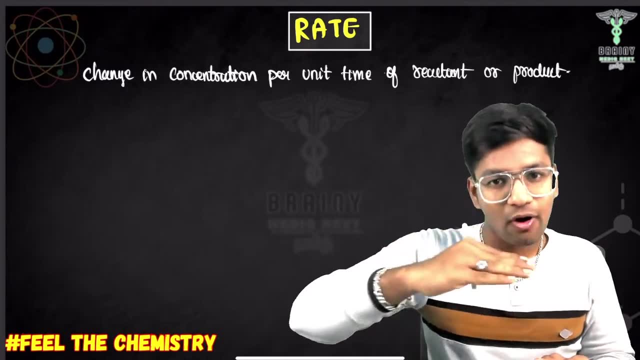 It cannot be negative. There is no chance of being negative Because One is less. Ok, I will tell you what is less, But instead of going forward, you cannot go backward. You can go backward, but you can only indicate the direction. 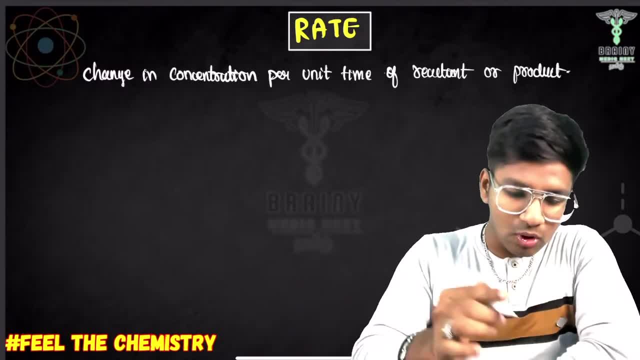 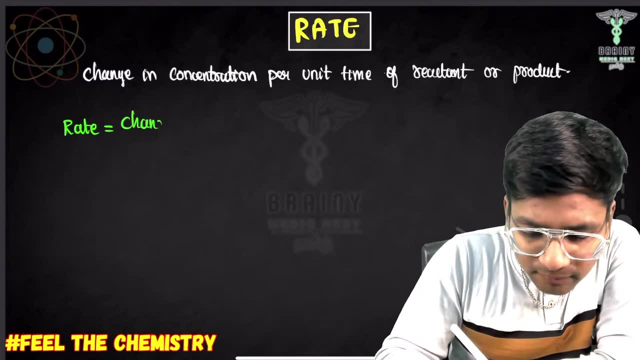 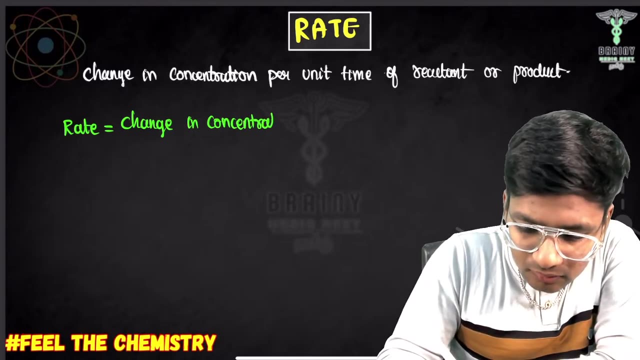 Instead, you can only indicate the rate in negative. But instead of going forward, you cannot indicate the direction. Ok, So if you see, here I have told you the formula for rate I have taken. the formula Rate is equal to change in concentration divided by time taken. 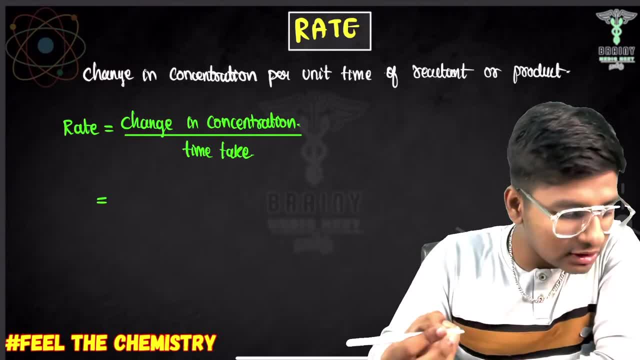 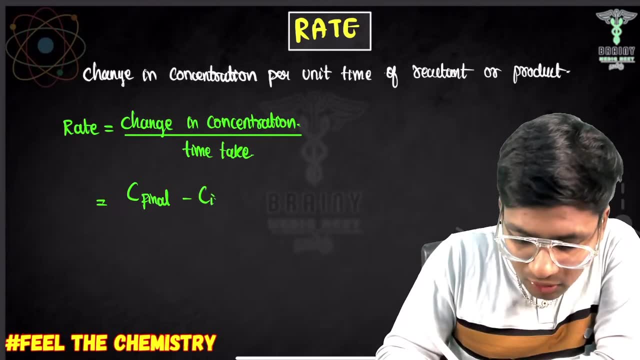 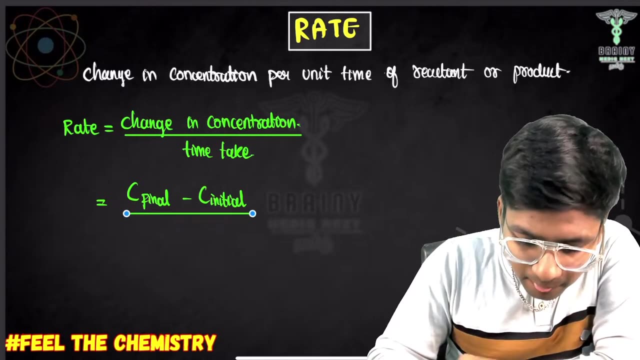 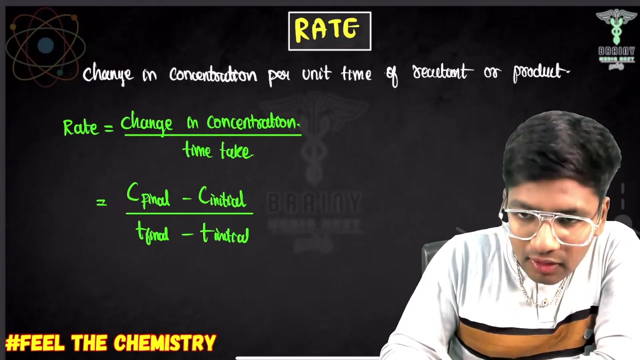 Time taken. You must have known this formula, So change in concentration. I can write it: See: final Final concentration minus initial concentration. Initial concentration divided by time is the same: T final minus T initial. Correct: T final minus T initial. 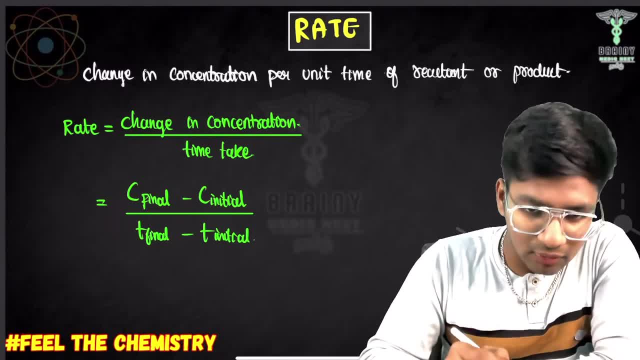 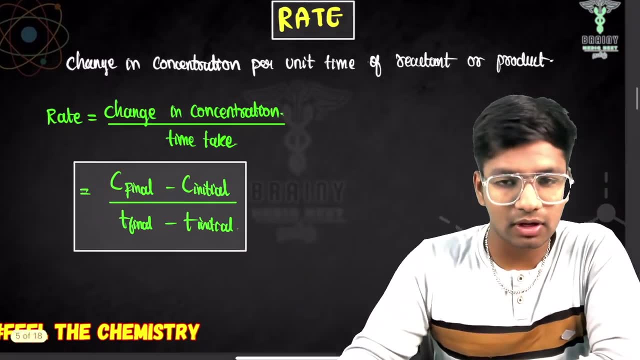 Done. So this is something that all of you must have known. So, Ok, If you do not know the collision theory, I have told you that I will write the lecture on collision theory. I will cover the lecture in full, For example, 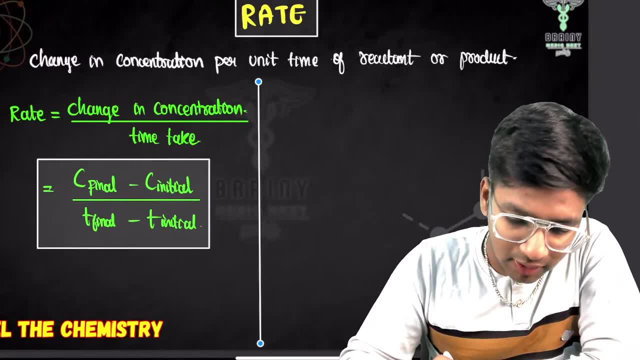 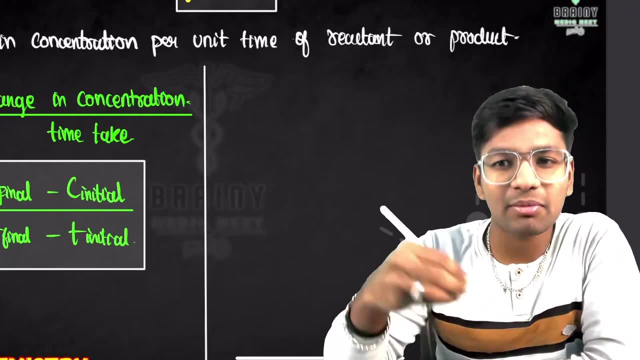 I will tell you an example. See this example. Let us go with the example. And who else thought that physical chemistry is boring? Is physical chemistry boring? Tell me, Is it possible to conduct physical chemistry like this? I will bring it. 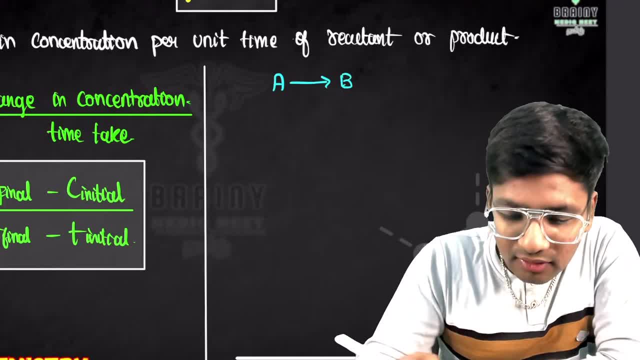 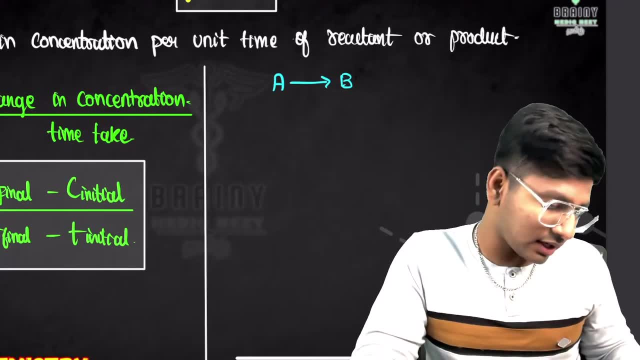 I will tell you how to conduct it. A to B: Ok, B goes from A. Ok B goes from A. B is a reaction Suppose, if you are not liking it. If you are not liking it, At least subscribe and watch. 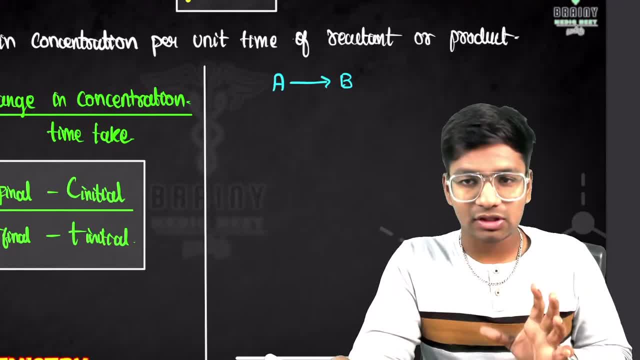 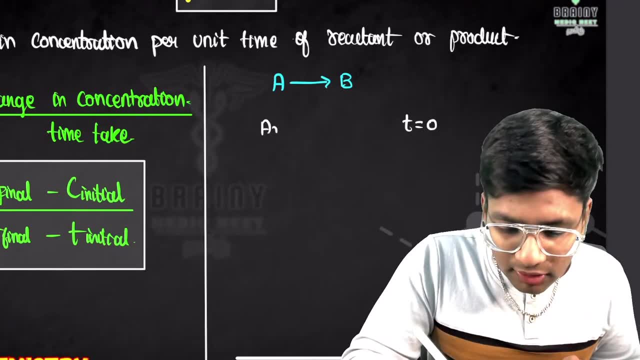 If you are not subscribing, At least subscribe and watch. B goes from A towards a reaction, Initially, Initially. In T is equal to 0, I will write A as A naught. T is equal to 0 times when I write A as A naught. 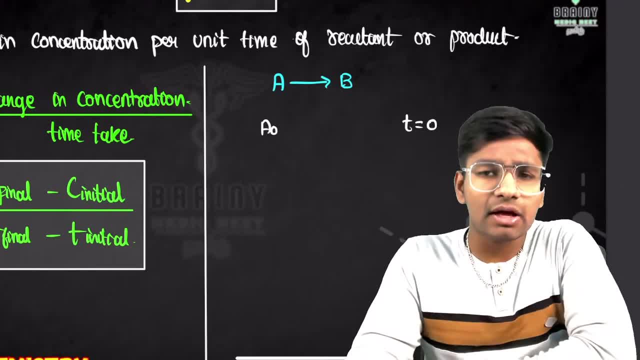 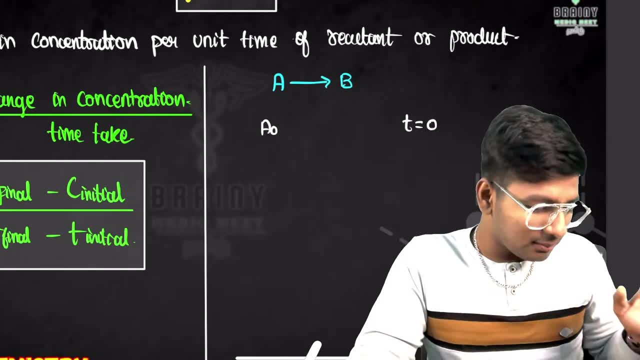 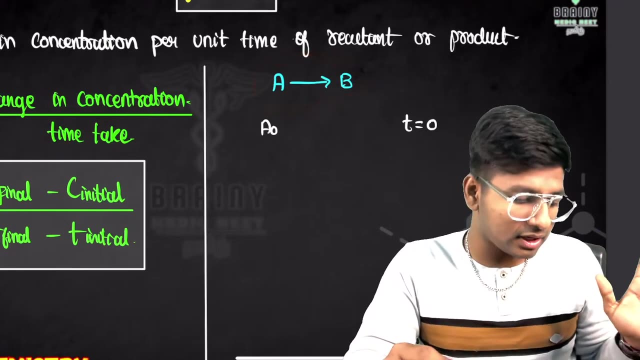 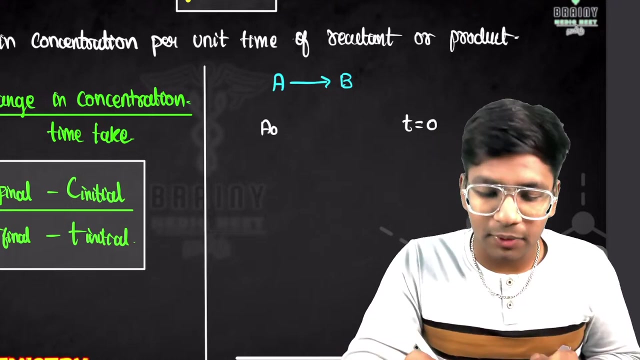 Ok. So what will be B? What will be B? Ok, What will be B? T is equal to A, t is equal to 0 in the concentration of A. I have just started the reaction: ok, see, the reaction is 0,. many of you will not understand how it is 0. 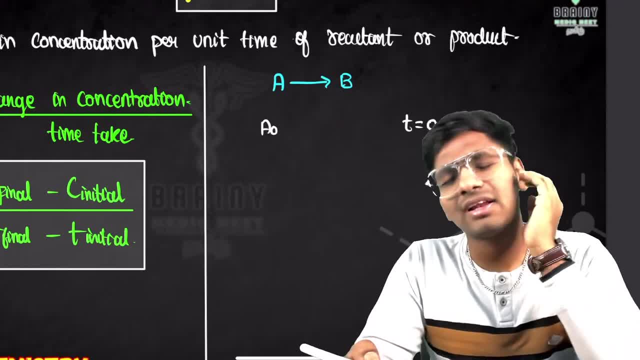 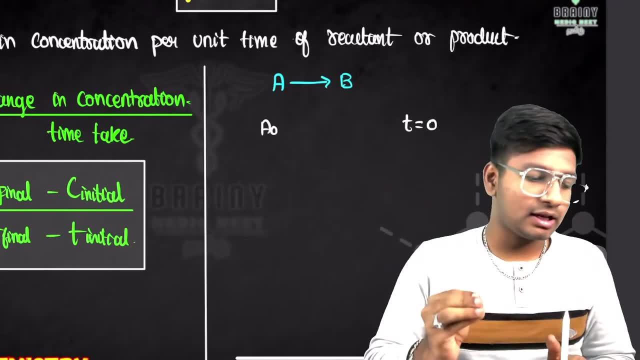 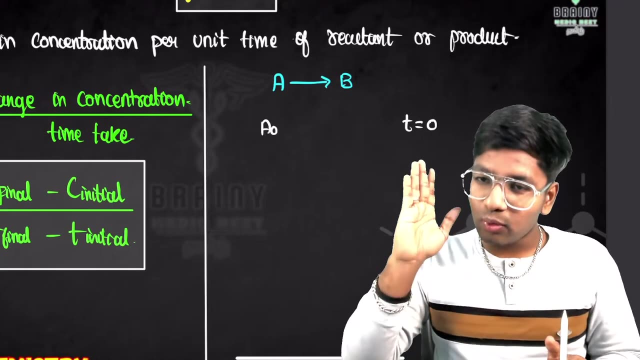 you will ask me: I don't know, sir. I am also thinking from 3 concepts. for example: suppose a girl is hitting you. what did you do yesterday? you went to propose to someone. suppose a girl hits you in time 0, she doesn't hit you. 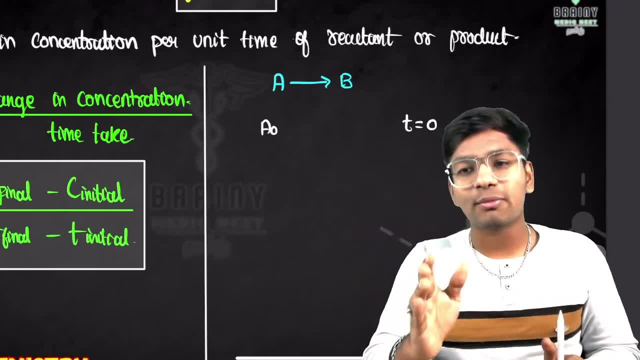 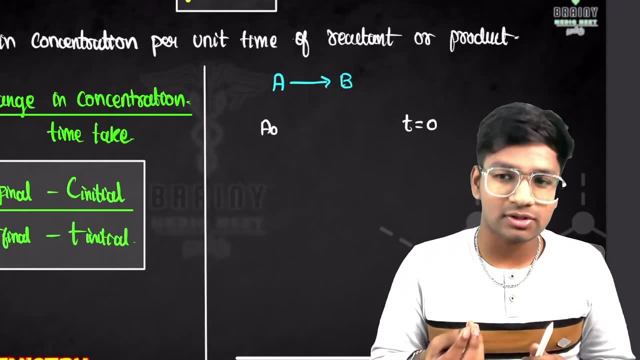 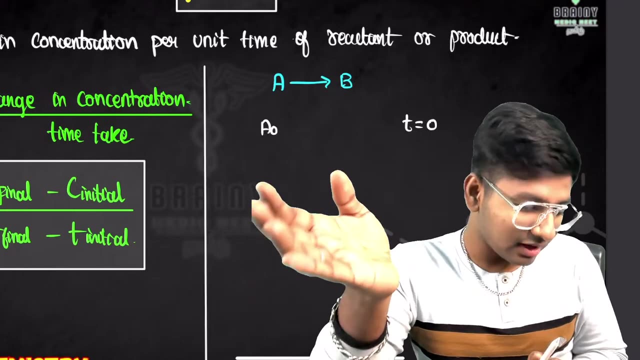 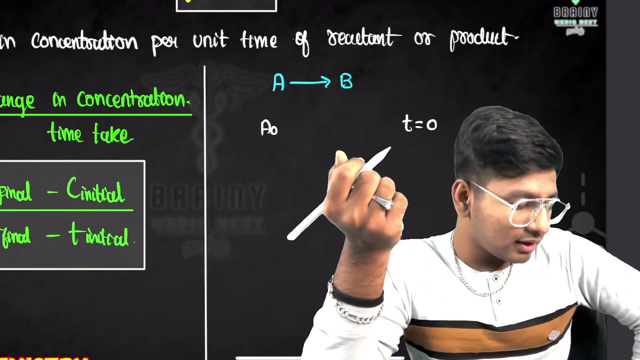 in a fraction of seconds of time. only then you would tell: please, please- you will think it material needs to be on the floor. the time 0 did not hit you, then how you can call this plan a reaction process simple. this is a simple question, so in time zero, many of you may have doubt about this. 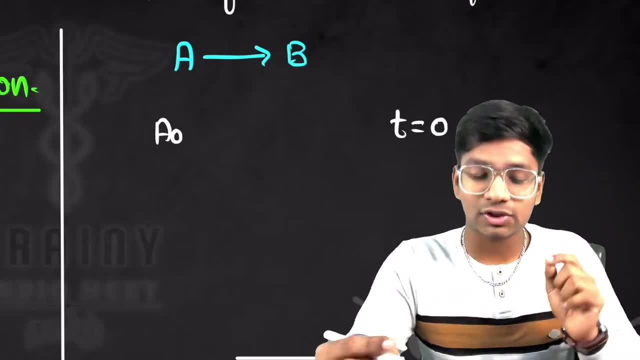 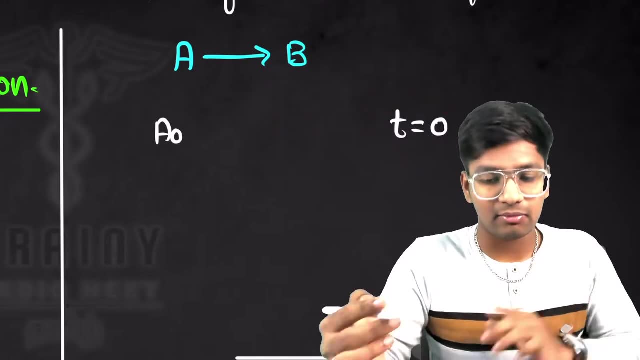 because when I was studying this, I had a big doubt about this, how this becomes zero in time zero because I did not know the basics. I did not know the basics, so I am telling this in this time. so in time zero, reaction is not proceeded, only this side is concentrated. 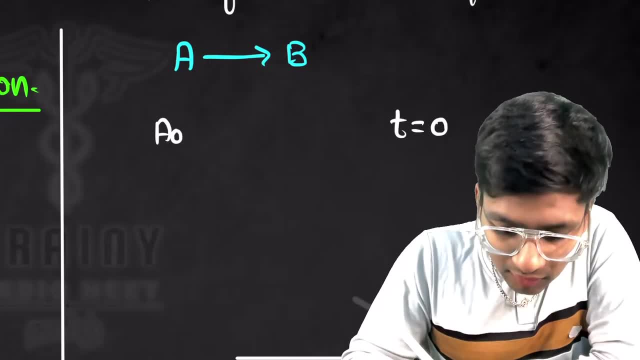 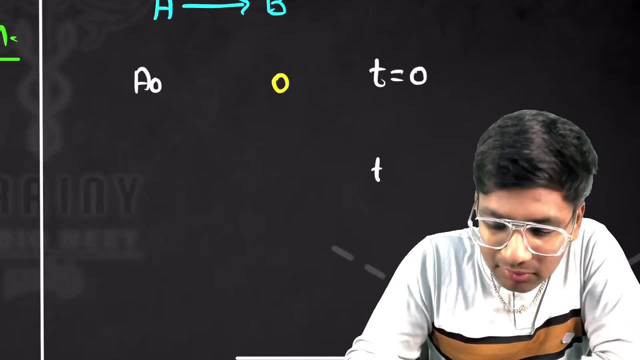 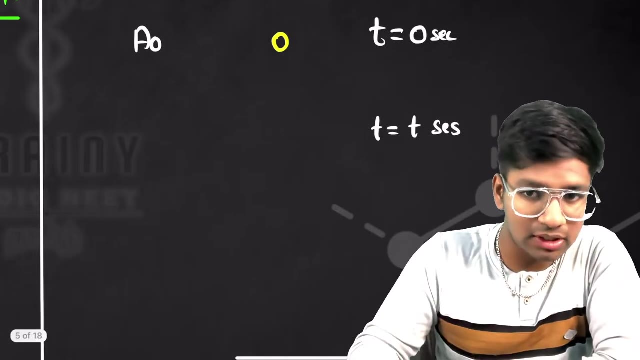 it is not hit yet. you will know when you get the answer. so this is zero in time, zero next time: t. what is time time? t becomes t seconds. this is zero second. this is t second. when it is in zero second, it looks like this: 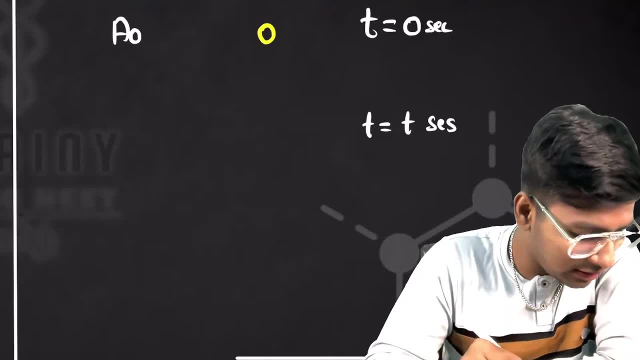 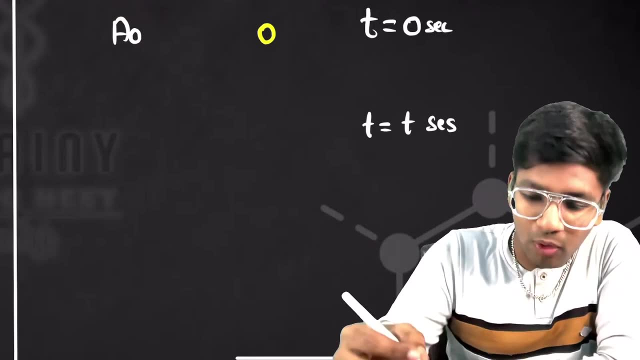 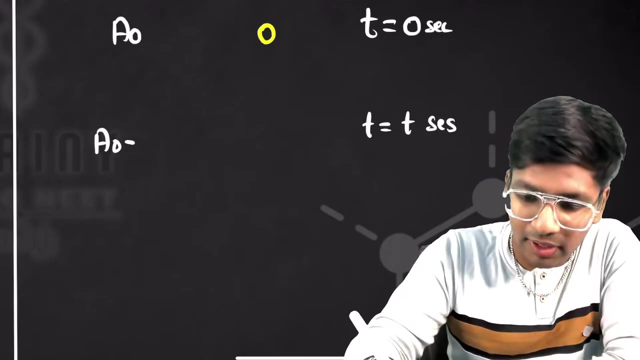 ok, now what happens next? what happens next is from here. a certain concentration goes out. a certain concentration goes out. it will not give all the energy. it will give some energy from the energy it has. so from that a0, a certain energy will be minus. 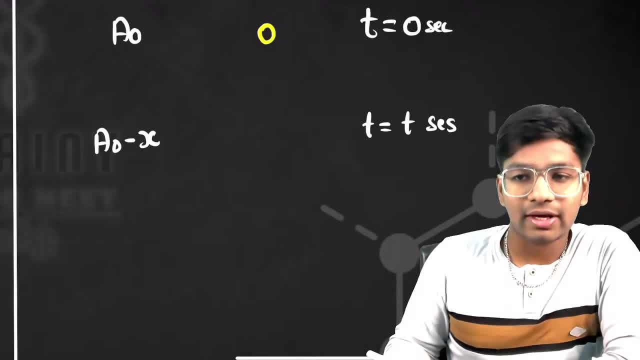 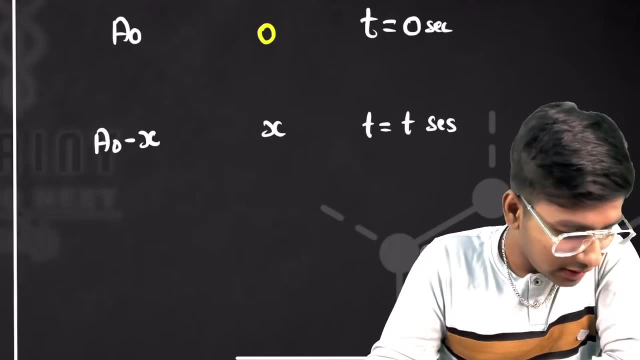 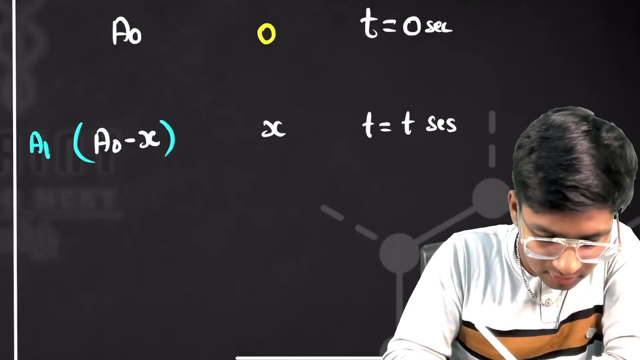 a certain energy, or let us call energy as concentration. so x, this x, will go to that place as concentration. so that x will come here, correct, that x will come here. so what I can say is this is the concentration in a t. ok, I am sitting and conducting the mole concept. 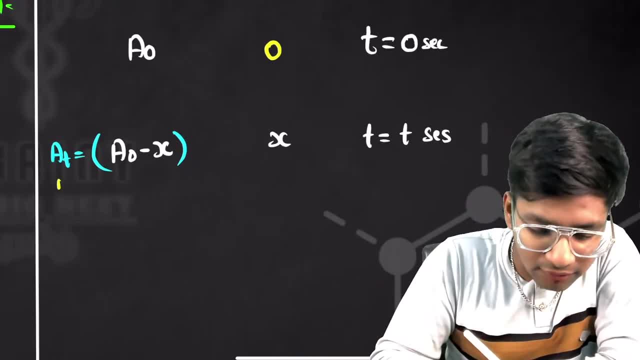 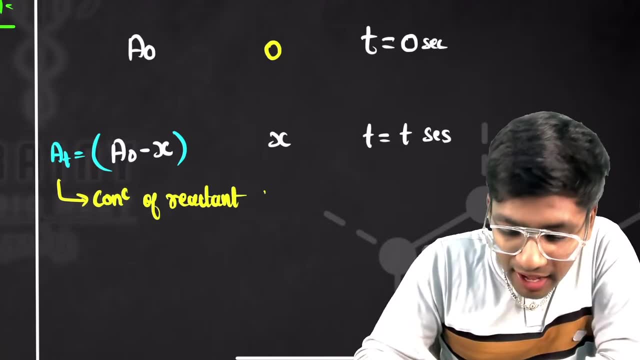 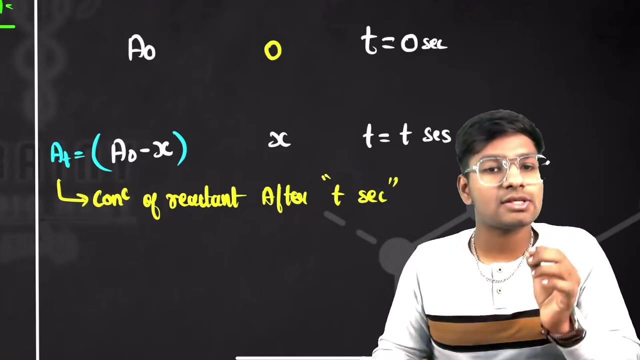 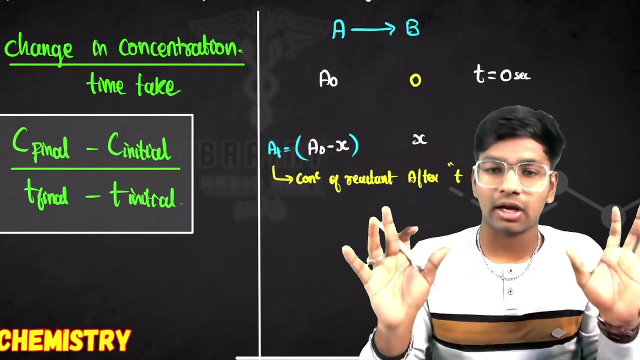 concentration in a t. concentration of reactant. concentration of reactant reactant after t seconds. t seconds after t seconds. what is the concentration now? come now, what you can do is you can measure the rate separately for reactant. you can measure the rate separately for product. 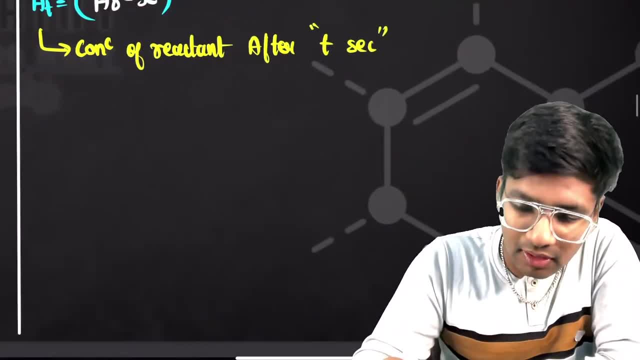 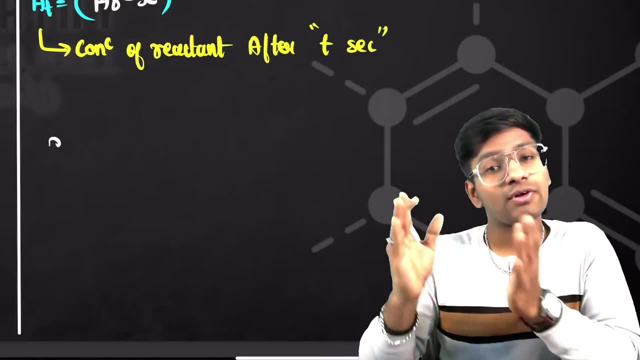 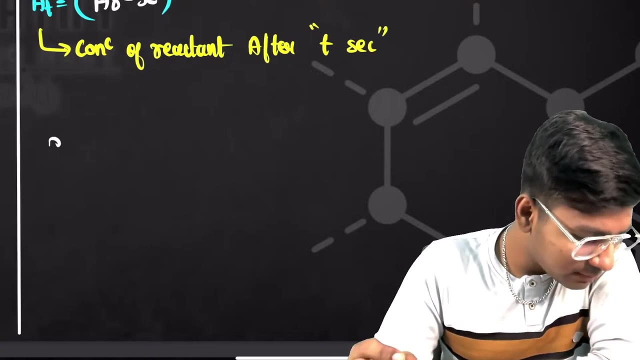 but everything is equal. I will say that again next. now, for example, reaction, that is rate of reaction, not rate of reaction, just rate. rate of reaction is different, rate is different, which means rate of reaction is different. in the rate of reaction is different. 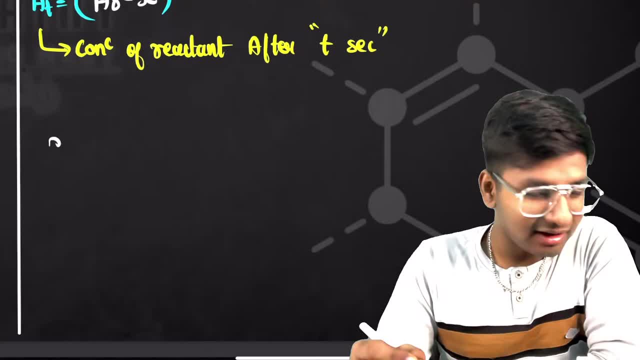 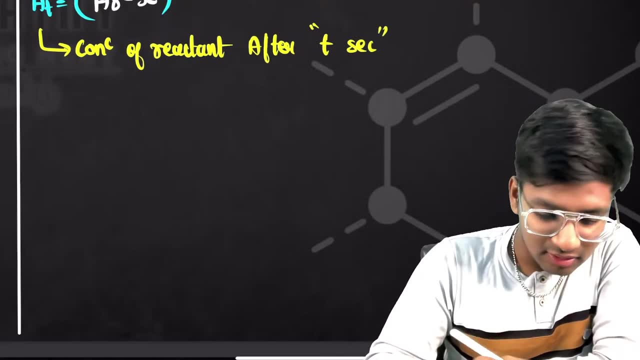 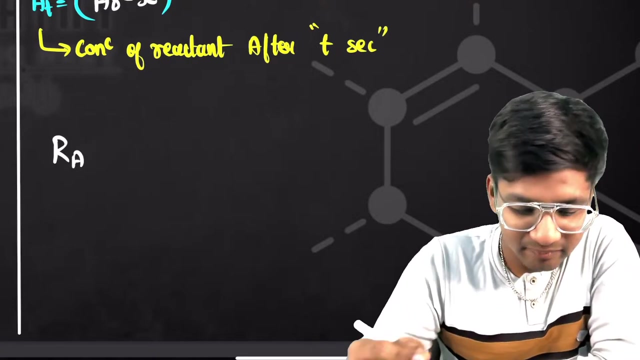 now let us see something like this: ok, it seems like it contains experience. yes, it has, just a little. I have not taken the proposal and received it, but it is a pump in school time. rate is rate of A. why am I not proposing anything? does it seem like I am proposing anything? 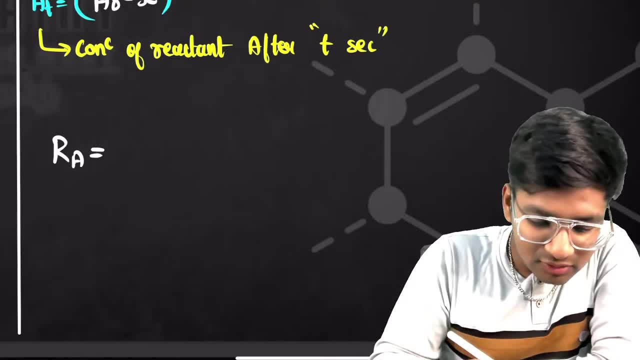 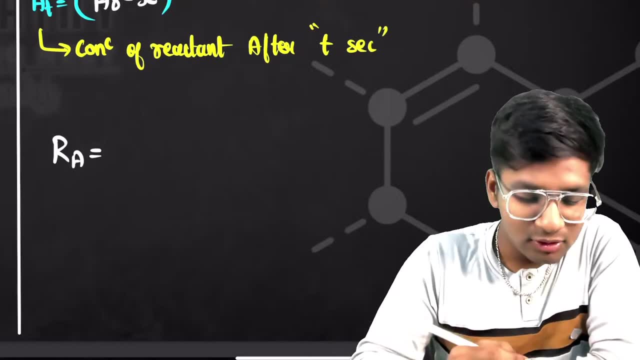 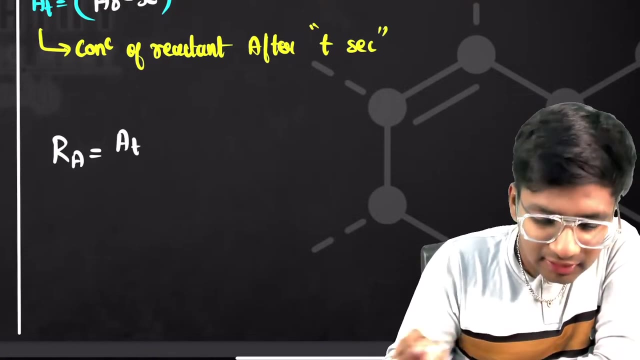 ha okay. so experience, experience on there. when they give them an experience, I think you're gonna get it decent on experience it so see. rate of the reaction. neither solar power first in a nap alone, yeah, but yeah T okay. rate of the reaction. final, final night of the. 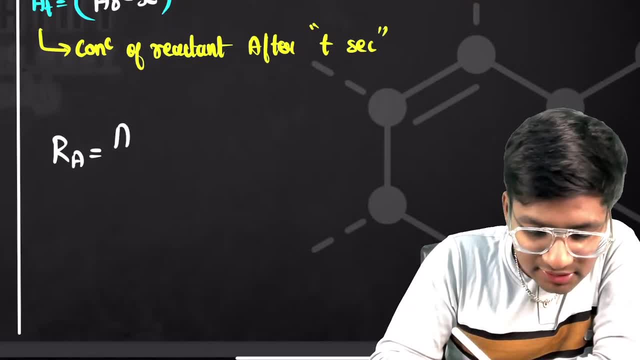 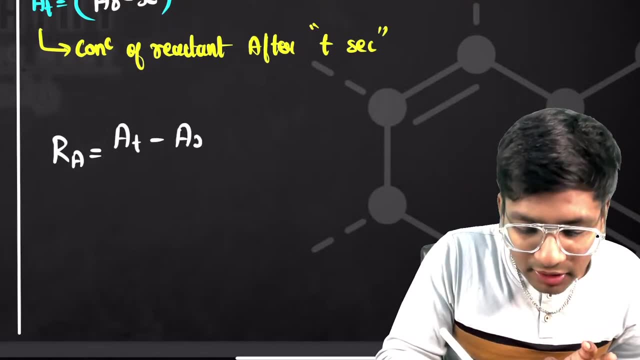 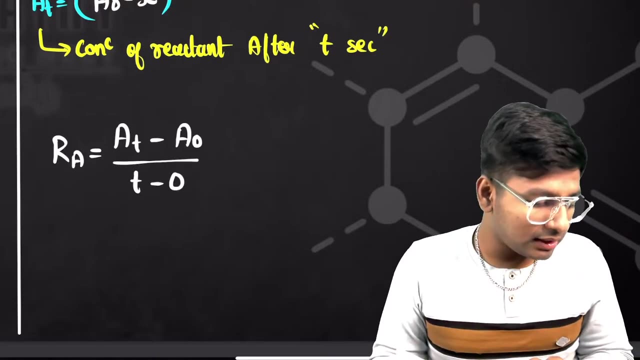 poor. okay, final reaction at the foreign, that is rate of reaction, the a or a concentration. a or a concentration after T seconds minus a or a concentration at initial. that is zero seconds. time for a final time: T minus zero seconds. a minus zero seconds, correct? ah, so even I end up. 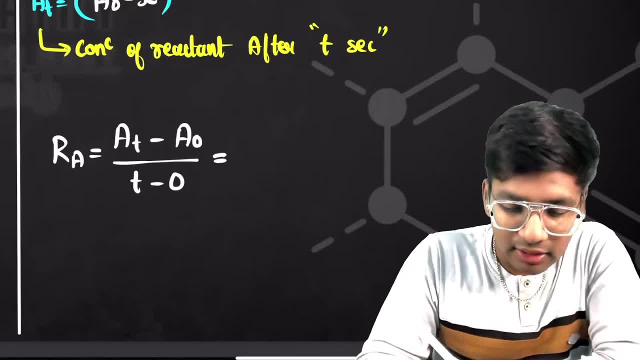 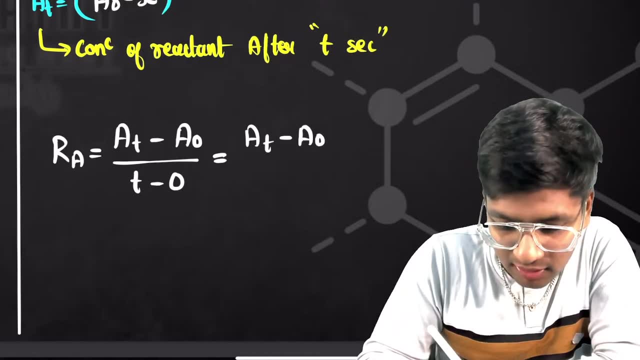 on line by 80 and I will either the foreign, yeah, yeah, okay, yeah, T minus. you know another than I'm a polar now concerned about for me I'm for a year to the one, a pro level go gonna do it, but even the rate rate will rate rate. 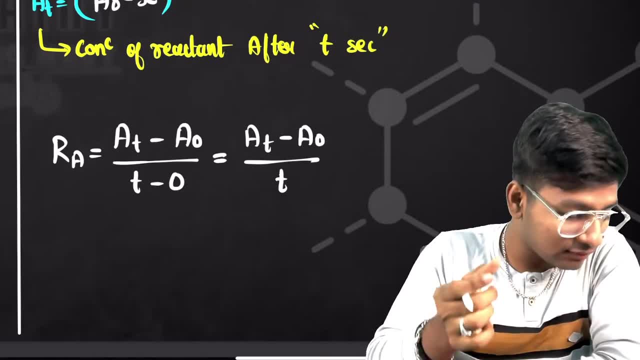 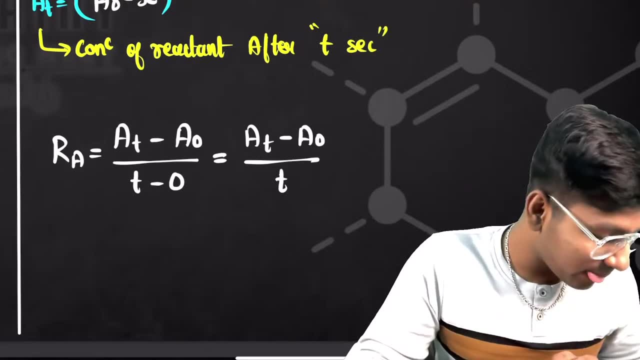 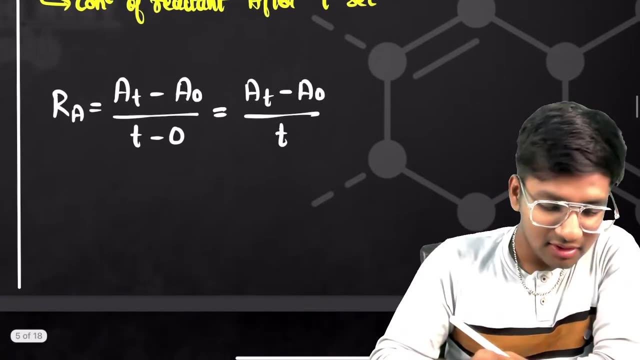 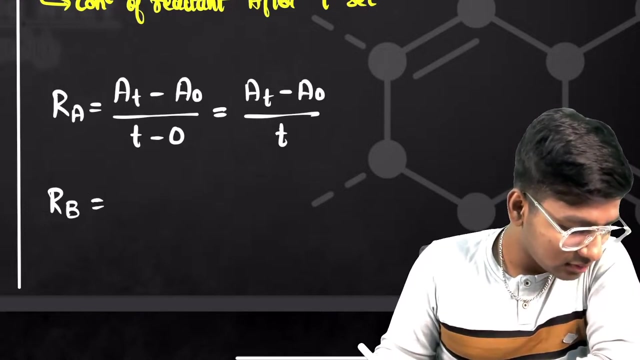 of reaction career. rate of reaction career. they're on you, the black boys. a nigga give up when I black boys repair which are kind of so near one next year rate of be gonna put a rate of be no more. I don't have the comment section. 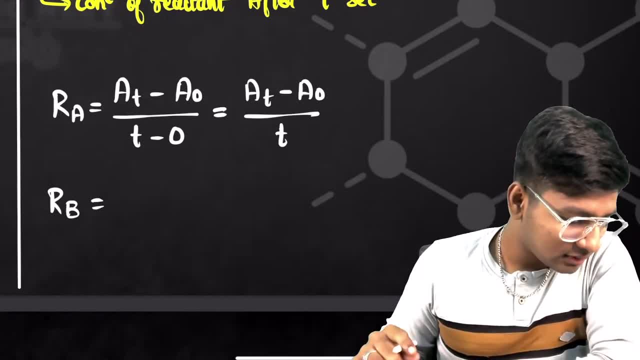 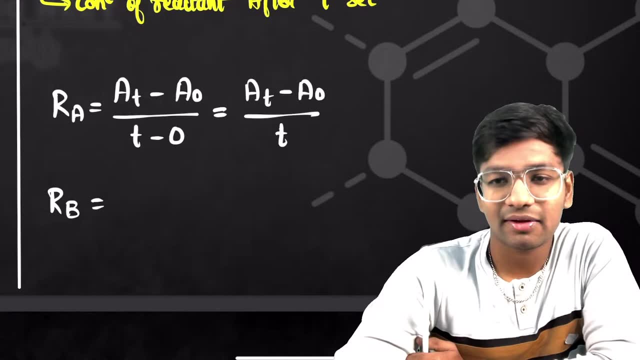 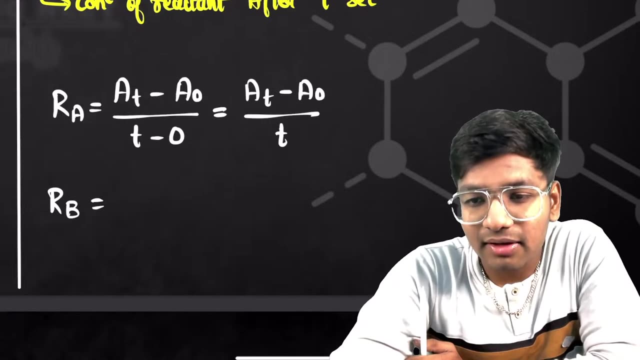 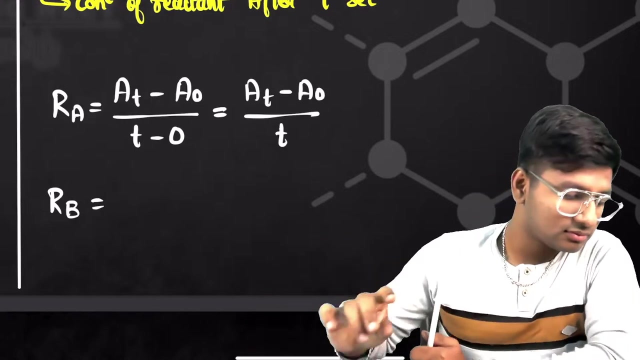 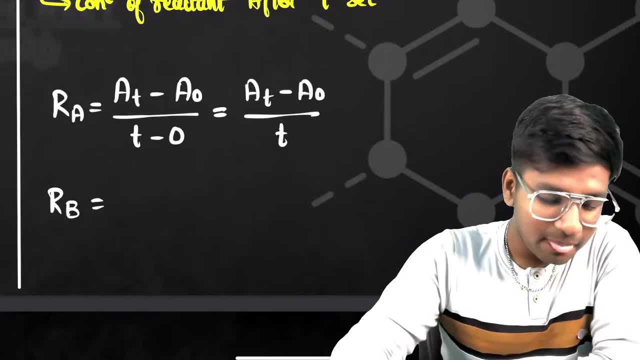 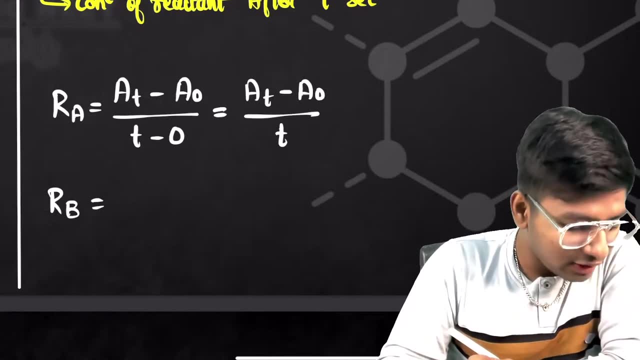 read alternative. so once you have all the time, yeah, dude, you want any reaction. get frustrated, read all this time. such an attitude, not worth to turn the supply but go enslaved, but you are. what was the result? I don't have any connection with this. I will not tell you anything. 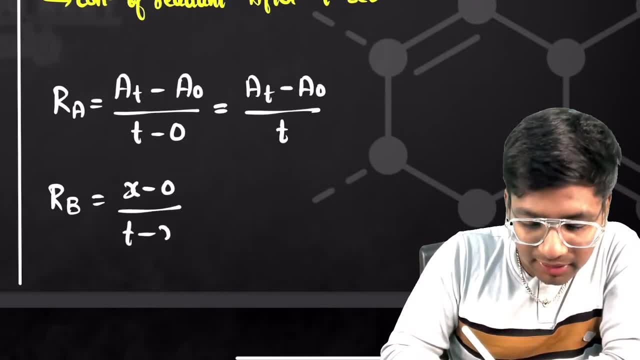 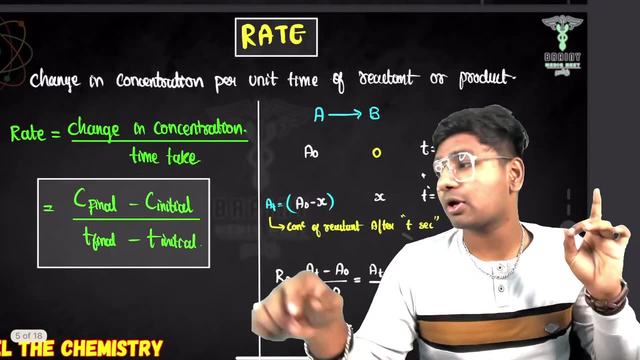 you don't get caught: x-0 divided by t-0, which is equal to x by t. till now I have told you. if you have any doubt, ask me in any step, because we will get the question from rate rate of the reaction, from molecularity. 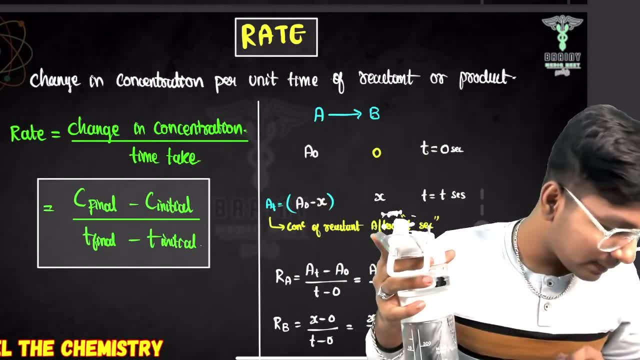 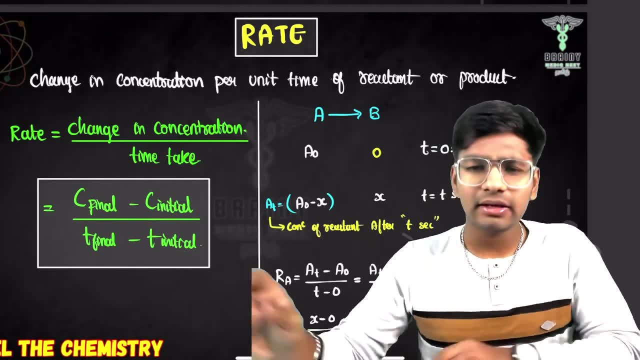 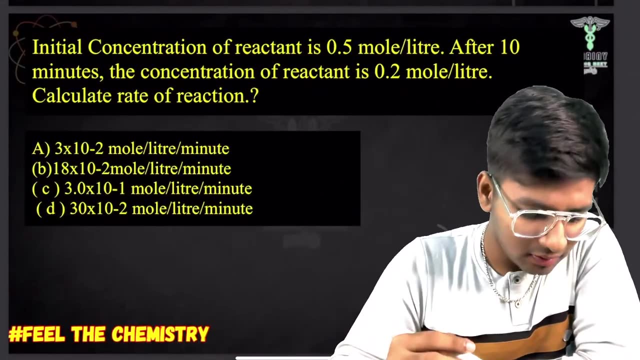 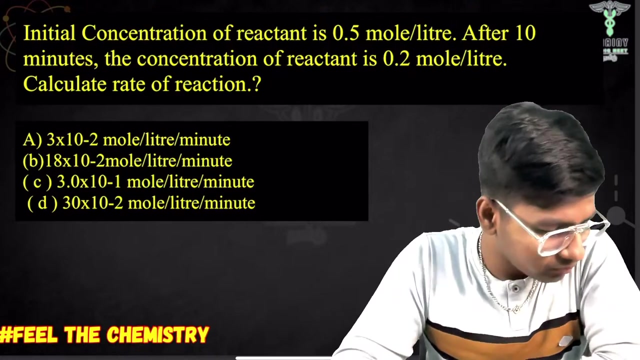 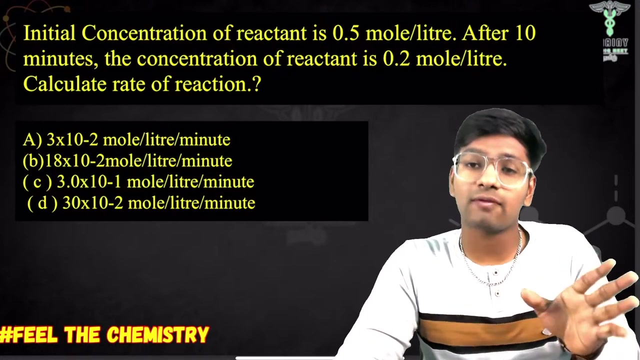 chances are there. ok, shall we go next? shall we go next? shall we go next? where are we going now? I will answer this question. very simple question, very simple question. answer this question. physics already has video. what subject you are expecting? video is already there. 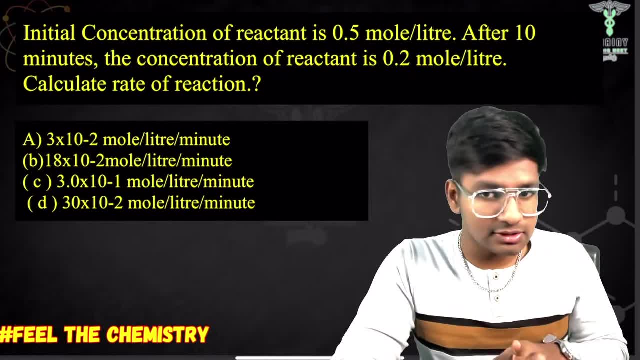 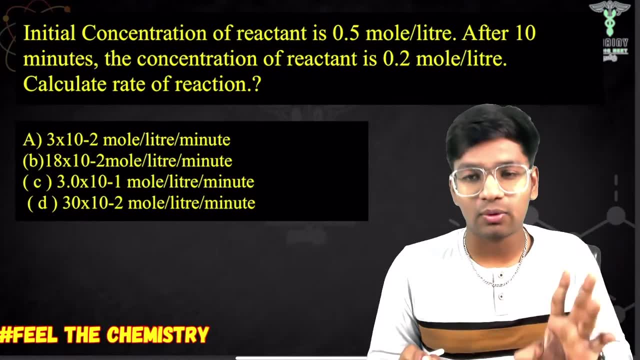 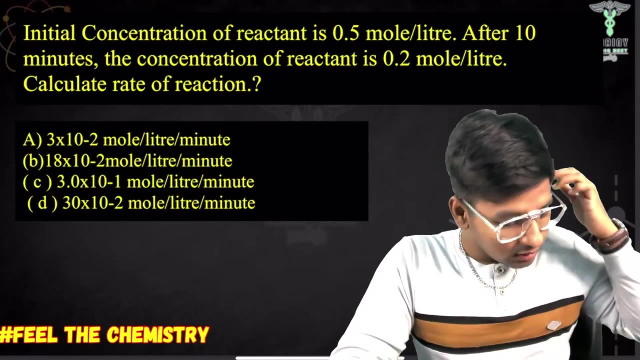 just go and watch the video, don't ask like this. there will be no questions. there will be only one statistic for physics. there will be only one statistic for chemistry. there will be only one for biology. ok, c- someone is asking: c: 10 power minus 2. 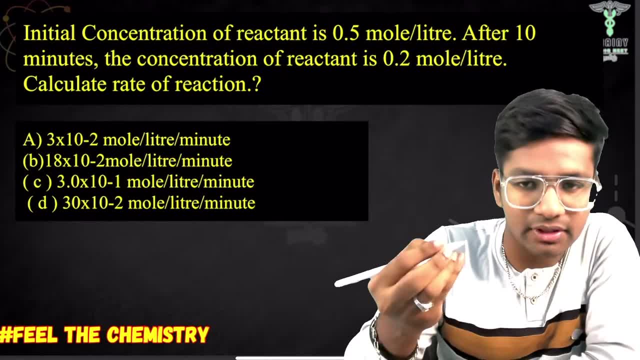 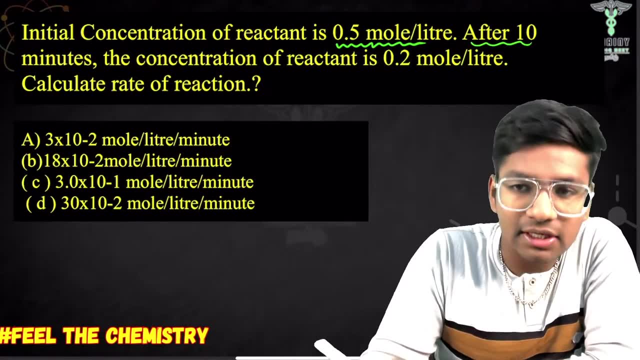 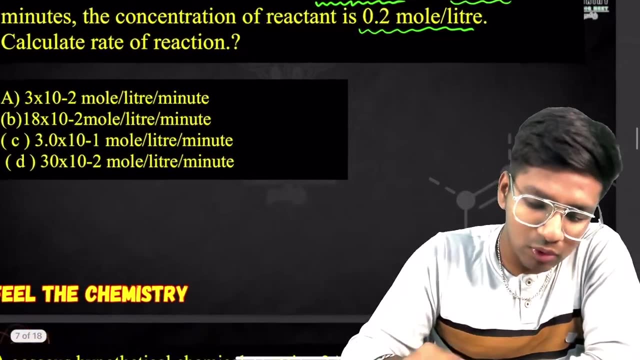 no, c is not there. probably just try this question first. they have given initial concentration- see here 10 minutes. this is final time after 10 minutes. similarly, the concentration of reactant: after 10 minutes they have given, so don't do anything. initial concentration is 0.5. 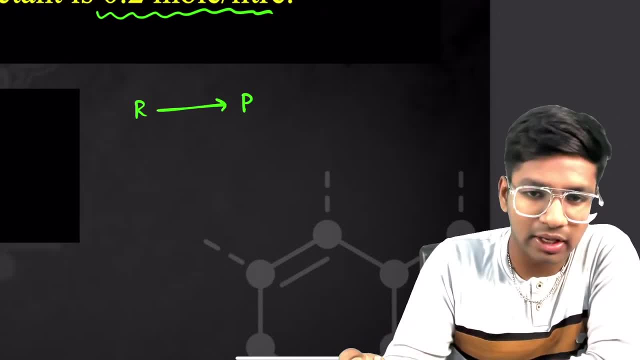 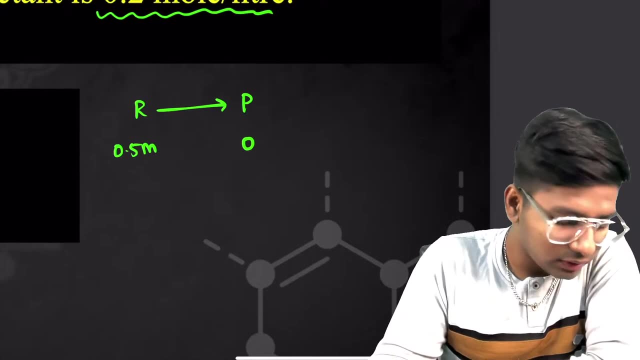 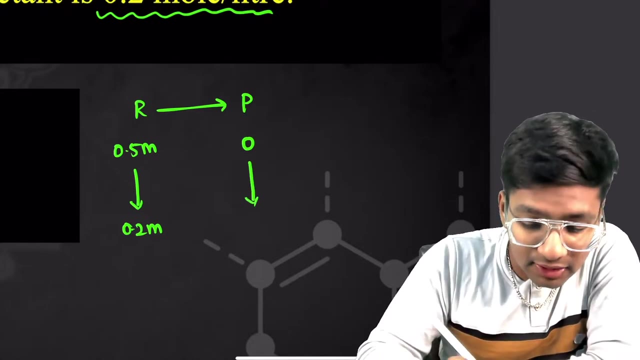 initial concentration: product goes from reactant, initially 0.5 moles, product will be 0 moles, product will be 0 moles. ok, finally, what they have given: 0.2 moles. when, after 10 minutes, after 10 minutes, rate is equal to. 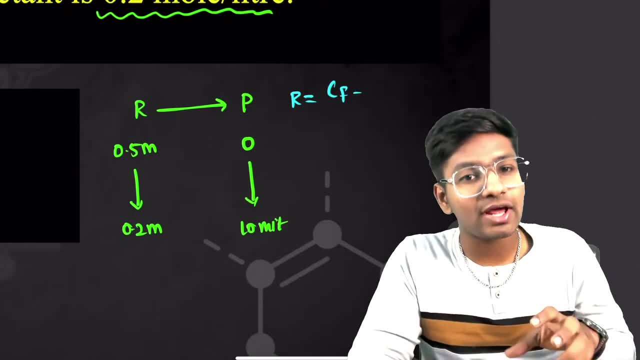 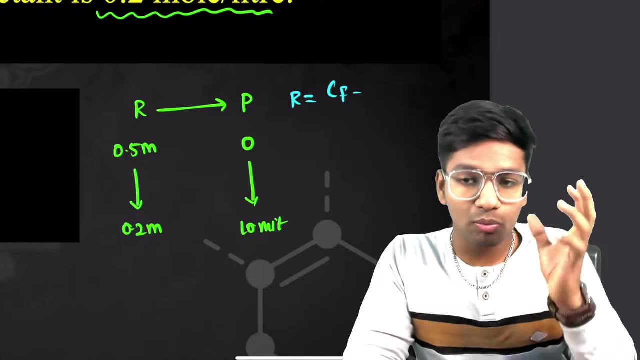 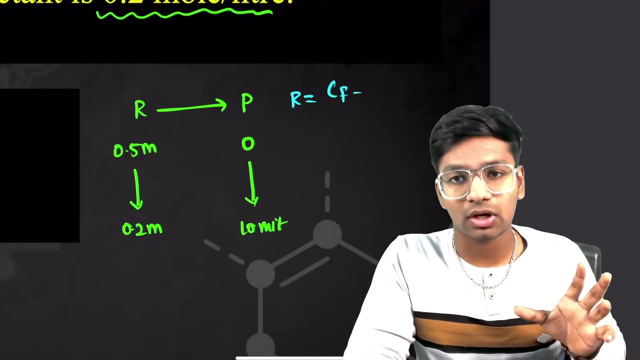 rate is equal to c, final minus. actually, here, rate of reaction is given. wait, this is rate of reaction. rate of reaction is measured for per mole. for mole, rate of reaction is measured for mole. that is why they have given rate of reaction. ok, I have not put any moles. 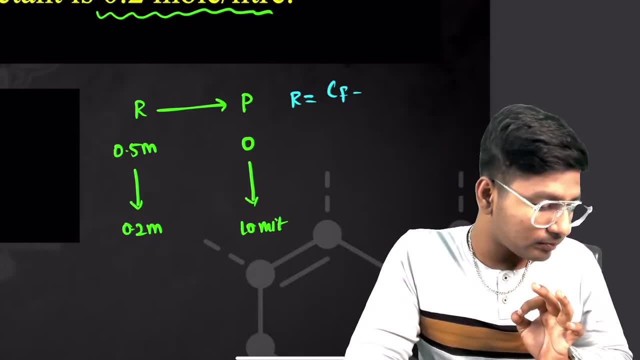 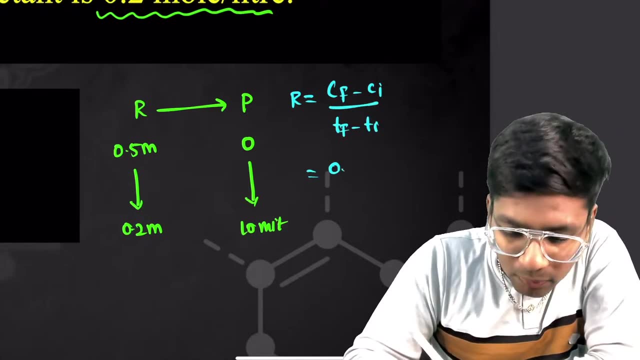 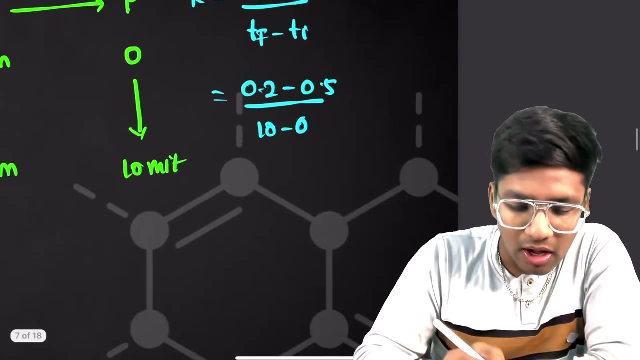 I was just measuring concentration. ok, so see c final minus c initial, divided by t final minus t initial. then what will you do? 0.2 minus 0.5 divided by 10 minus 0, 10 minus 0, then what will be the answer? 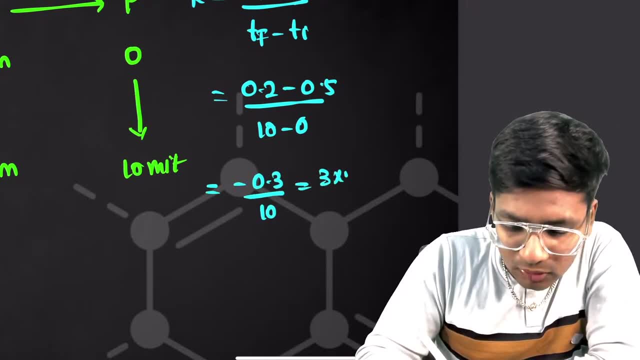 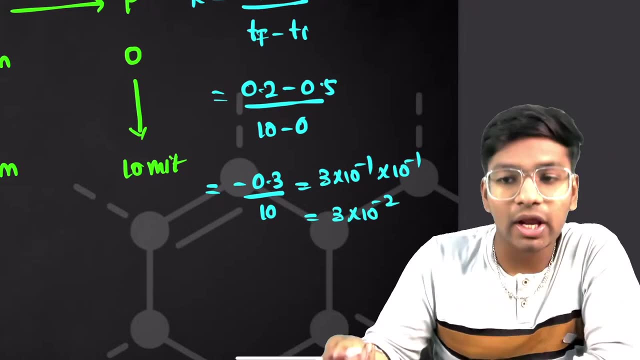 minus 0.3 divided by 10, what will you do? write 3 into 10 power minus 1, then 10 power minus 1 will change. 0.3 minus 1 will change. 0.3 minus 1 can be 0.8. 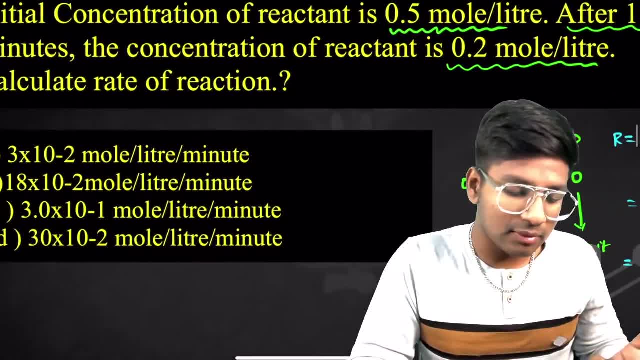 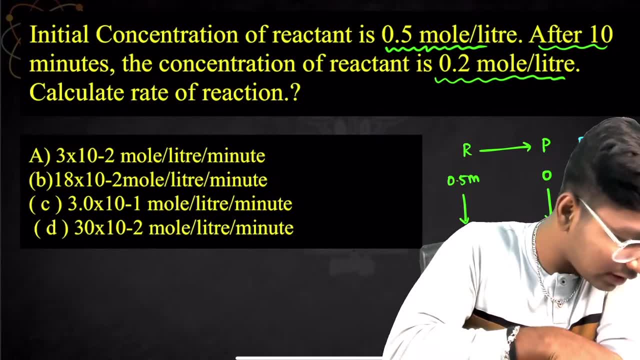 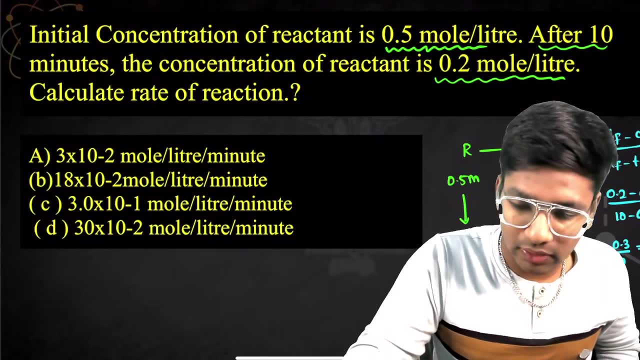 then 2 plus 1, which will be tan. so what will you do? write 1 times together, then, how many can be 0, 2 the value of punitive part, 0.3 into 3 sub radians. have, a gentlemen, 2 by 2. 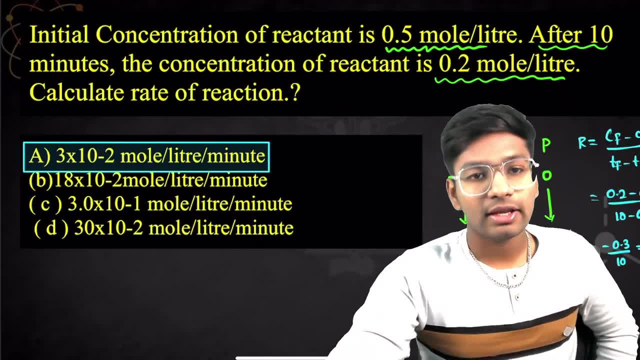 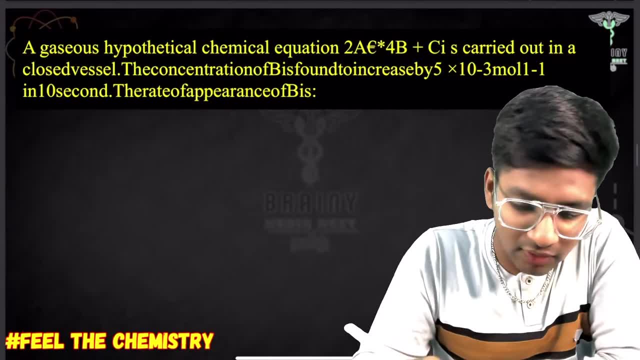 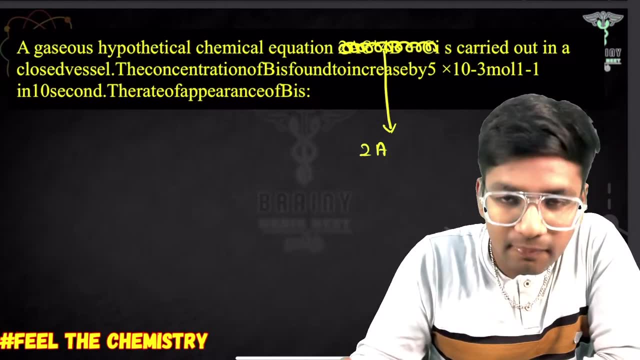 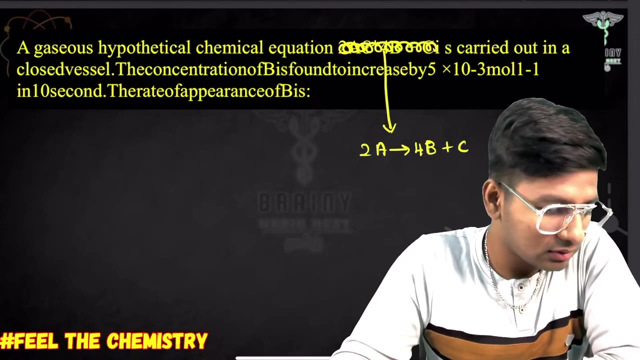 1 by 2, done, done, done. next question. next question, next question: even when they in the egress in a chain, this number, because not copy paste, fundamental over la in gail either, either achieve in: either in a banana to a gives for B plus C of the negative. oh, plus C of the negative, oh, apart from. 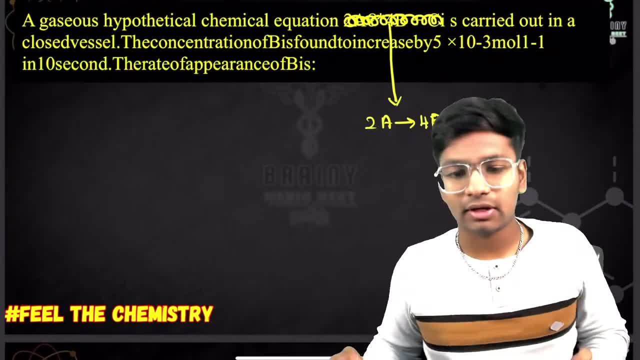 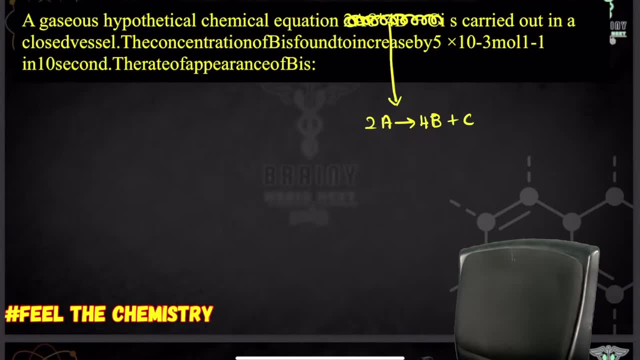 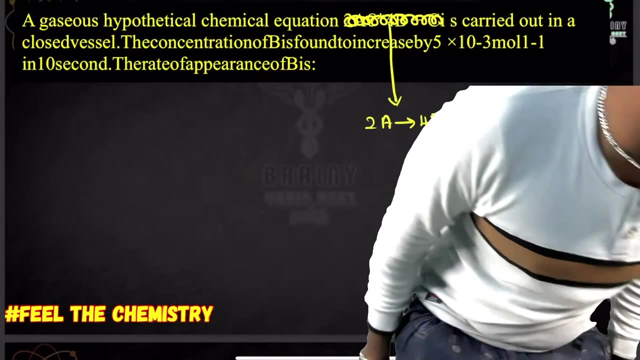 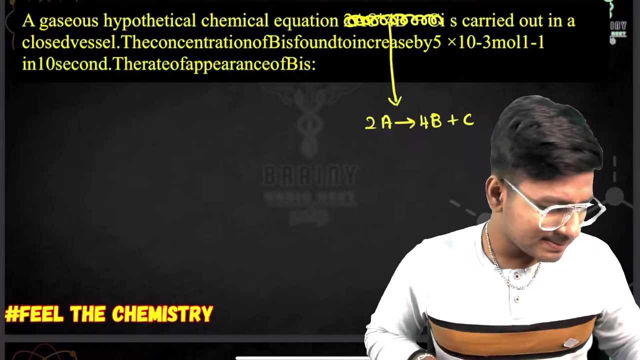 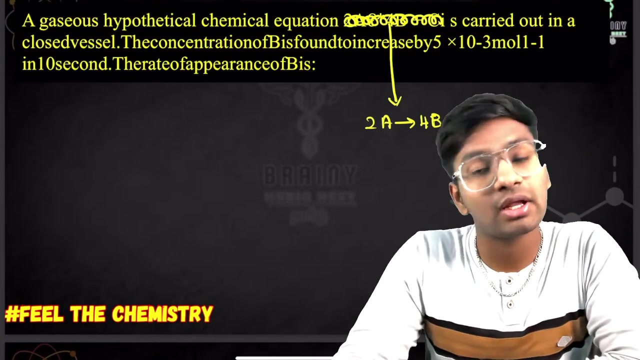 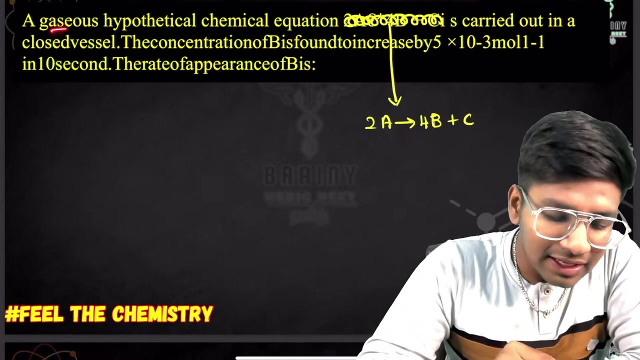 this okay, medium, a character- wait, someone is calling me one- that she is in a method, a lecture program, in a. your lecture may be in your lecture. probably I will take some more time for that, okay, yeah, first question of body: a gas is hypothetical, hypothetical. this consider. 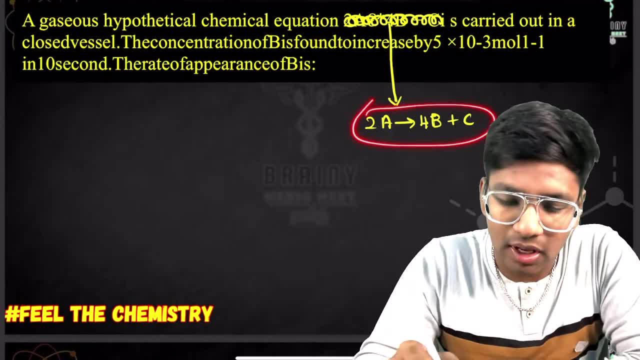 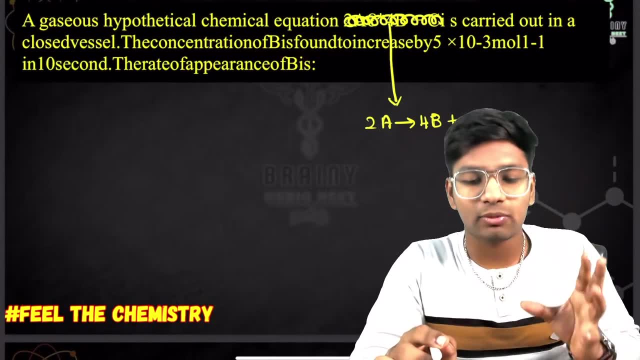 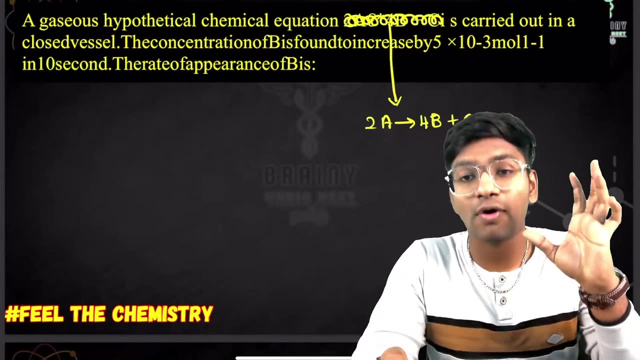 when you're gonna hypothetical equation, you may equation put it on, is carried out in a closed vessel. in closed version, the concentration of B is found to space in the middle. a conjure: manage money, go to increase by in your power only B. concentration of B is found to increase by no. 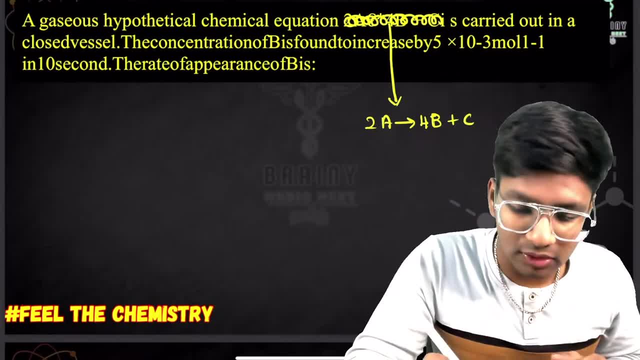 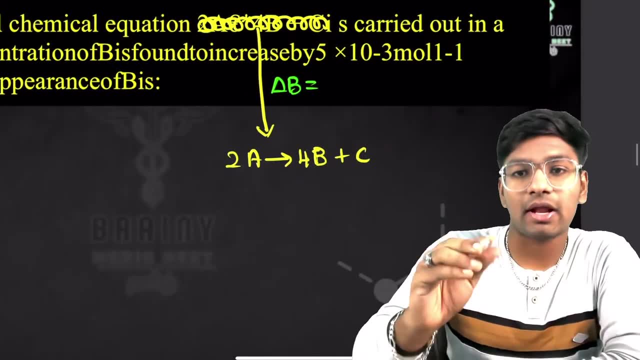 value. put the RUG ANGEL IN A dreamer. oh, my director, change in. we put the tongue. delta B is given them another. Delta B is already given a more. never not a change in concentration or concentration of B is found to increase. because, yeah, in the 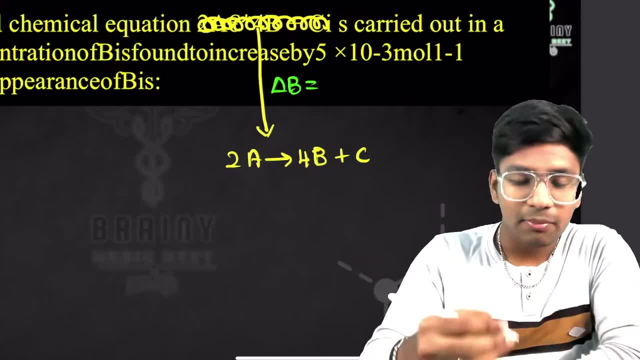 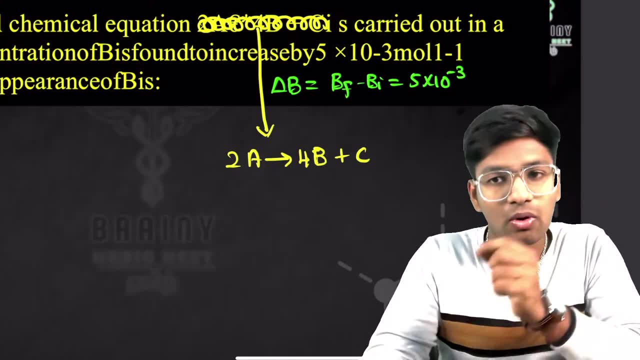 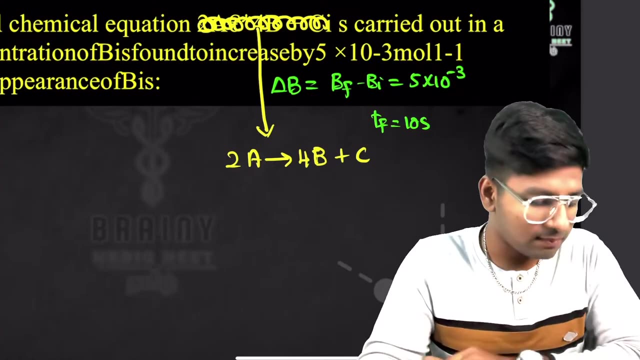 similar to be in the same that the B increase the correct, but delta B, another B final minus B initial is equal to 5 into 10 power minus 3 of mocca tar and in 10 seconds the time time in the final time, t final, is equal to 10 seconds. just put answer, put answer. put it r b. 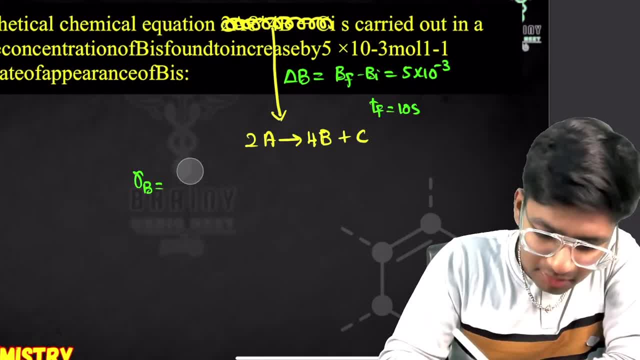 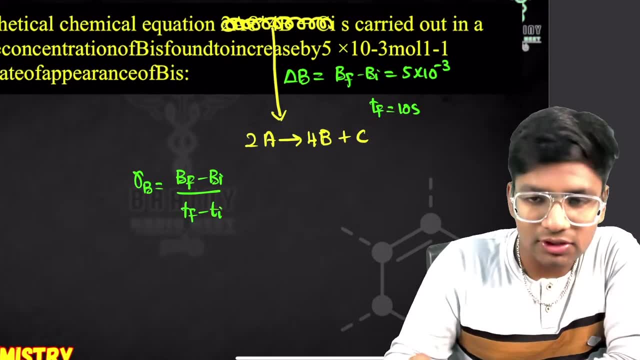 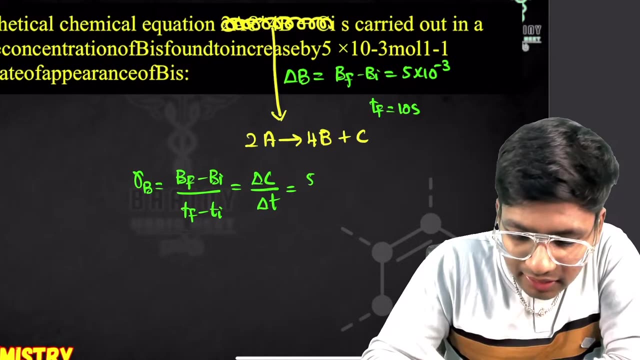 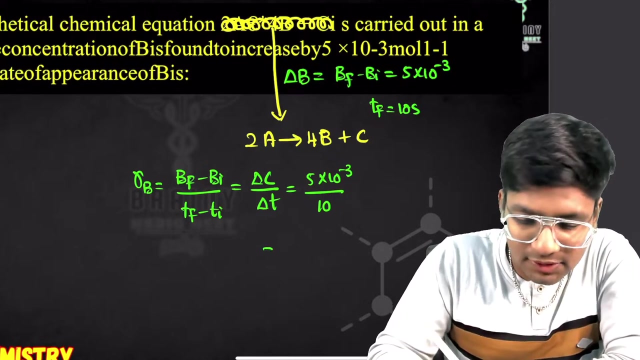 is equal to c final concentration, b final minus b initial, divided by t final minus t initial, so which is equal to delta c by delta t. so 5 into 10 power minus 3 divided by 10 seconds, put answer directly: put 5 into 10 power minus 4. 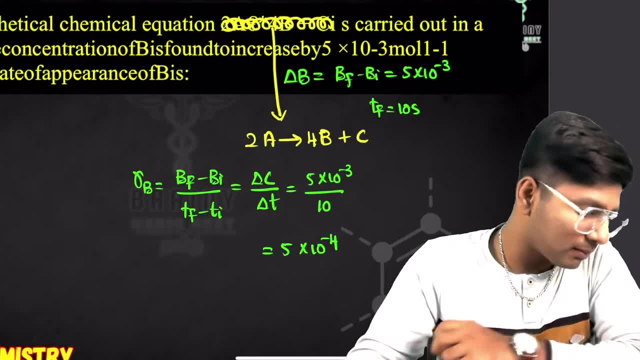 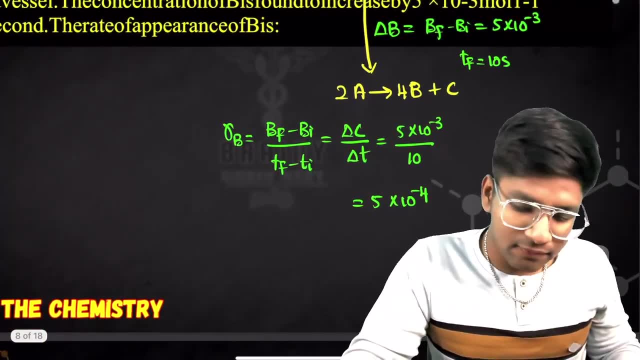 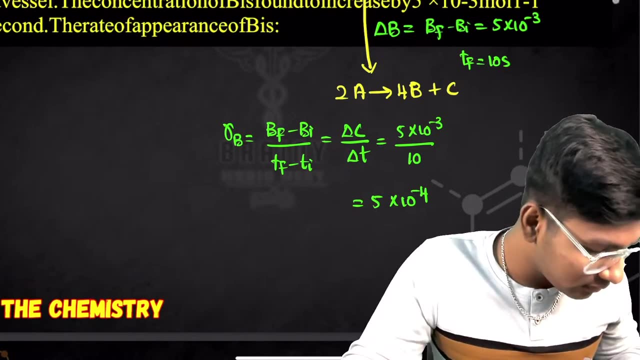 ah, super, madhu mitha, madhu tamil, neat aspirant. many have got answer, i think so in a half half into 10 power minus 4, how did you get ganesh? but the hunter will come. that day the hunter will come. what hunter will come? 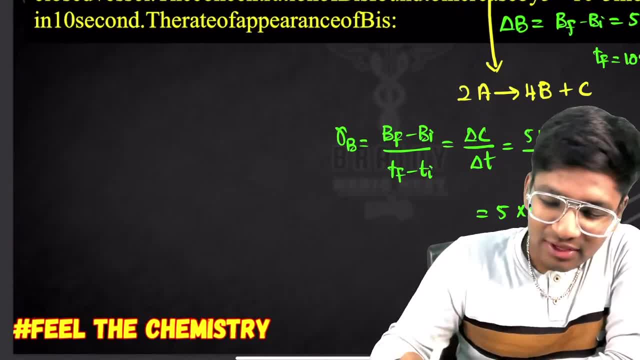 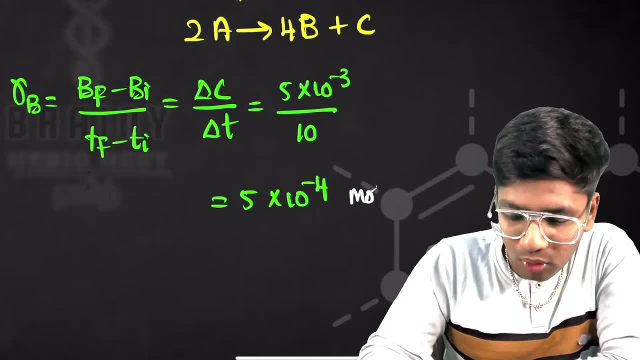 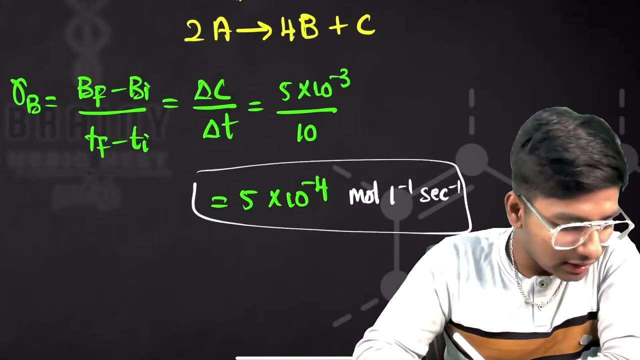 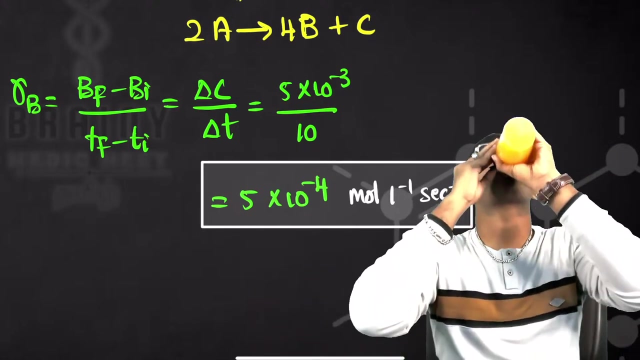 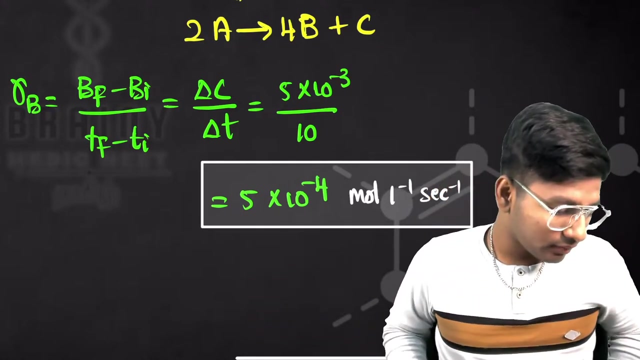 oh, hunter, oh that day in organic chemistry. so this is your answer. ok, i forgot to put unit unit. unit put unit mole liter inverse, second inverse. done, done, done, done, done, done. anyone has any doubt about this? if you have any doubt, tell me. ok, ok, ok, ok. 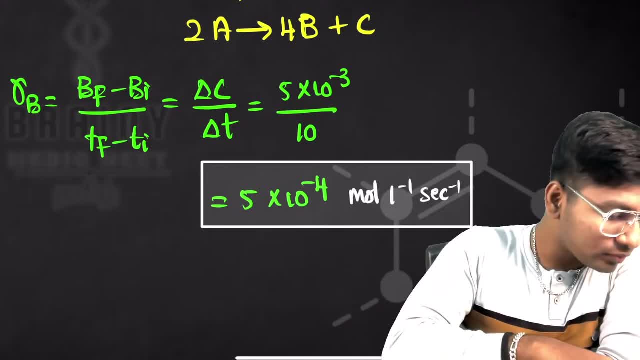 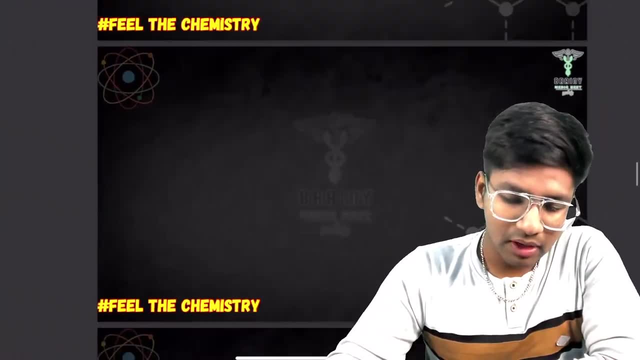 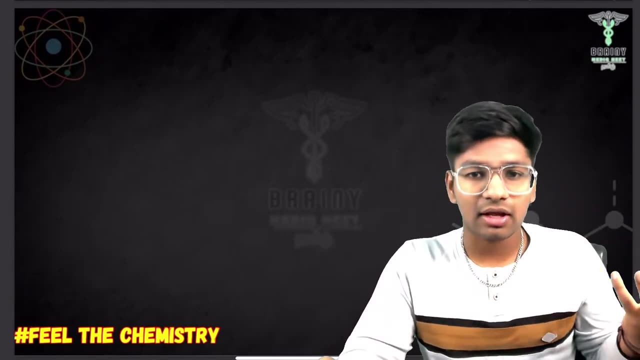 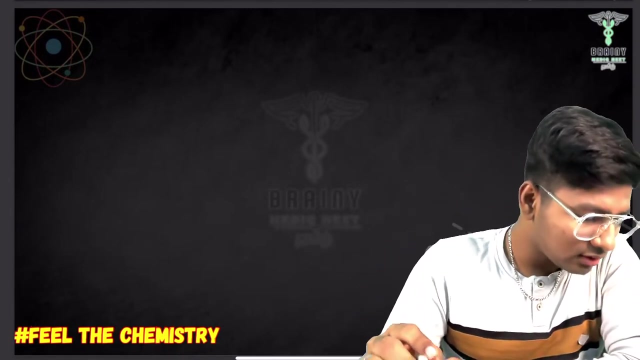 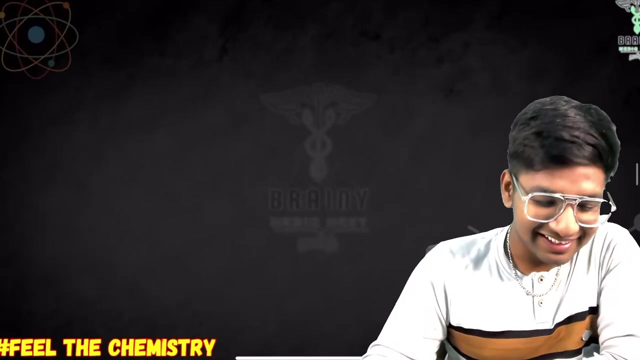 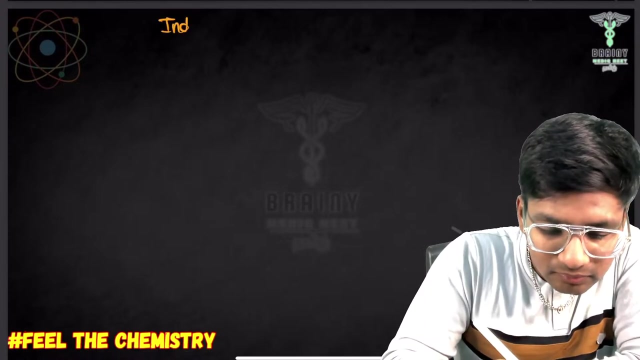 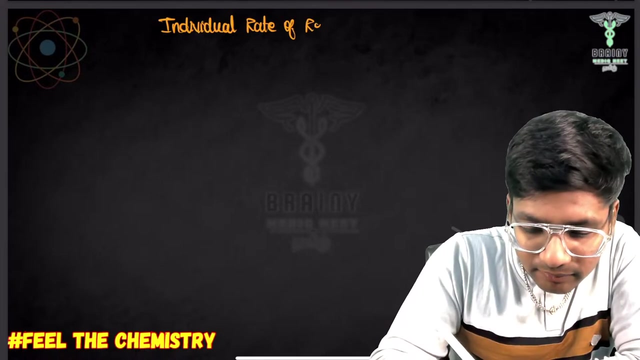 ok, yes, yes, there is, your comment is visible. ok, next let us go come. we are going to other concept here. i am going to write most of the questions written because i am not knowing how to type reactions. i have done all ok now, so ok, ok, ok. 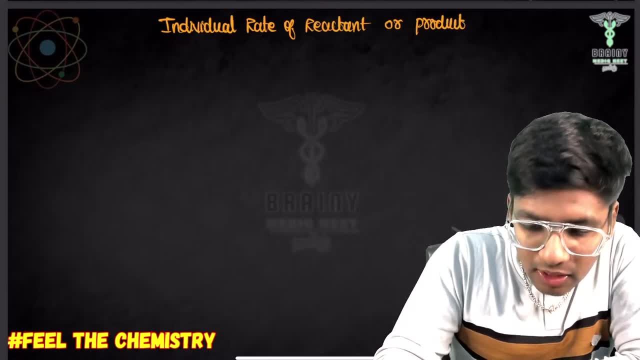 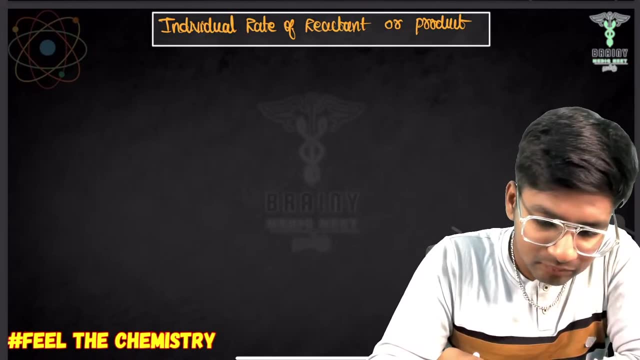 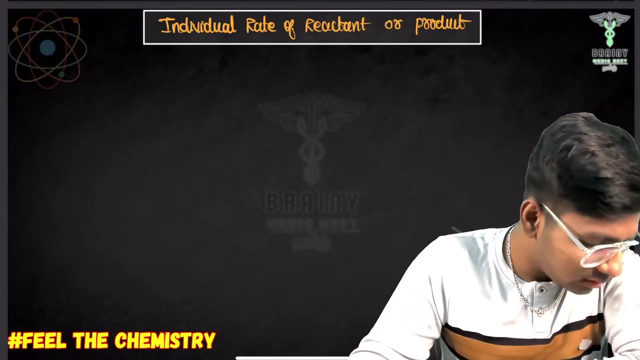 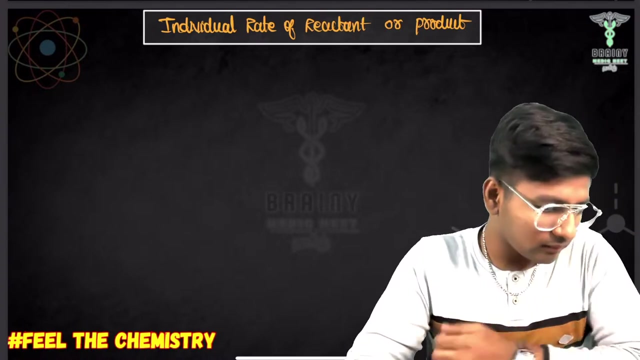 now one would say, ok, so. So I am going to define the rate of B separately. I don't understand. How did you find the rate of B? by looking at the question, The water has turned orange. The orange has turned yellow, Wait. 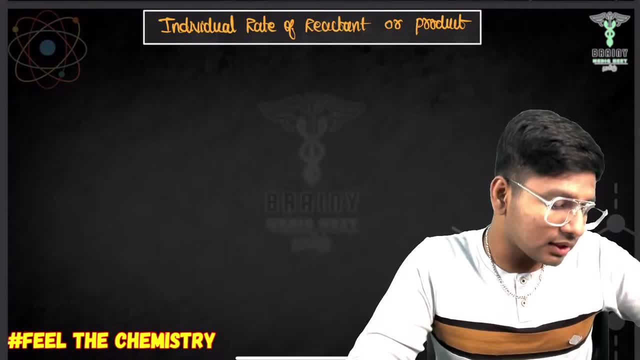 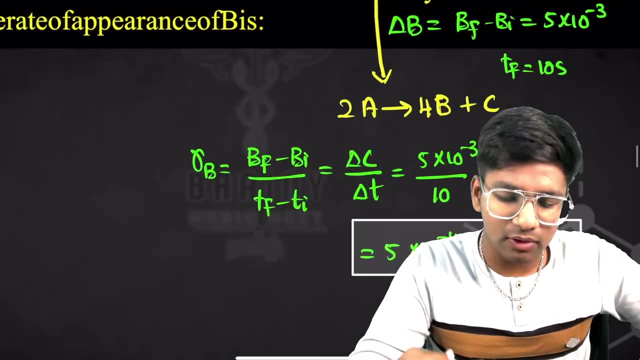 Someone is asking a question. How did you find the rate of B? by looking at the question. Look here. They have asked the rate of appearance of B. Why did they give appearance of B? Because here the water is more and here the water is less. 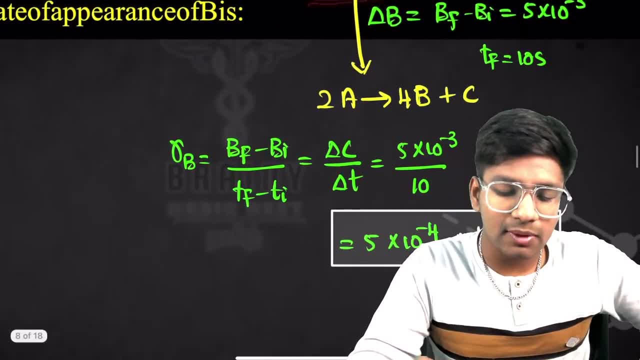 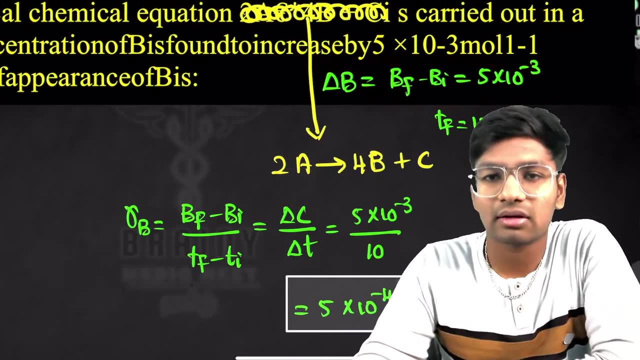 That is why they gave appearance of B. Look here: Increase by. Why did they give increase by? Because here the concentration will be increased for B. That is why they gave increase by. They have given everything directly in the question. Nothing is complex. 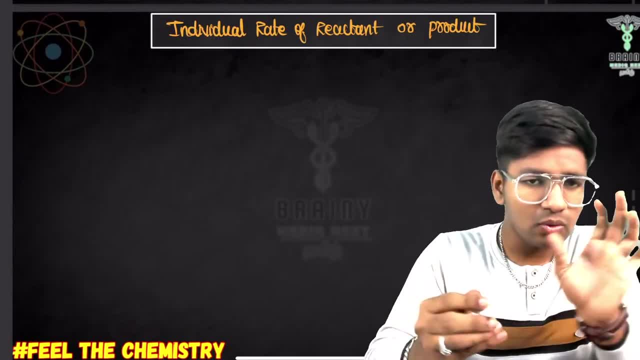 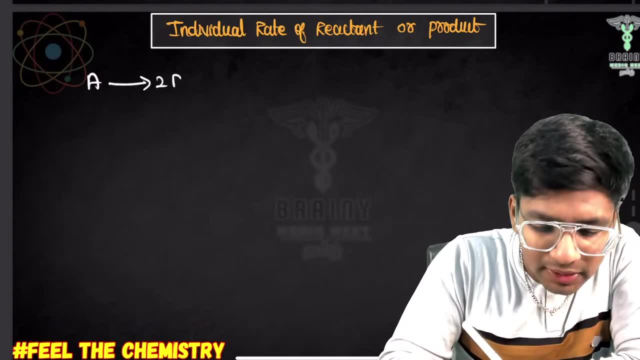 Okay, So look at the next one. Next one: This is a small explanation. This is a small explanation. A gives A gives, A gives 2B. Okay, A gives 2B. At time t is equal to. 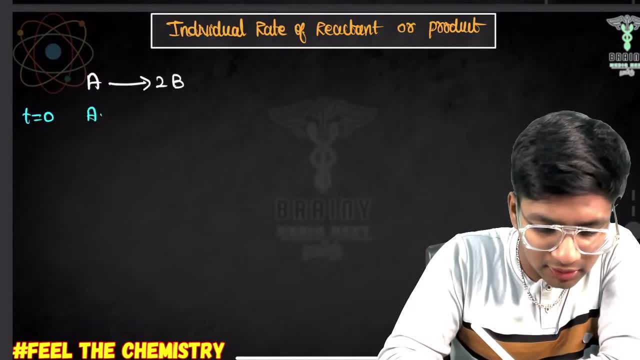 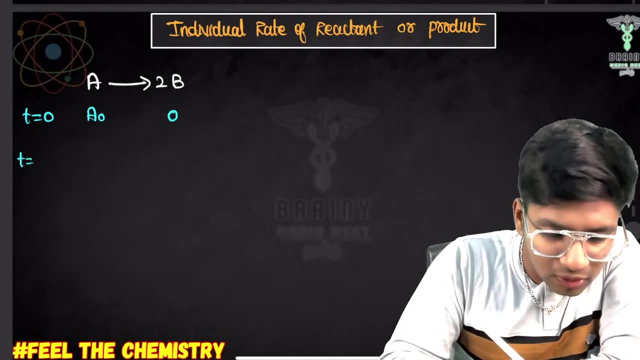 Time t is equal to 0.. A is equal to A0.. Again, B is equal to 0.. Because That is when the reaction starts, Then time t is equal to In t seconds. In t seconds, What happened? 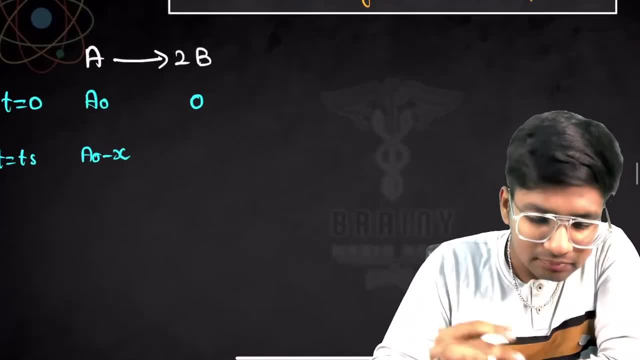 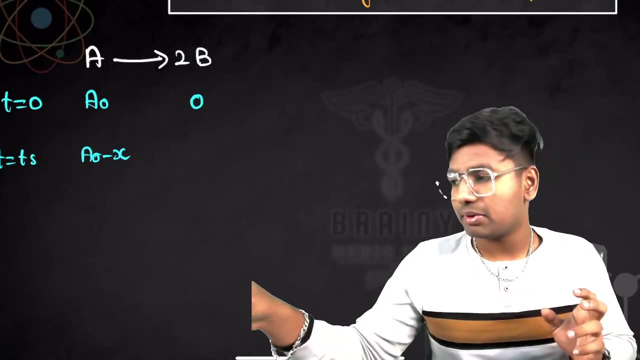 A0 minus x happened. What will happen? What will happen to B? Someone answer it quickly. Someone answer it quickly: B, B. What is B, B, B, B. Say it quickly. What will happen to B? What will happen to X? 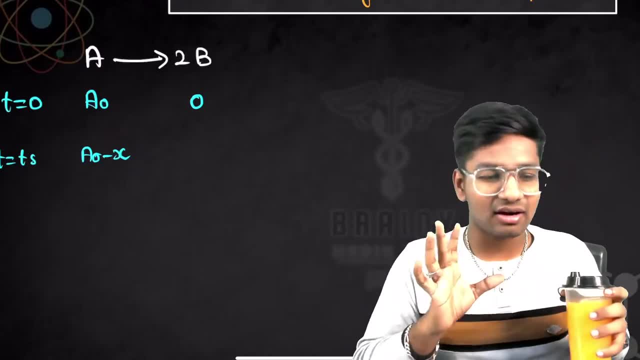 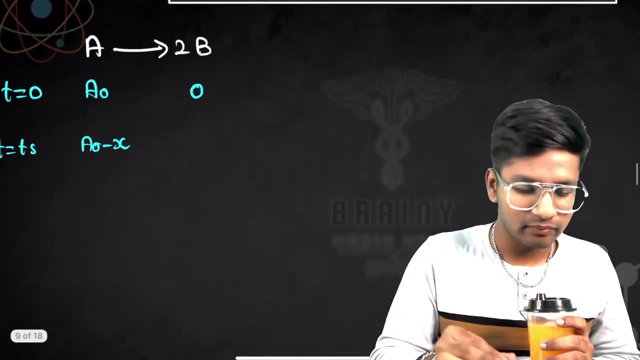 A A Akhila. Very nice, You are on a right path. Did you see How many people are making wrong answers? How many people are making wrong answers? For example, There is a girl. She has already. She has already. 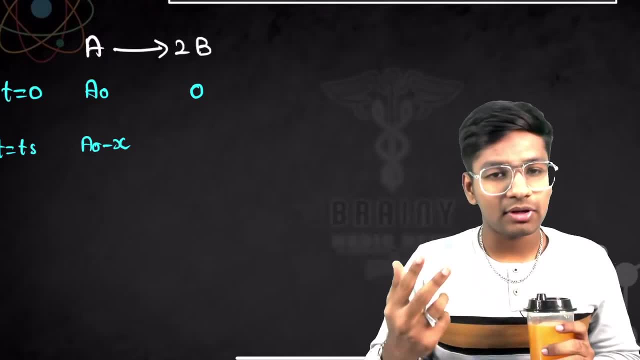 Already 2 pairs of shoes. Already, there are 2 pairs of shoes. Already. there are 2 pairs of shoes. Already. there are 2 pairs of shoes. moon, are they not on the diagram? you put that with it and I didn't. 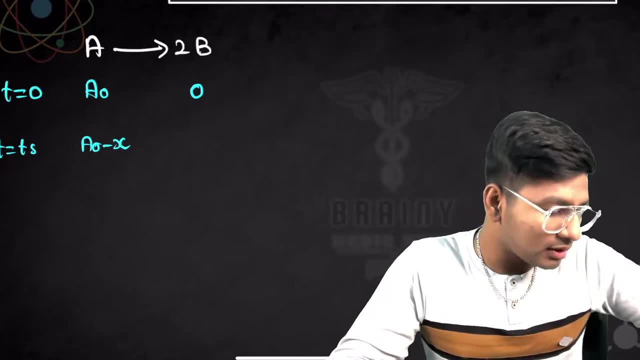 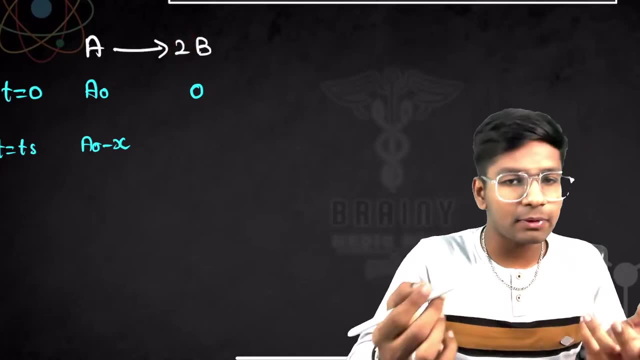 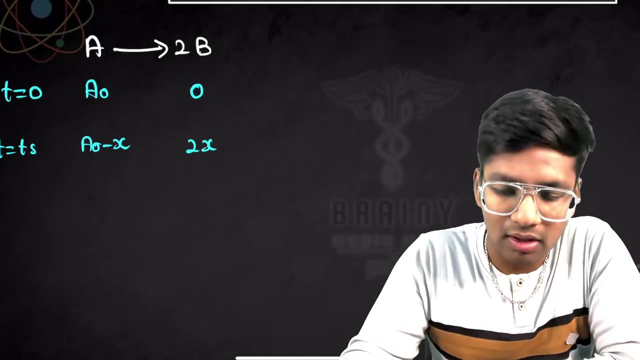 it's by do not only a pretty little mood a little up, or in the earth on a coefficient to a children, correct? ah, in the render on the X of a two X on our 2x. okay, log is in ionic equilibrium, okay, so 2x is the answer. 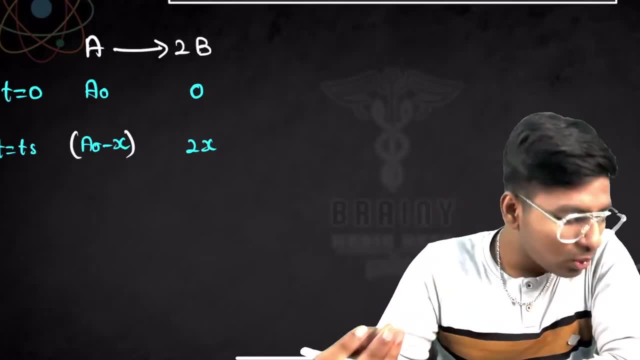 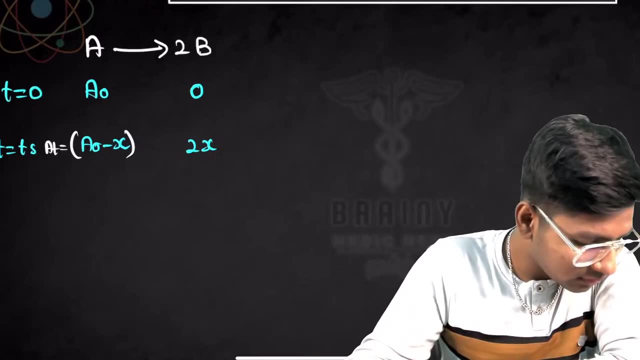 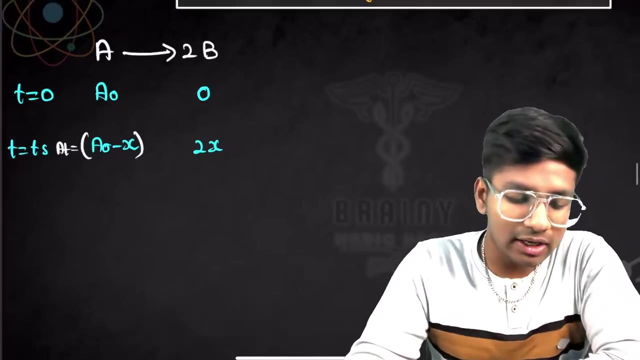 in this place, correct moles, coefficient. who will multiply coefficient? who will multiply coefficient? so this is your A t. okay, this is your A t. after time, t. what happened? A t, A, t, A t? initially, there was A naught. so what I am going to do with this? first, I am going to write A rate of 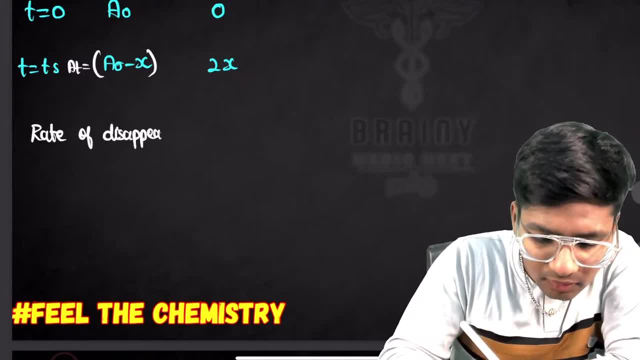 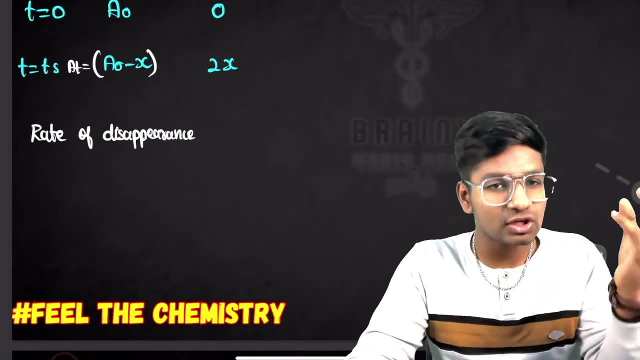 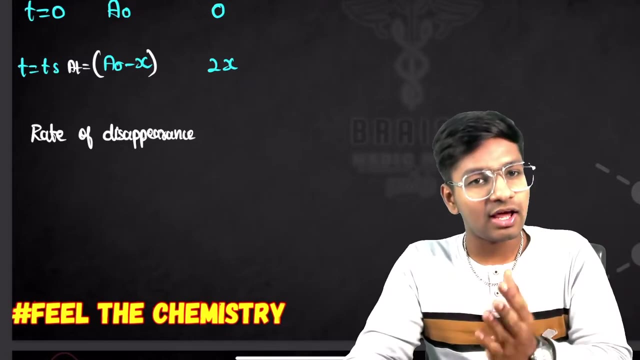 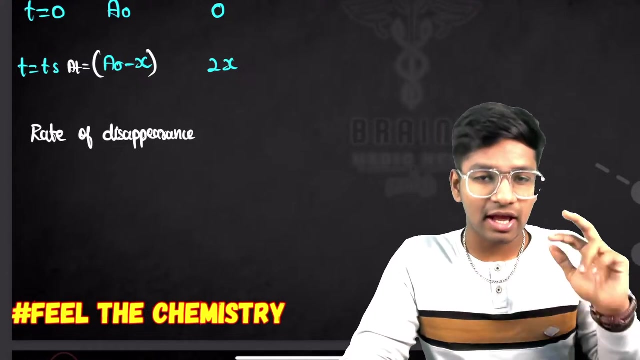 disappearance, disappearance. why disappearance? because reaction proceeded. in this place, energy will be reduced. correct like this: because of relationship proceeded during valentine's day, for boy money will be deducted and for girl money will be deducted. remember that. okay, if reaction proceeds, If the girl says ok, then the boy will have less money. 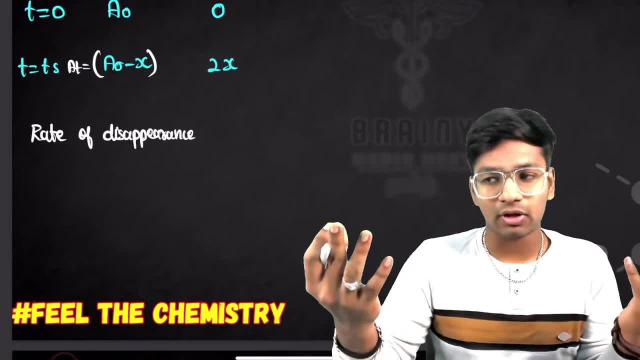 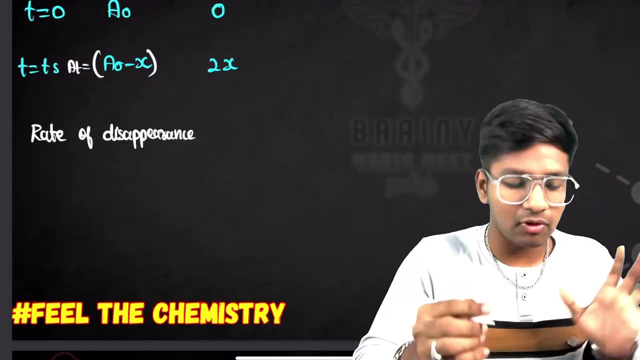 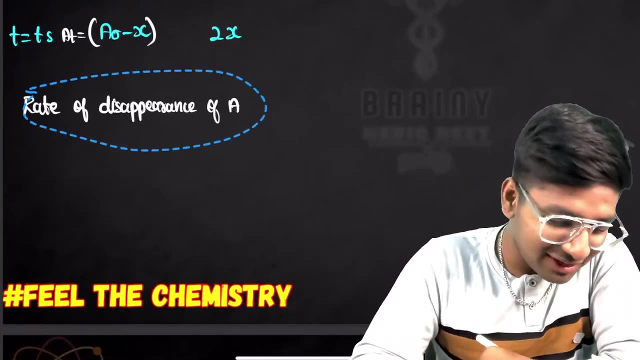 Similarly, in this case, A is the boy and B is the girl. The girl is buying and the boy is giving. Simple, Ok, Keep it simple. Rate of disappearance of A. In the end he will disappear, That's it. He will lose his life. Don't be like me. 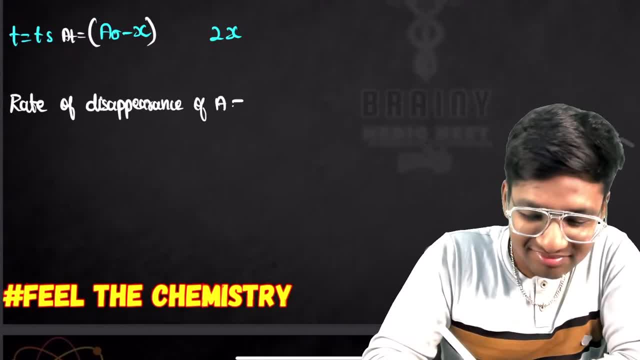 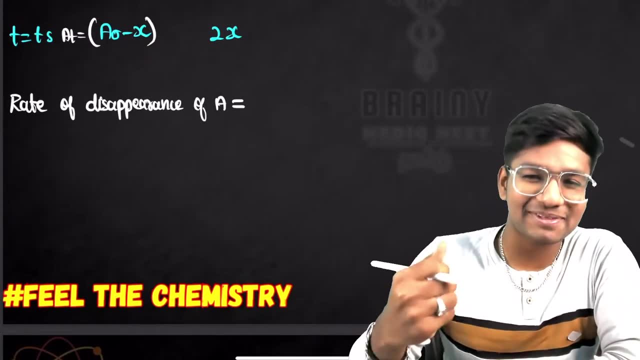 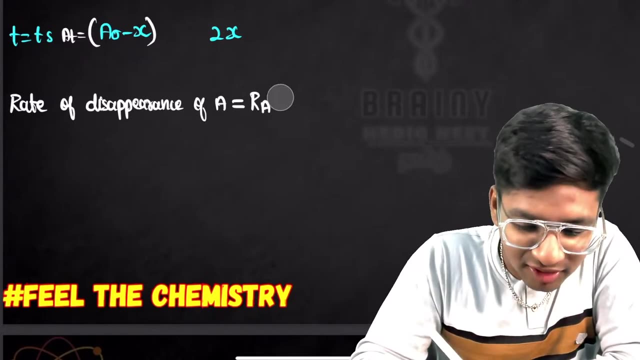 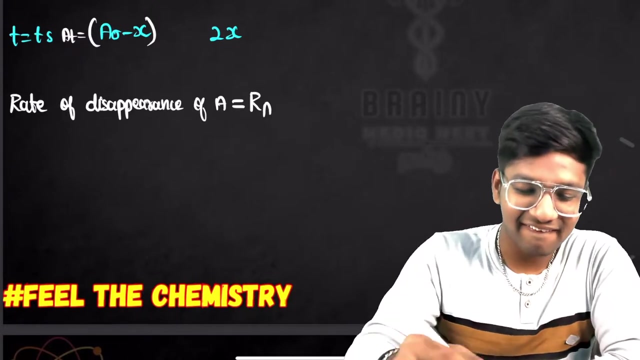 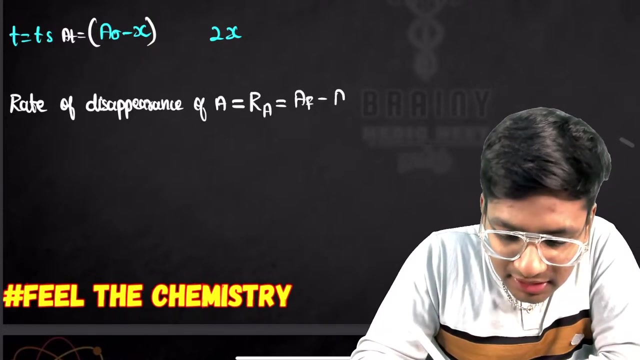 Ok, So Supporting the boys, Of course, boys are the ones who have suffered. Boys are the ones who have suffered. I will speak for the boys. Who knows how much we have suffered? Riyaz will speak for the boys. I have written RA. So A final minus A initial divided by 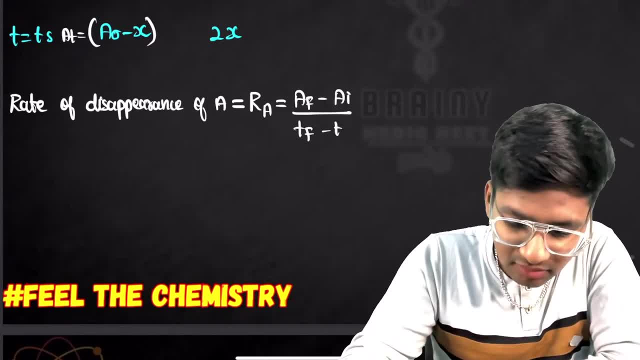 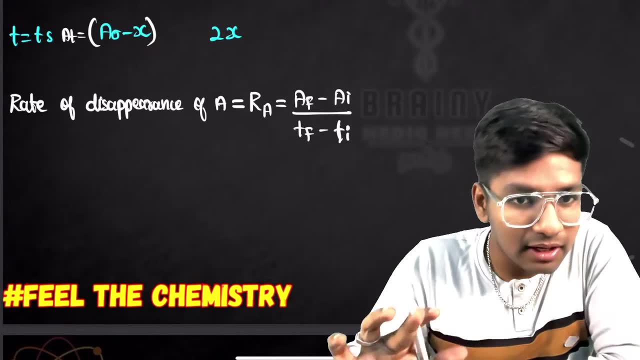 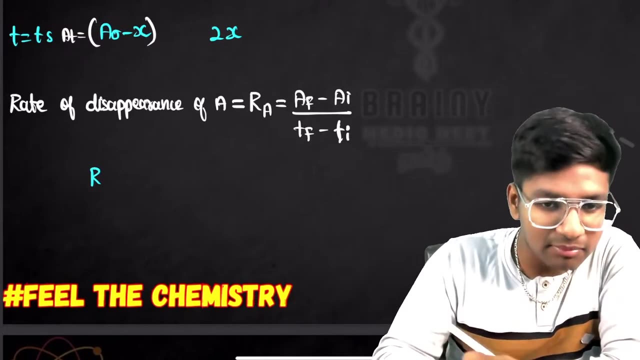 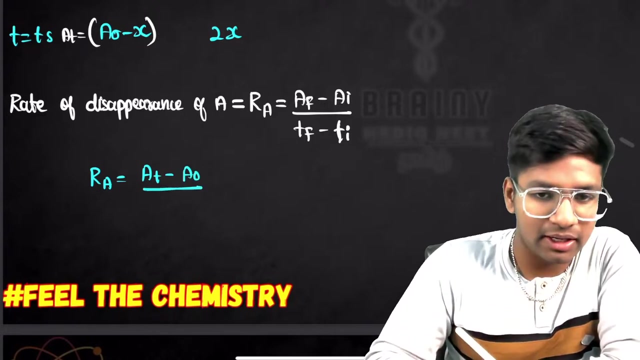 T final minus T initial, T final minus T initial. I have written. What am I going to do now? See, No one should be afraid. I have written it, Ok. Ok, No one should be afraid of what I have written. RA is equal to AT minus A naught divided by. 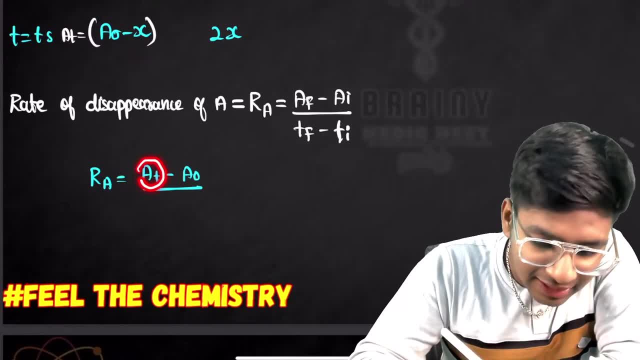 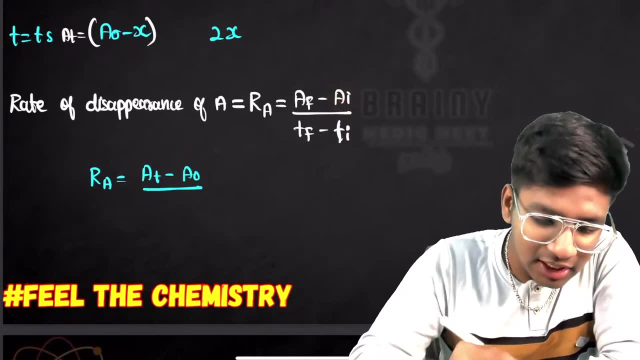 T. I have written it simply AT What is AT At time. T. I have written AT as A final. I have written A initial as A naught. Ok, I have written A initial as A naught. Correct And time of our final time: T and 0. 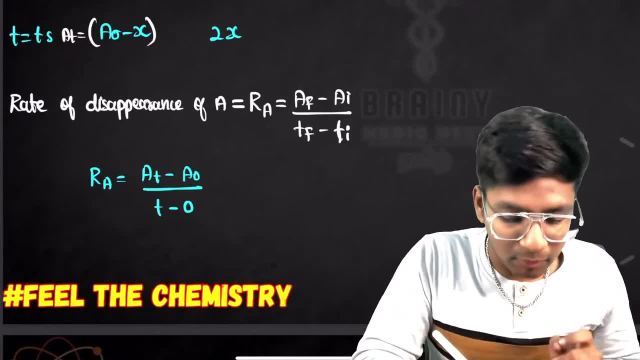 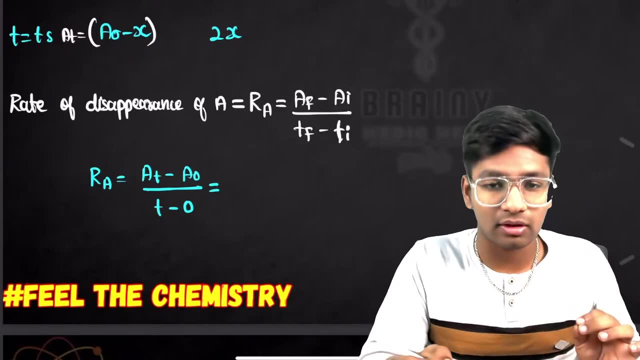 I have written. No one has any doubt in this. What am I going to do now? Don't be afraid, I am just substituting. Don't get confused. Please don't get confused. There are many people I will be sitting confused without knowing the math. Ok, I am going to substitute AT here. 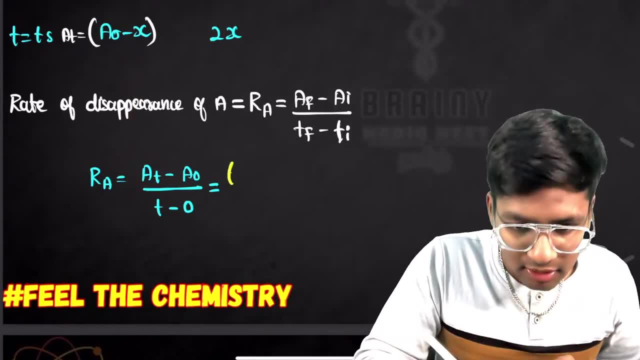 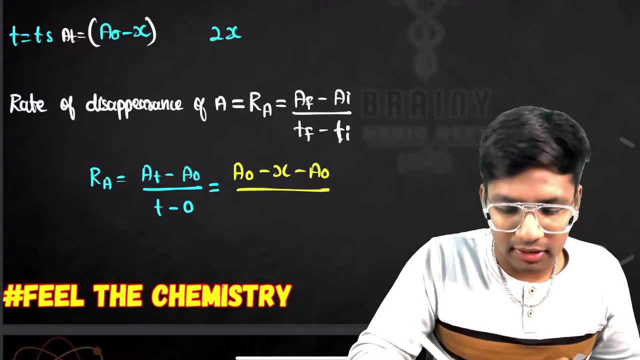 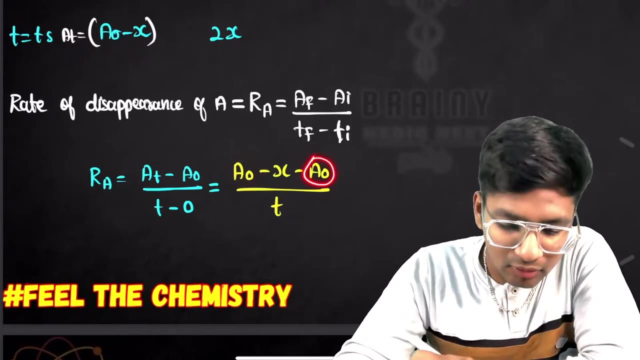 I am going to substitute AT Ok. So see A naught. A naught minus X, Minus of A naught Divided by T. Ok, Ok, A naught minus of Ok, If I subtract A naught minus X with A naught, What will I get? 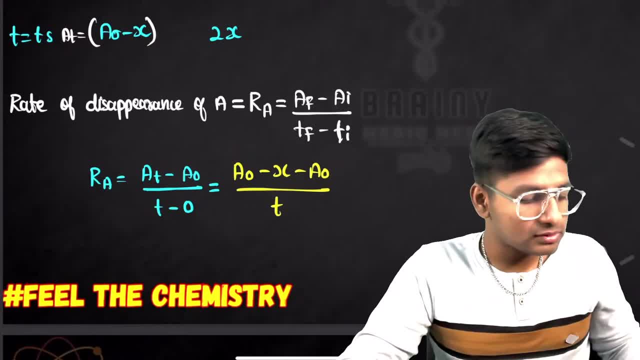 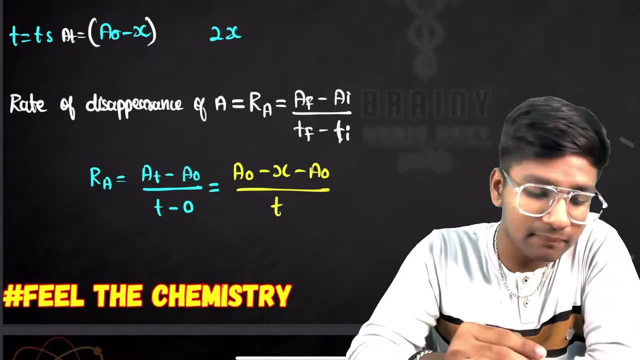 What will be the answer? What will be the answer? Tell me quickly What will be the answer. What will be the answer for this? What will be the answer for this? Minus X by T. What is it? Minus X by T? 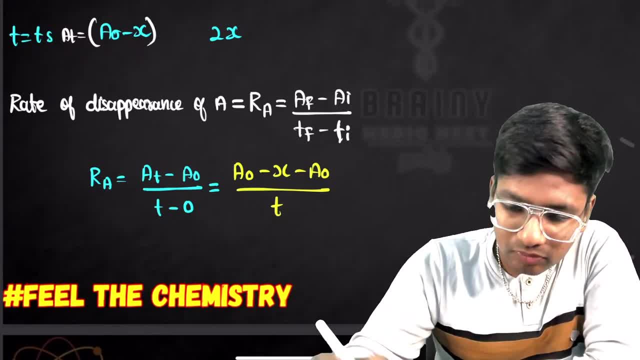 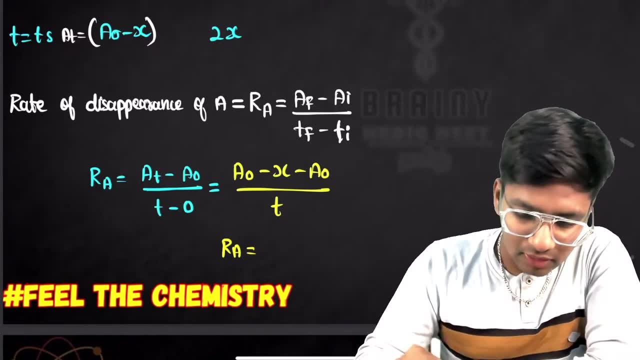 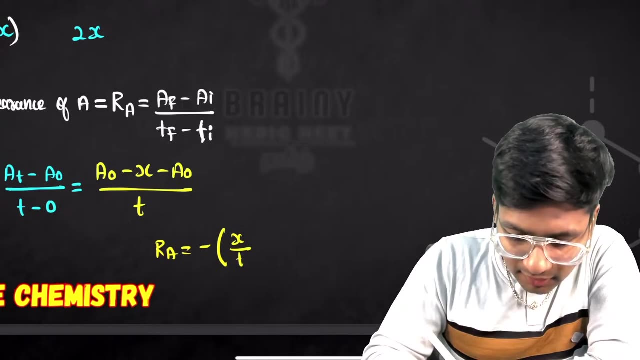 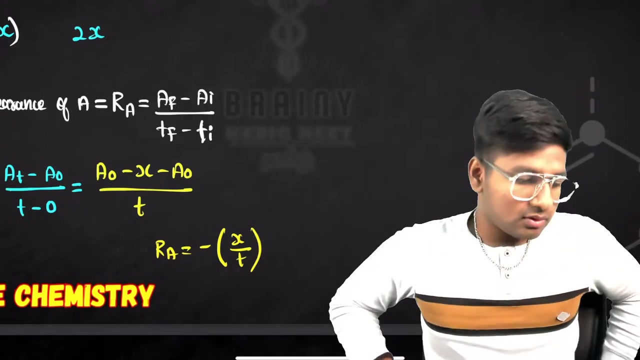 RA. RA is equal to minus X by T. Let me write this side correctly: RA is equal to minus of X by T. Rate will not be minus. Rate will not be minus. I meant that the rate won't be minus. Is this correct? I meant that the rate will not be minus. 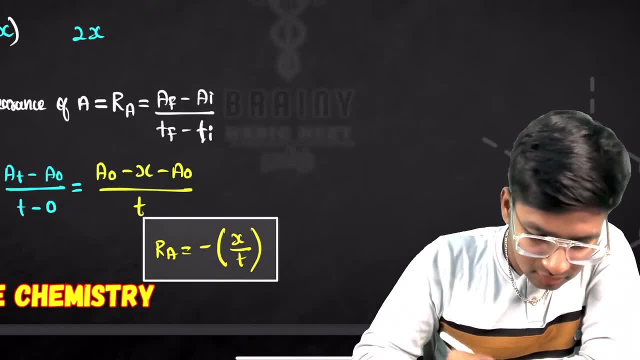 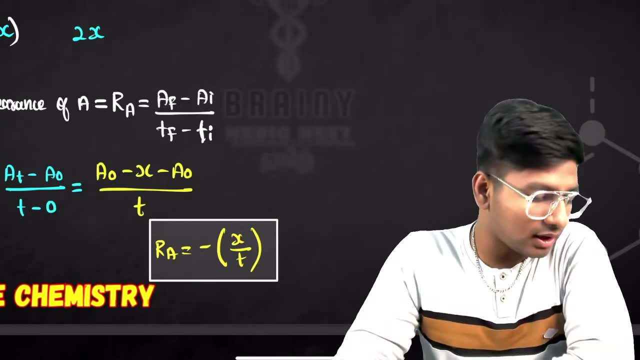 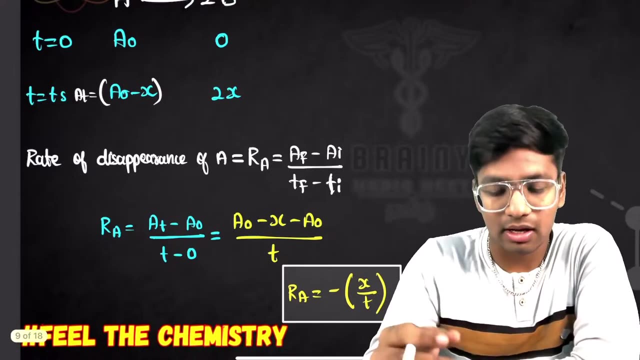 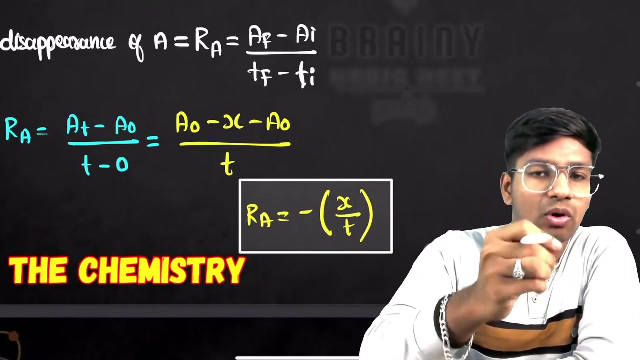 Why is it minus here? Why is it minus here? Why is the rate minus here? Explain why it's minus. So the rate should not be minus. Is this correct? I pulled here Reactor, Reactor Jadi: Reduce, Disappears, Reduce. If I had done it, I would have gone by saying that it should be negative and the disappearance should be negative. 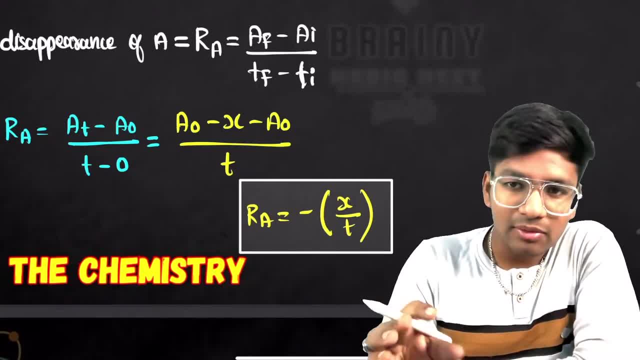 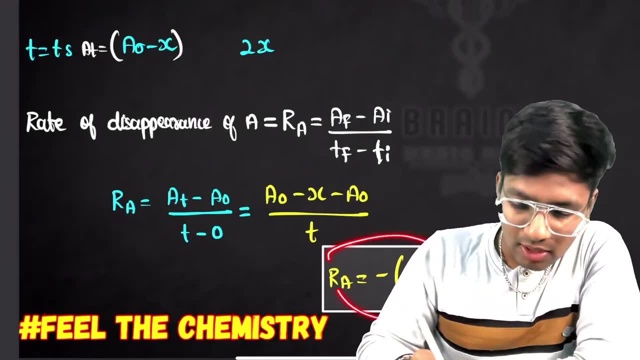 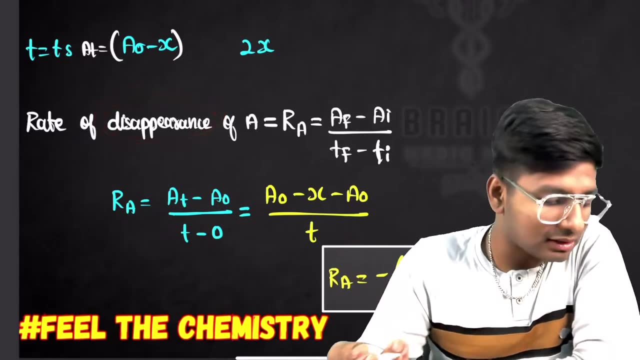 What I am saying is: this will only decrease If it decreases. you can write minus, But I have proved it to you. Have I proved it? Why does it become negative? I have proved that it becomes negative because there is a decrease and disappearance here. 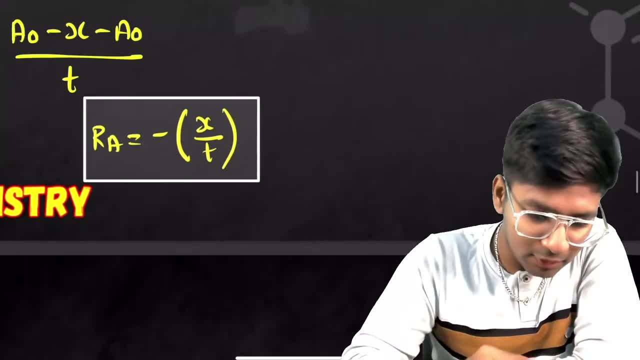 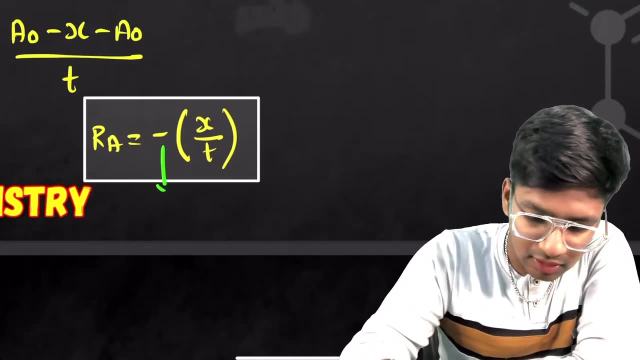 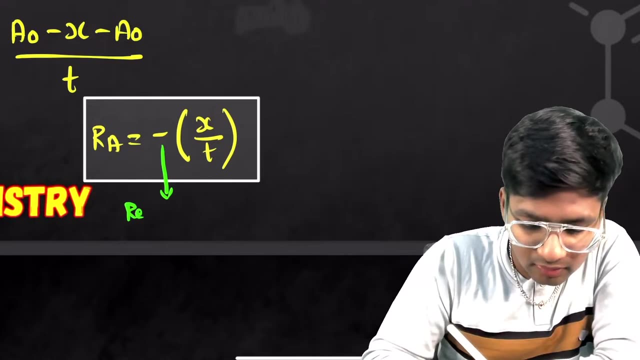 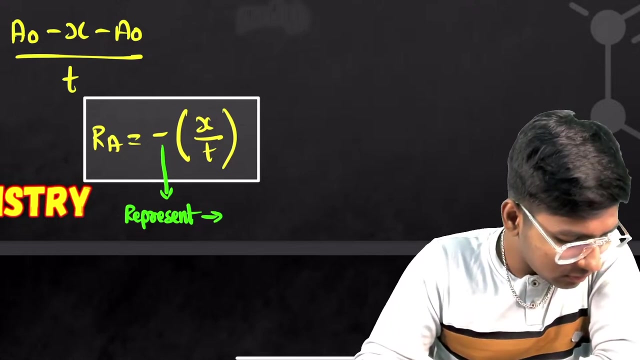 Next I have to prove the appearance right. For negative, I have to say the reason. If I write it here, the notes will be incomplete. So represent the: How much is your college fee? 8.5, around 8.5.. 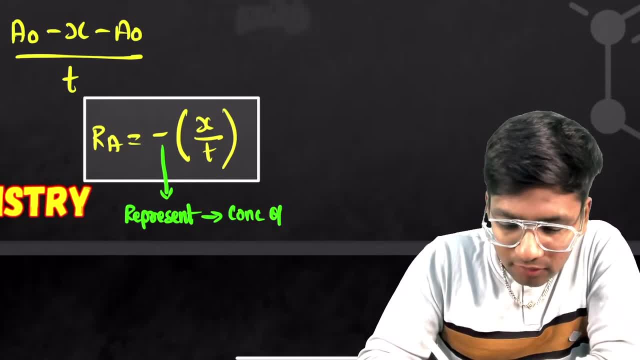 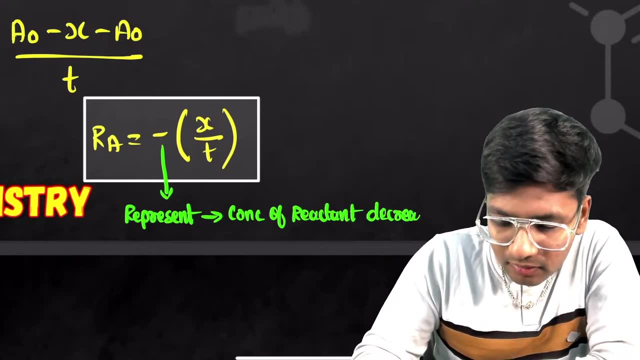 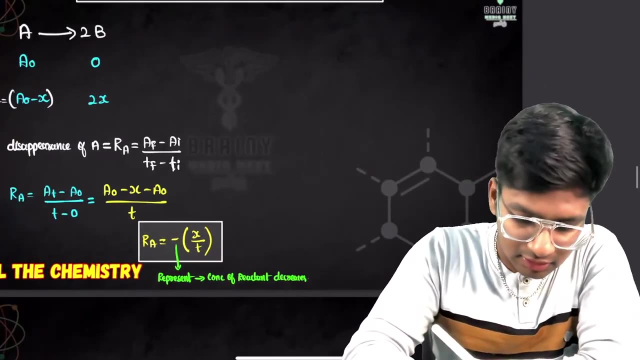 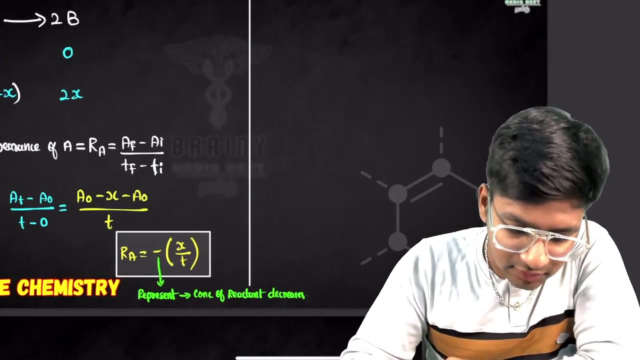 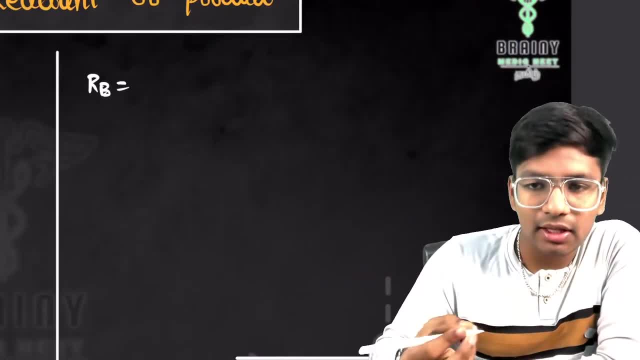 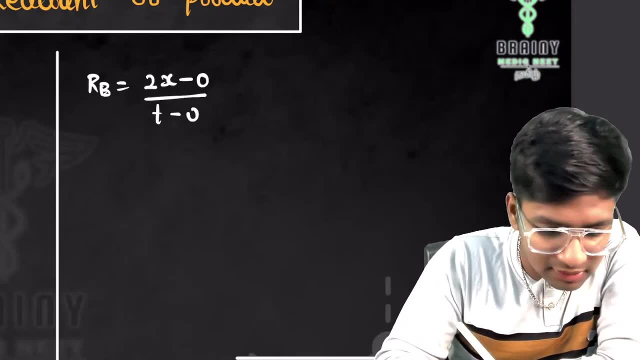 Next write Rb. Write rate of B. Rate of B: 2x is final. Final is 2x. Initial is 0, divided by final time, t minus 0.. Okay, So what will we get if we subtract this? 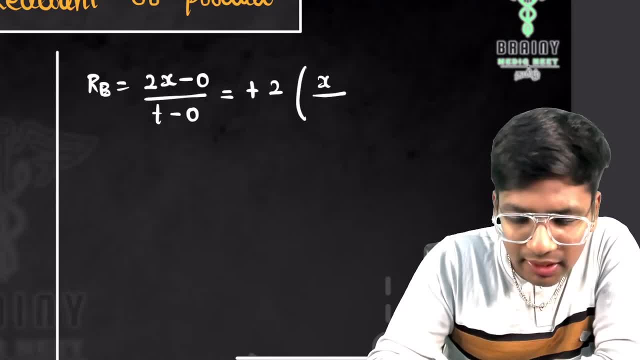 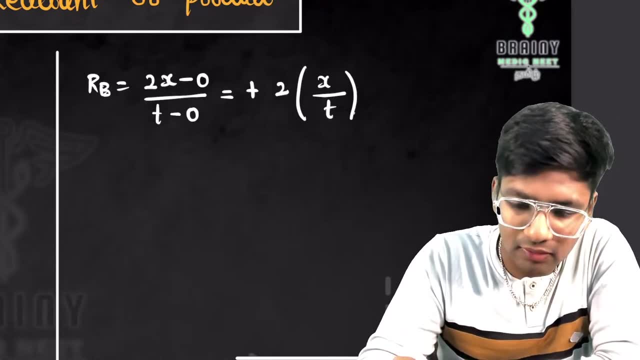 Plus 2 into x by t. Plus 2 into x by t- Oh, I have written 2 here, That's right- Plus Who has donated? Sorry, who has denoted? It is not donate, It is denote. 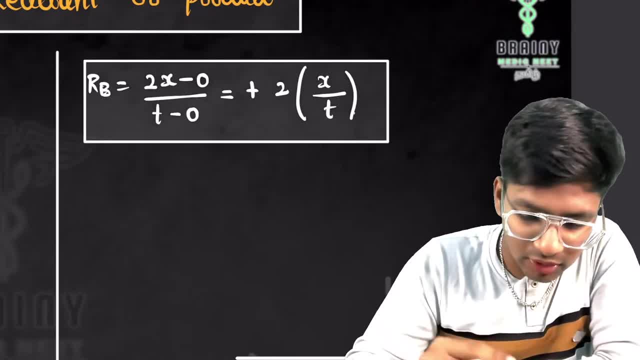 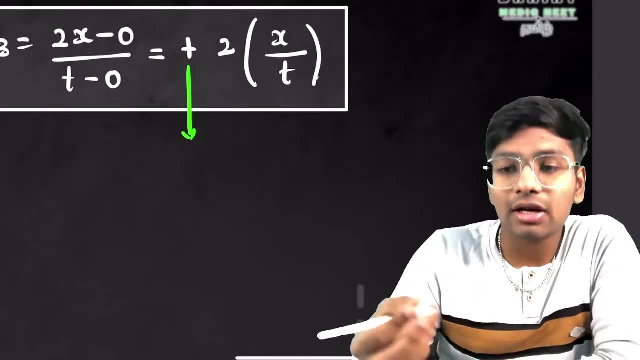 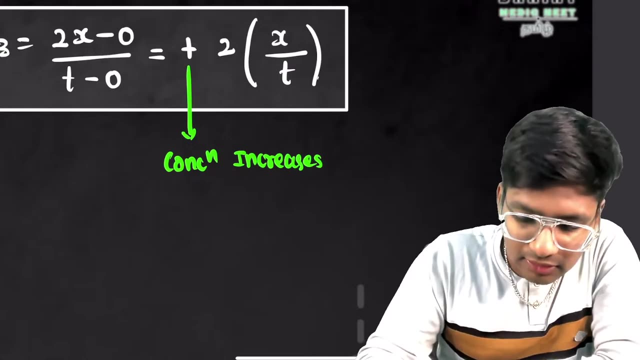 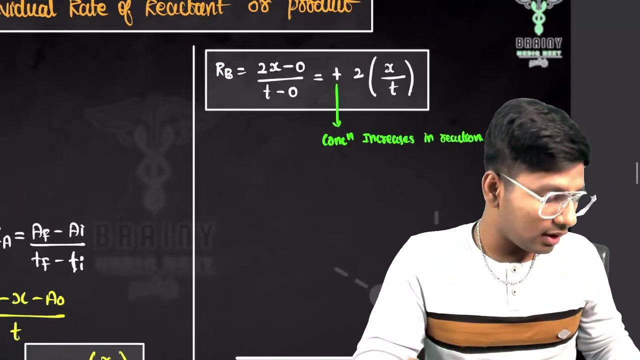 We have donated a lot. Organic chemistry has donated So C plus denotes that during reaction, concentration increases. Concentration increases, Increases in reaction. Okay, So till now is it clear. Till now is it clear. I will not solve many rate questions without pen. 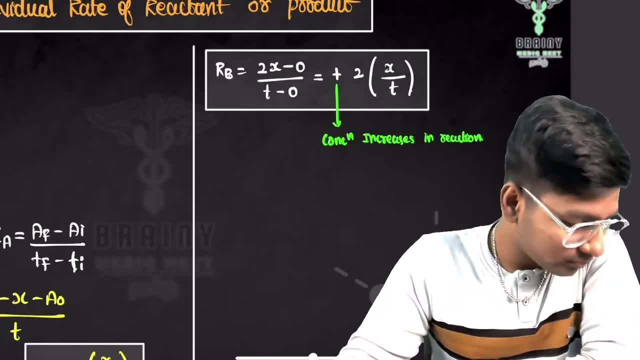 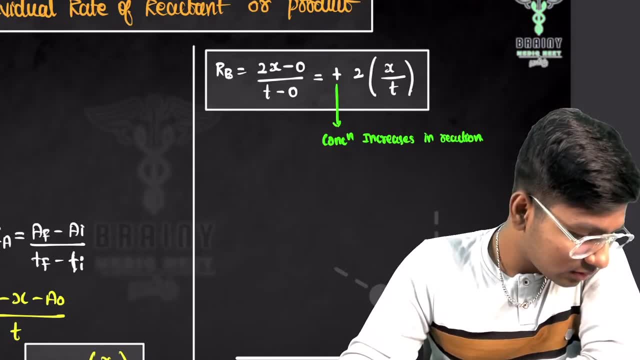 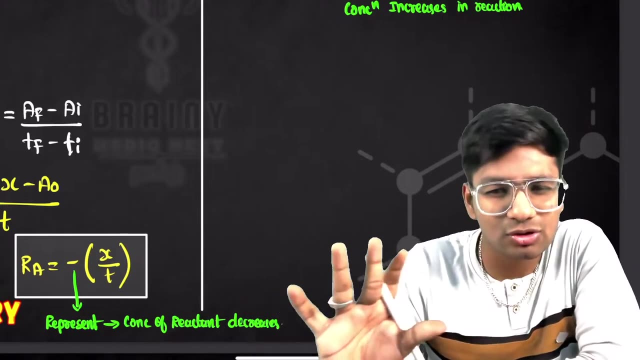 Rate question. If we solve, we will solve. Without pen, we will solve. Sit down, Write Clear, Clear, clear, clear. So look at this: What is A and Rb? What can we say if we say a relation? 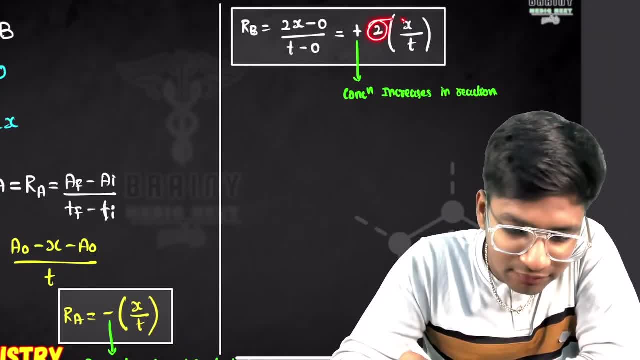 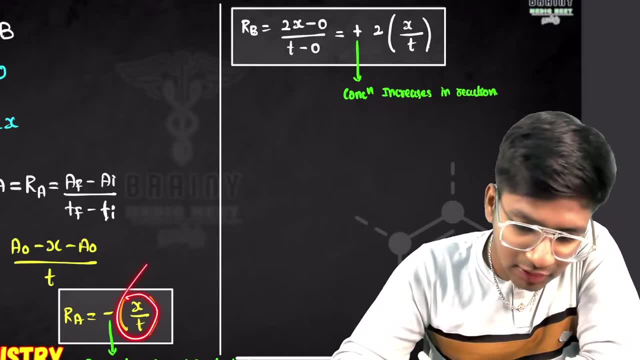 Look here, Look here. Here. 2 times of x by t, Here, x by t. Okay, Here. x by t is there Here. 2 times of x by t is there Here. 2 times of x by t is there. 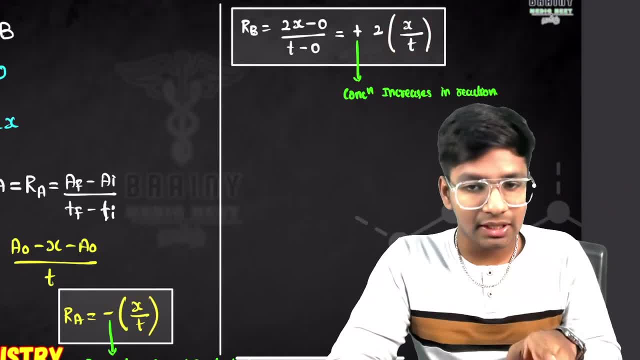 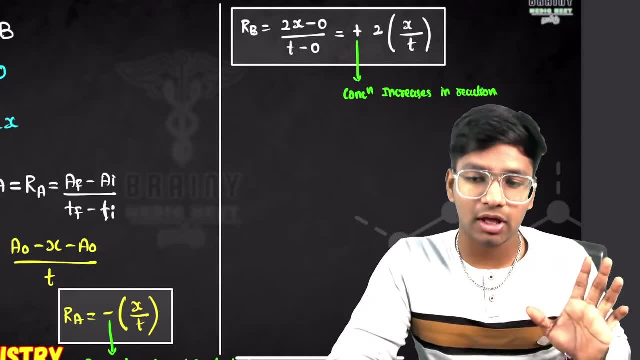 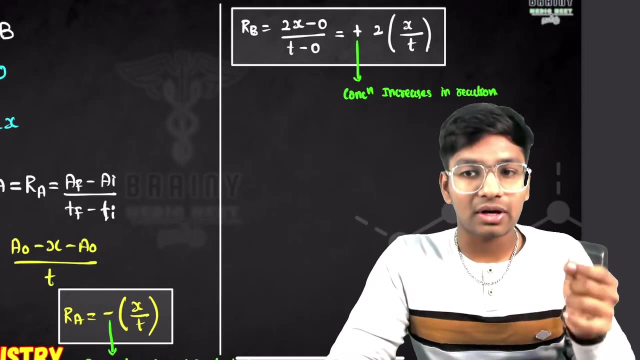 So what can I say? Rate of B is equal to 2 times of rate of A. Can we say, or not? Can't we say- Look here, Ganesh, You said it correctly, But I have changed it: Rate of B is equal to 2 times of rate of A. 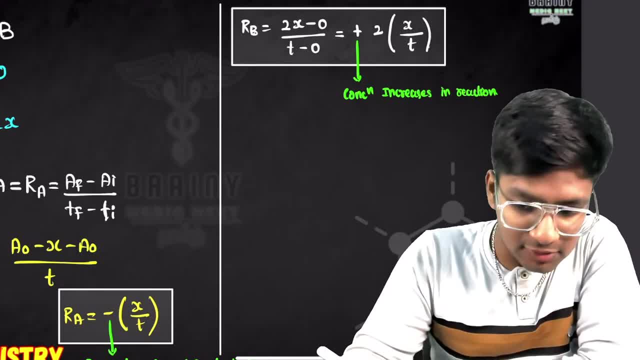 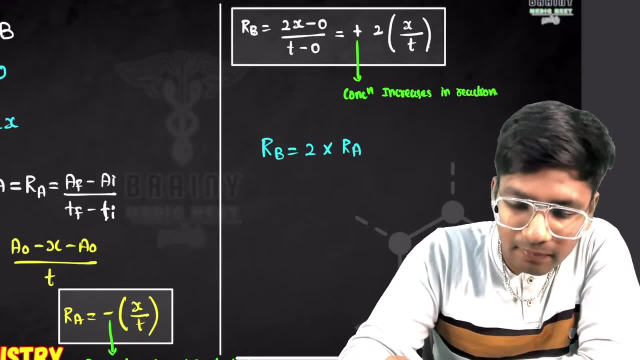 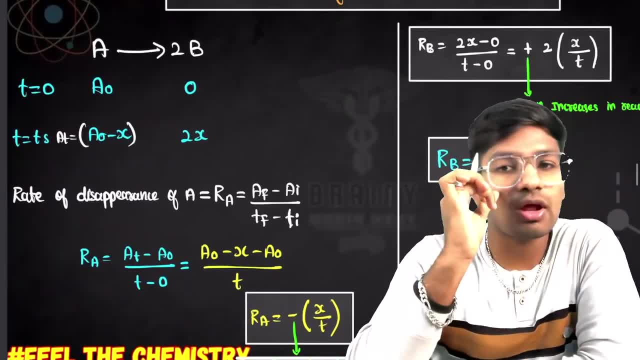 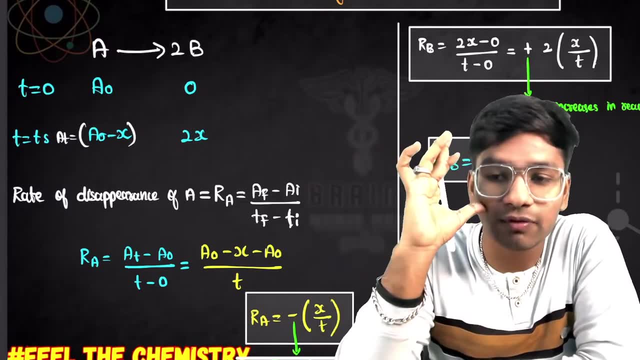 Okay, Date of B is equal to 2 times of rate of A. The thing that I want to tell you through this is: the rate of reaction is proportionally proportional to the moles of the reaction. The ratio of the reaction, The ratio of the moles of the reaction, is the ratio of the rate. 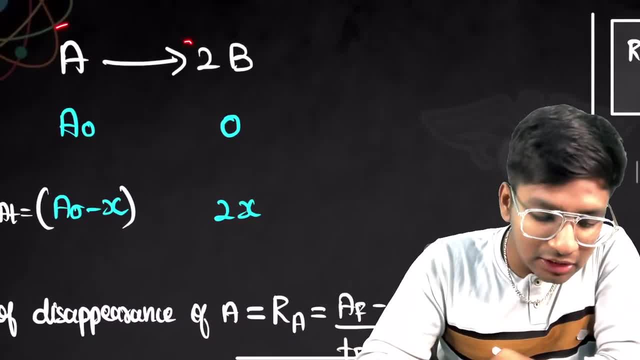 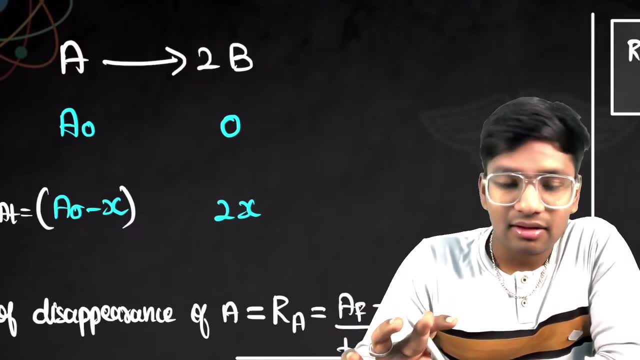 of the reaction. I am telling you, Come here. How do I say that rate of reaction is 2 times more than the rate of reaction? rate is also 2 times more than the rate of reaction. is it correct? is it correct? 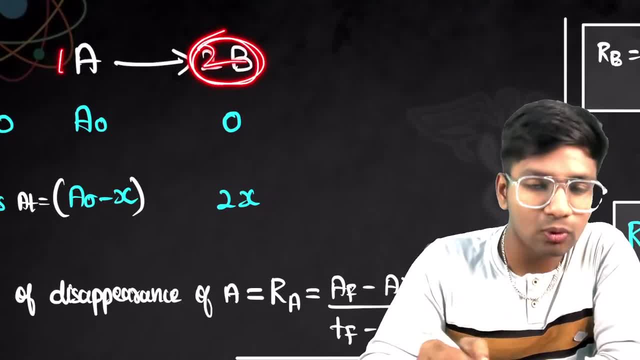 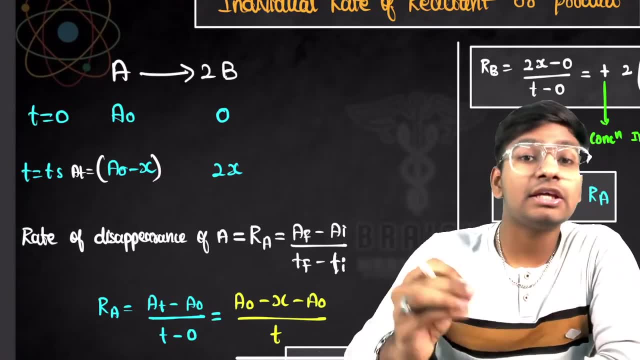 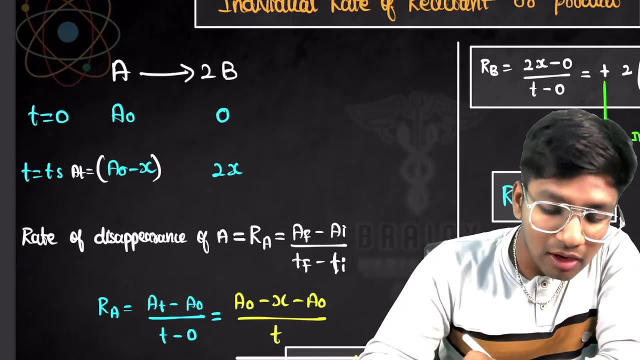 do you know what I am saying? see the ratio of moles here: 1 is to 2. see the ratio of rate: 1 is to 2. done, done. this is valid, always, always valid, always valid. we can write the answer after seeing it. 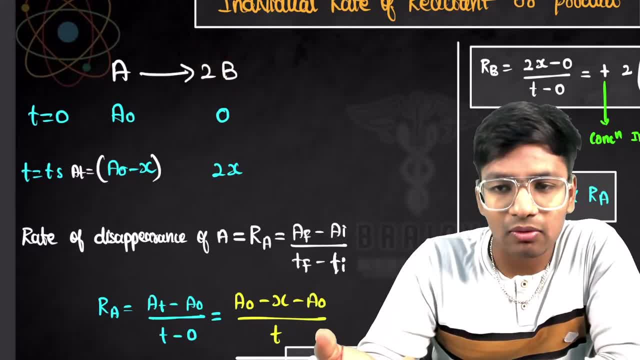 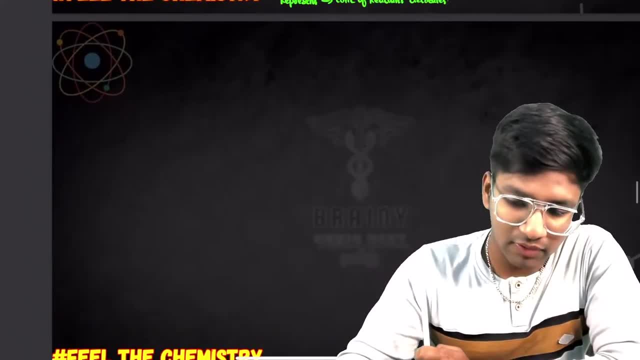 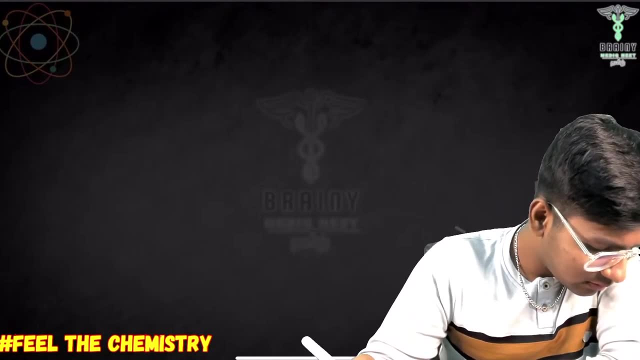 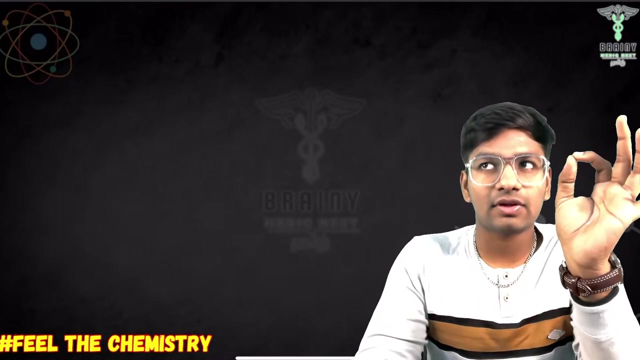 so what we can do is 2 times more than the rate of reaction. simple, simple, ok. many more people may not understand this. I will make them understand. many more people may not understand. I will make them understand, ok, for example. for example, for a substance A has X. 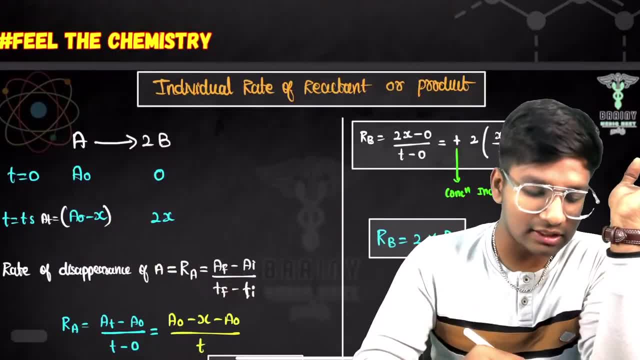 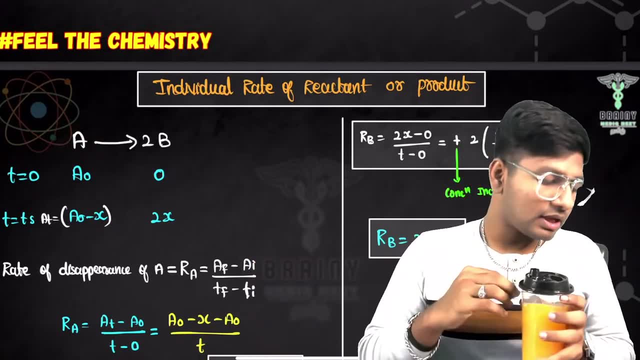 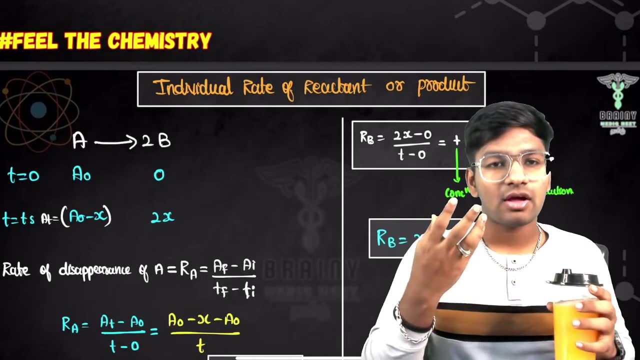 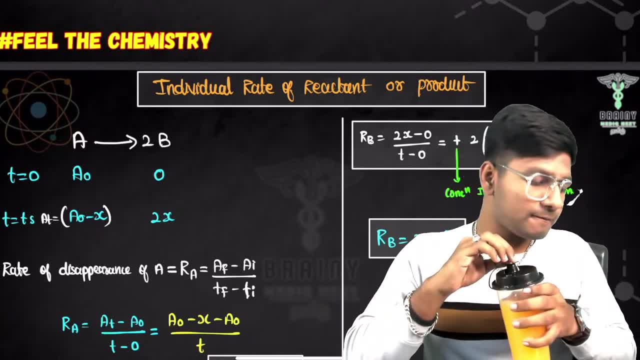 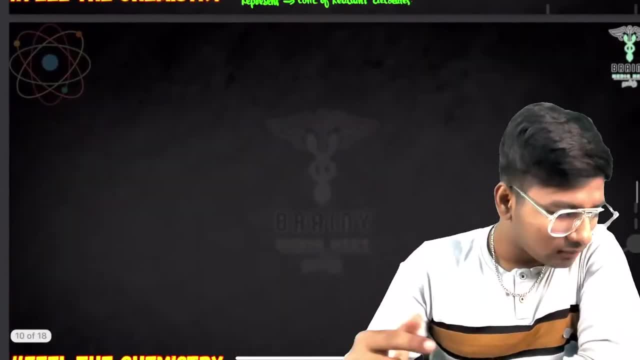 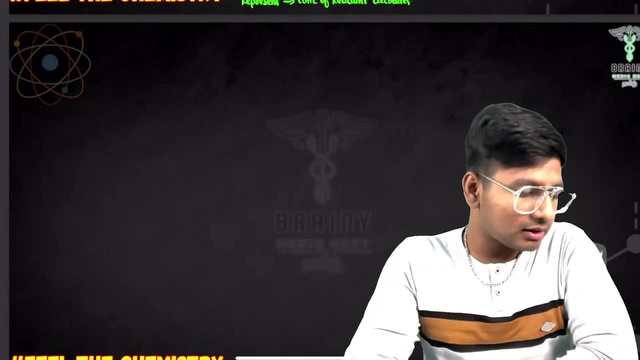 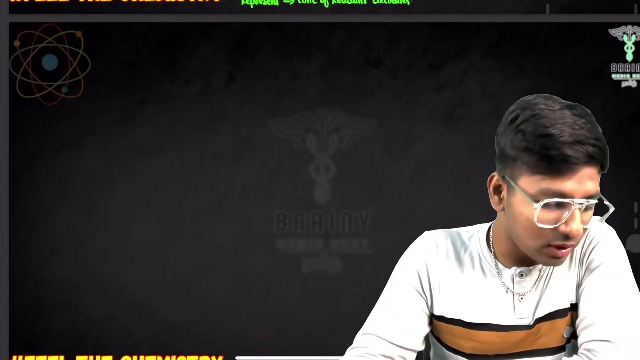 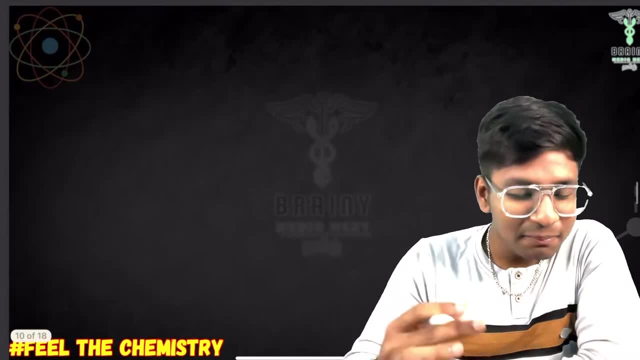 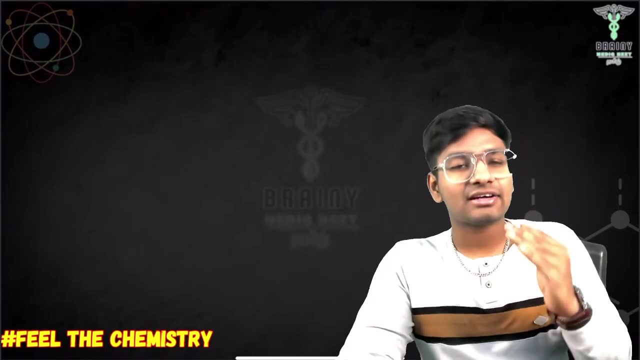 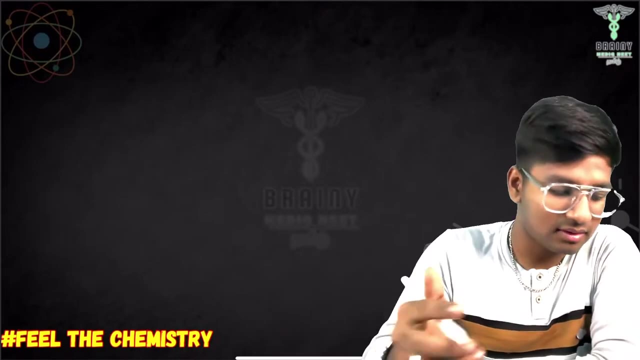 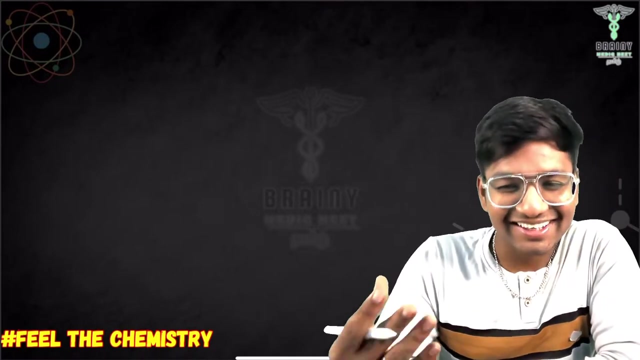 pocketing it. correct our life, what about it? but this is not what I'm probably gonna bother today. that is where bravely medic name stands: active users in our channel. are they active user? users are a high in our channel. now, bottom one left 40,000, 150,000 subscribers. but this party 13, which 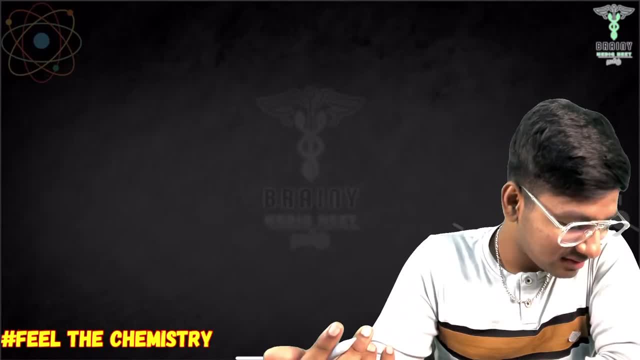 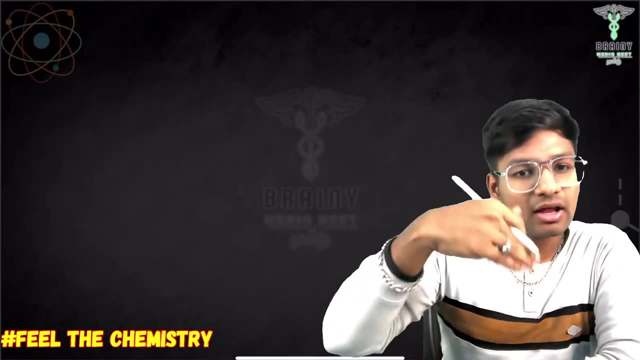 would it return promotion by ad? now only a little, promote my shots for the good a time. you're gonna know shots. put in an area per pop on area of our own shots in time. in the shots for a particular shots it's Tanya shoot. you're gonna know shots for a particular shot. 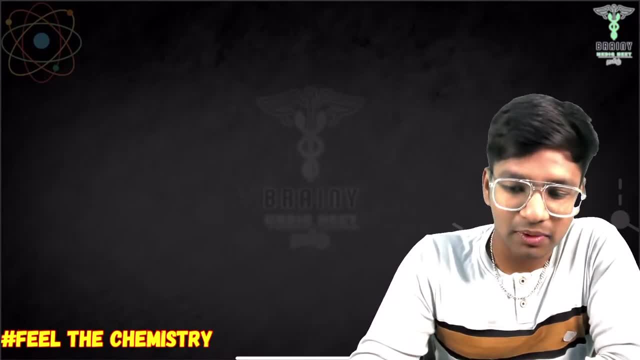 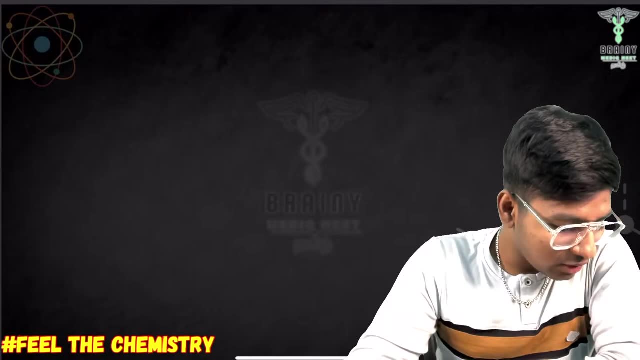 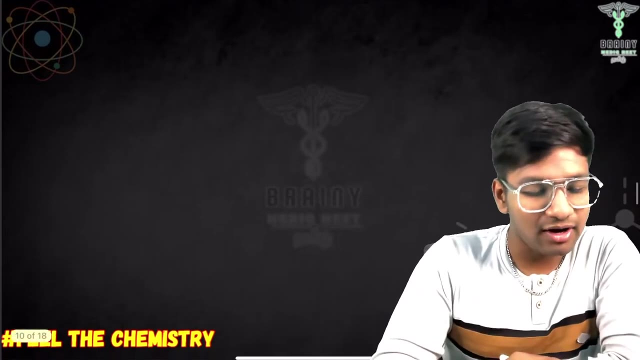 from shots of you like one another. did it burn shots super and time in the. okay, I reach out, but some see recorded content speaks okay. so see, in the other part I recorded a lot. summa, you can gossip. a record, a poplar. now the video. you're gonna know what the my 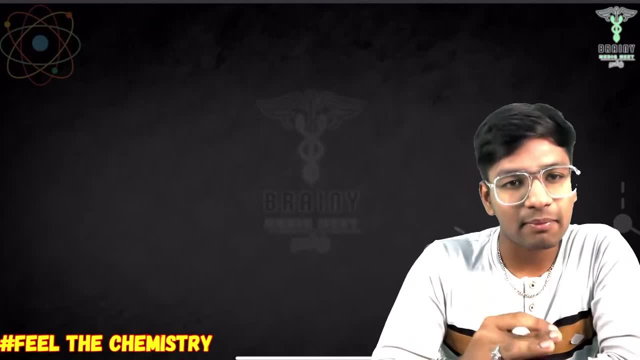 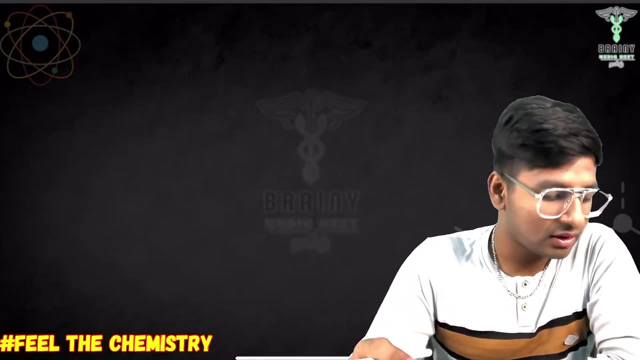 argument on the bottom one, on the skip on you in here you're gonna see a problem about the map from a part of an. so the part, part, part of a poem, a tower record. no one will be able to read the whole thing. I know that very well. 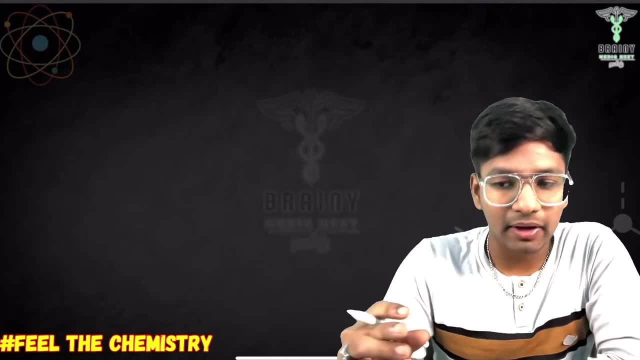 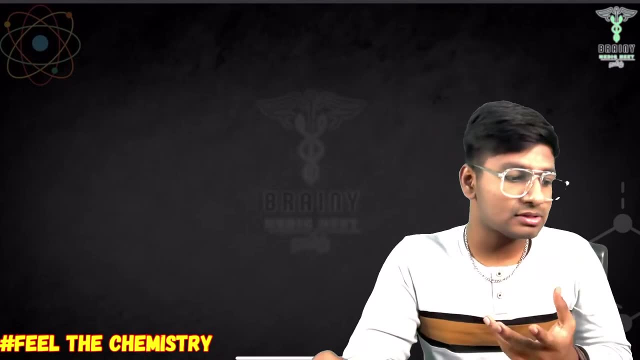 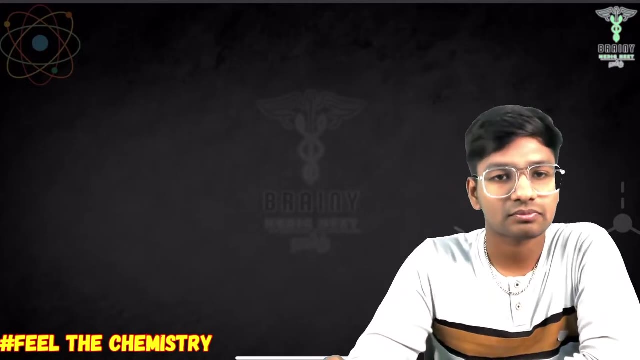 when you are watching live, you will be able to read the whole thing, each and every word you can catch. when you are speaking, you will be able to catch a lot of contents, but the recorder is not able to watch the whole thing. for 4 hours you have to watch the whole thing. 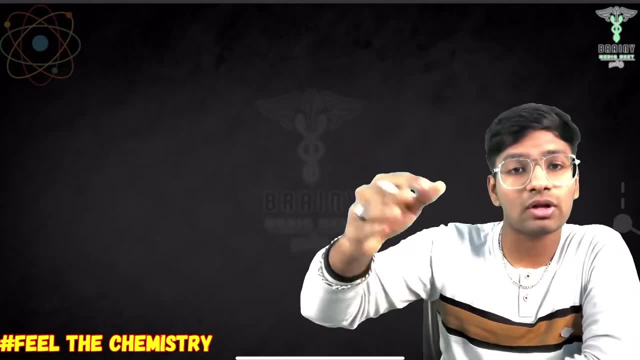 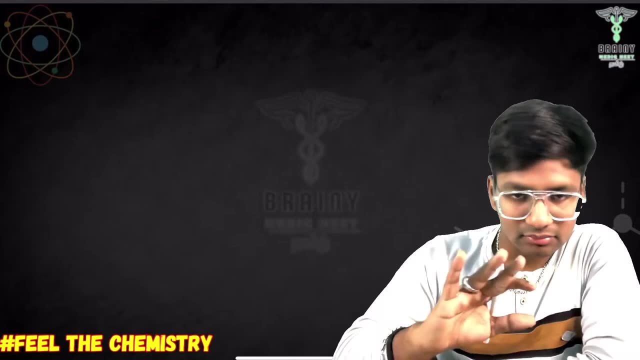 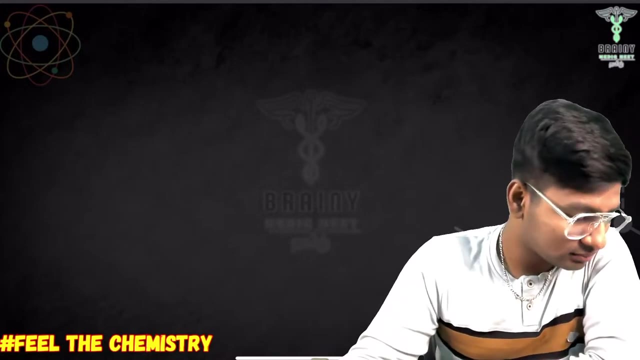 but when you are watching live you will be able to watch it constantly. when you revise it you will be able to watch the notes correct. like that, recorder has some issues in your preparation. you can't do that with recorder. bro, watch it for 8 hours. 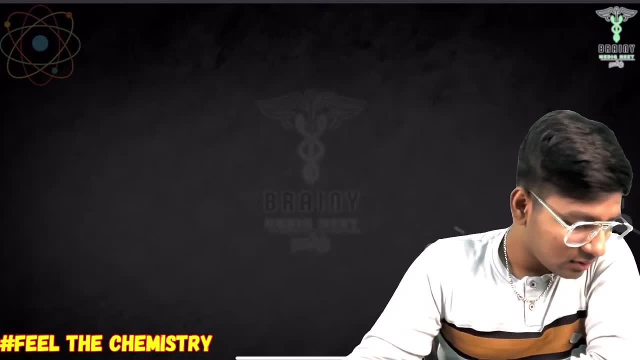 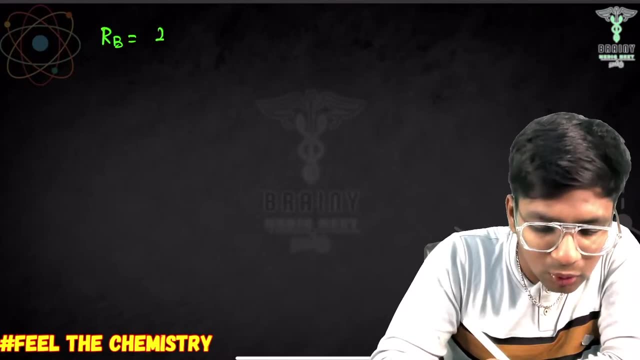 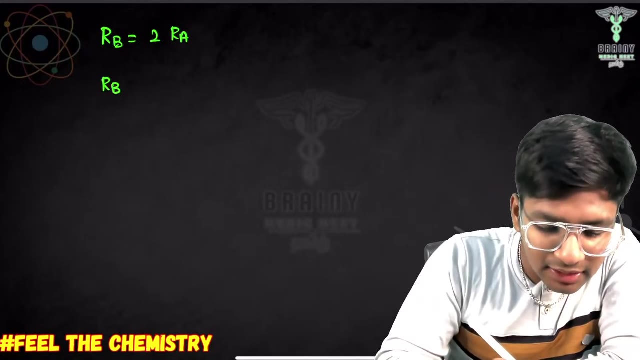 ok, so see, see, see, see. what I have written is: rate of B is equal to 2 times of rate of A, 2 times of rate of A, 2 times of rate of A. correct rate of B divided by 2 is equal to. if you don't understand, 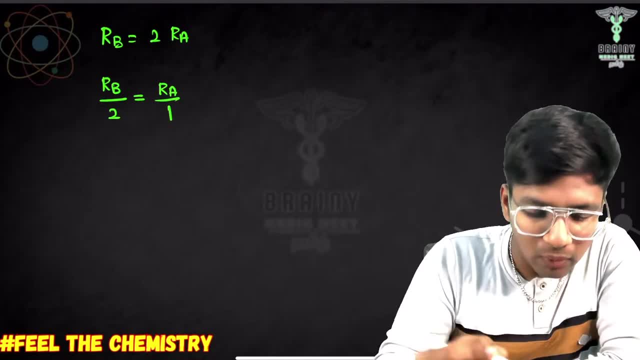 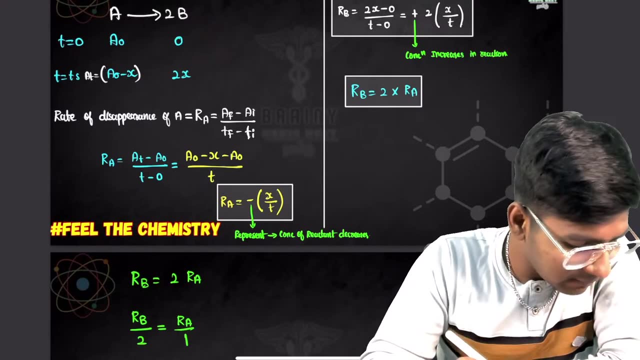 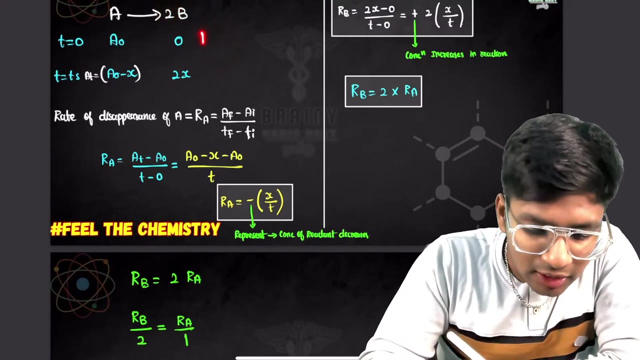 I will tell you next time. rate of A divided by 1. do you know how I have written this? rate of B? rate of B: see see. rate of B divided by its coefficient- sorry, 2 divided by its coefficient. rate of A divided by its coefficient. this is your second method. 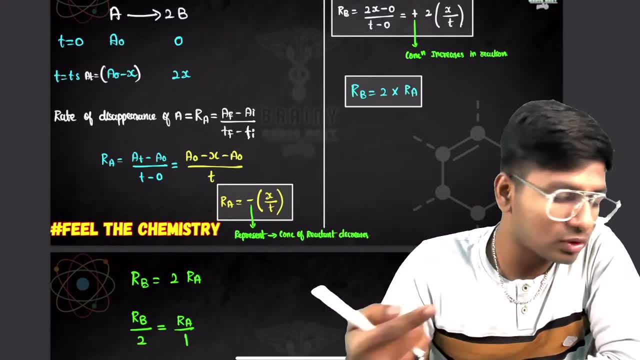 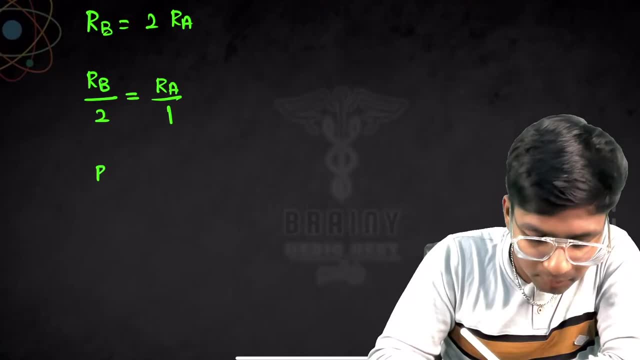 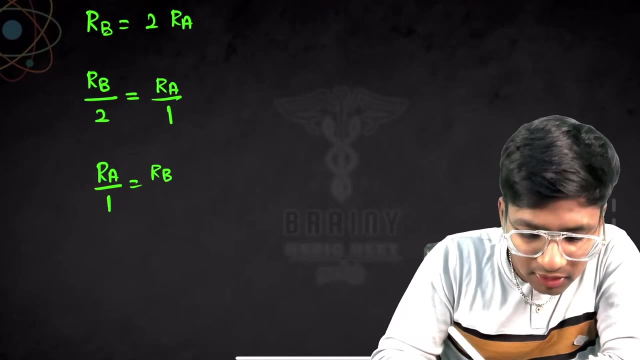 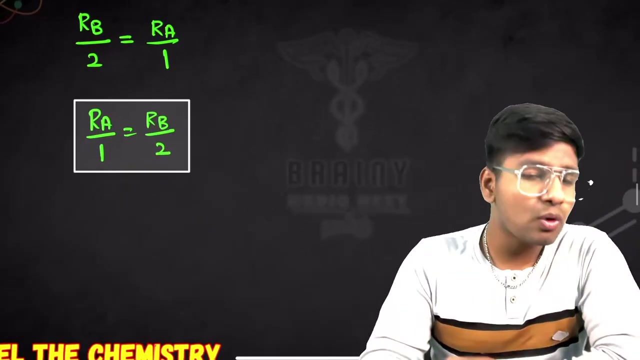 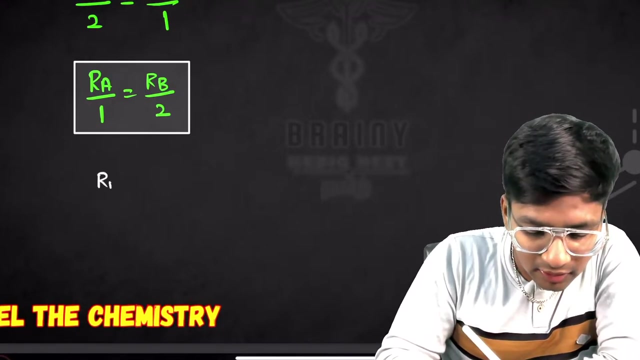 what. this is your second method. solve the question like this: directly: multiply and write. write like this, if I write properly: rate of A divided by its coefficient. rate of B divided by its coefficient. ok, ok. next what you will do is let me write again: rate of A divided by. 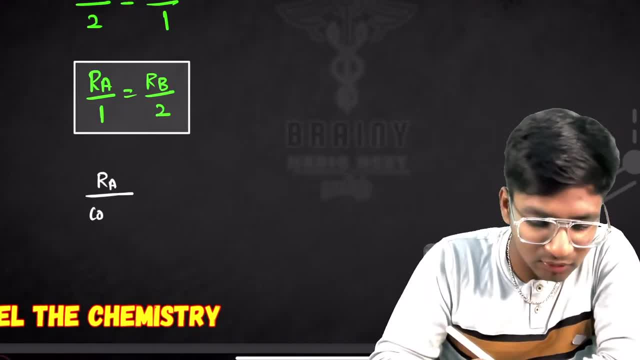 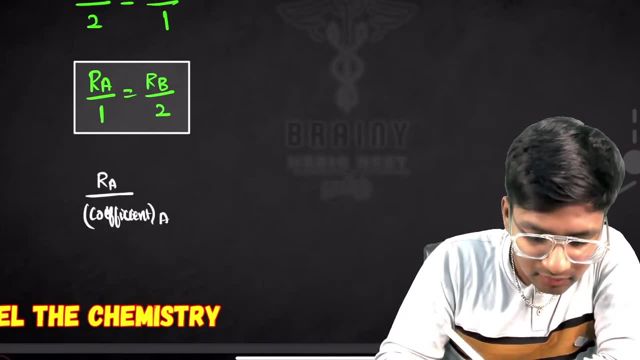 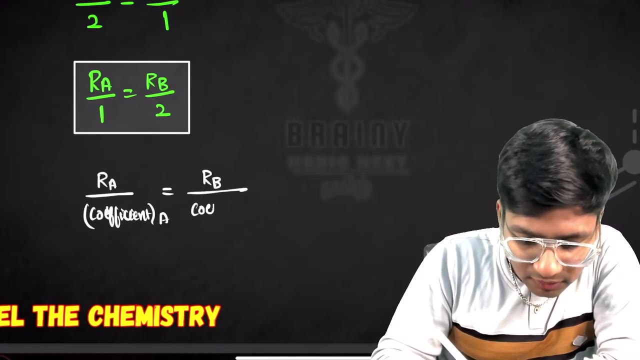 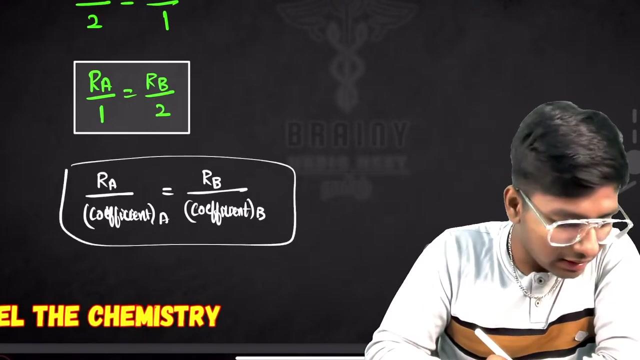 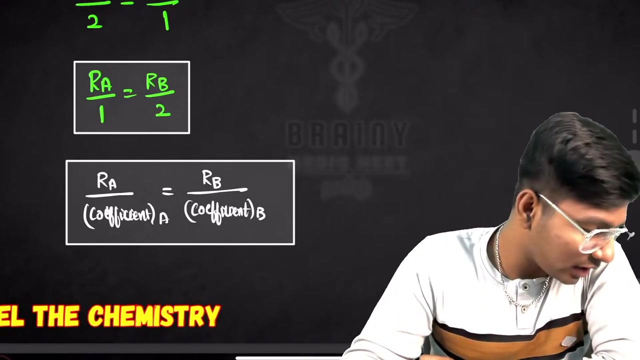 rate of A divided by rate of A divided by coefficient: ok, coefficient of A, coefficient of A. coefficient of A is equal to rate of B. rate of B divided by rate of B. coefficient of of B: Danna, Danna, 160 plus of 180 super on a shri molly, nice upper in a Korean, or unity out of. 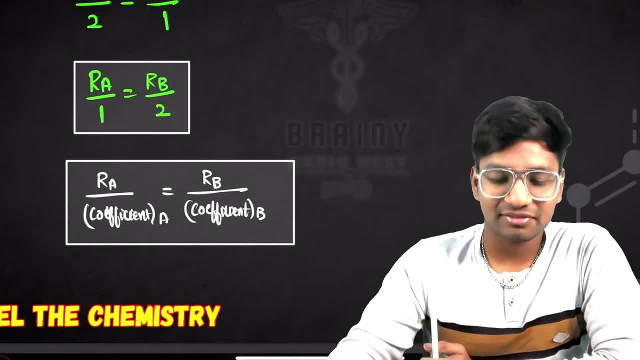 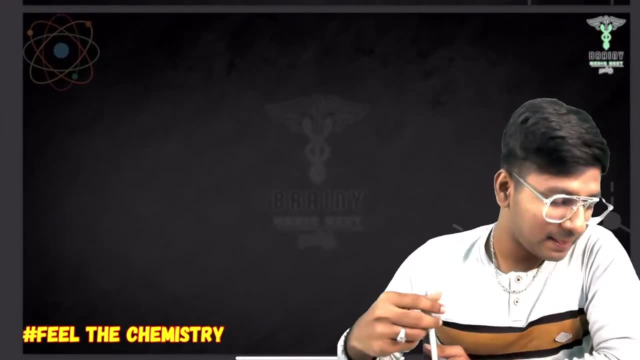 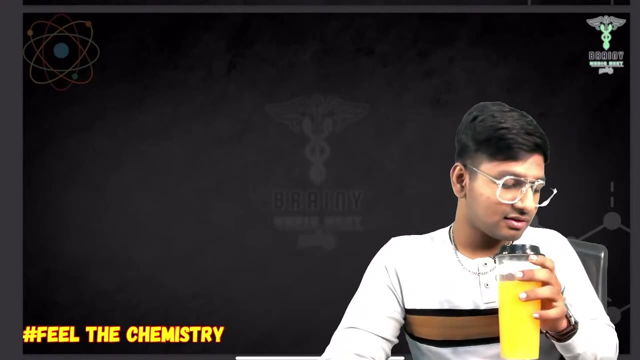 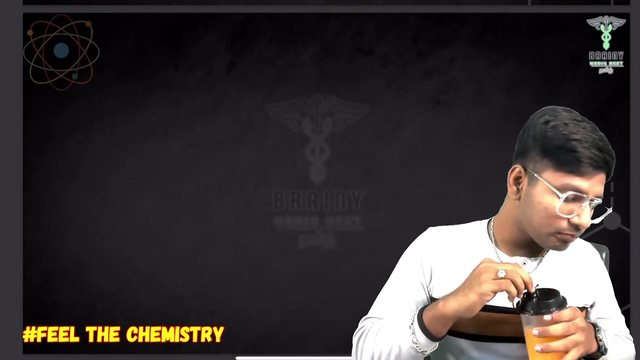 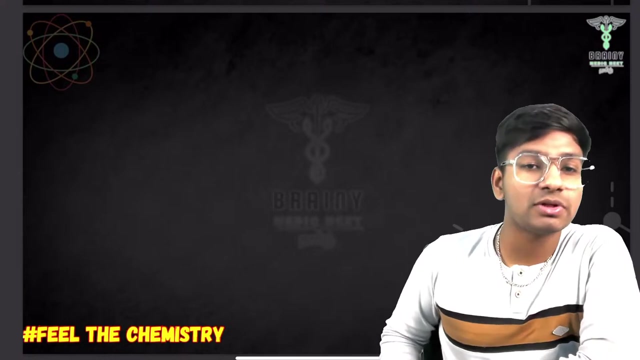 on it as you were, ma in the ocean. can I get from my students? students get on there and I would, 180 out of 180, explain my expert Paloma. explain Paloma at least 270, 175, 170, 175 and Karen giving so much of hard work. okay, I know knows that could. 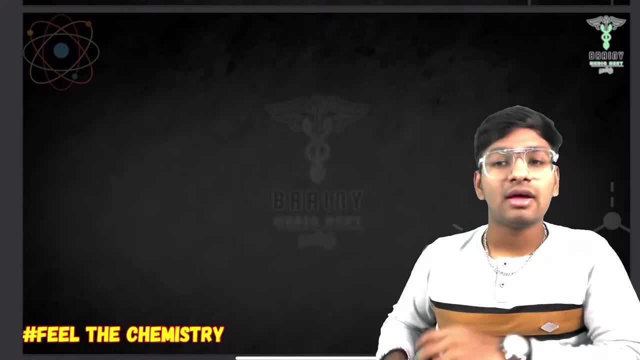 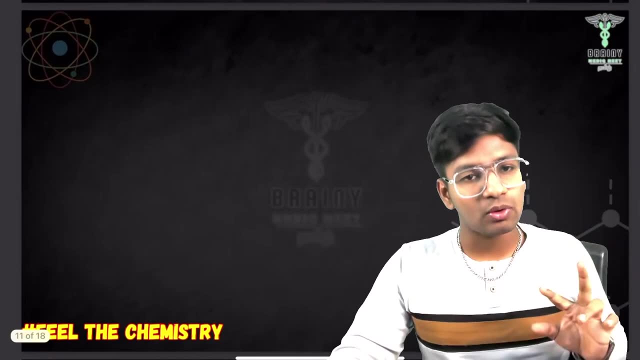 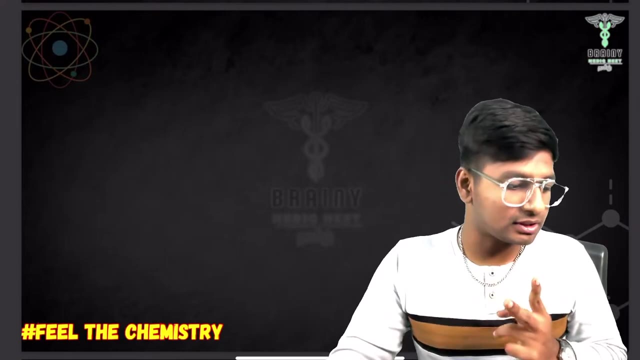 start from lab or app could understand from their normal it because you need a car seal in eye, am I have. I have a money. okay, I know, payment in the payment which in a mood in China start, funny course, lunch for nine or in the muscle, but nine upon them. 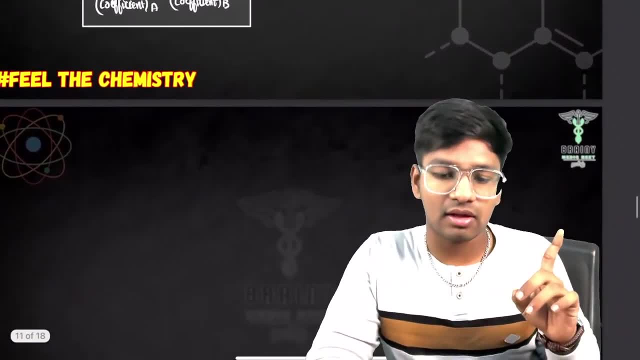 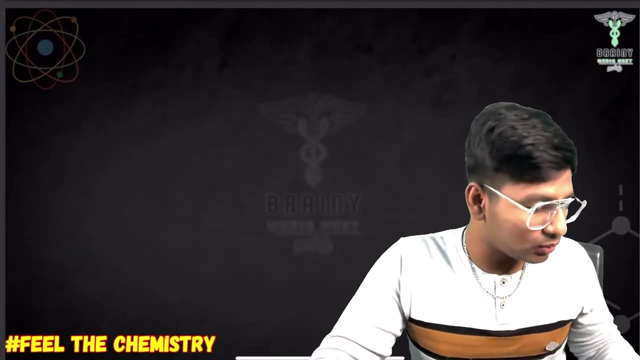 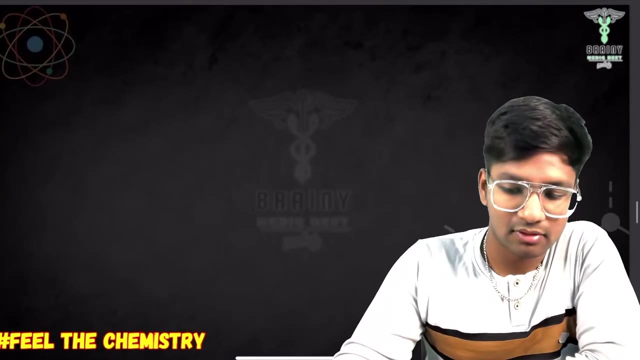 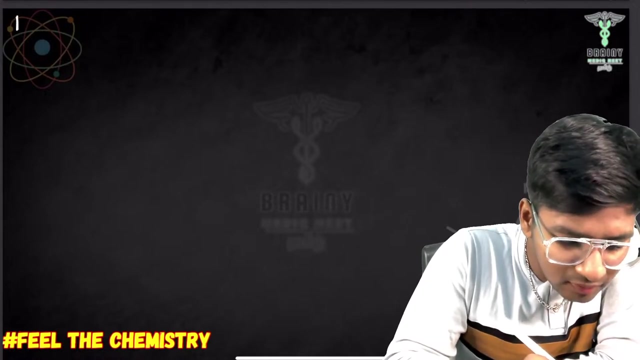 Martin, you know what I'm saying. mark or not, like all of the seed Madhubita Madhu, I remember you okay in the country and then in the market for the other pole. that's enough. see next one there in the other level in a parana be M and D. 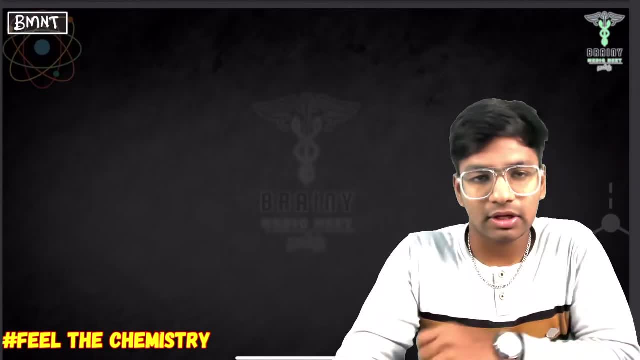 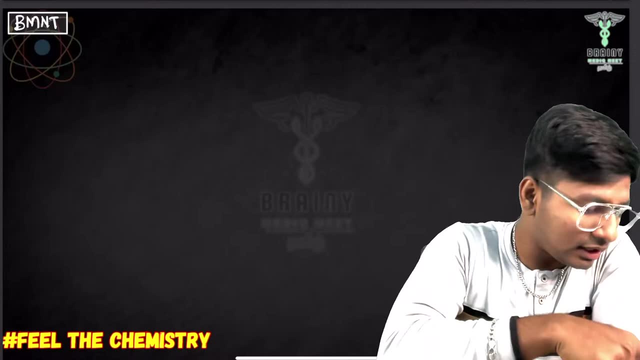 be a maintain protocol. okay, be a medieval to go. it's a trick or a trick in the particular in the page in our movie. a lot of them, a lot of you on there now in the area of a okay, well, either way. another thing: I in the lecture like: 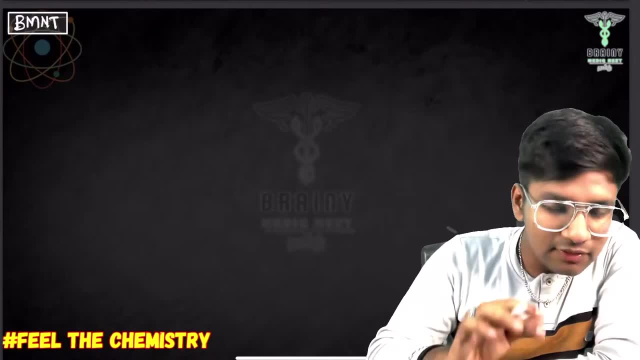 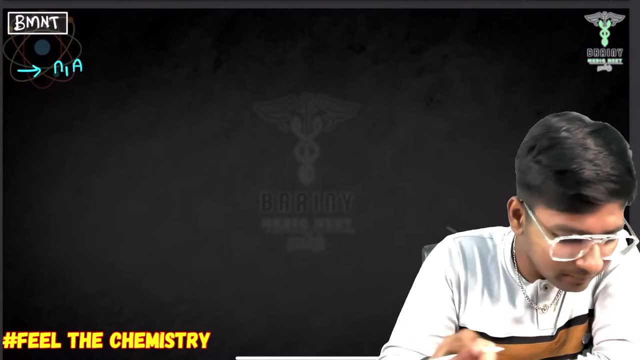 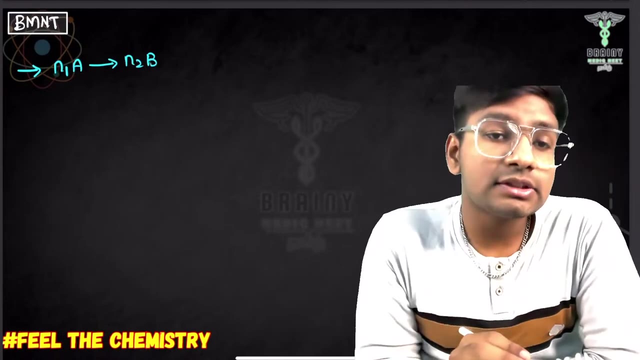 cover our concept and I know what a page on the monitor. so see either China in a, you know Tina, you know she and I. you know, for example, young one a- okay, young one a gives n to be general reaction editor and general reaction editor, and one a gives n to be general. 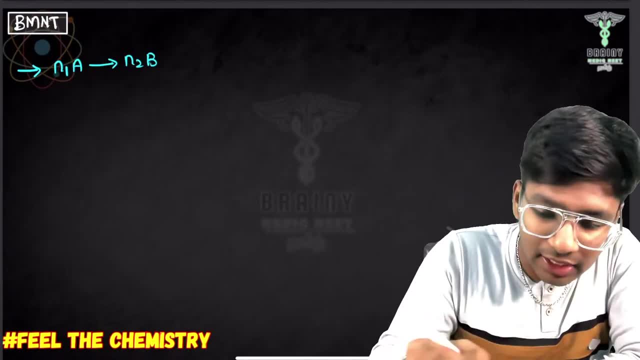 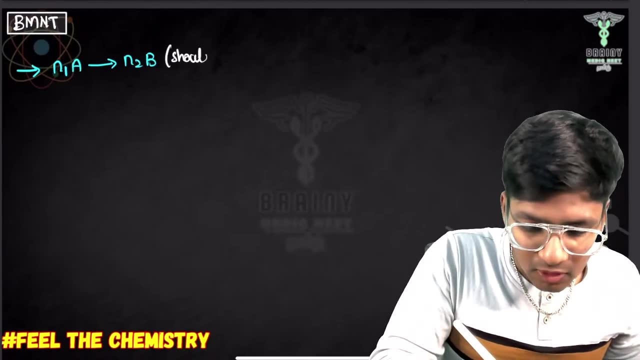 reaction: my editor n 1 a gives n to b. general reaction: editor n 1 a gives n to b to b and India. it should be balanced. actually, no, the body should be balanced. should be balanced. balance the reaction. I income okay either in the area the 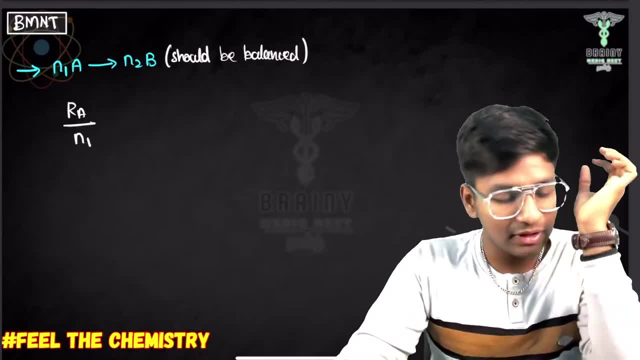 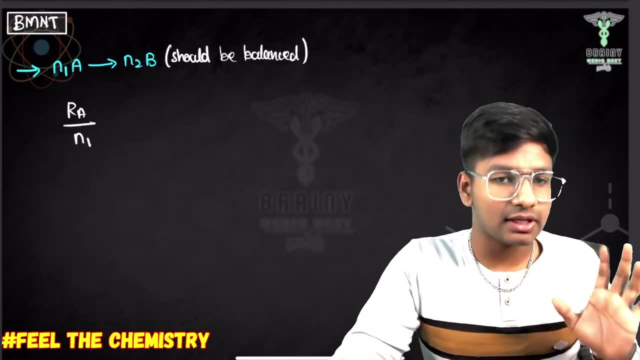 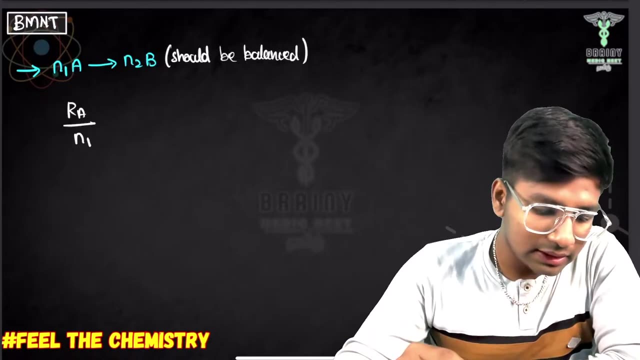 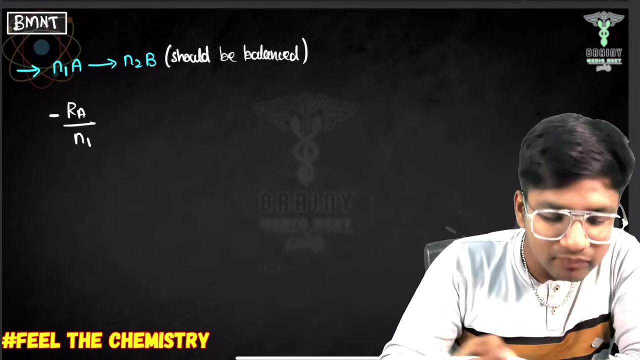 ok, correct. ah, I know, Mary, we don't really tell them what he did not correct either. if I read another correct or the path, it is correct and correct. you tell, tell, tell in the correct other go Tom. go Tom got the answer: negative polar because nine the money I didn't. 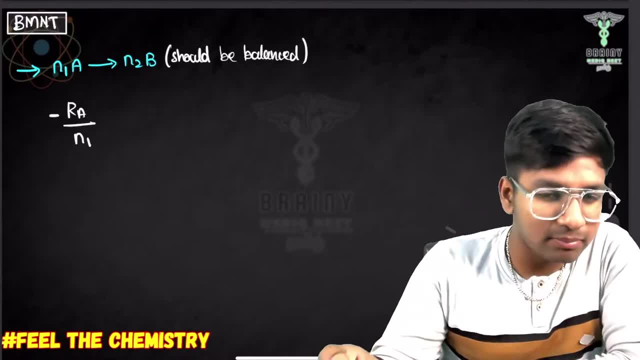 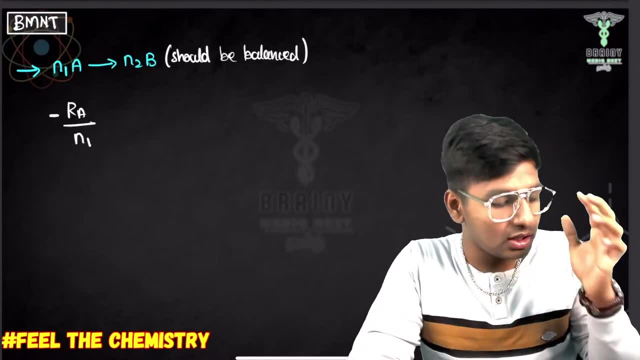 know what the negative pot answer. correct our own okay. well, negative mention for no. okay, option, select it. you have to put the command on the most of most probably options. negative command on button important, both organized. the only character catch funny Erica. negative, not portal is equal to positive of R B. 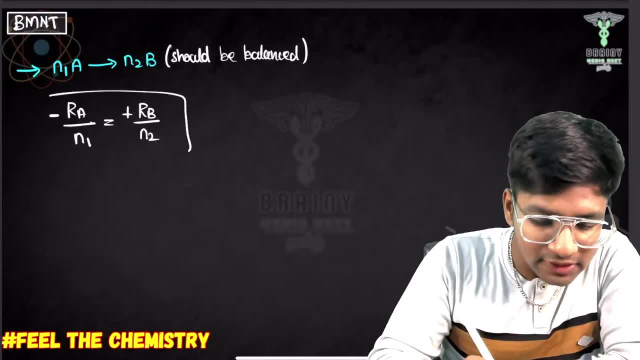 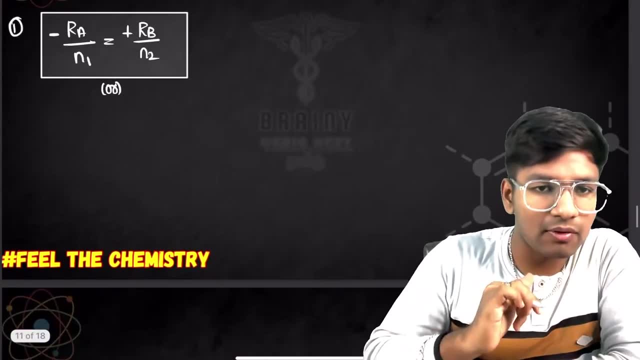 divided by n. to generalize the one. you know the first formula. you know what a first formula. you know you don't want to. they will either easier on the formula. ah, it's a very cross multiply panna. it's a cross multiply panna. you know formula. 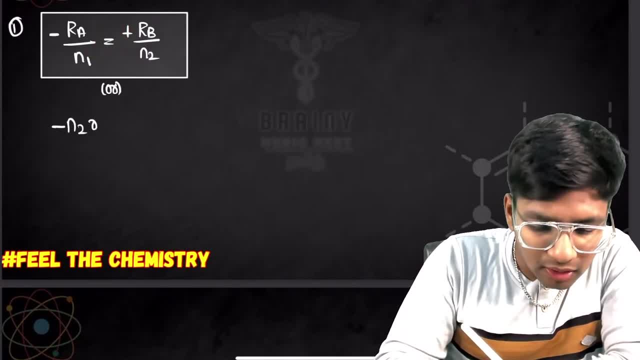 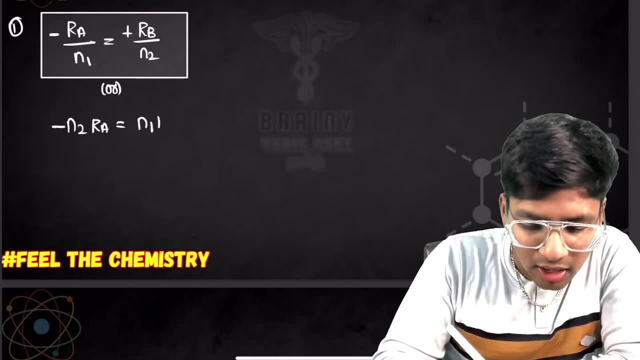 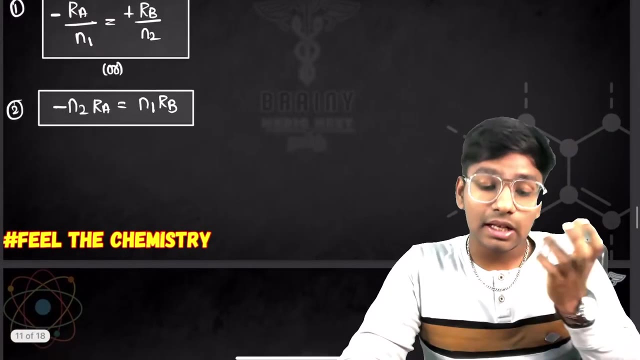 correct. you know, minus of n to R a, that is a rate of reaction. a R a is equal to R. a is equal to n 1 R B. you know what a second formula. you know what a second formula. okay, you know you don't have a lab in our. 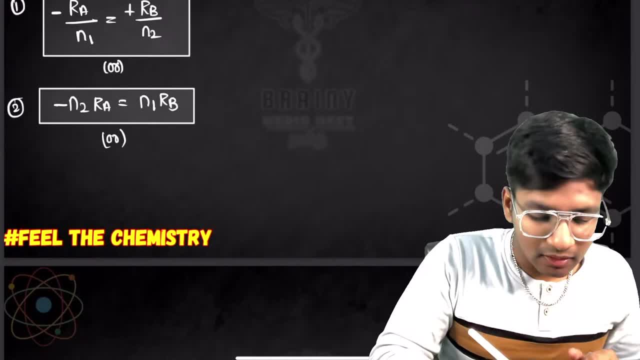 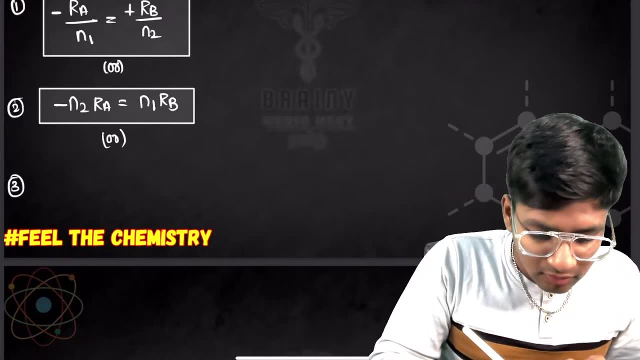 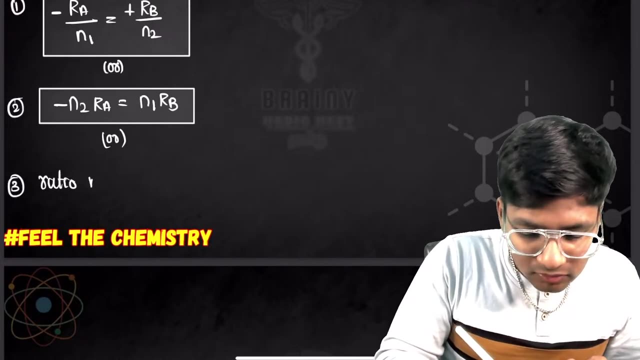 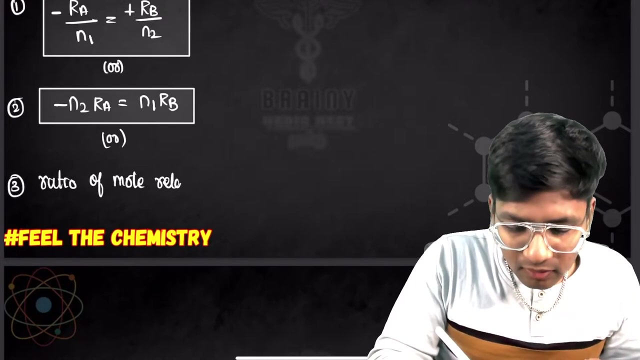 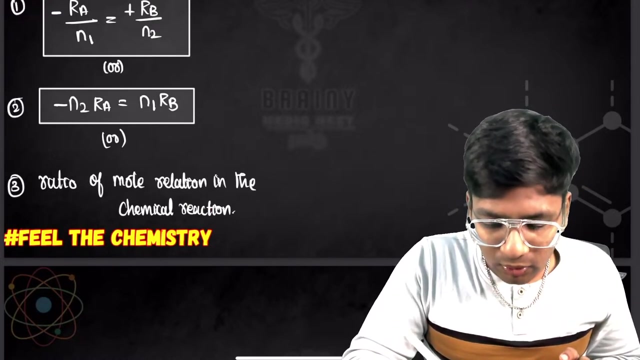 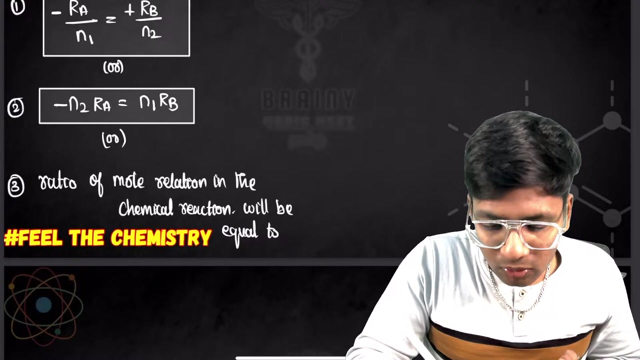 last one, very simple one, very simple one: more relation, more relation in a little more relation, or ratio of more relation, ratio of more relation in the chemical reaction will be equal to rate. will be equal to. will be equal to be put on a major will be equal to rate. okay, will be equal to. 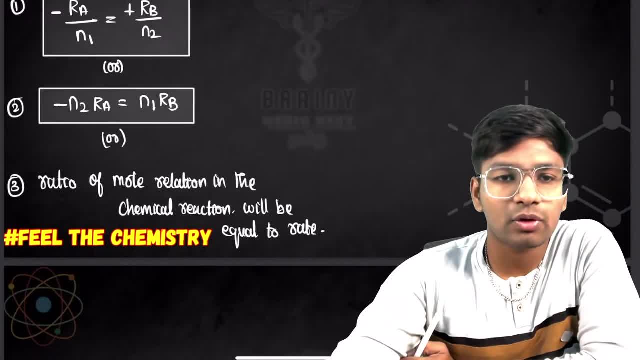 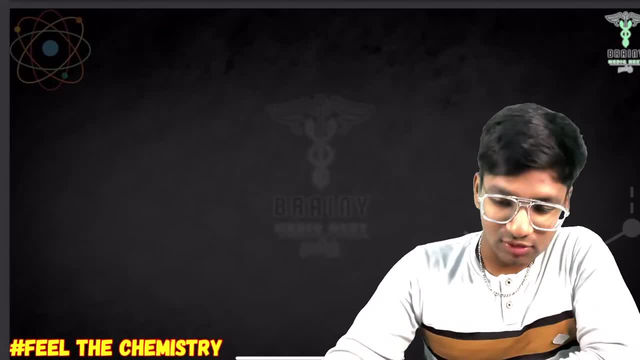 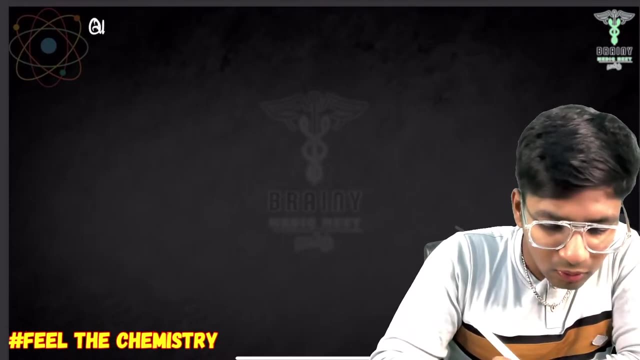 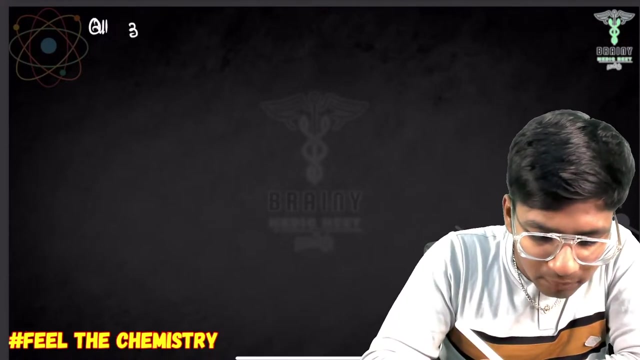 rate random question. but Lama random question. but Lama yo-yo now boss or the boss order? it doesn't a soldier either, given the pussy in the other part. now we're questioning with Graham. question is: is 3br2, 3br2 question and a lot of money? 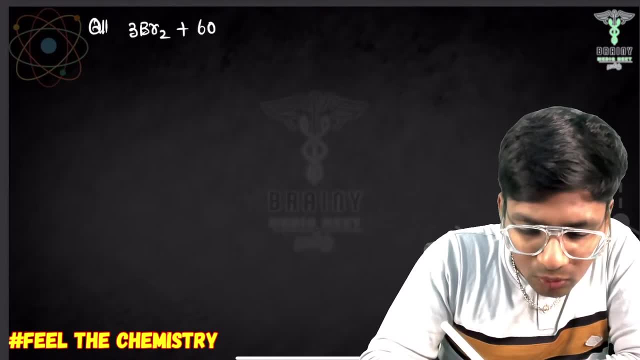 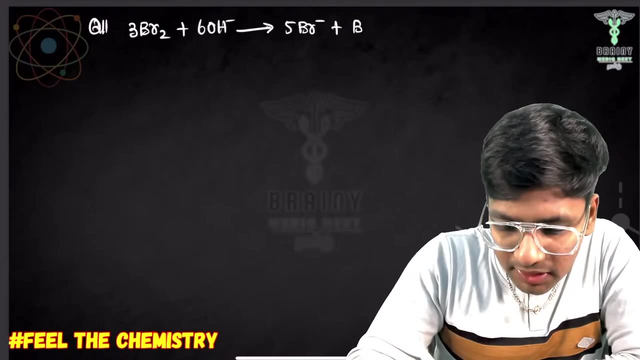 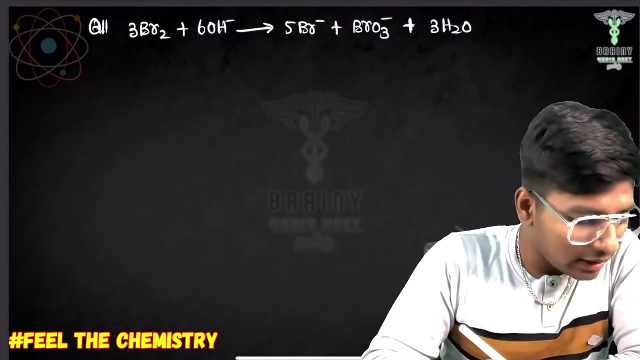 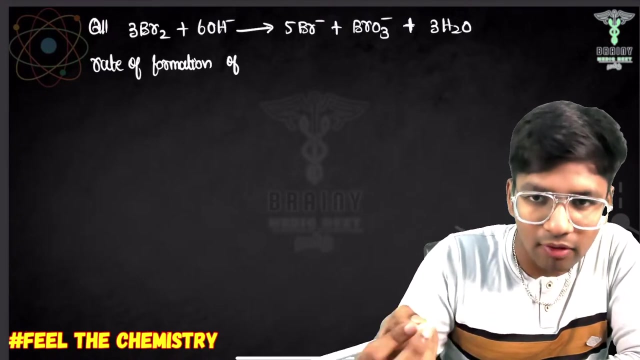 for 3br2 plus 6 ohm minus 6 ohm minus, give 5 BR minus plus BR o 3 minus plus 3 H 2. oh okay, you know when I get up on your camera. rate of formation: rate of formation of BR o 3 minus my total. 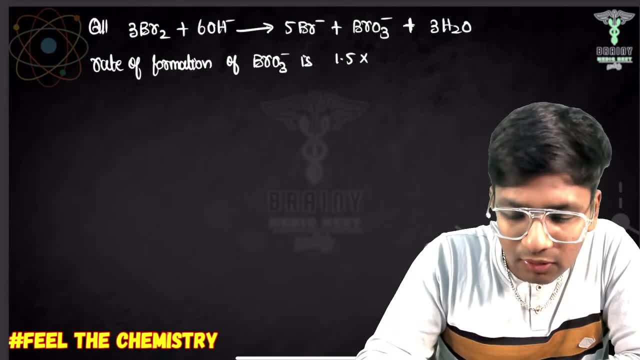 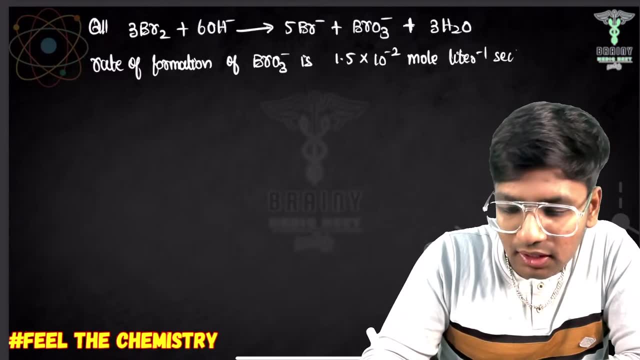 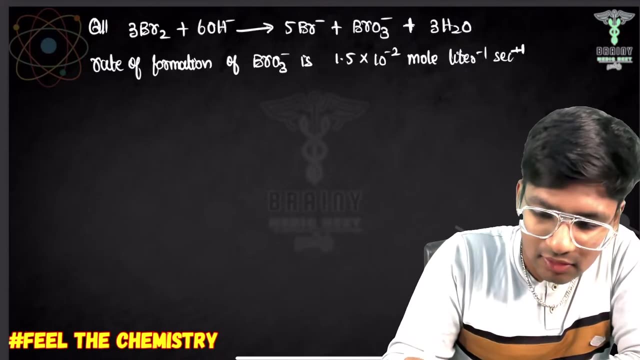 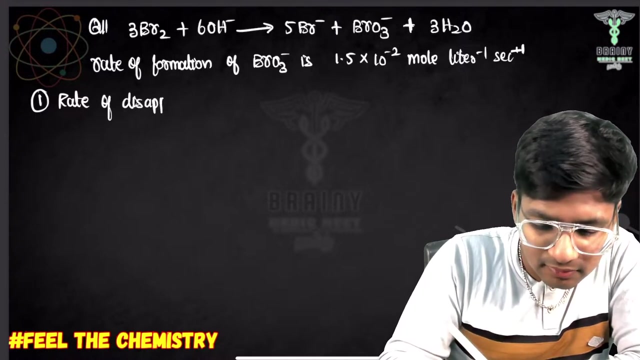 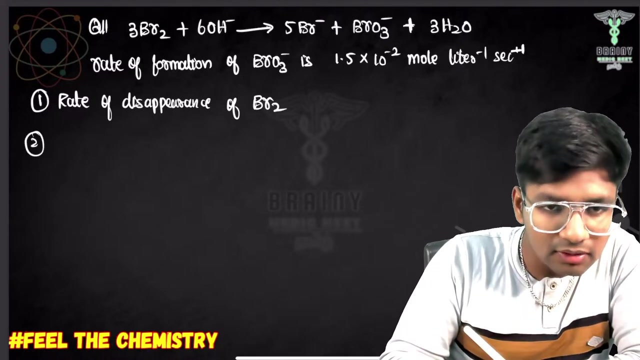 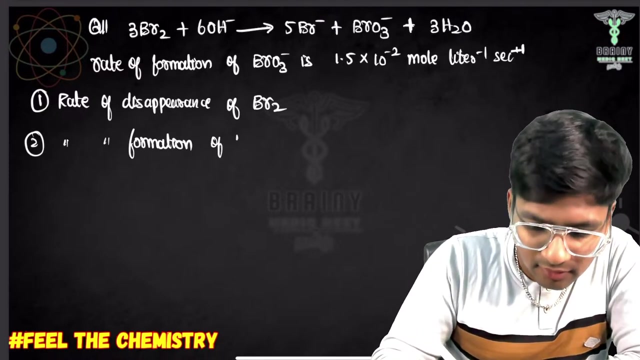 computer and then it is 1.5 into 10 power minus 2 mole liter inverse. second inverse. okay, when I question and they get around up in our question where question is: first question: find the rate of disappearance of BR? to. second question: rate of formation: formation of BR minus third. 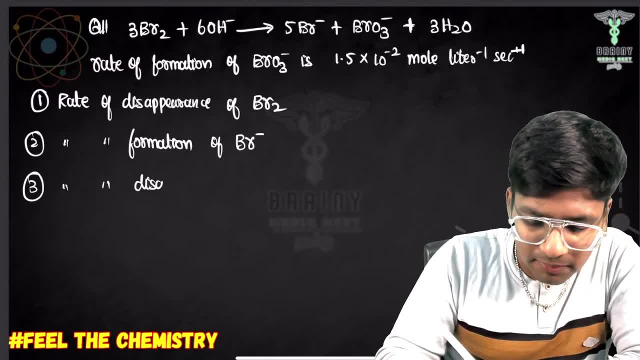 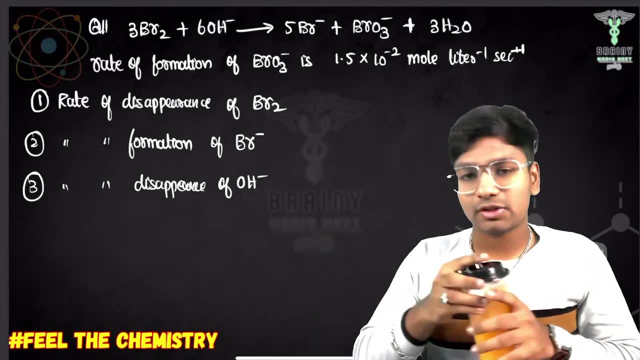 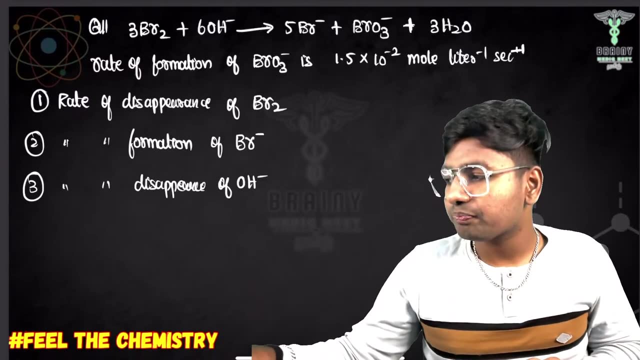 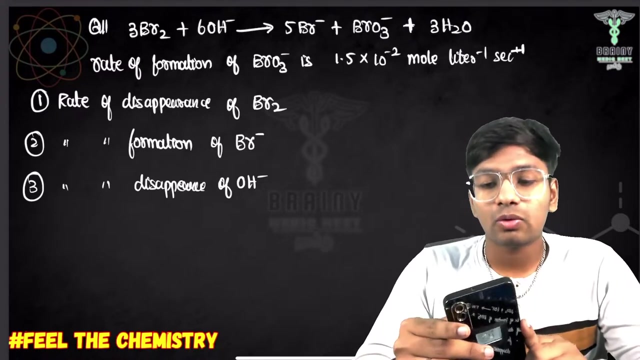 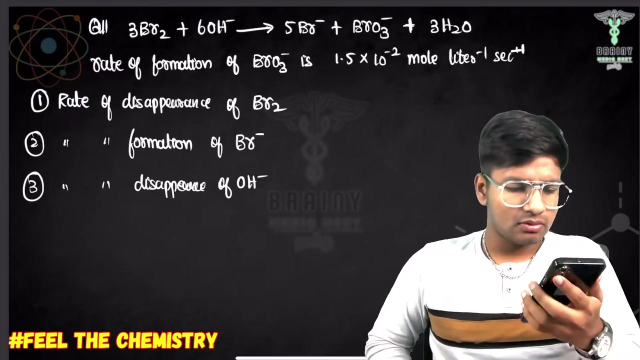 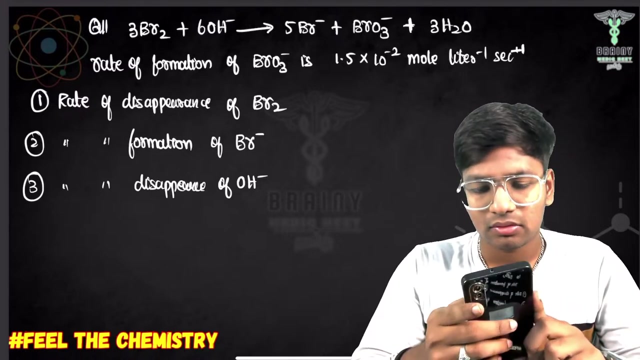 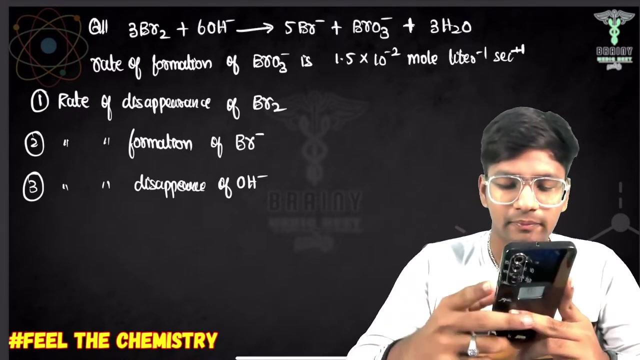 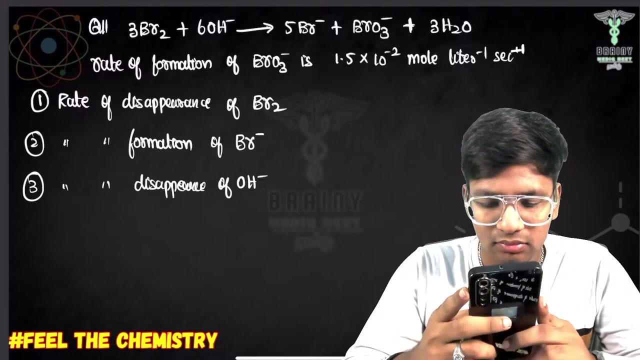 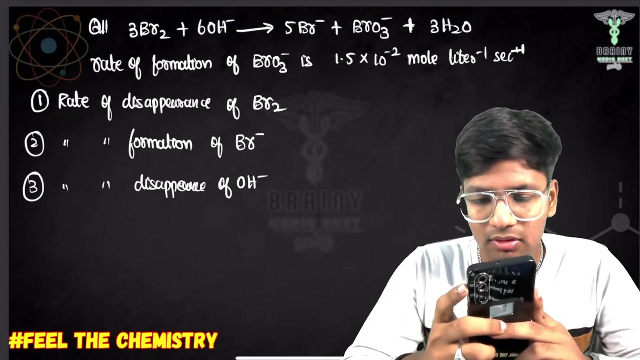 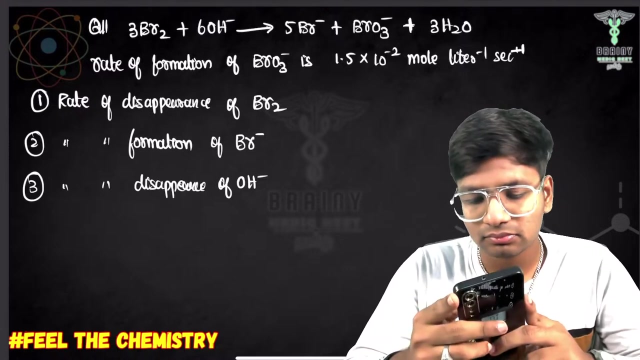 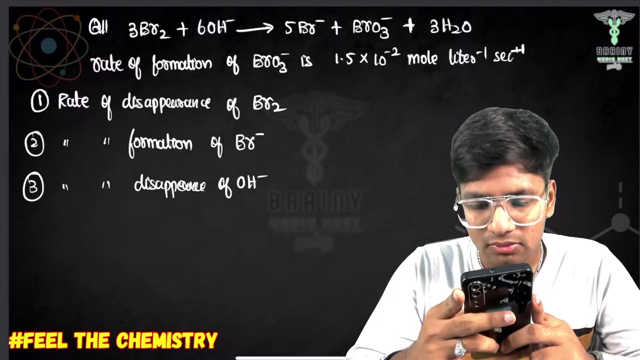 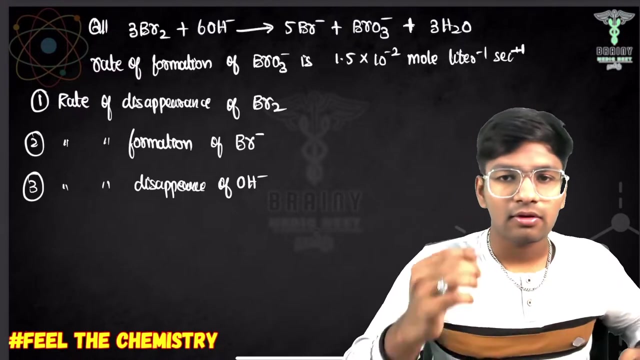 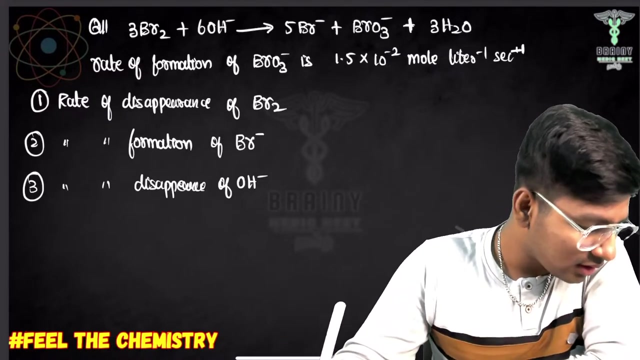 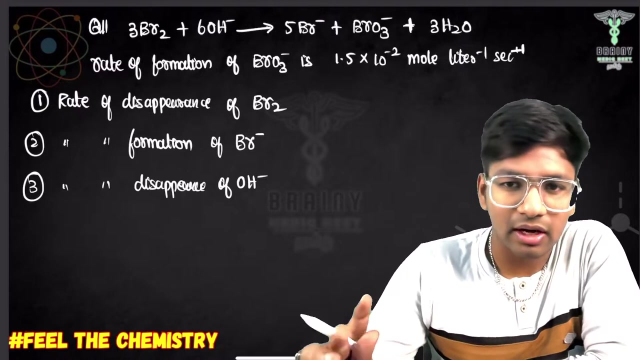 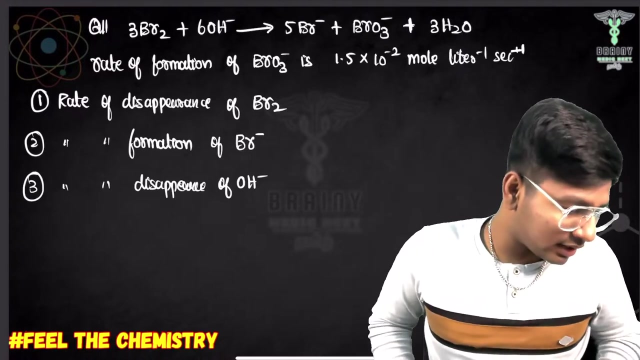 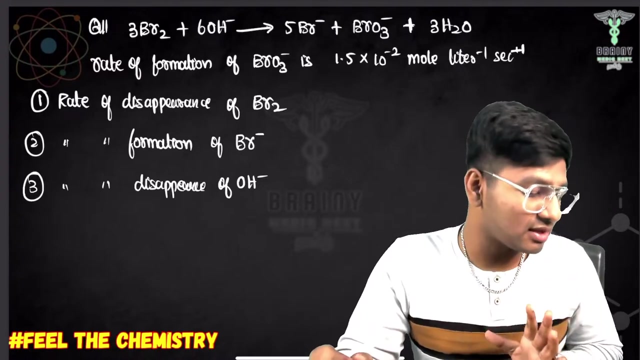 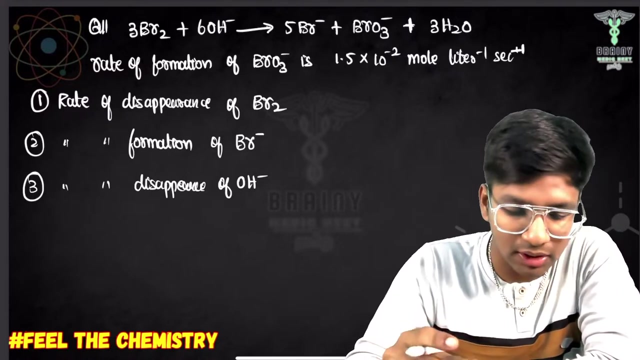 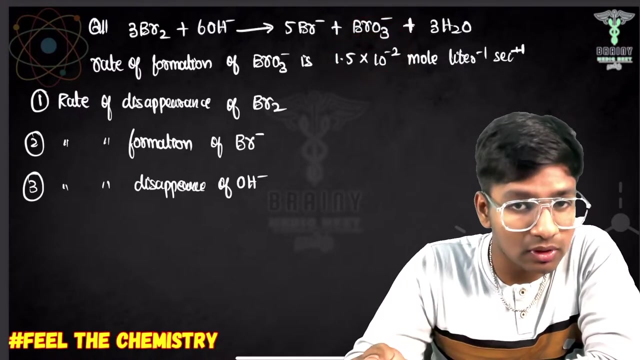 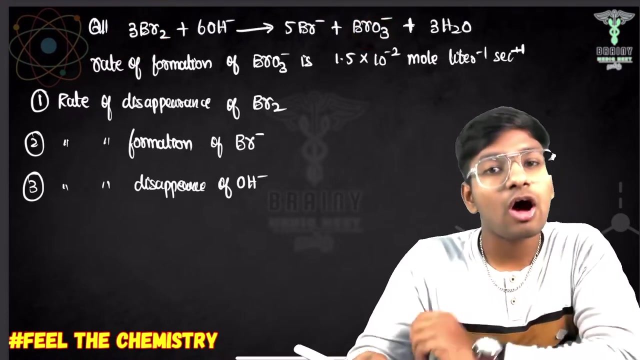 question: rate of disappearance of OH minus the moon amenity: conducive solar port. oh, oh, oh, oh well, I mean the question again. we're listening time for this question. you, you, you, you, mmm, Thank you for watching, Thank you for watching. Thank you for watching. 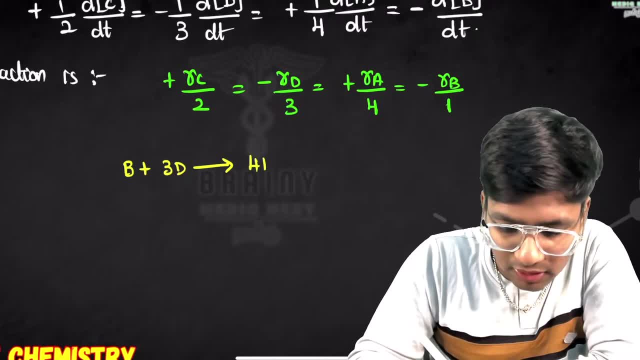 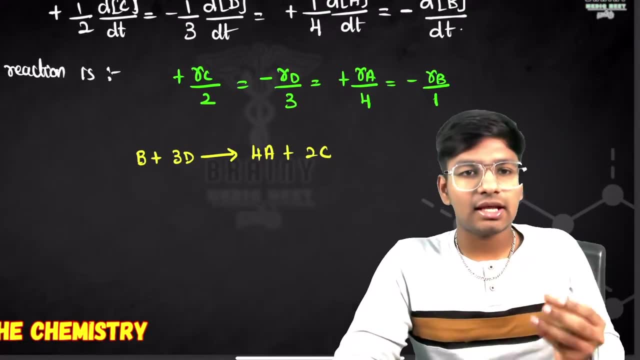 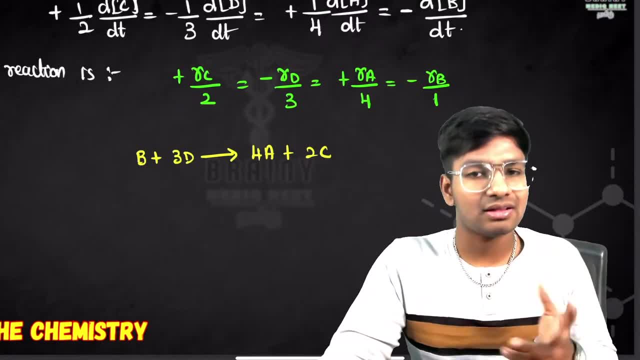 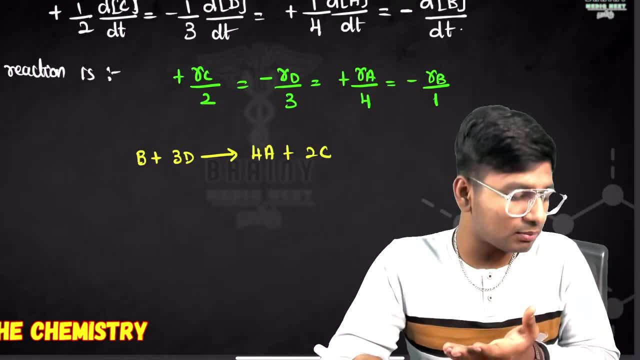 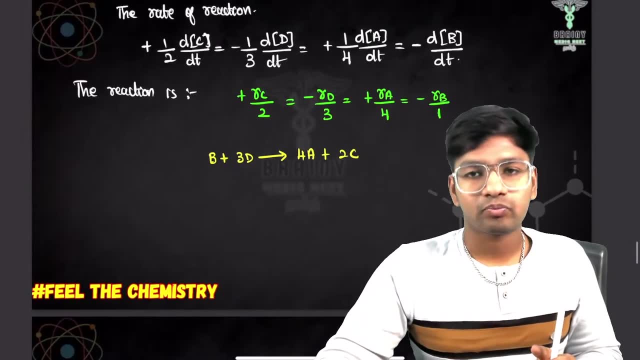 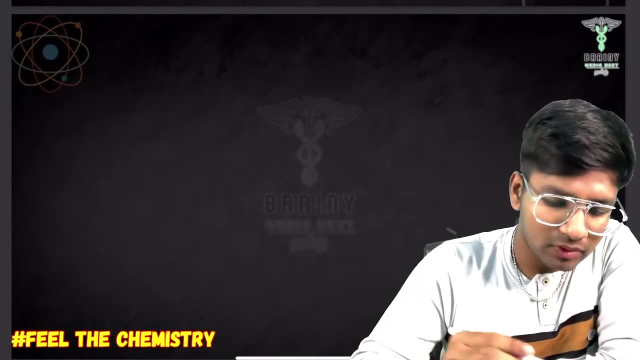 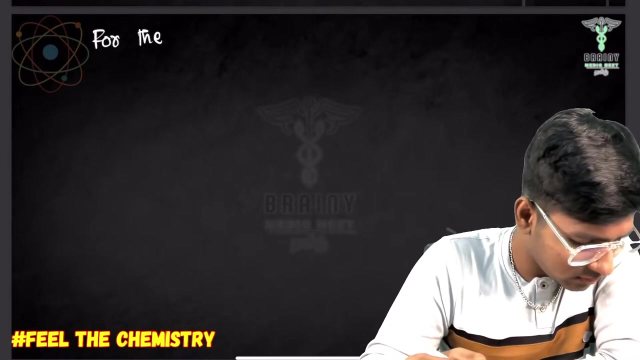 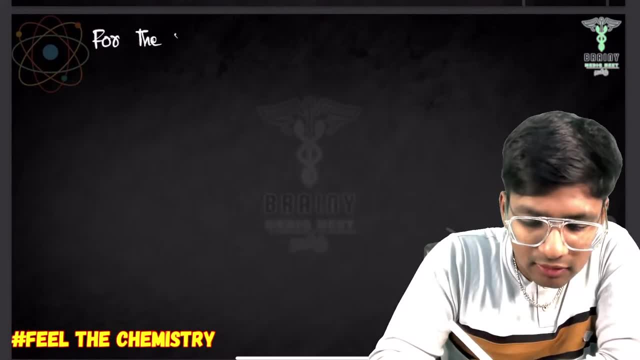 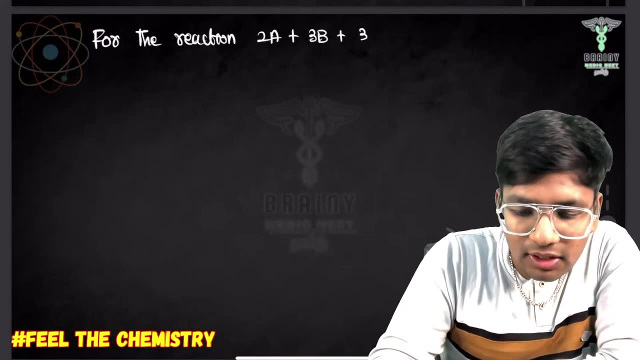 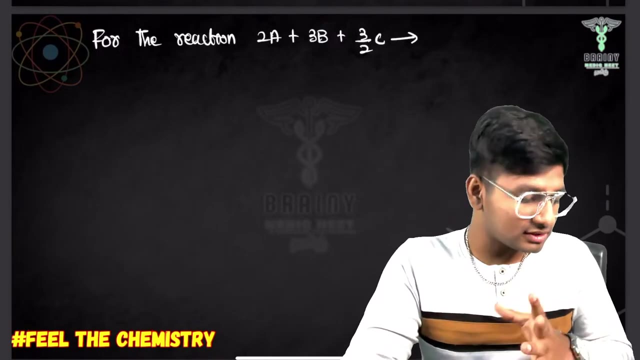 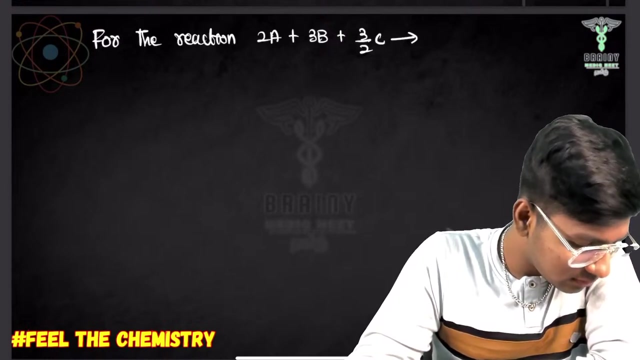 enemy or a movie camera company or in class for the reaction to a plus 3, B plus 3 by 2, C is a long question. I either. the options are options are edited options, they were in it. you just answer: okay, now, so much concert, but also lead. 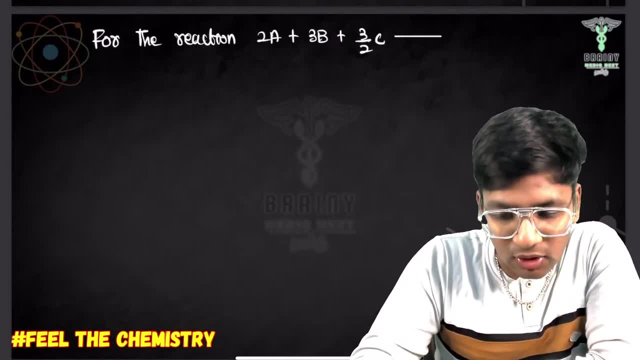 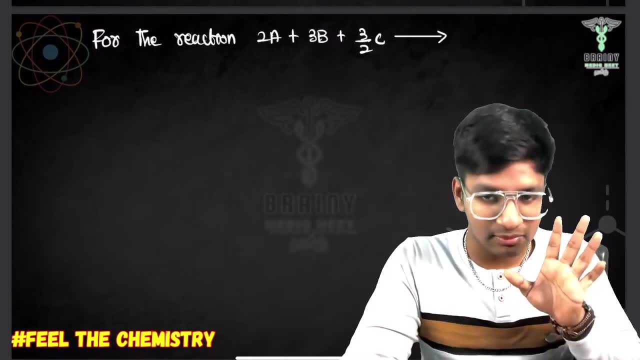 upon on the classic, even the earth, we know for it seriously. I'll search for the lectures in the lab which have more questions plus concepts on the market here. but on our peer to peer, depend on the lecture, on the time you like it. by night it come out to come out on the 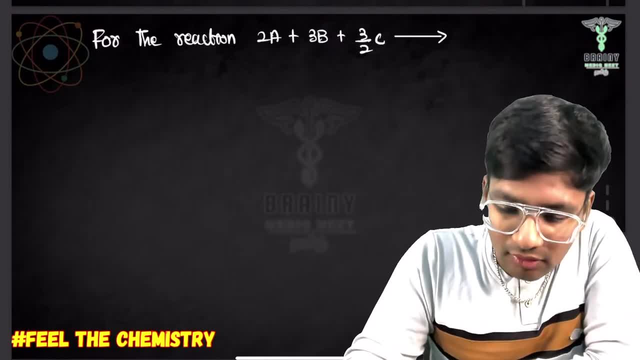 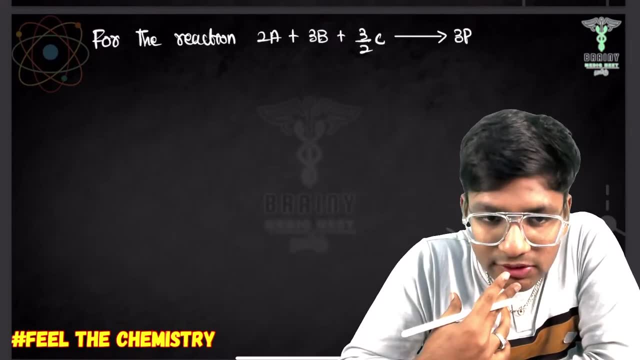 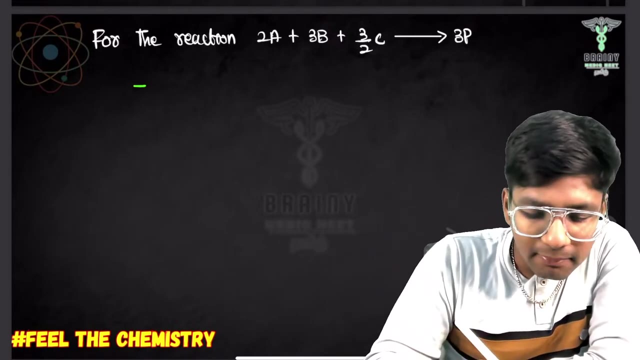 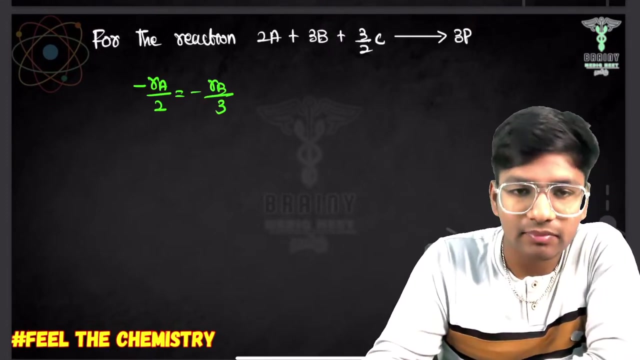 concept of what I explained: money today, yesterday, okay, even upon the 3p, put together it is a great solution at the auto question: rate, rate, rate rate. see again very easy question: minus of re a divided by 2 is equal to minus of our B divided by 3. 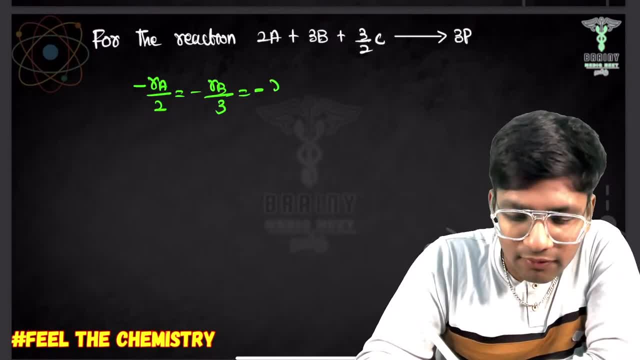 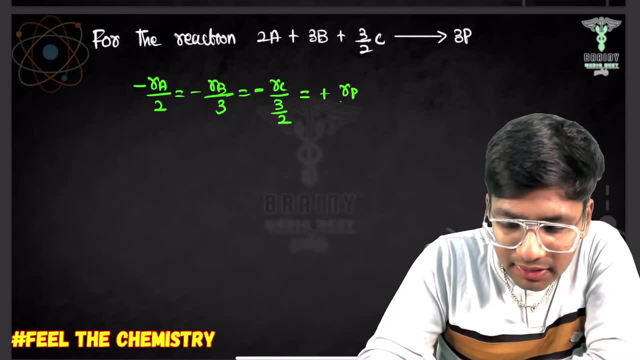 okay, which is equal to, which is equal to minus of RC divided by 3 by 2. correct, a 3 by 2, which is equal to plus of our P divided by 3, plus of, okay, plus of our 3, sorry, our P, divided by 3, you know, I know. 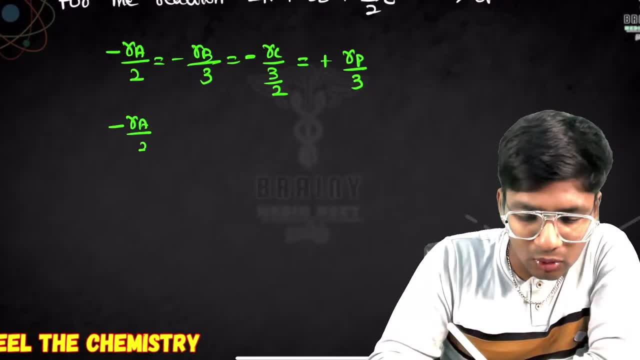 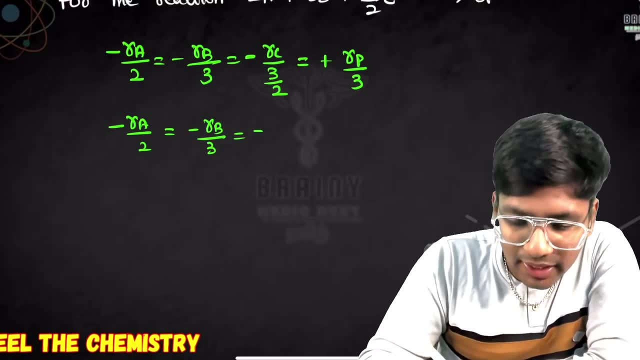 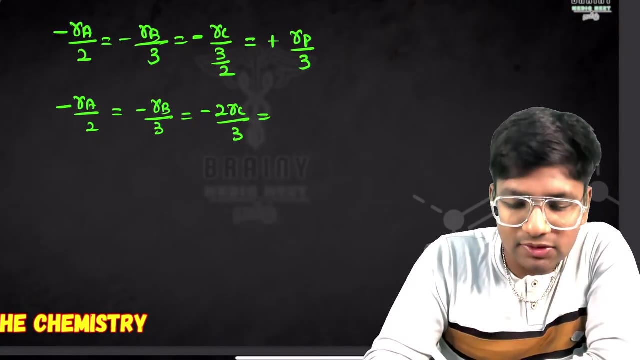 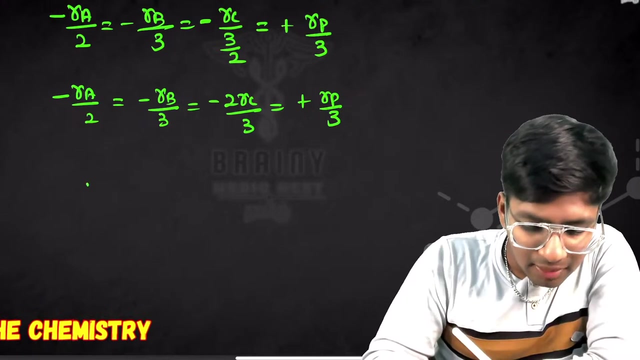 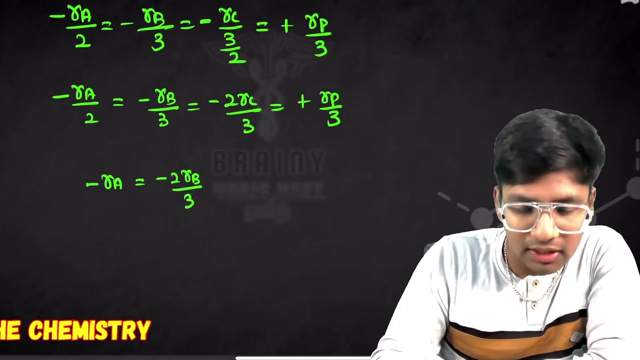 simply for me you're gonna be now re: a divided by 2 is equal to minus of our B, our B divided by 3, which is equal to minus 2, the 3 by 2 matter for it. okay, three seven, which is equal to 3 by 2. now it says 36 Beautiful. 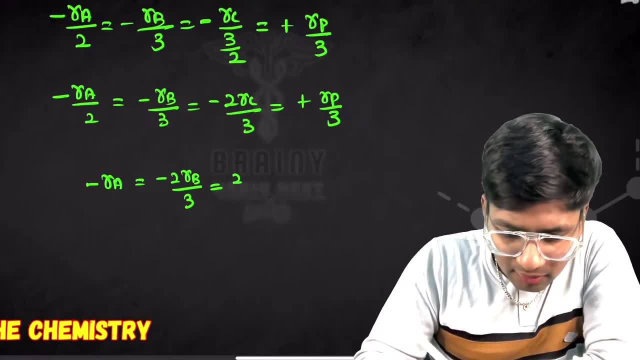 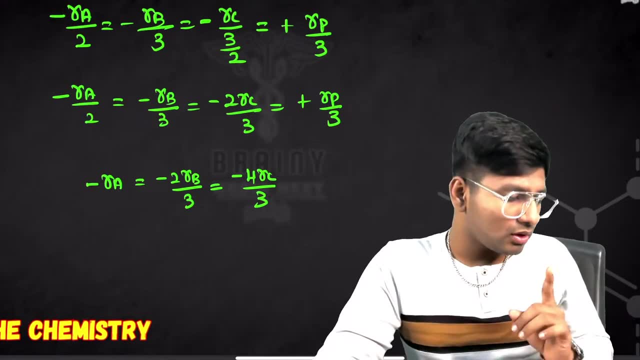 B divided by 2 minus R. a by B divided by 3, which is equal to most of our P parler by three. okay, this is the emotion. you will not be 4RC divided by 3. they will give like this: ok, mathematics, mathematics is all mathematics. 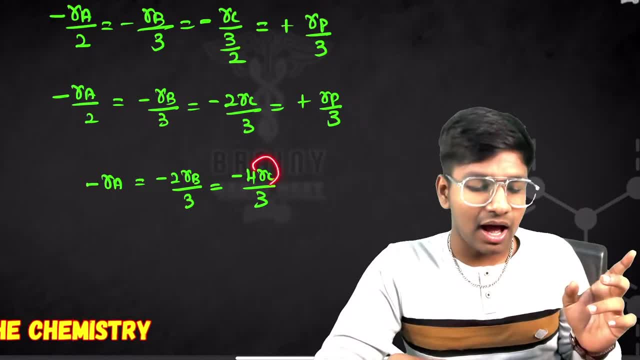 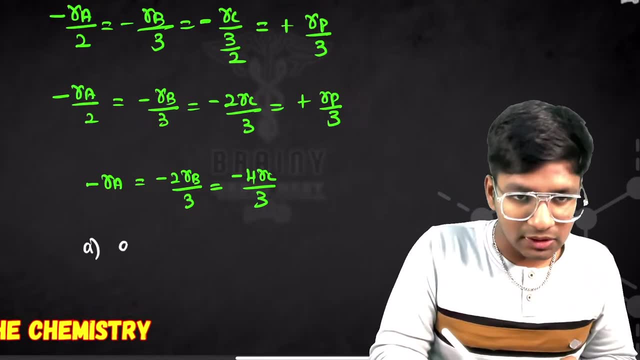 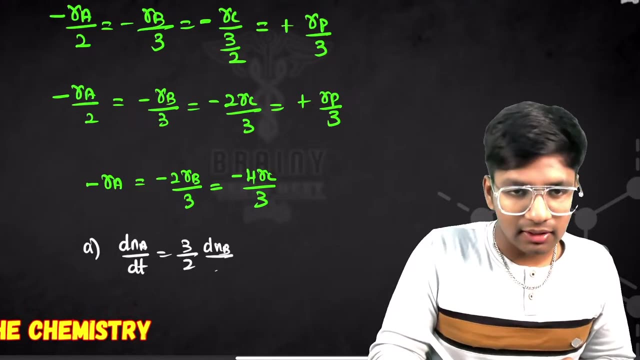 then another thing is they will not give RARC. how will it be? I will tell you what is in the option. it will be like this: dNa by dt is equal to 3 by 2 dNB by dt. it will be like this only if the rate is equal. 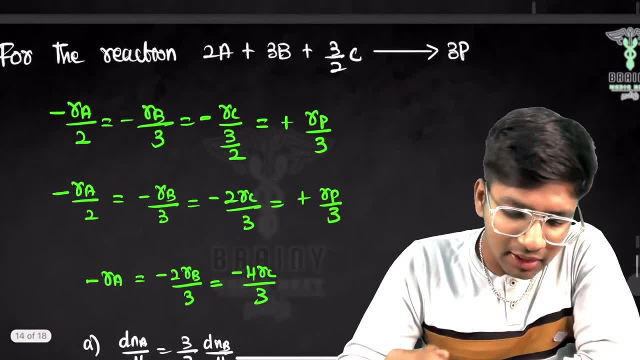 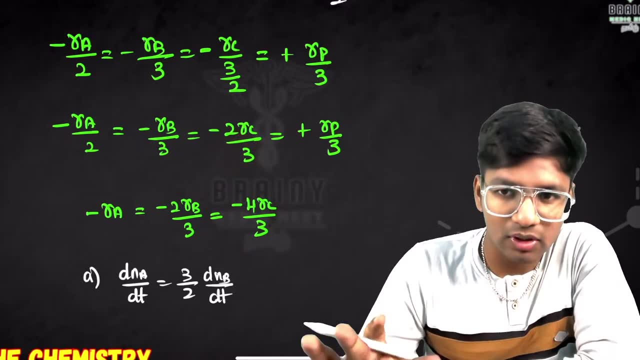 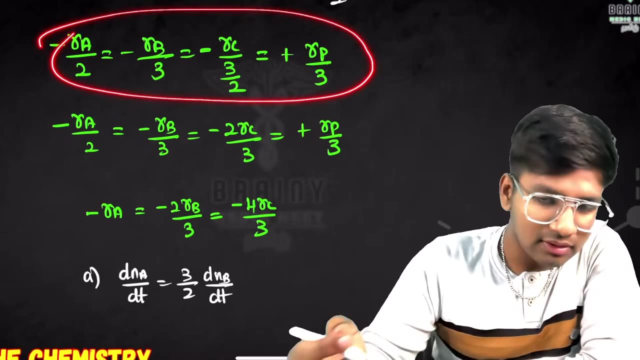 then we can divide the coefficient. yes, I have made all the rates equal. I have made all the rates equal. I have divided the coefficient simple. I have done what I said. if the rate is equal, yes, I have made all the rates equal. I have made all the rates equal. 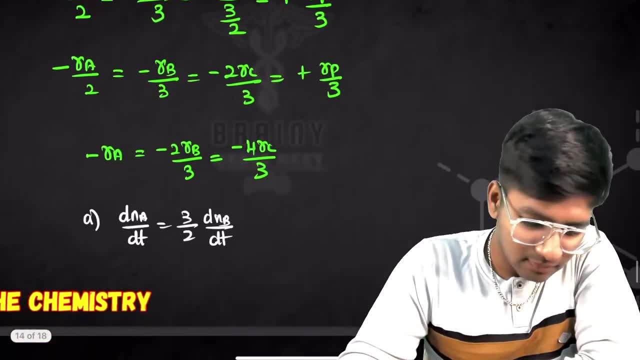 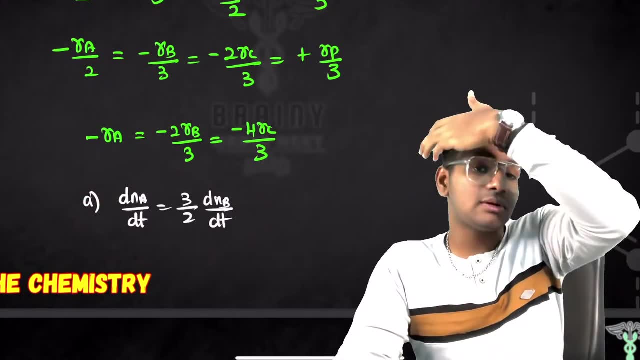 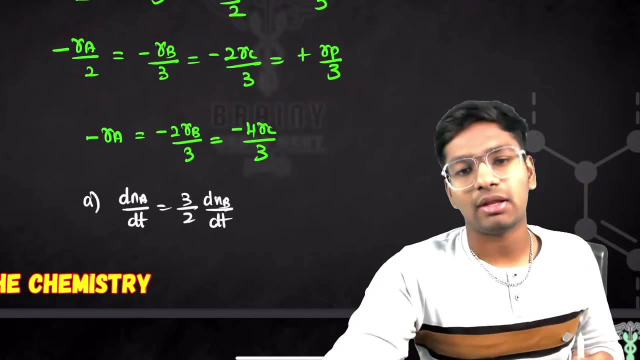 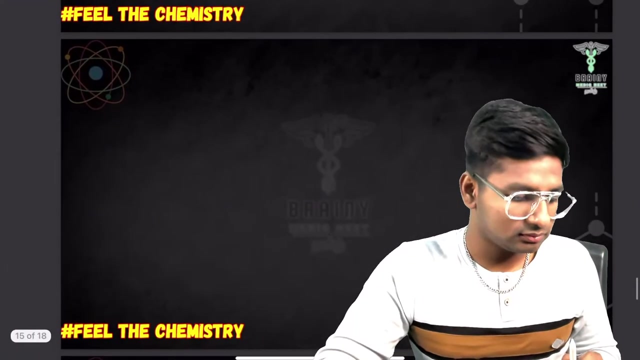 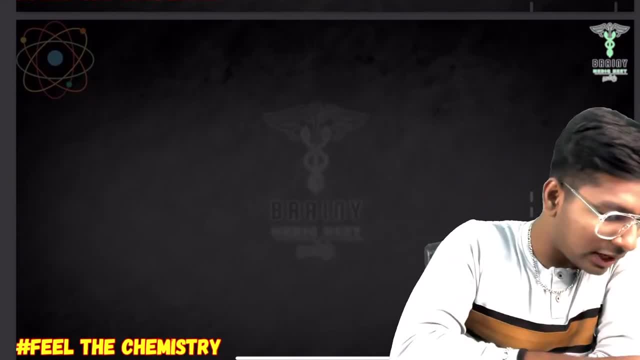 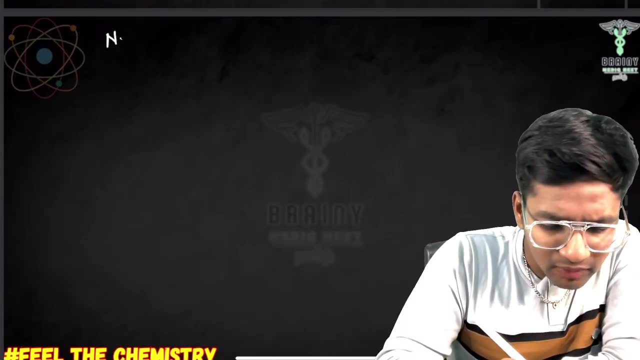 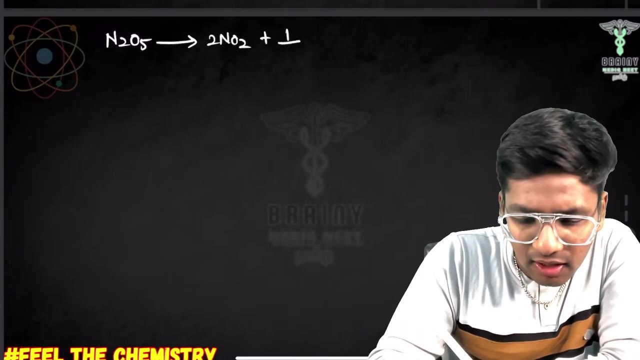 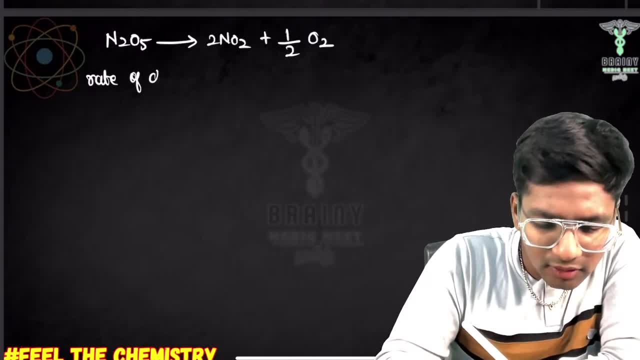 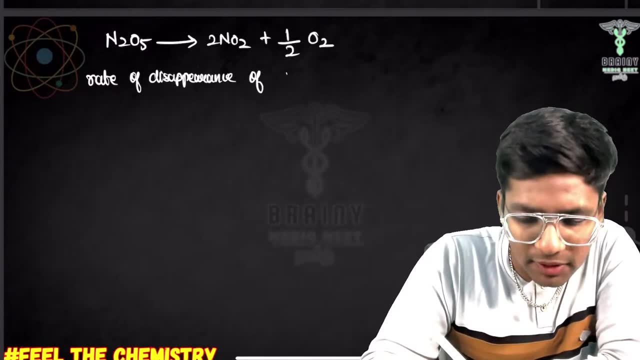 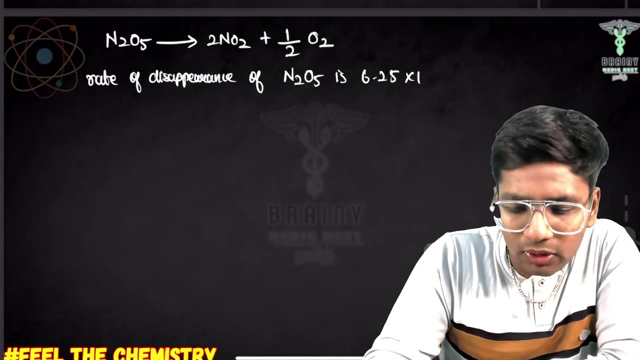 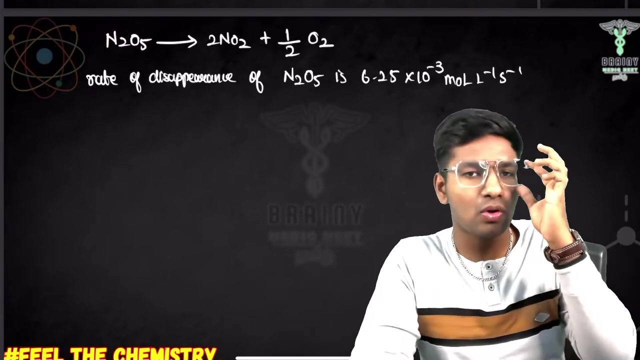 So rate of rate of disappearance, of rate of disappearance of N2O5 is 6.25 into 10 power minus 3, they have given, ok, mole liter inverse, second inverse, ok, this they have given. 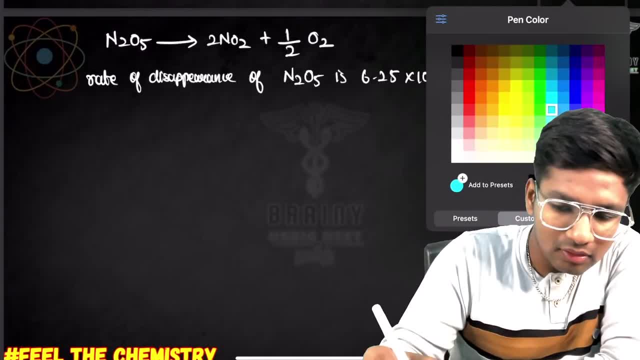 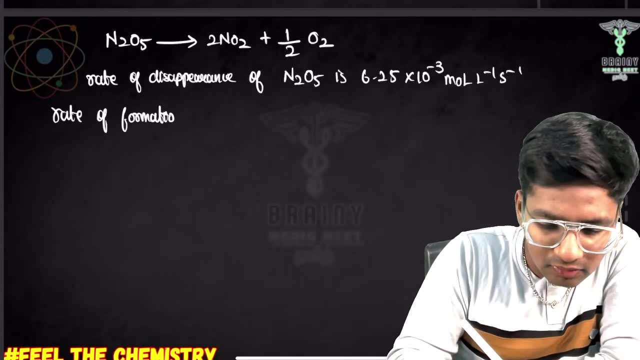 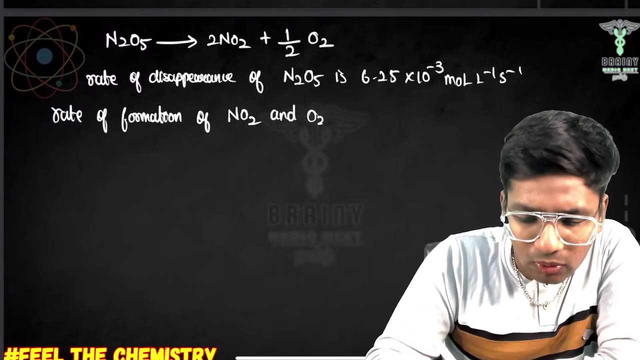 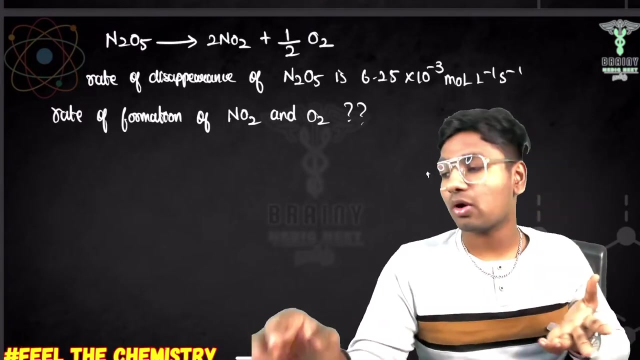 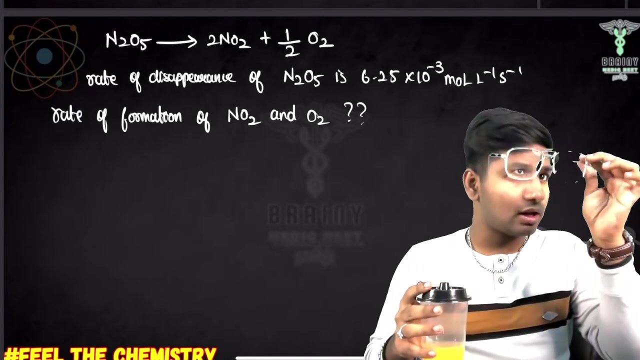 So what are they asking in the question? what are they asking in the question? They are asking rate of formation, rate of formation of NO2 and O2, they are asking you in the question. answer me rate of formation. they have given the value. they are asking you the rate of formation. ok, they have given the value. solve it in our method. solve it in that method. take time. 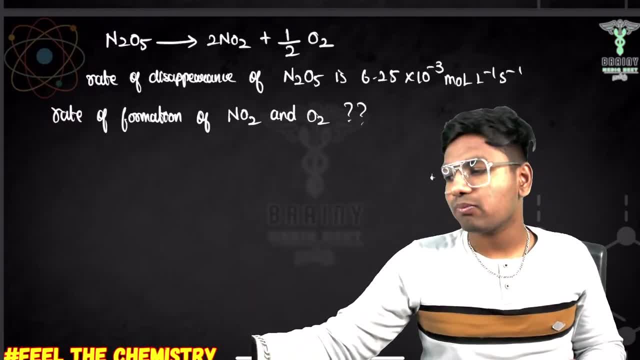 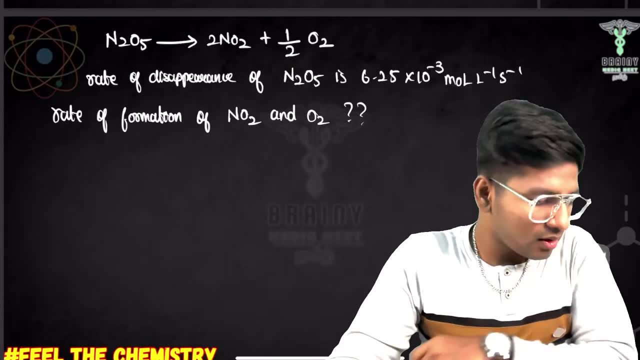 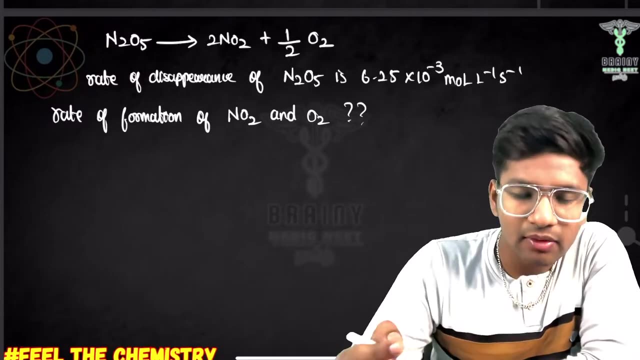 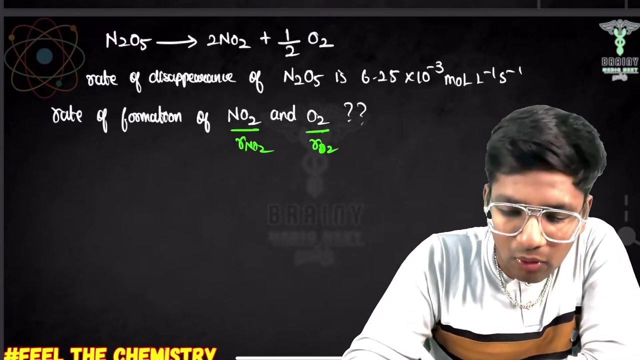 Anyone answered See. very simple question again. very simple question again. See, here they are asking for these two RNO2, R02,. this they have given RN2O5, correct, john, So R N O two. 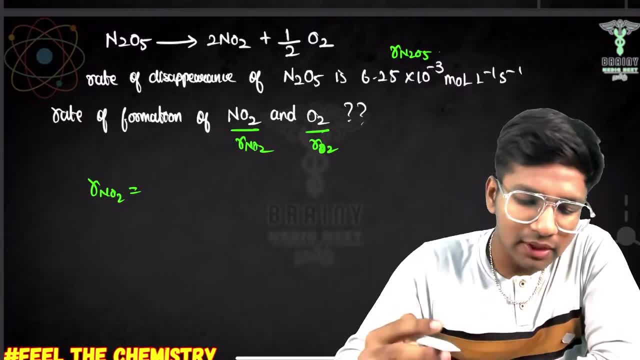 particular, and R, N and N 2 is equal to rate of formation of NO2, see moles. see here 1 and here 2, multiply by 2, that's all 2 into 6.25. 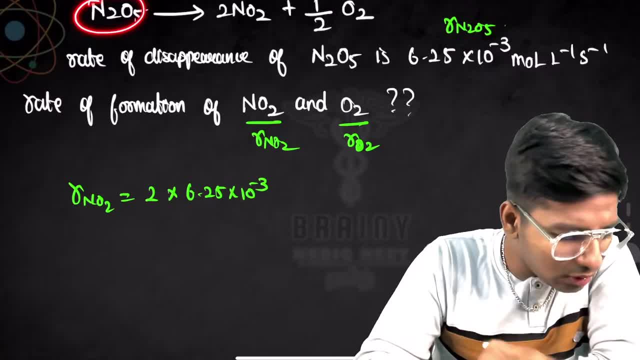 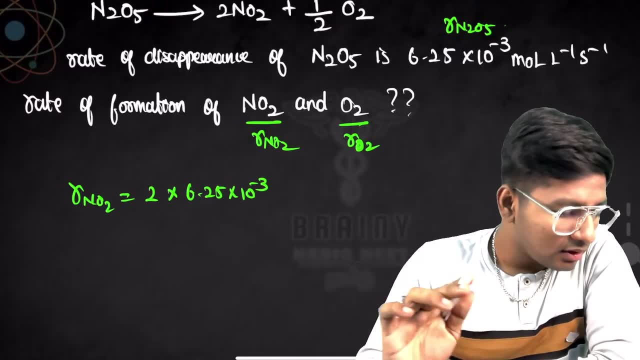 into 10 power minus 3, here, if this mole is 1, this is in 2, correct, then double the moles, then double the rate. correct, moles are double. if moles are double, then rate is double. 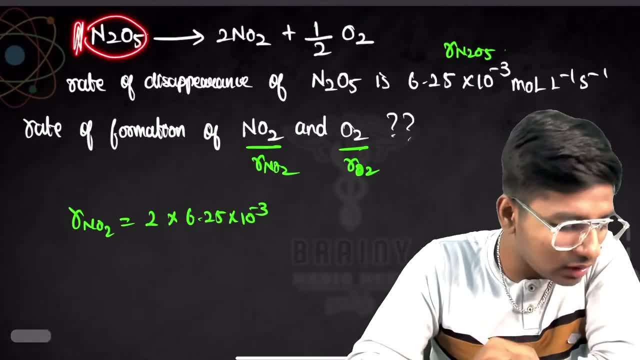 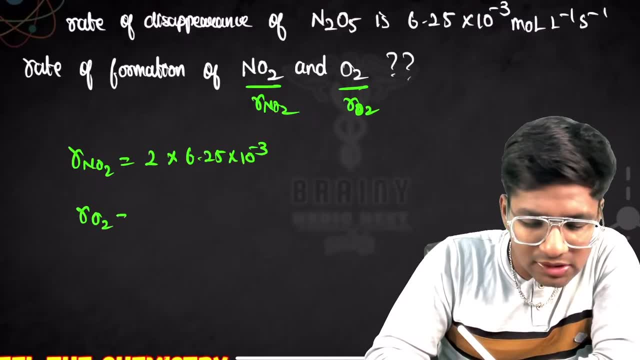 next see here: if this mole is coefficient 1, then this coefficient is half, then rate is also half correct rate is also half. then R O2 is equal to half of 6.25 into 10 power. 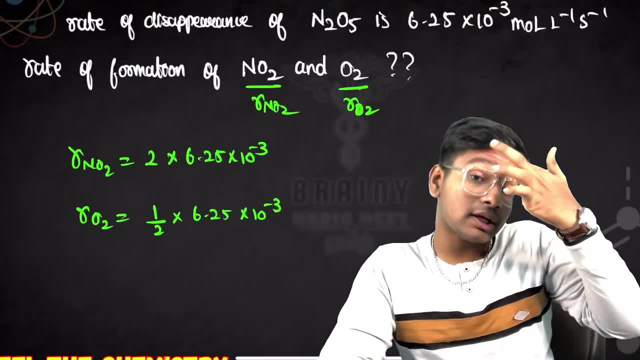 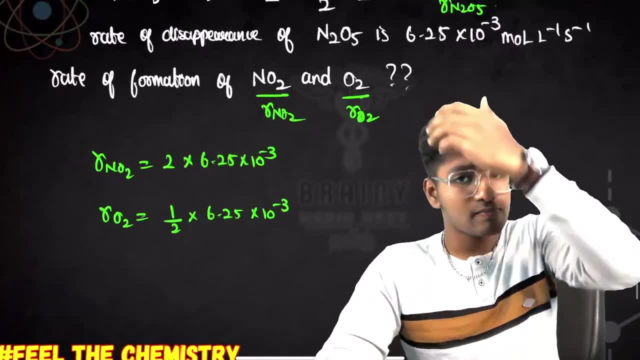 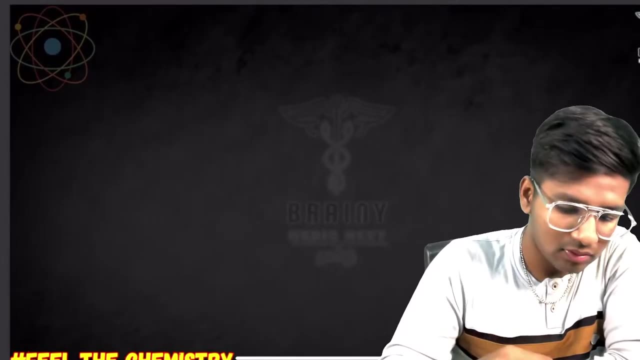 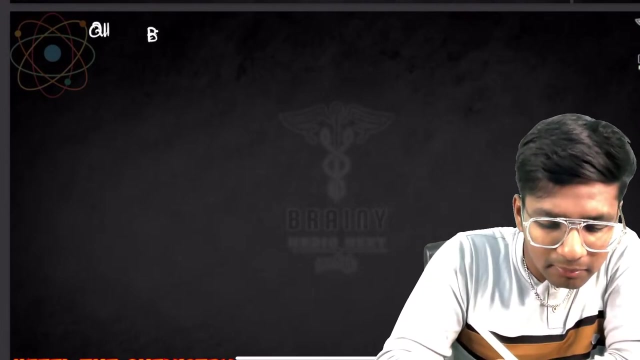 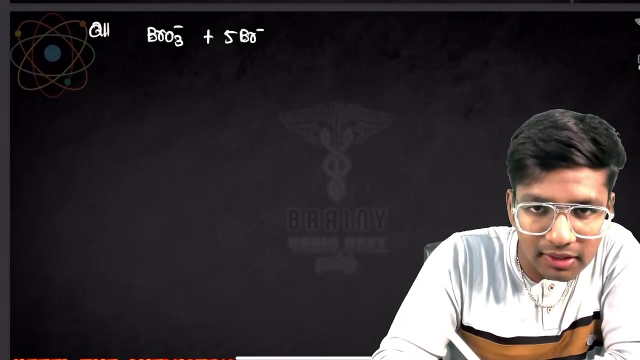 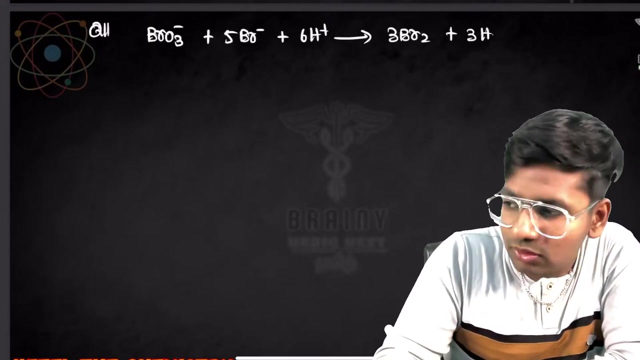 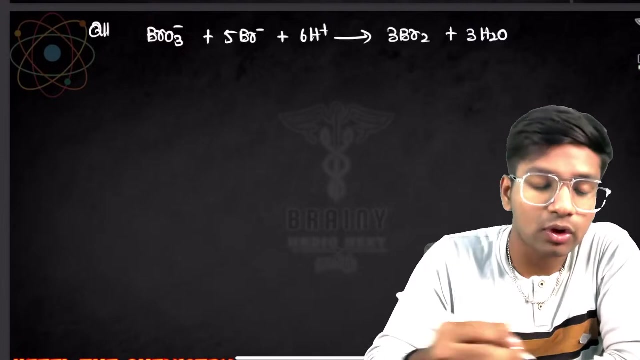 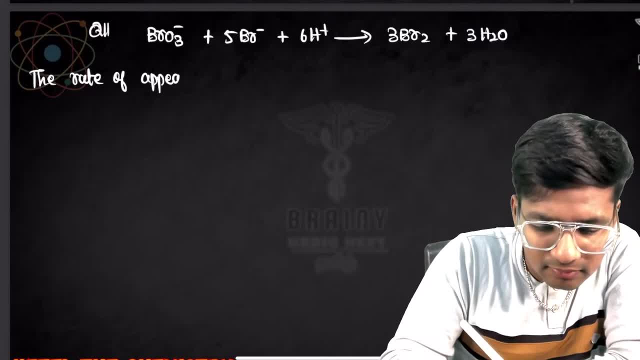 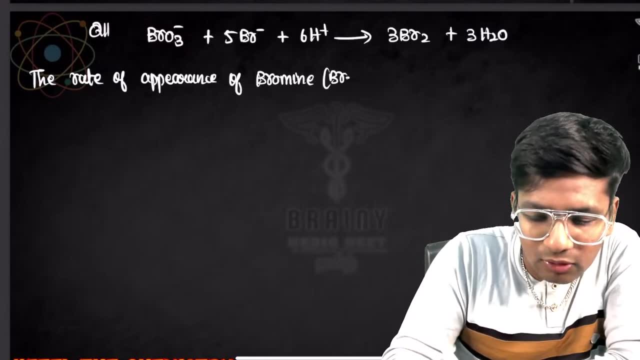 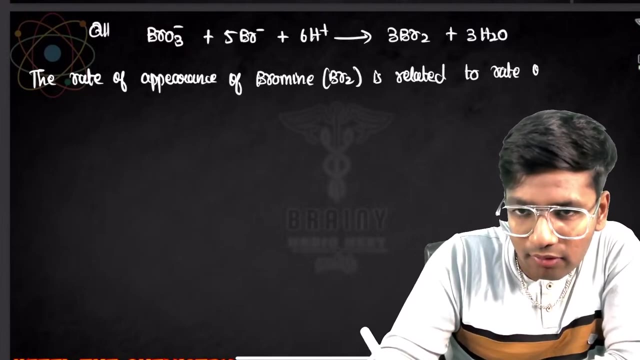 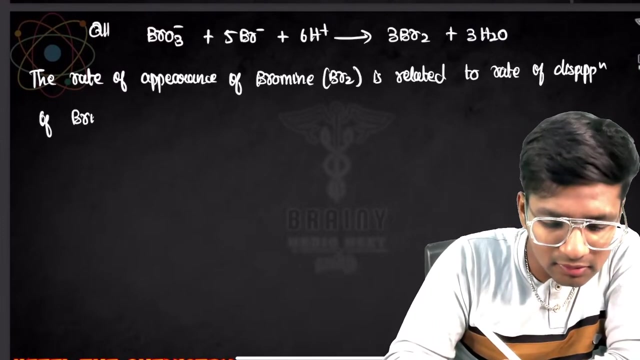 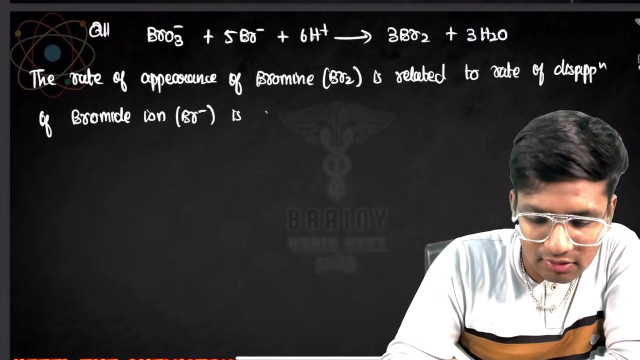 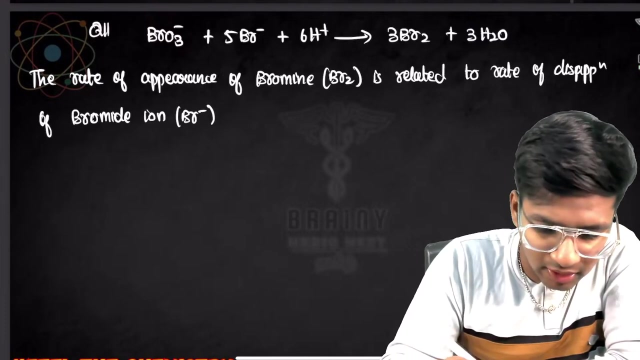 Rate of appearance of bromine, that is, Br2, is related to rate of disappearance of bromide ions. ions that is Br minus, okay, bromide ions- Br minus. how you will relate- this is your question- is as follows: why all these question mark? this is your answer. 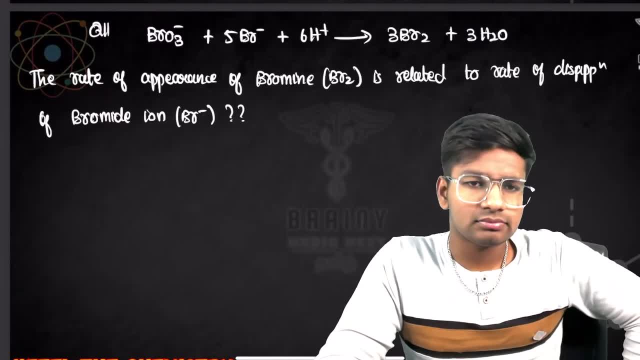 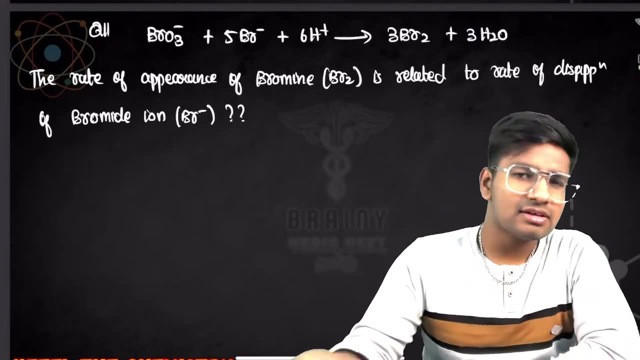 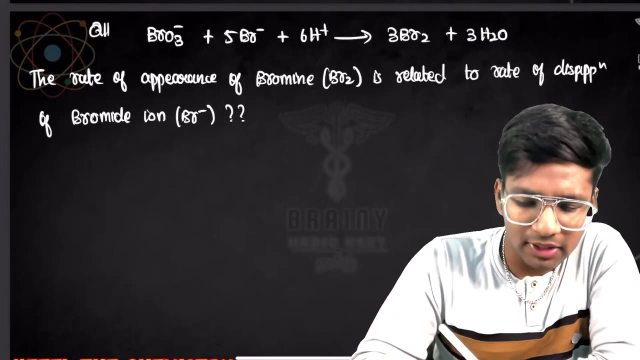 very simple question again: how you can relate this Rohit 3 by 5 times. wow, what will answer on the clip? nice, very simple, right. it is a kind of a trick class with either the button answer part of the government, you part of an interior bromine, bromine given up in our BR 2. 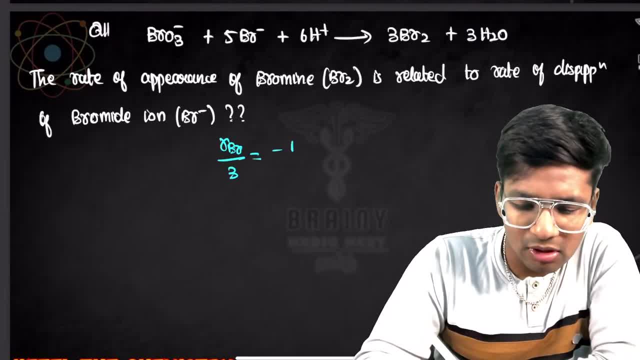 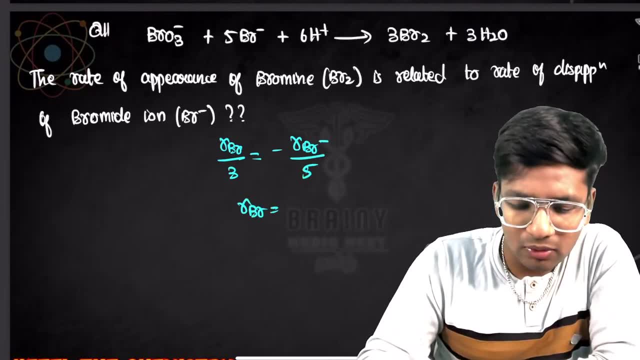 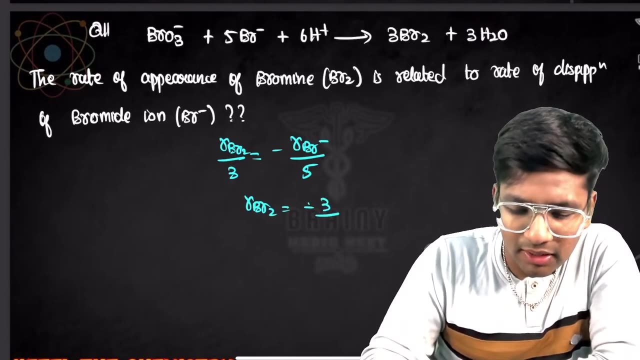 divided by 3 is equal to Bromide ion minus of Br minus RBR minus RBR minus. divided by 5 in the way up, our BR is equal to BR le BR 2. sorry, RBR 2 is equal to Br minus of 3 by 5 RBR minus. it is already given. our own, it is already given. 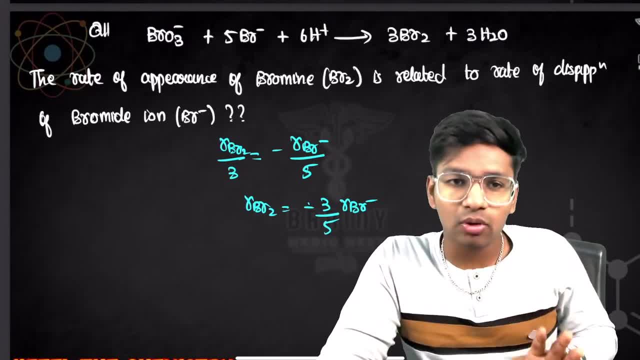 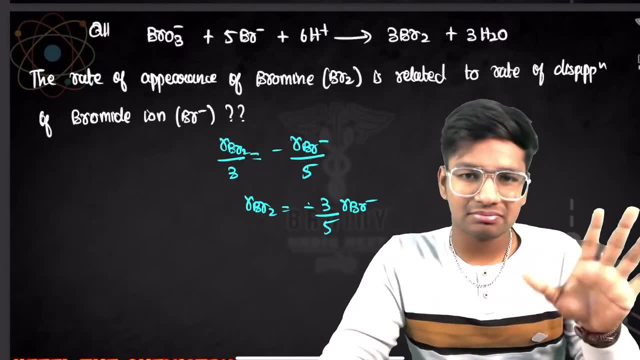 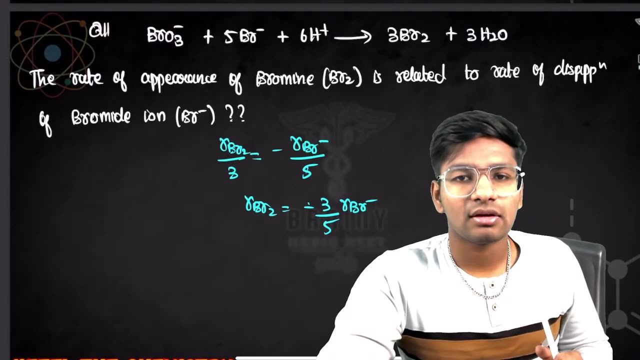 our own simple, but in the Marley RR now we could come at a D of bracket le BR 2 divided by D D D of BR minus divided by D D of being put up on the path. only answer money right now. correct up done in the my question. get answer funny via in the. 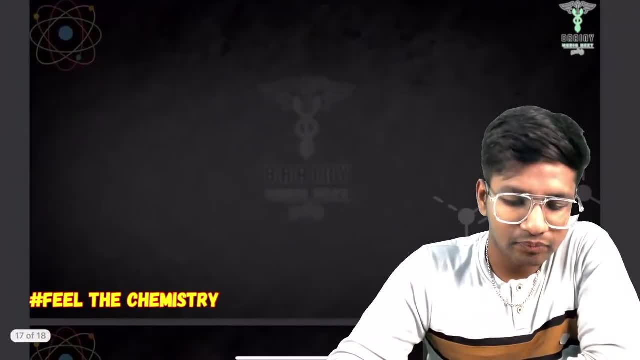 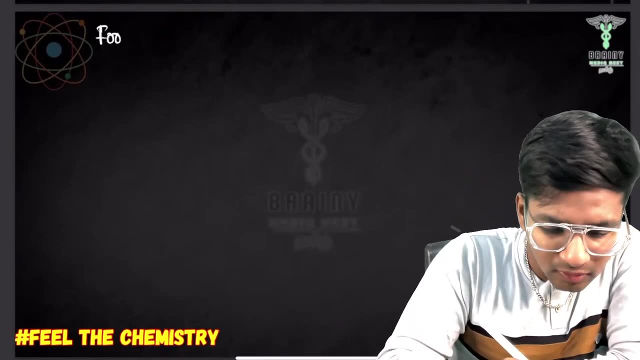 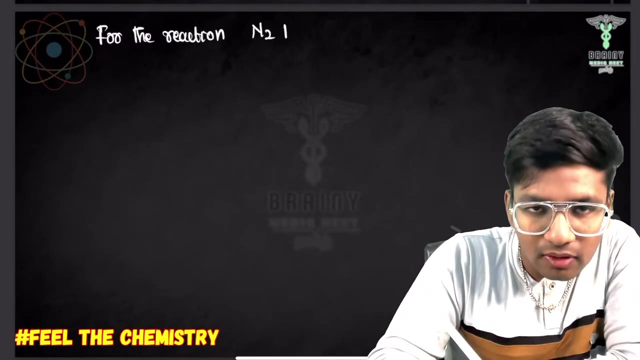 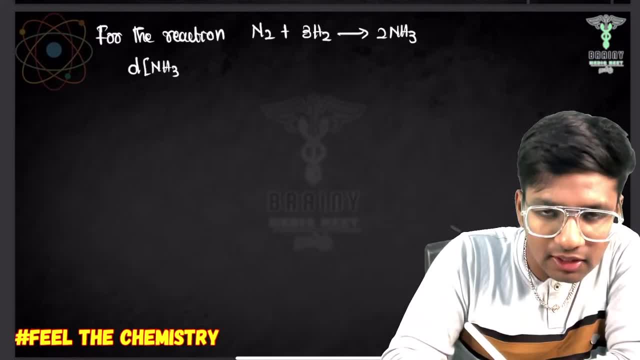 give. we are clear concepts of reaction. N2 plus 3h2. give. we are clear concepts of reaction. t of n. h3 divided by DT is equal to two into 10 x minus 4 d. совет by Eаны and Yoonevich. he or an inter ul paper. e avaa in inability to read for a two into 10 to minus 4. Eana and h3 divided by DT is equal to two into 10 power minus four. it is obstructs Hunter theory from B gear it now the. it is the finds a higher lake near звонIC, the last. 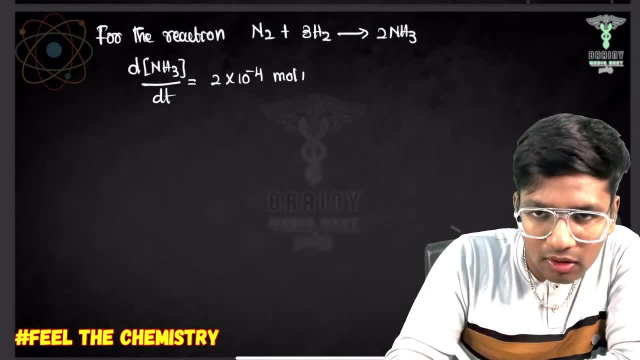 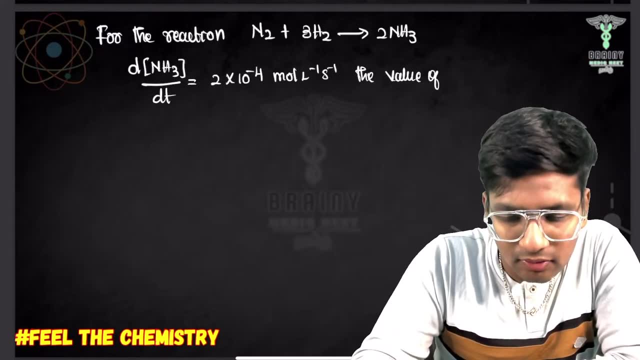 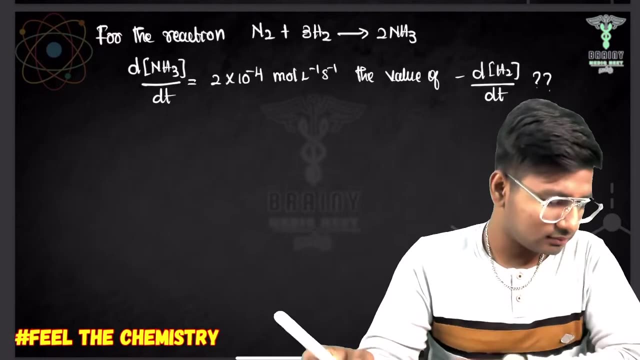 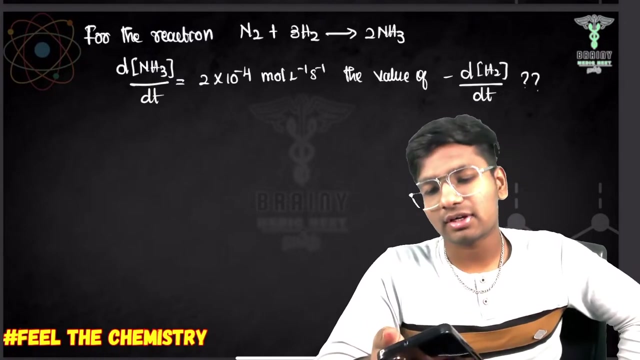 10 power minus 4 mole liter inverse. second inverse: the value of minus of d of h2 divided by dt. that is your question, very simple question. again, this is a simple question, simple question, suppose. if you understand that method, it is very easy, we can answer it easily. 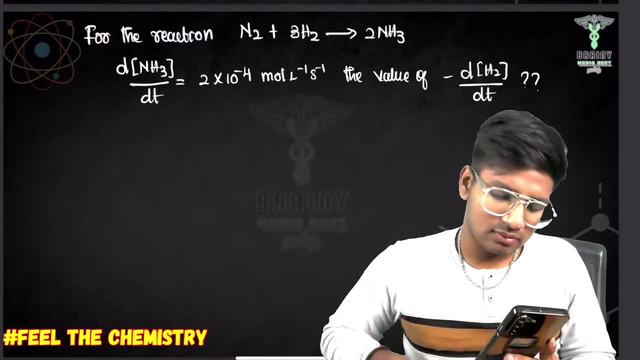 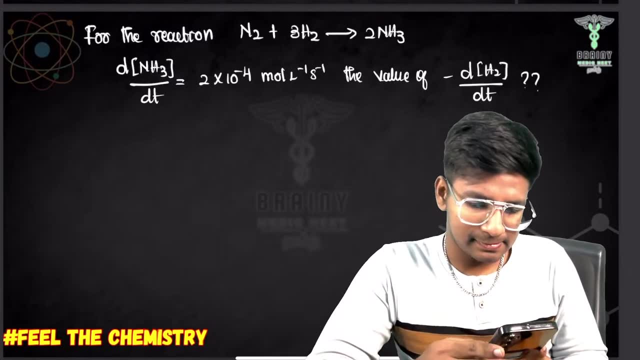 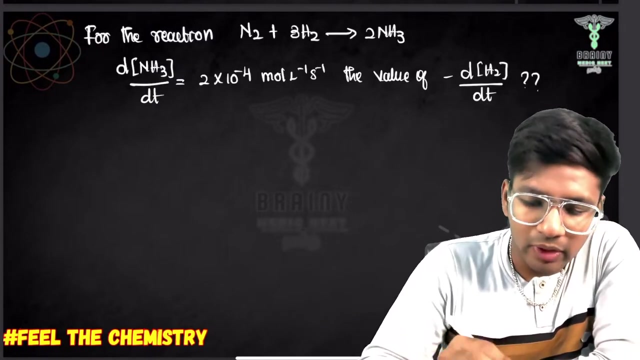 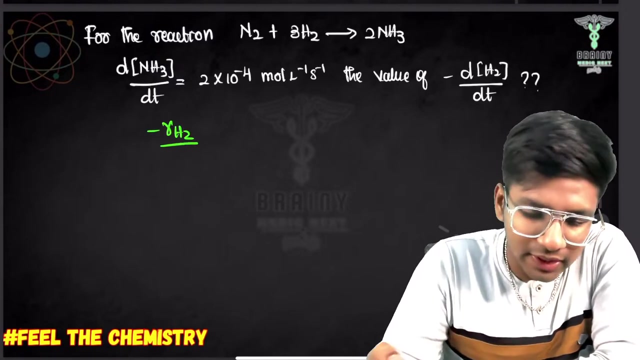 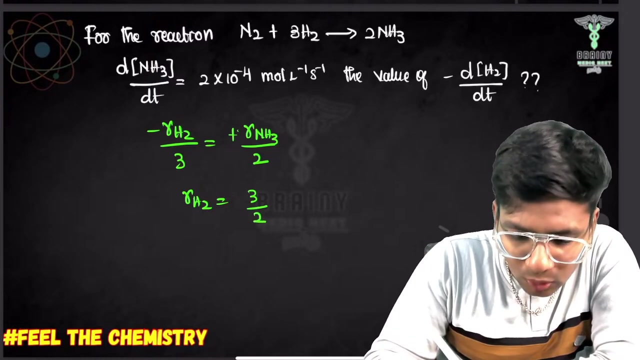 thank you, very easy question. so see again the same method. minus of h2. rate of h2 divided by 3 is equal to plus of rate of nh3. rate of nh3 divided by 2, rate of h2 which is equal to 3 by 2 times. 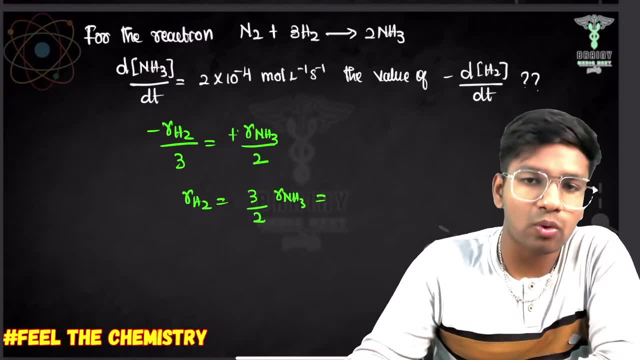 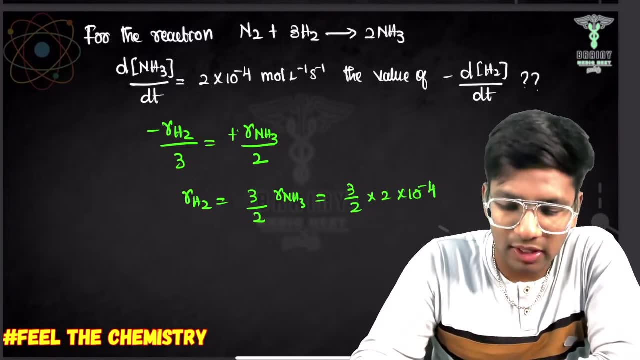 3 by 2 times 3 by 2 times of rate of nh3, of rate of nh3. in your question you have given everything. then 3 by 2 into 2, into 10, power minus 4. that is your answer, which is equal to. 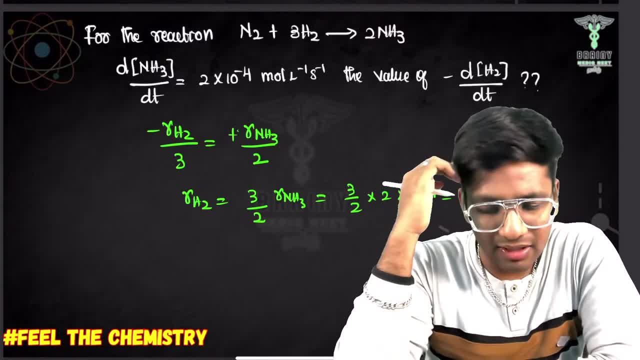 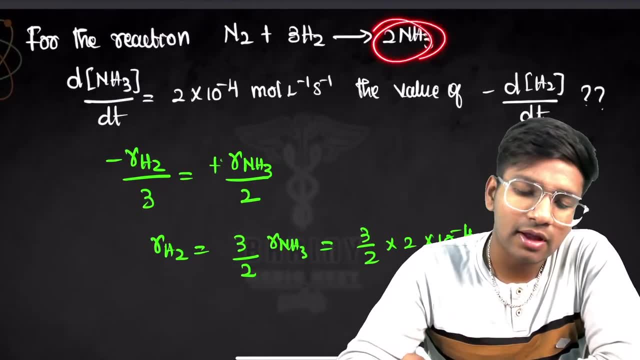 minus 3 into 10 power minus 4, rate is not in negative. so directly write 3 into 10 power minus 4. is it not like that? we can write it as we see. rate of this is in 2 times. we can write as we see. 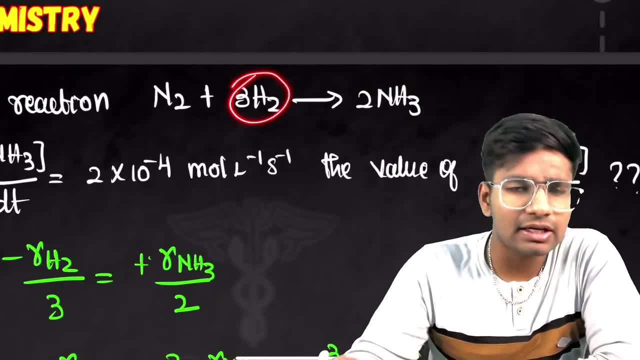 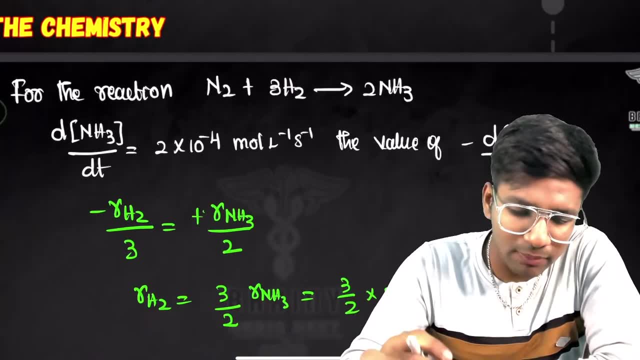 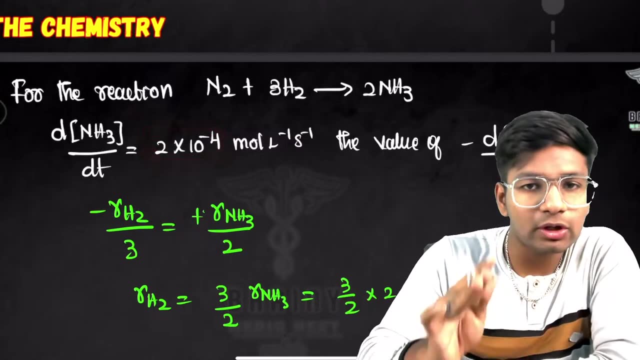 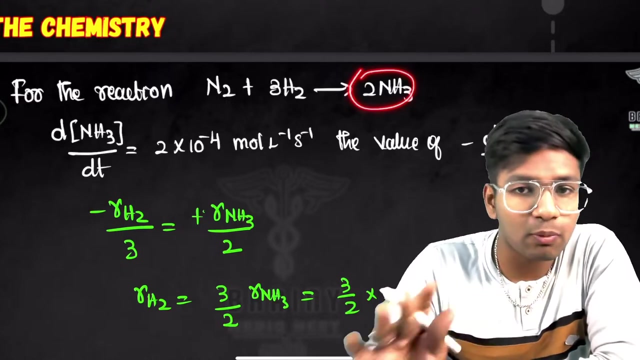 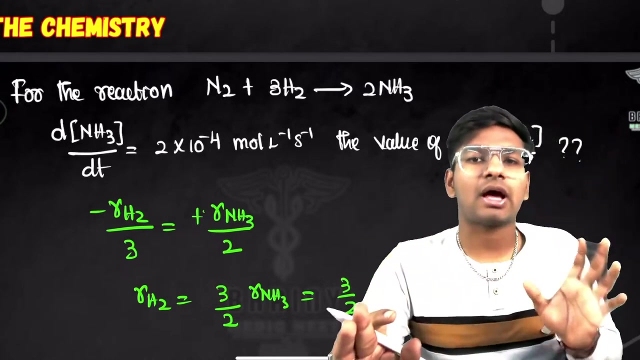 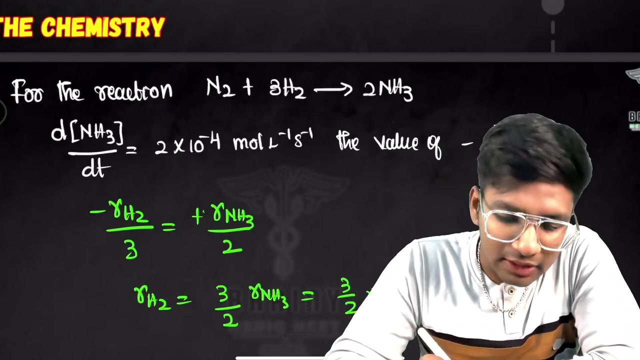 this is 2 times, this is 3 times multiply. this is over ok, one. you can write: respect 2 ok if you do this. so this is perfect, perfect answer. If you want to change this to 1 ratio, then it will come down correct. 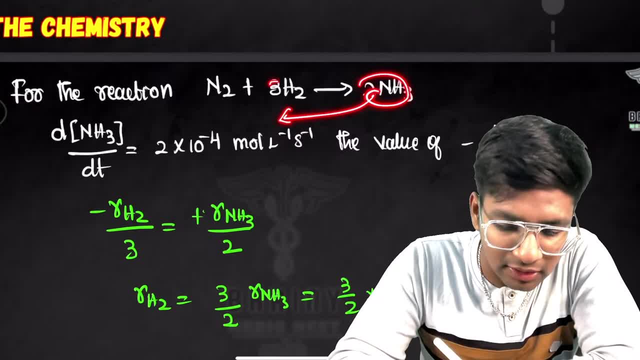 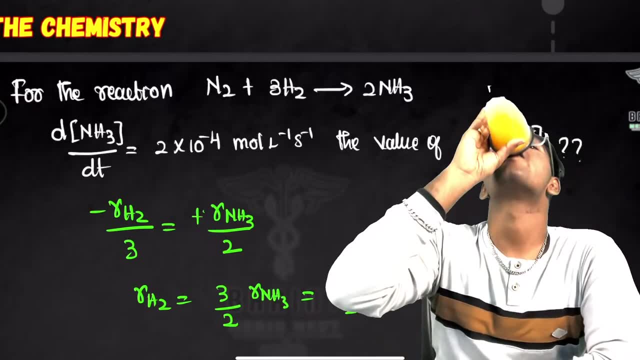 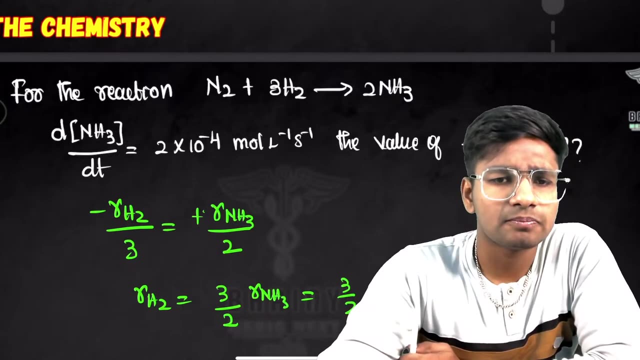 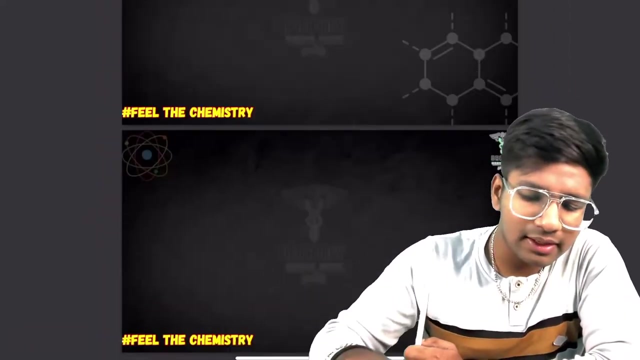 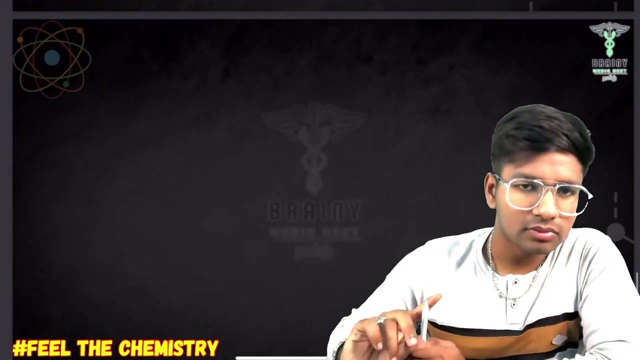 Do you understand what I am saying? If you want to change this to 1 ratio, then you have to take this down and put 3 by 2, only then the ratio will be balanced. Next, there is another concept. This concept is not asked in NEET, but there are chances to be asked. 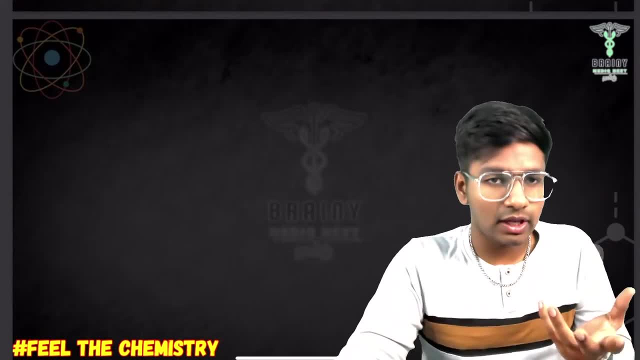 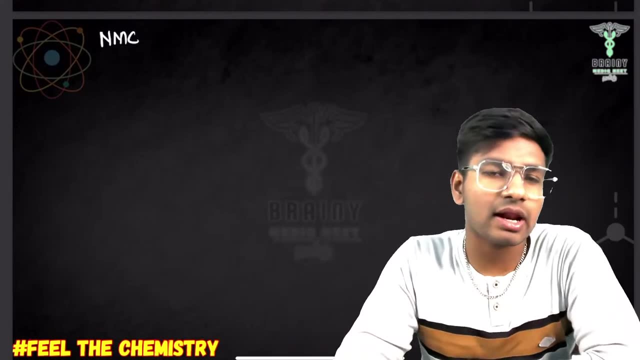 This concept is not asked in NEET, but there are chances to be asked Because the patterns have changed and many things have happened in NEET. So this concept was asked in JEE twice, But this concept is not asked in NEET. 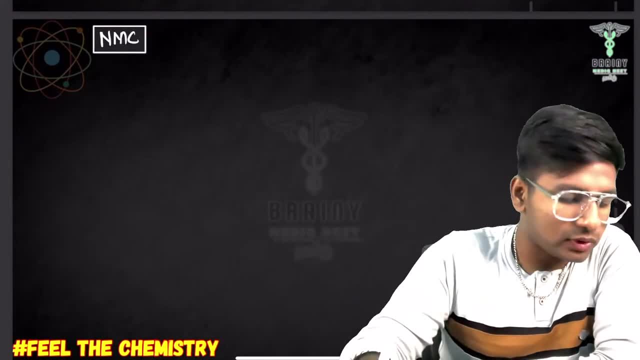 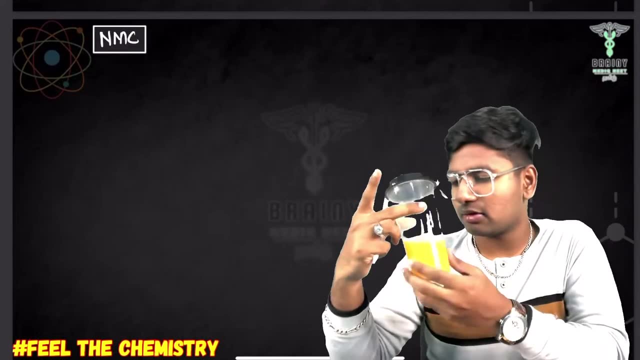 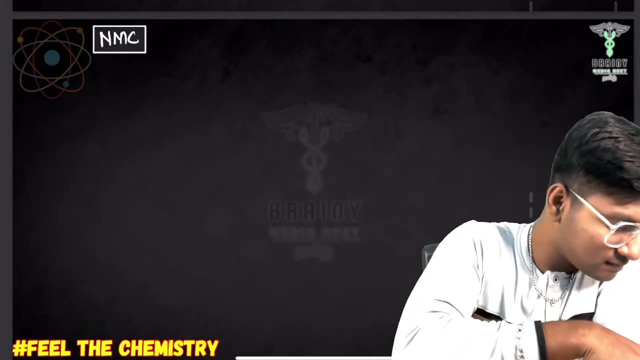 So someone asked this question in a difficult way. Now there will be a question in this pattern in NEET: This is not cold and this is not pure. This is not chilled. This is not chilled and this is not pure. It is just Citrus. 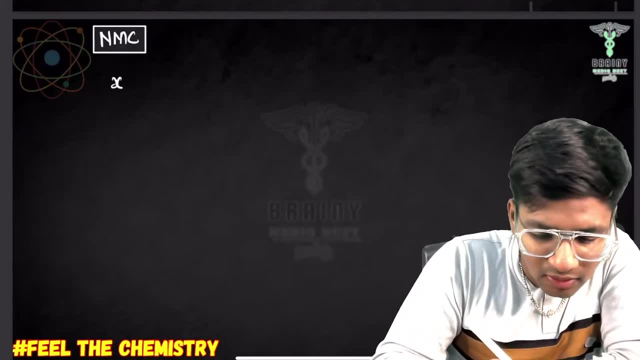 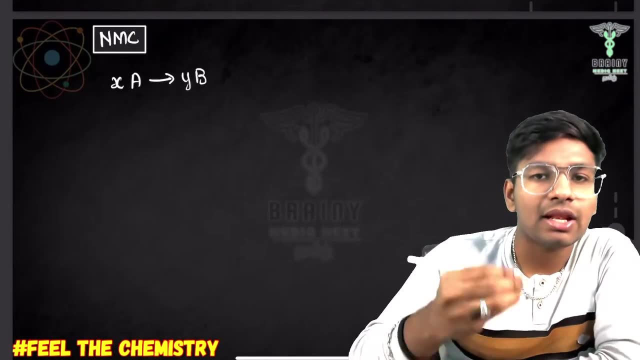 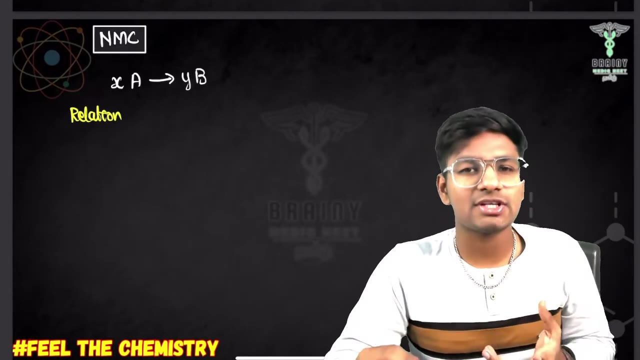 So see: X of A, X of A gives Y of P. This is your Reaction. In this reaction, what am I going to do? Relation between Relation, Relation between. I am writing the question without telling you the concept. Wait, I will tell you the concept first. 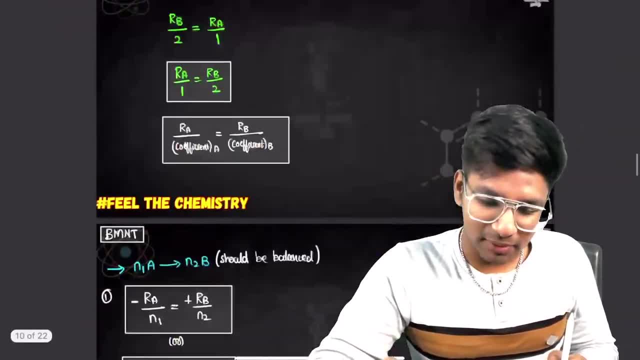 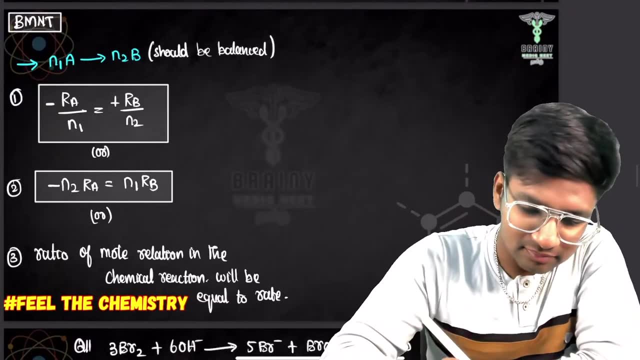 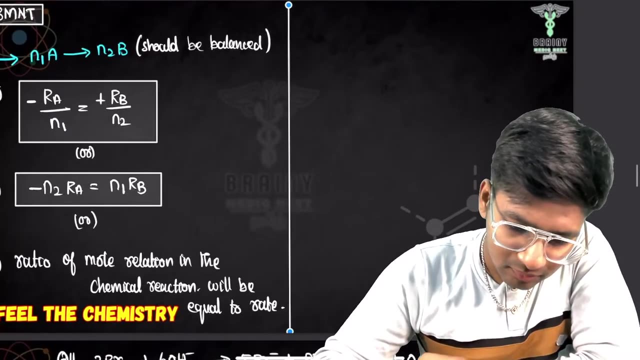 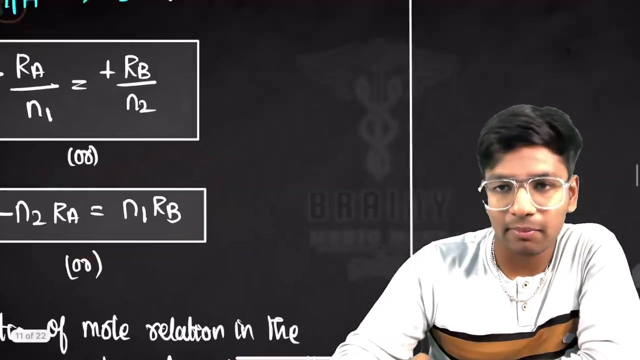 Where is the concept? Here it is. What am I going to do with the concept? I am going to write it here: PMNT, PMNT, PMNT. What will they do with this format? They will multiply this format with log. That is all. 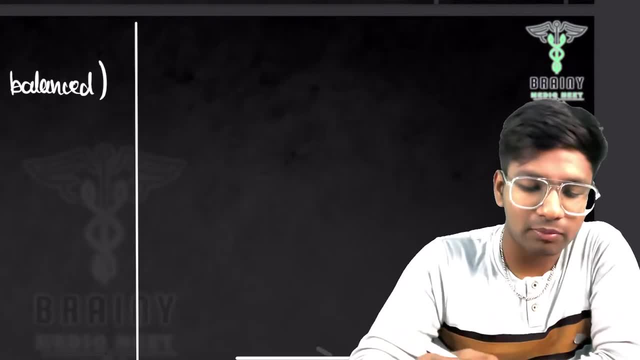 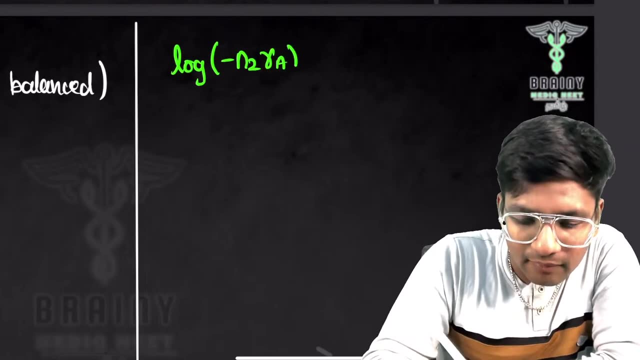 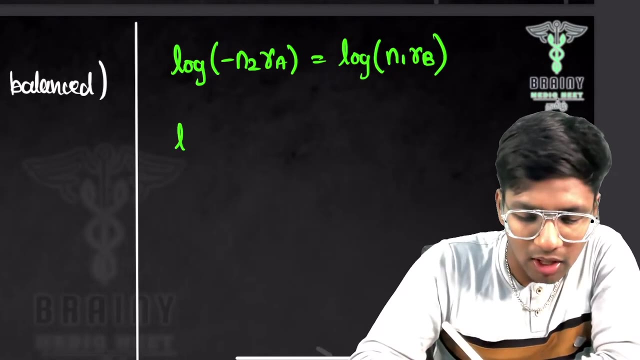 That is all Suppose. the question is a bit tough, I will tell you what they will do. Log of Log of Minus N2RA Is equal to log of Log of N1RB. If I have to simplify this more and write it: 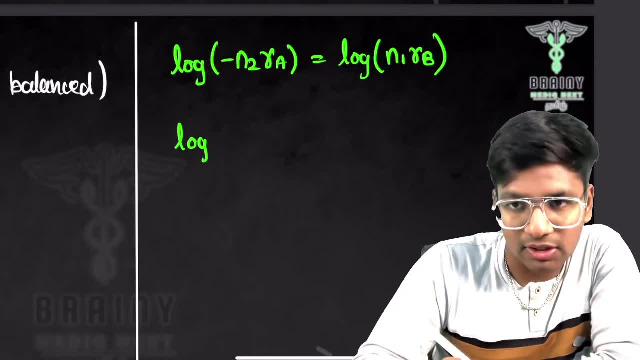 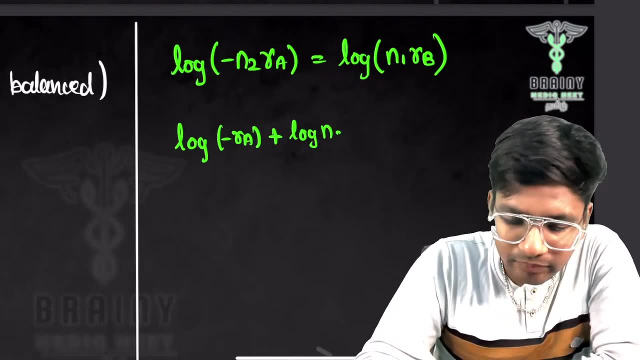 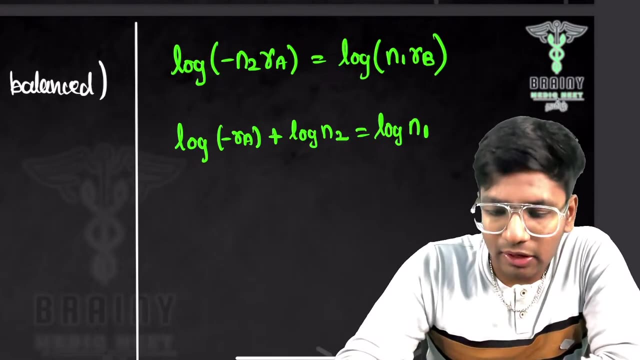 It is in multiplication. I will divide it in multiplication, Correct. So Minus RA Plus Log of N2 Plus log of N2 is equal to Log of N1. Log of N1 plus Log of RB. Can I write this in this way? 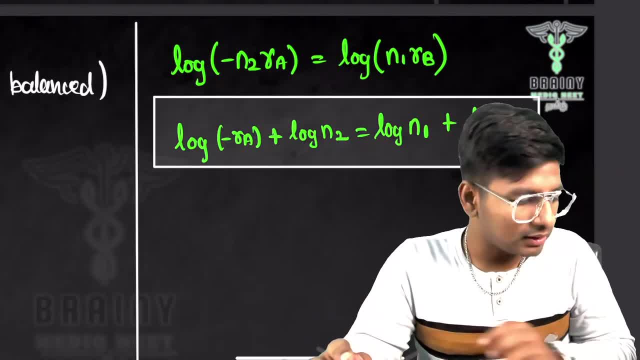 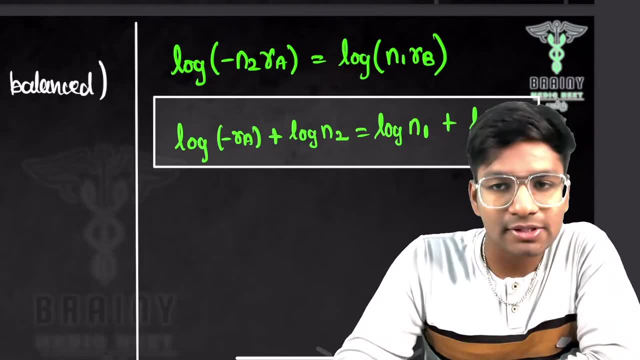 Can I write this in this way? I can write this in this way. Done Because in this basis the question has come in J. Log of M1 is equal to log of M plus N. As you all know, Log of M1 is equal to log of M plus N. 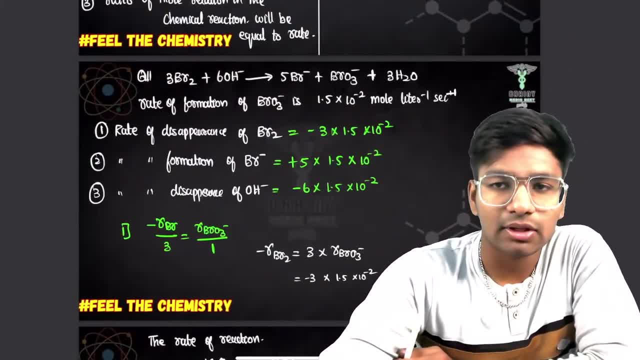 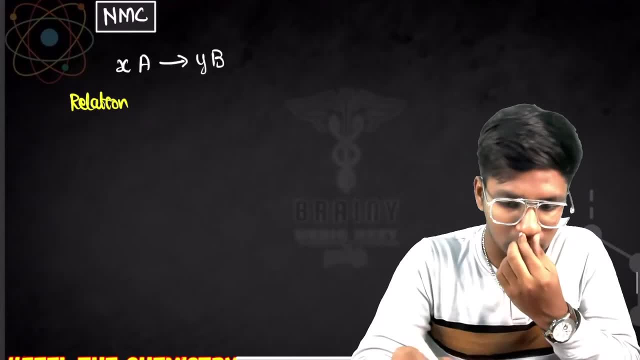 If you do not know the log form, it is okay, I will teach you again, I will teach you again. Okay, I will teach you again, I will teach you again. So the question is Question. The question is Relation between: 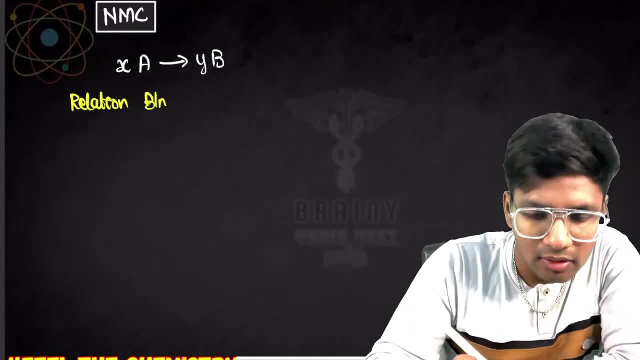 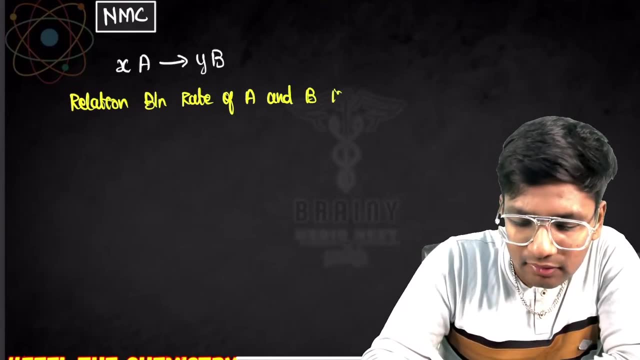 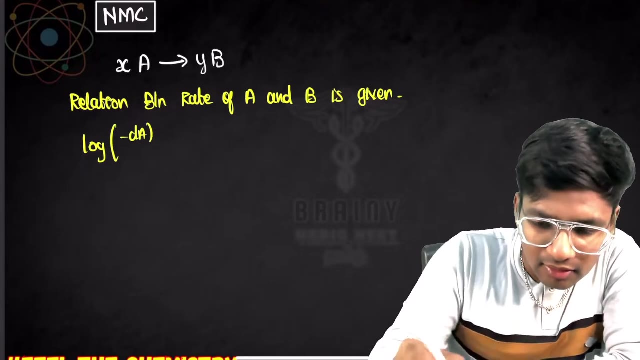 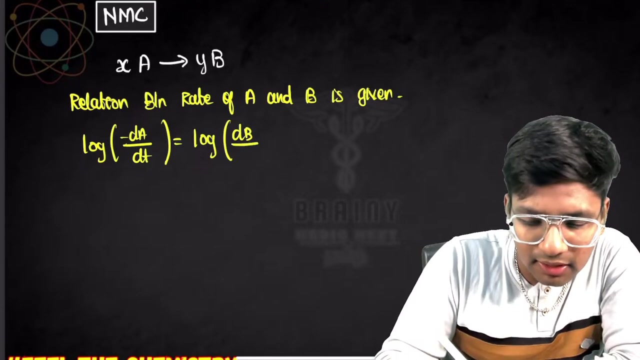 Relation between Rate of A. Rate of A and B is given, Rate of A and B is given. That is Log of Minus DA, Minus DA by Minus DA by DT is equal to Log of DB by DT. Okay, Plus 0.3. This is given to you. 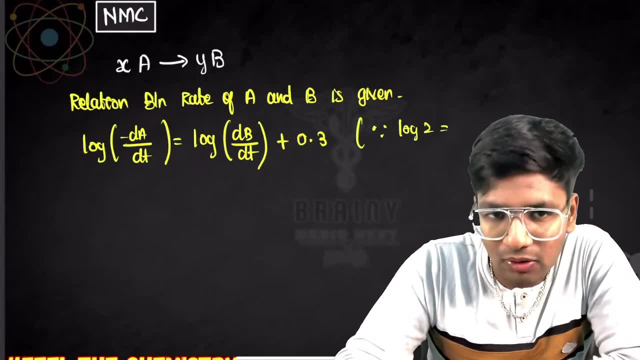 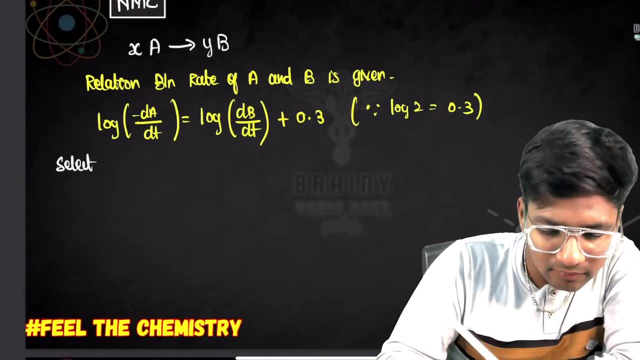 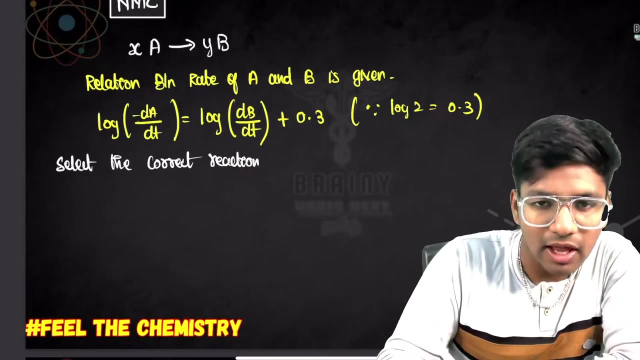 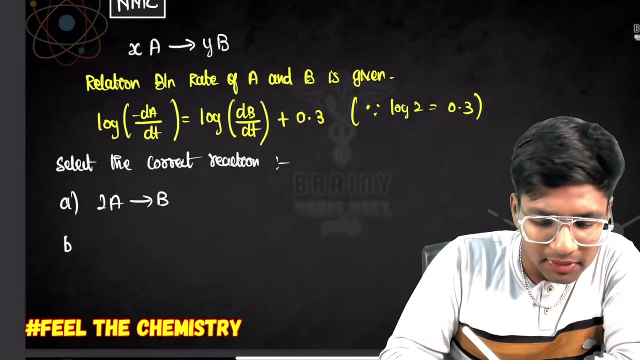 And Another thing is given: Log 2 is equal to 0.3. Select the. Select the Correct Reaction Reaction. Select the Reaction Reaction. Select the Reaction Reaction. Select your Reaction. Select the Reaction Reaction. This is to 1 to 3 With Team. You will need: 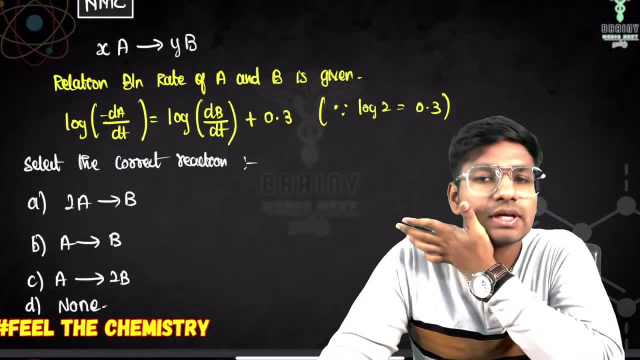 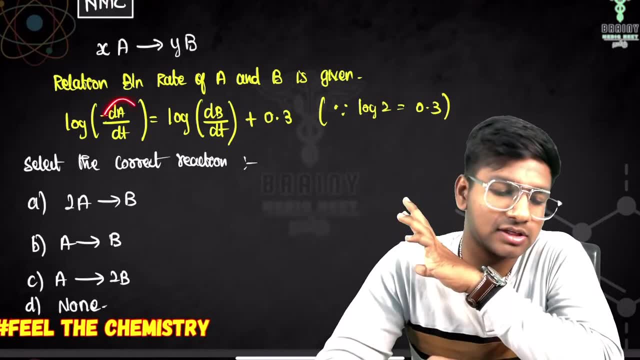 3, 2, 3, 7, as You can see What is N. Okay, If you Rei Sleep, Sleep O. So this is MK, This is. if I was able to proceed like that. then, If you proceed with the rate, the answer will be very easy. 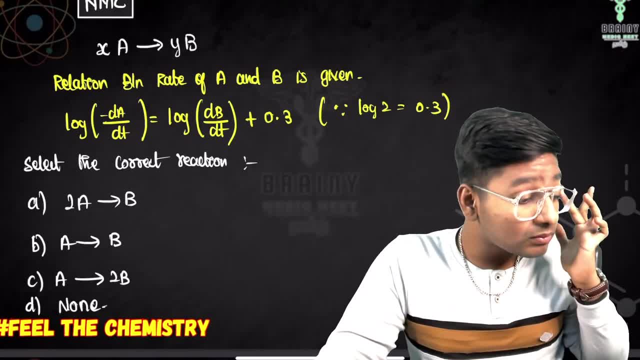 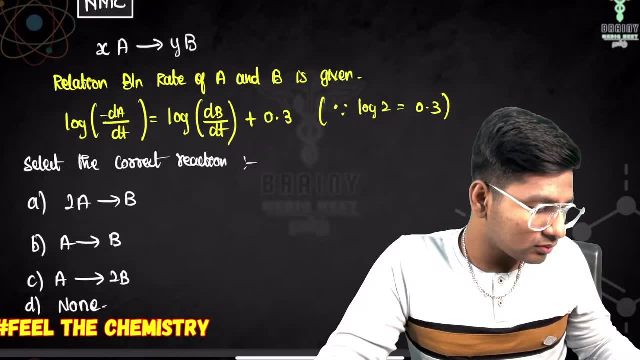 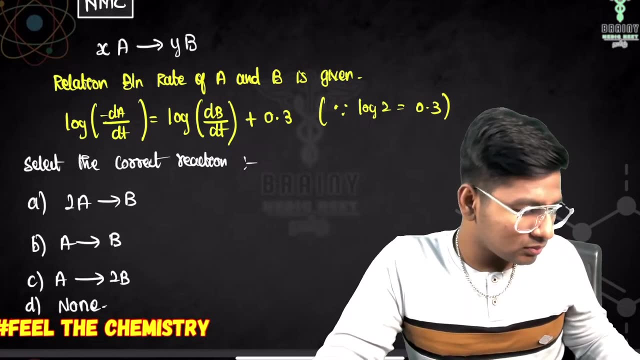 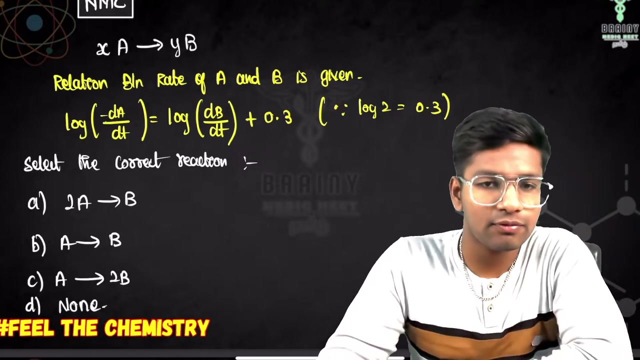 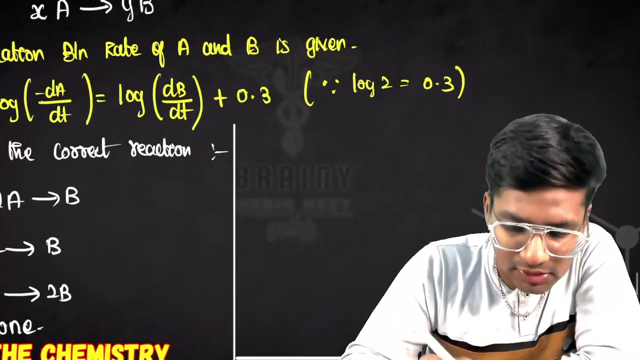 Rohit is telling A. How many of you are telling A? How many of you are telling A? Let's see what happens. Many of you may have understood this easily, but this is a very simple question. So what is the question? 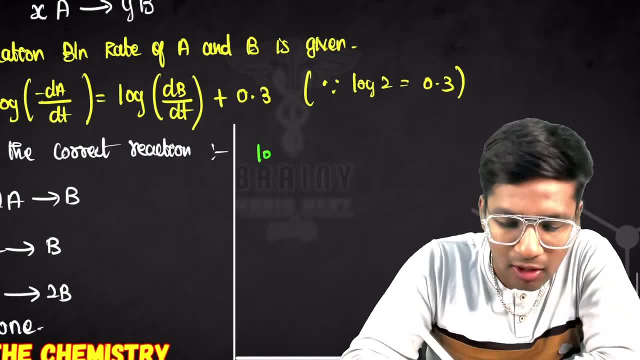 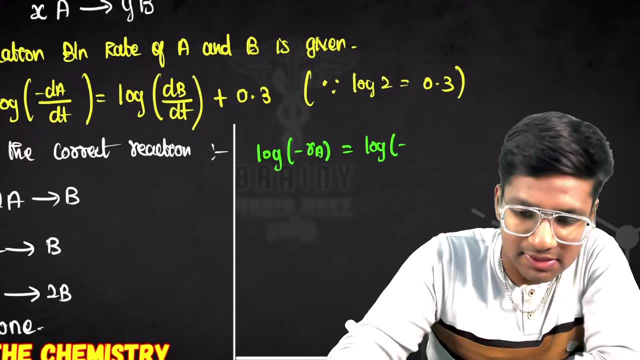 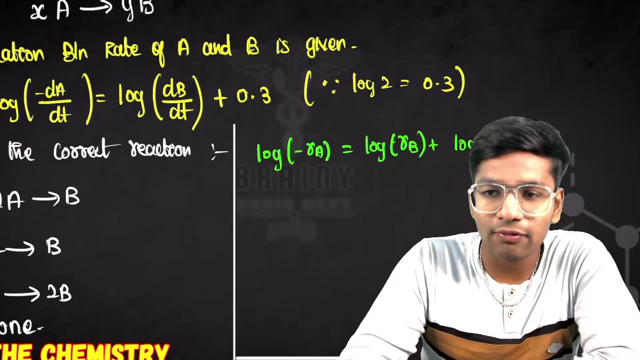 What is the question? I will simplify it and write: Log of minus rate of A is equal to log of minus. minus is not plus, plus, plus Rate of B plus log of 2.. Okay, plus log of 2.. 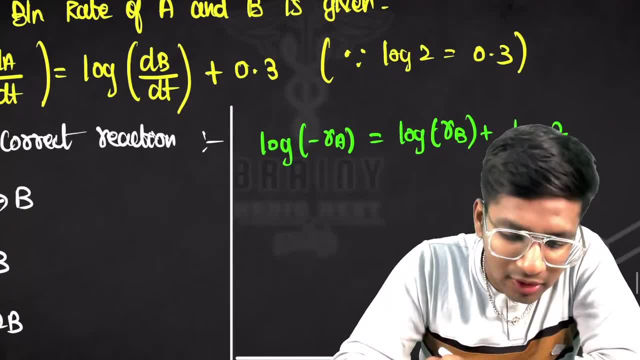 Why? Why did I write log of 2?? Why did I write log of 2?? Because 0.3A- 0.3A log 2 can be written. Can I write 0.3A log 2?? 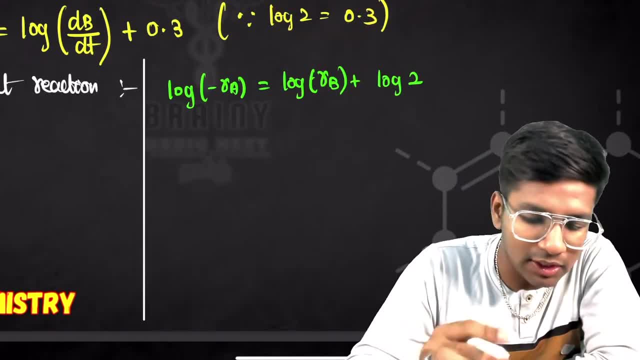 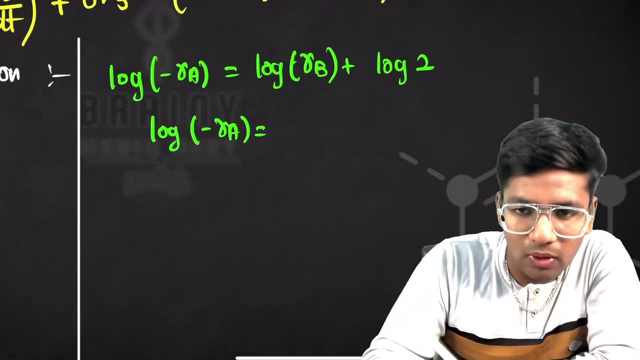 Can you see I have given value here 0.3A. log 2 can be written. So in the next step log of minus RA is equal to log of A plus B. log AB can be written. Correct Log AB. 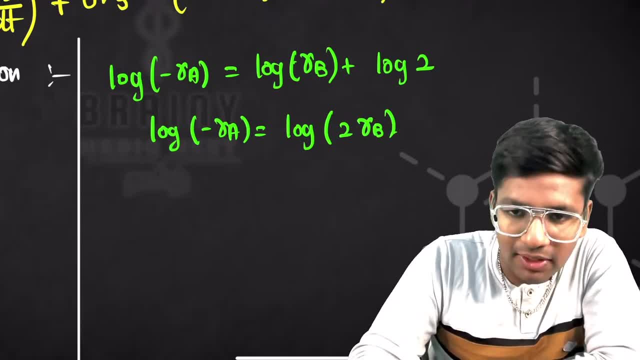 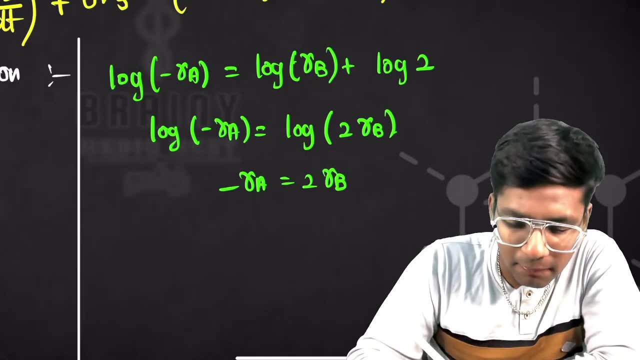 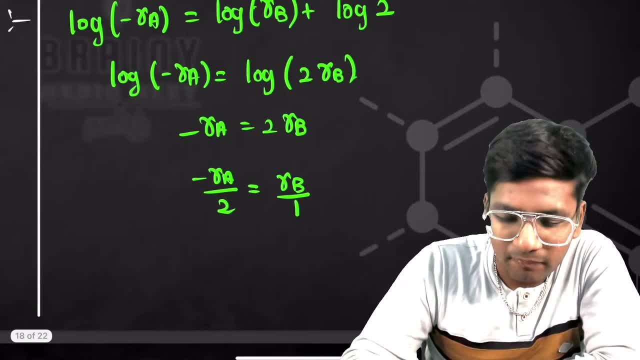 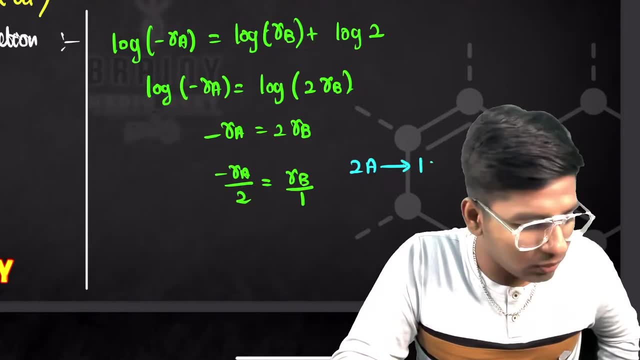 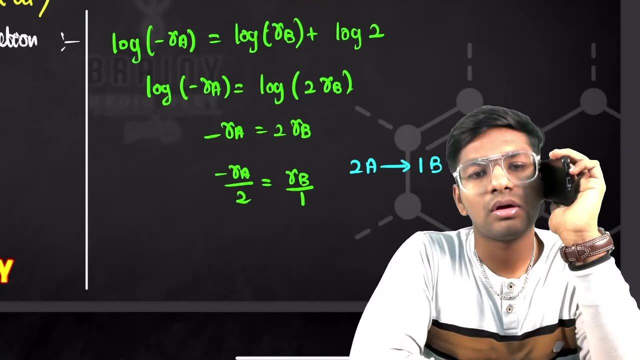 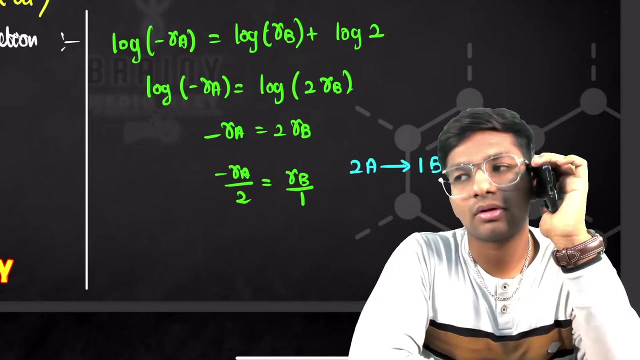 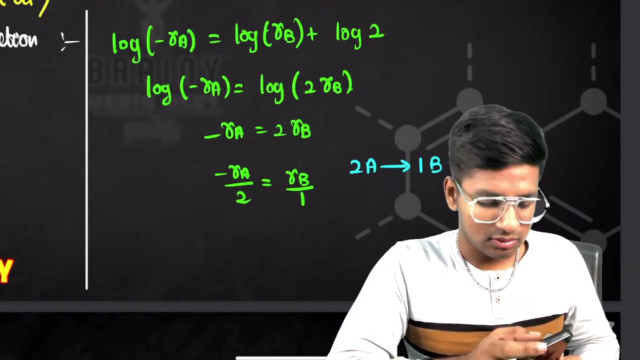 What is the reaction? I have written coefficient below. Then 2A gives B. Nice question. 2A gives 1B. Hello, Tell me, I am taking classes. Do you want me to teach you? Ok, Did everyone get the answer to this question? 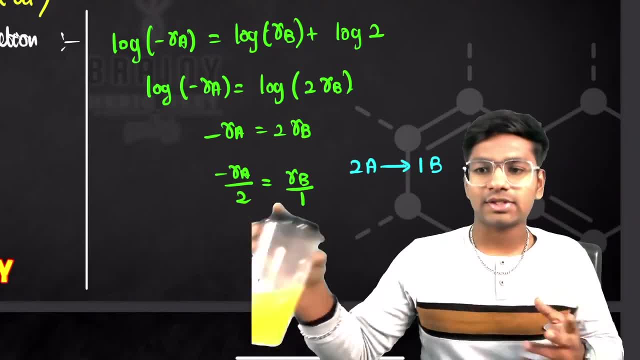 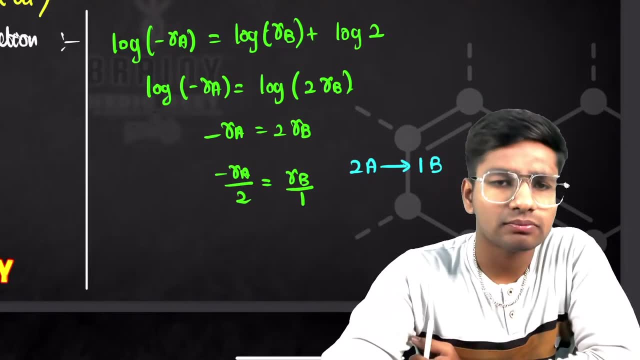 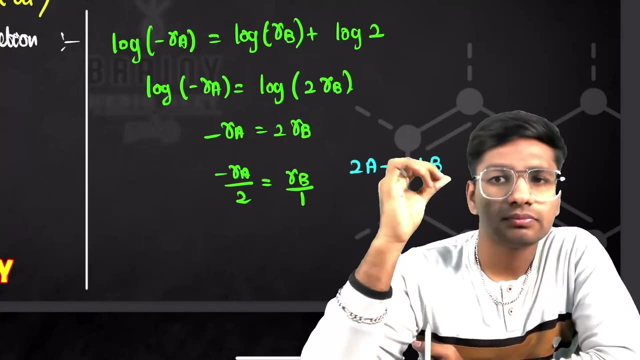 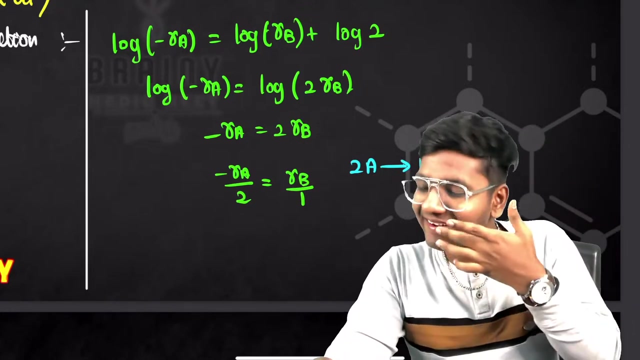 Did everyone get the answer to this question? It is not a good question. It is not a good question. Shall we move on to the next one. Shall we move on to the next one. Do all of you understand the question? Don't hit the drone, it's on your phone. 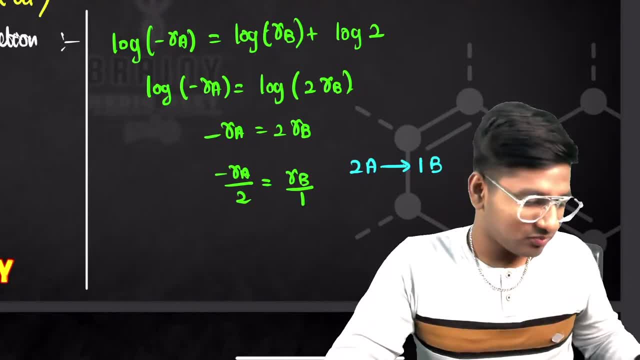 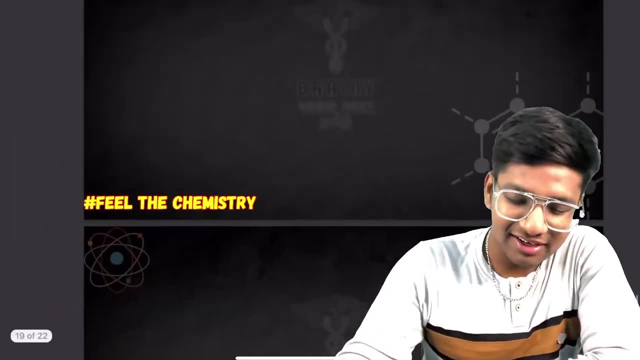 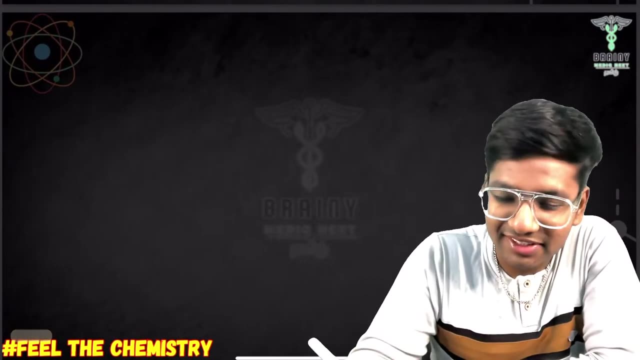 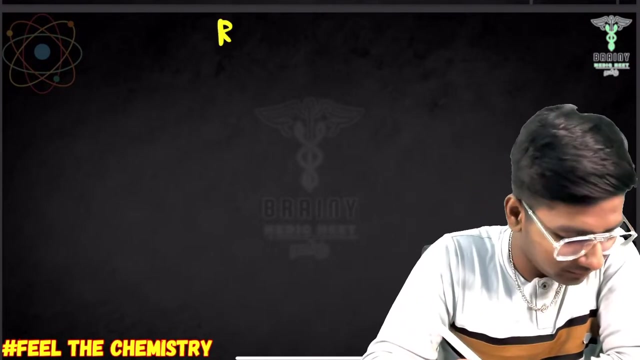 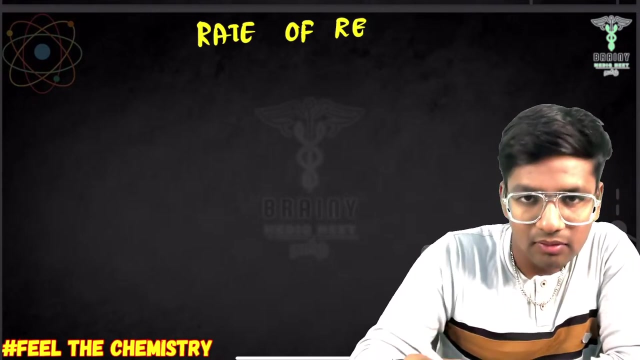 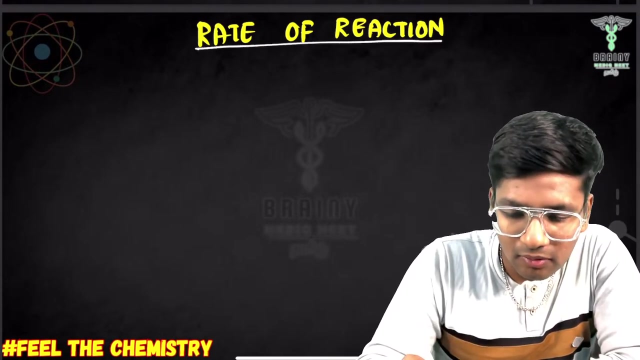 I don't have a phone. why are you doing this to me? How do you see me Tell me? No one is believing me. Okay, leave it. What to do? The world is like this: Rate of reaction. Rate of reaction. 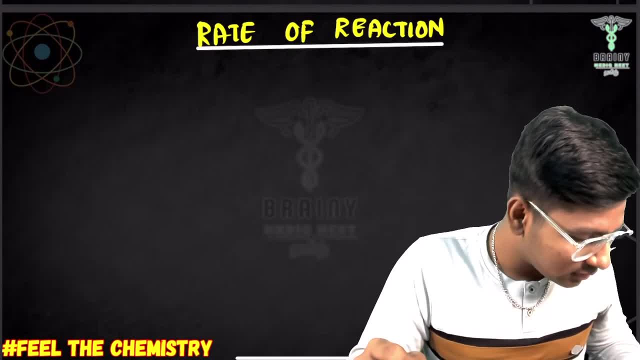 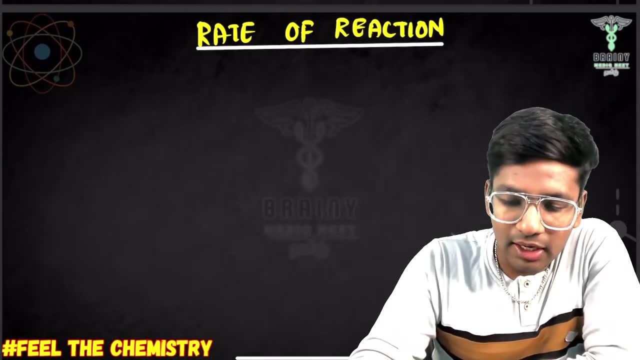 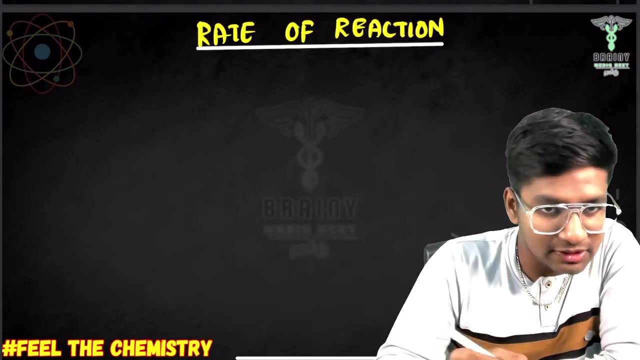 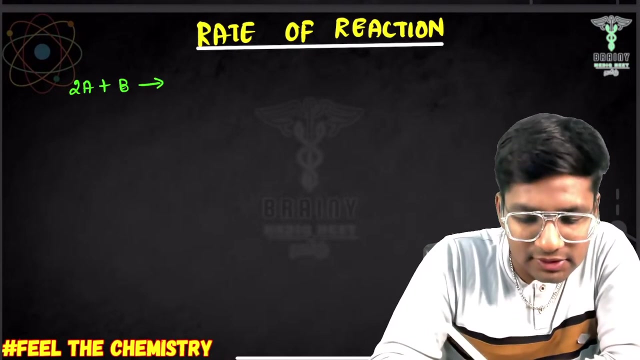 See What is this? No reaction. Another question with this type. Next is rate of reaction. I am going to simplify and tell you a concept. This is the rate. Next is rate of reaction. 2a plus b gives 3c. 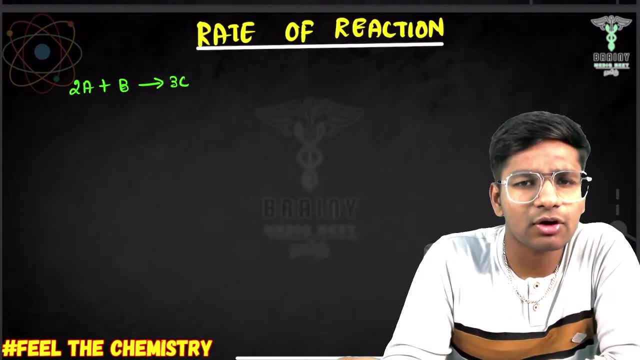 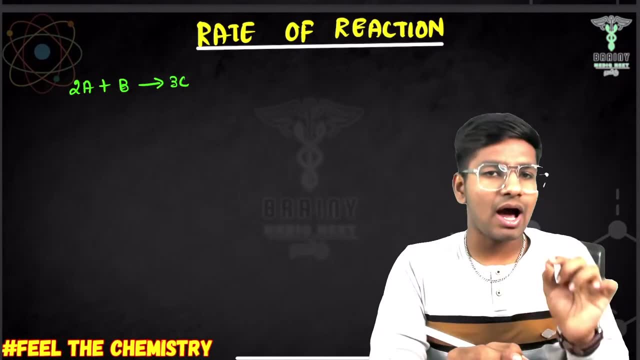 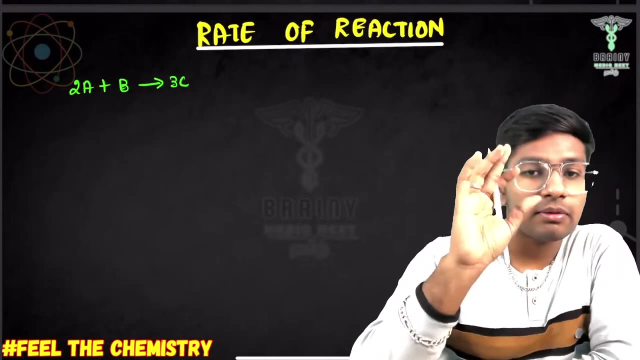 What is the rate for this Rate? rate rate. In most of the cases- rA, rB, rC- The rate is equal. What is the rate? Let me explain. I don't know if the rate is equal or not. 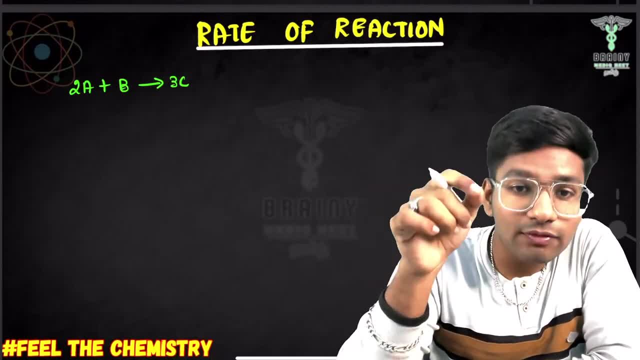 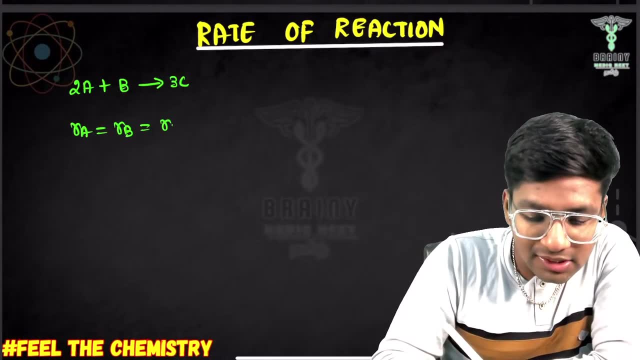 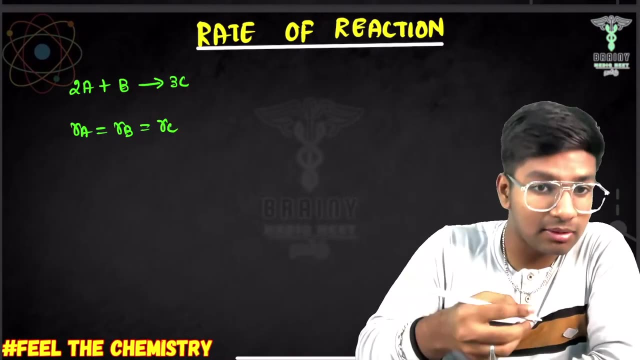 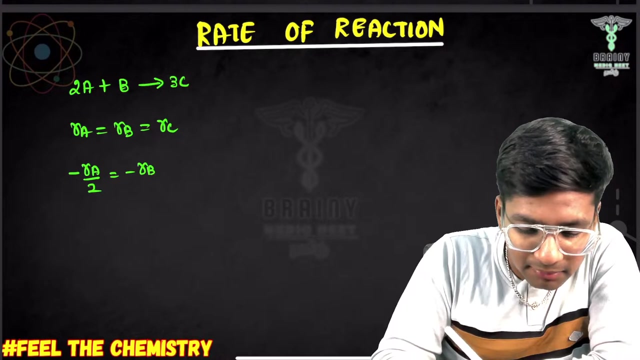 I will explain it in a better way. But the rate of the reaction is equal. The rate of the reaction If we write rA equal to rB, equal to rC. If I write it, the rate will be equal. If I write rA equal to rB, equal to rC. 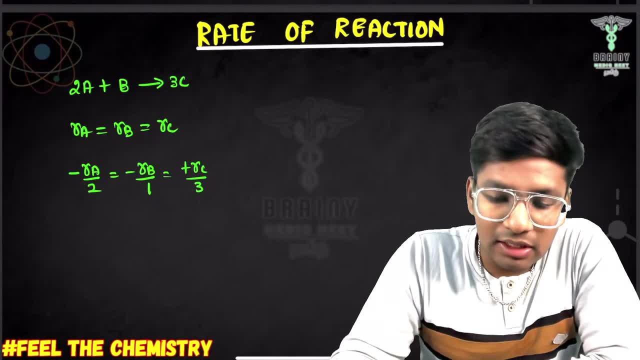 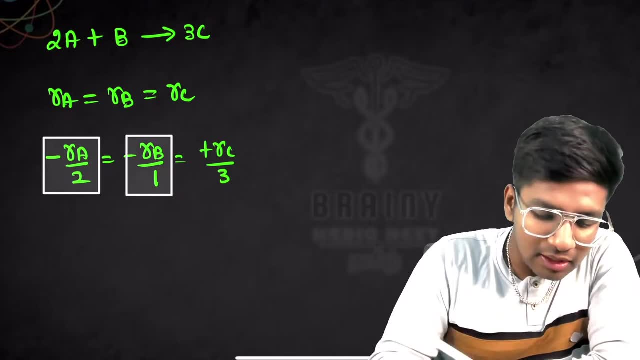 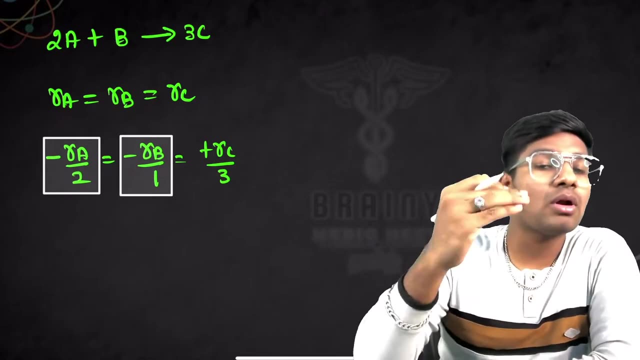 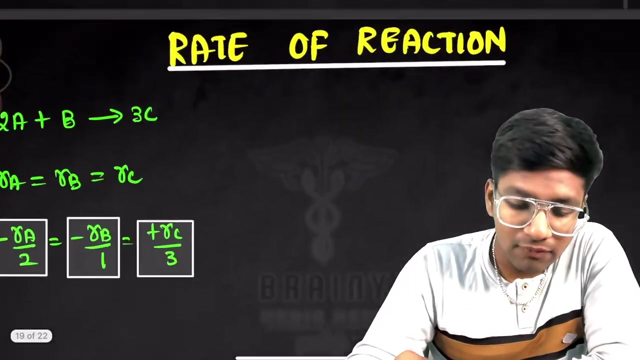 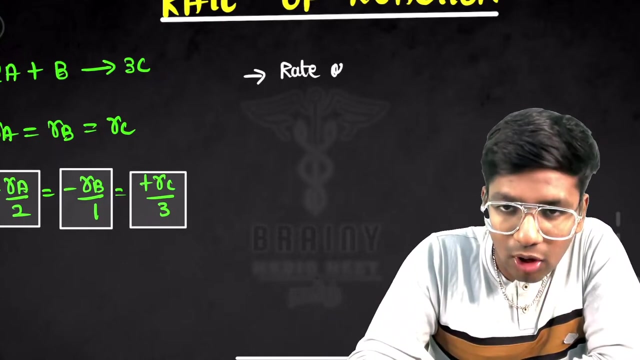 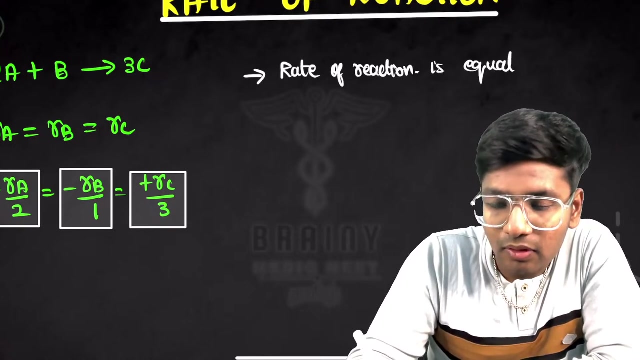 The rate will be equal. Let me explain If I write it. let me explain it again & again. If I write it, let me explain it again & again. The rate was equal. So this is the rate of the reaction. When you mention per mole, then it is called rate of the reaction. So the definition is: rate of the reaction is equal to rate of reaction. 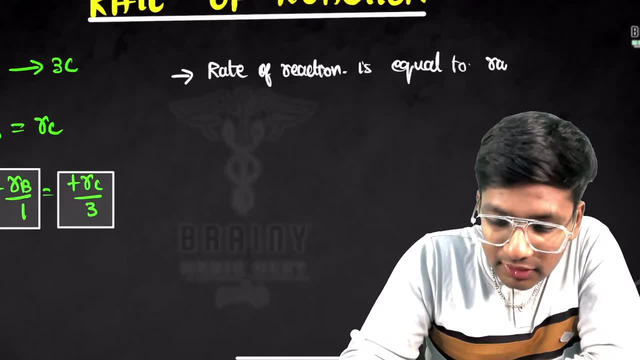 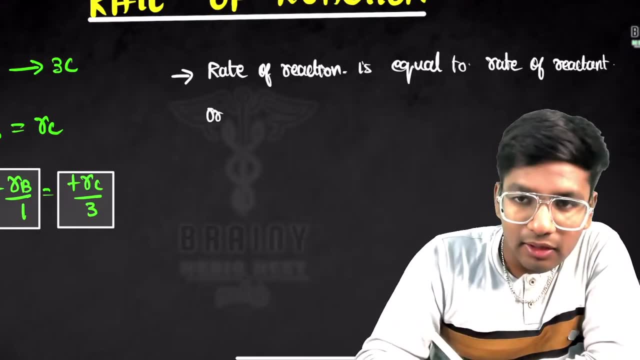 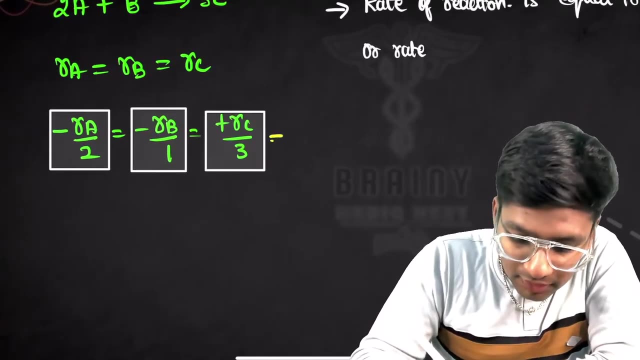 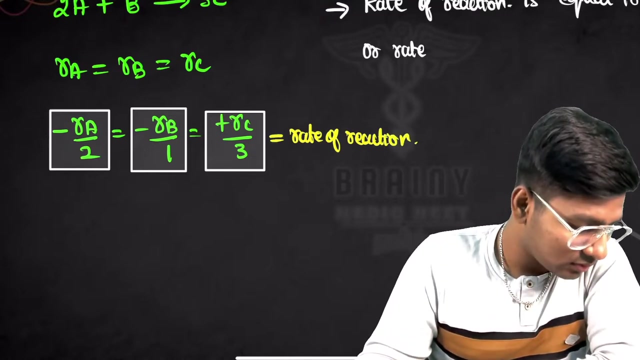 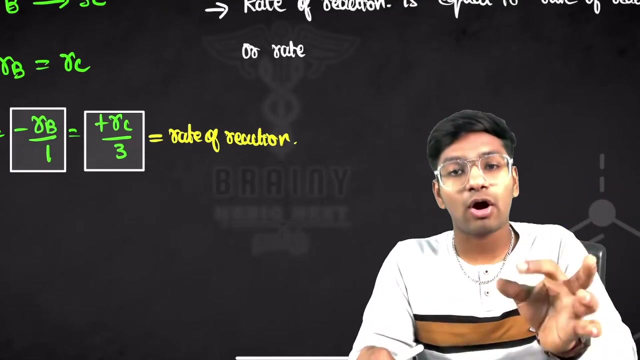 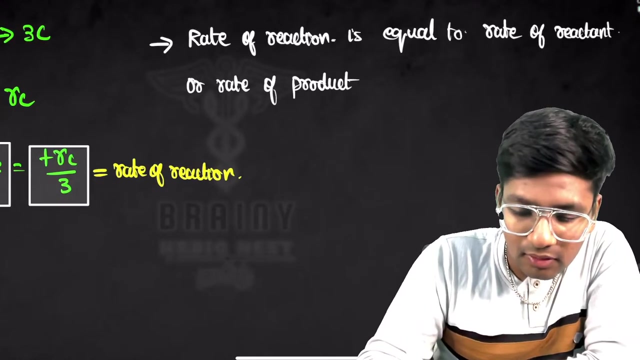 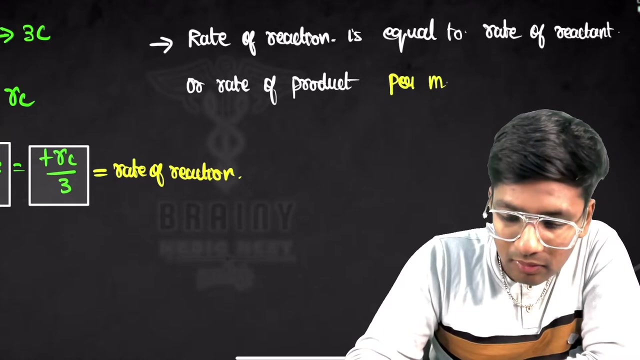 or rate of product. So this is the definition of product. I can write it as rate of reaction, Reactant rate of product per mole, Product per mole, Per mole- And the word is important- Per mole Done, Done Per mole. 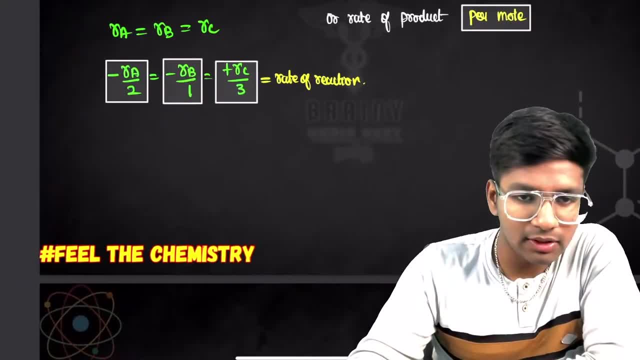 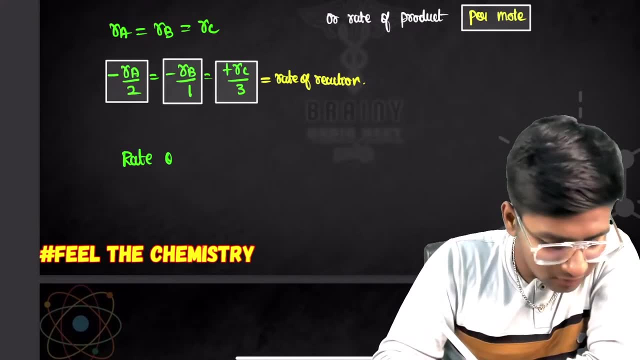 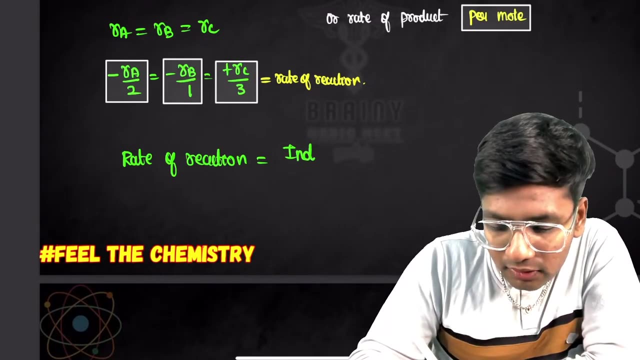 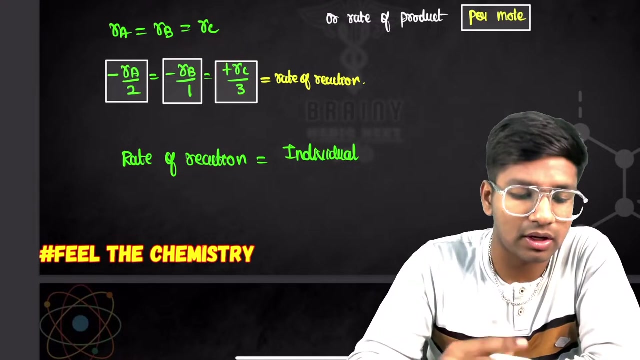 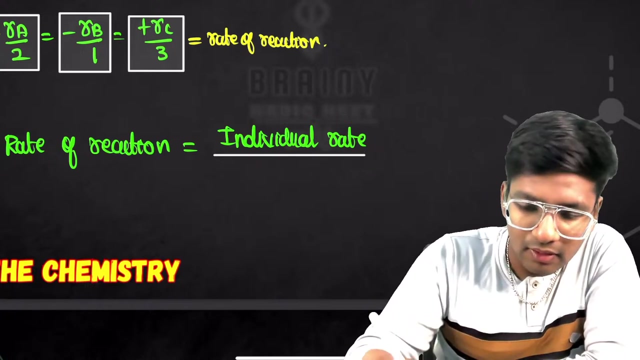 Per mole Per mole. So general formula is again: Rate of reaction, Rate of reaction. Rate of reaction is equal to individual rate, Individual rate, Specific rate, That is individual rate, Individual rate divided by coefficient. Divided by coefficient. 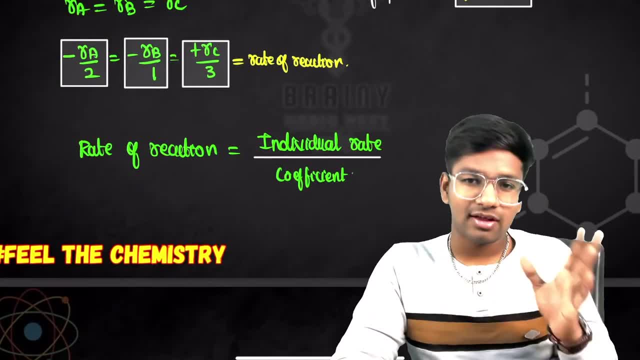 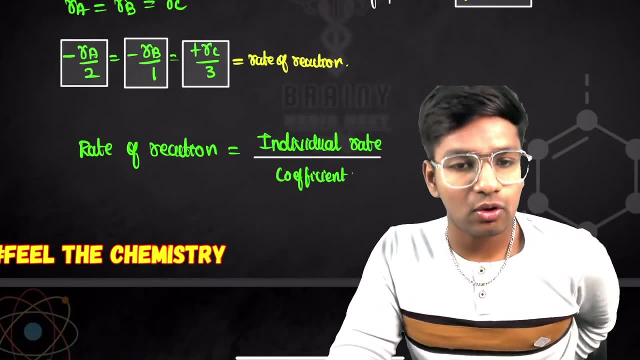 Okay, You will know that I have written everything. Rate of reaction: Okay, I just explained that definition. Try it. Do you understand? Clear? I hope this is clear to everyone. Okay, What are we going to do with this? 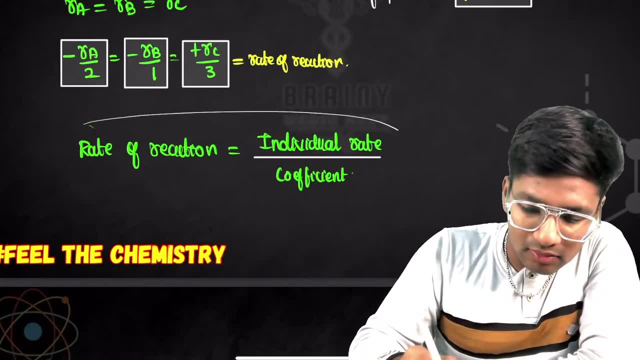 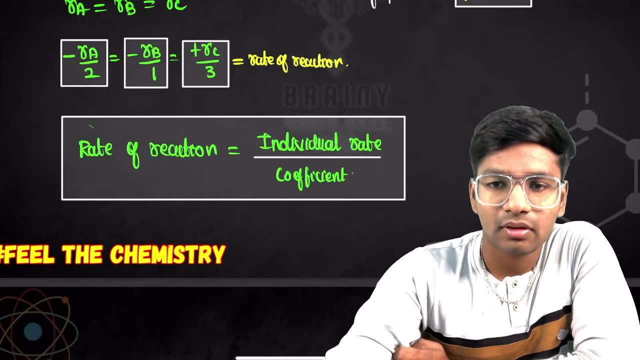 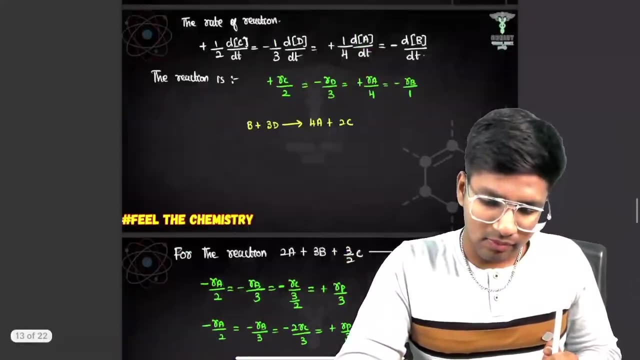 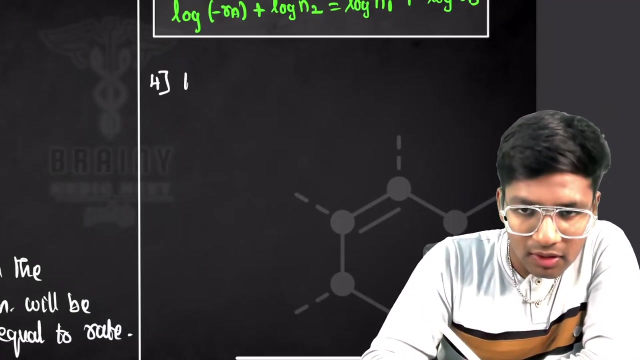 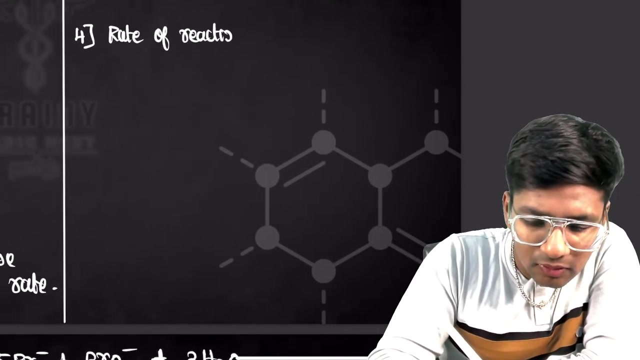 We will mention it in PM&T. We will mention it in PM&T. Wait, No questions. We have questions. No, some concepts are there? All the concepts that I have taught are here. The fourth one is rate of reaction. The fourth one is rate of reaction. 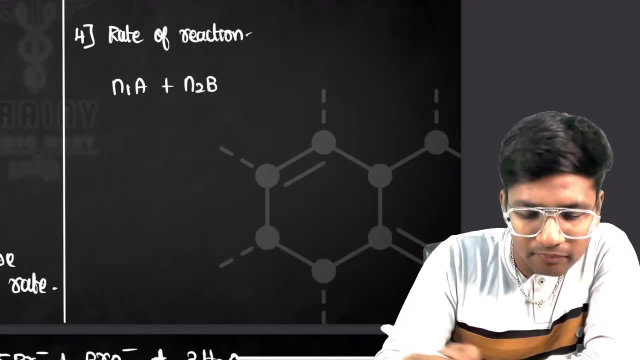 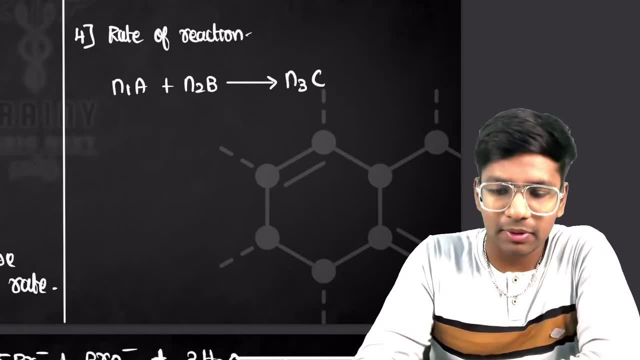 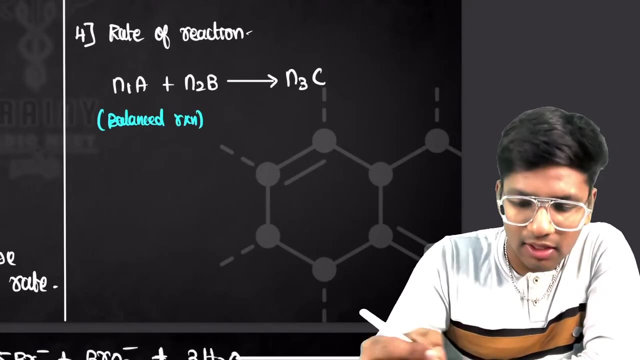 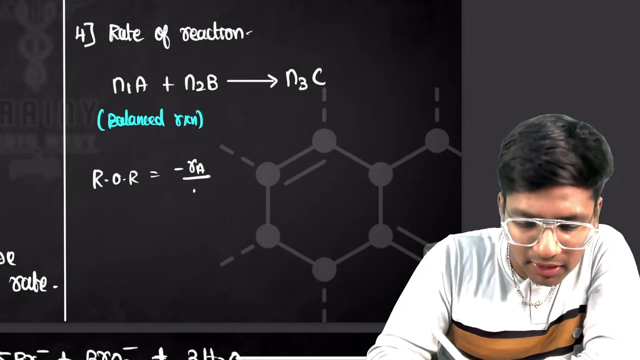 N1A plus N2B gives N3C. These are all balanced reactions. Okay, This is a balanced reaction. This is important. So rate of reaction: How do you write it? Minus of RA divided by N1 is equal to minus of RB divided by N2, which is equal to plus. 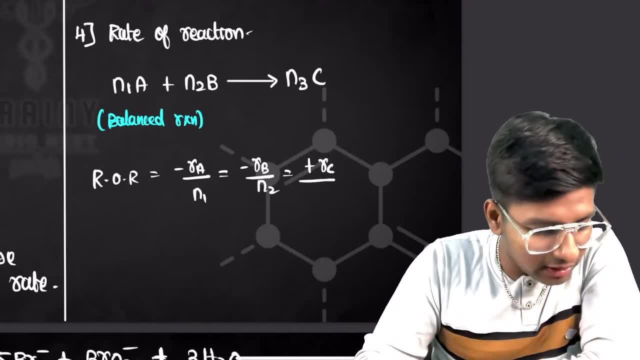 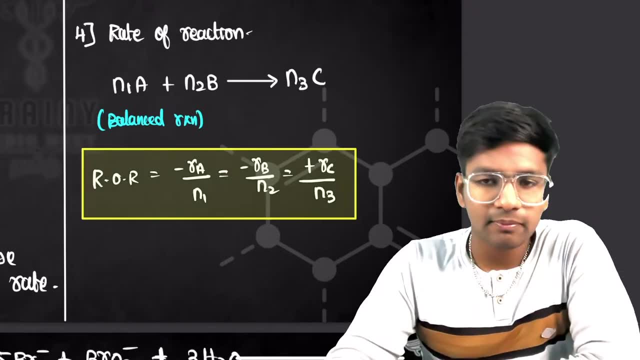 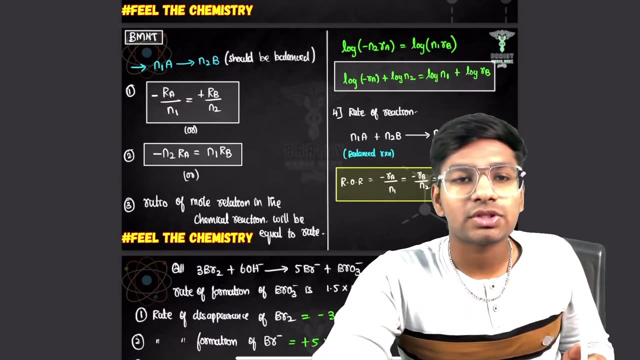 of RC divided by N3.. This is the rate of reaction. Done, Done, Done, Done, Done. You are clear? Next question: Question, question question. What is the question Here? it is Okay, Tell me to answer. 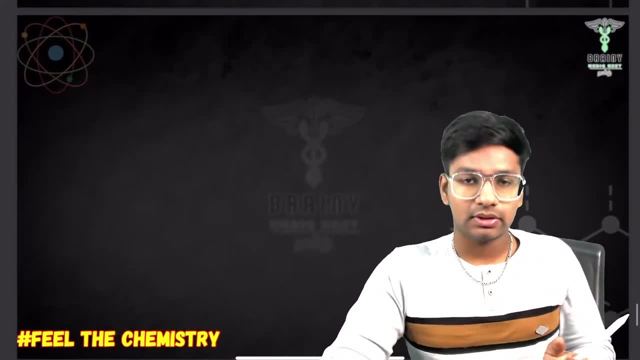 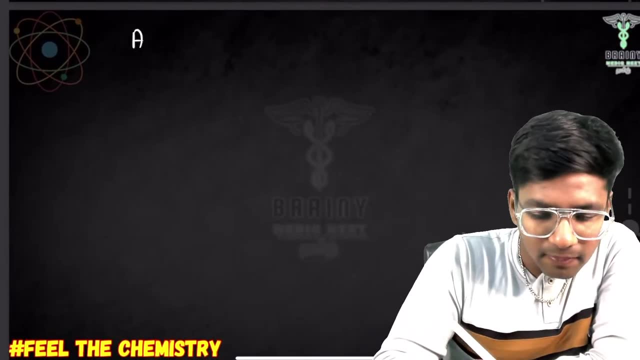 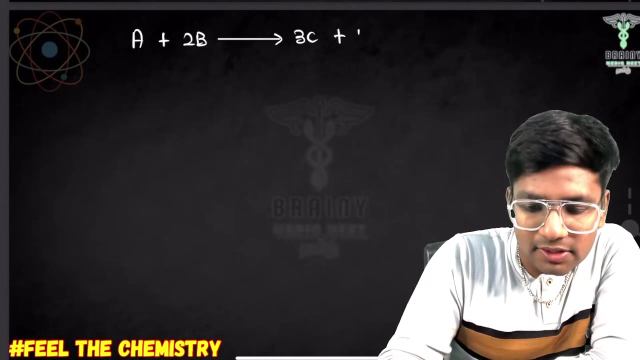 No, I have not written the question yet. Wait, I will write the question. A gives A plus 2B. gives 3C plus 4D. Okay, Okay, Good, 3C plus 40. In this, what I am going to do is: 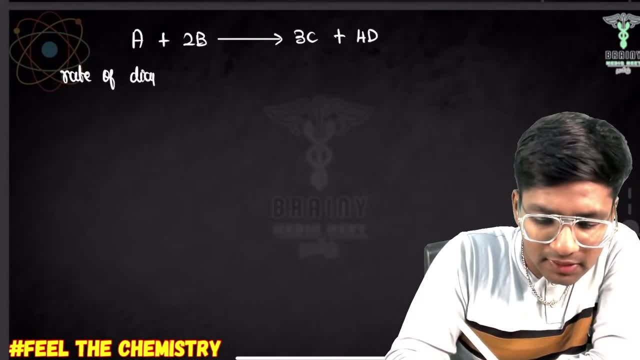 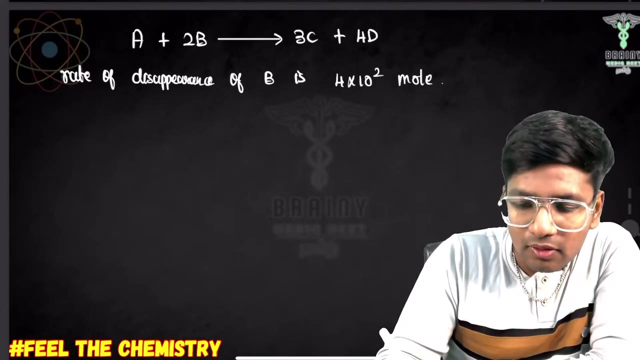 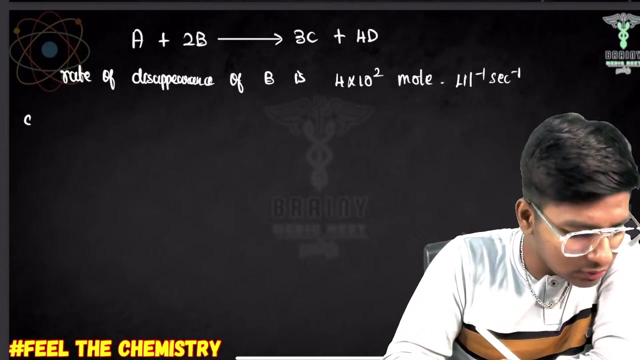 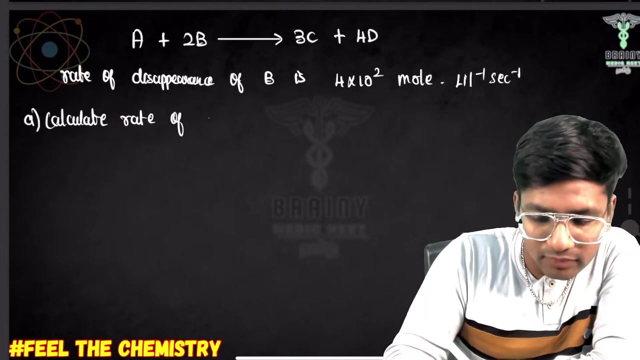 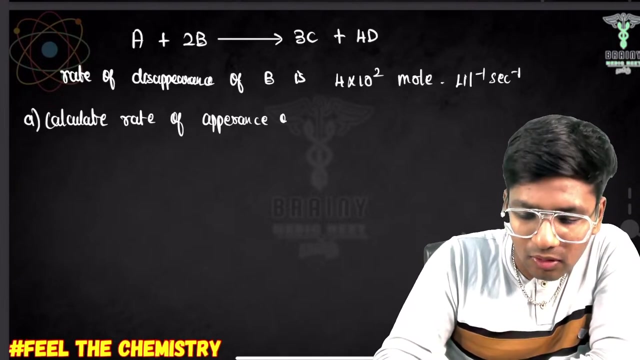 rate of disappearance of B is 4 into 10 power 2 moles, liter inverse, second inverse. I have told it Okay, First question is: calculate: calculate rate of appearance of B Options. I will write. Wait for a minute. 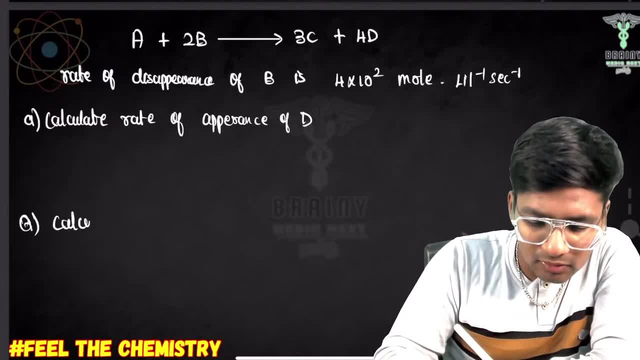 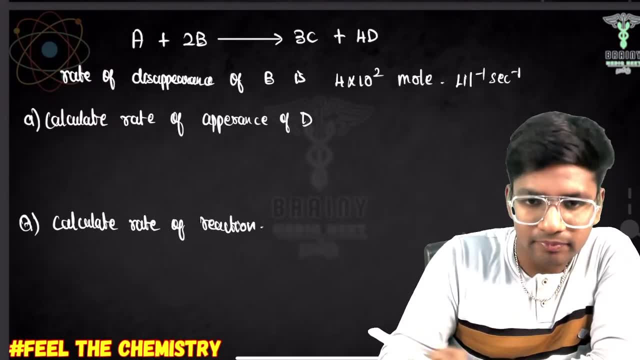 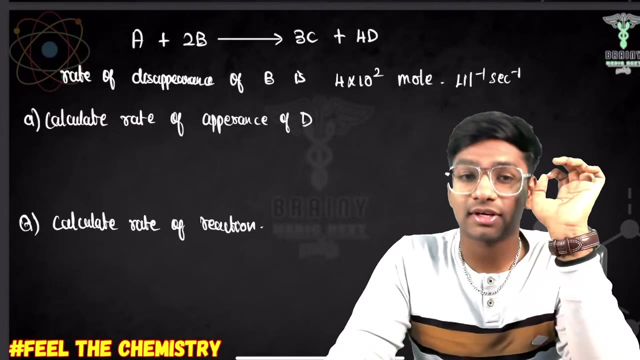 No, no Calculate rate of reaction. It is one of the questions. There is a difference between the two. There is a difference between the two questions. You have to find out and answer. A is 4 into 10 power 2.. 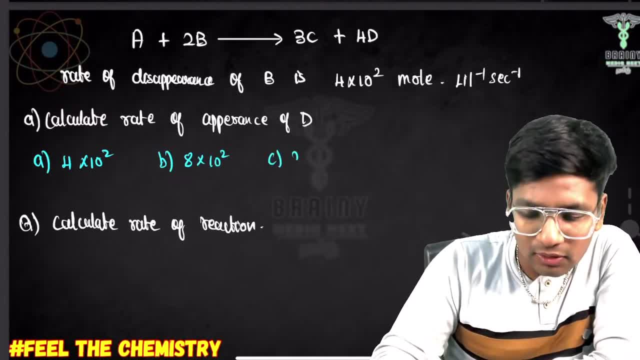 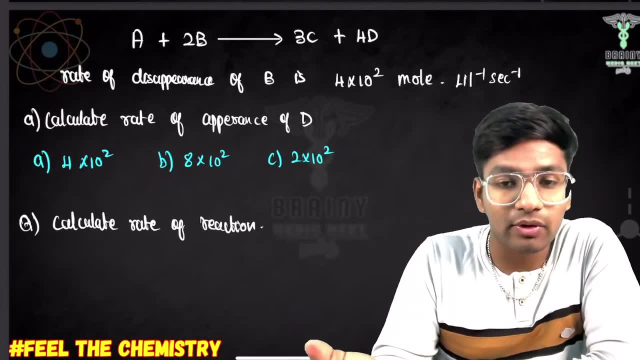 B- 8 into 10 power 2.. C- 2 into 10 power 2.. I have asked individually, I have asked one specifically. I have asked the rate of the reaction. It is just up to you Tell me your answer. 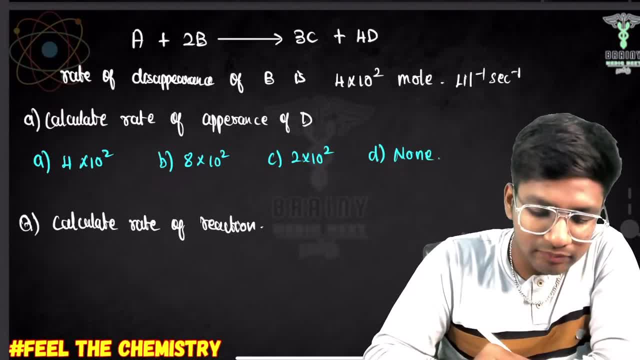 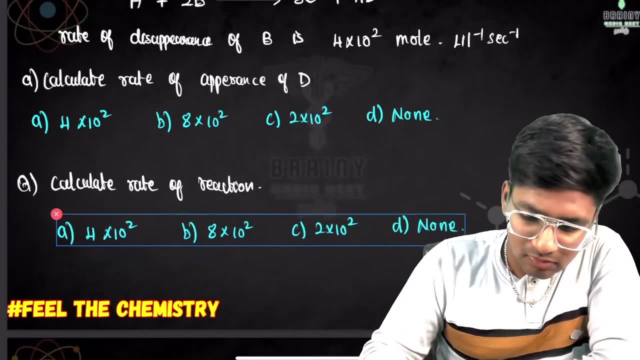 B is 0.. B is 0.. B is B. Is it just b? It is p. Is it impossible for 100%? we can get Basics from in 1st person: мат, Rape R, 게임 1st person to. 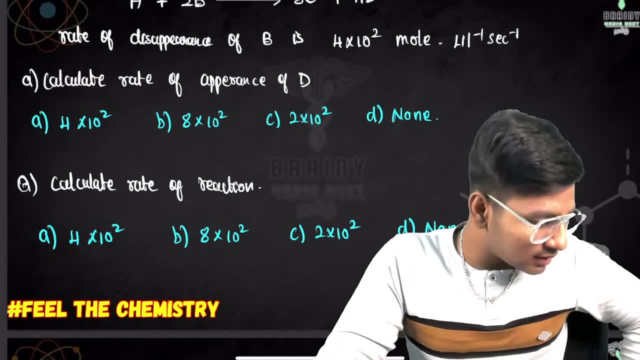 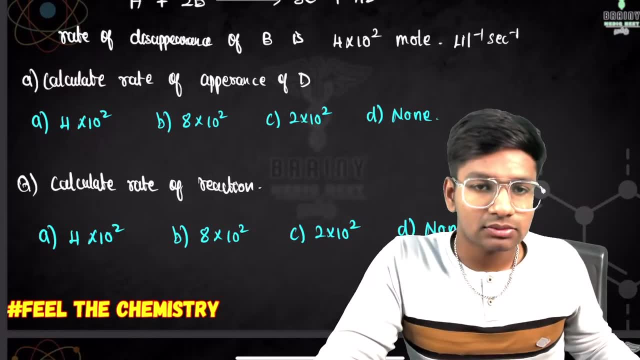 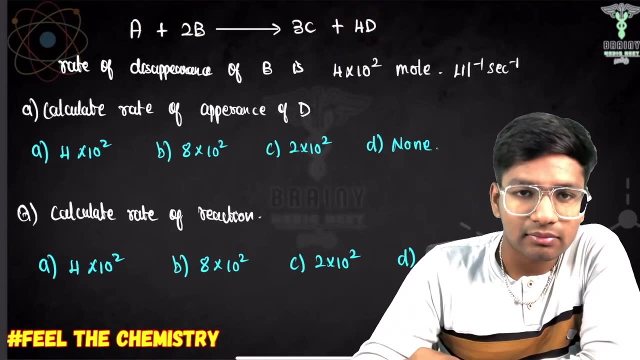 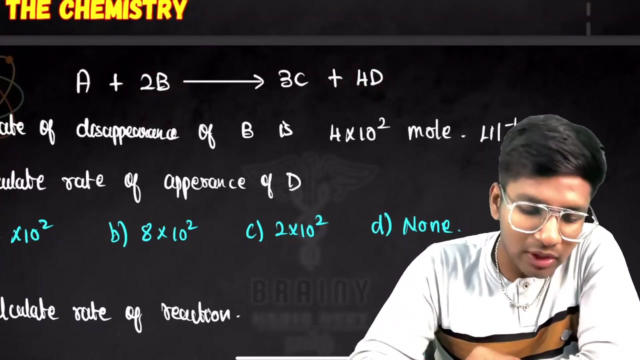 answer: A: two, 700 thousand plus much crazy, almost one thousand 200 points. I see 10, 200, 50 income, only 20, 60 Windows por uns are: Here is 4D and here is 2B, but if you convert both of them into one it will be simple. 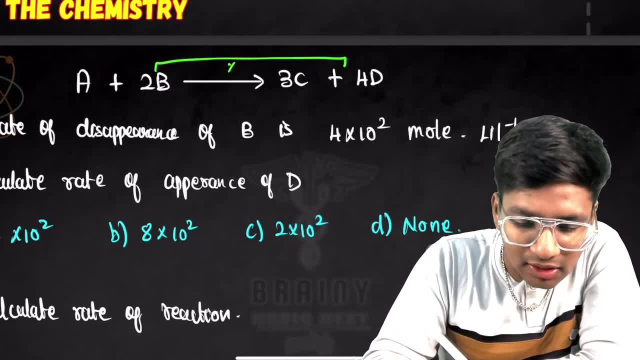 Or here I will tell you simply: this is increased by 2 times. is it increased by 2 times? Look at this and this ratio: 2 is the ratio. then just do into 2 and you will get the answer. 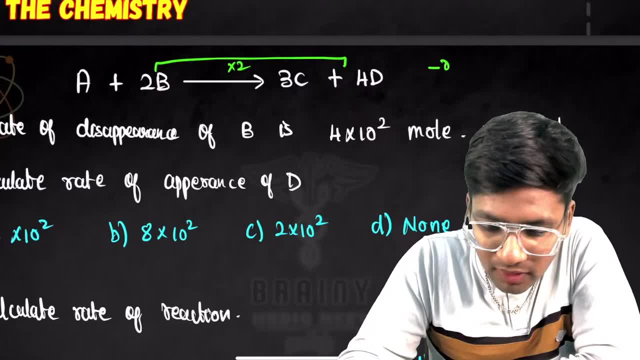 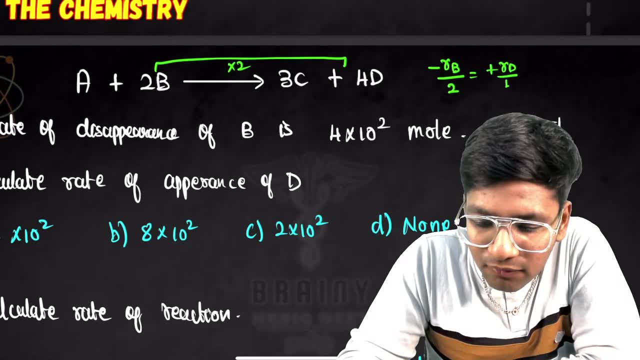 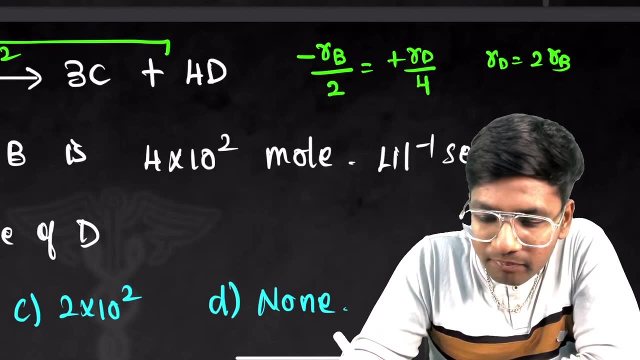 If you do this into 2, you will get the answer correct. Or shall I say it in a simpler way? The rate of reaction of B- they have given disappearance- Divided by 2 is equal to plus of Rd by 4, Rd by 4, then Rd is equal to. Rd is equal to 2 times of Rb. it is double. 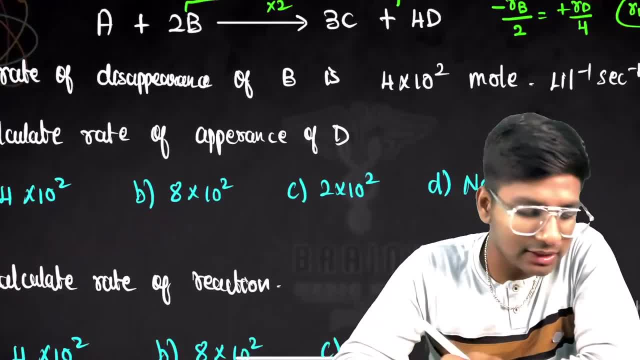 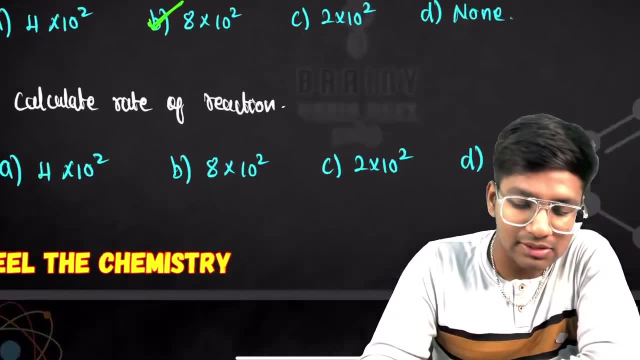 Because the mole is also double, so the rate is also double. So the answer for the first one is this: B. But what will be the answer for the second one? C is given Gautam, exactly C is the correct answer. 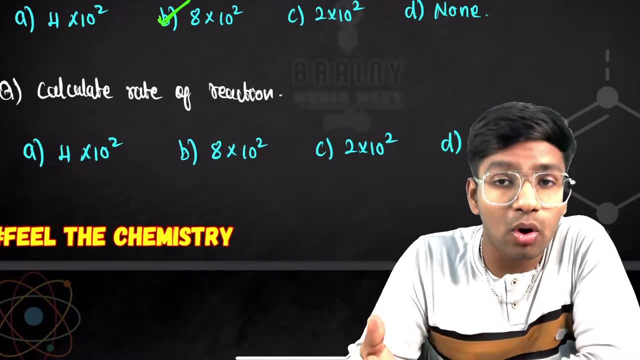 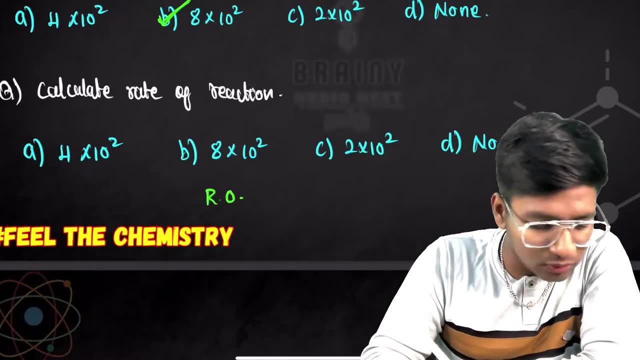 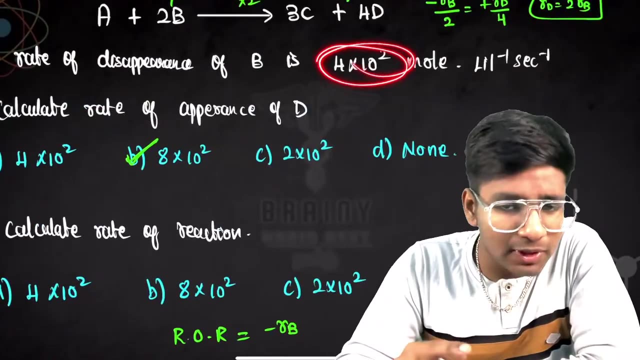 In C they have asked the rate of reaction per mole Specifically, whatever you take. whatever you take, for example, they have given the rate of reaction for B. rate of reaction is equal to minus Rb. their rate of disappearance of B is given. 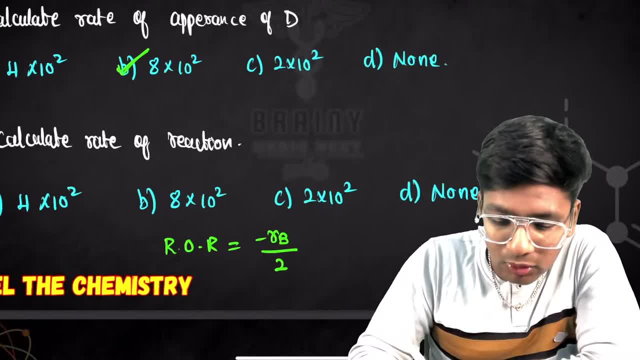 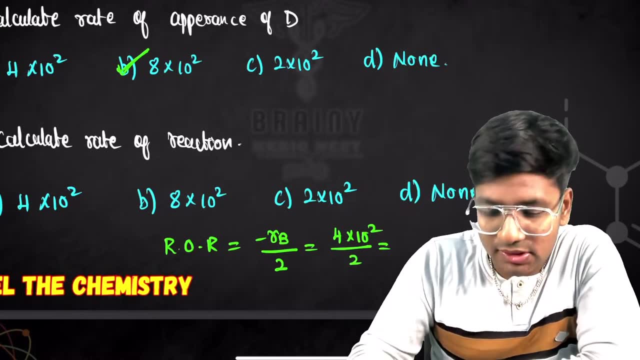 but for me, per mole, what is the coefficient? Divided by 2, which is equal to 4, into 10 power 2,. divided by 10 power 2, divided by 2, which is 2, into 10 power 2.. 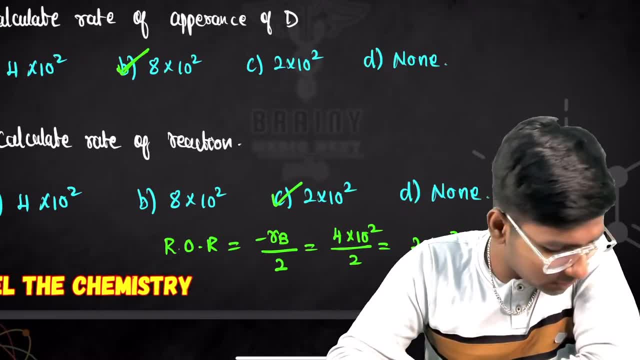 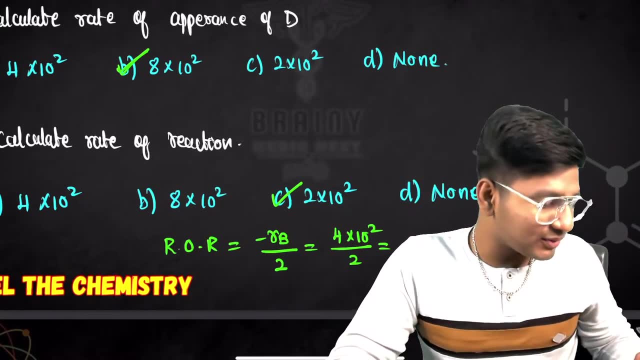 This is your answer. What happened? Madhu Mitha Madhu, You are going to cry Why you answered wrong. Very simple question. but you answered wrong, Right? Happens, Happens, Toppers, all the toppers, like you. they do this many times. 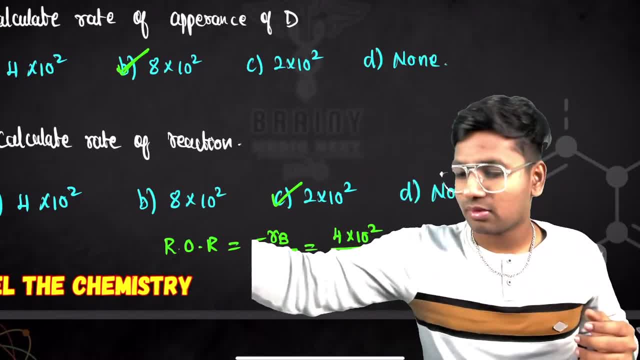 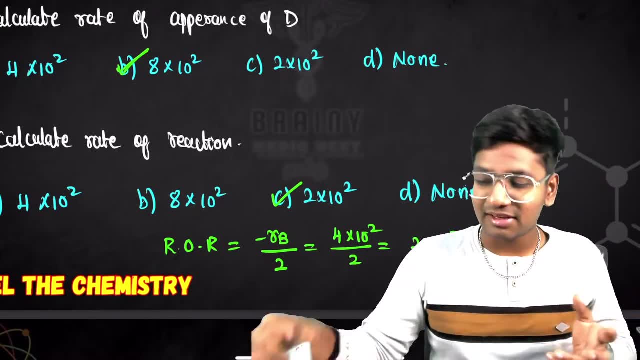 Don't take it too big Pray. and Silly mistake, Silly mistake happens, Don't see? please avoid silly mistakes. Silly mistakes means I have lost many marks. I have lost many marks, Many, Many. 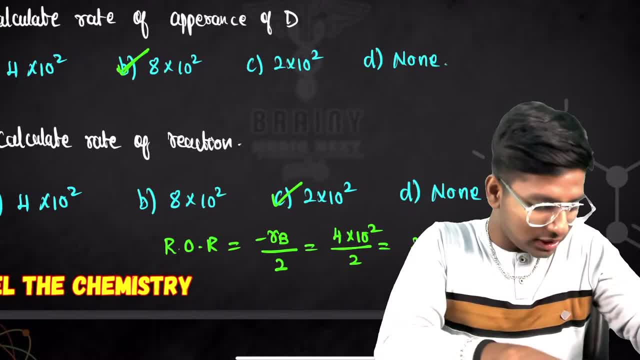 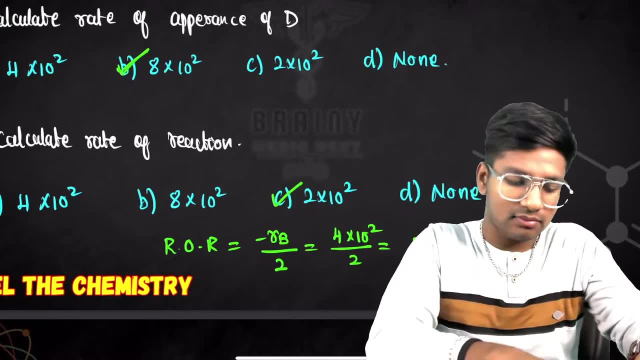 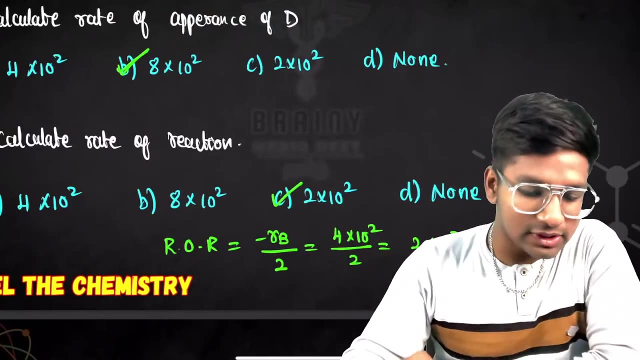 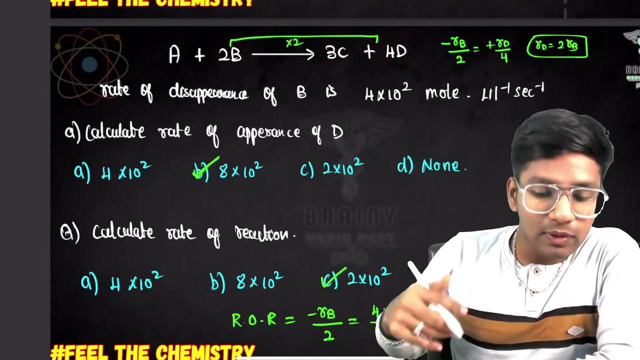 Marks, four marks. Silly mistakes, I understand. I will say another time: wait, Wait. I will say another time. See here In the first question what I asked. I asked individually. individually, I asked the relationship between individual B and D in the first question. 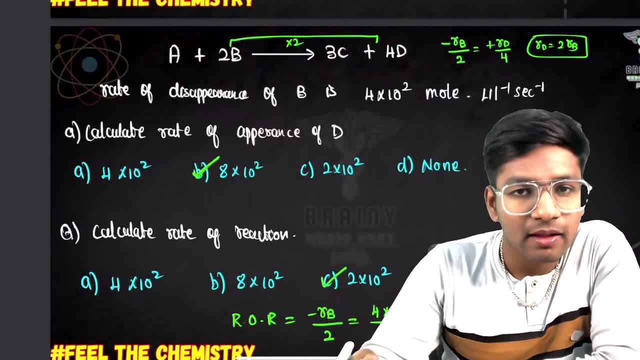 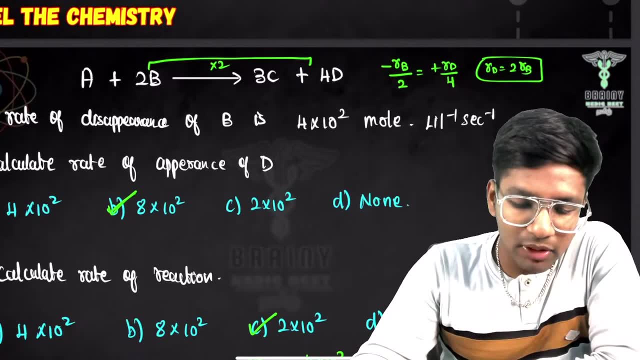 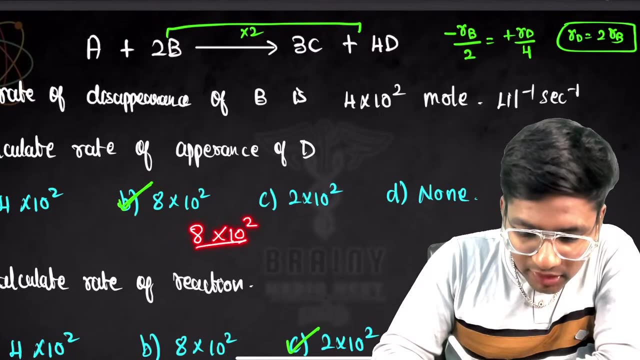 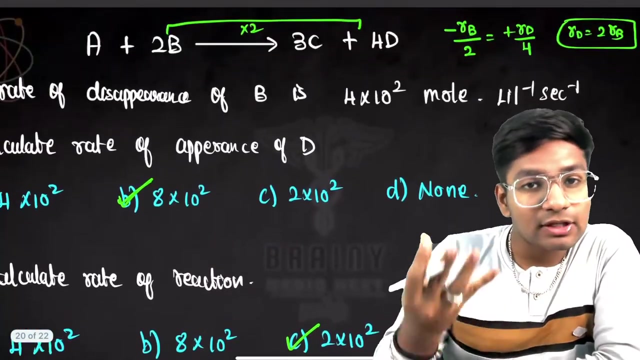 In the second question I asked. I asked the relationship between individual B and D in the first question. In the second question I asked the rate for the whole reaction. there is a difference between the two. but if you take this formula and put it in the same formula, if you take the d and put it in the same formula, 8 into 10 power 2, divided by its coefficient 4, what will it be? 2 into 10 power 2, the same answer will be given. do you understand what I am trying to say? 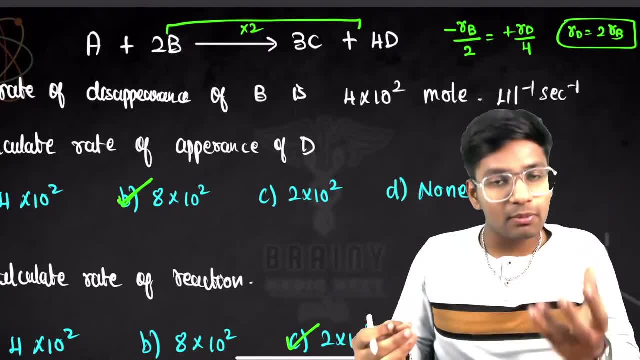 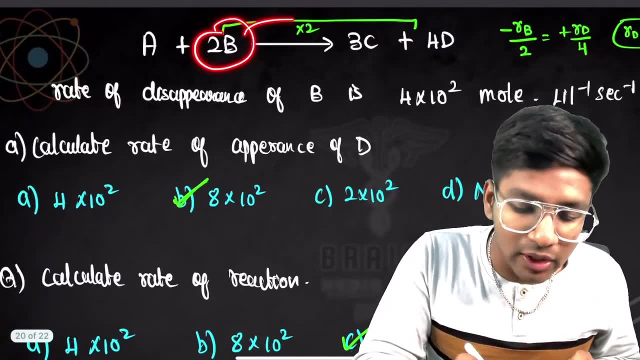 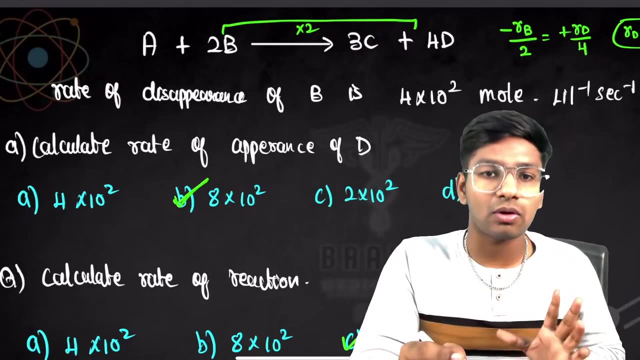 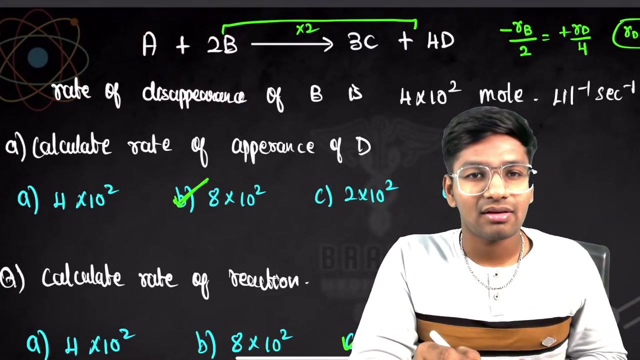 Do you understand? Specifically, the per mole is the rate of the reaction, but in the first question they asked the relation between this and this. if you simply feel it, you will understand. if you find it for all, if you find it for all, the same answer will be given. do you understand? 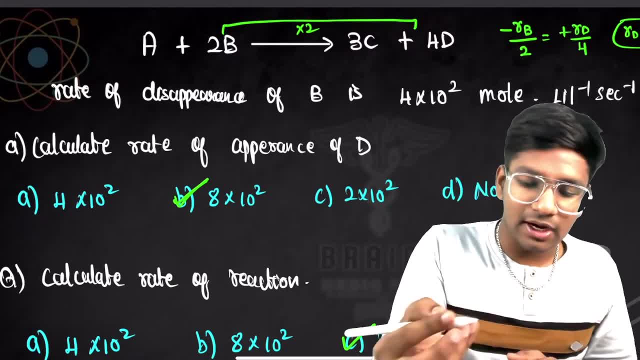 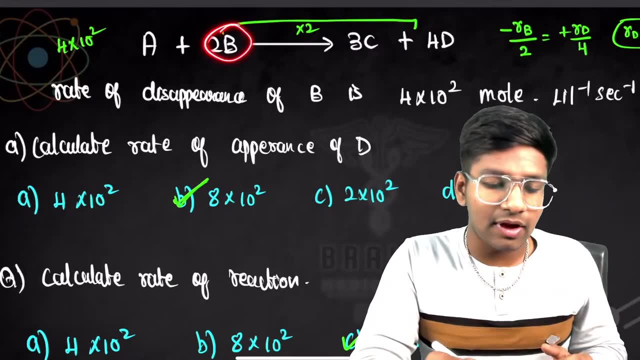 Do you understand? For example, take a: 4 into 10 power 2, correctly, 4 into 10 power 2 is the value for b. a and b have one different mole, then it would be half for a. do you know what will happen for a? 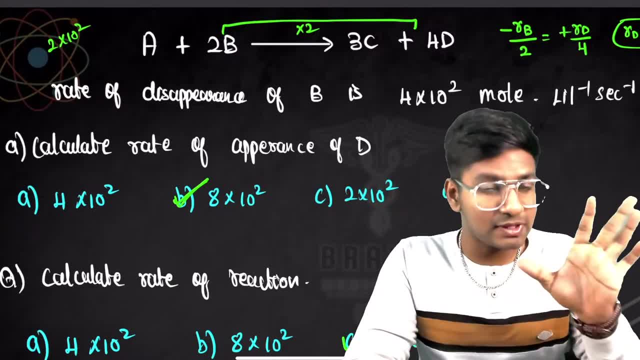 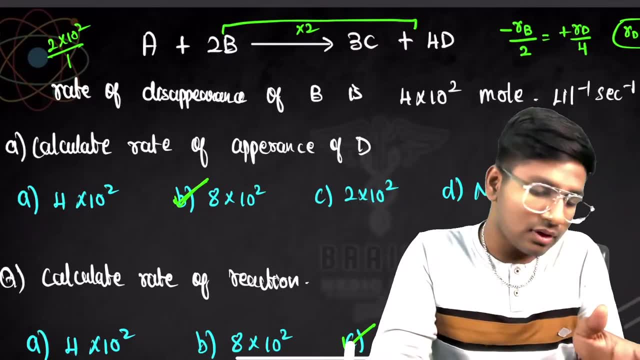 2 into 10. power 2 is particular individual rate of a. if we find the rate of the reaction using this, we will divide it by the coefficient 1, then what will the answer be Now? why I have named it as rate of the reaction. 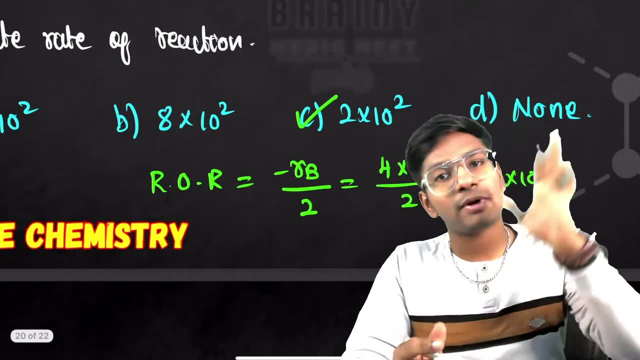 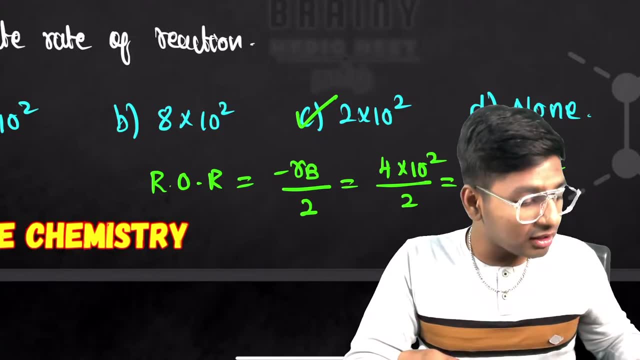 This change of the reaction. This change of the reaction, this change of the reaction, reading this lesson without understanding it. reading this lesson without understanding it. what is the rate of the reaction? what is the rate? I don't know. what is the rate of reactant and product? 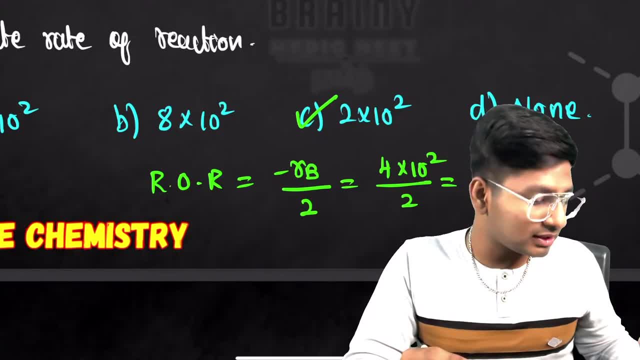 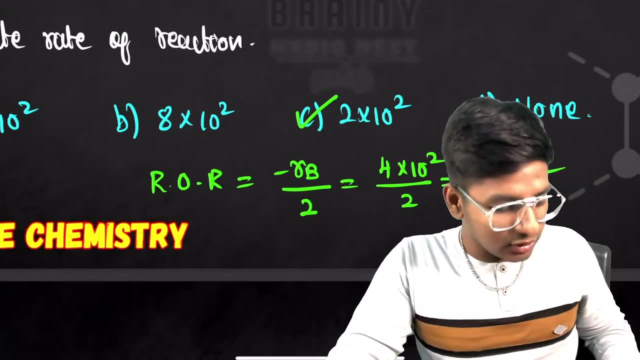 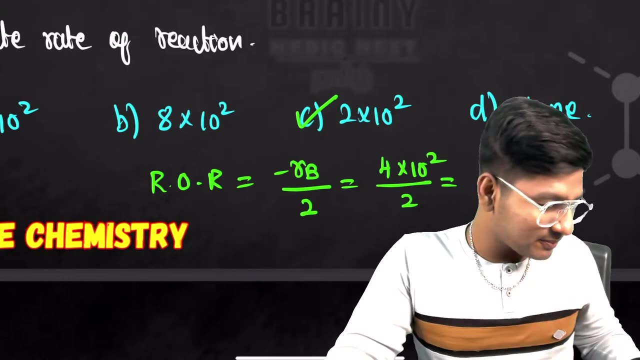 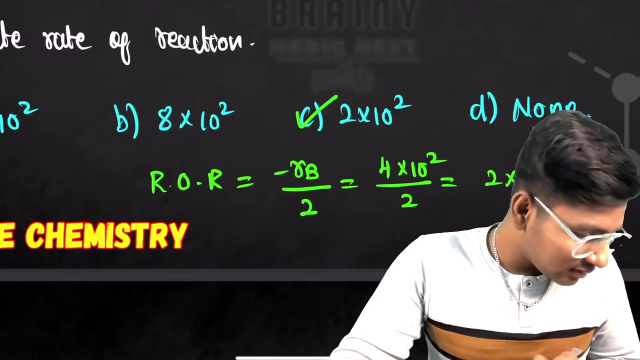 I don't know, but the lesson will be over. the lesson will be over. I didn't do the physical chemistry well. it's ok. I thought I didn't do the physical chemistry well. I am not teaching in the thumbnail. what is the trick? I don't understand. 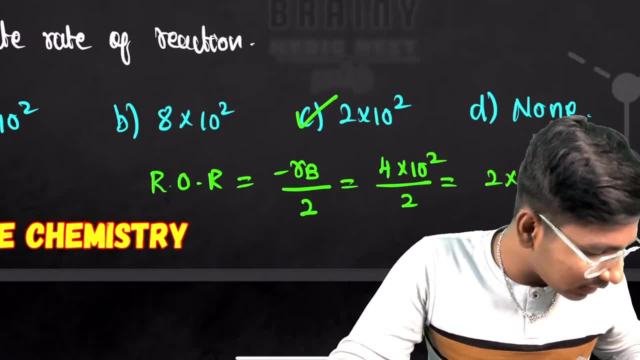 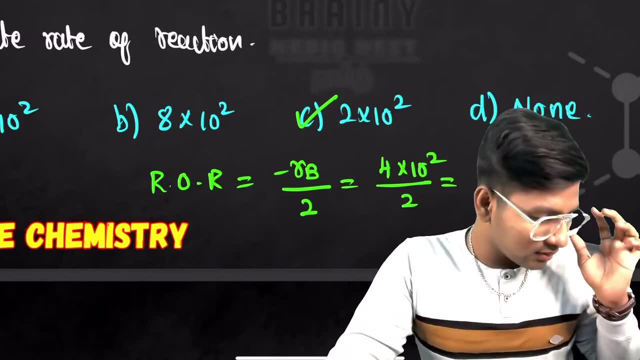 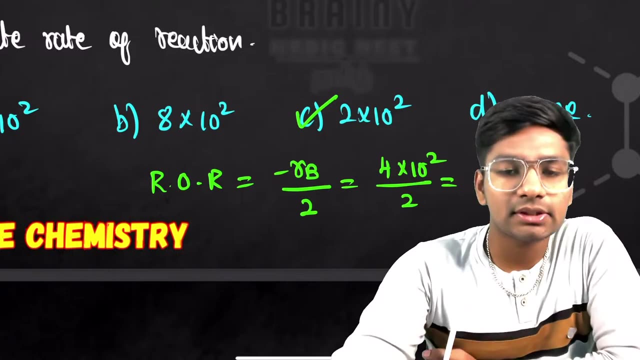 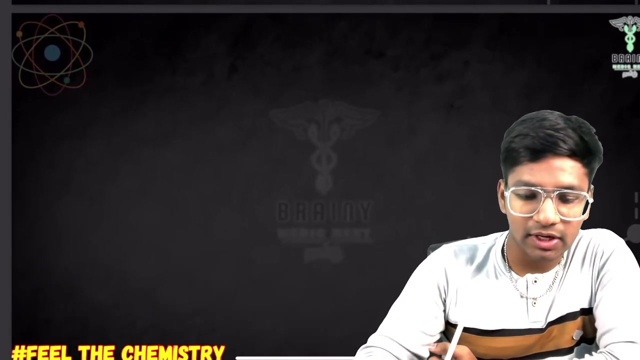 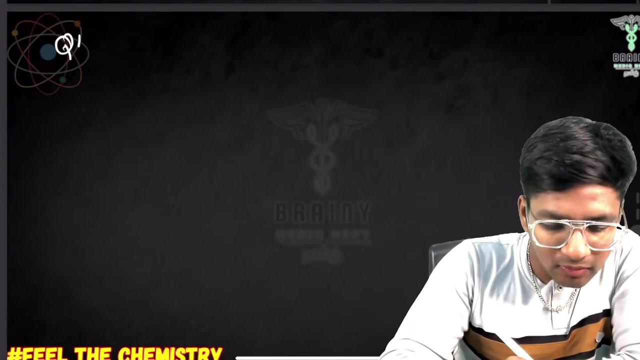 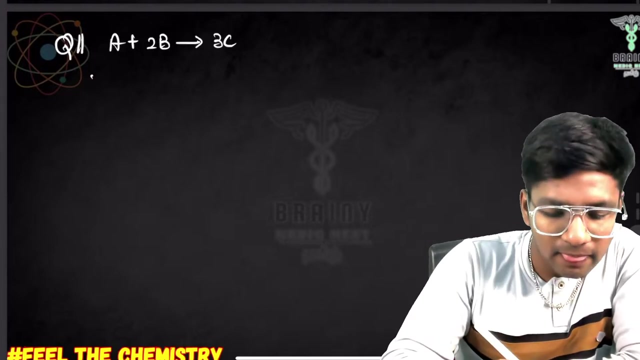 what are you telling? spelling mistake, yes, spelling mistake. TRICKS. you are doing super ok, fine, next, next, next. what is the problem here? hmm, let me pick the question. first question is: question: is: a plus 2b gives 3c, ra is equal to. 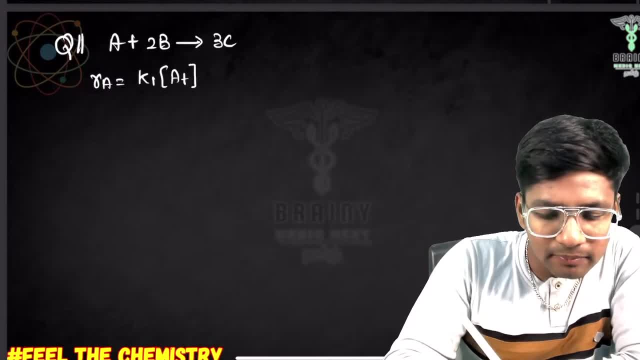 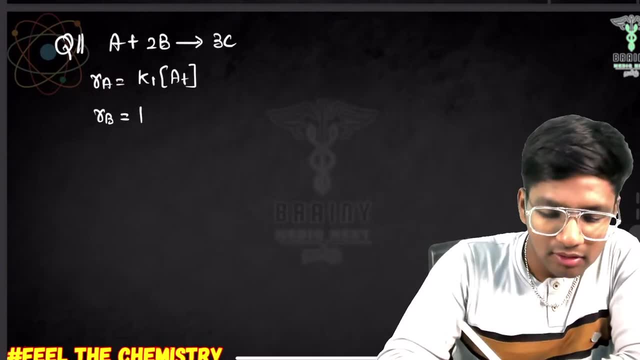 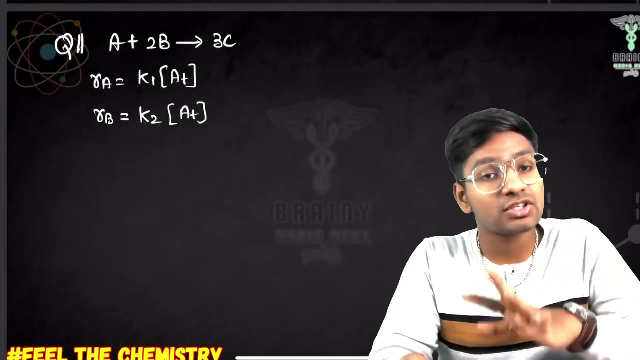 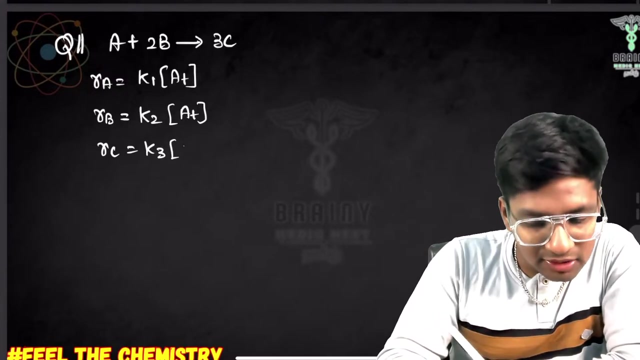 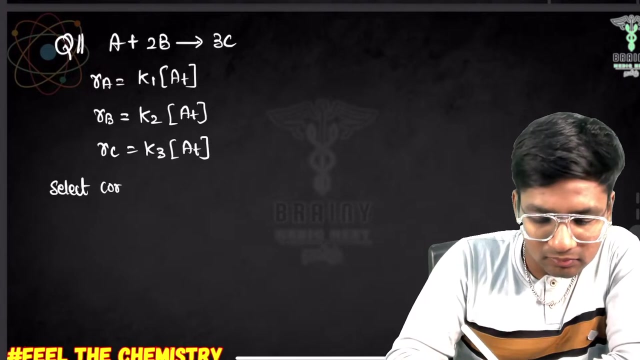 k1 of kd rb is equal to all chemical reactions, all chemical reactions, naming reactions, only one session. all structures of chemistry, all the things in your syllabus, I will give a separate session. what else? all reagents of your chemistry, I will give a separate session. all these are for revision purpose. 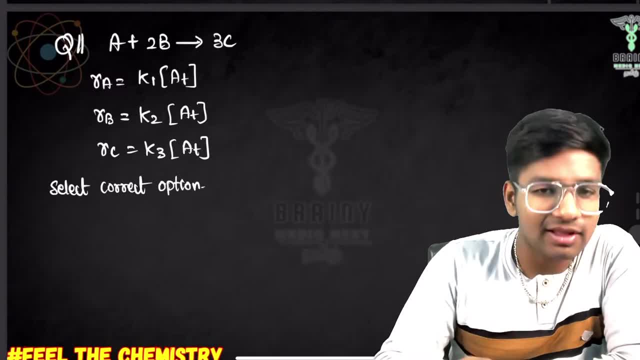 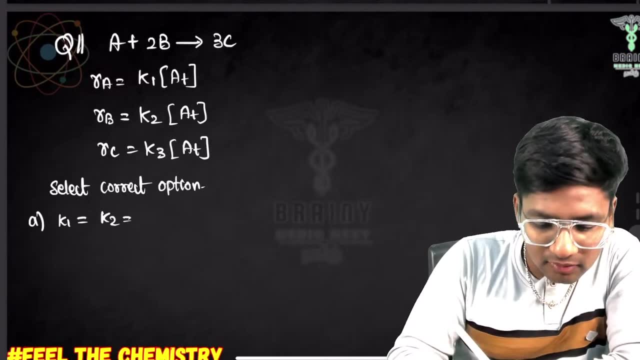 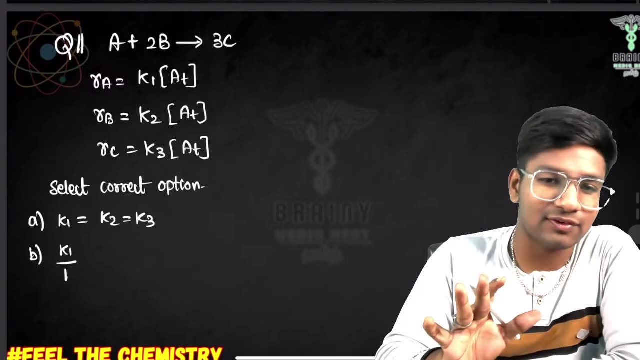 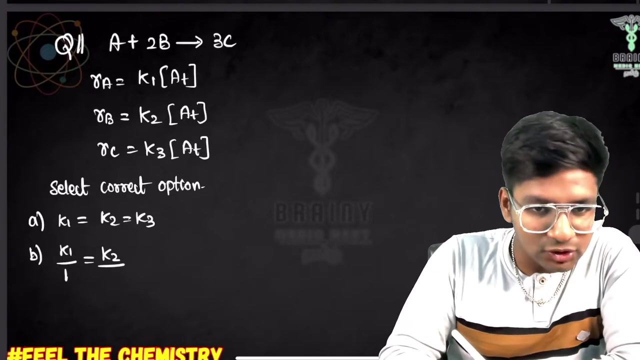 not for reading. remember that revision purpose. you will revise after reading. I am not saying that I will do physical chemistry perfectly. I will not do it perfectly. I will cover everything. I can finish this lesson in 1.5 hours, in 2 hours. I will finish this lesson in 1.5 hours. 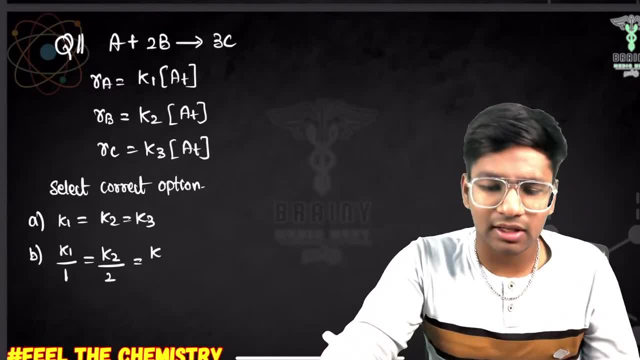 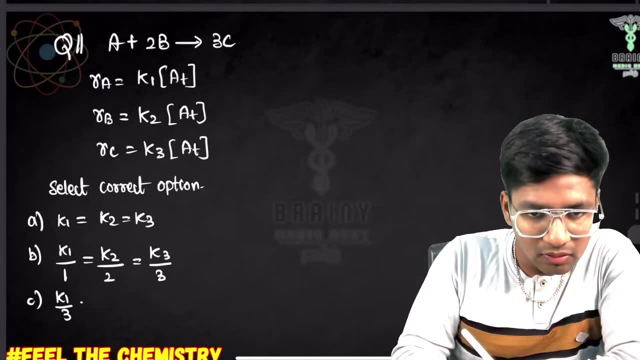 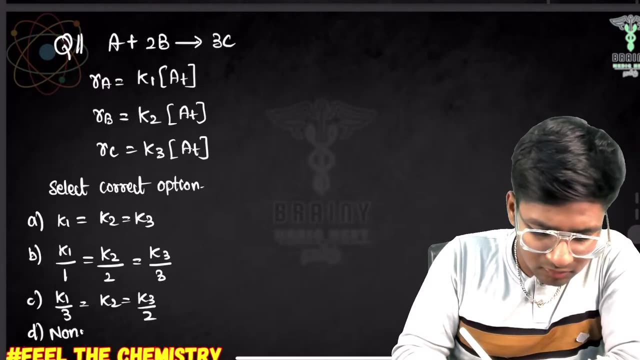 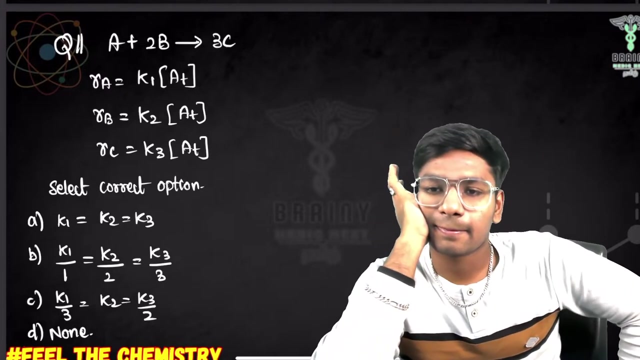 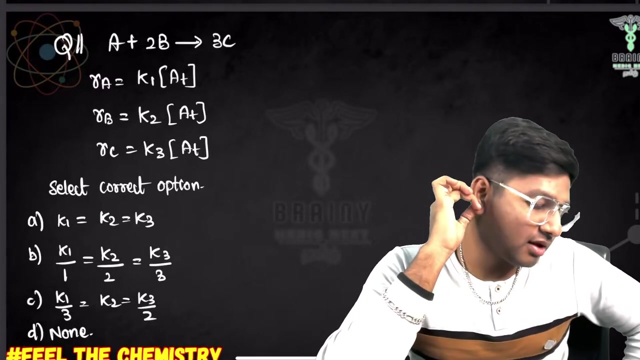 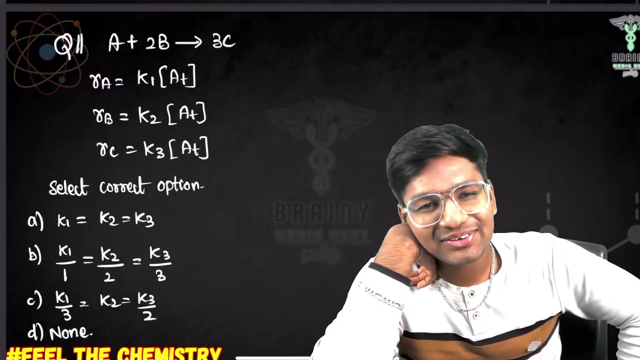 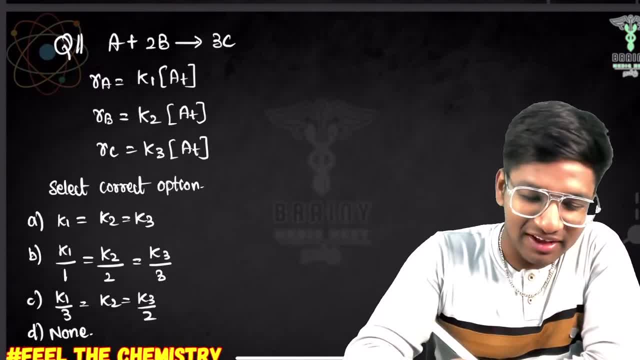 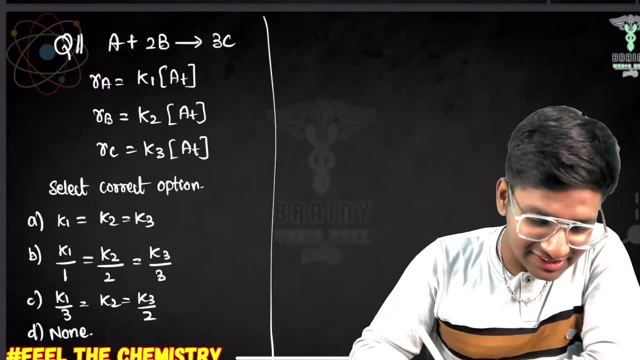 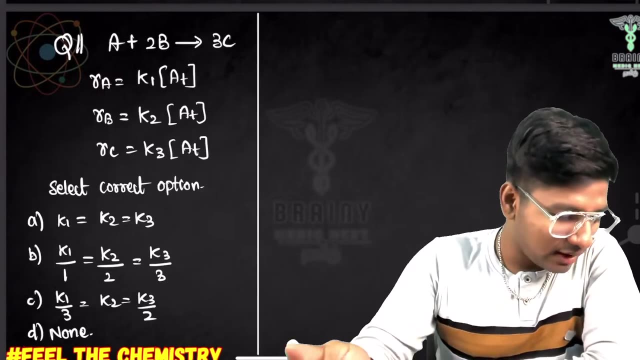 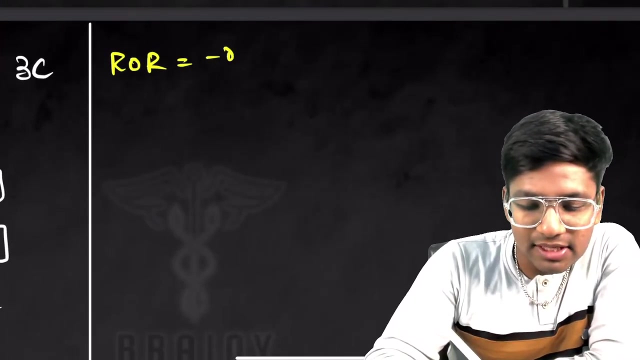 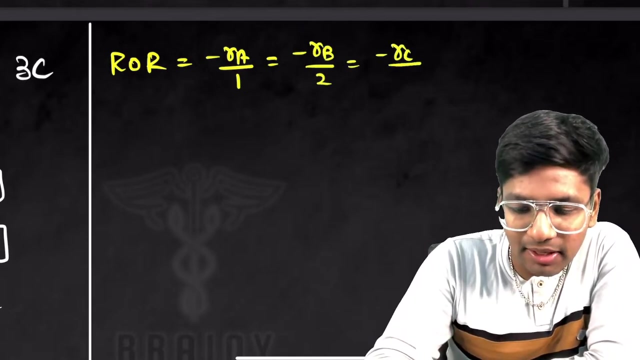 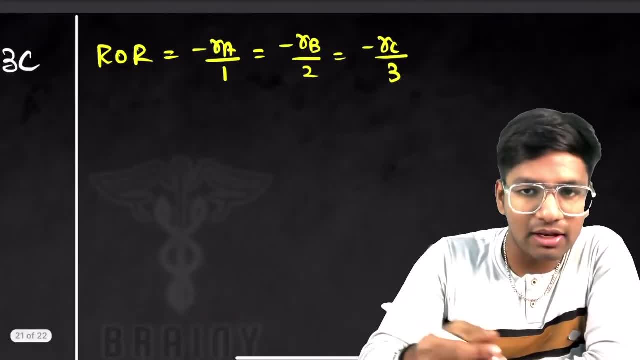 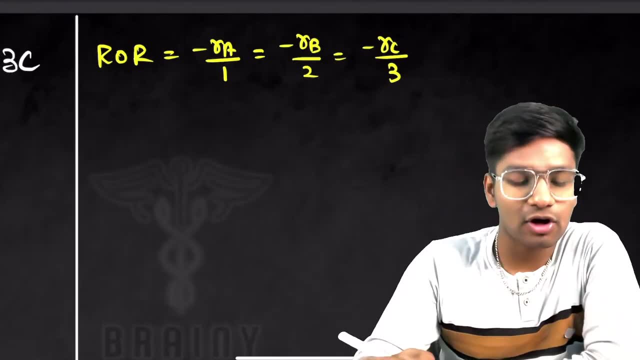 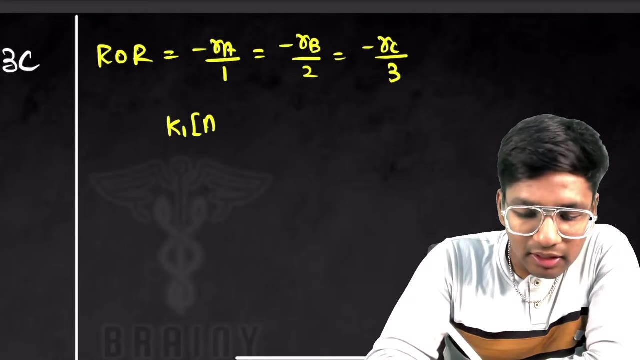 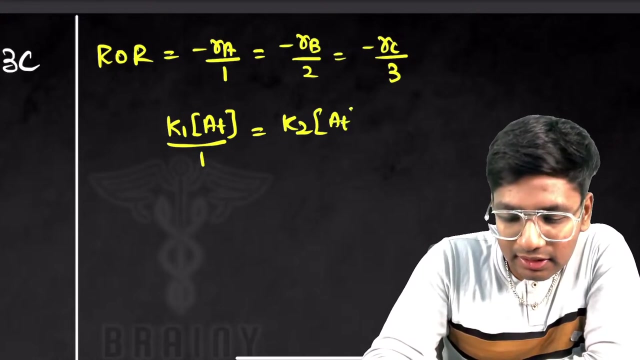 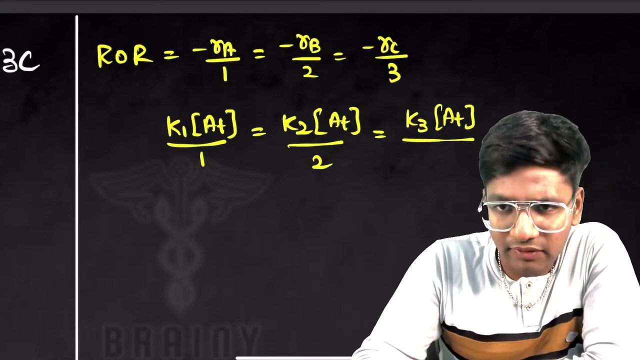 so just substitute the value of r, a, r, b, r, c. these kind of questions will come up now. take p y q. ok, take p y q. k. 1 a t divided by 1. k. 2 a t divided by 2. k 3 a t divided by 3. 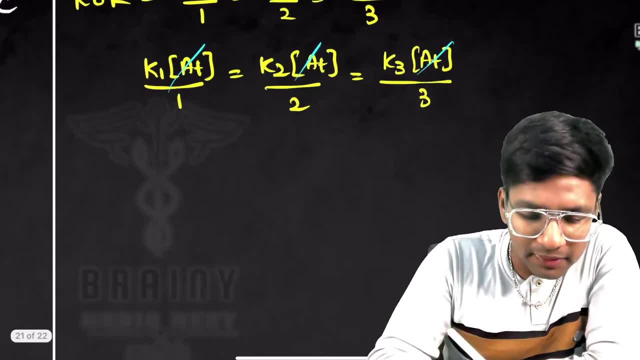 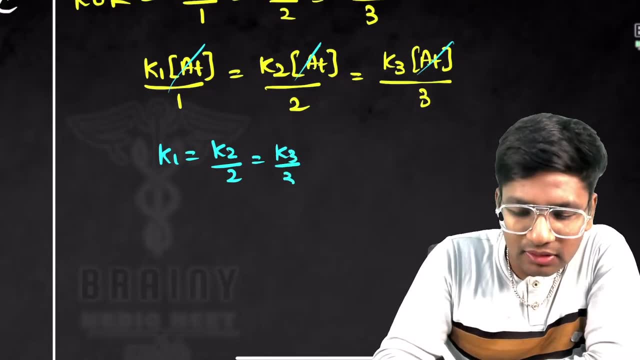 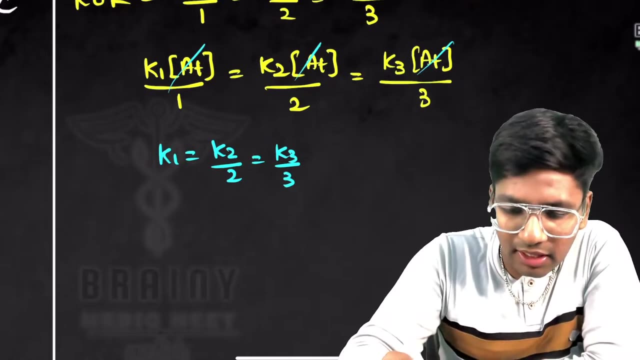 this common are the a, t, a, t, a, t cancel. k 1 is equal to k 2 by 2, which is equal to k 3 by 3, correct? for example, if I take p as the value, all these are the rate of the reaction. 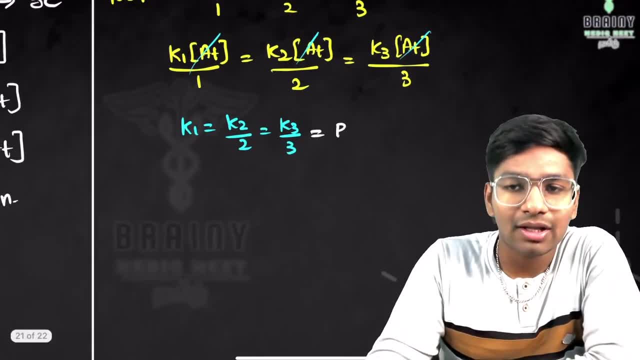 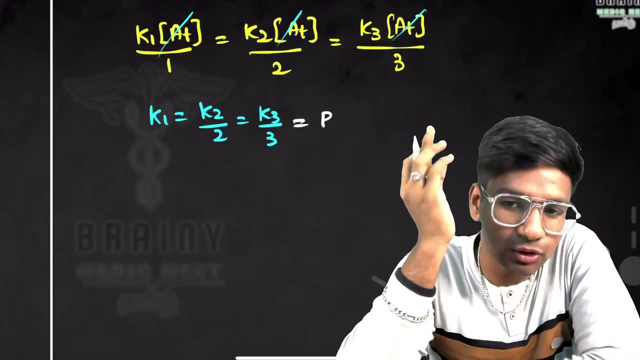 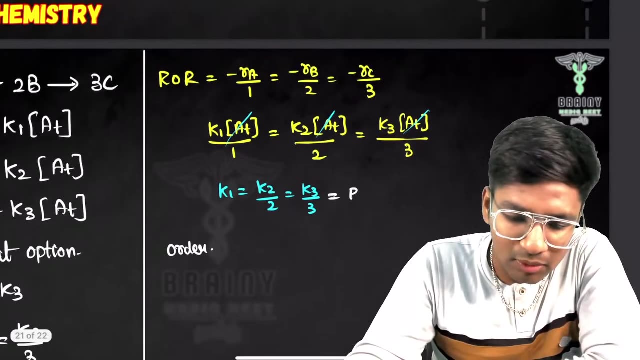 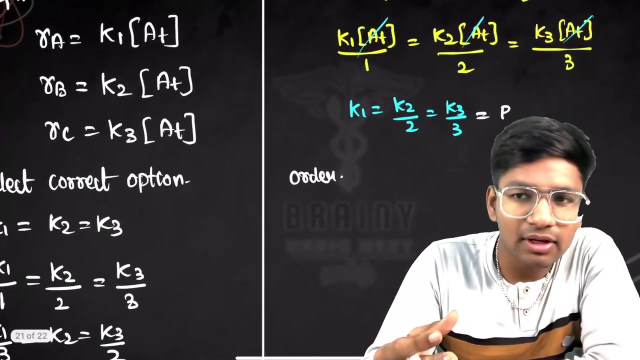 p is the rate of the reaction. what will be the order? what will be the order of the rate of the reaction? what is r c? what is r c? I don't understand. what is r c? I don't understand. what are you saying? 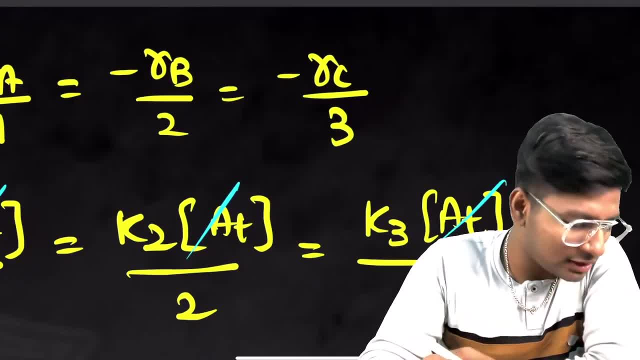 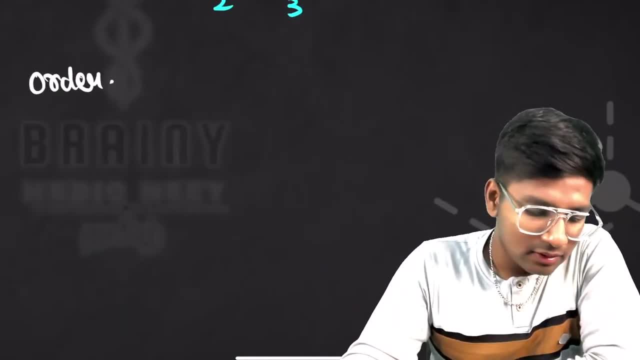 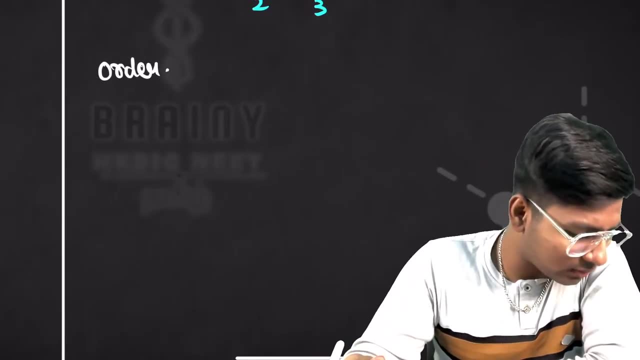 the question is: the question is ok. ok, I have put minus here, minus, minus. I have put. now it is correct. now it is correct, I have put minus without knowing I have put minus. which will have more rate of the reaction? individual rate of the reaction. who will have more rate of the reaction? 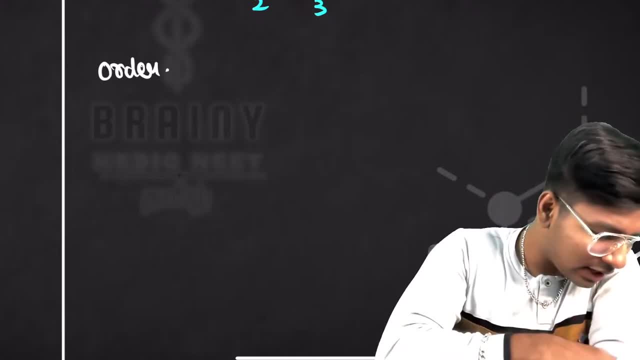 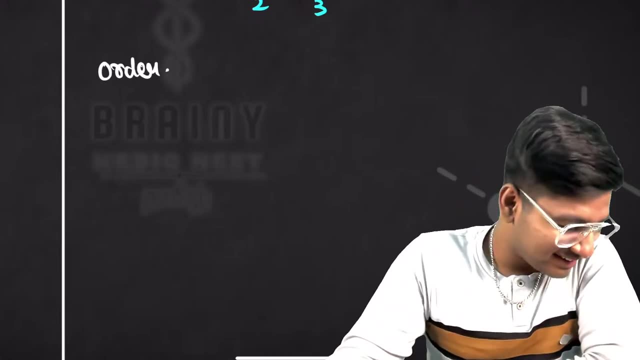 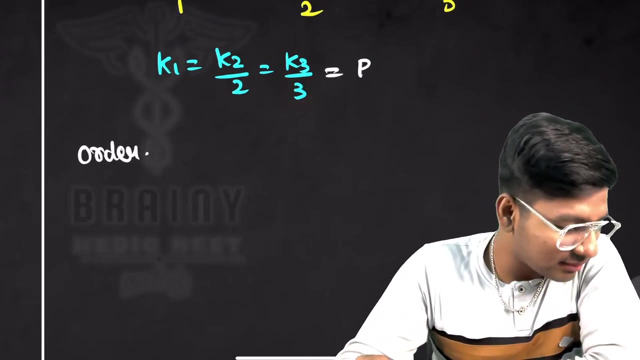 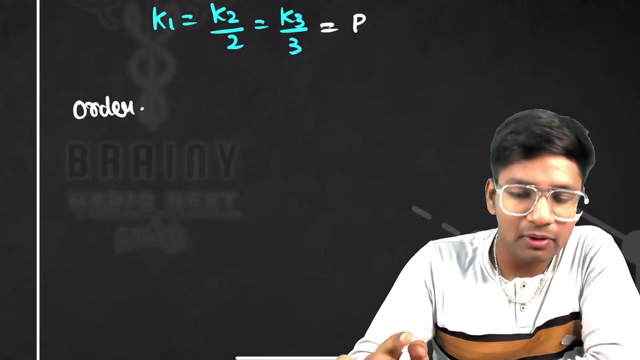 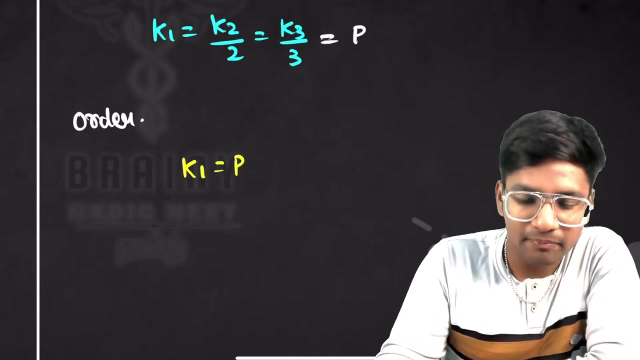 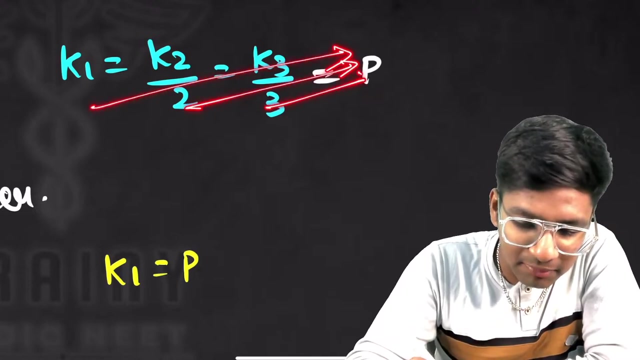 I am looking for the option which is 6k 13k 2. I am looking for the option which is 6k 13k 2. I have putIP. look at the question: who has more rate of the Co? efficiency is more than. 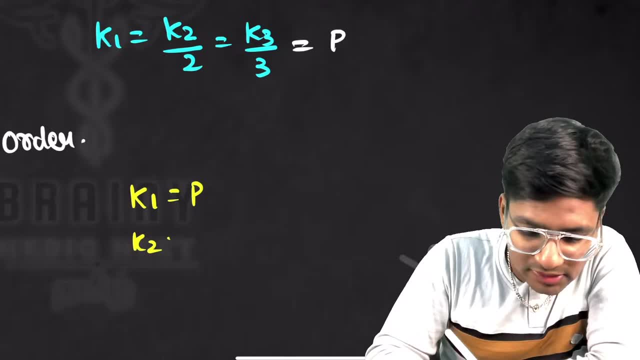 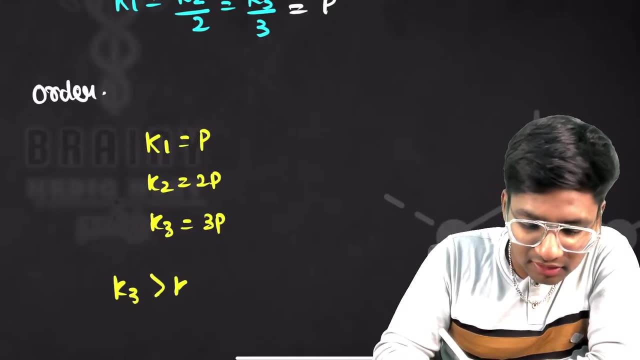 here. then what will you do? k2 is equal to 2p, k3 is equal to 3p, then what will you do? k3 is greater than k2 is greater than k1. no one can explain this easily. I will explain it quickly. 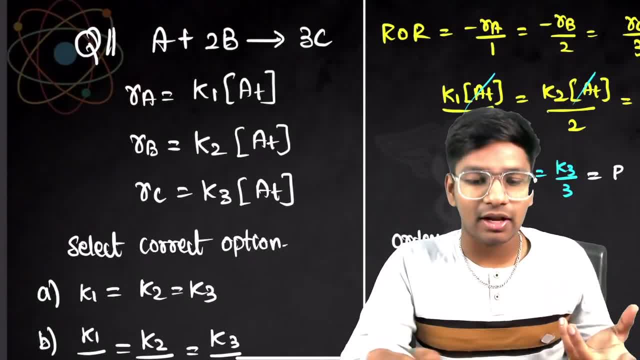 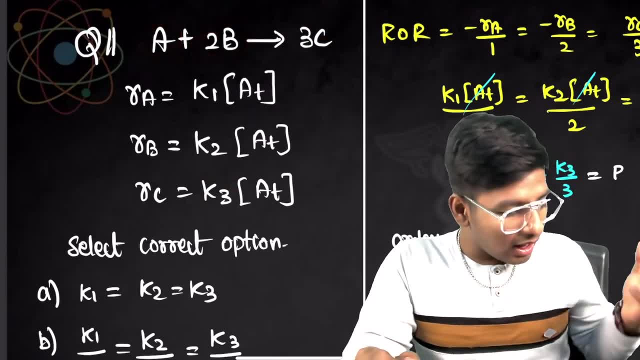 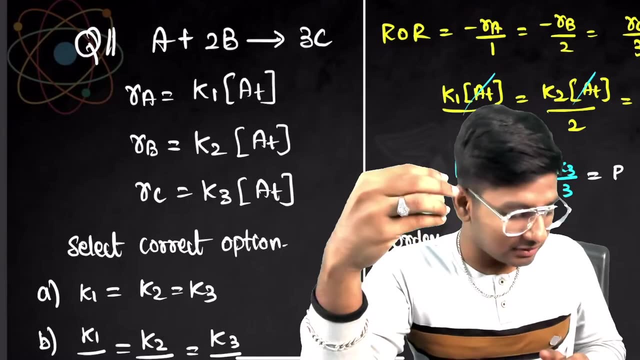 what I have explained easily is: co-efficient and rate have same relation. then third one, c is k3. that will be more, then this will be more. I have explained 2-3 methods. I have explained this method to you. I am literally telling. I am literally telling. 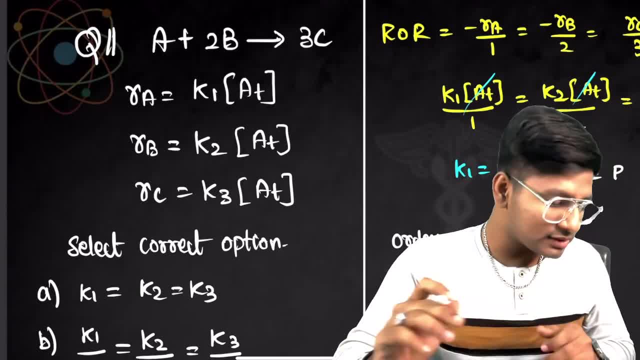 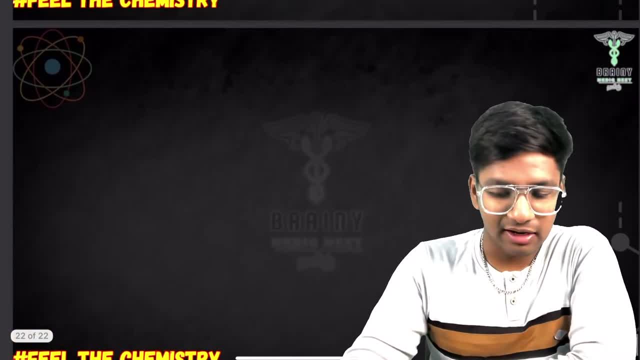 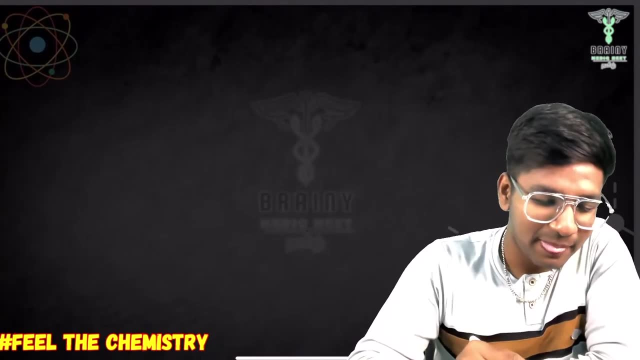 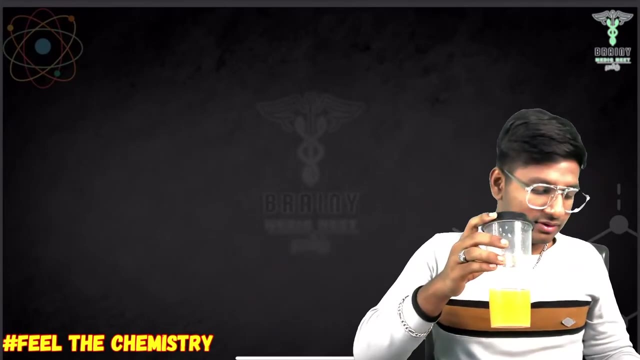 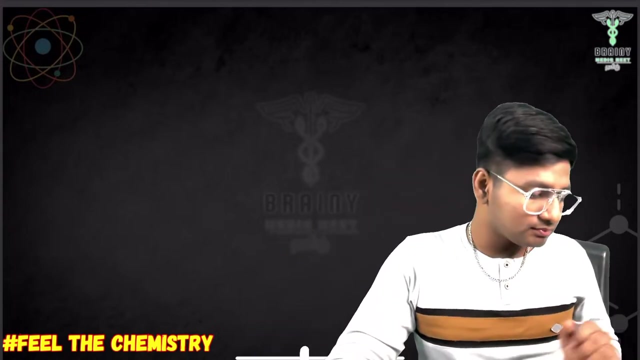 every youtube channel has more viewers than bmnt. thank you, Undertaker. Undertaker has more viewers than bmnt has more viewers than bmnt. Undertaker bro is there in competition. Undertaker bro is there in competition. Undertaker bro is there in competition. Undertaker bro is there. 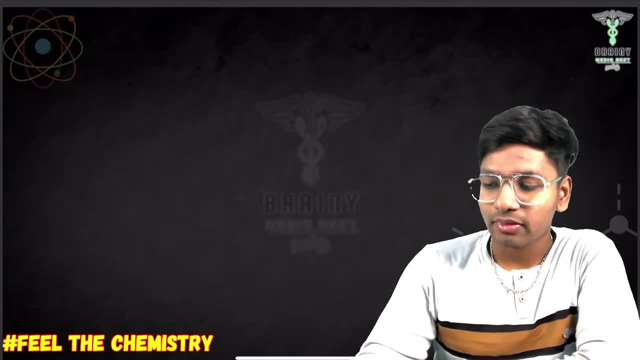 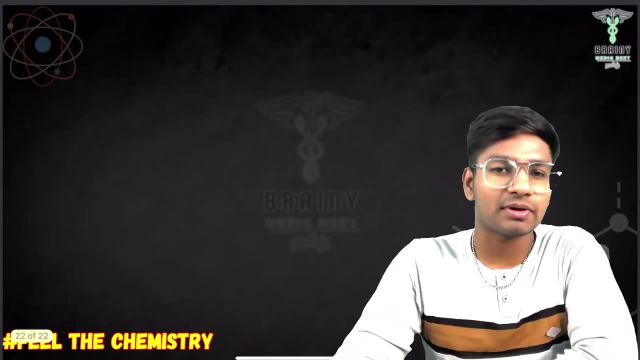 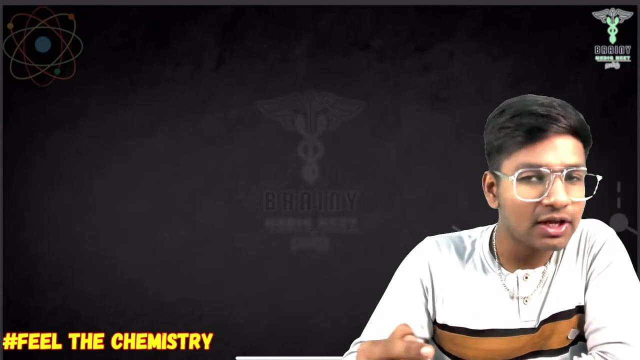 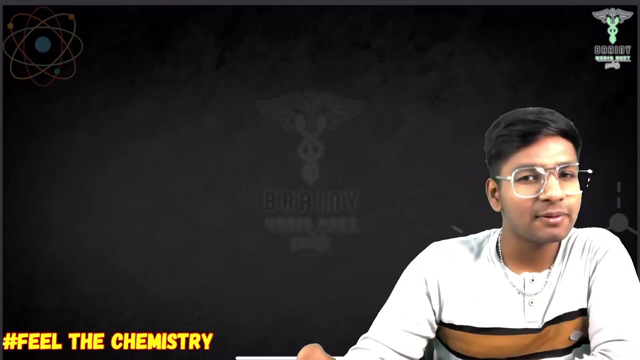 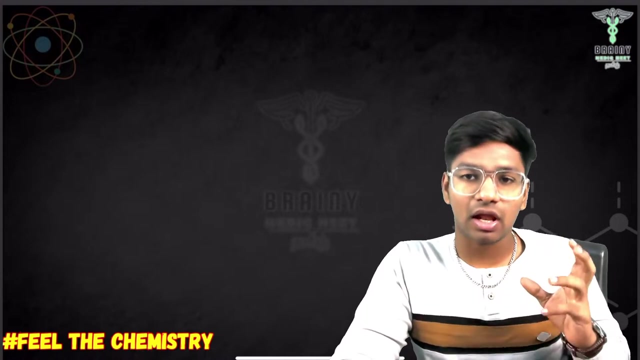 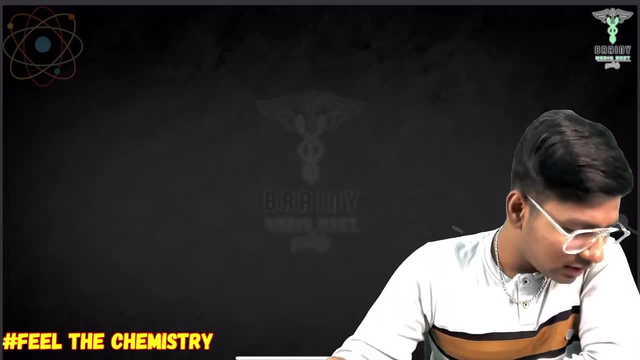 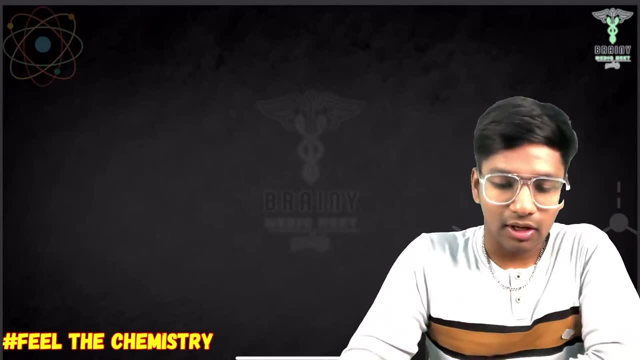 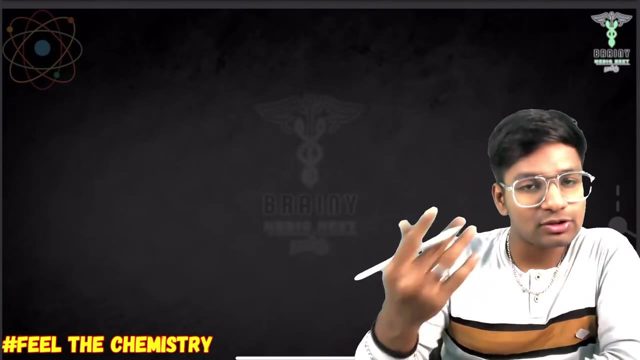 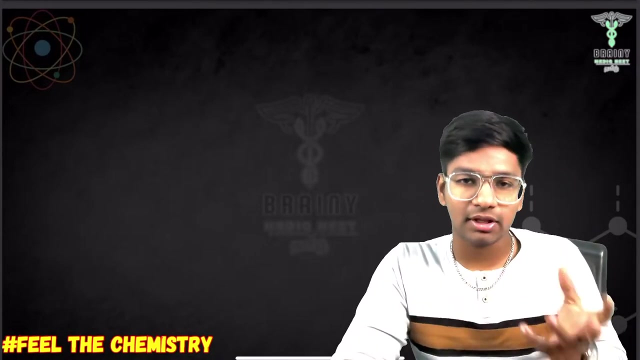 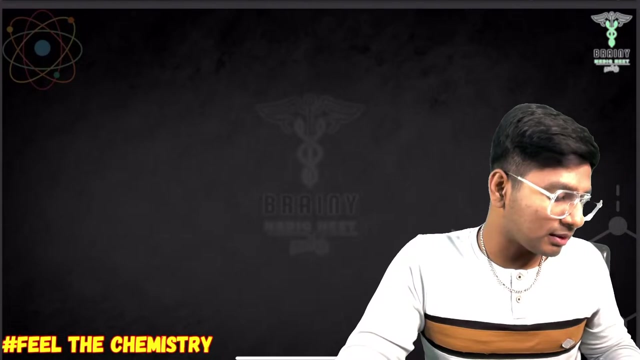 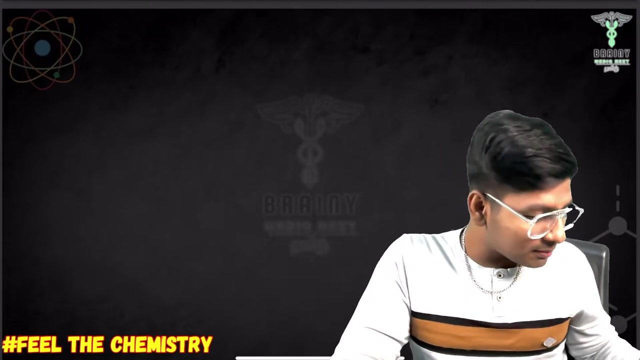 okay, okay, uh, um, um, um, um, um, um. option with my subscribe button in pocket and then membership. now either you're on for membership, on in there, but I don't want to be the membership options for the nodular area. you're gonna? members, come on to the Nia live. 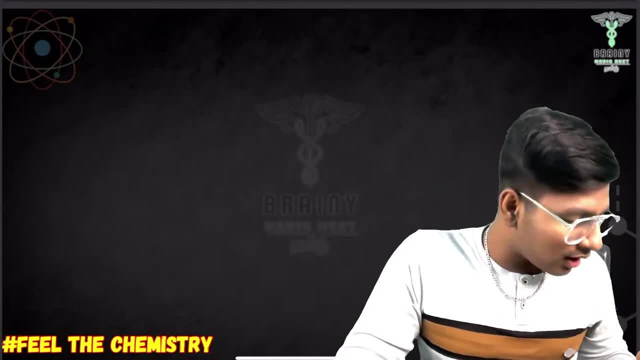 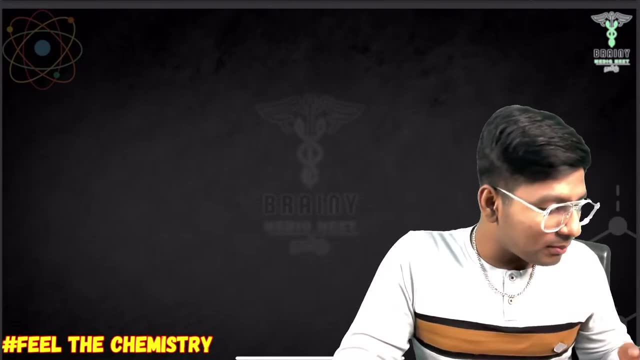 for a lot. members. come on to the Nia. don't solve a lot from I ended a shout-out to photo status update. Murray and I'm over here currently and again I'm gonna tell you: okay, I know, membership, membership you can put on a solo in the channel. 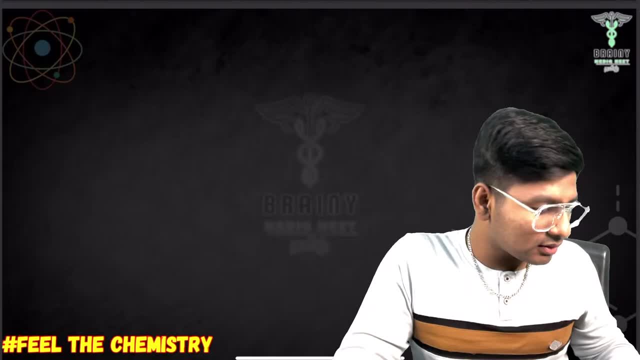 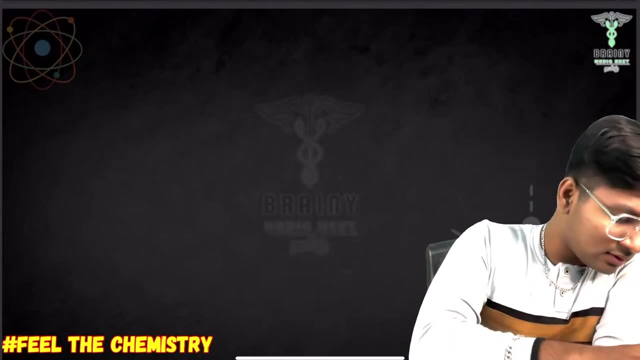 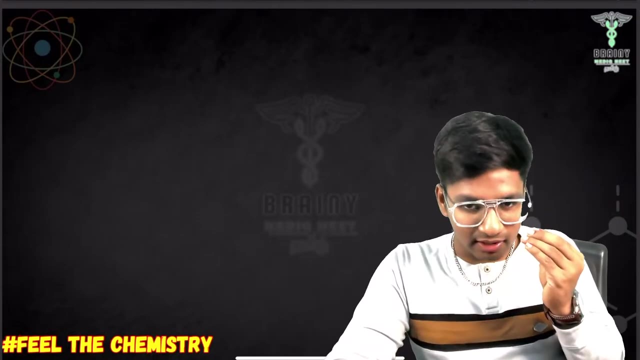 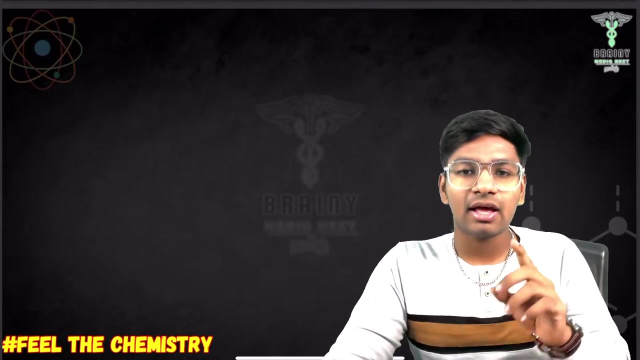 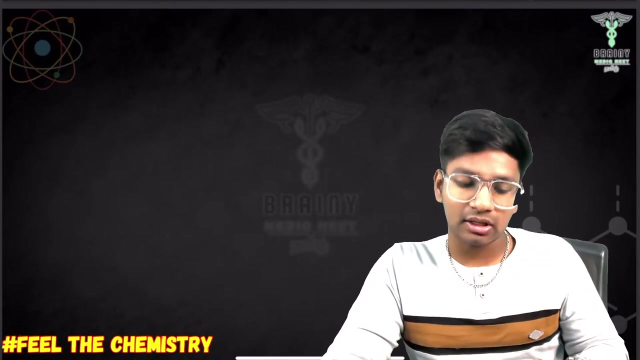 now you're going to go to the truck strategy videos. what to me? what's it on you tube? let me play my strategy video. what don't put it on in the channel a? not portal of the lecture. written part of the you, you, the solo in the individual channel and not portal of the lecture here in clear. 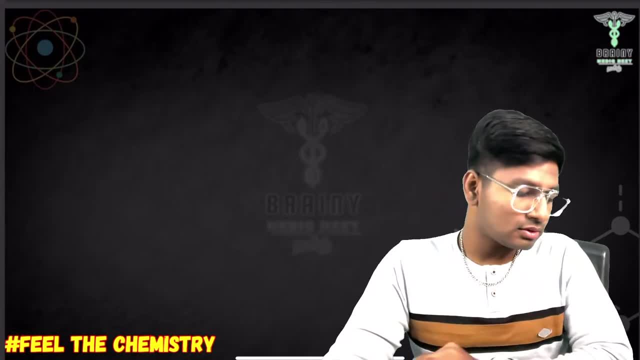 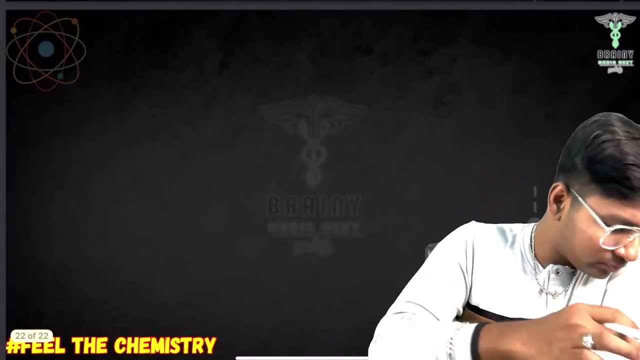 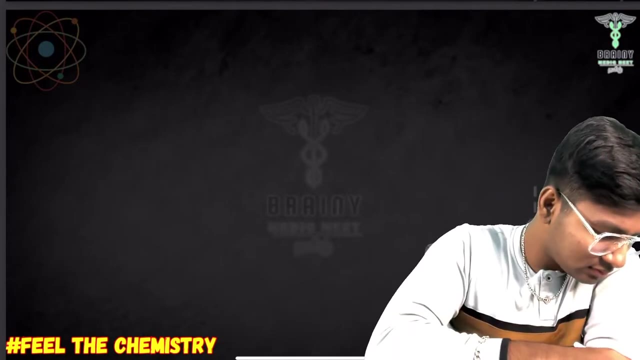 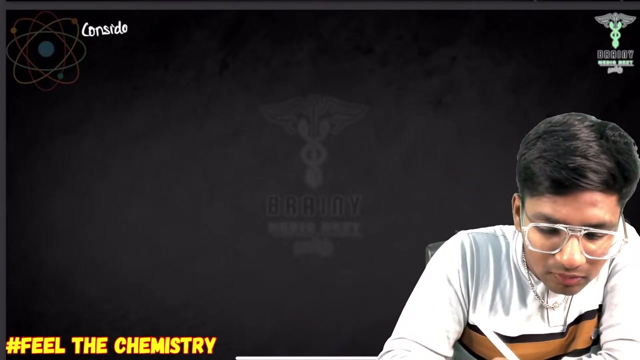 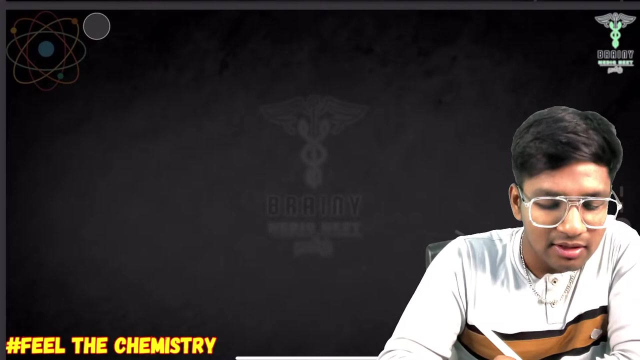 of in. so we part of our other moon is objective, even moon moon. a teacher, such in our program, could I? you know what? I'm not on only strategy, strategy, strategy, strategy, matter what she would you? okay? so if I let it be a question either. if I give you a question, you ask me. I'm not the kind of person I am. 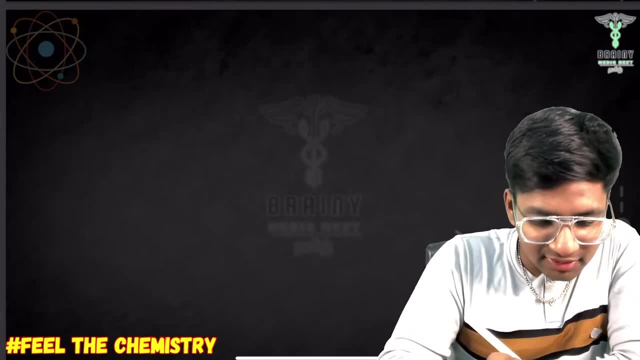 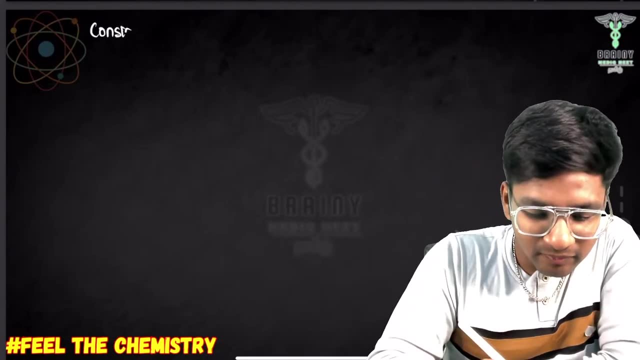 you know that you are a quieran, or would be the question that is asked, a question and guess you're not the one who will answer that question. you know we're going to be in the same class right today. I think that. again the question: clearly I need the entrepreneurial. 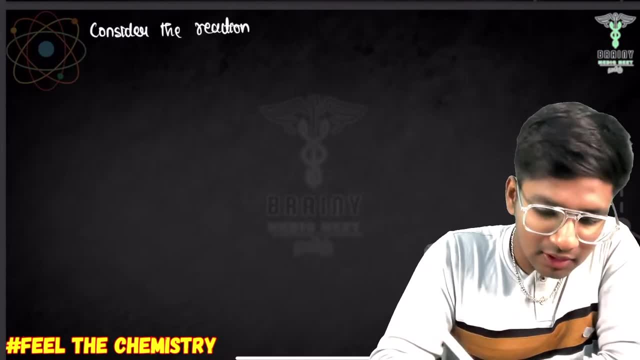 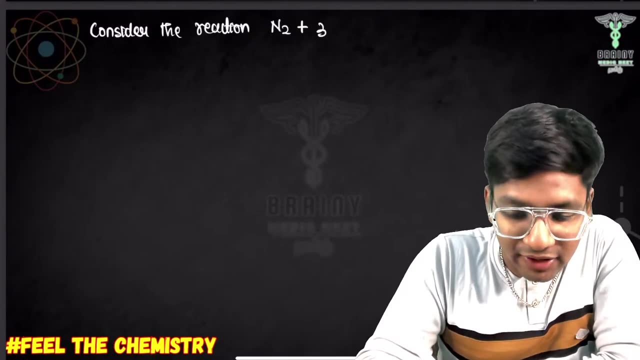 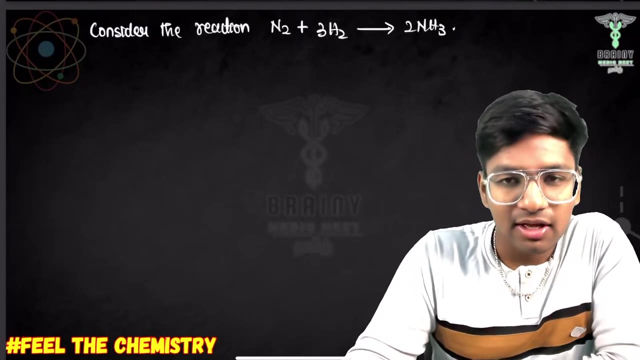 time would be quite different, right, and I think that it's a totally different. That's a factual thing. okay, 2NHT, I think I can make a strategy video for the whole week, but I won't make two videos per month. 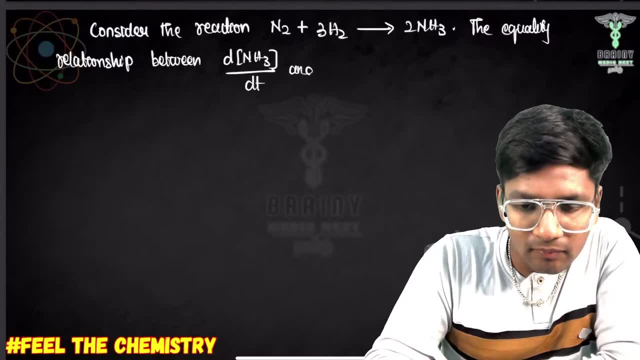 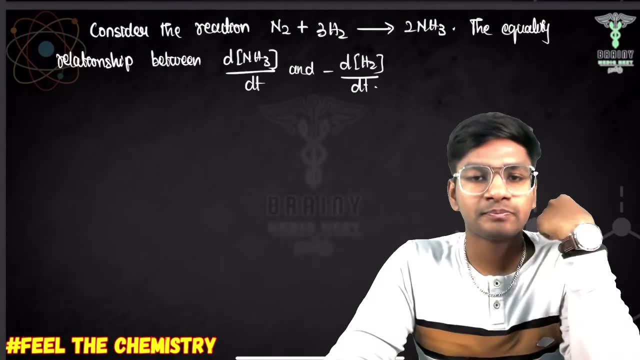 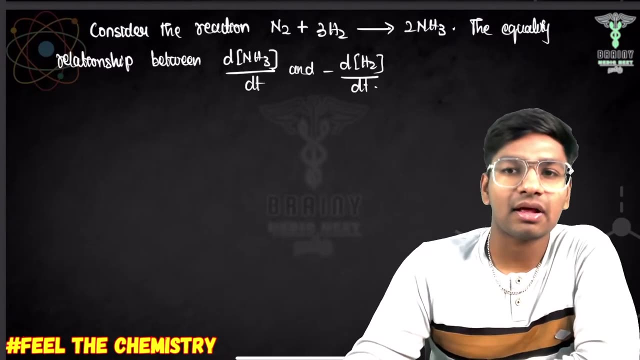 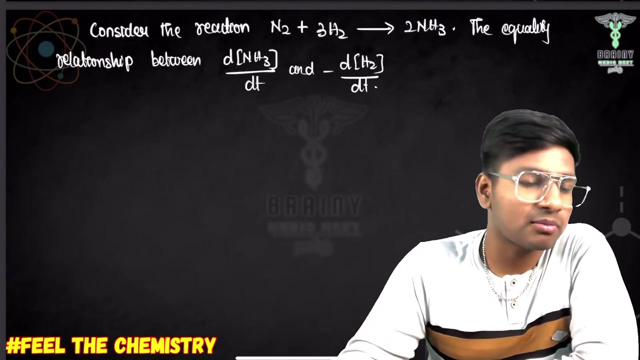 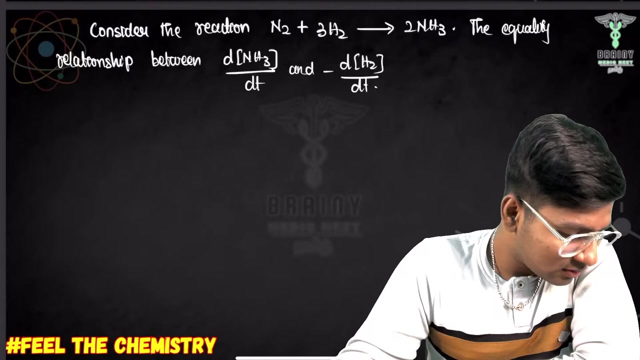 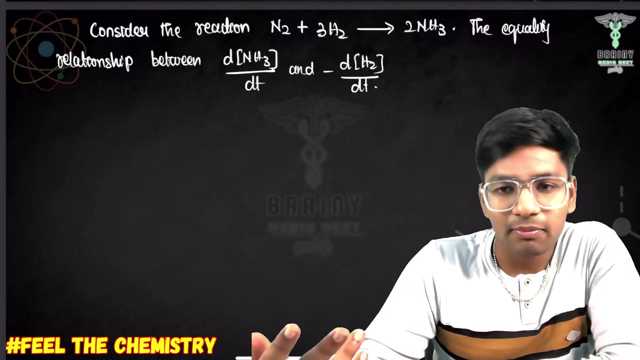 Answer question paper hasn't come yet, exam hasn't happened yet. I don't know how the question will be. the pattern has changed. the cutoff is telling for his wish. it seems like his father is taking the question paper. Even if I study now, I can get 180 in chemistry. even if I study now, I can get 180 in physics. then why are you studying for a year? you have to study for the last two months, right? 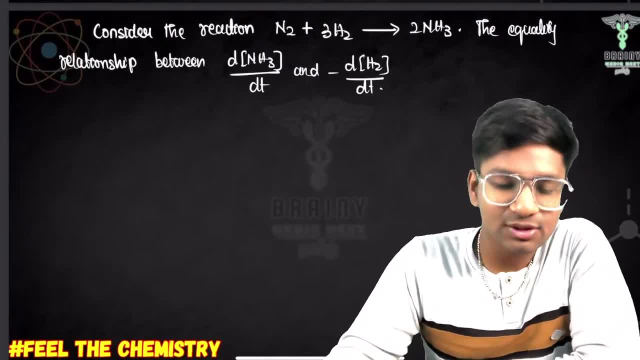 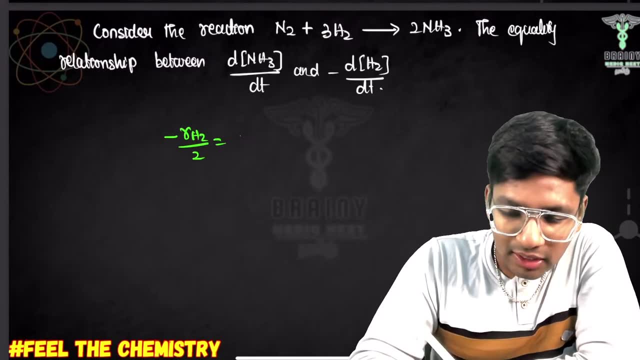 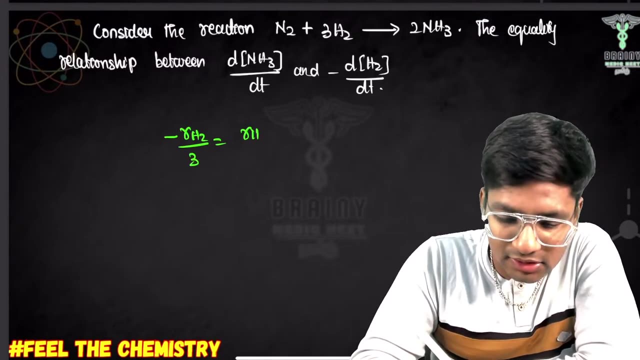 Minus 2 by 3, direct answer. this is what I want from you guys. Okay, so here: rate of H2 divided by 2,, which is equal to rate of NH3 divided by 2, 2, sorry, 3, 3,, which is equal to rate of NH3 divided by 2, correct. 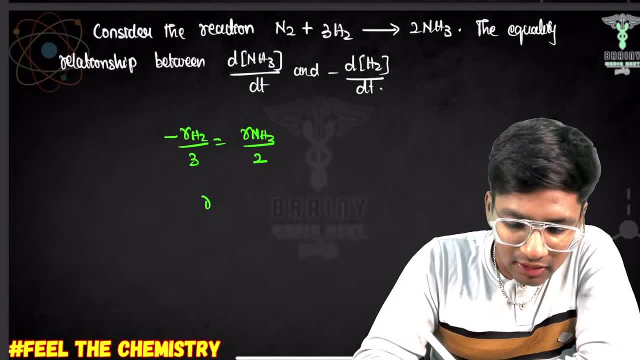 Now, what is the rate of NH3?? Rate of NH3, you have asked the relation. NH3 is equal to rate of H2 minus of 2 by 3.. So 2 by 3 into rate of H2.. 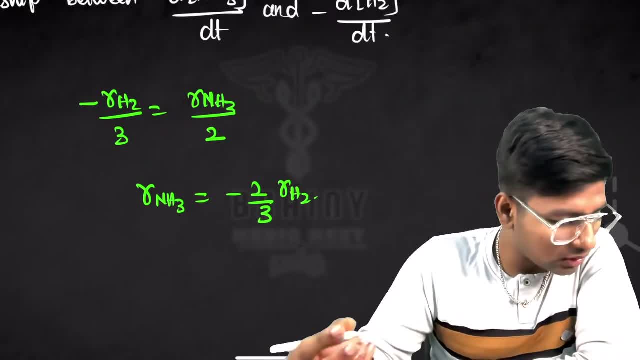 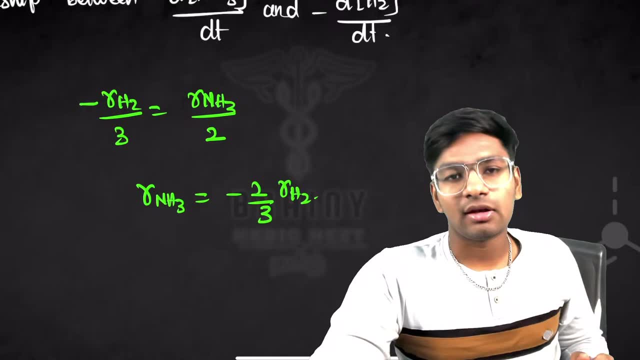 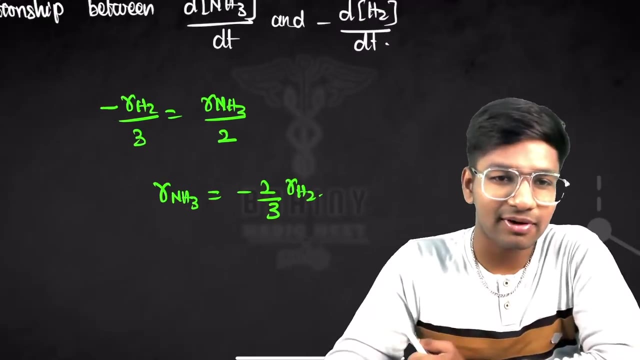 Rate of H2, okay, Hey, if tomorrow is 4 days, they will write it today. In one night they will write the same thing, like the song in the movie Suryavamsaam. Okay, there are still types of rate. let's go to types of rate. 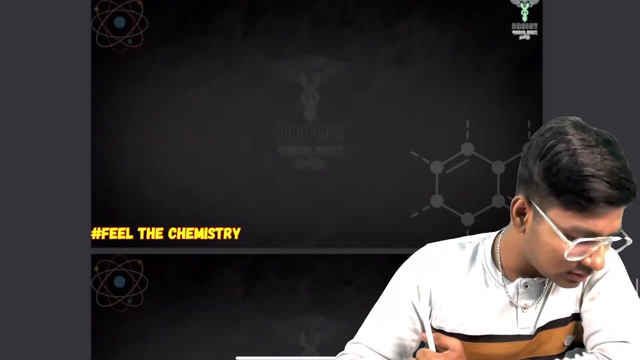 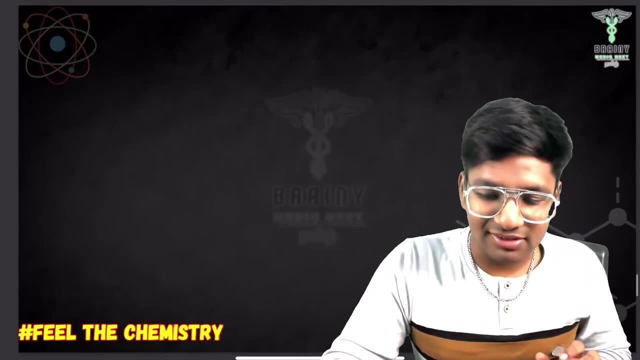 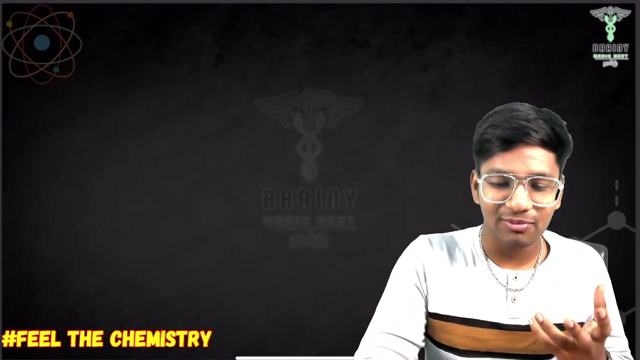 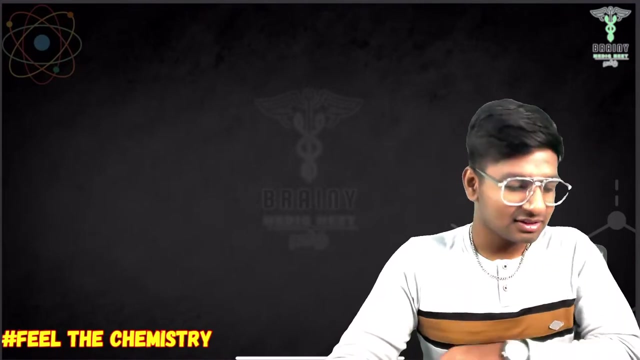 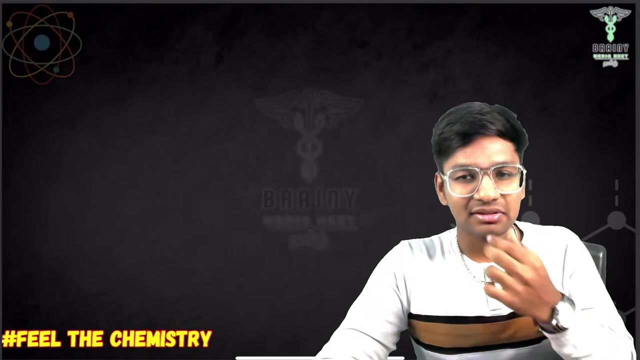 a mother for her child. if a father works hard for his child and earns money, you are making a crash course. will the food you eat get digested? will your gastric hormone get secreted? will the pepsin get transformed properly? will the proteases get activated properly? 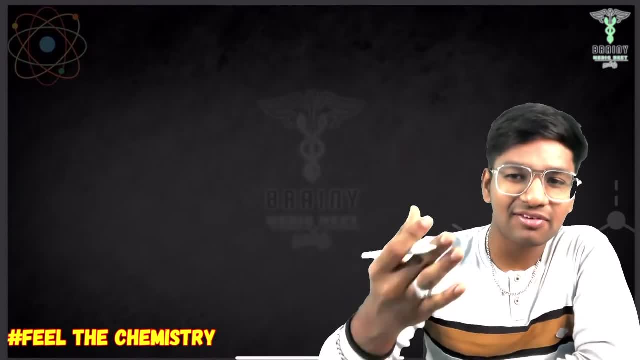 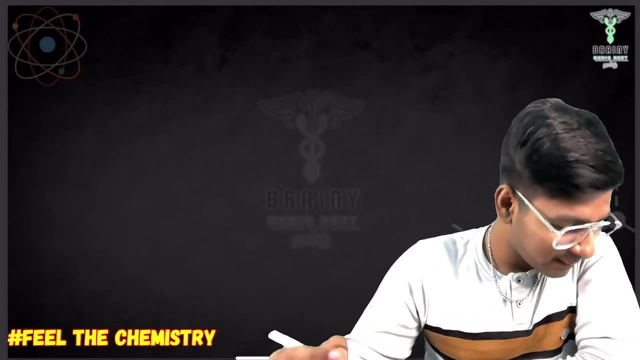 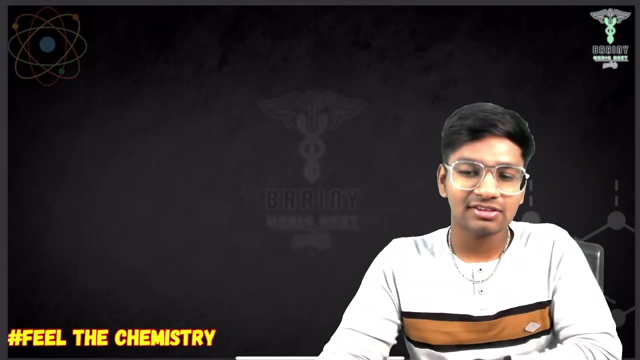 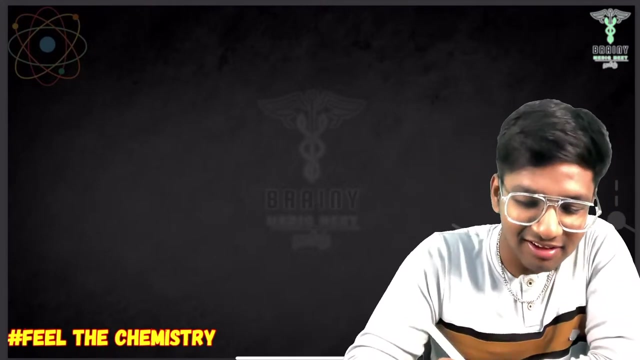 will there be no ulcer in the pyloric and fundic portion of the stomach? tell me, will there be ulcer in the deodorant? will there be cancer in the deodorant? will you do like this? how many have worked so hard and made money for their children? 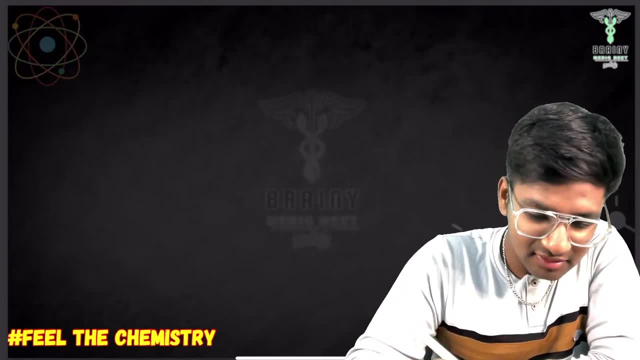 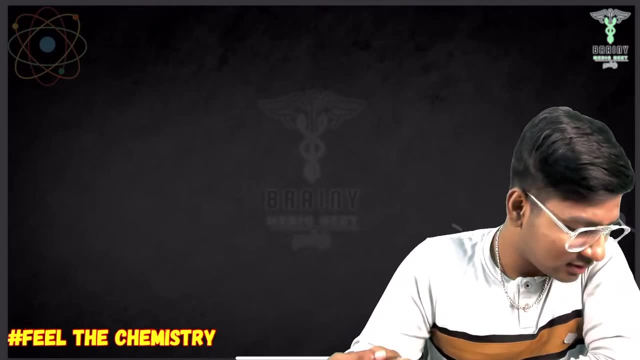 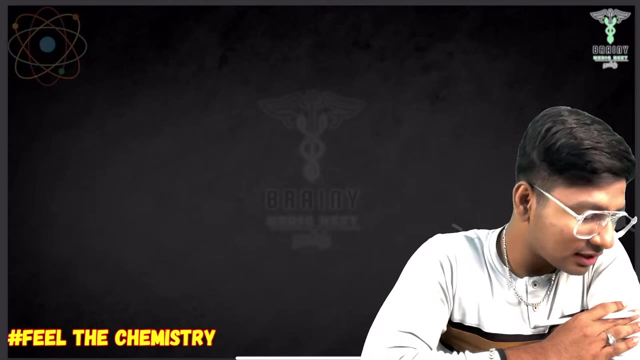 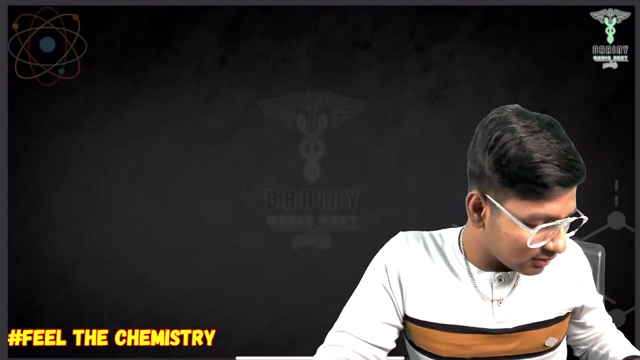 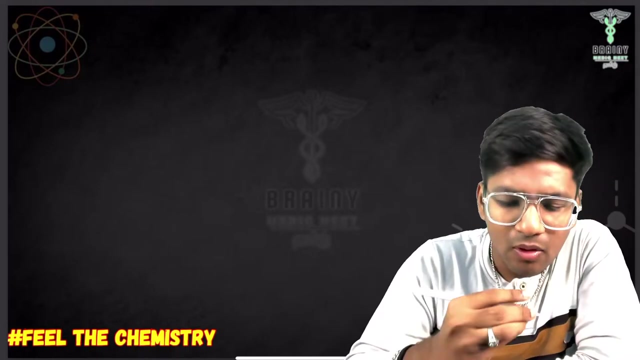 do you know what they do? what is reduced? what is reduced type of rate? please tell me how to study Electro chemistry and chemical kinetics. please tell me how to study it. what is reduced for digestion? ah, digestion chapter reduced. ha aiyo dey mbbs le reduce. 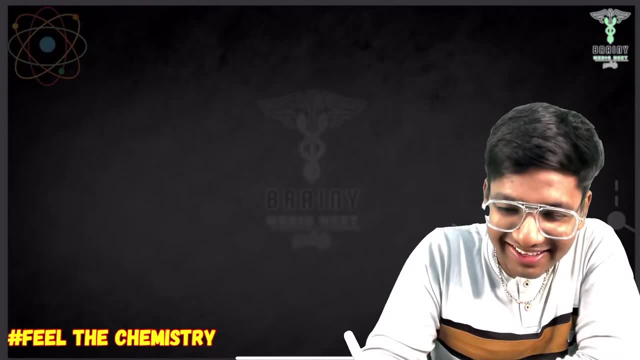 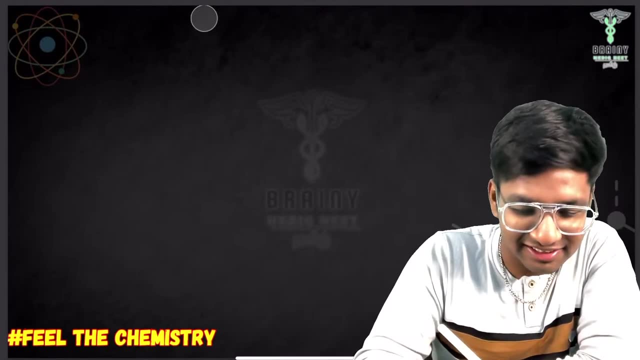 hagele daa why daa yobti pandreyenge mbbs le irukk le eneke mbbs le irukk le g8 chapter mo g8 ne tanya aur fisiology lesson ne irukke eneke anatomy le ne padipai allathe om type. 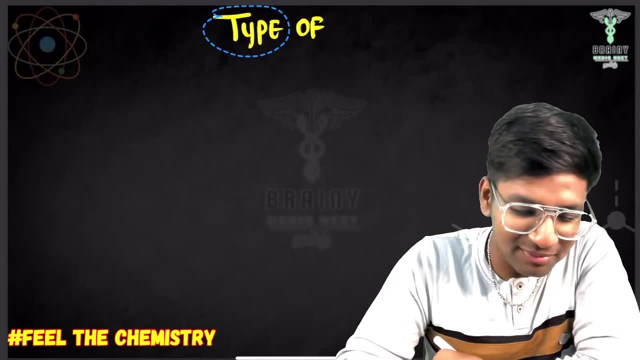 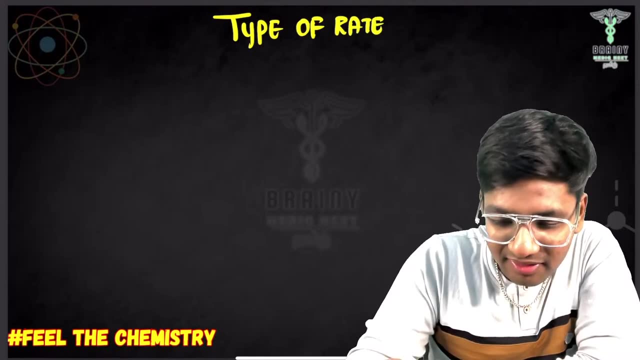 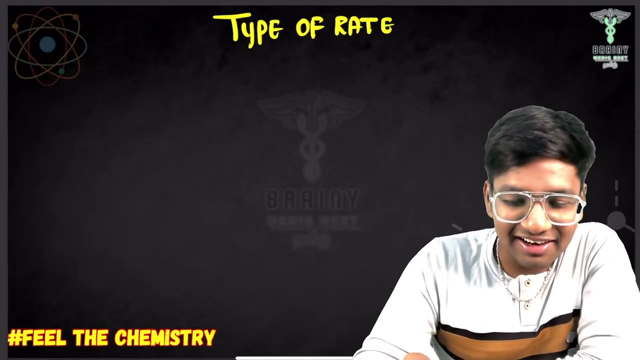 of i mean teacher le daa student ra manandhinge pora daa denge: why daa yobti pandreyenge great na neet, na neet, neet, neet nadathren ne ne teacher ra consider pandeya yobti yobti. 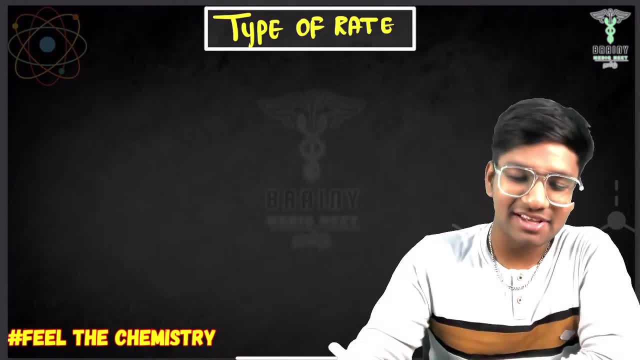 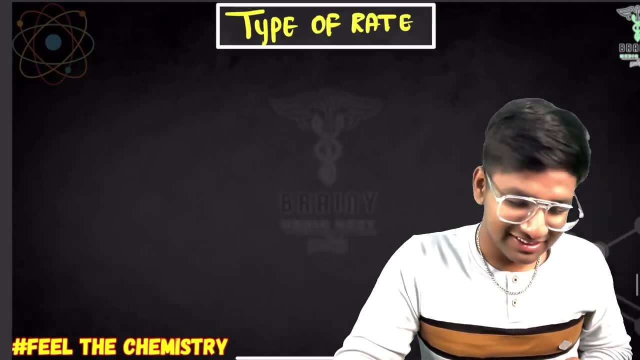 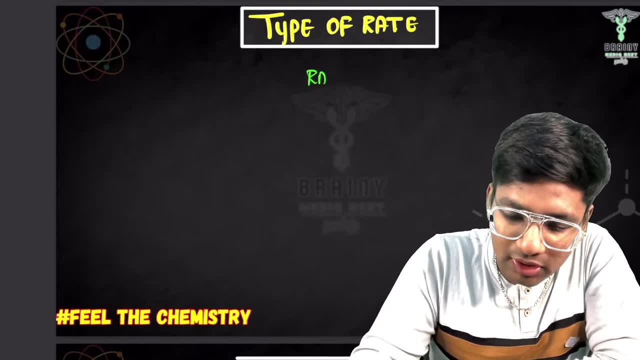 anu type ruku. sorry, rendu type ruku na moμα. namoa n s stacking so leta. ok, it see, rate is whole of 2 types. there are 2 types of rate. ok rate vaisted terre ru kî sannai mirano. 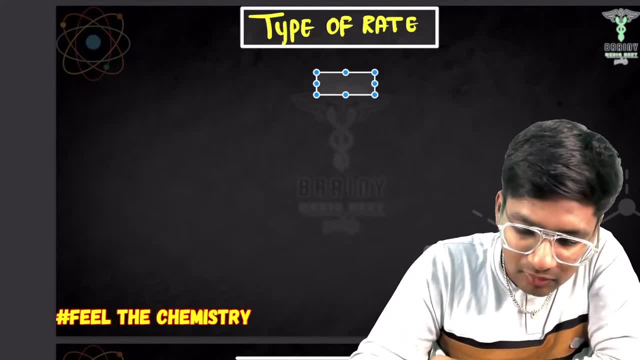 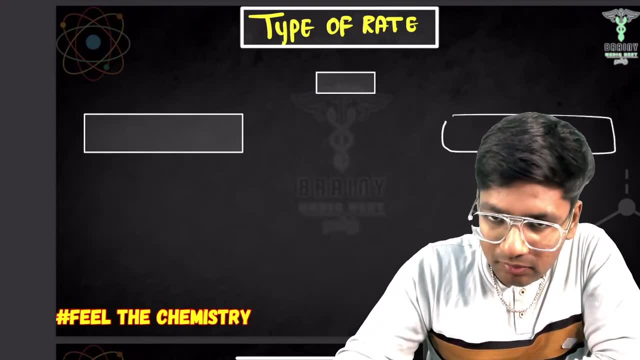 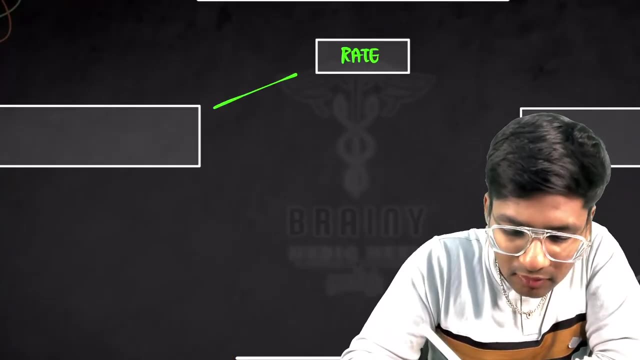 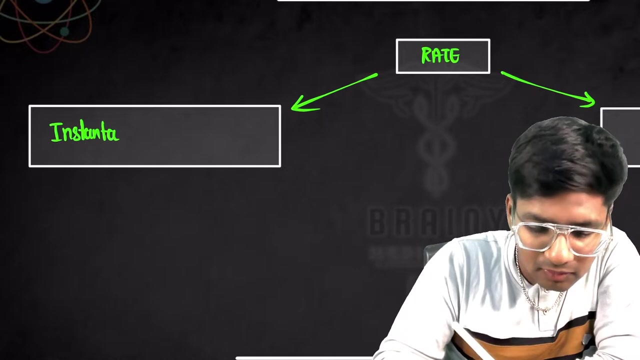 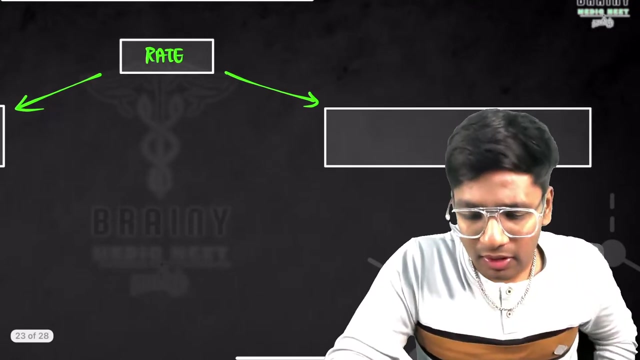 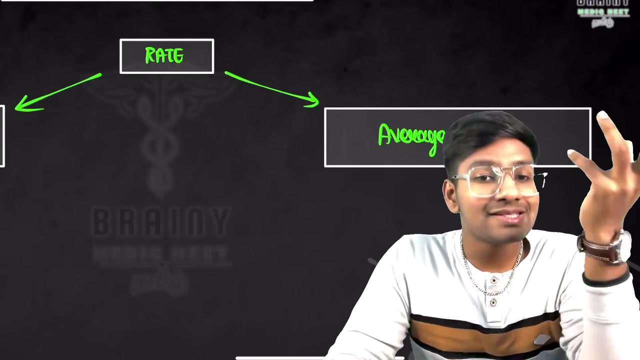 pe ai tu nedai anka kya pu s beschovum wha mai apap rate, yet u touch ok rate, yet u touch. rate is of two types: one is instantaneous rate, instantaneous rate, and the other is average rate, and the other is average average rate. 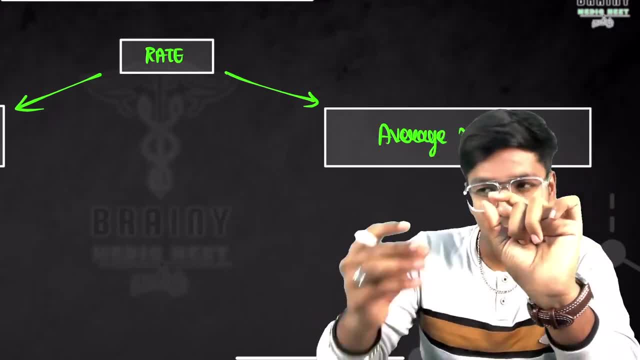 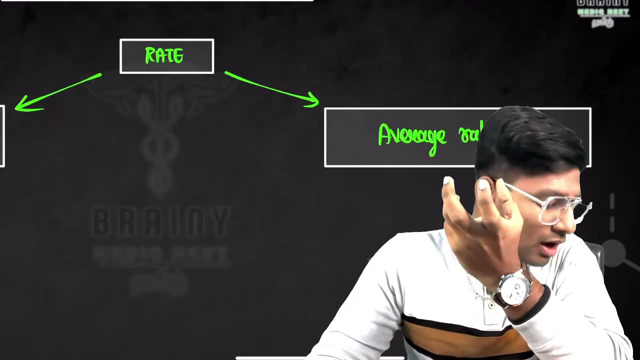 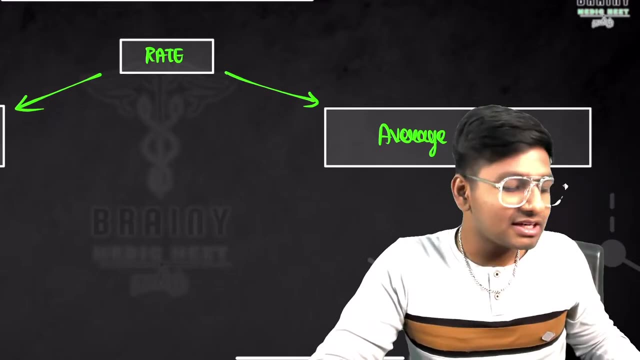 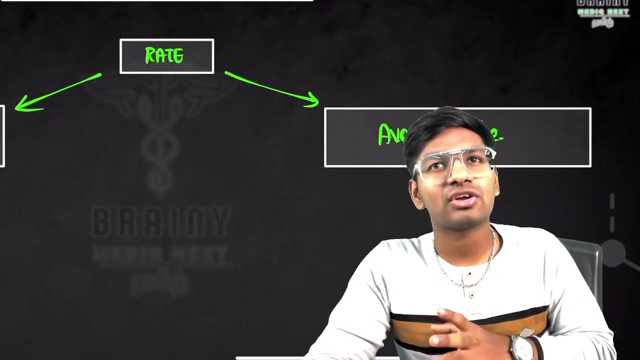 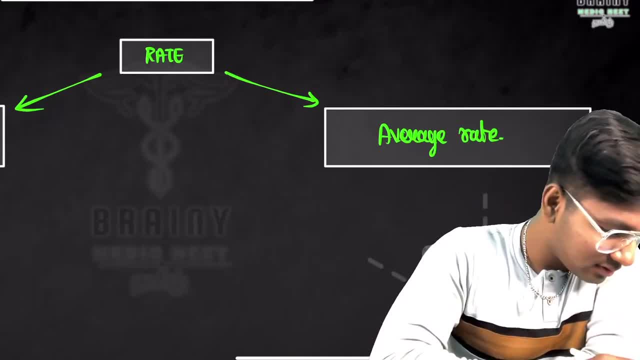 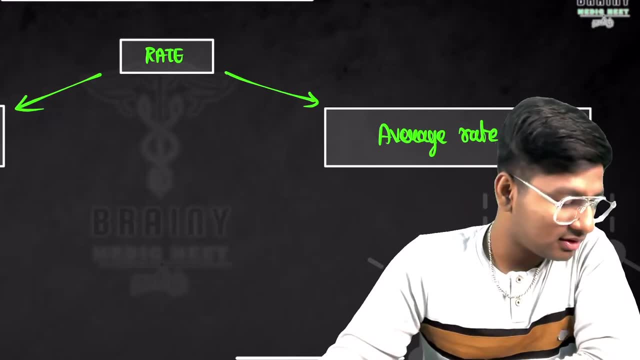 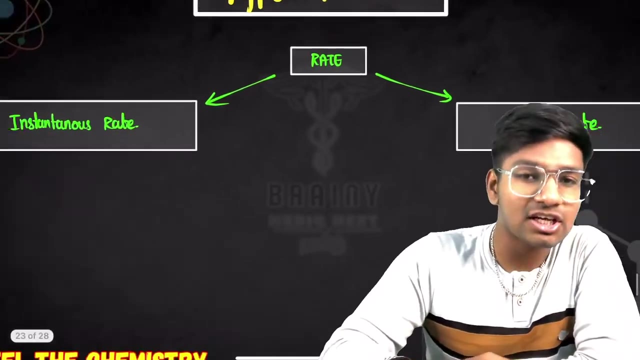 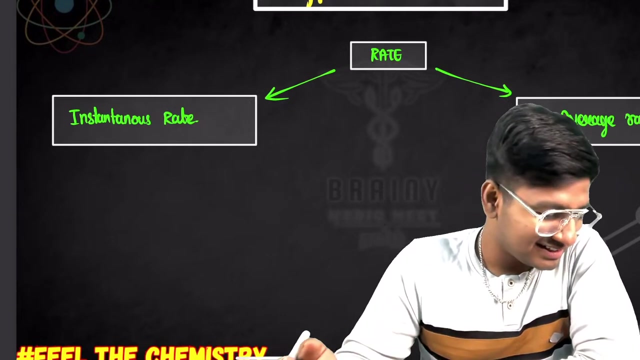 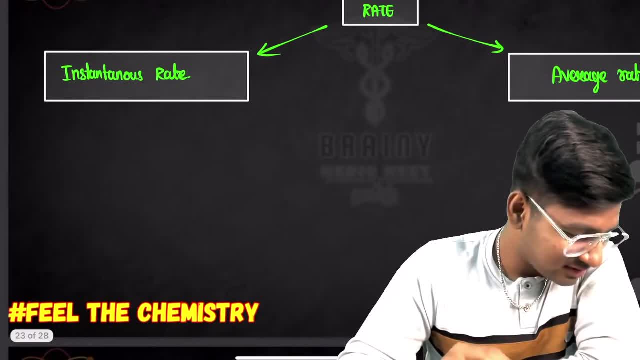 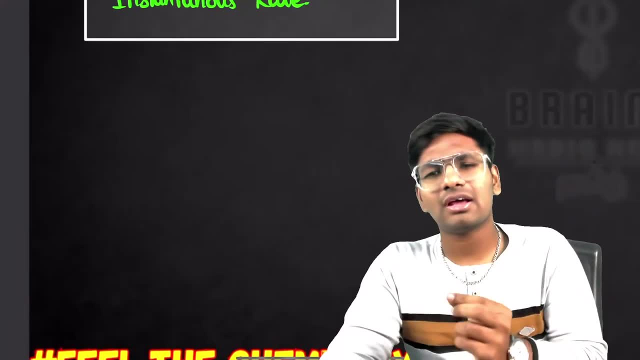 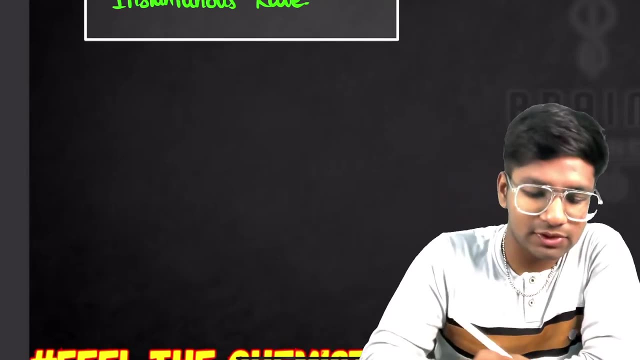 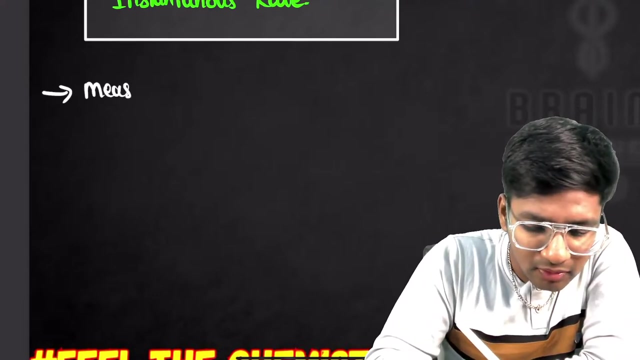 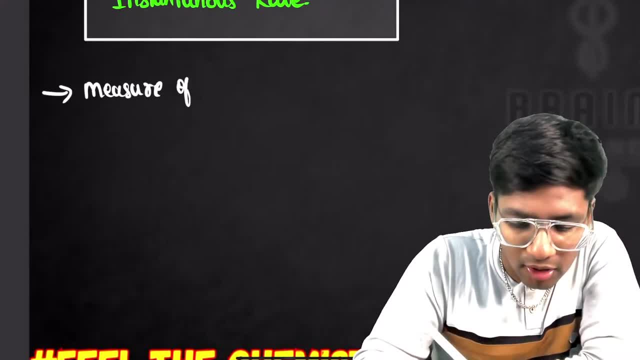 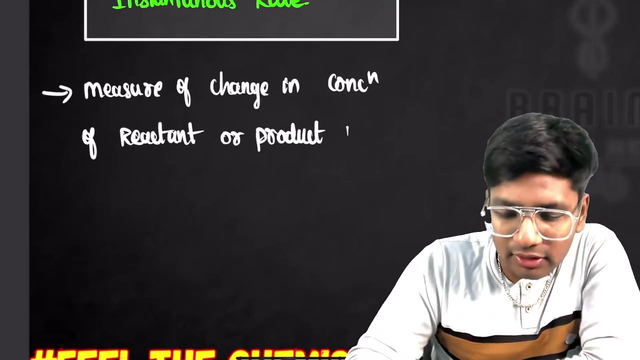 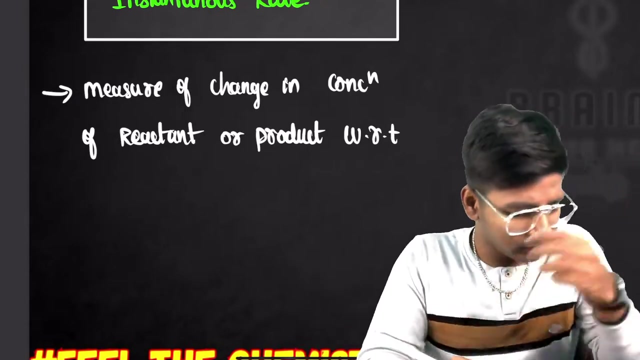 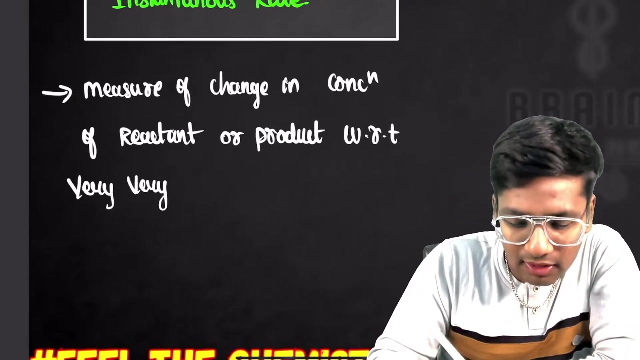 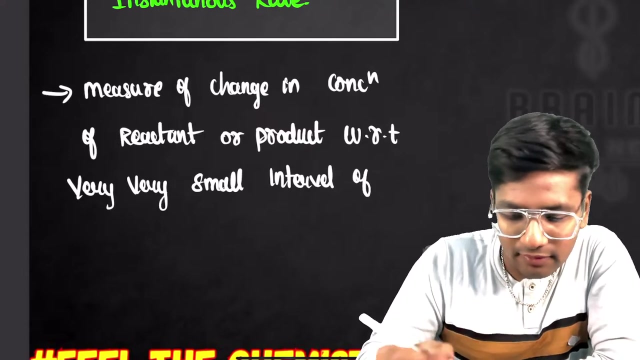 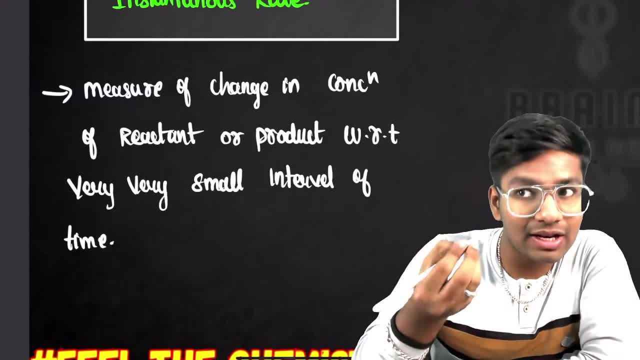 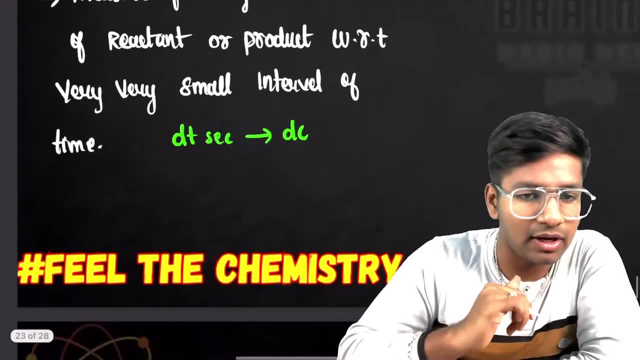 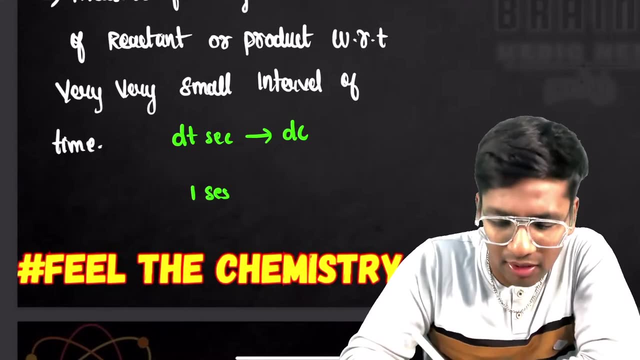 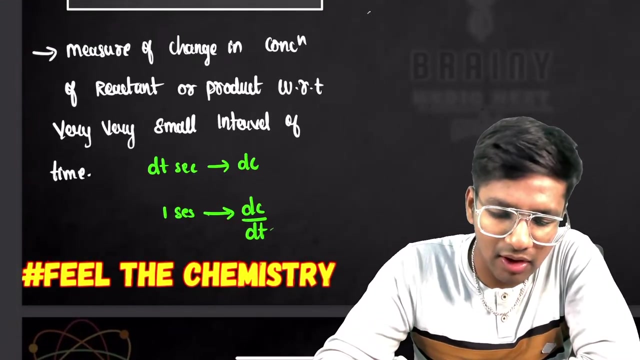 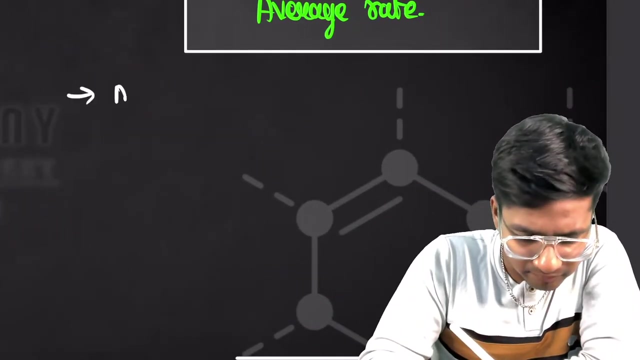 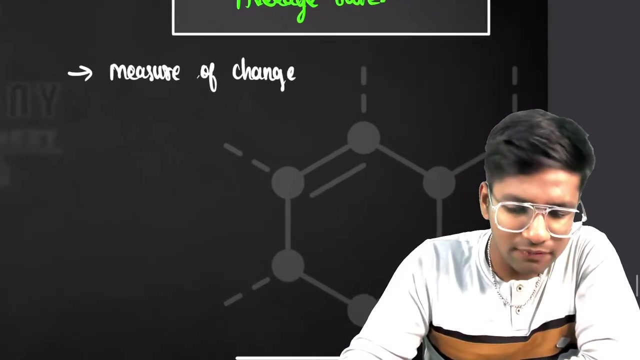 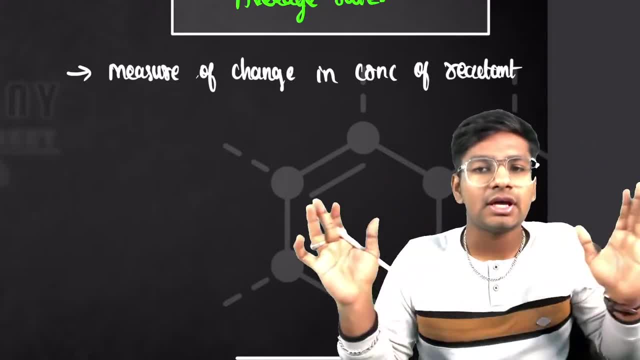 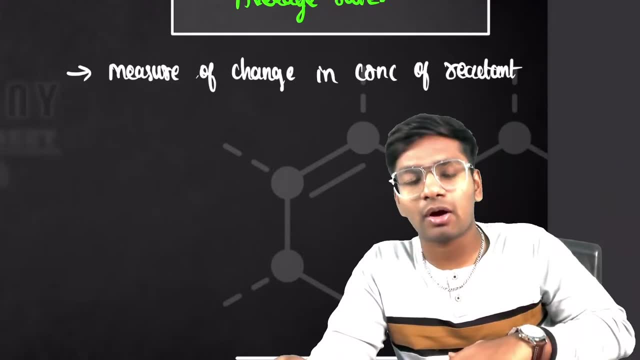 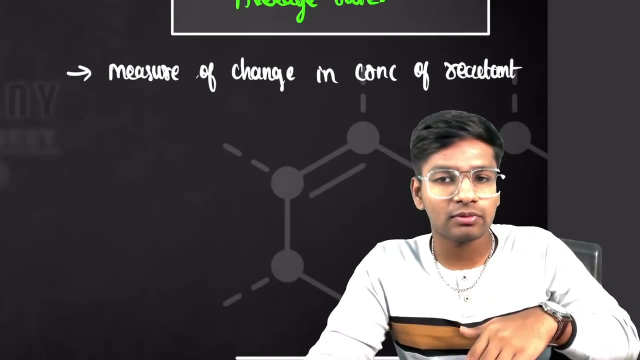 Reactant is a big, large gap interval, Large time interval. For example, when is your last break up and when is your next break up? There is a big gap like that. For example, if you propose for Valentine's day, you will have a break up in the next month. 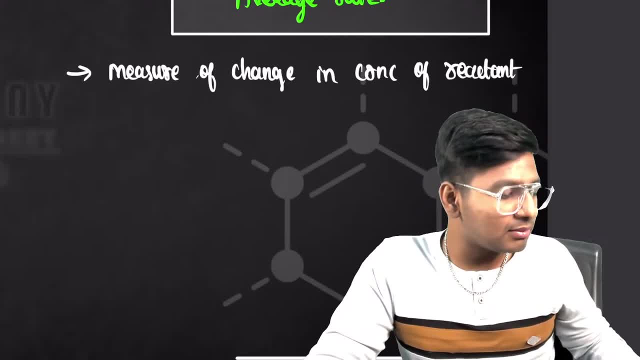 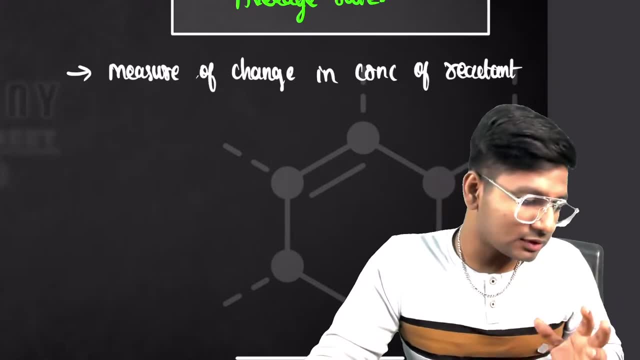 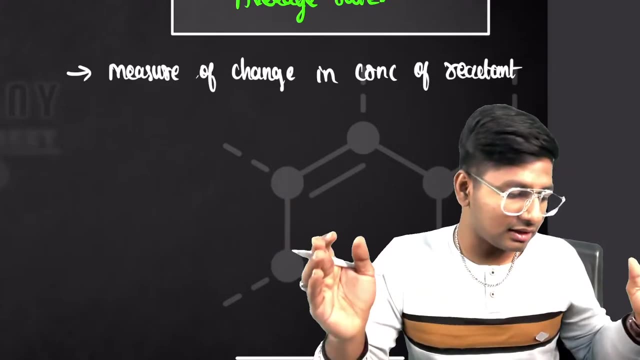 It is a large time interval. If you have a gap interval in a month, you will have a break up. It is like that, Do you understand? You will be stuck at home. You will be beaten up in your house. So the time gap interval is a big gap interval. 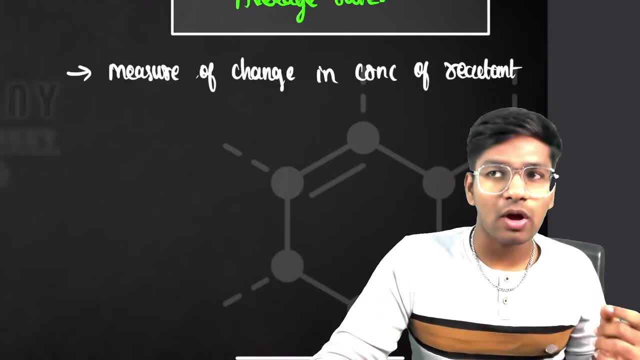 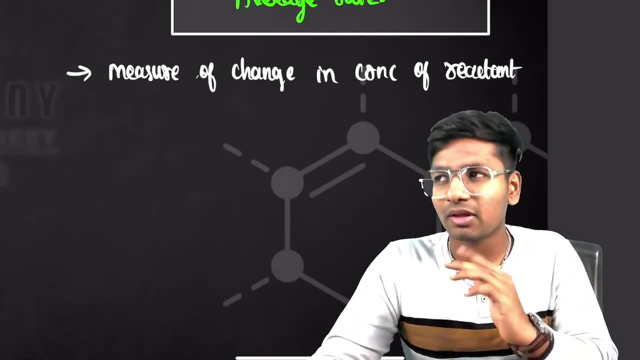 If this is instantaneous, like if you just sit and look at the girl at the first bench and see her, you would have seen her for 2 seconds. That is the instantaneous rate. Just you see her and that's it. That's it, That's it. 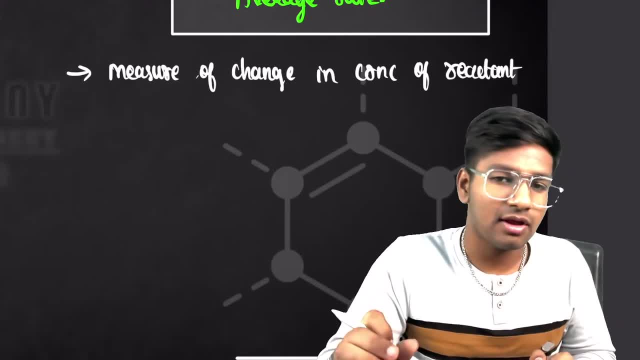 This is the instantaneous rate. That is a small gap interval. You would have gone to the supermarket. You would have gone to the building, You would have gone to the car. There would be a girl in the building. You would have talked to her. 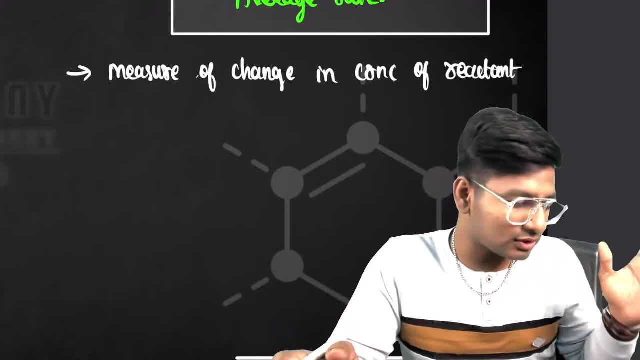 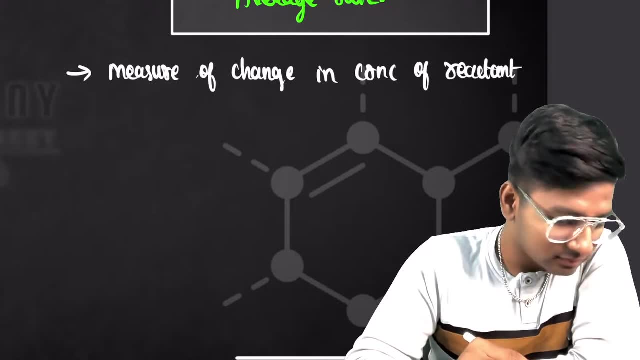 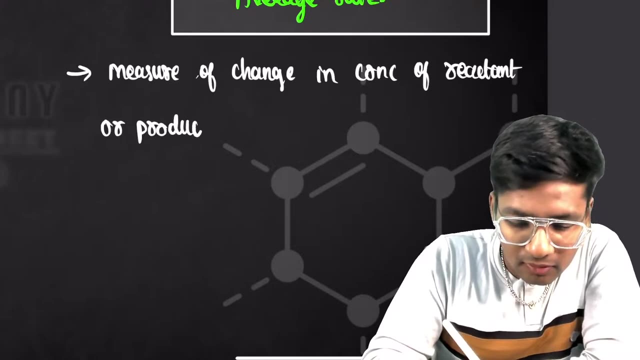 It is a small gap interval That is instantaneous. It would have ended then itself. If it had happened, then itself, you would have sang a song of love and growth, But that girl would have already grown up. Okay, See So. concentration of reactant or product. 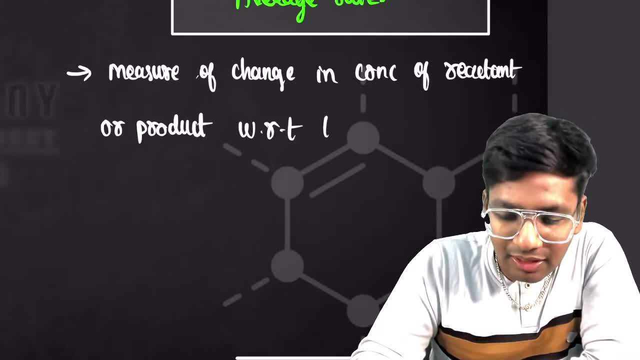 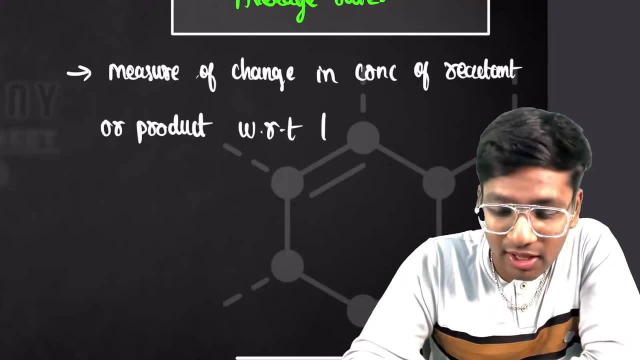 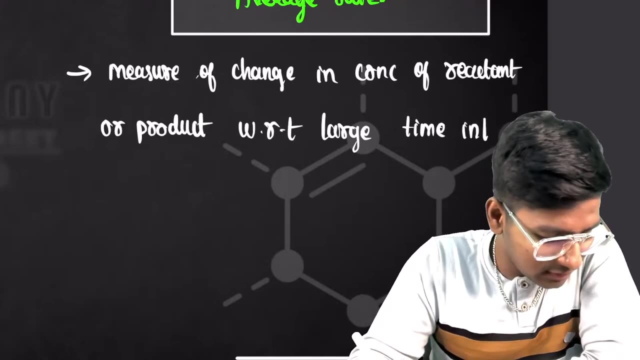 Or product, with respect to large, with respect to time- Okay, I have told you that- with respect to and time, Large time, interval, Time, How to think, bro, How to think it will go in a spot. What can I do? 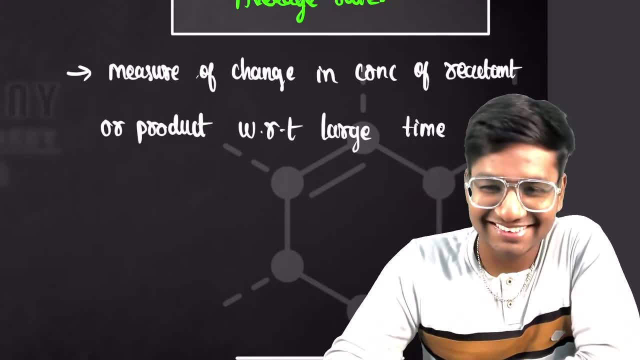 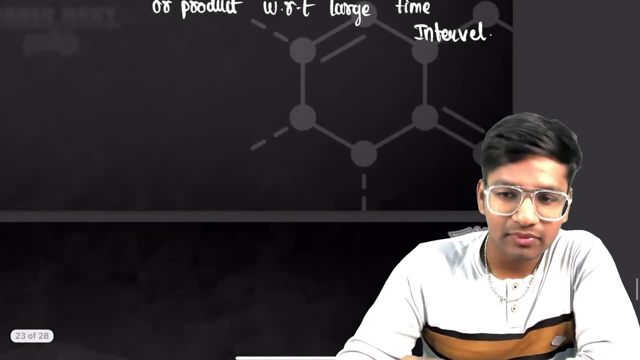 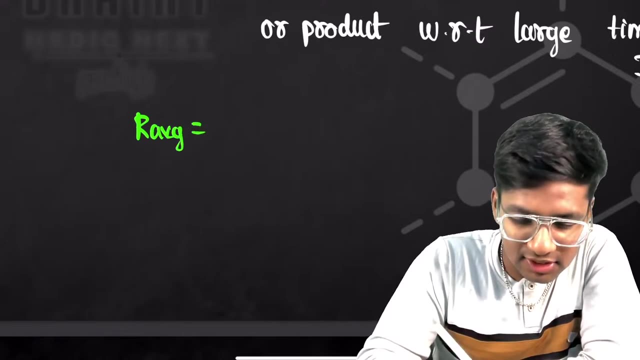 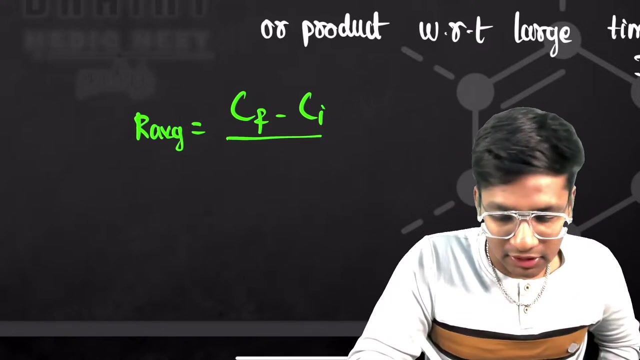 My mom raised me very smart What to do: Large time interval, Okay Time interval, Okay Time interval. so our average is: our average is equal to final minus C, initial concentration of final minus concentration of initial divided by T. final minus T ish. 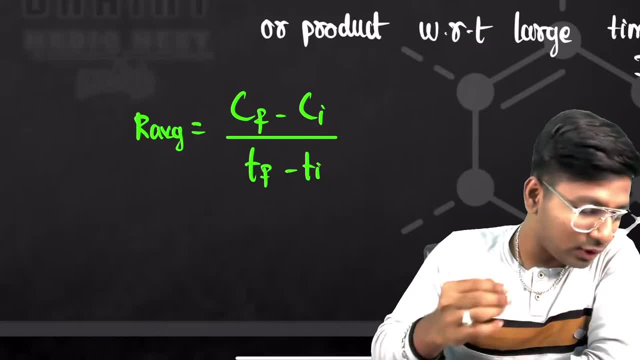 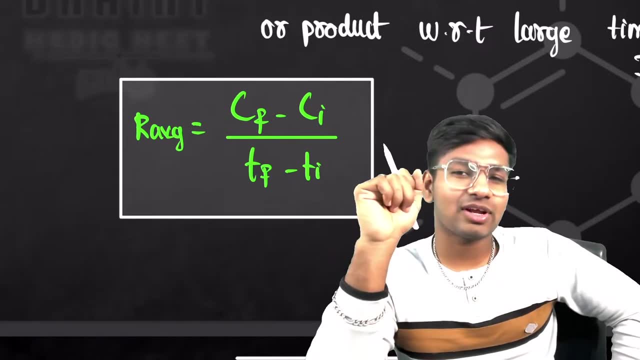 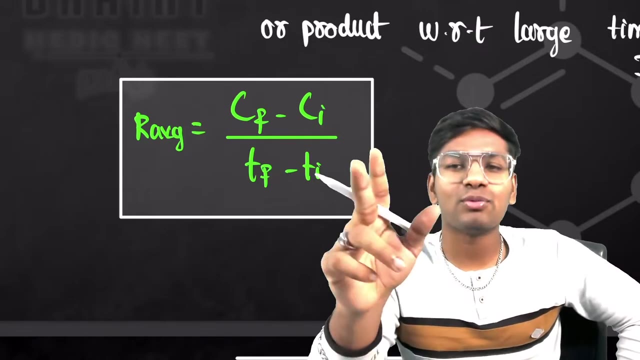 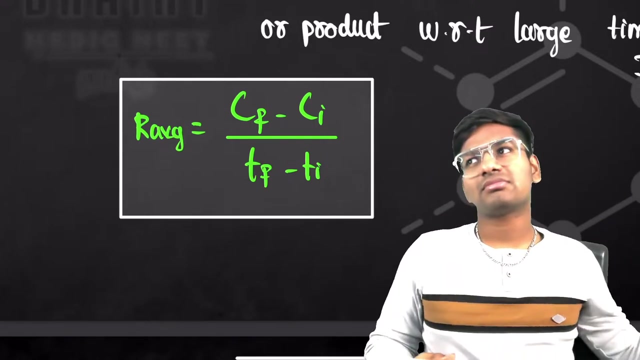 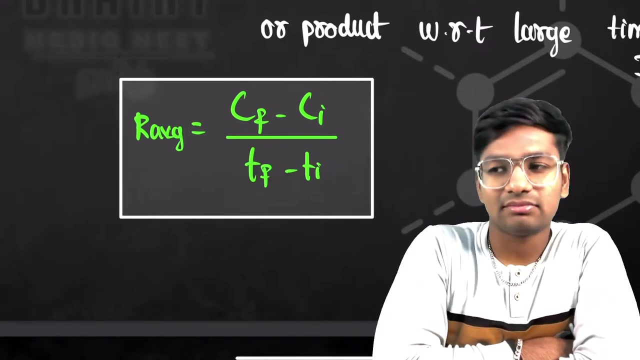 okay, T initial. in the daily schedule there are catered angle. I need to go see. now we plan what is happening. so, Lee, another, another knowledge. knowledge a Saturday, an attempt to give a lecture? okay, physiology, mundane, a good test to tell. but that's good portion, nana. 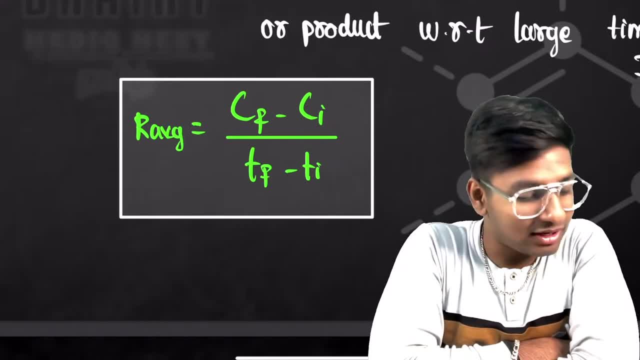 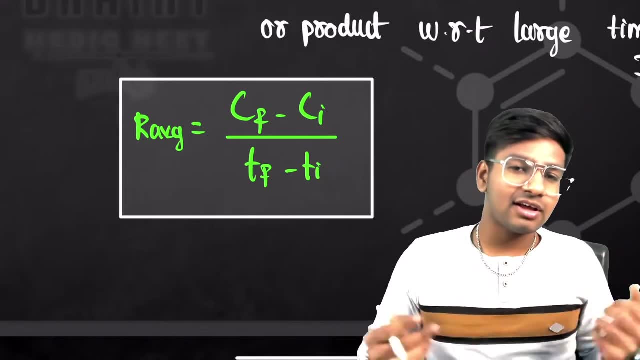 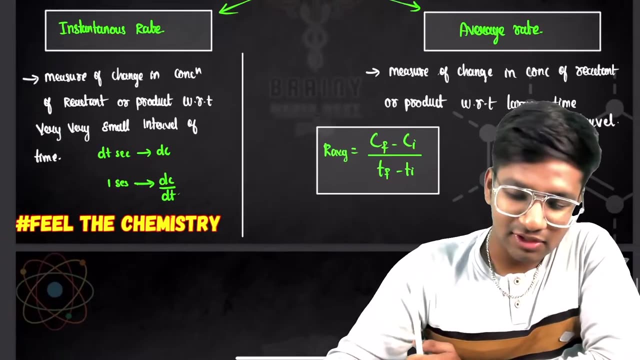 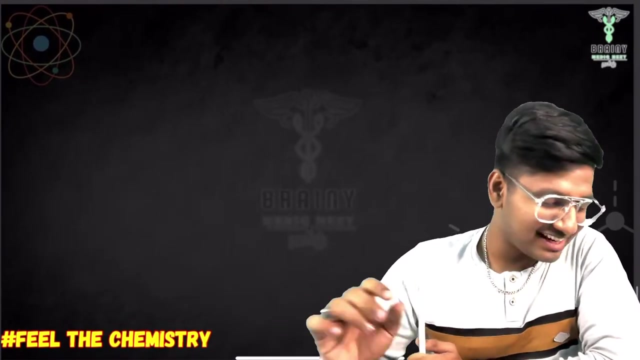 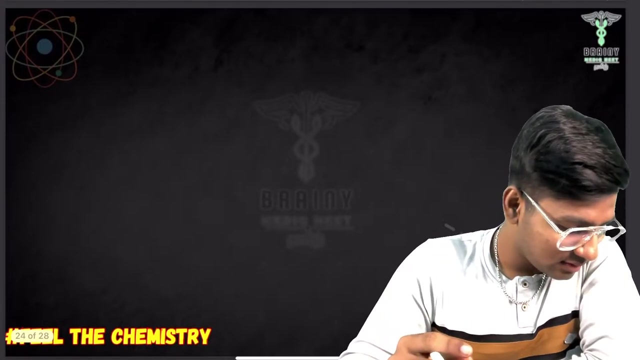 you wanna get it right, because reproductive univerine, reproductive univerine physiology- okay, reproductive physiology- people in the facility, that's what we're telling you examiner again. so no problem, and manage number three: other reproductive physiology- okay, sorry, okay, fine, nice work. MBBS exam is failed. 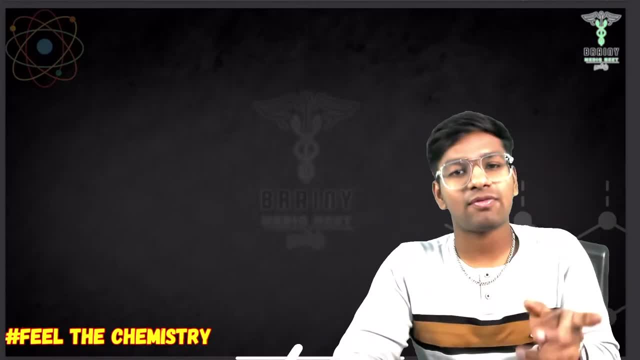 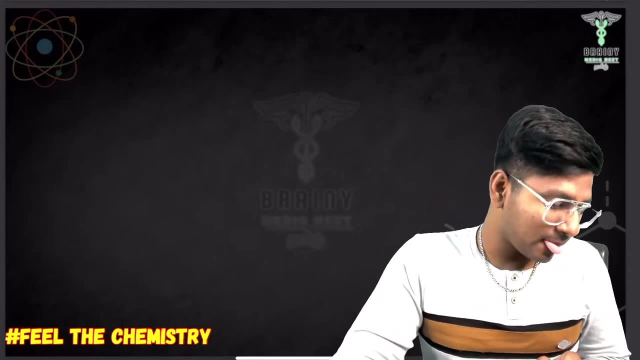 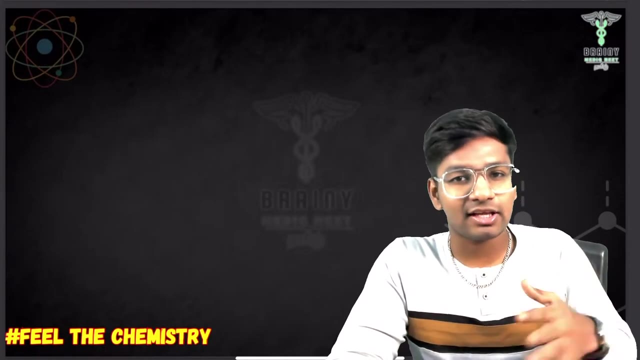 I will be surprised if I don't pass the MBBS exam. You can pass the MBBS exam if you study hard. You can pass the MBBS exam if you study daily. But I don't take classes and write. I have passed the MBBS exam recently. 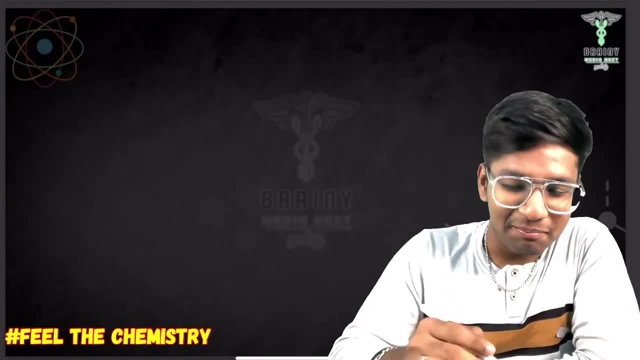 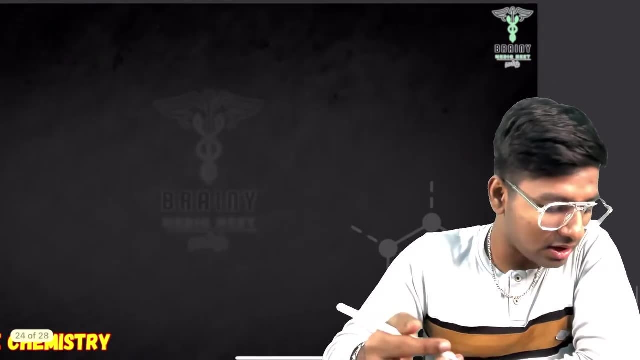 I don't know how I passed the MBBS exam. I have passed the MBBS exam, but I don't know how I passed the MBBS exam. If I take the classes well, I can write. If I take the classes well, I can write. I write only if I take the classes well. 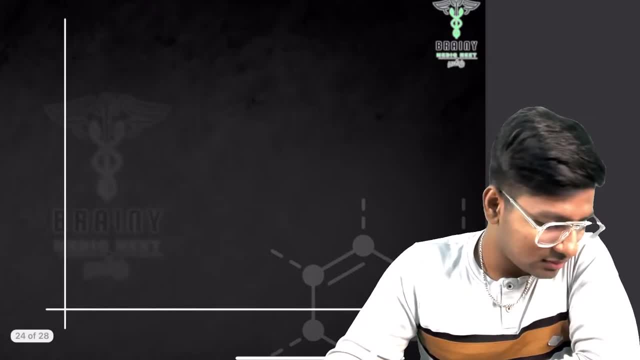 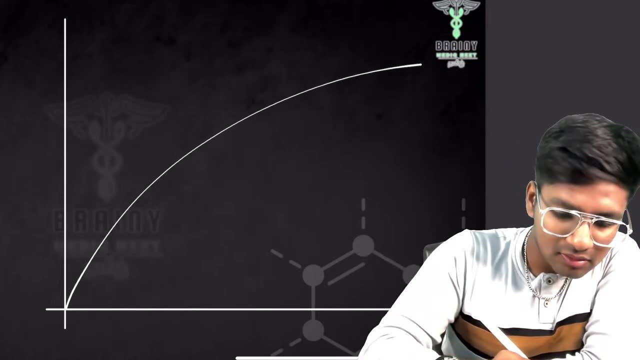 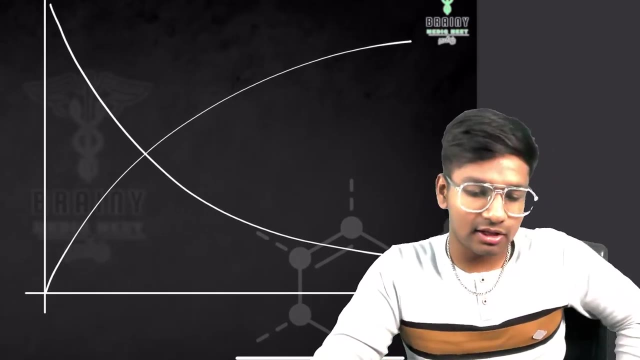 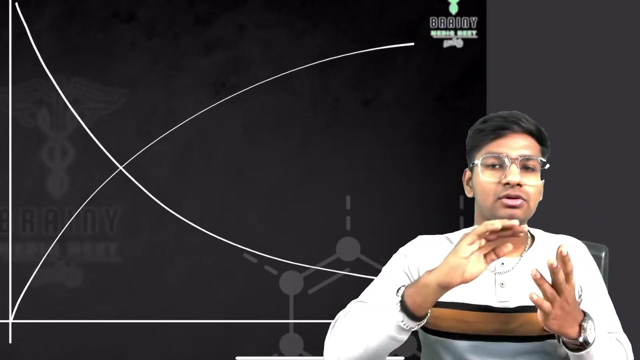 Mostly, I write only if I take the classes well, I write only if I study well. Now, if you study well, you can take the gold medal. In anatomy. we have superior relation, inferior relation, posterior relation, anterior relation, medial relation, lateral relation and so on. 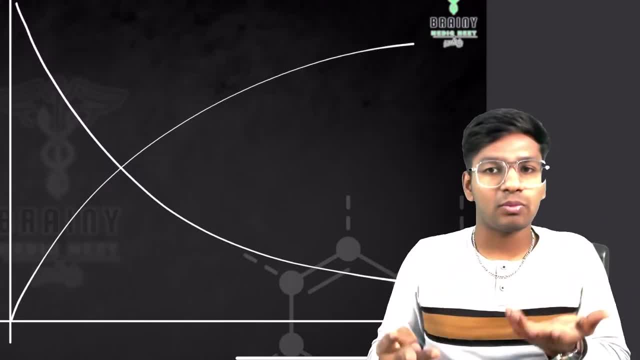 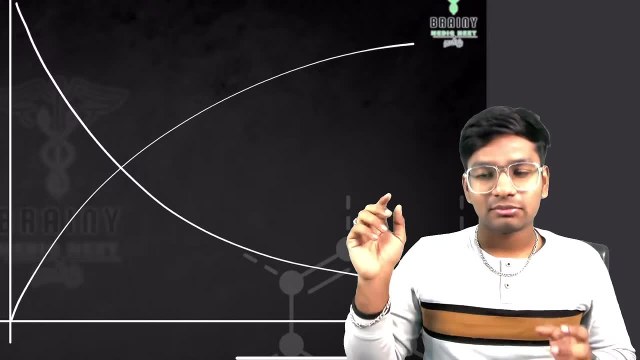 If you book it and read it like a madman, you won't understand. What I do is I ask the mam to come and show it to me and I take the mam alone. I take the mam to explain and I do the same for many questions. 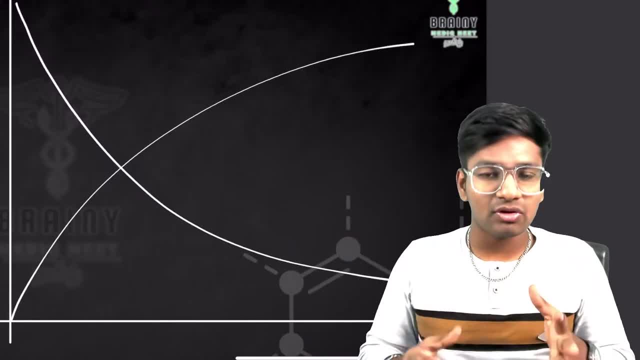 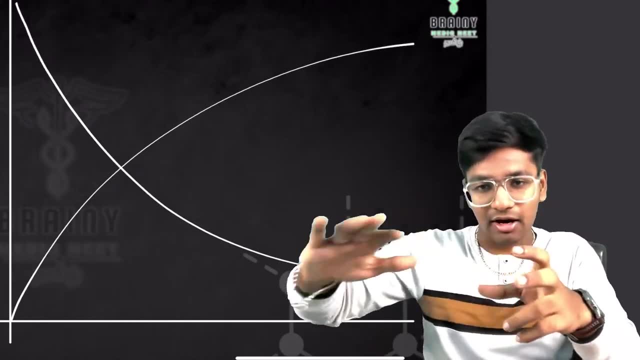 Everyone will read it the same way. what I do is when I am in a bad mood, I won't be able to understand. I will take the book and see the relation and see what is above the specific organ. what artery is going, what organ is there? 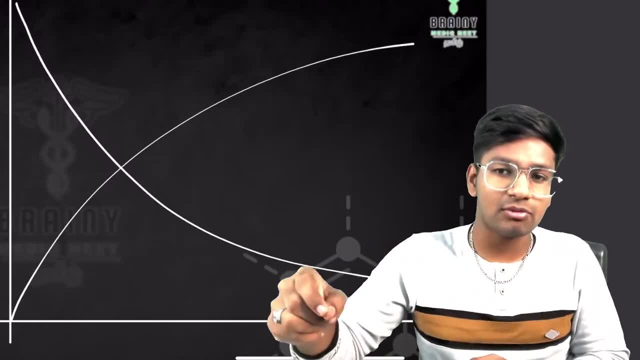 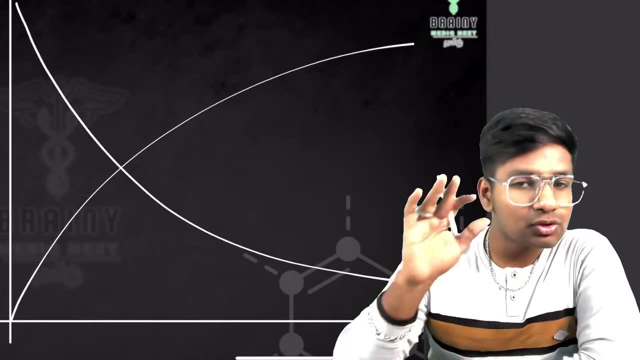 I will see what is below. so when I imagine, I can imagine and write. If you do like that, you will be able to remember things. well, If you do the book alone, you won't be able to remember. You have to look at it. 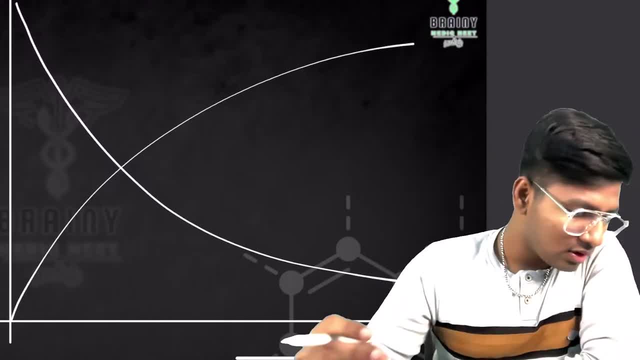 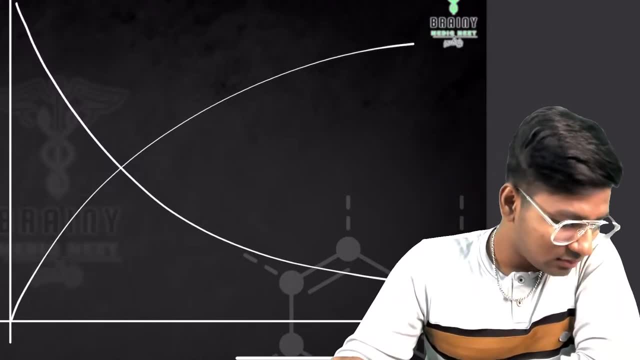 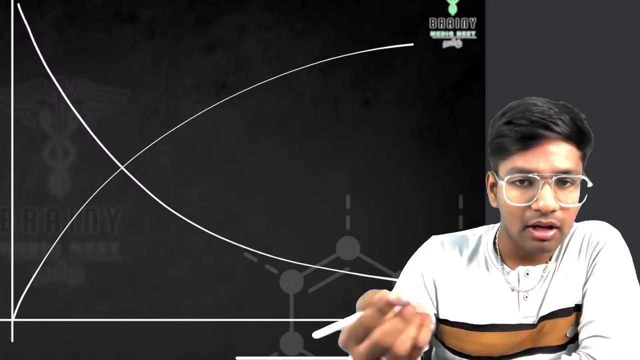 If you look at the anatomy, you can read it. If not, you can't do anything. I will go and see. If I understand, I will go and see it. If not, I will imagine and read it. Ok, fine, let it be, I will put a graph here. wait. 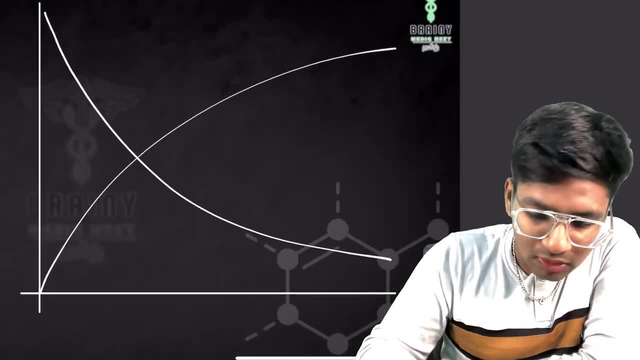 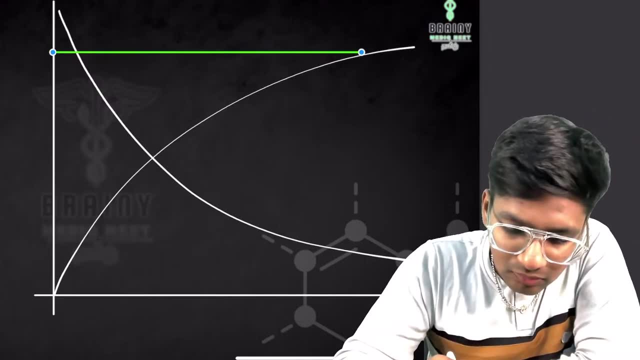 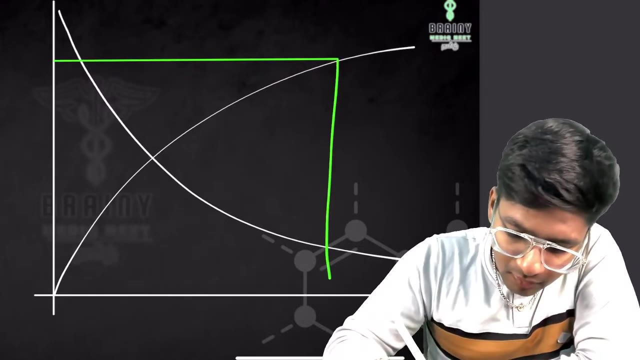 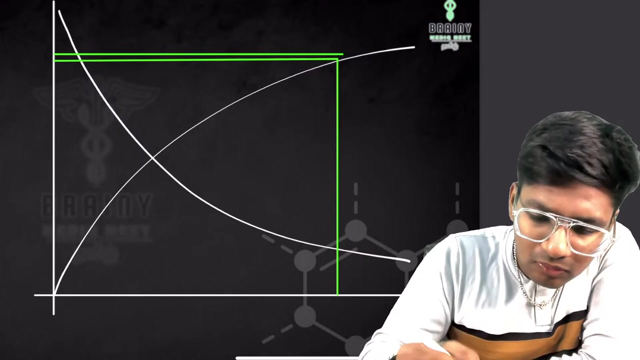 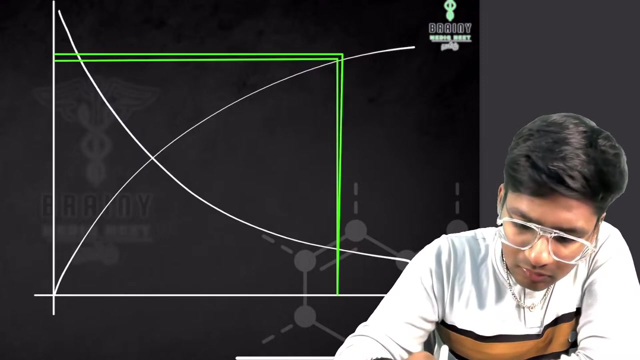 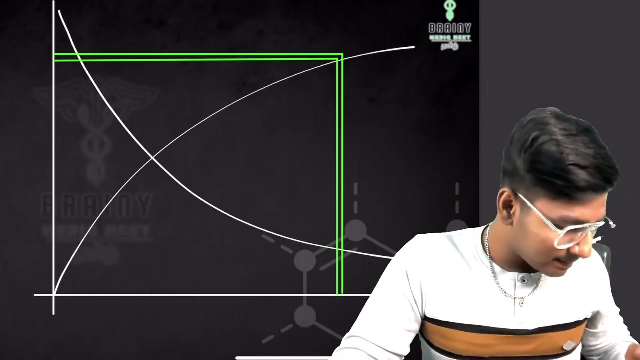 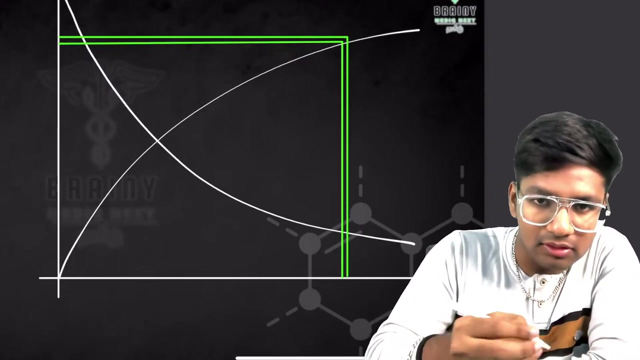 If I put this code, it will take some time. It will be pretty fast. I will go and read it. Ok, it is ready. I can study. only that way. I am first year student. see next 2 things I will tell you. I will draw this graph. 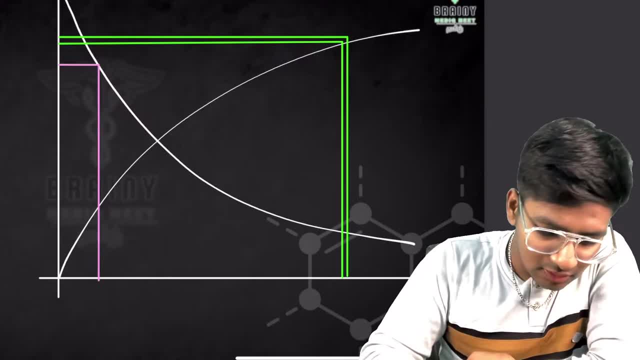 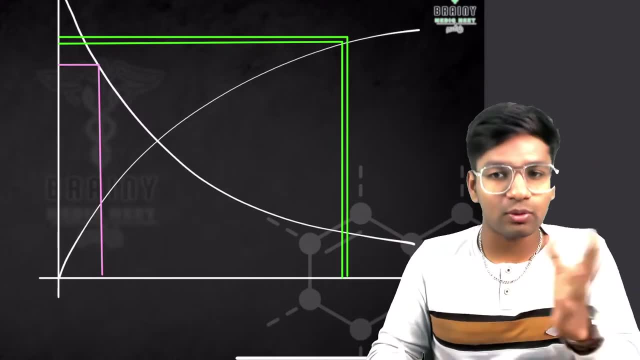 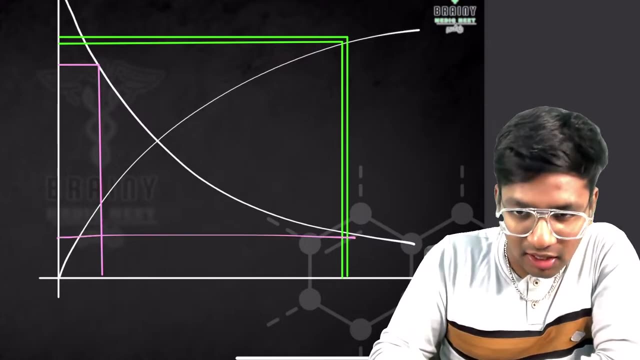 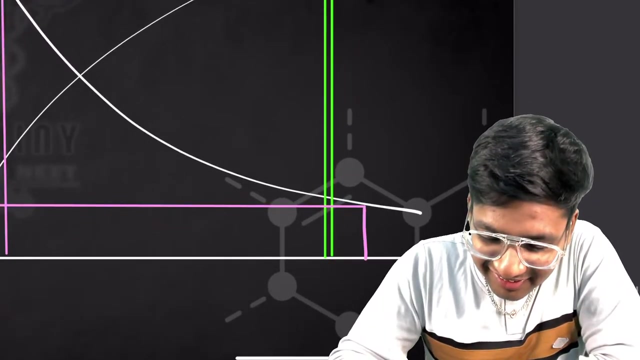 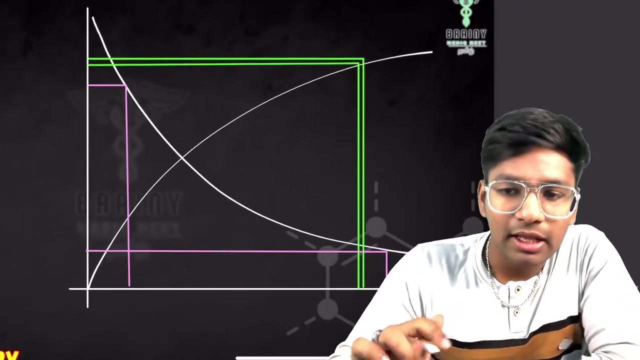 I will tell you in anatomy period. I will tell you in anatomy period. I will tell you in anatomy period. Recently I don't talk much with anyone. I am studying. I won't talk to many people in my class. This is time in seconds. This is time in seconds. 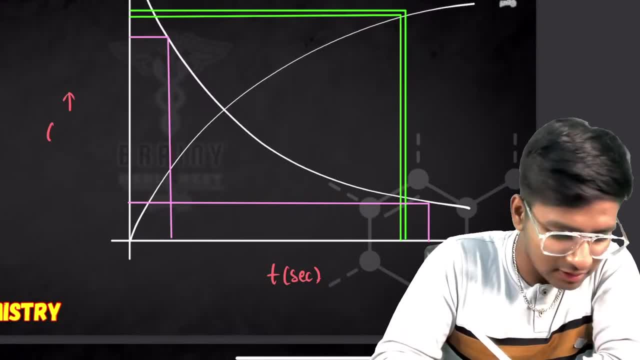 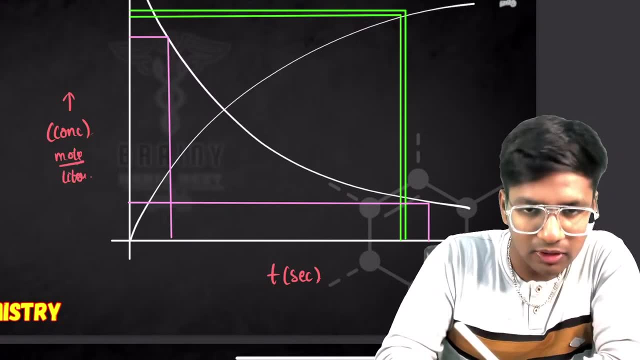 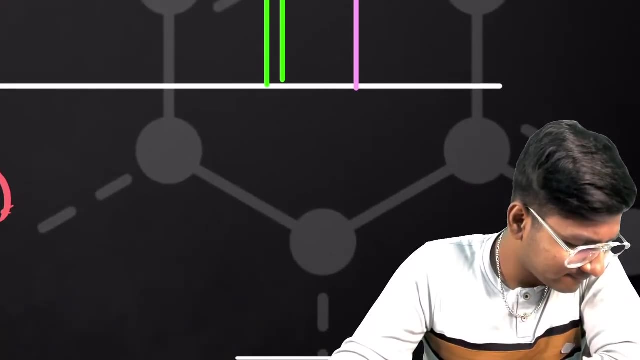 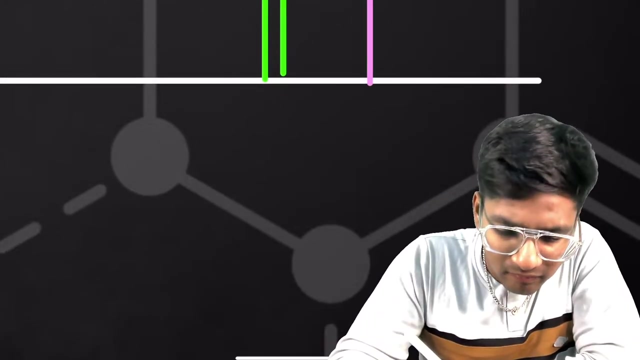 This is concentration. Concentration is mol per liter. Concentration is mol per liter. So what I am going to tell you is: So what I am going to tell you is: Why private college? I choose this because I am in chennai. I choose this because I am in chennai. 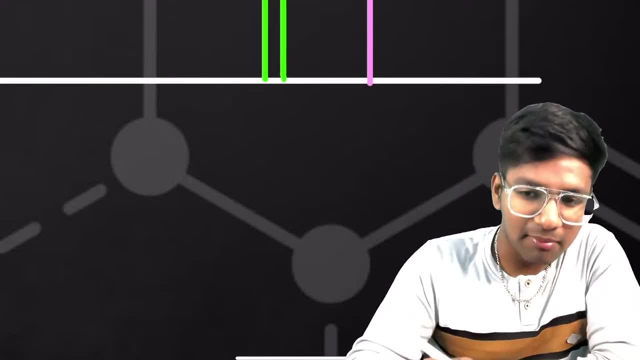 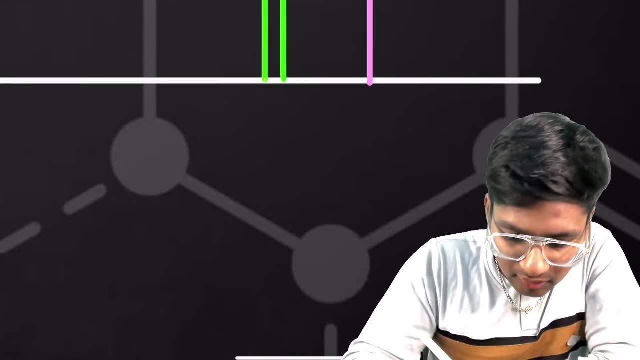 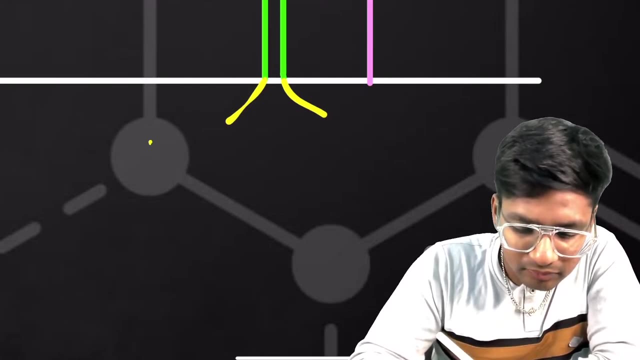 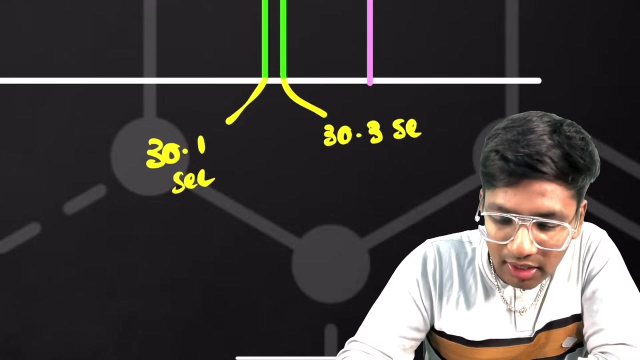 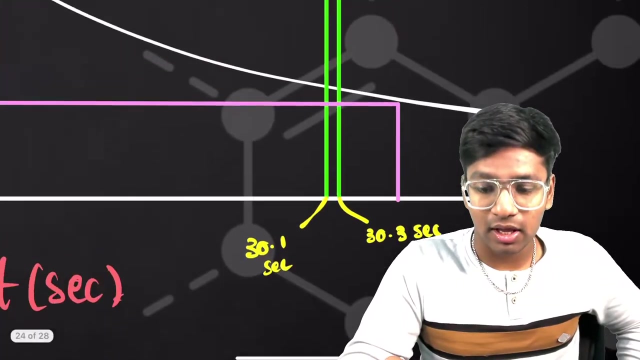 I have left this for so many years. If I had studied, I would have written this, But I didn't. I have wasted it See. See 30.1 seconds, 30.1 seconds. I told you that it will be in minute seconds. okay, my new tennis. I can still run. so now I don't know. so I think, Audrey in. 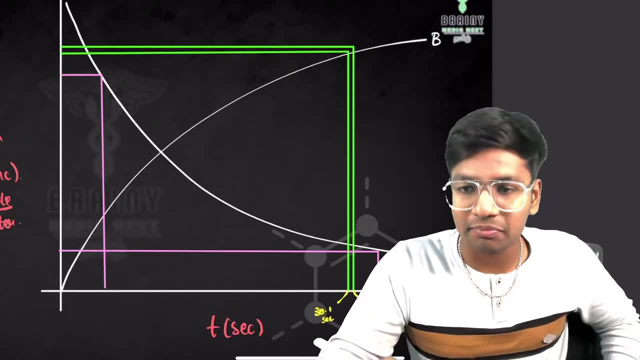 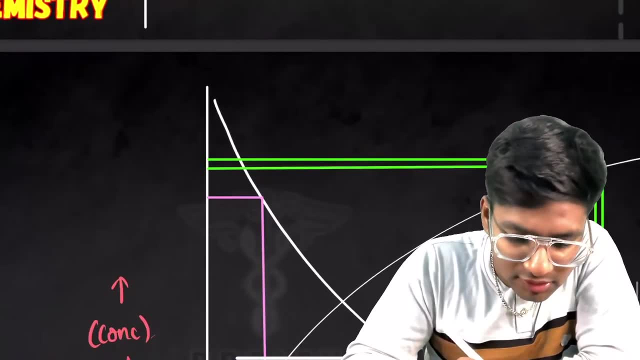 there at the lab. this is your concentration with respect to time of B, either one or a. okay, my a degrees and the BNF even the product. okay, you know, I know in the diagram a movie killer, I'm Richard. I mean pendant a 200.2 and 200. 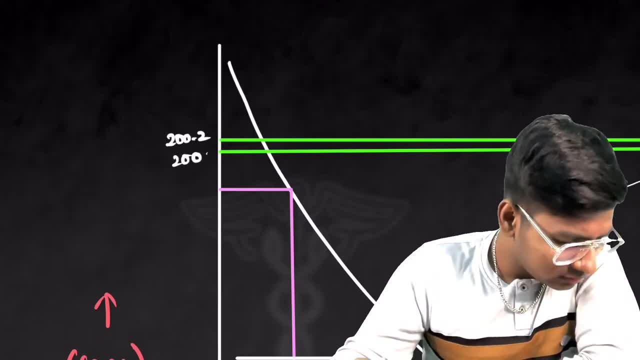 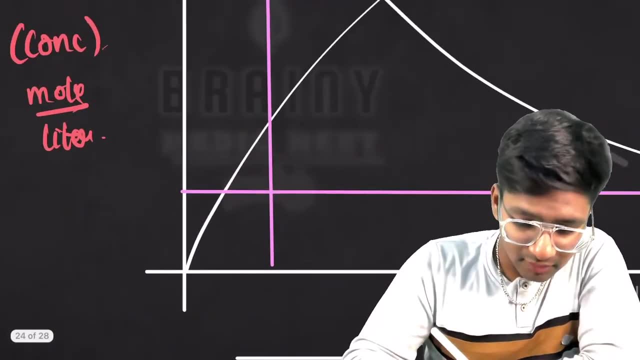 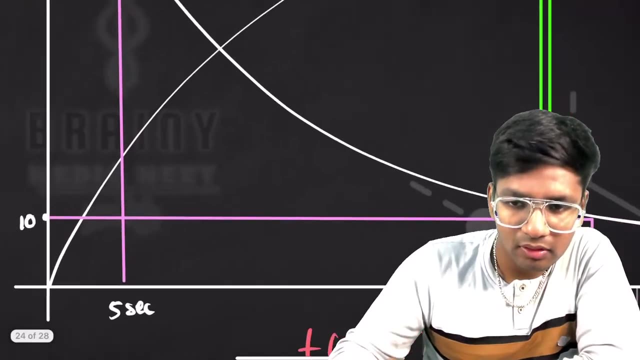 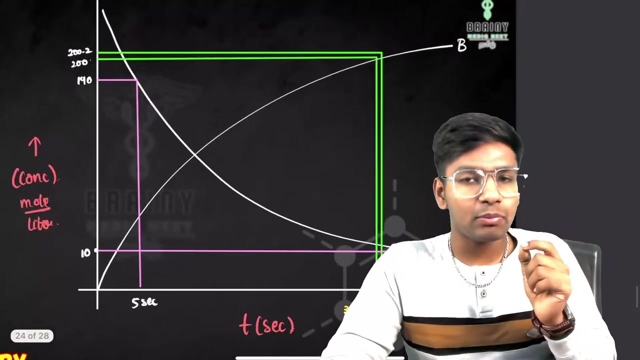 point to either on the 200, either 200, and in there on the 190, it'll know that 10, either, no, that 5 second, you don't know that 45 second. say the booty, booty are in the limiter color. advocate: instantaneous measure: panavia in. the pacifist are in the pink line. 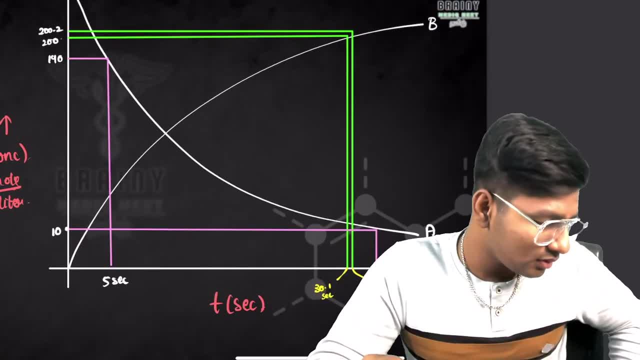 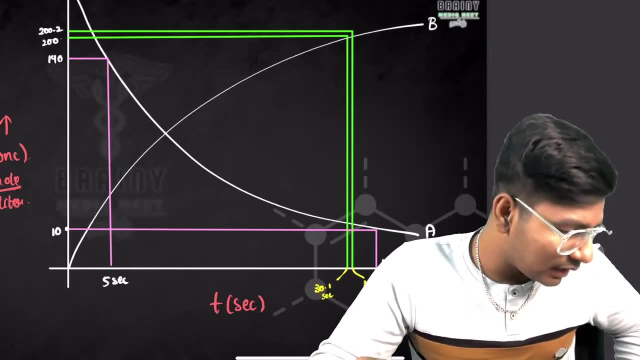 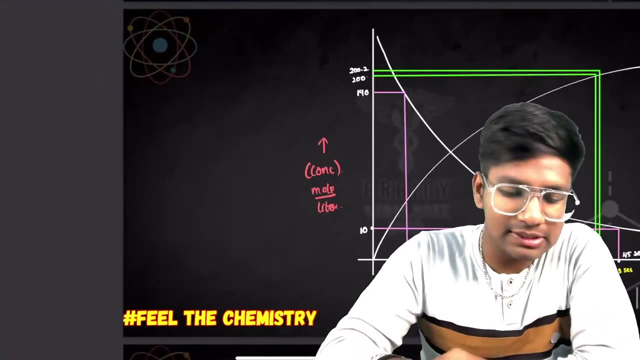 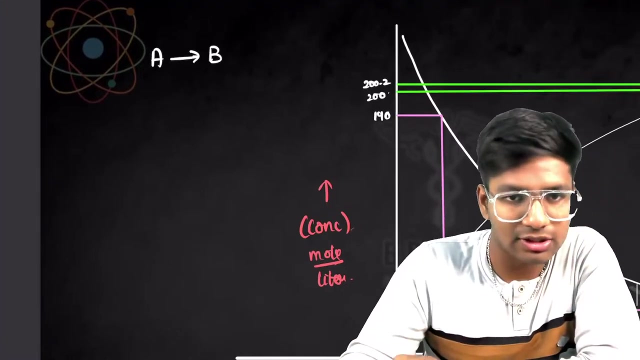 border can, amazed, Prepare to shoot channel in there. that's in a little bit in the instantaneous pressure panavia. so either it is a reaction, it is a reaction a gives B. okay, this reaction A gives B, now the grap בे genocide. so the bacteria, it's affected by integrity and 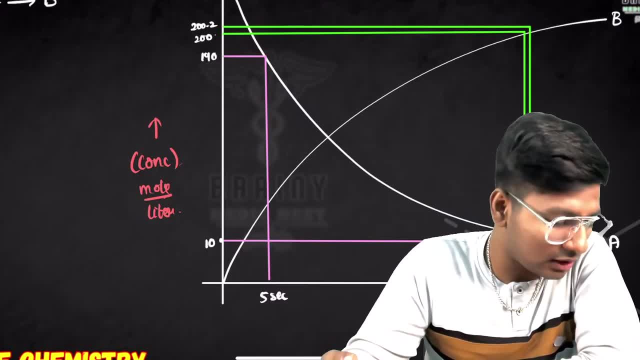 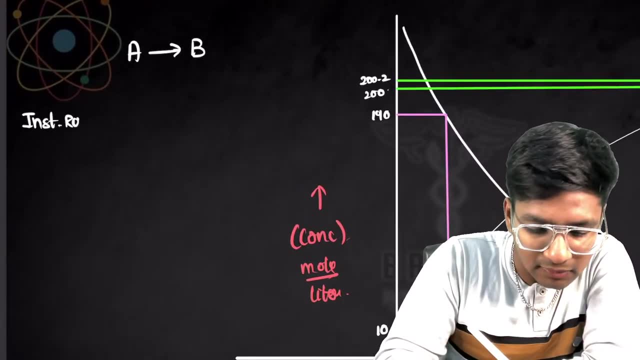 B 의� cosine cousine, 프로 viral concentration with respect to time, increase our room can at the Latvia. okay, I'm gonna turn a lot of video, so I know I'm gonna bring the instantaneous rate and I'm gonna get more instantaneous rate, instantaneous rate and I'm gonna 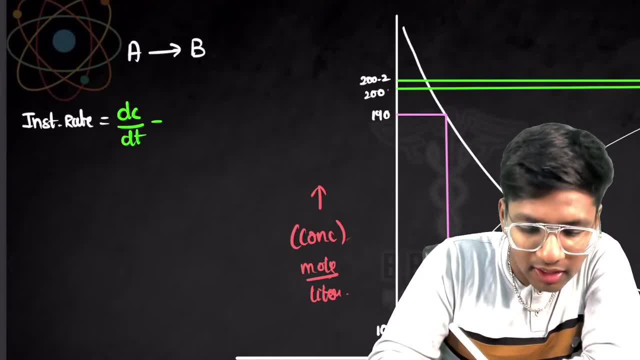 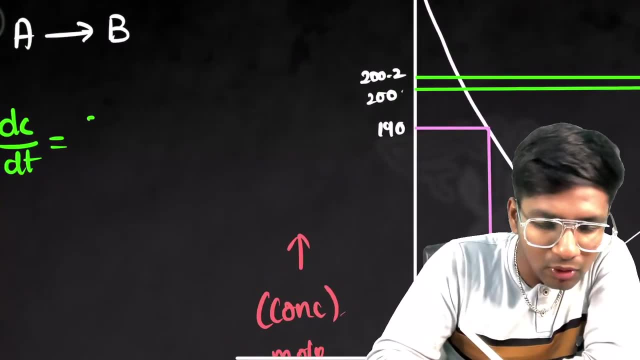 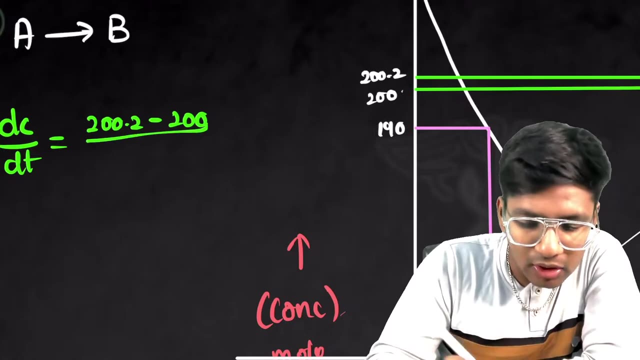 jump in. ah, DC by DT port, okay, DC by DT, no, no, no, no see, pardon, rumba way, my Utah car 200, 200 point to find a little 200 point to minus of 200. okay, big little, a small in small in so big line of summary the thing about in: 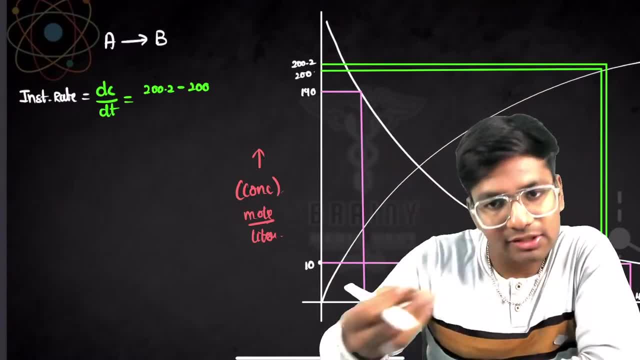 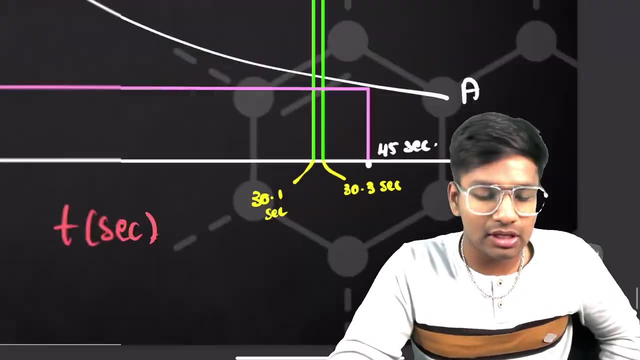 the render curve line: party now. party now. look at reactions of proceed boundary. if the procedure of the car to the corrector and the seconds per seconds: 30.1 and 30.3 seconds, 30.1 and 30.3 seconds. finally, no final level: 30. 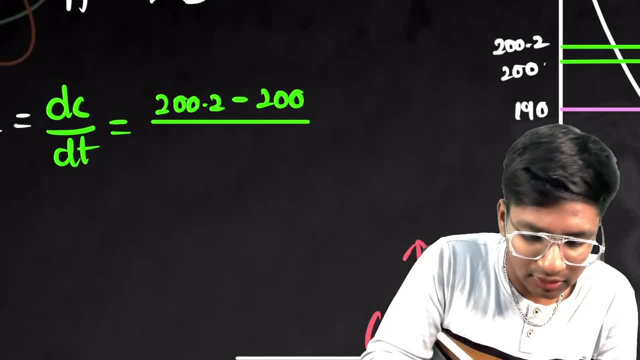 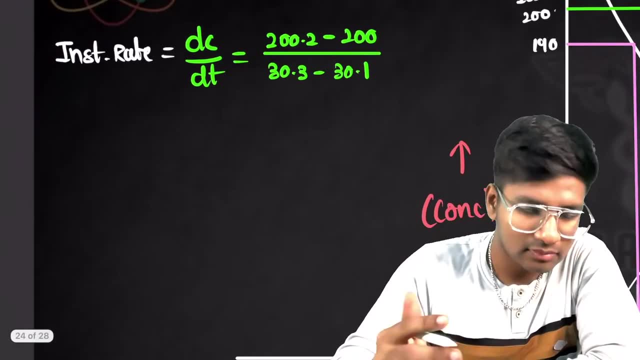 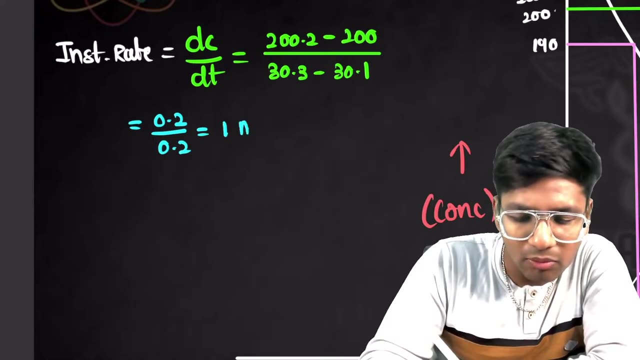 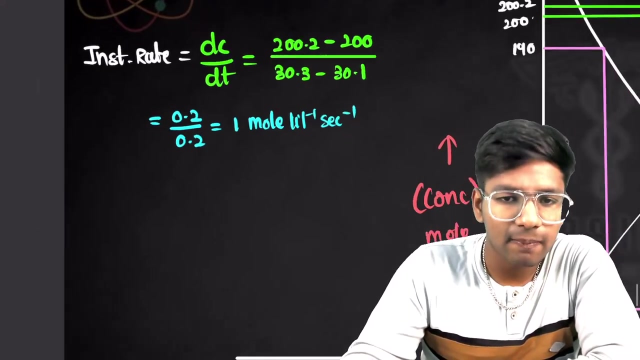 point three, final is 30 point three minus 30 point one. what is the answer? tell me the answer. and the solar. so it is 0.2 divided by 0.2, which is 1 mole, 1 mole liter. inverse, second inverse: correcta, correcta, Siri. 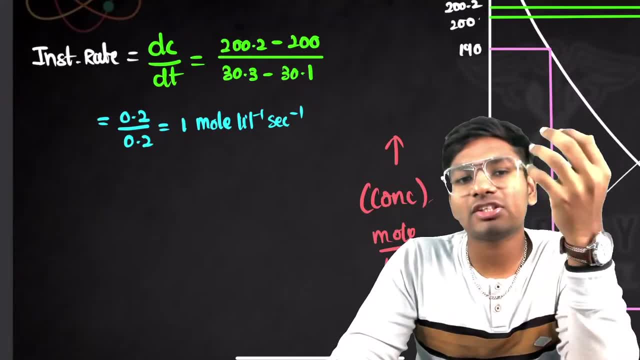 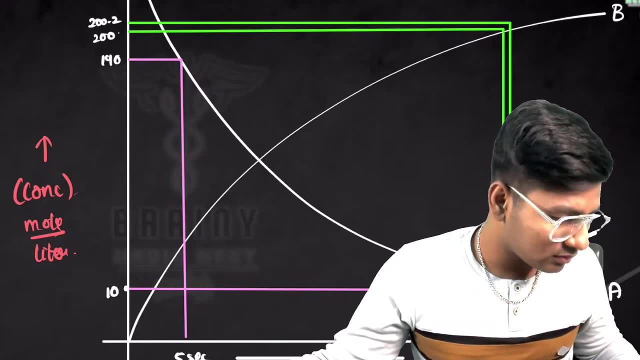 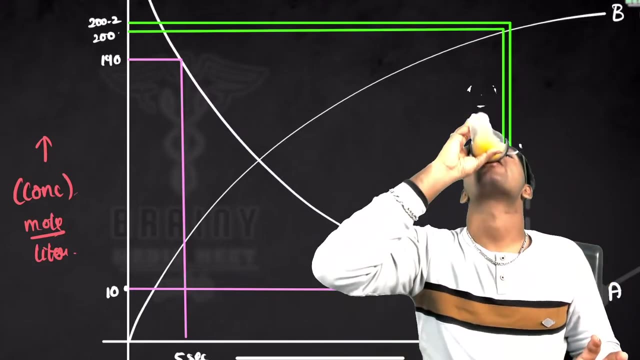 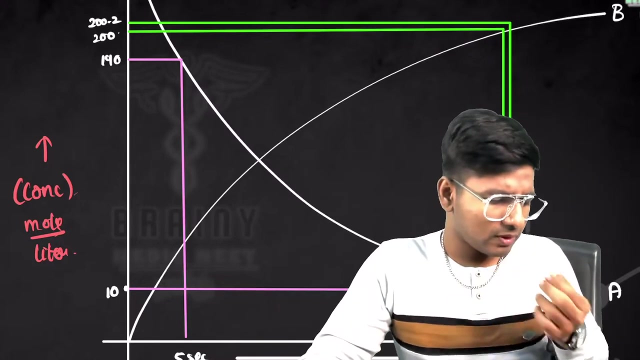 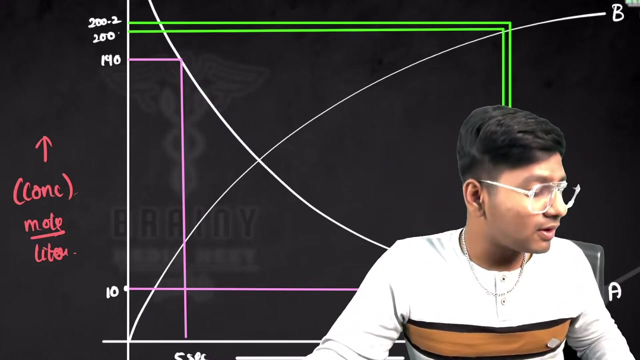 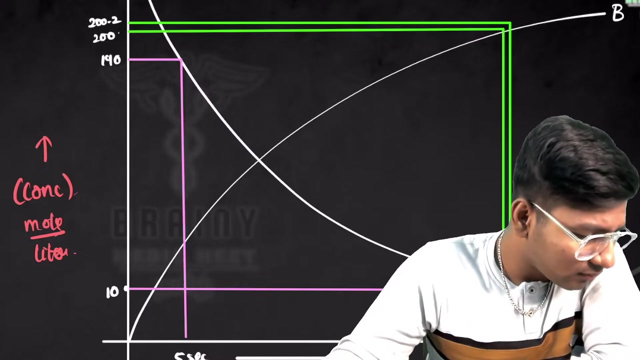 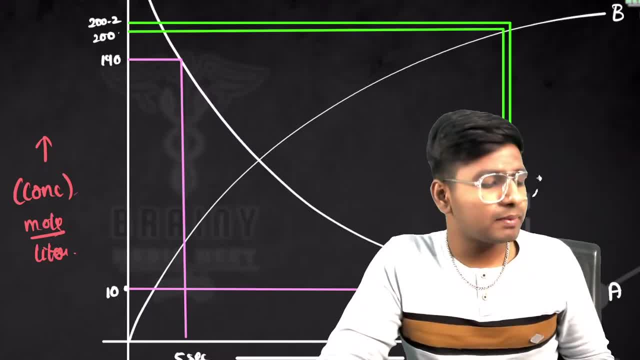 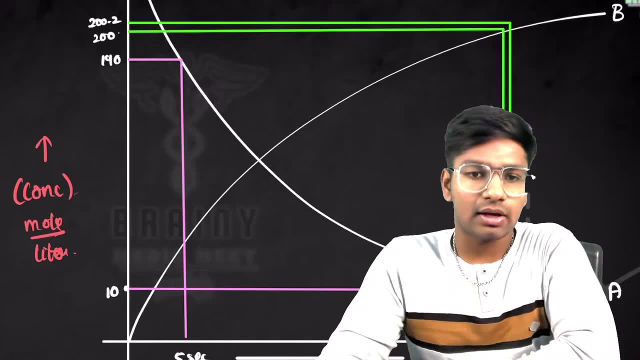 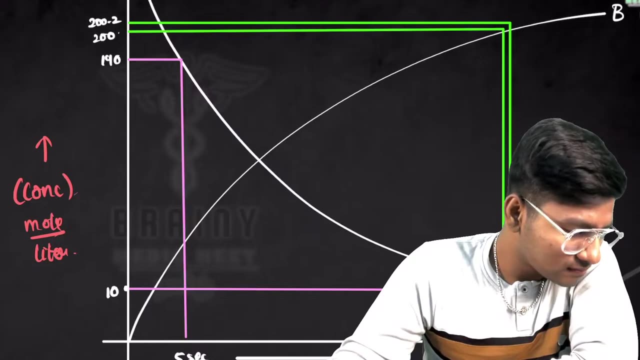 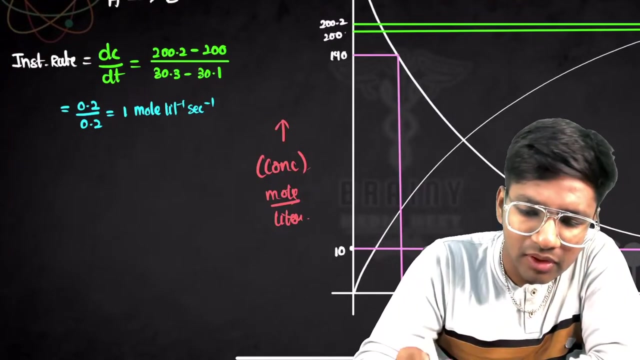 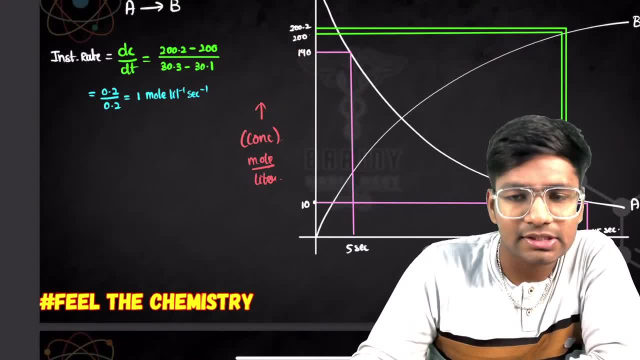 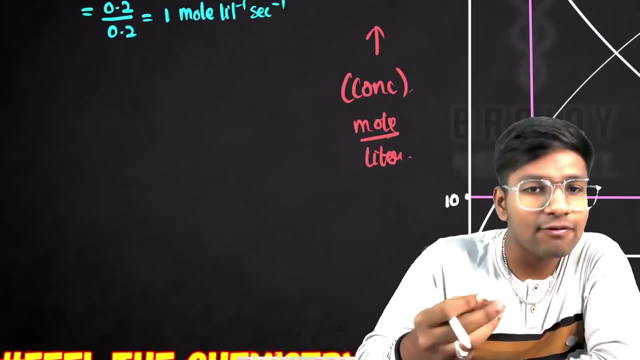 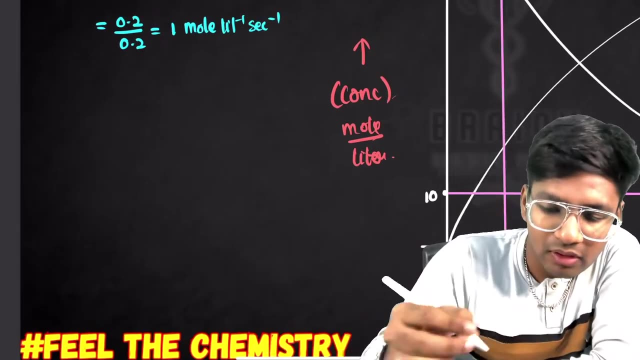 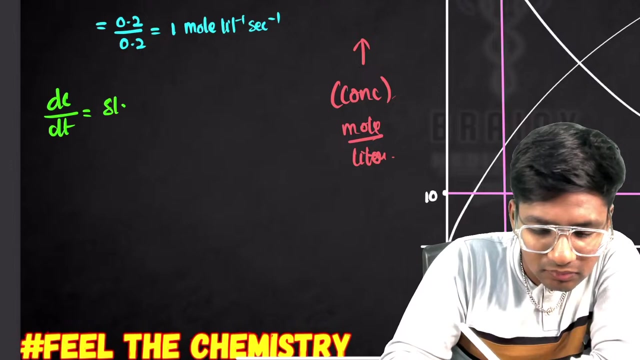 Y by X, opposite by adjacent correct tan theta: simple divide by slope, multiply by area. go and see in graph lecture. if you haven't seen graph lecture, go and see. we will be in live section. last live section: DC by DT slope, slope of curve. 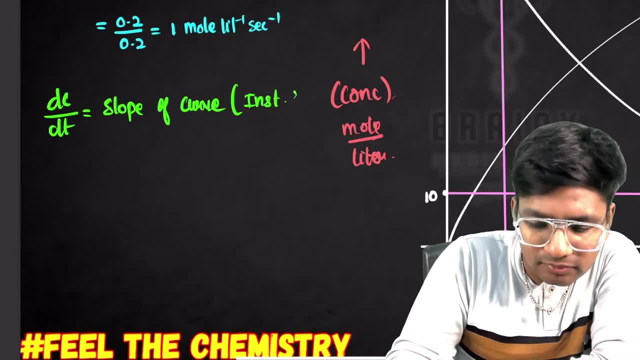 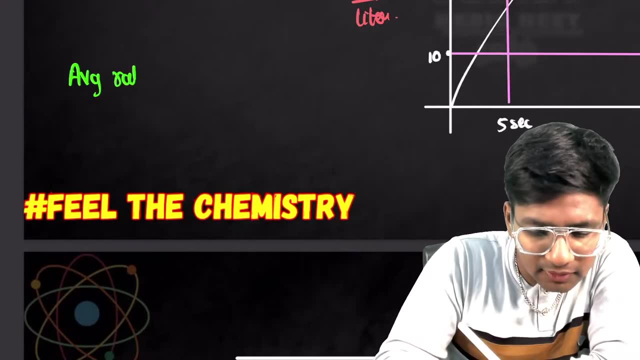 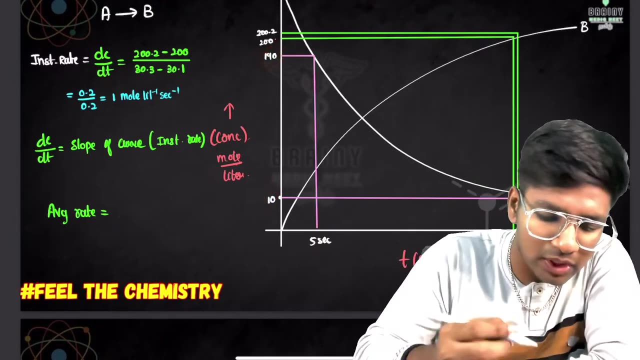 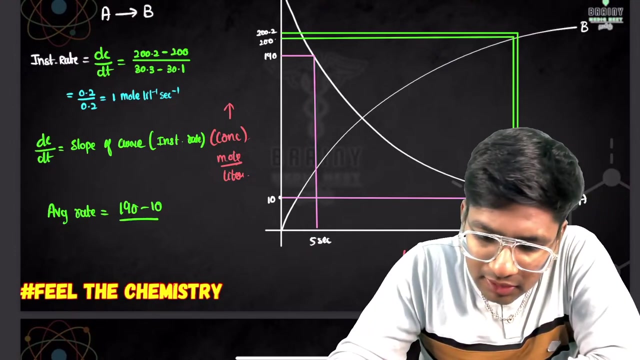 which gives instantaneous rate, again instantaneous rate, next average rate. average rate is equal to, in this diagram, 10. initial concentration, final concentration: 190, so 190 minus 10, divided by time: final time is 45, initial time is 5, so 45 minus 5. 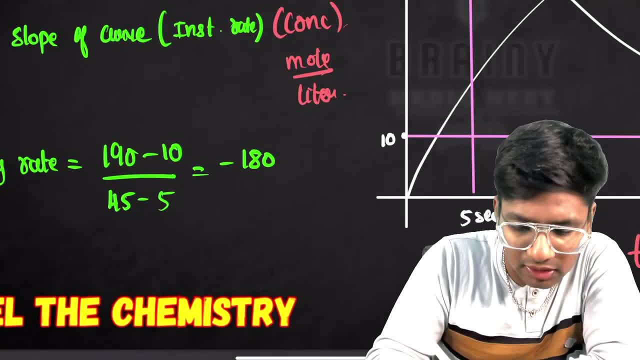 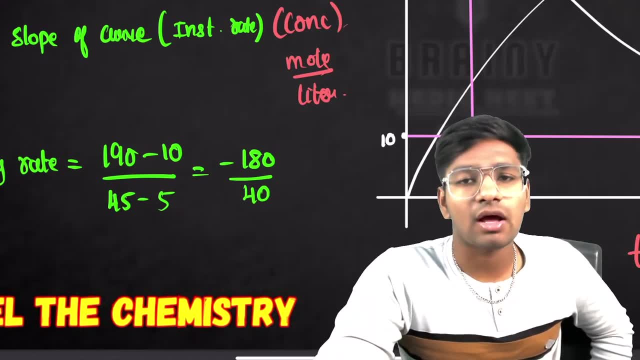 45 minus 5, which is equal to minus 180 divided by 40. done minus 180 divided by 40 average: do you understand all this? do you have any doubt in this? there are only 2 topics. along with that, there are 2-3 questions. 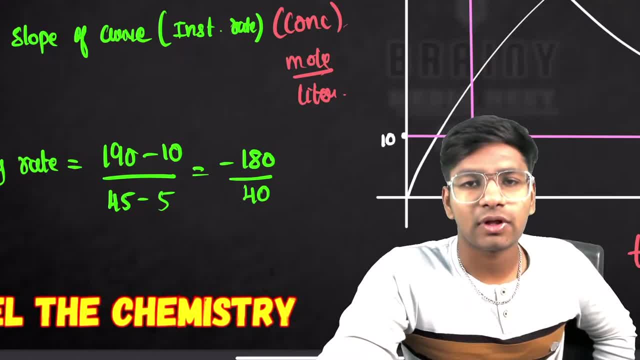 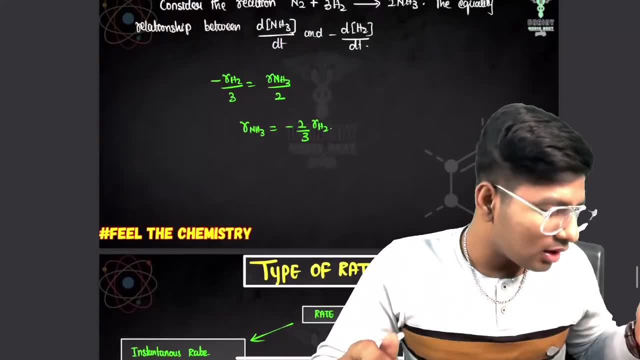 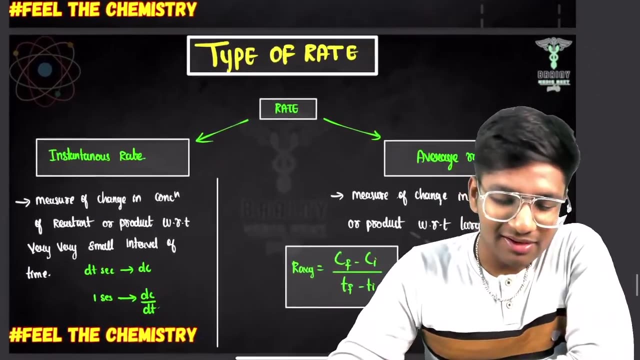 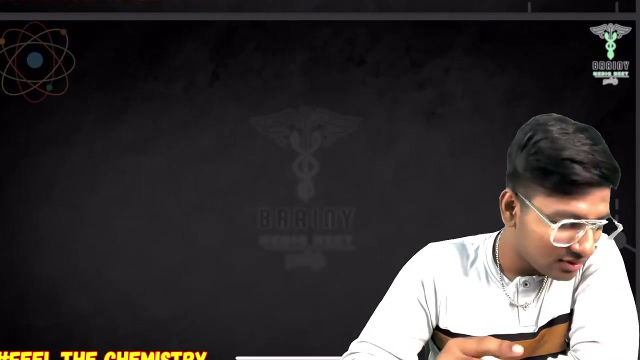 we will complete within 15 minutes probably, I think. ok, do you have any doubt in this? 500 votes, 500 votes. 500 people have voted without any conscience. they don't even look at the class. look at this: 499 votes, bro. what is this bro? 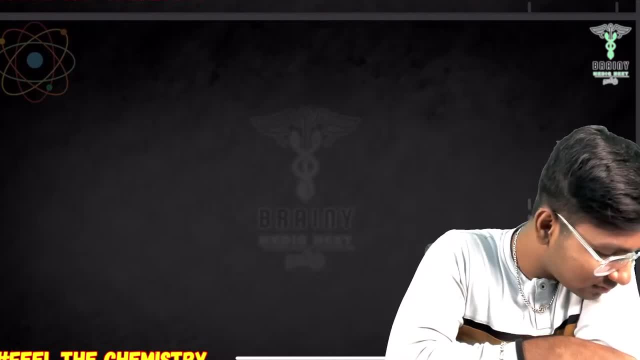 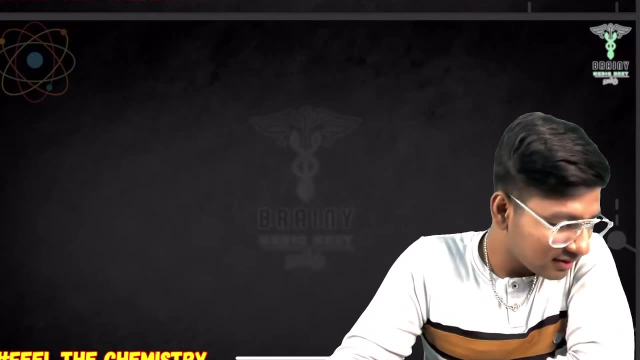 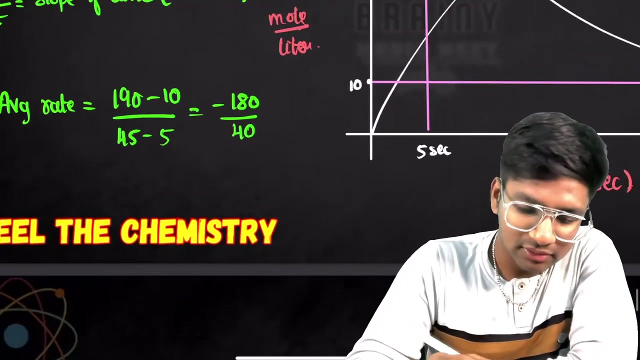 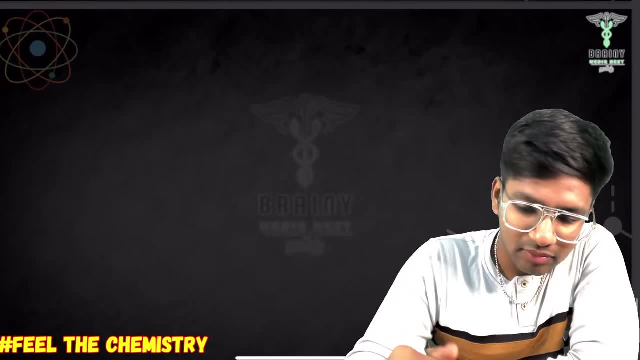 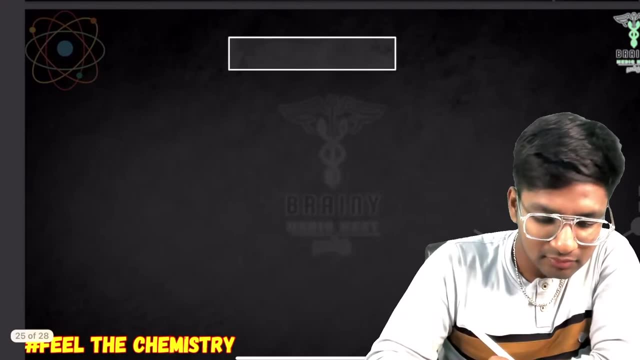 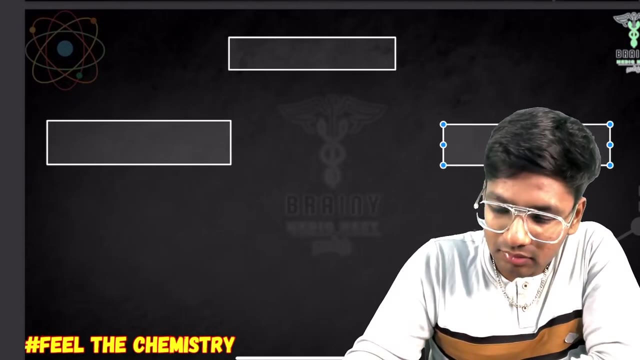 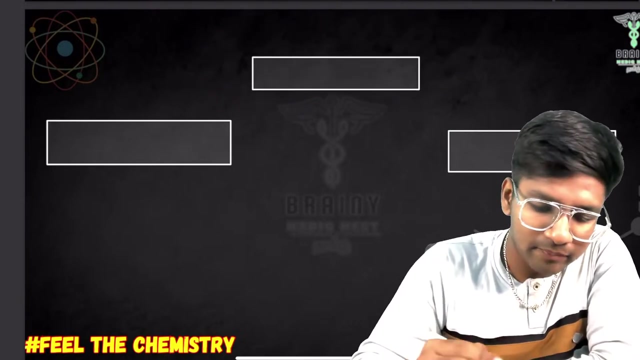 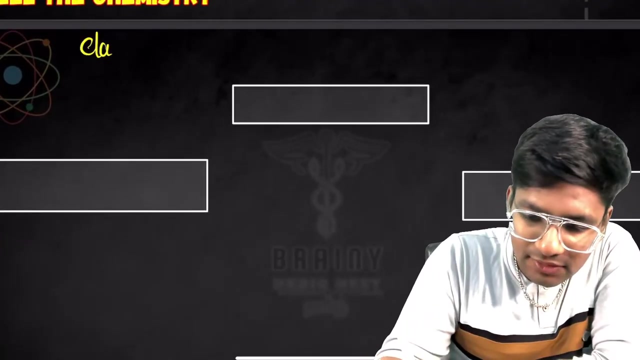 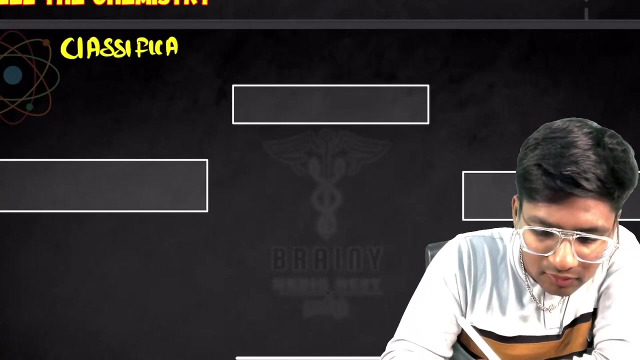 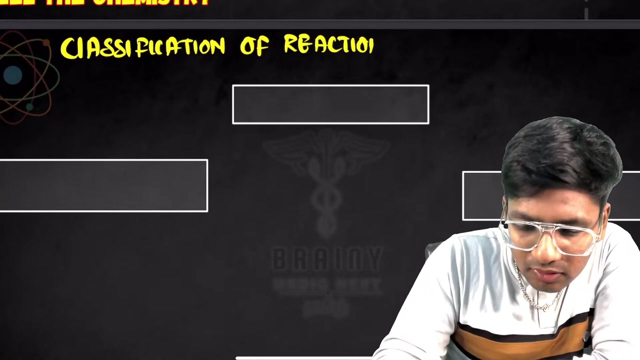 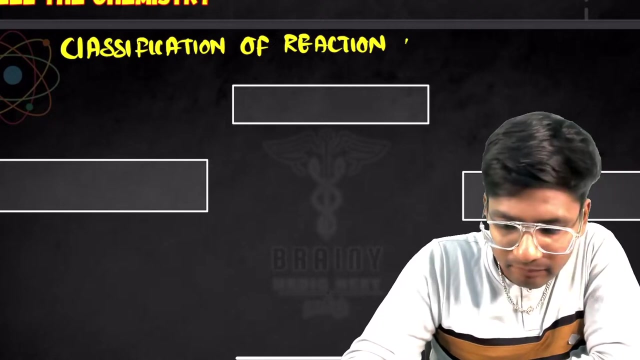 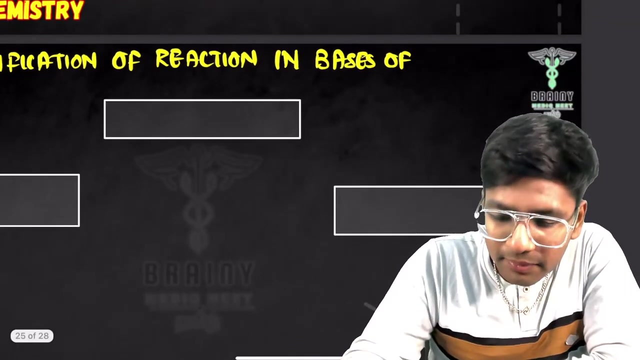 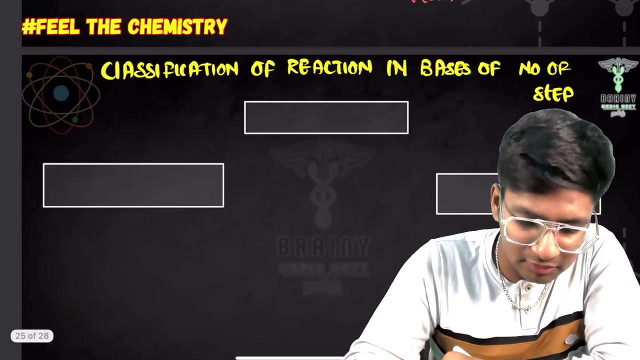 ok, come next, again, next, ok. so see here. classification of reaction. classification of reaction of reaction. classification of reaction in basis of basis of number of step. number of step. ok, this is what we are going to see in this chapter. wait, let me write this like this: 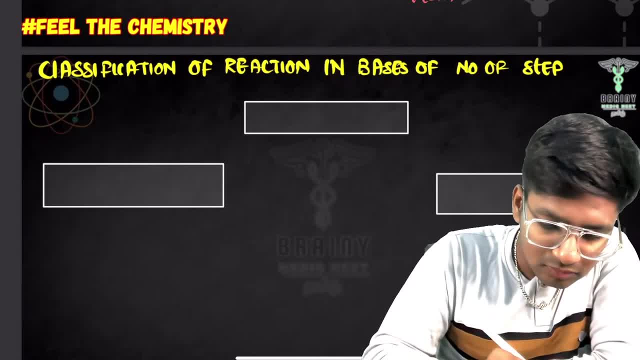 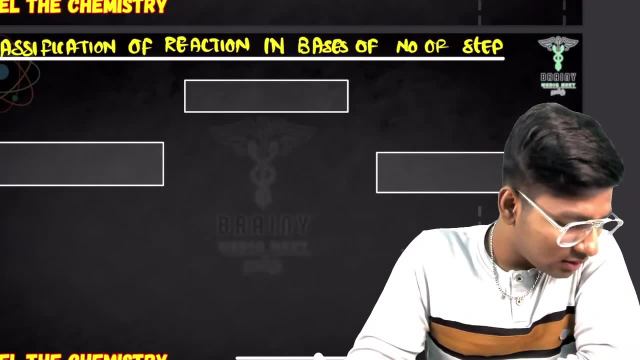 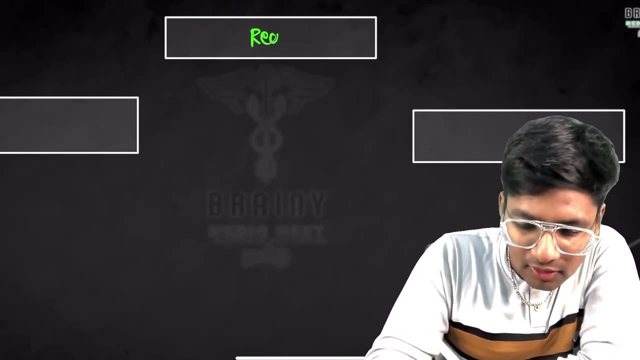 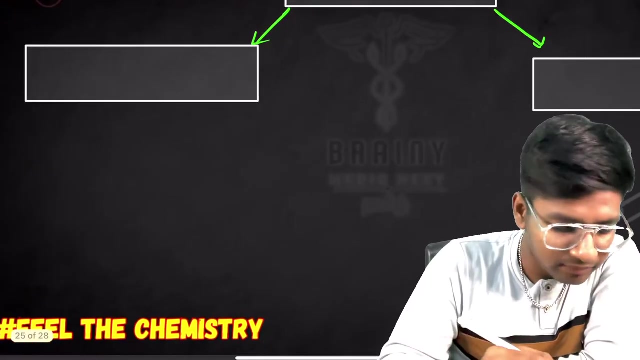 ok, classification of reaction. sorry bro, I am seeing nitrogen from me. ok, fine, no problem. see now. look, we have two types of reaction based on this reaction. based on this, we have two types of reaction. one is elementary reaction. elementary elementary reaction. 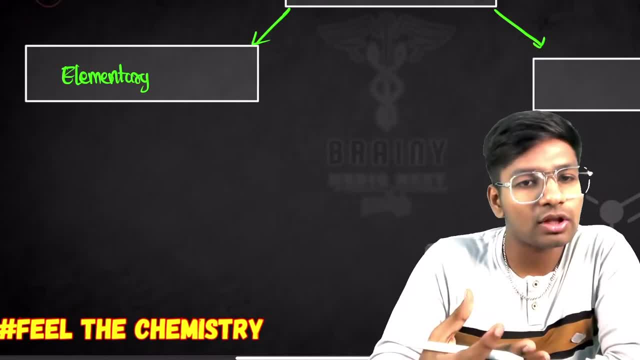 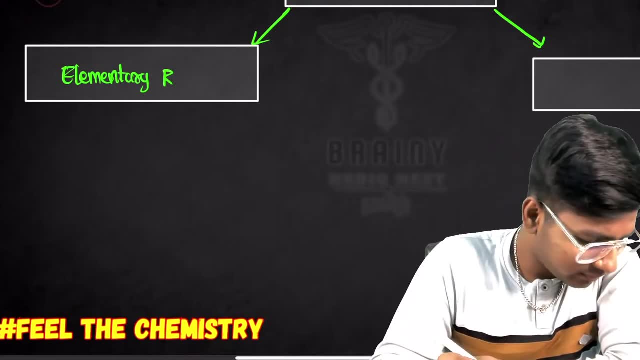 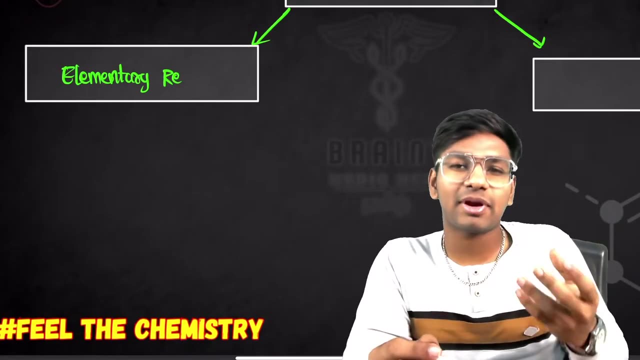 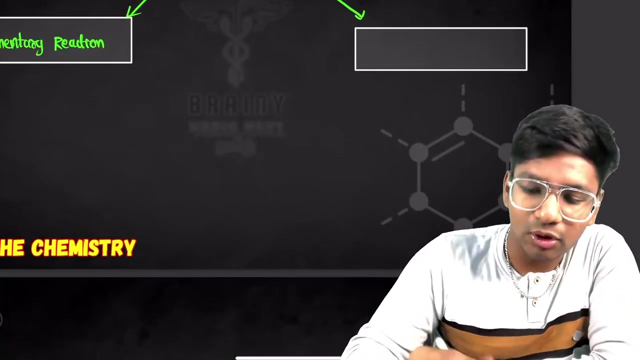 elementary school. like elementary reaction, one is the same. ok, when you were in 1st class, what all did you do? ok, that class only. let see that elementary reaction. BMNT, Bche, happ, Franck. ok, I am now writing here: elementary reaction. 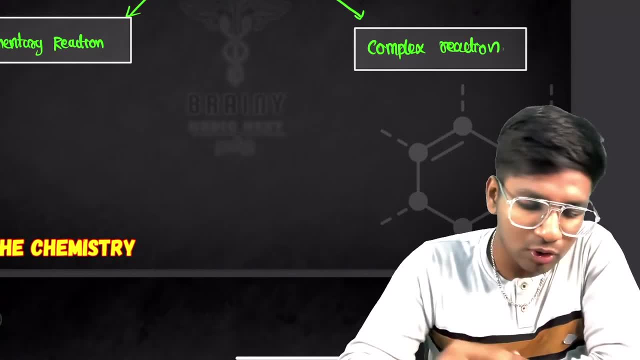 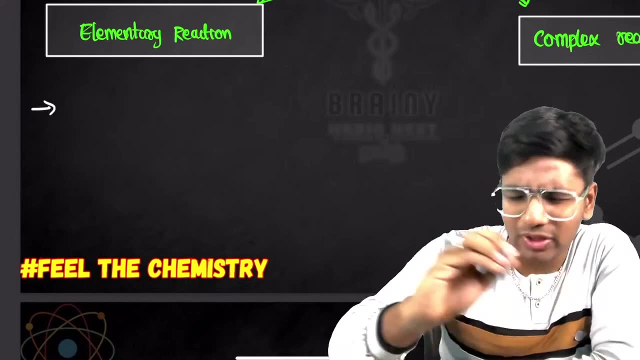 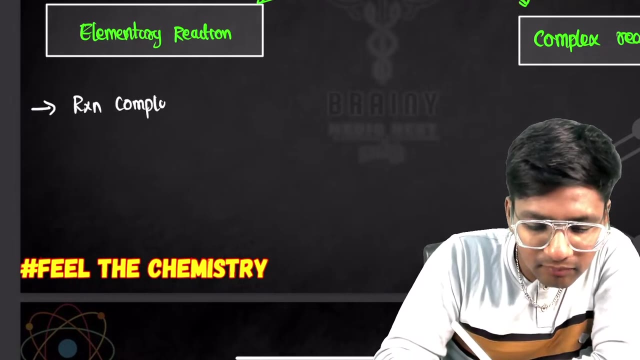 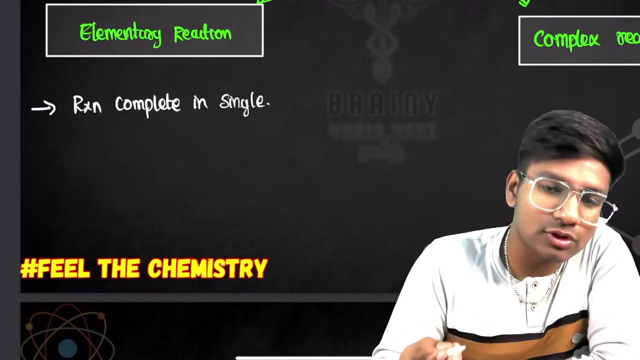 and then complex reaction. ok, then another complex reaction, elementary reaction, and complex reaction, very simple, elementary reaction里서. reaction, reaction complete in very one step, single step. and I'm already single, I'm going to rather: reaction complete, reaction complete in single step. okay, single single. I'm going to like, for example, I mean the statement of 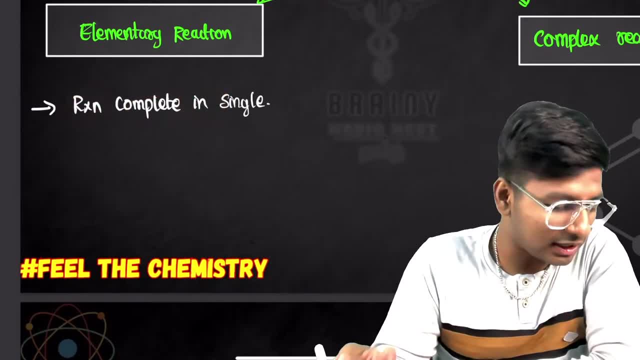 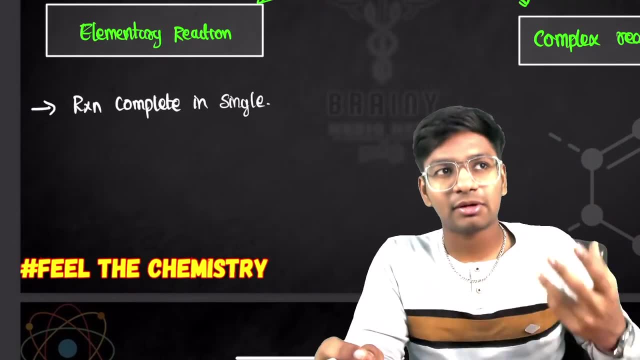 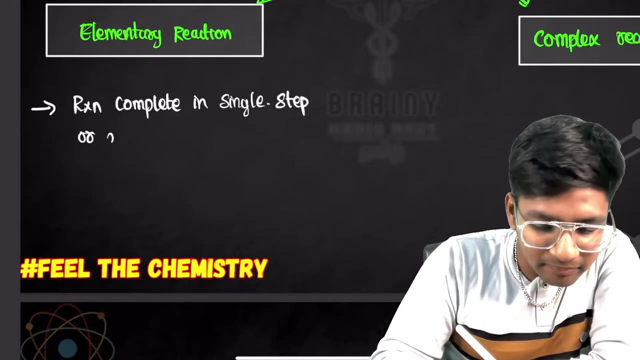 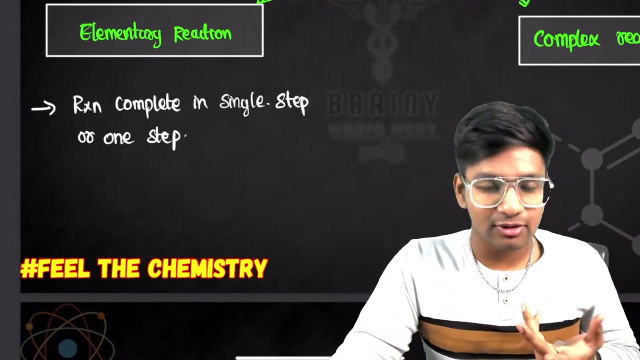 Matthew, reaction complete in real step of the name of the correct career and I will end up on a reaction complete in real step of the running. understand how a single step missile around. okay, single step, or one step. okay, or one step. so in the money we're gonna be able to, because NTA pretty. 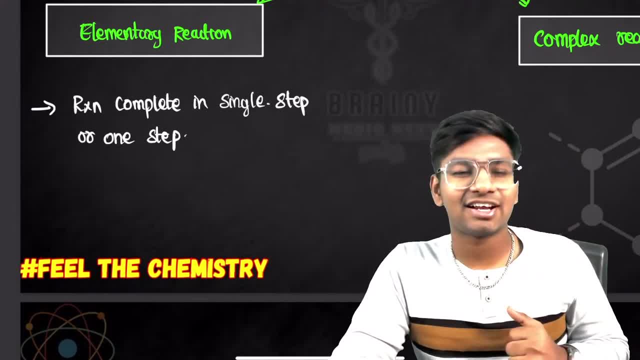 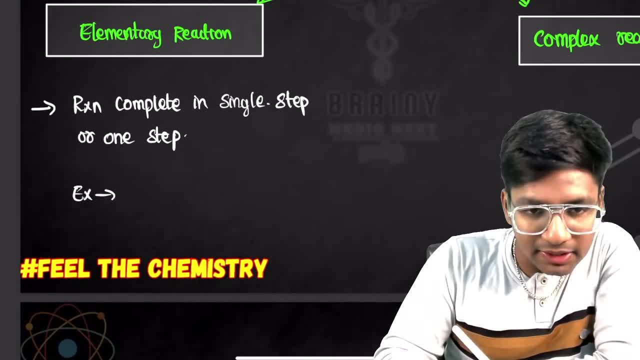 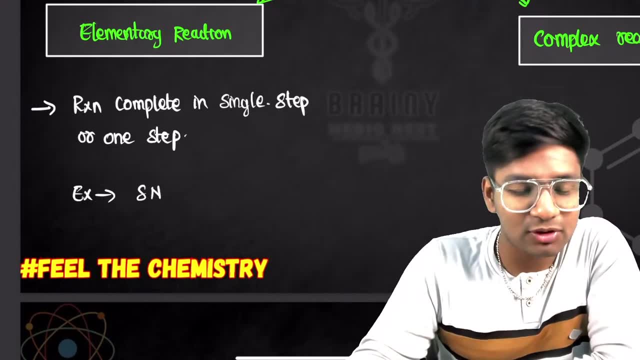 give you a single step. and then I'm going to give you a single step, slightly answer for another one. so example for the asked near a s and two reaction ended: a mother, essential reaction, sometimes reactional, been performed a pretty single organization in to be action. okay, by its an action. 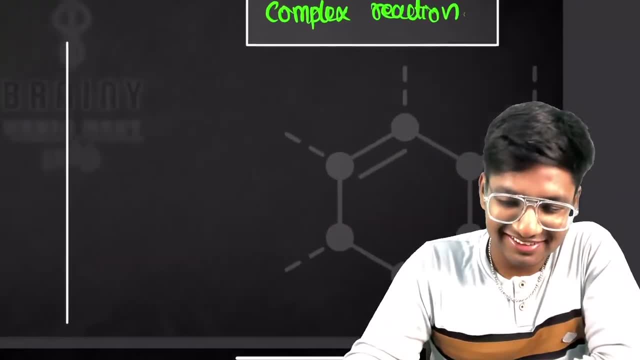 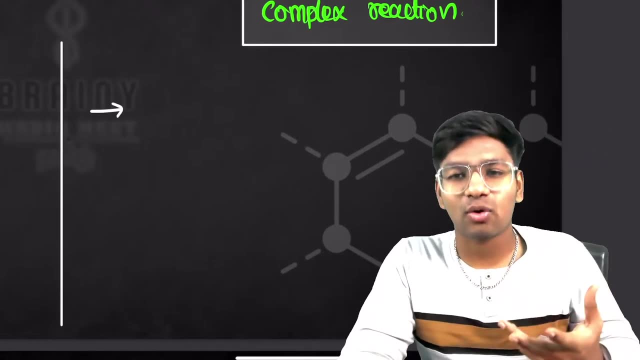 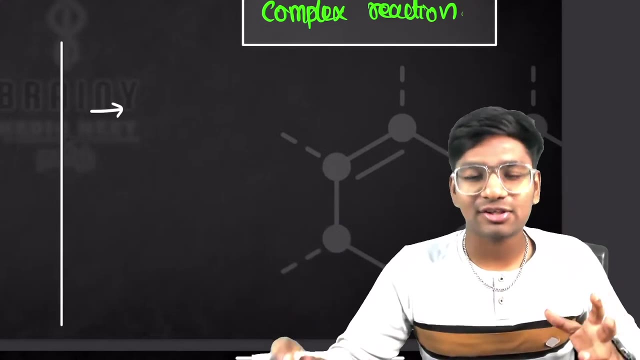 madam NANiera, entirely upon da to see a picture next to party in a reaction, complex reaction, and we just know, I agree. ok, not every hojea performs upon a and up in the cell, or call in the cell, or call, or your reaction, so in the cell. 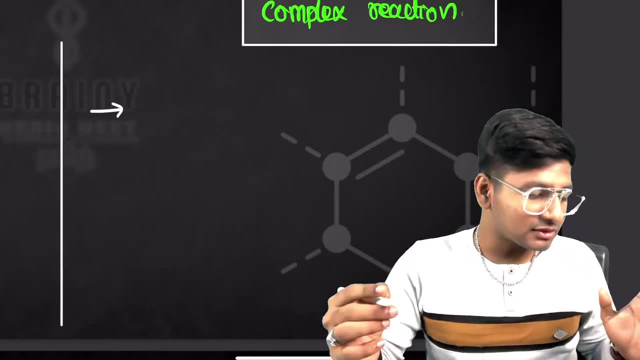 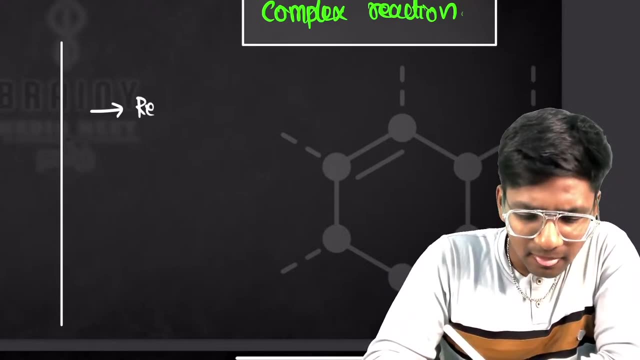 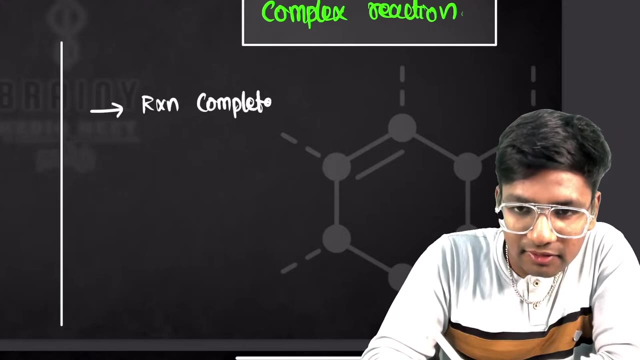 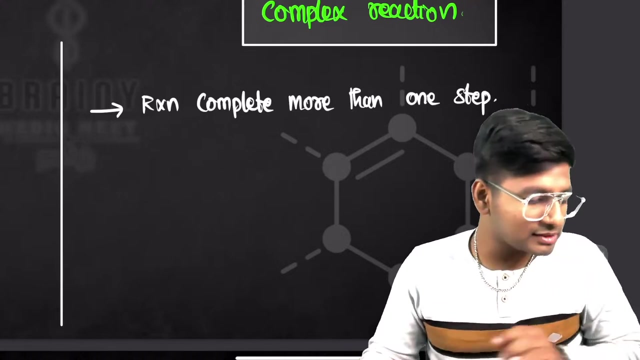 or reaction on the cell, or reaction up in order okay, on the body in which now the complex reactions reaction even when they either coin of a summer together, the action complete in more than one step. more than one step in the cell, or step one on the cell, or step on to put in покkama. 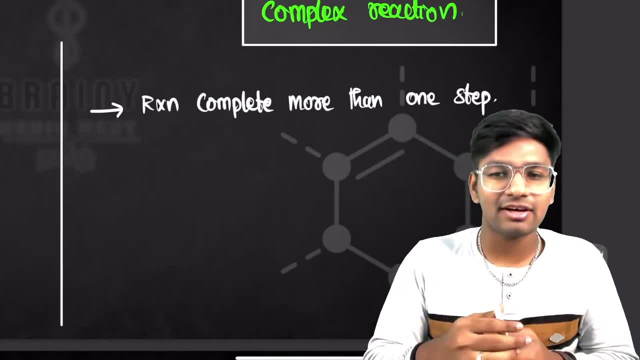 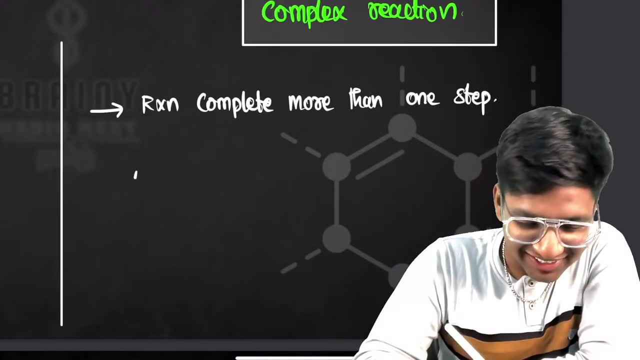 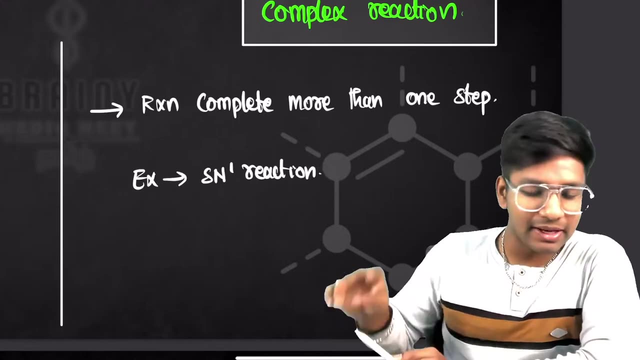 I only install outside it what's a blue cell snapchat. or say the elliot me, one day I'm going to cut on the moon, for you know, in the mother a is sorry in a area to the salmon role. example s and one reaction: okay. example s and one region: its. 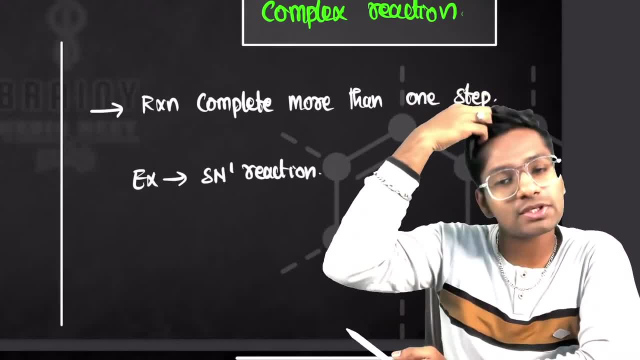 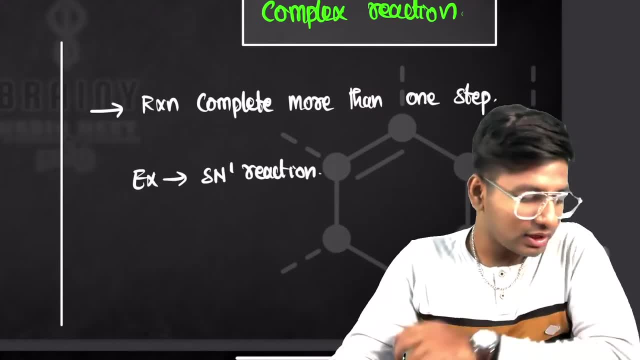 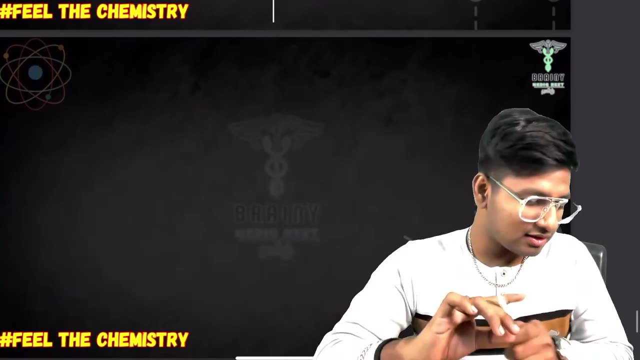 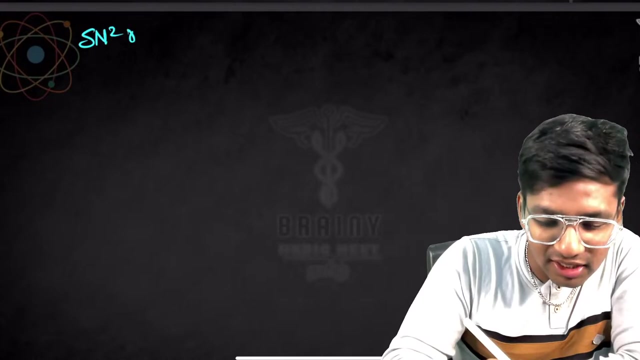 a single direction. let for stores that are proper. no car work at information are the proper reaction. ok, that is your complex reaction. for example, I told you about the complex reaction. ok, fine, no problem, what to do if you don't believe me? SN2 reaction happens. you would have known about it. 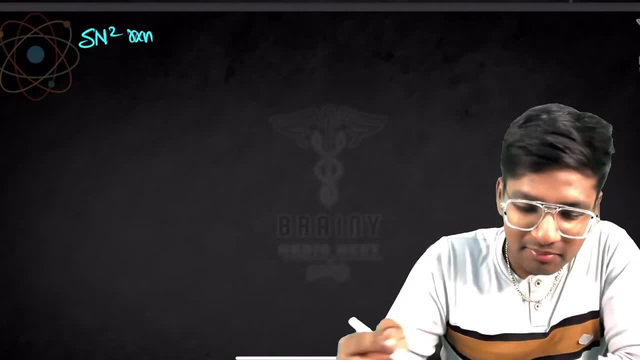 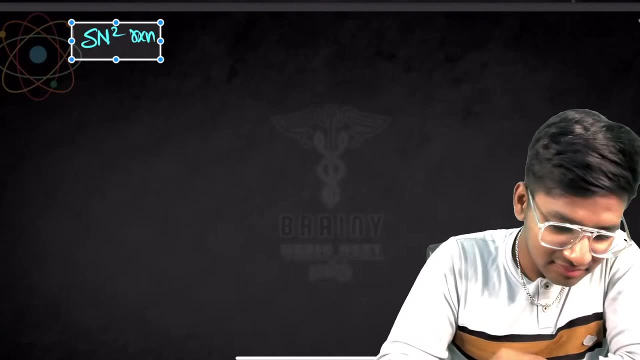 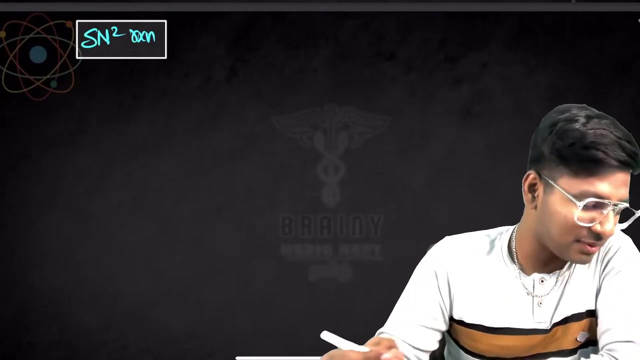 I have told you about the SN2 reaction in detail. I don't think any of you have seen the lecture of Hal-Holkins-Halloran. I have told you about it. I have told you about the chapter. I have told you about it. we all are the same. 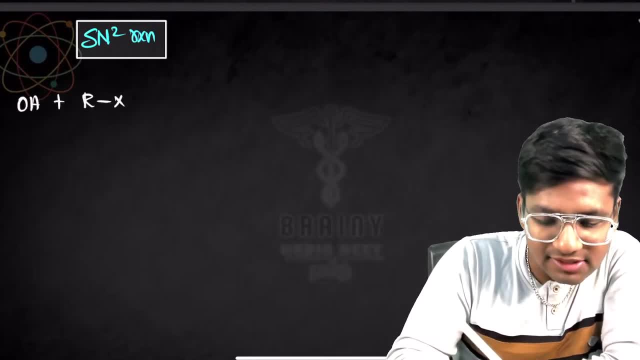 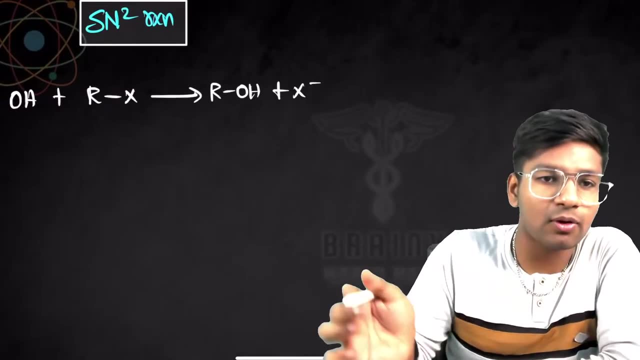 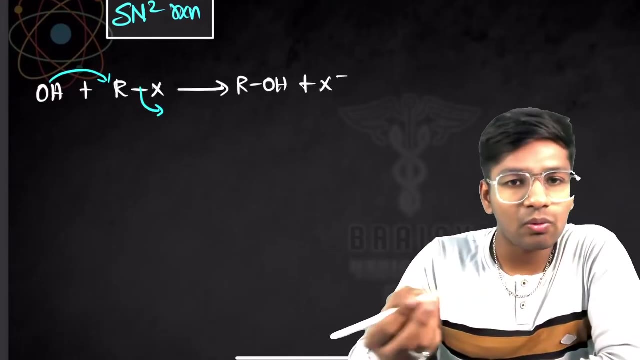 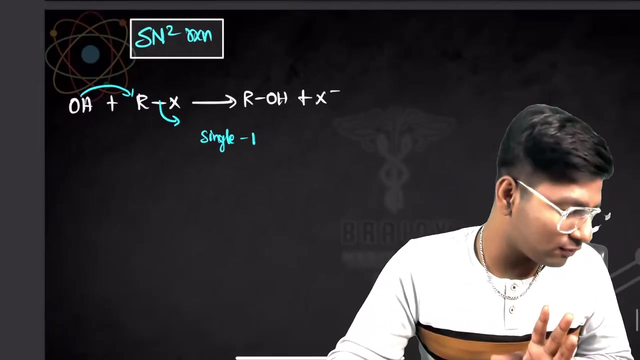 ok, so see: OH plus RX gives, ROH plus X minus. all these will happen in the same step in this process, in the same step. if we attack here, it will come out from here. in the same step, single step. it will happen in RIAZ. step in single step, this whole process will happen. 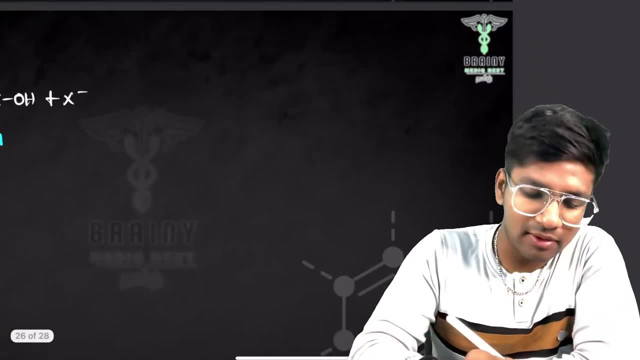 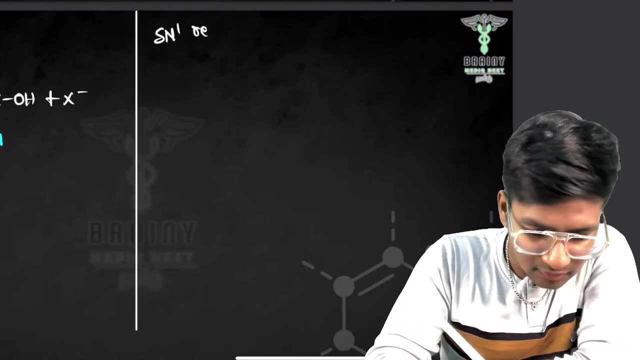 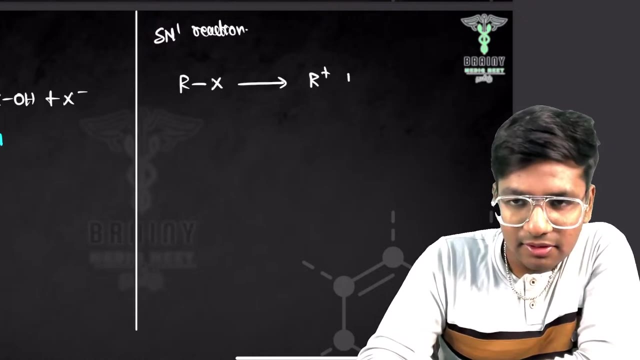 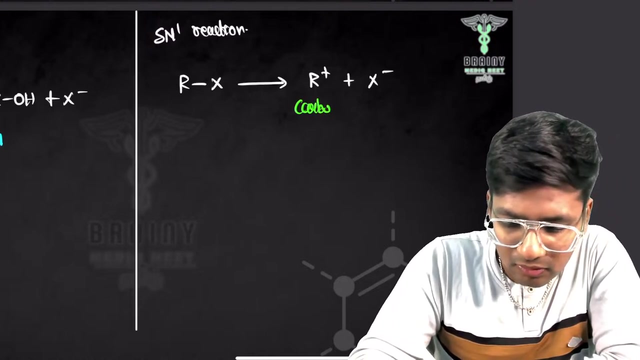 ok, but if you have taken SN1 in the same place, SN1- SN1 reaction, there will be RX, R plus, X minus will form. ok, but R plus is a carbocation. it is a carbocation. how, what will happen? in the first step? this will go out. 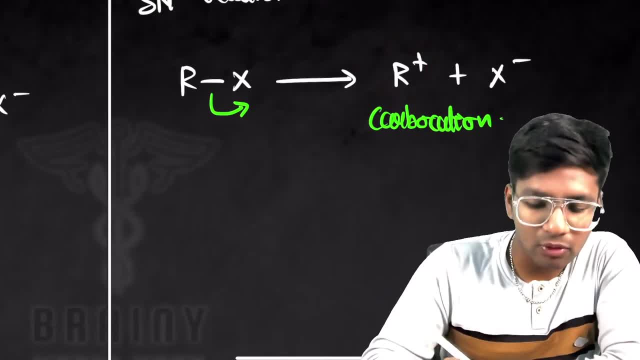 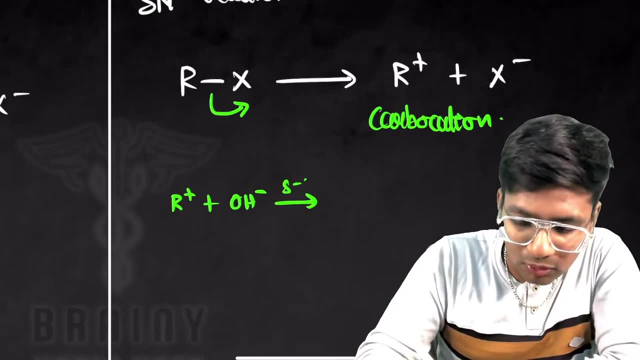 after that, carbocation will form here. next, this carbocation will be attacked by a nucleophile. ok, OH minus will attack. this is step 2,. this is your step 2, this is your step 1. after that, ROH will form. this is your complex reaction. 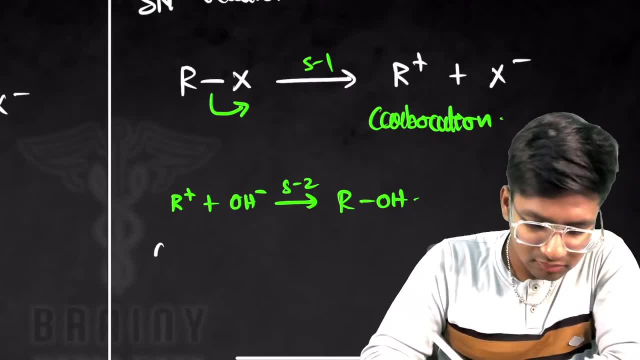 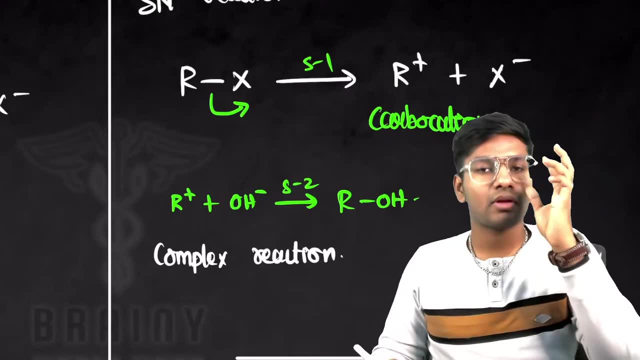 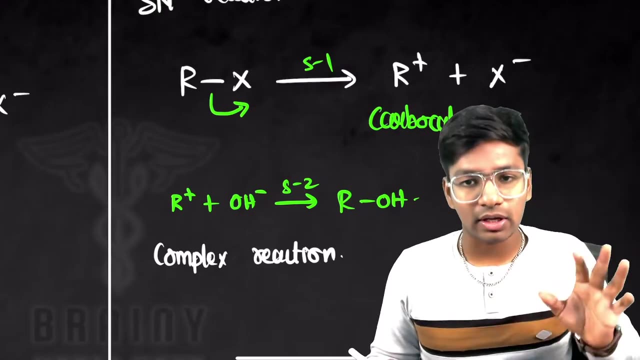 this is your complex reaction. see, I have sent the link with the video in private, sent the link and asked them to take it. I have sent the link and asked them to take it, that is, asked them to be public, but no response. not even they are replying. ok, I can't do anything. 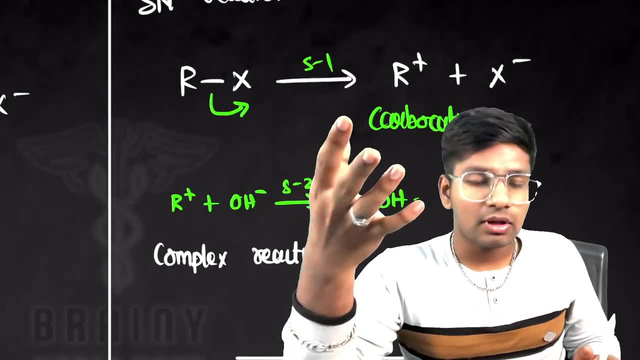 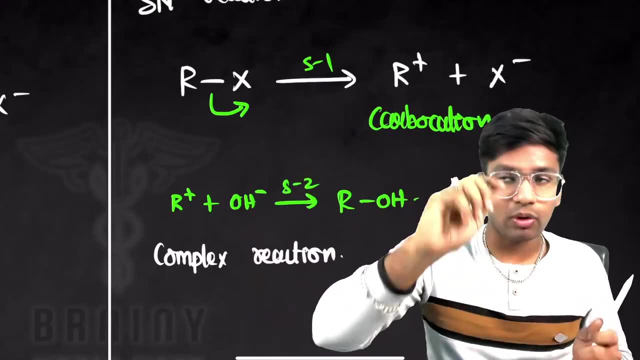 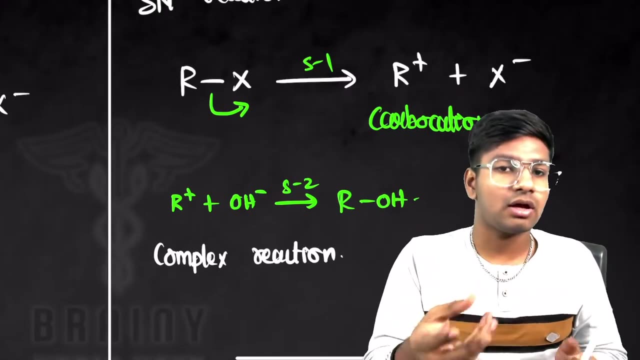 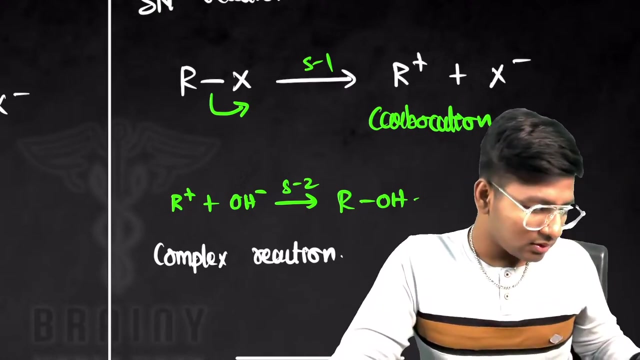 they don't here. see, I can't do anything for the sake of my students. I even searched for the link in my whatsapp and insta and published it. that's all I can do. I don't have any connection with that channel. oh, it's been a long time since I asked Vivek to see the lecture. 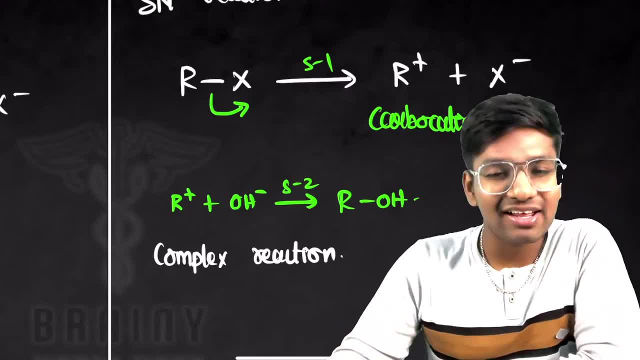 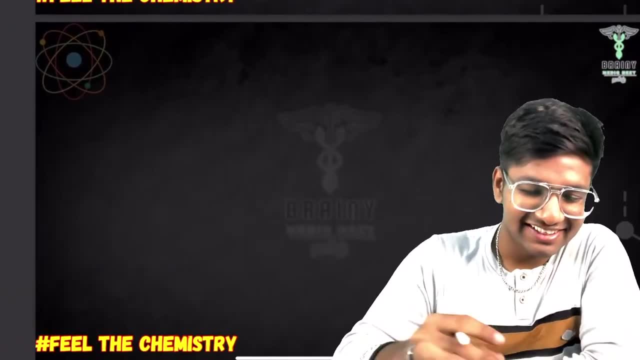 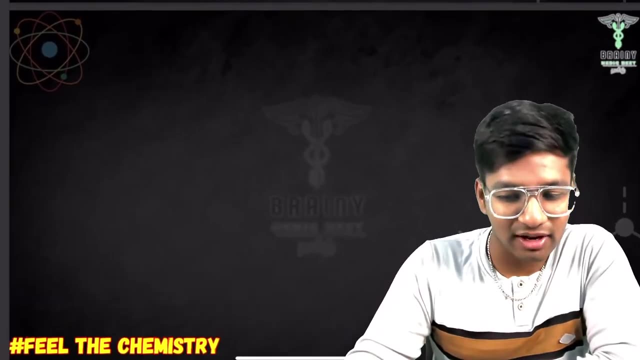 I told him that I have done my job and asked him what to do. ok, fine, let it be. sometimes we have to lie for the sake of the place where we are. we have to talk a little, but we can't. that's why I started to face problems. 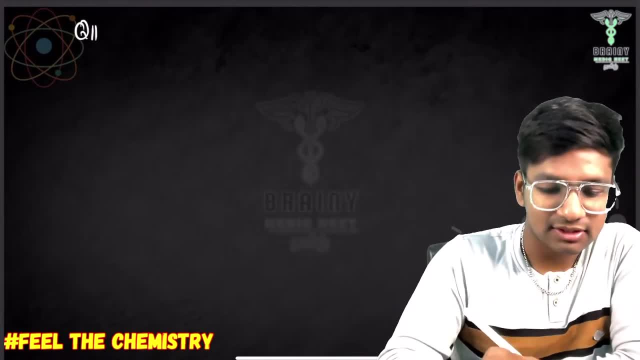 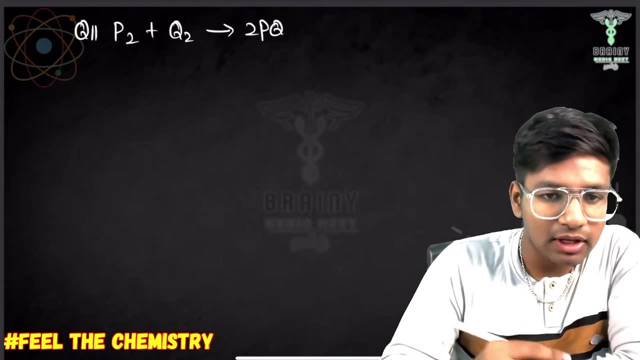 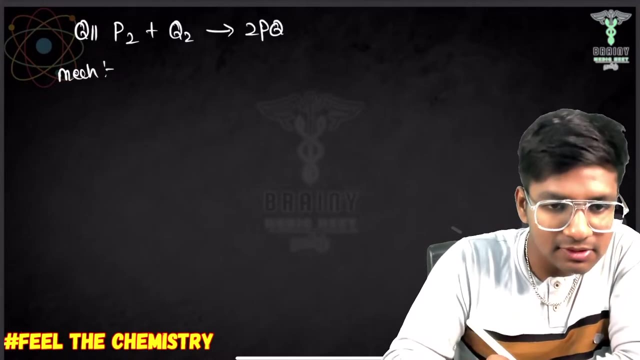 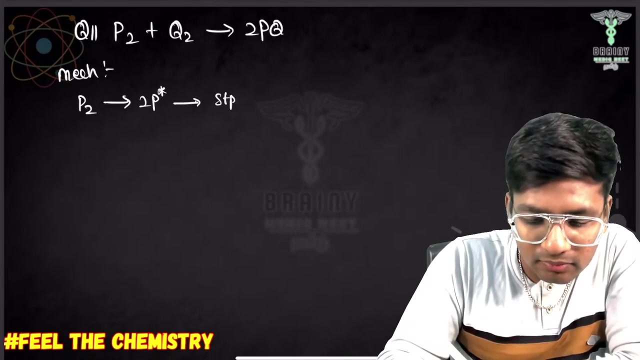 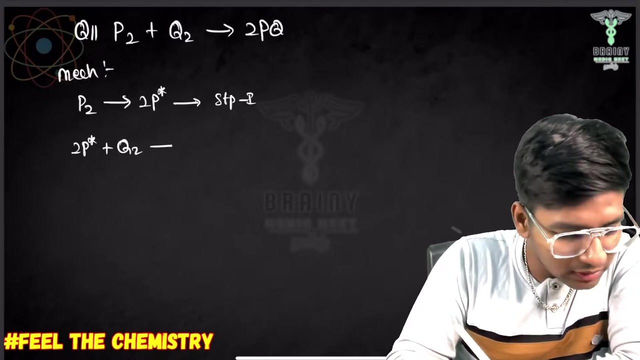 I wanted to be honest: p2 plus q2 gives 2p cube. ok, what am I asking? mechanism? mechanism is: p2 gives 2p star. ok, this is step 1. step 1: 2p star plus q2 gives 2p cube. 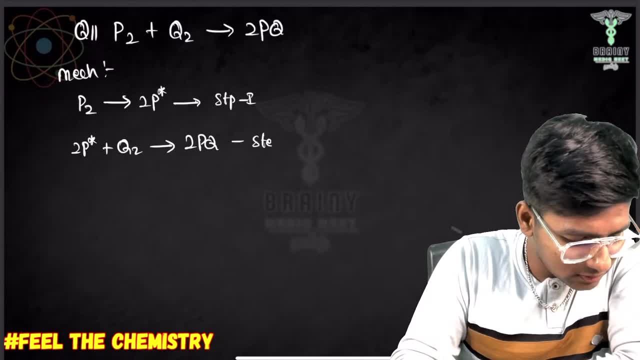 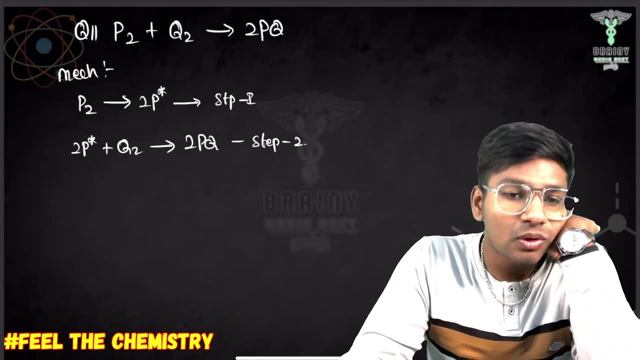 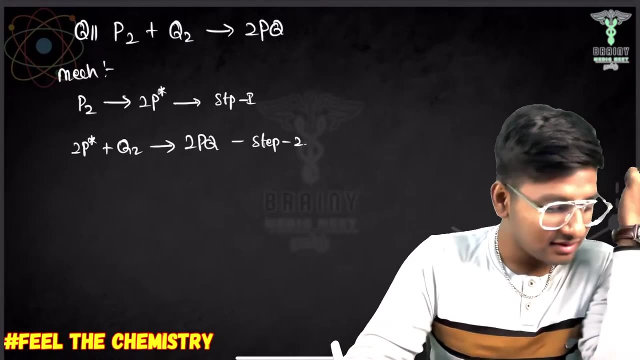 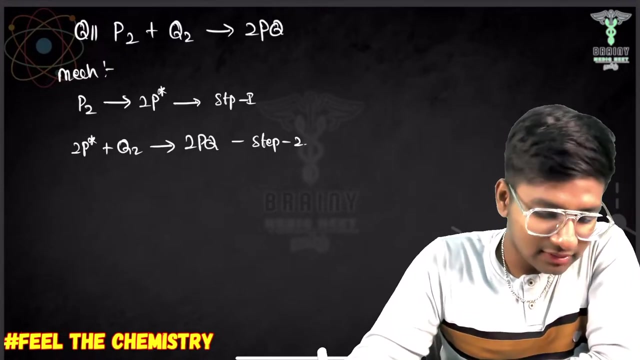 this is step 2. now let's talk about p2. see, what reaction is this? what type of reaction is this? do I have to give you all the options, maybe? what type of reaction is this? a reaction ah, Riaz reaction or normal? 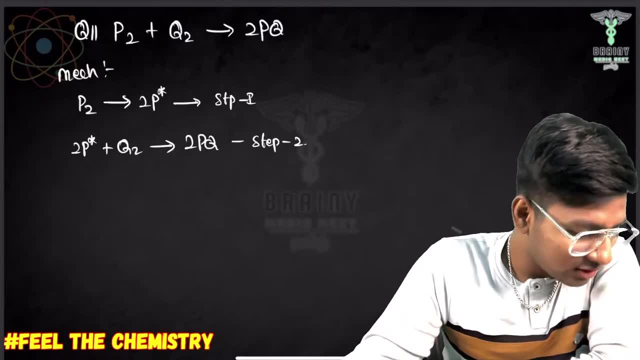 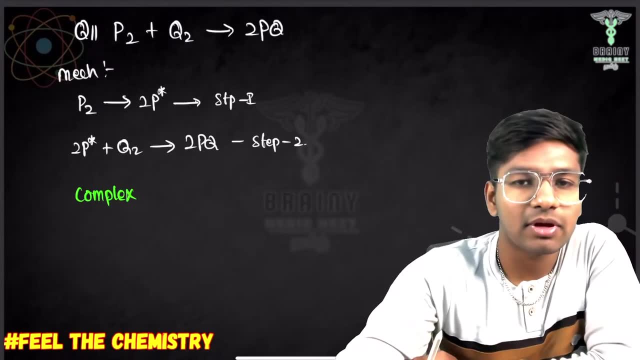 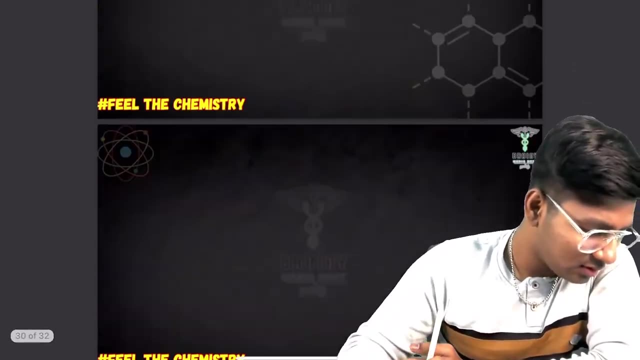 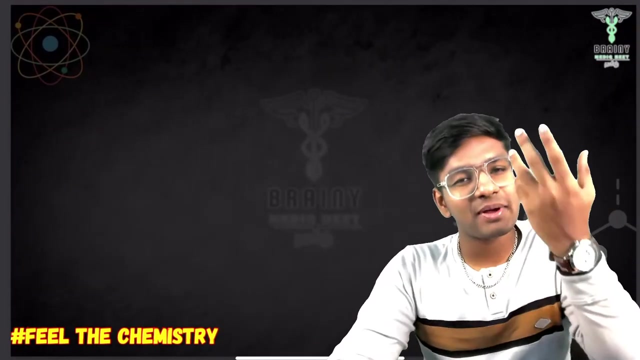 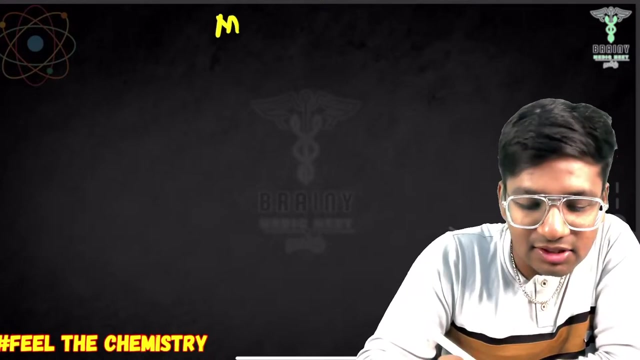 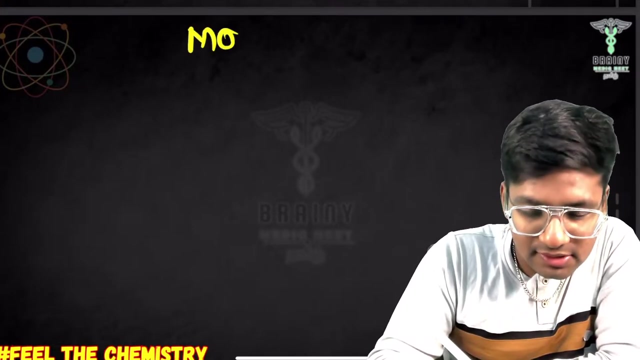 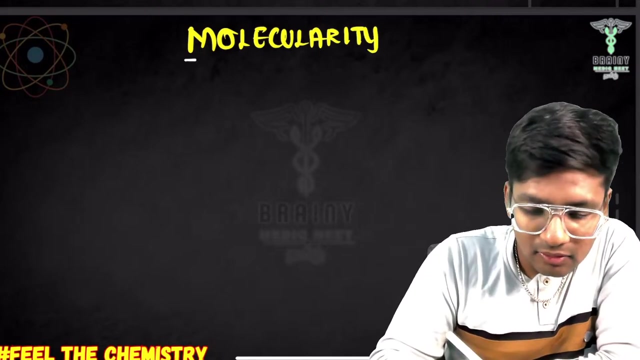 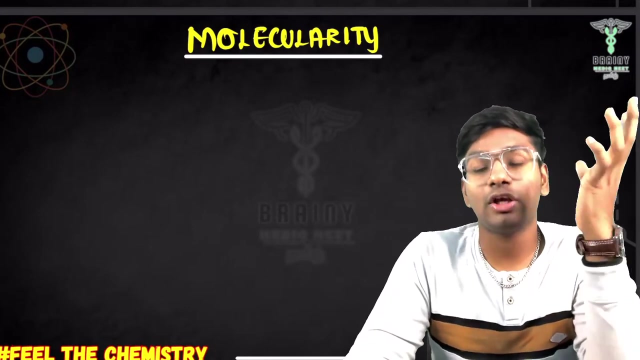 other reaction. say it. what reaction is this? should I even answer to it? it's a complex, complex reaction. next, molecularity: last concept of today's class, last concept of today's class: molecularity, molecularity, molecularity. what is molecularity, molecularity, molecularity, molecularity. 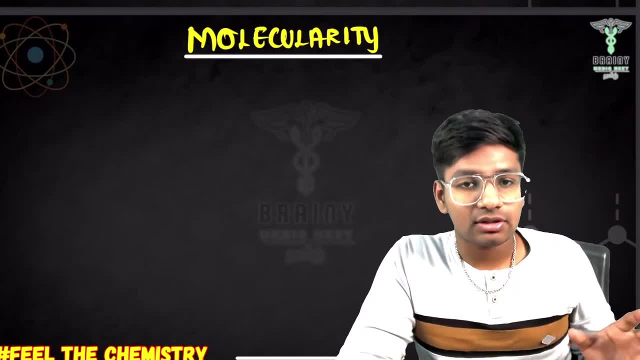 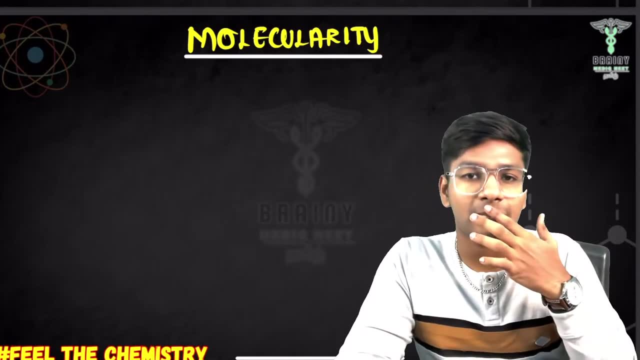 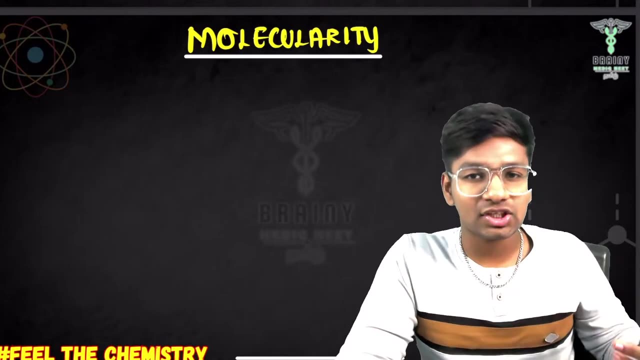 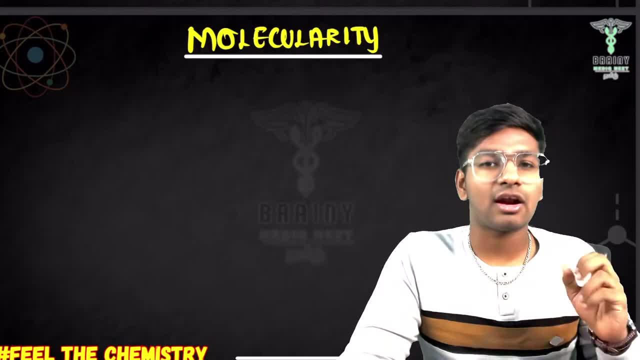 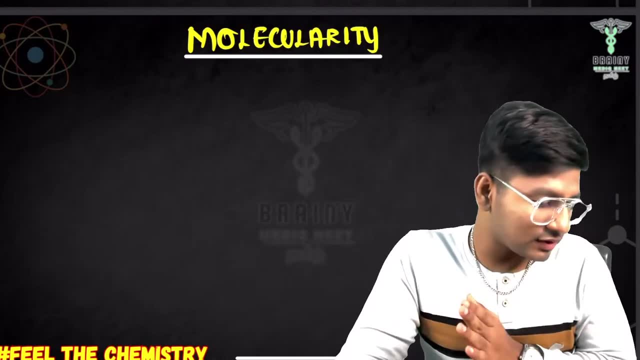 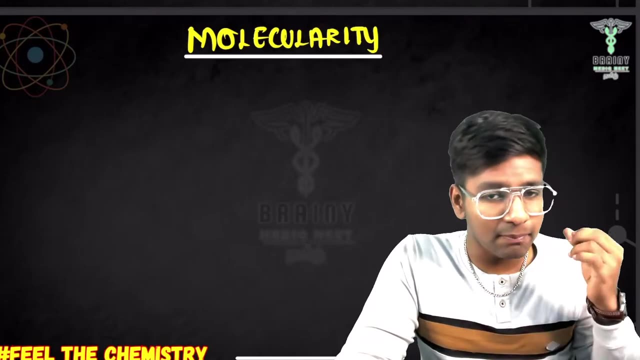 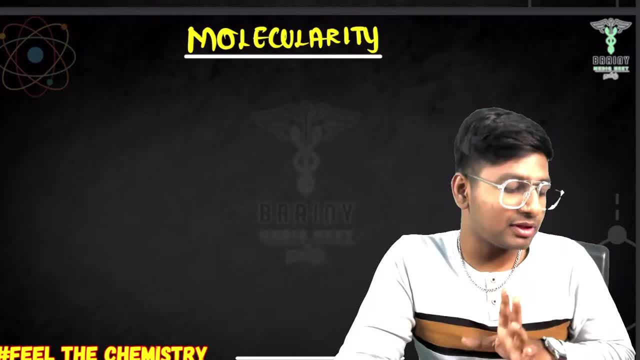 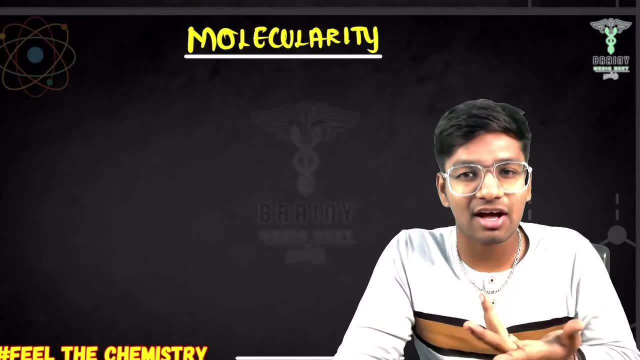 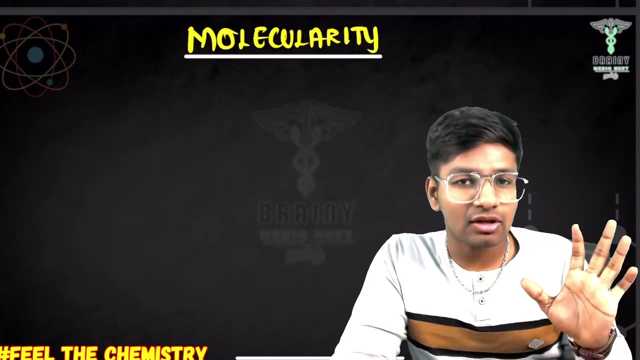 you don't know that your life will be ruined and then you won't live like this. you won't be able to clear your NEET exam. you won't know that, but you will think that you need it and you will go and beat them. at that time, a reaction will happen. 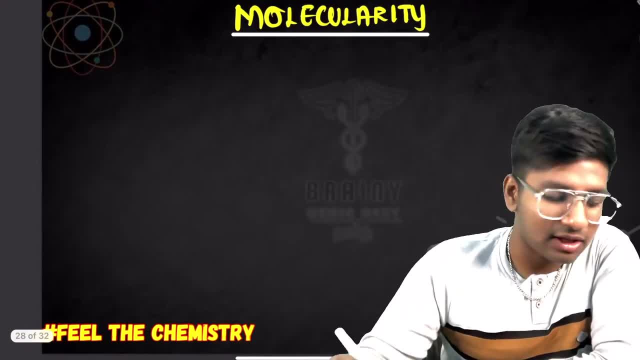 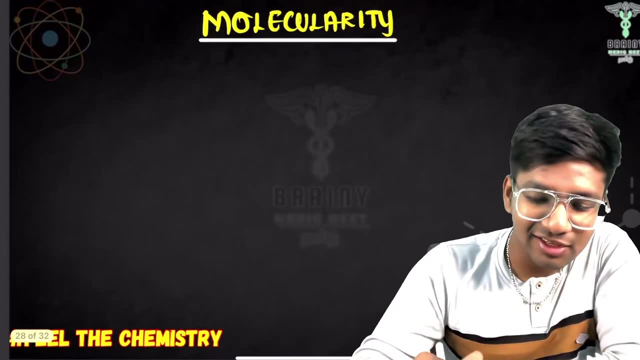 if you beat them, the reaction will happen, or else it won't happen. I will explain that here. understand that if you beat them, the reaction will happen. you will be beaten by them. then the person who asked you to beat them you should have told them. 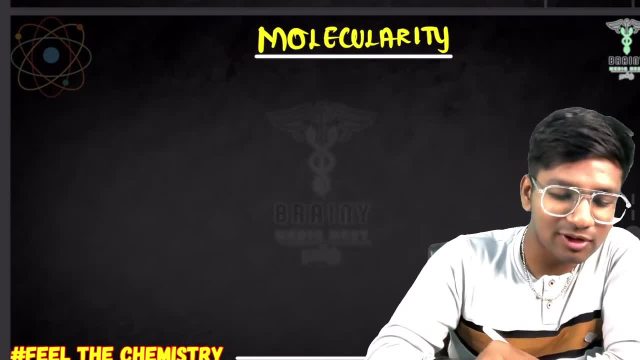 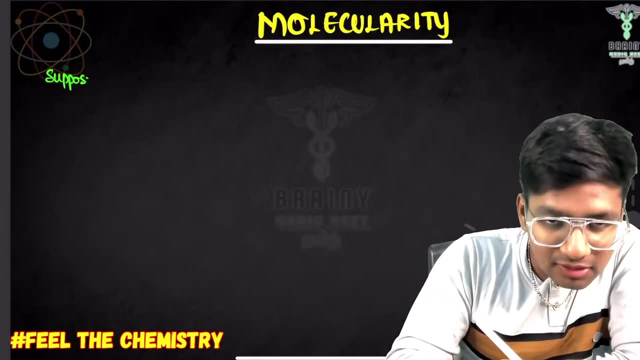 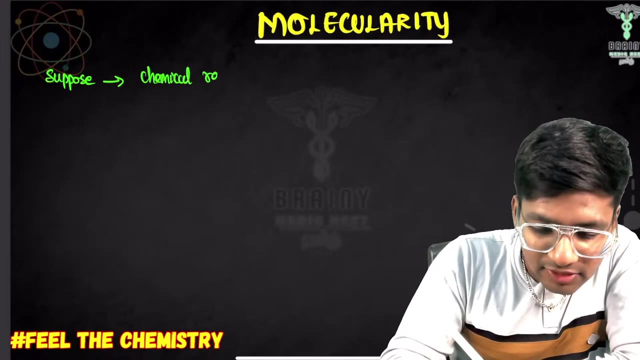 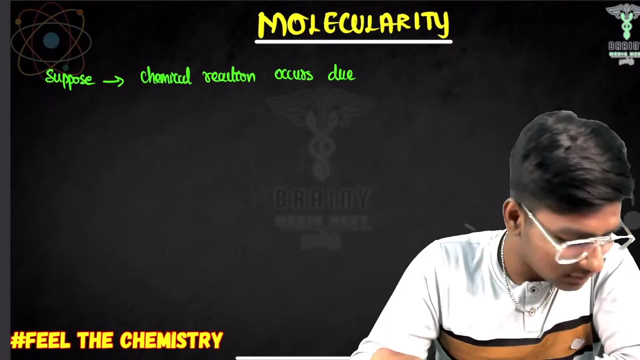 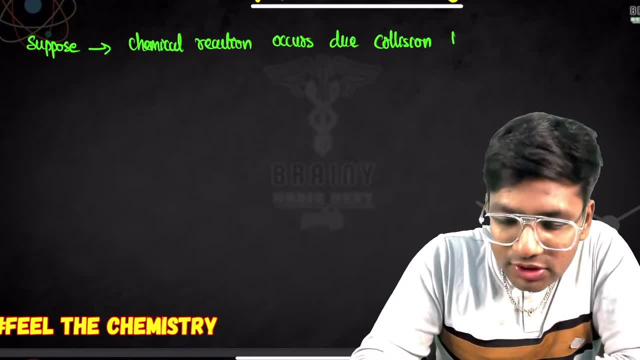 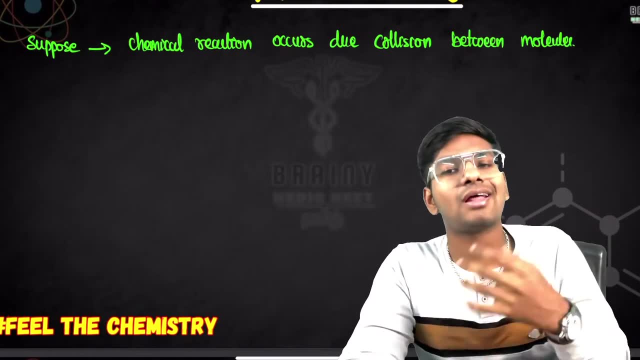 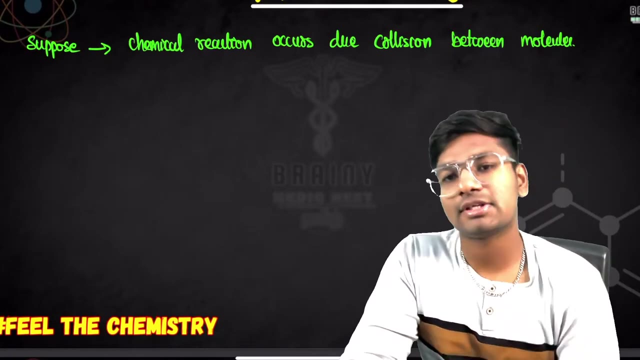 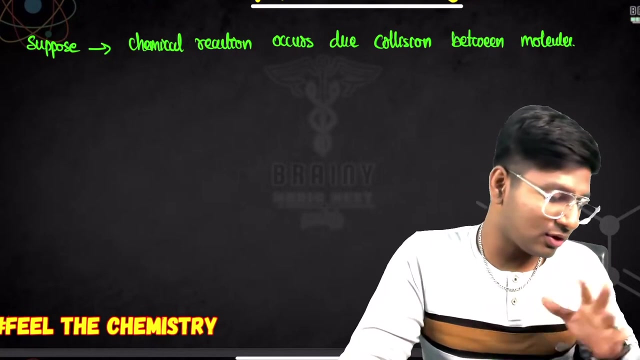 collision, collision between molecules. ok, collision happens only then reaction happens. you go and break it. then, like in the movie Vallavan simbook, you wake up in the morning and call me. like that, you will get caught. I don't have any connection with that, ok. 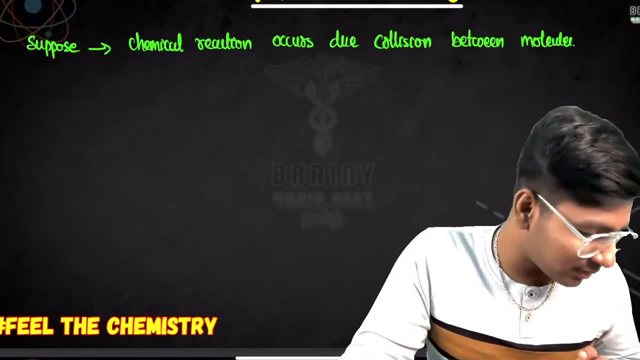 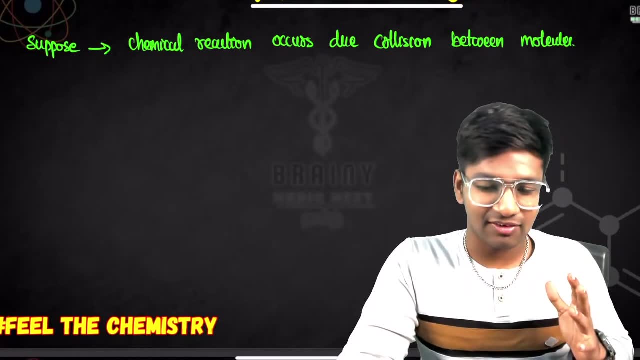 I am just in the opposite side of the pool. they will catch me and throw me away. ok, then you have to talk to me all night long like that. you will get caught. Valk is close to you. ok, you go and break it. he will say like this: why? 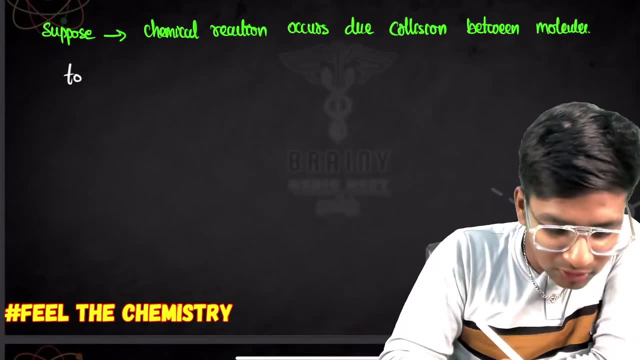 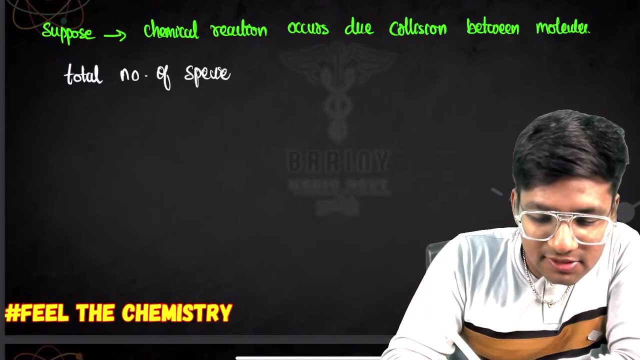 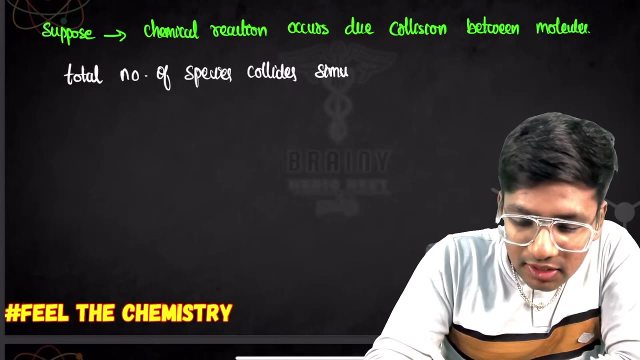 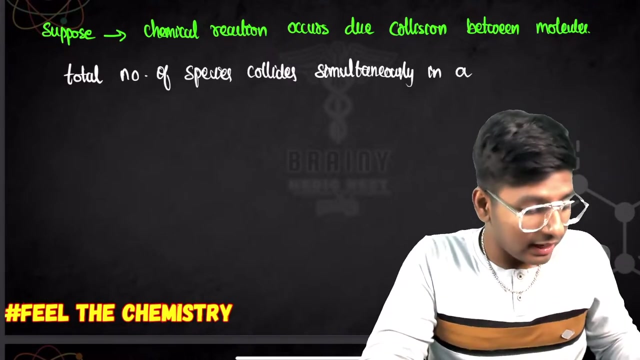 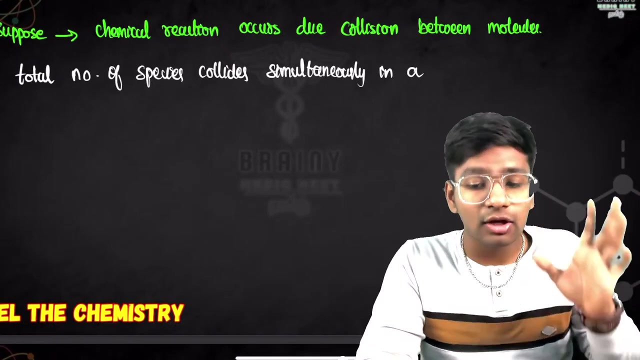 so close it and let's see how it works. so, total total number of species: total number of species collide simultaneously: collide, collides simultaneously in in a, in a, in a. I am going to write an important word here. this word is very important in an elementary reaction. 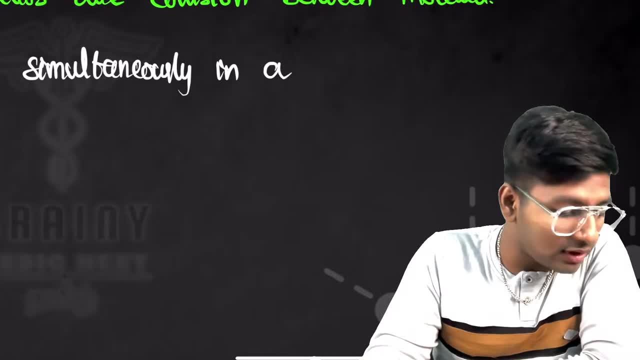 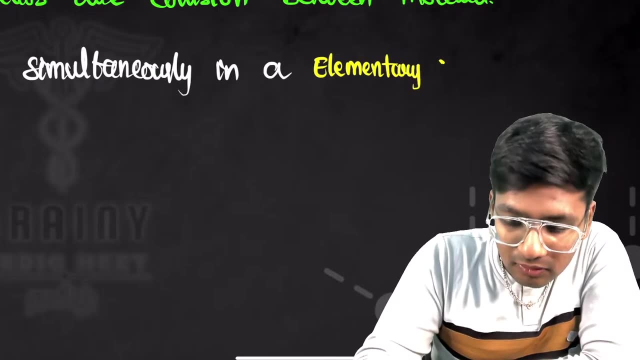 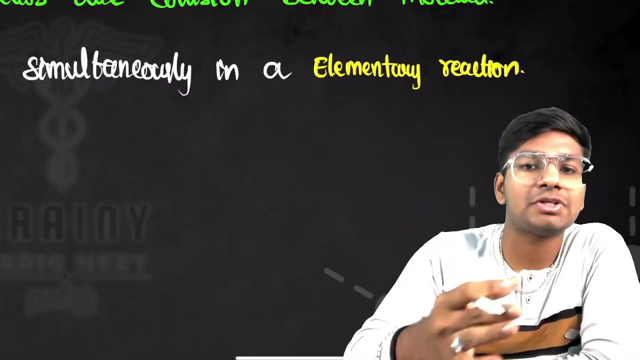 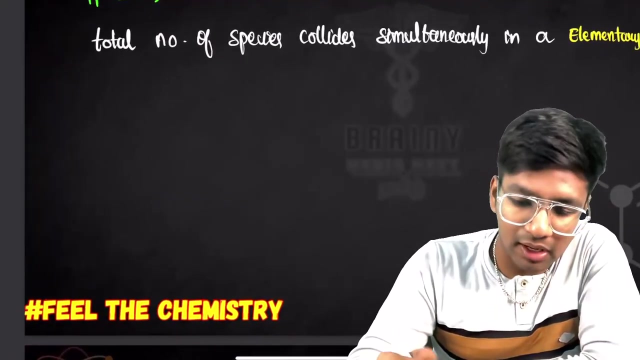 it is not a complex reaction, it is an elementary reaction. this word is very important: elementary reaction. it is an elementary. it is an elementary reaction. you can measure the molecularity in an elementary reaction. only you can measure the molecularity in an elementary reaction only. it is not defined in a complex reaction. 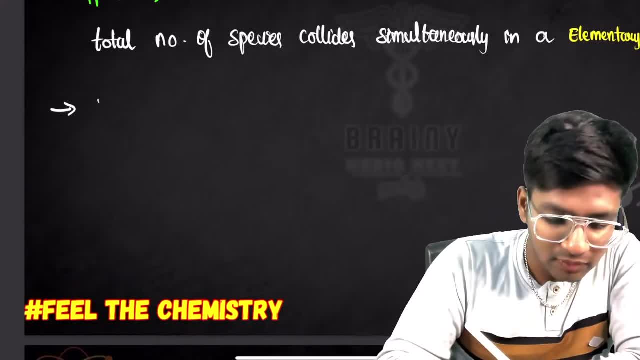 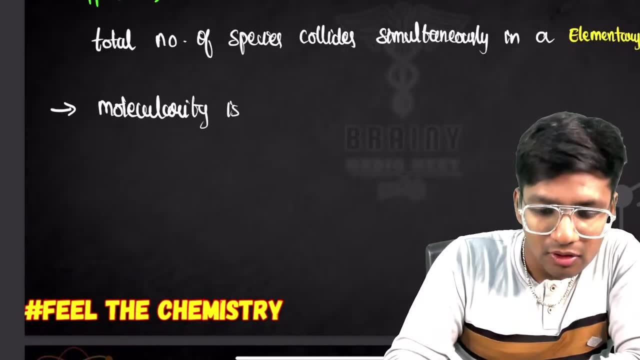 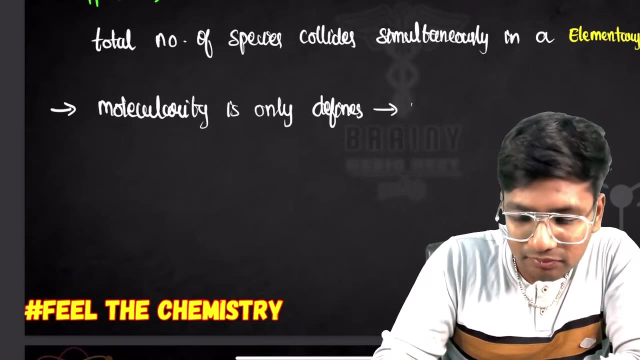 so what are you going to do here? molecularity is only defined for, molecularity is only defined for, defined for, defined for five years in college, and in college, in a few years, and in a few years. in a few years, yeah, and inctorium, I am going to show you. 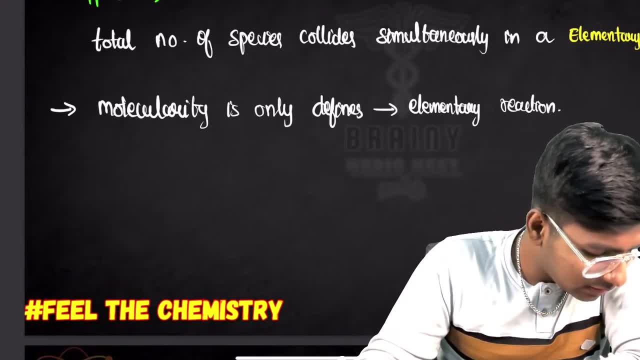 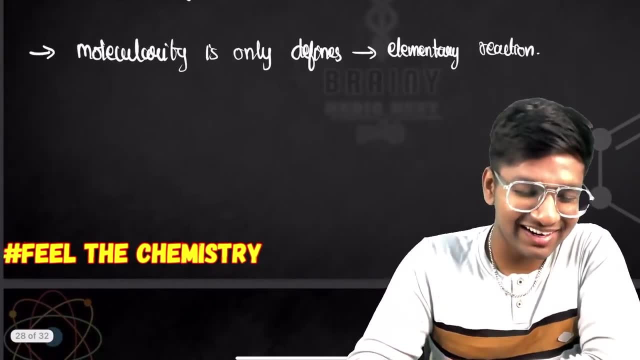 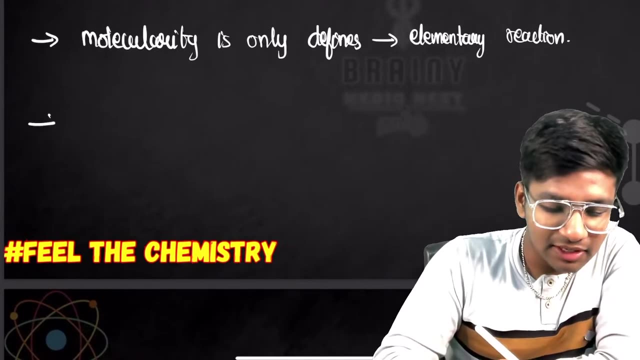 a story of that and the general science, language and math research anyways. so the way you're going to talk or talking, and now you need to, you need to speak your language In college. if you waste a seat, you have to pay a fine of Rs 50 lakhs. 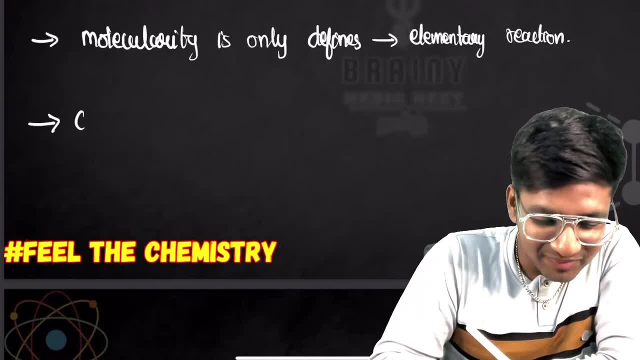 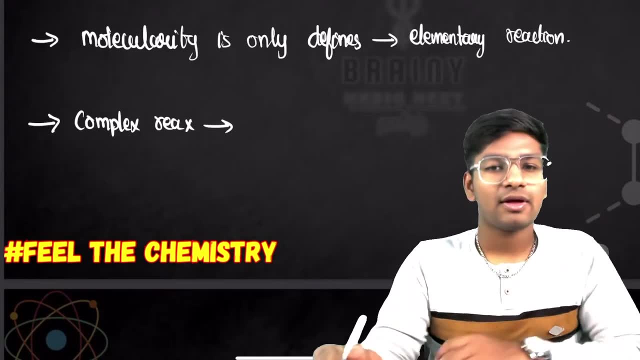 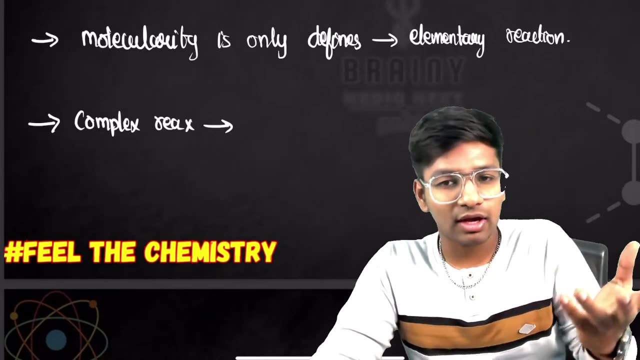 Where will I go with Rs 90 lakhs? This is a good story. In complex reaction, molecularity is meaningless. For example, a person who is single, like me. if someone hits him, it is fine. Reaction will proceed. 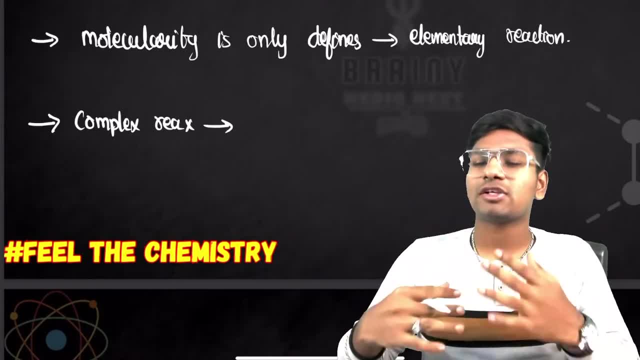 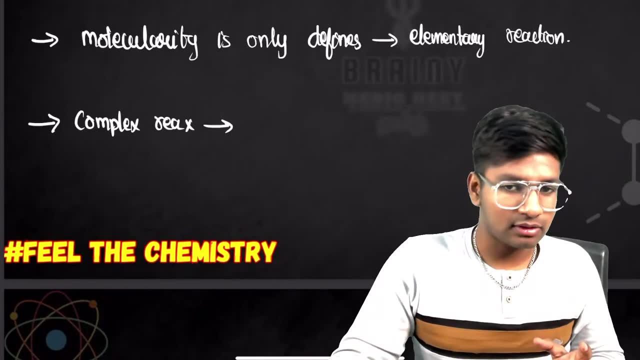 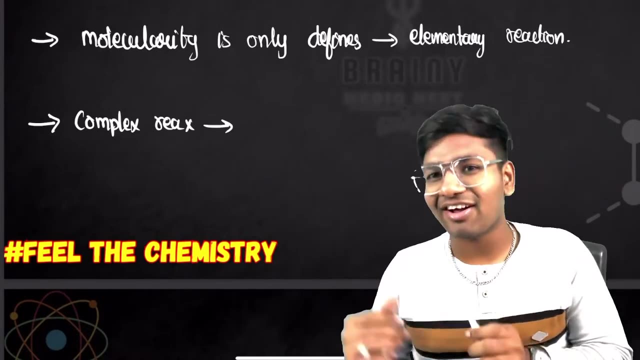 If we have eyes, we can sing and do whatever we want. We can proceed with the reaction and go forward, Because you hit only one person. This is a group of people. If I hit 20-30 people and do the reaction, will it happen? 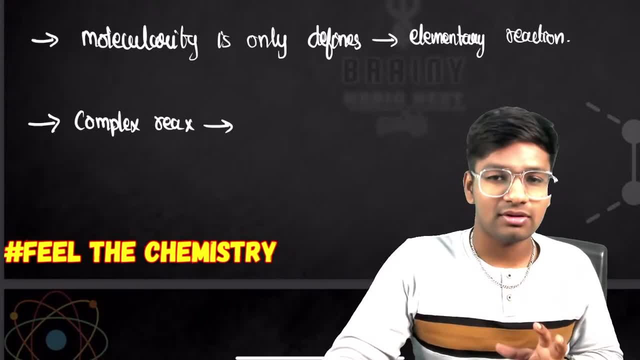 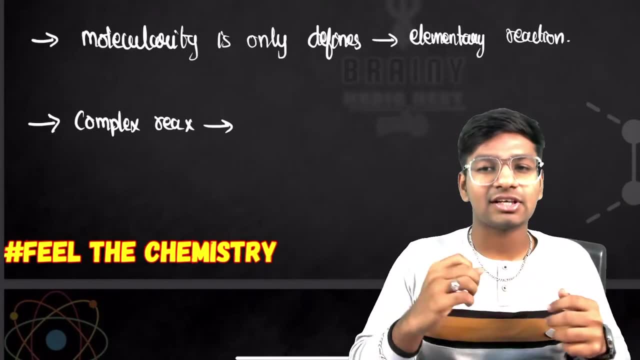 Will it happen? Will it happen? You tell me, If I hit 30-40 people and do the reaction with me, will it happen? Will it happen? Will it happen? If I ask you to do the reaction with me, they will hit you with a slipper. 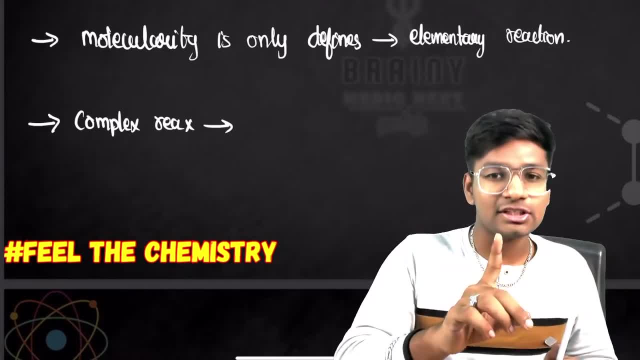 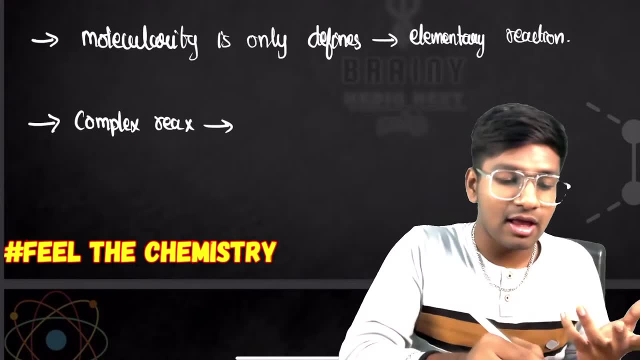 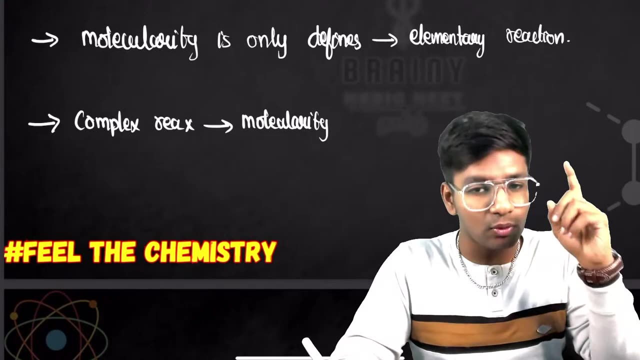 That is the same here. You can only have one relationship with molecularity. If you go to a great person, it will not happen. In complex reaction, molecularity is meaningless. Don't go around like a 90's kid. Don't go around like a Gen Z. 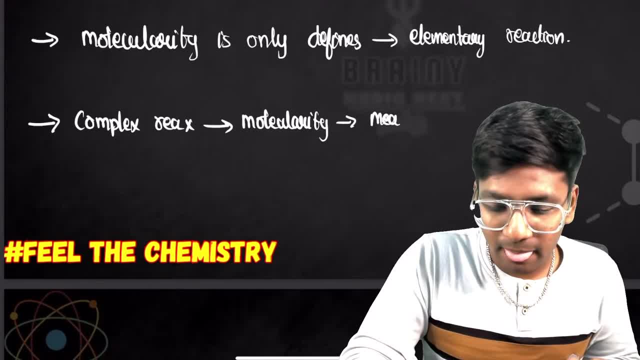 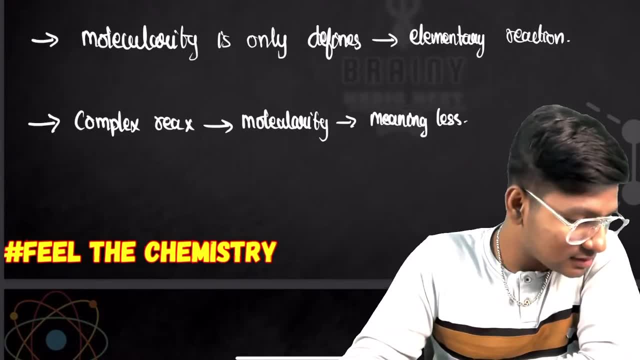 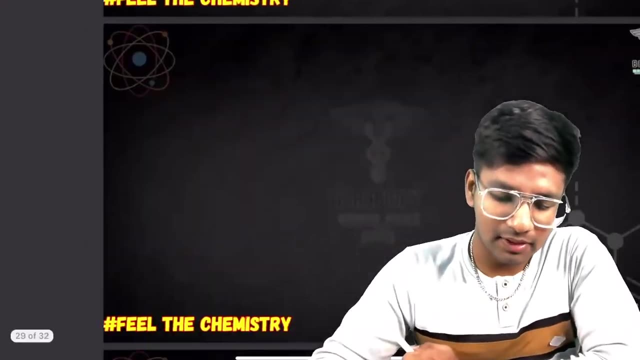 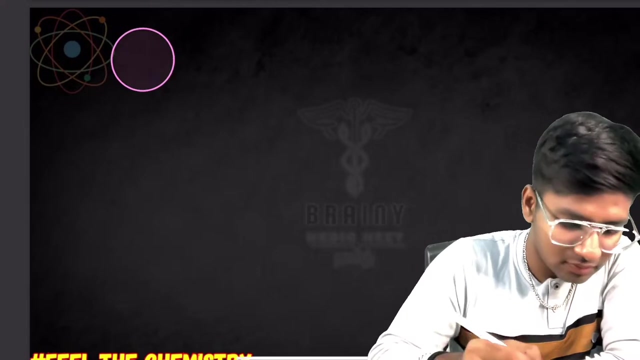 That is what molecularity says: It is meaningless. It is meaningless, Meaning-less, Done, It is meaningless. It is meaningless, It is meaningless. And I can explain this in a simpler way. For example, Here is an egg. I am 20-20-20.. 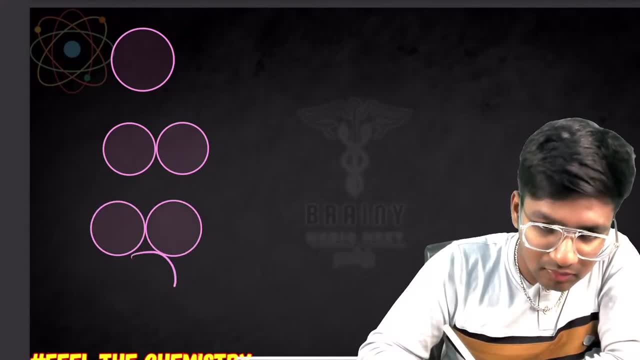 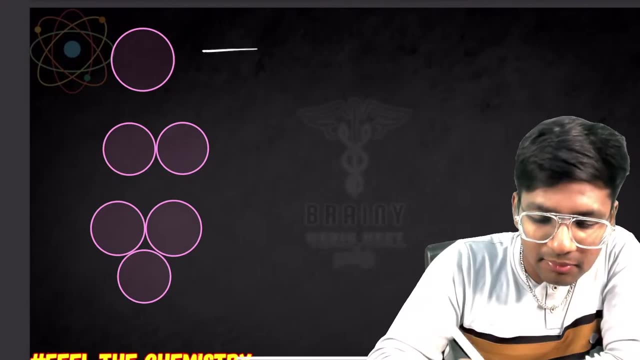 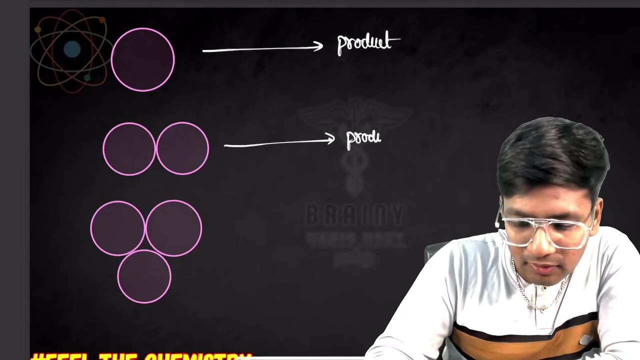 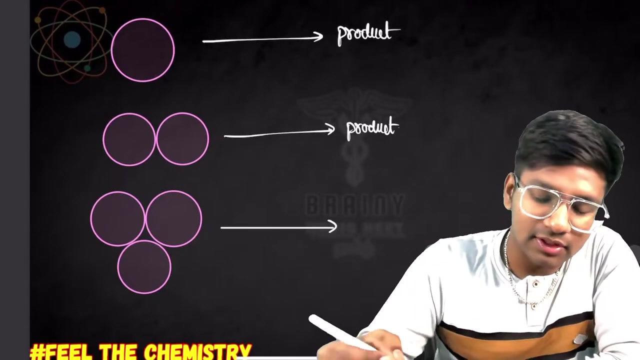 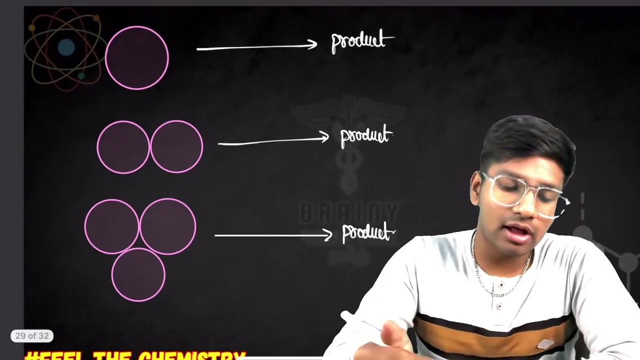 You should describe at a text that an egg is smaller than out size. I did not explain. It is Aegisynthetes, It is only the father of the egg. It takes 1-2 weeks to take the egg product product from one so product and now we know the molecularity, another in. 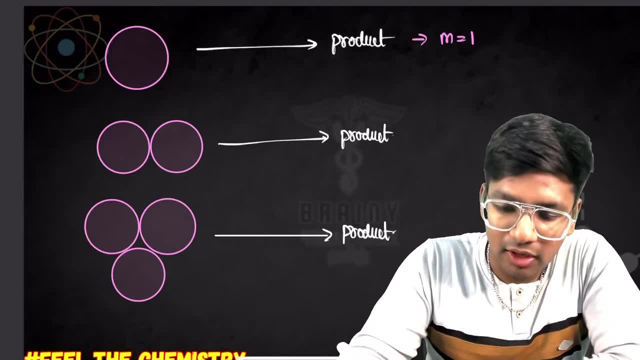 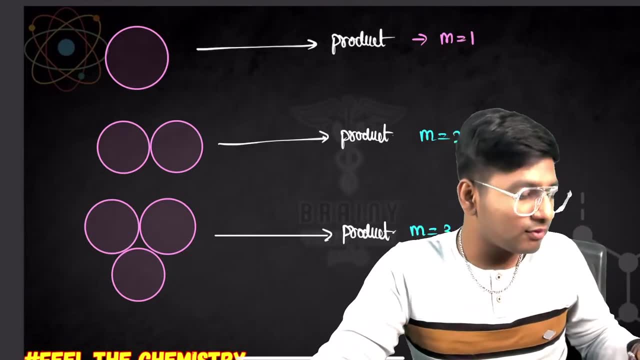 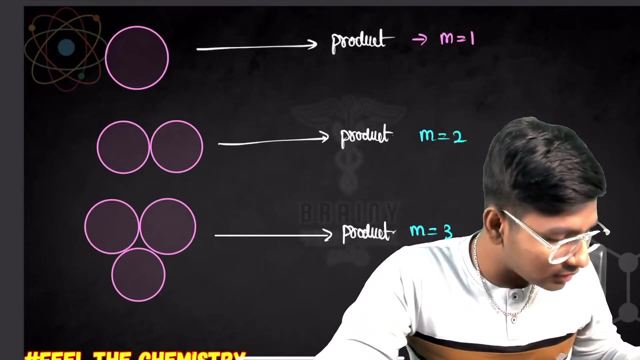 there the molecularity is equal to 1, again in the molecularity is equal to 2 and again in the molecularity is 3. so molecularity or a maximum value, way, freedom, okay, maximum value, the spark there, and that is part, that is fire. I am not saying. 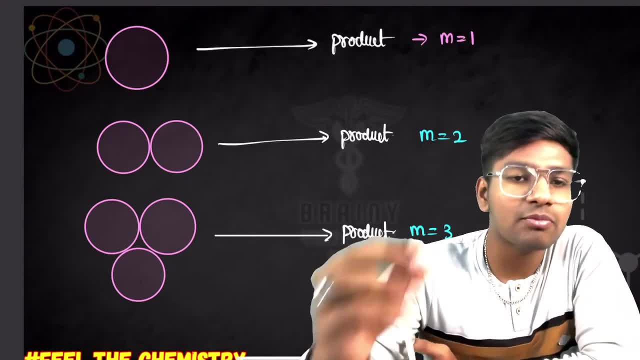 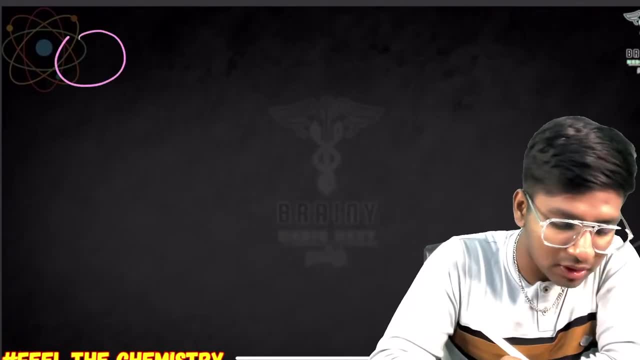 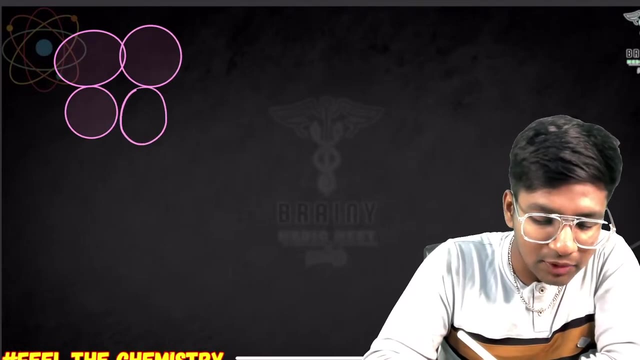 okay, so maximum, maximum value of molecularity is one of the Napa got you go. maximum value, a one of our, for example, now I'm going to get together, now I'm going to. you know I'm going to be together already. you know, not appear up, or you? 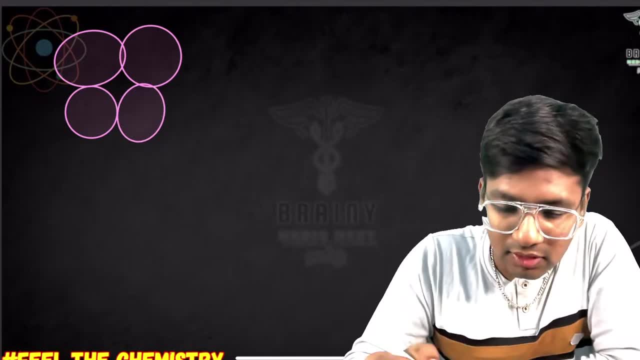 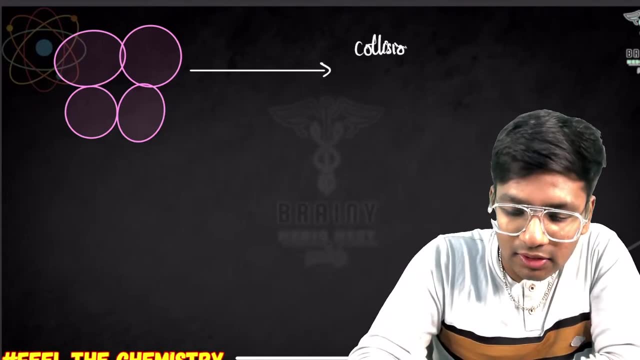 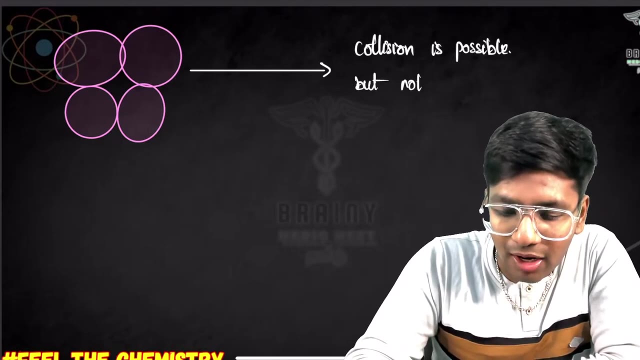 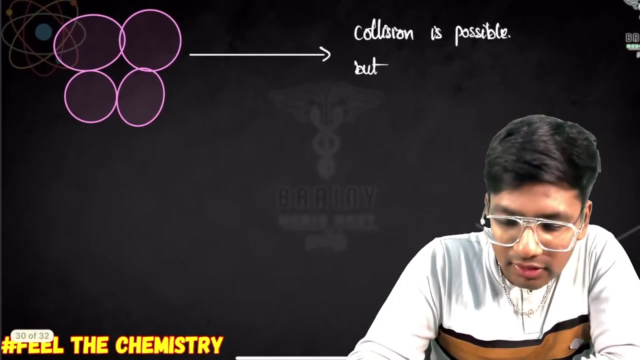 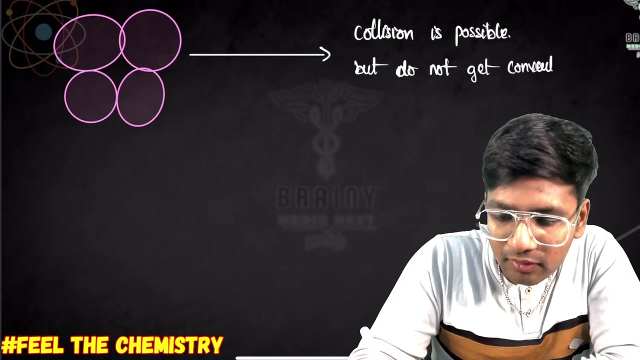 get it. ah, I look at the one that said you're all gonna watch it. you know I love the link. I'm gonna drink. yeah, didn't. so deep collision is possible. collision is possible, but not convert. do not convert, but do not get converted into product product. 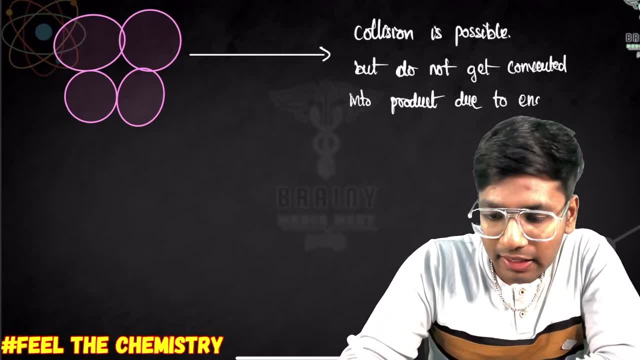 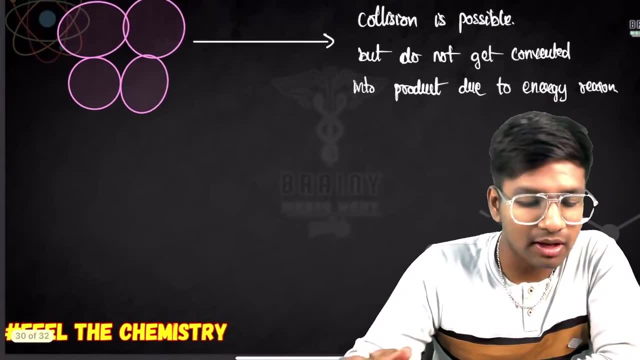 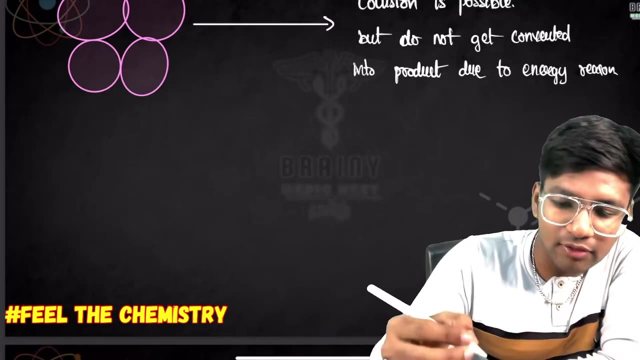 due to due to energy reason. right now, okay, will, often you need each of you know, yeah, will take your co-silo, polar dogs will up, or you teach a bunch of the planet. you come here, are you about you know? so I, at the end of this, what I'm trying to say is: okay, molecularity can be. 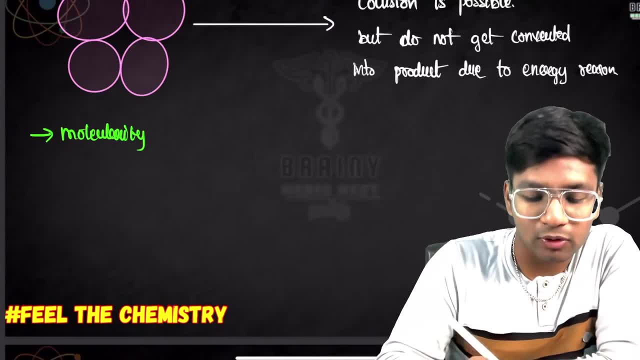 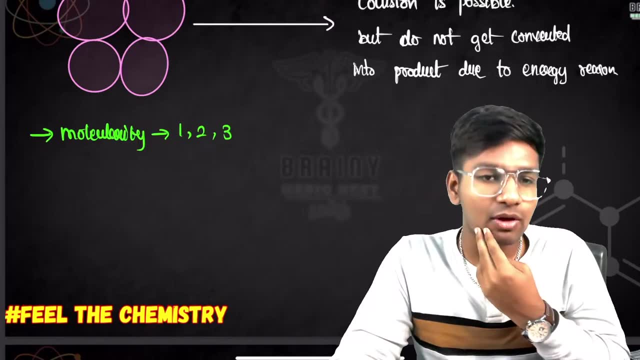 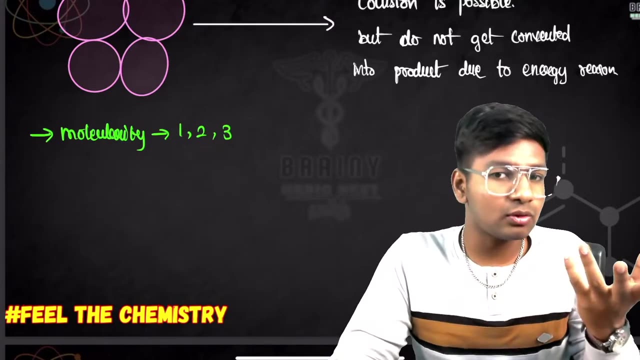 Instagram, whatsapp, snapchat in the moon or 79 minute by Maria so moon, when I had been under integrate on amuna. on it any time you want the memory for me, or If you want to message on Twitter or Facebook. you will not be able to maintain it from the 4th. 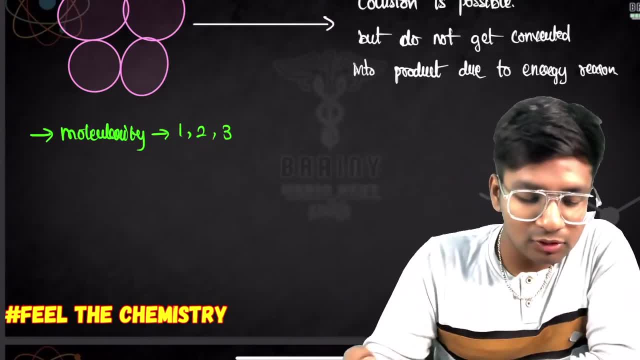 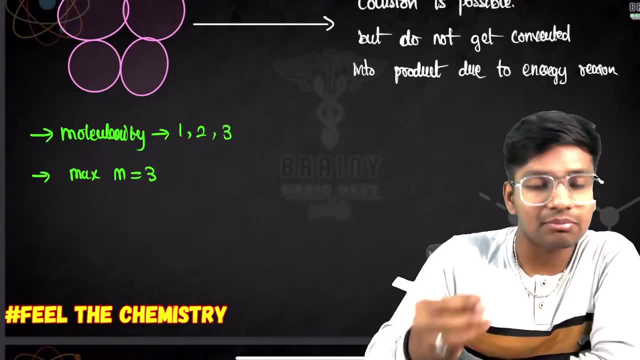 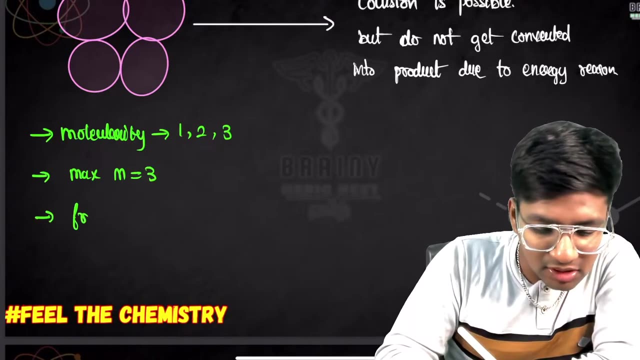 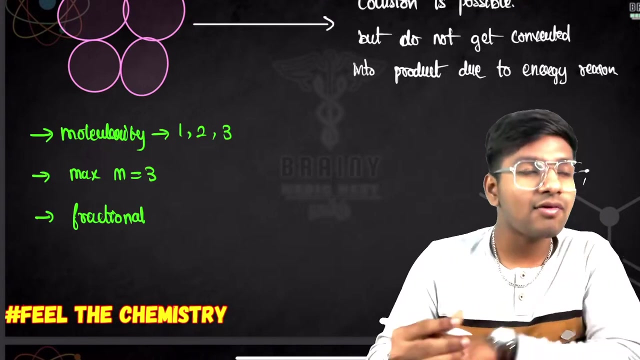 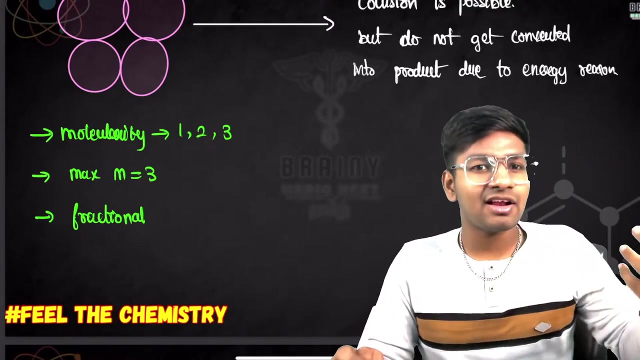 So the maximum molecularity is 3,, not more than that. So the molecularity is Fractional. I have seen only half of her. I have seen even half of her. can I say it like that? No, I have seen even the angel. can I say it like that? 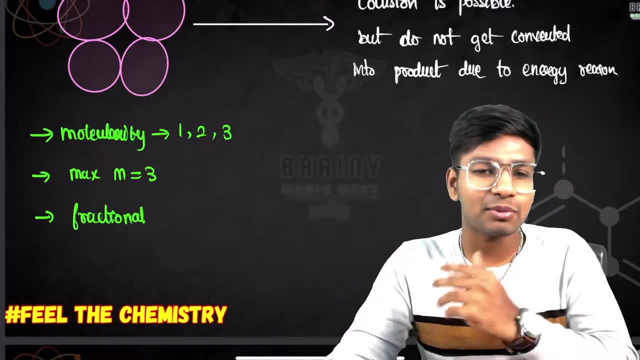 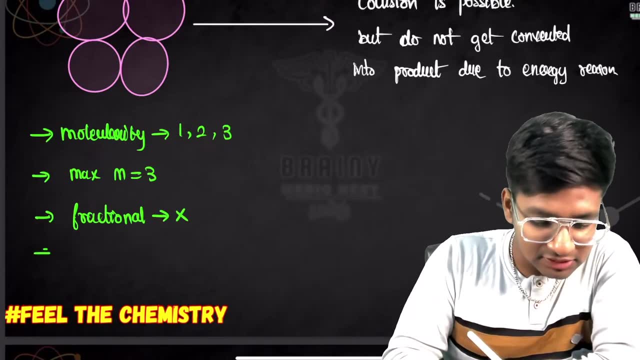 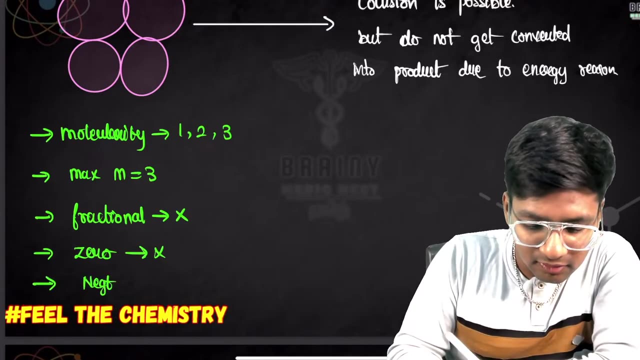 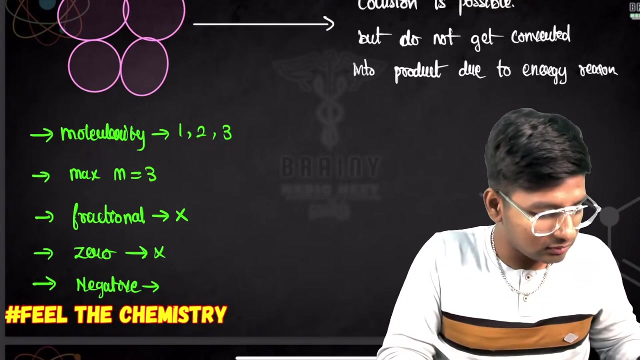 I have seen half of the angel. I have seen only half of it, but I haven't seen the remainder. So there is a fractional. Similarly, there is zero. Zero is the maximum will occur. zero possibility: color: negative, negative, negative, no, no possibilities for negative. also now the negative possibility: career. then. 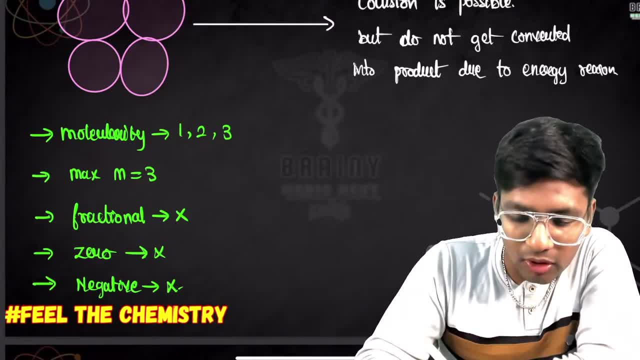 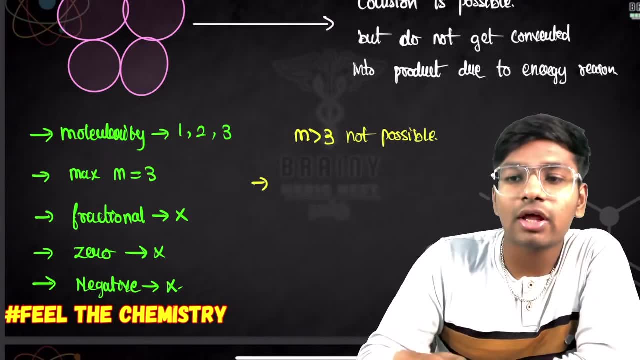 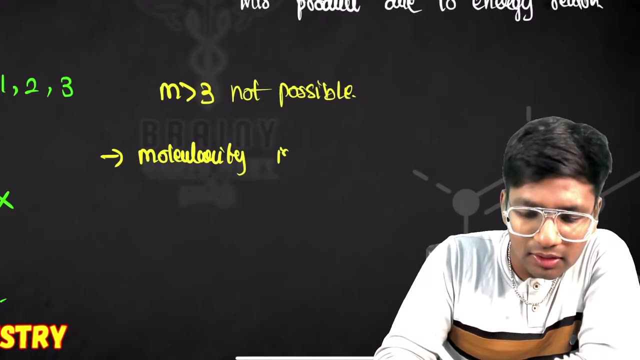 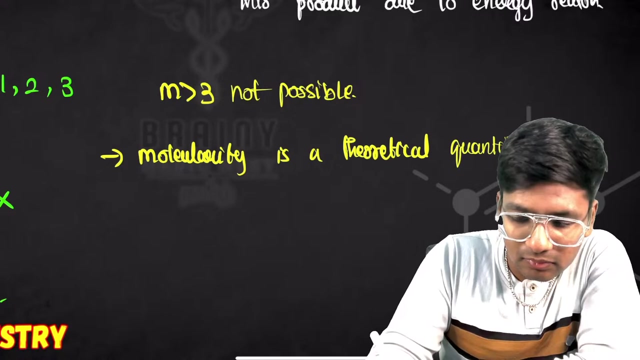 anyway, by clarity, are in or into pointer came to point in molecularity greater than three? not possible, you don't care, all they already listen to the. and molecularity said: theoretical quantity, practical quantity, career molecularity is a theoretical quantity, then, and then just just for example, 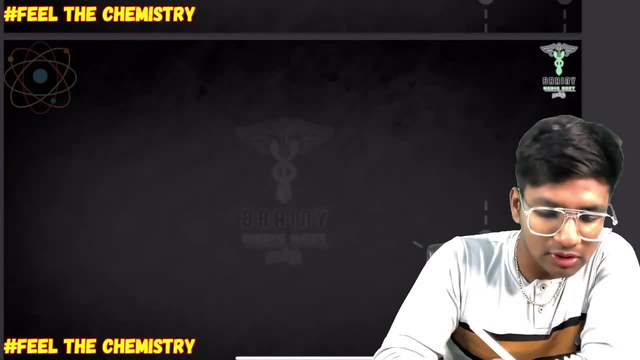 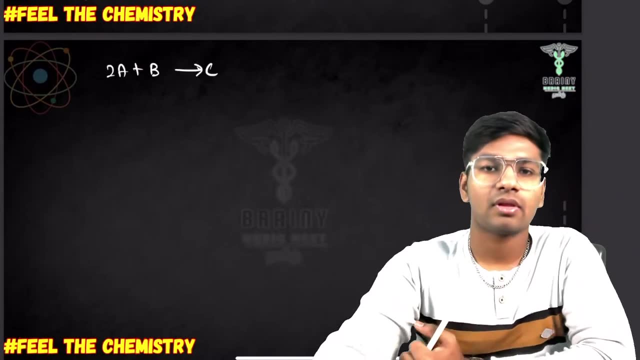 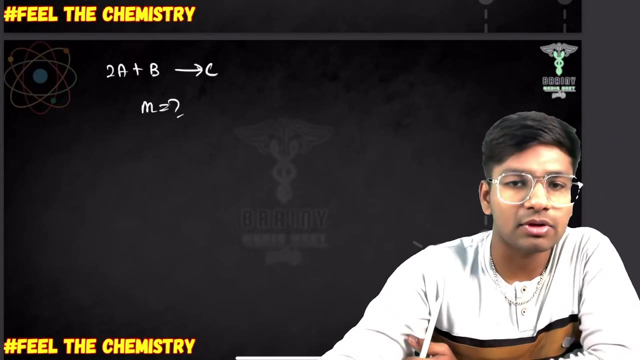 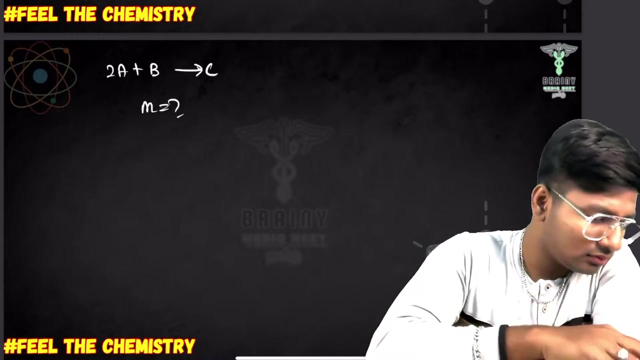 elementary, the elementary reaction, and 2a plus b gives c. what is the molecularity of this reaction? tell me what is the molecularity question mark. what is the molecularity of the reaction? it will ask: 3 maximum is 3, this is 2, this is 1 and this is 1. 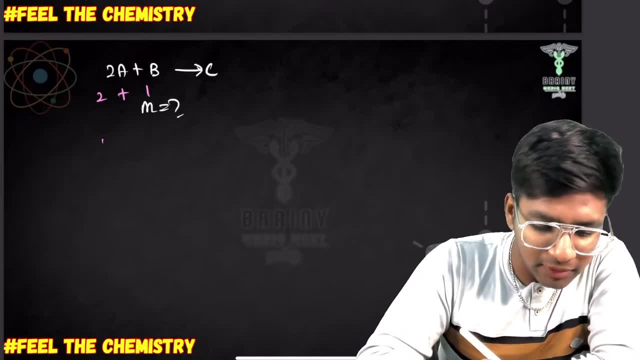 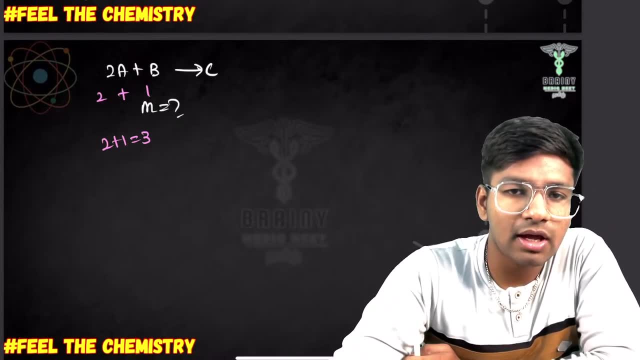 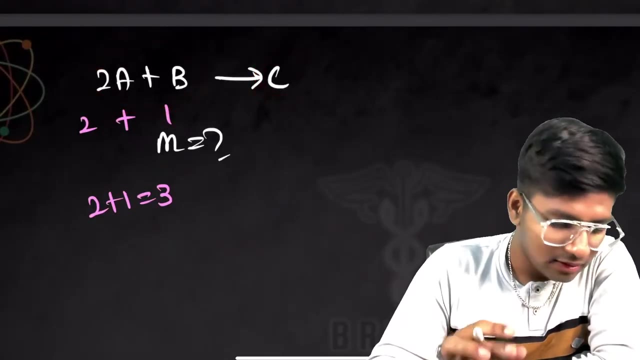 sorry, we have to add only this: 2 plus 1, which is equal to 3. done, ok, did you understand what I said? are you going to add anything in this? cell reaction is happening here. this is product. do you understand what I am saying? 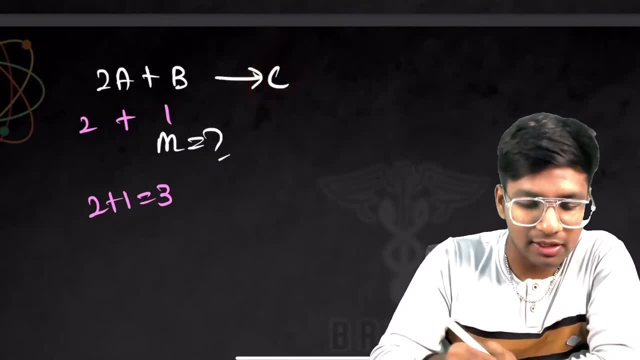 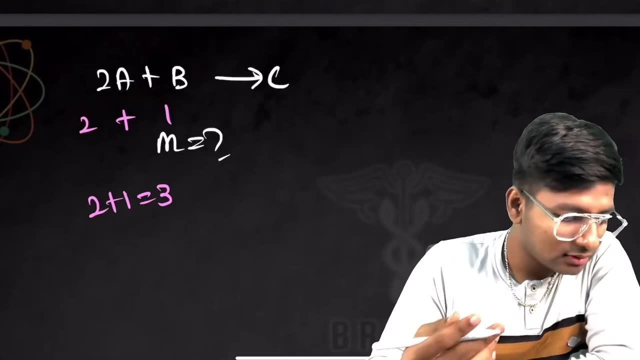 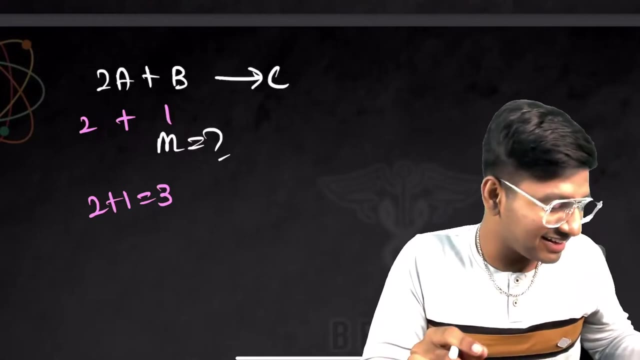 this is after marriage. this is after marriage period. this is before marriage period. this is before marriage period. do not go to this, proceed only with the reaction. I don't understand what I am saying. ah, you didn't understand. you understood before that you have to proceed only with the reaction. 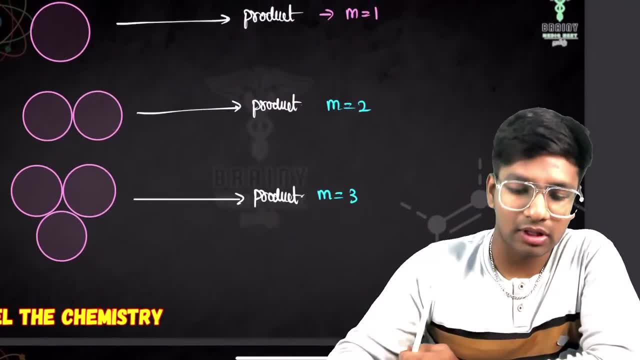 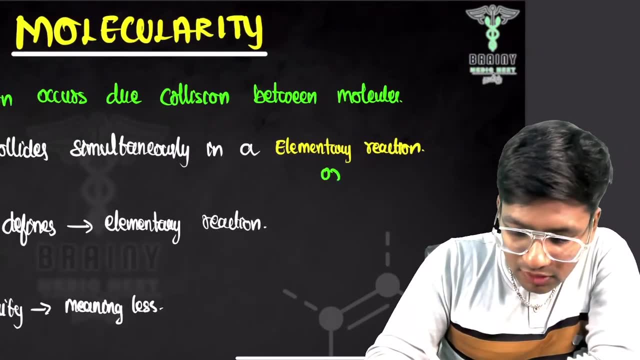 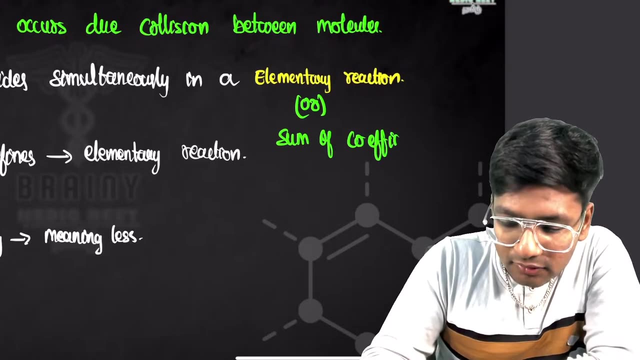 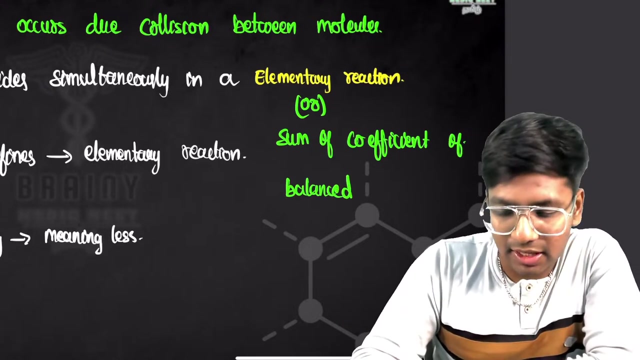 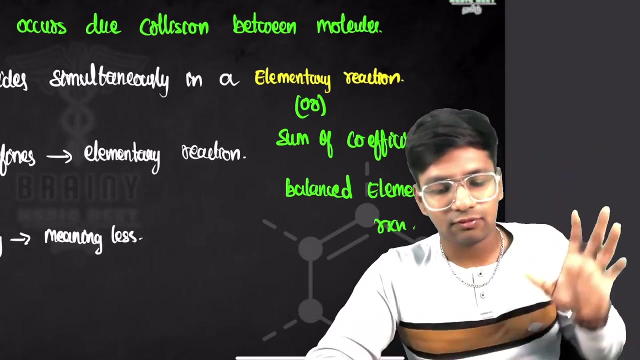 I will tell you another small definition. you can write it in this definition. so again, you can also give this definition, oh, or, or some more, some more coefficient. coefficient of balanced, balanced elementary reaction, reaction. that's it for today. that's it for today. any doubt till now. 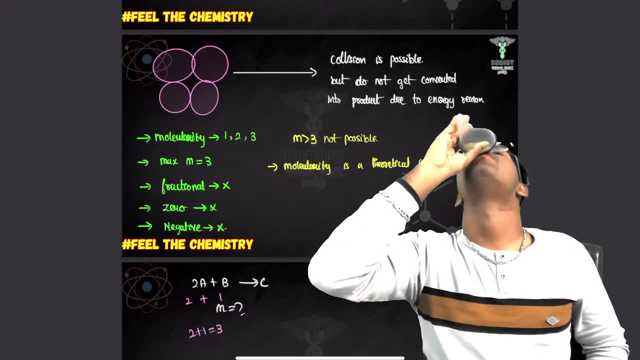 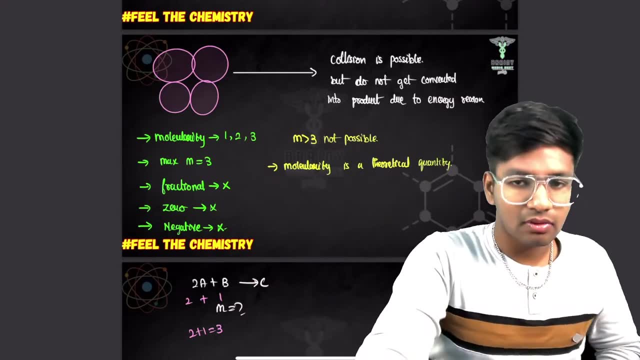 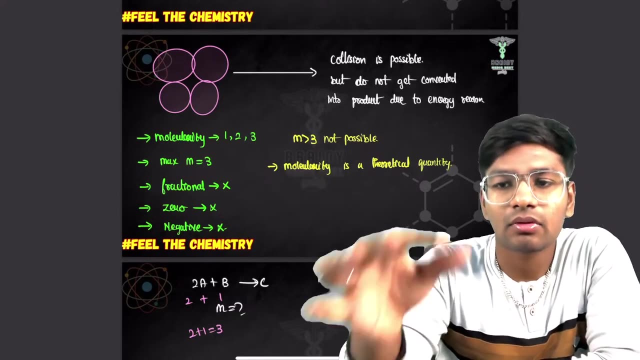 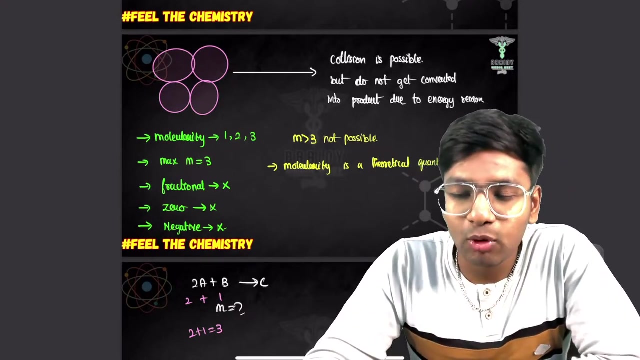 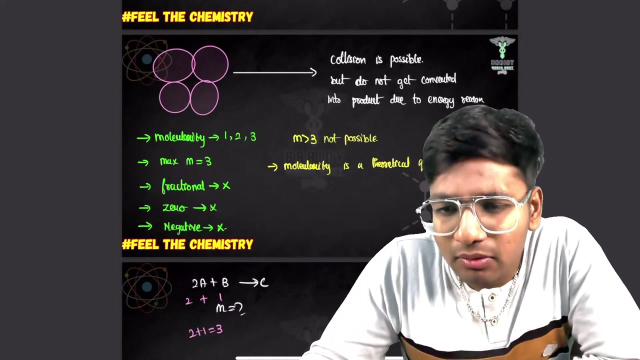 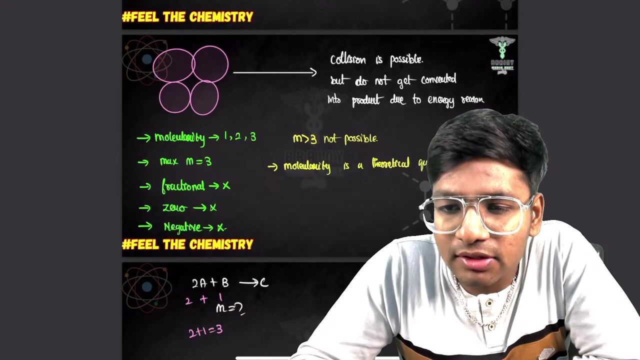 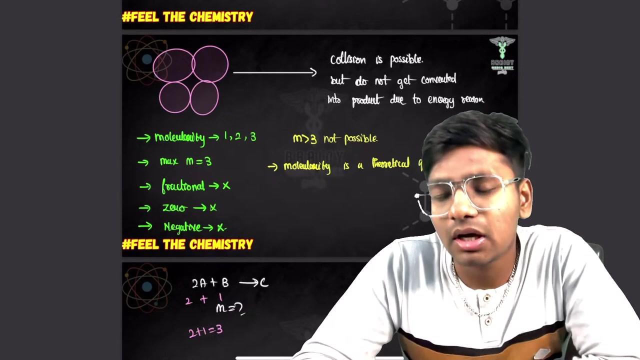 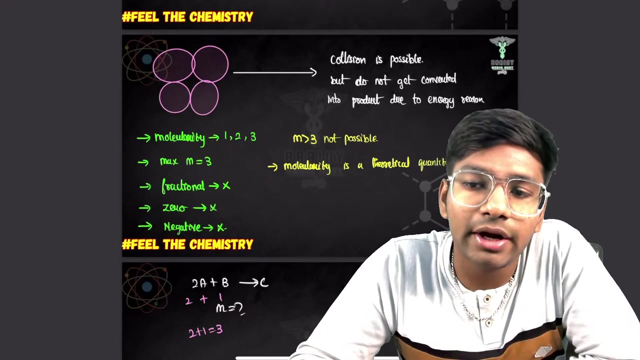 no, ok, How old is your iPad? I think it is 1993.. You have said that reaction with hydrogen acidity increases down the group. You have said that reaction with oxygen acidity decreases down the group. Acidity is something. How I measure acidity in hydrogen. 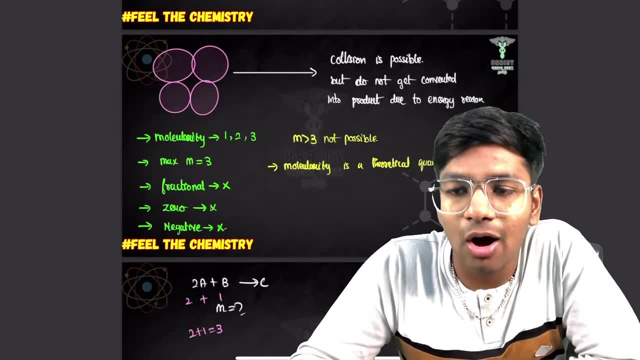 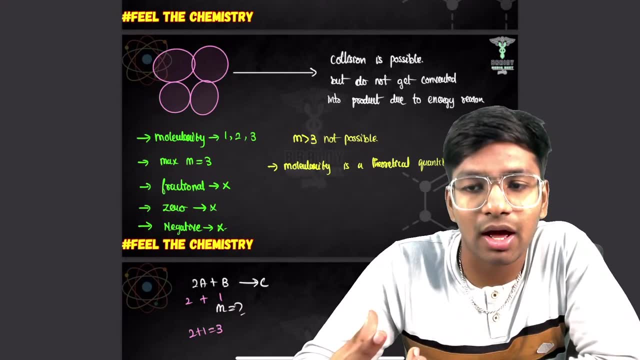 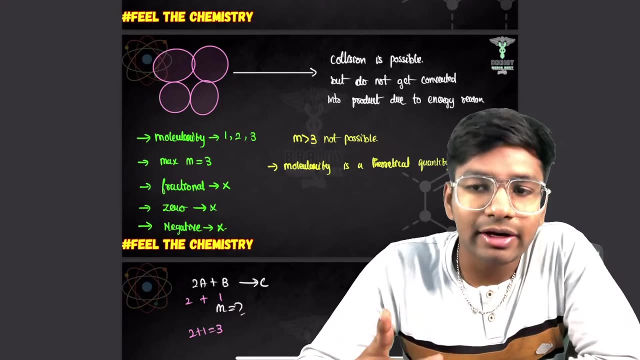 Ability to donate H+. How I measure in oxygen, I measured with electrons. If we accept the electron, more electron activity is required. So down the group: when oxygen is present, it decreases. When hydrogen is present, size increases. H plus is increased. 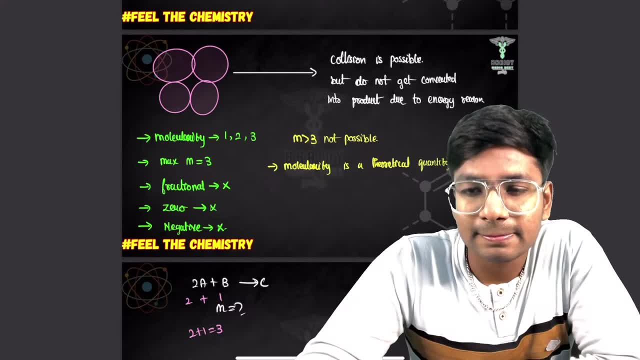 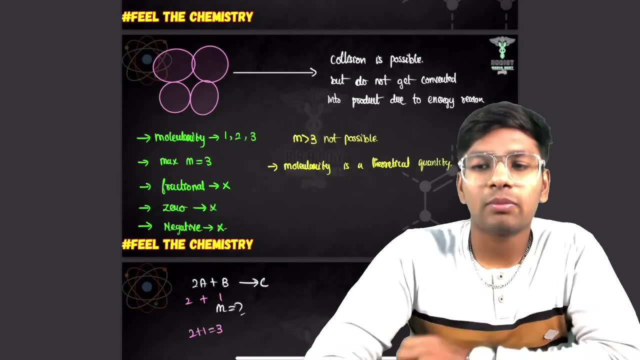 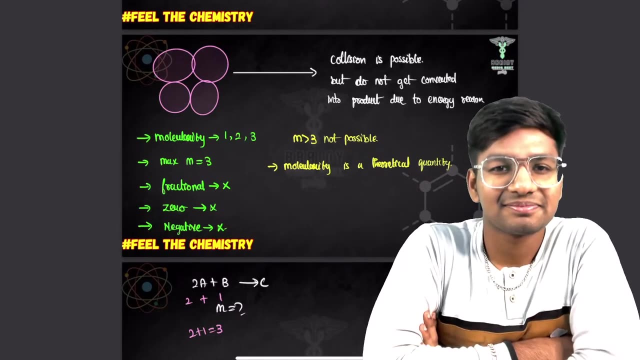 H plus donation increases. That is why I have said so. That is why I have said so. That is why I have said so. Okay, One post for tagging you, bro. I will sit like that, No problem, Yo, Yo. 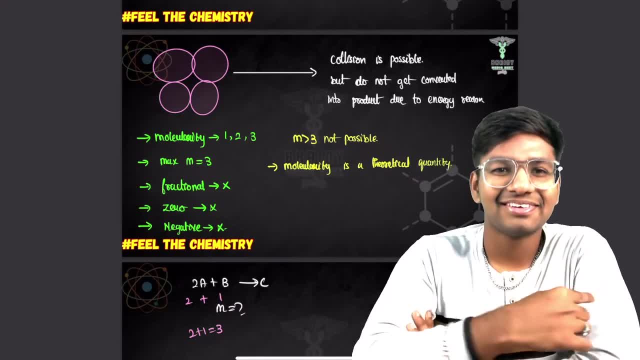 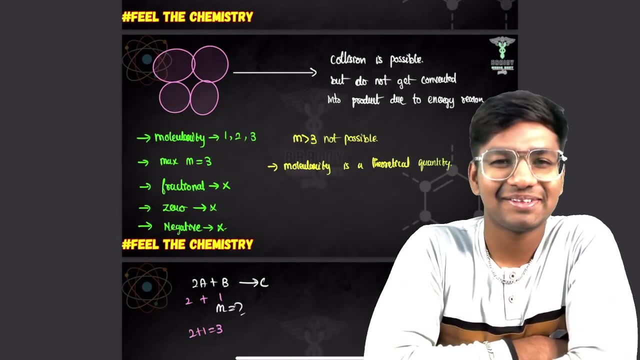 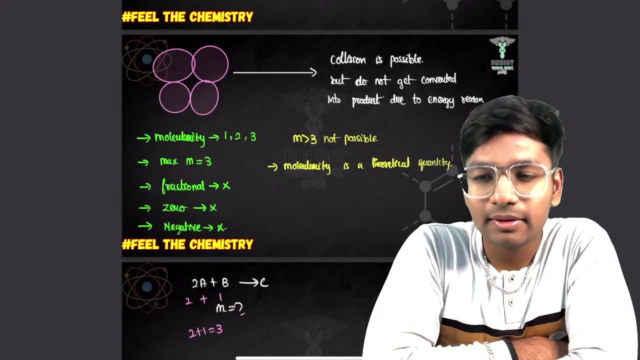 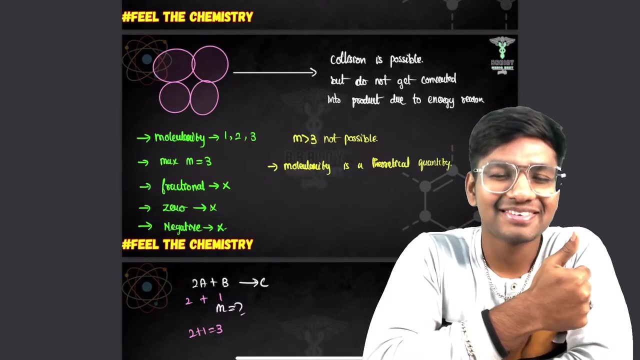 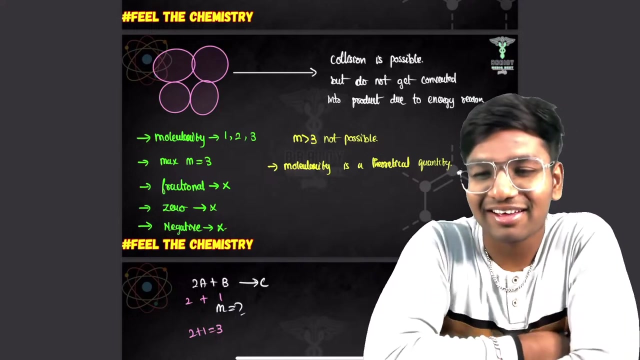 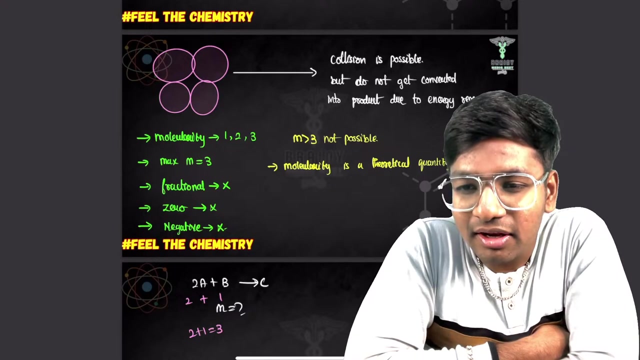 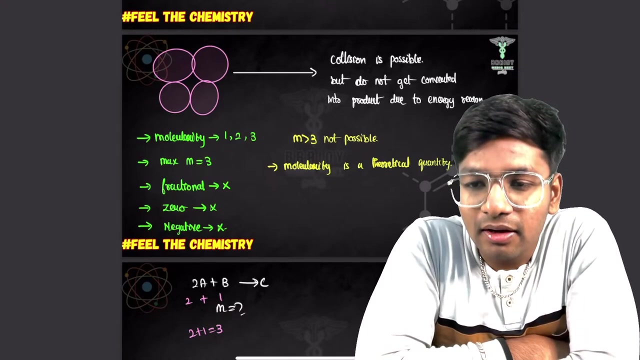 Yo, Yo Yo Yo. I will say the all the best. What happened? Smile, please. So, So The post. there is a girl with me. she will be giving this post often. ok, he has become a Tamil educator, is that? so he is running Tamil. he will post 2D. I will do it. I will do it. so see, they will put a meme old crash course in YouTube. ok, let's see, no problem, all this is the same. how is valentine's day valentine's day? I don't have any connection with that, please. 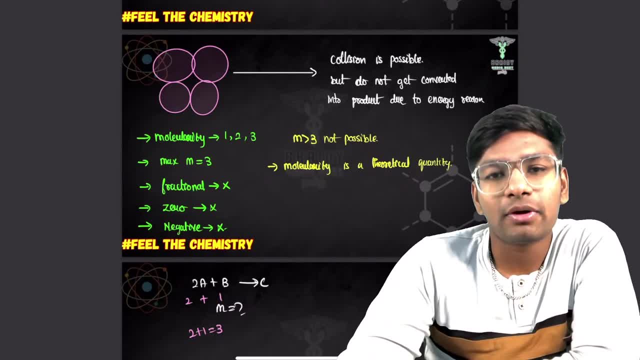 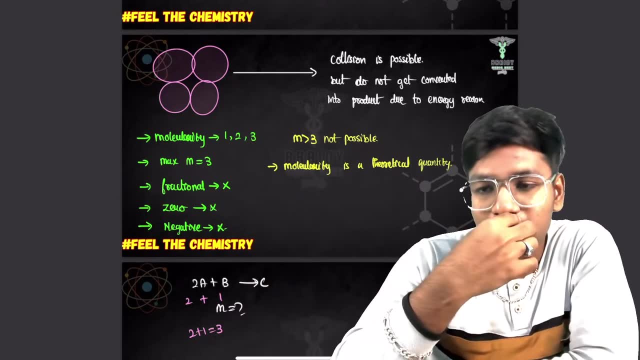 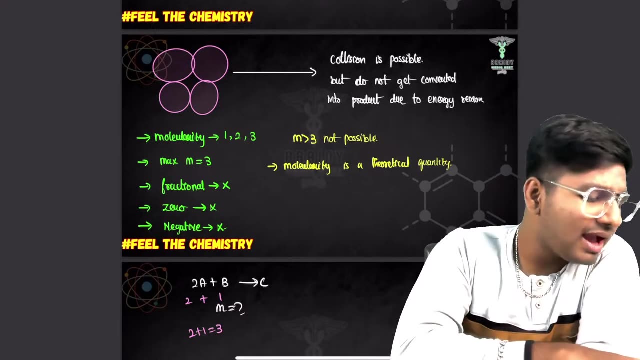 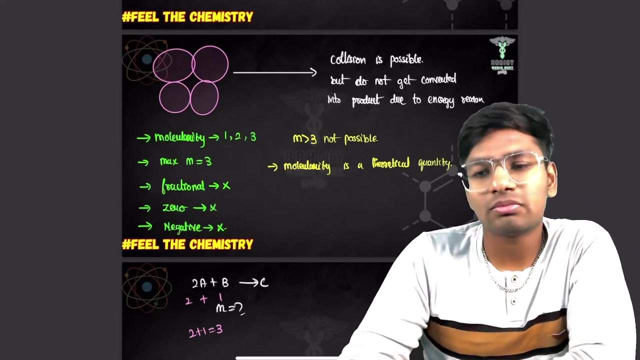 don't ask me anything. ok, see, I hope you guys will comment. ok, I hope you guys will comment. tell me how it was ok, tell me how the session was ok. then only I will know. and that question series- that is post-mortem series- share it with many people. it should reach many more people. ok, it should reach many more people. 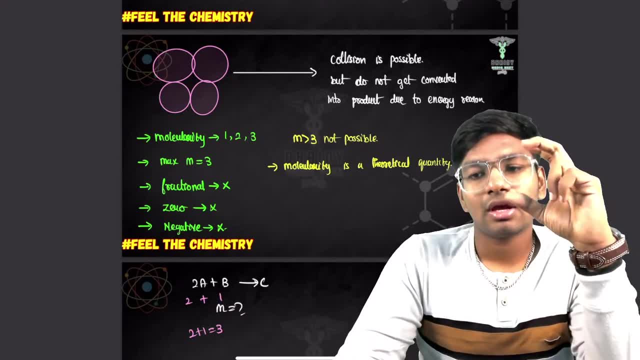 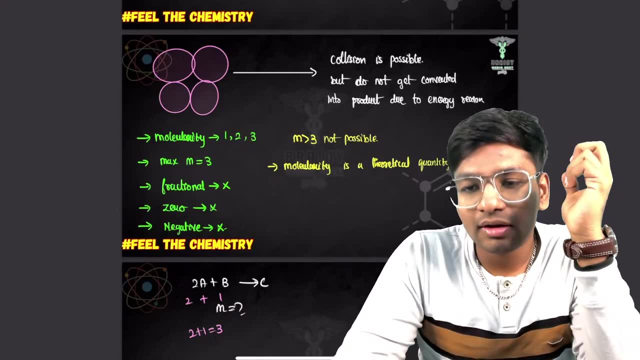 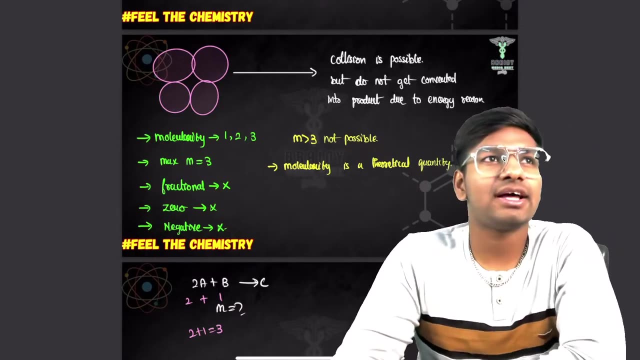 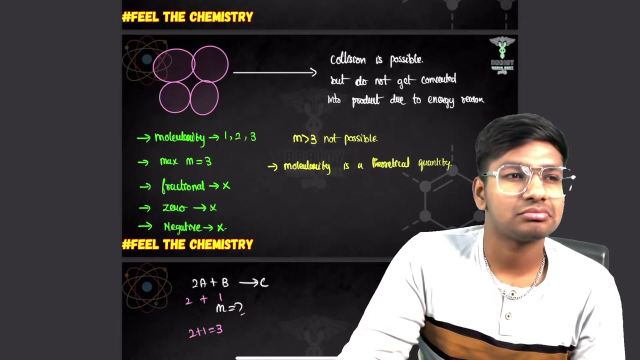 rate is something which you measure for an individual thing, individual thing. are you British? no, ok, so see. ok, tomorrow I will do the NCRT review session correct, will do small lesson. what lesson can we do? pblog, remaining pblog, can we do? 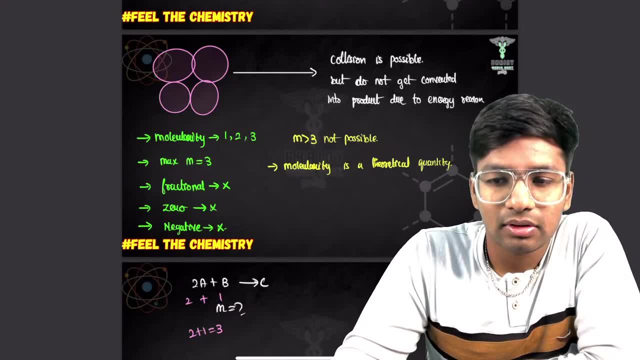 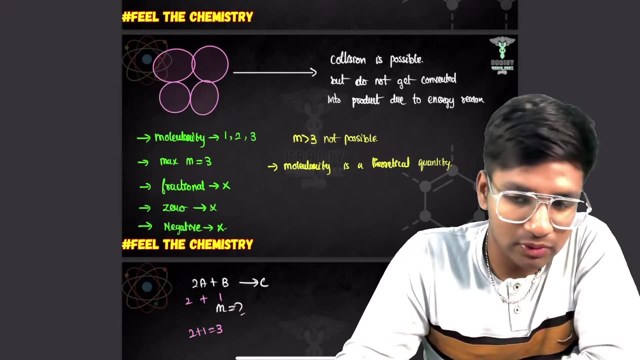 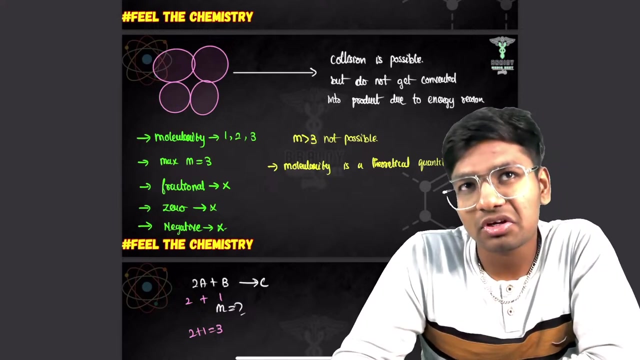 tell me what we can do. chemistry, yes, we have to do chemistry, but ncid review, what ncid review we should do. we don't know actually what to do. chemical coordination- electrochemistry, tell me in small lesson time, will be less coordination, chemistry remaining p block. 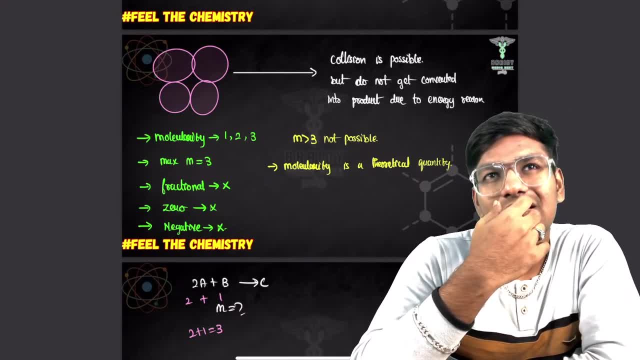 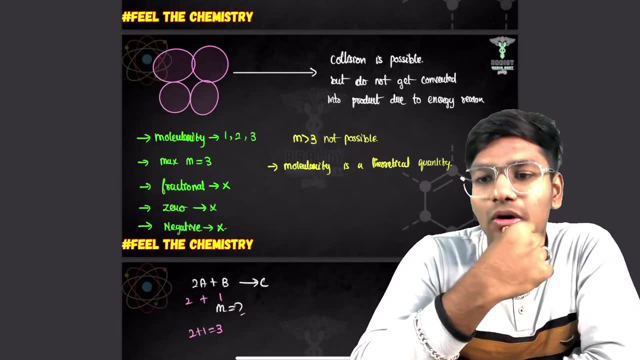 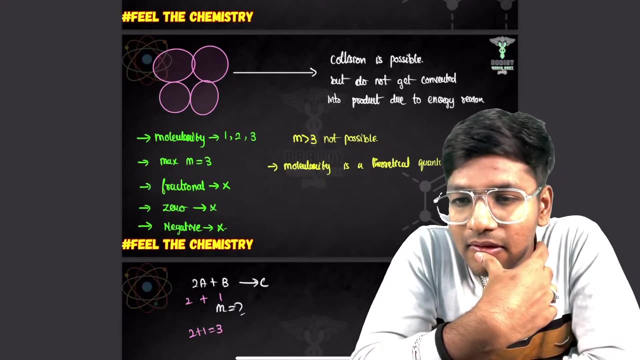 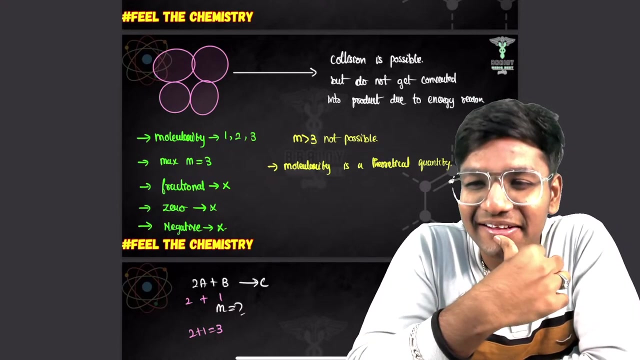 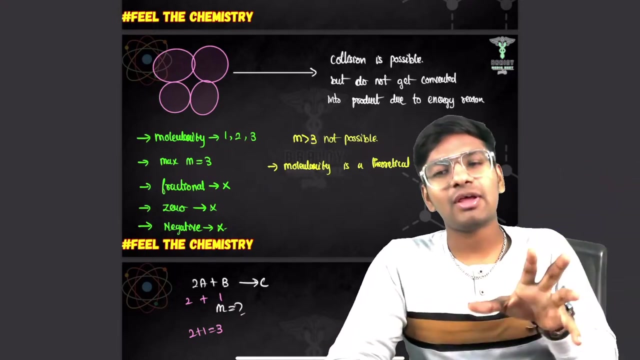 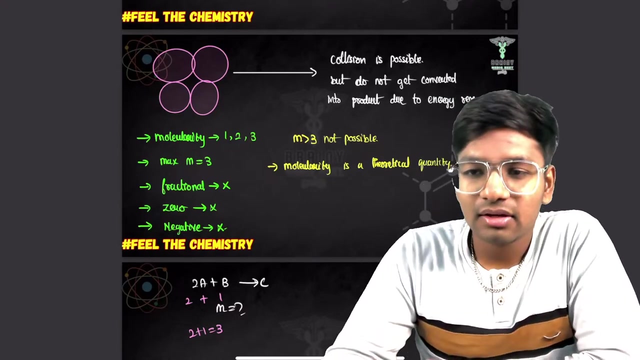 poc amines, alcohol, phenol. will they like it? what is this? why will they like it? rate rate is something. rate is something. rate is something. chemical reaction: you measure, that is rate, that is rate. ok, so see, we will meet tomorrow. i hope you guys will comment. 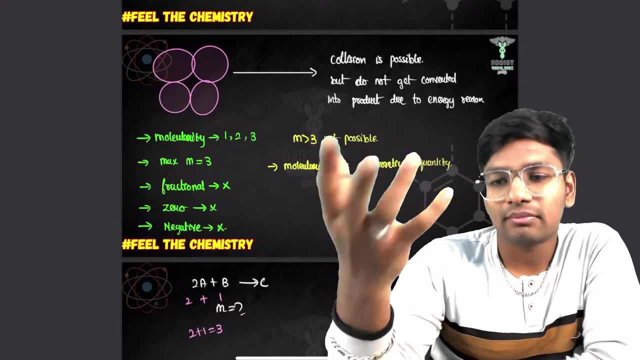 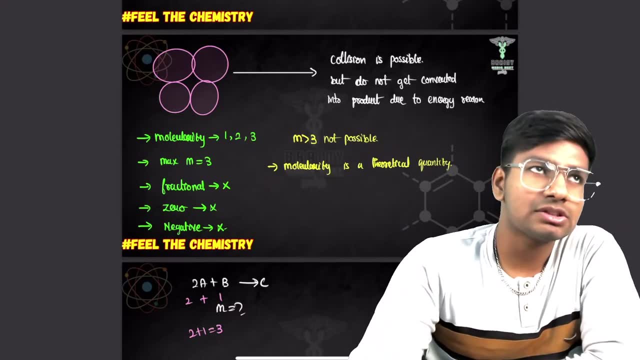 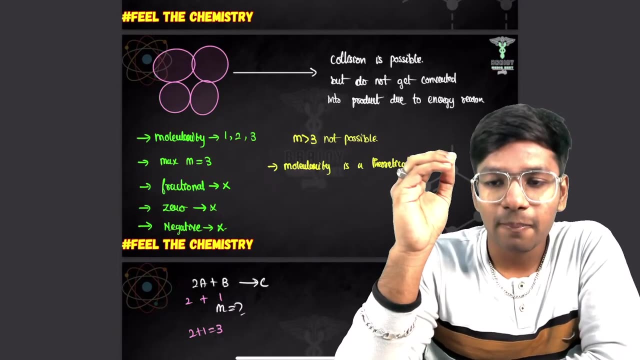 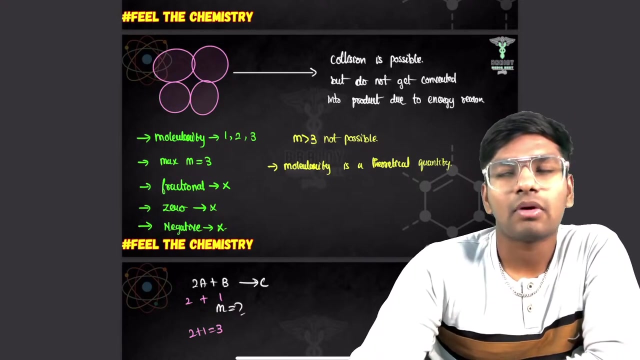 do comment. how was the video? ok and like share, subscribe, comment. next part of this lecture: i will take sunday because i need more time this lecture to complete it fully, ok, ok, tomorrow i will take ncid review session, or else tomorrow ncid review and chemistry. then saturday i will take nuclei. 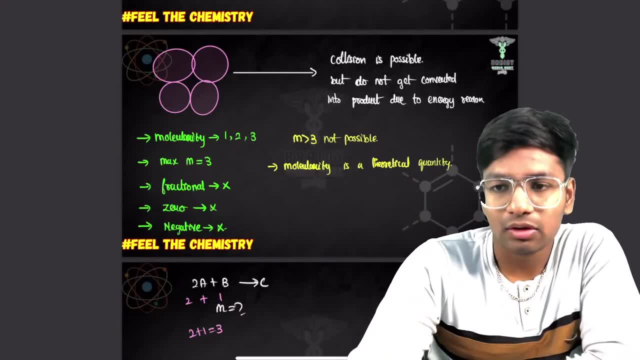 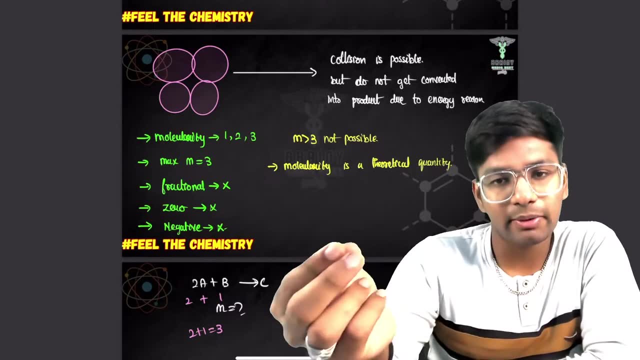 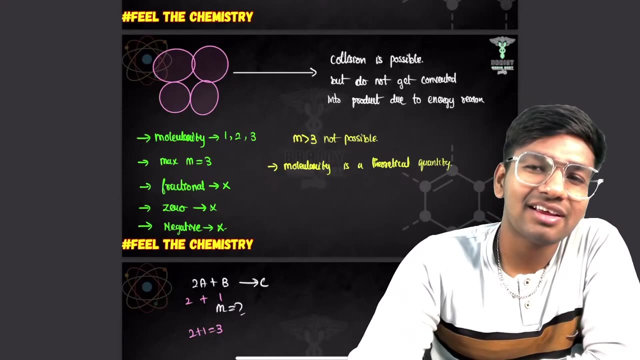 ok, i will take nuclei on saturday. saturday, i will take nuclei lesson start, but it will go to 2 parts. cute bro, you are here. please show, please, please don't know. please show me if you know, i don't care, i don't care, i don't care. 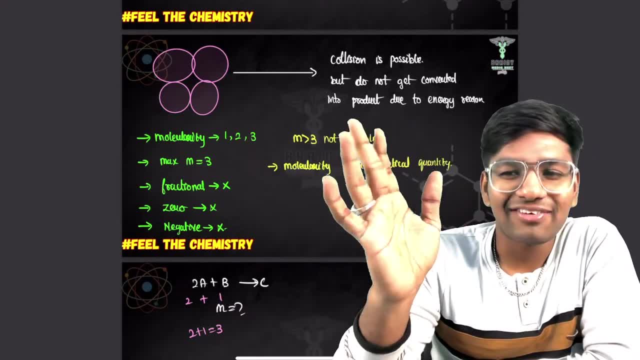 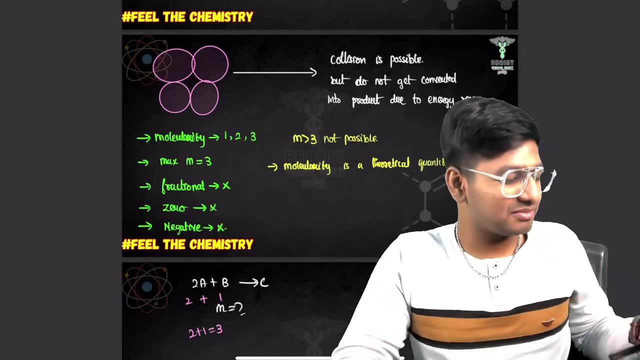 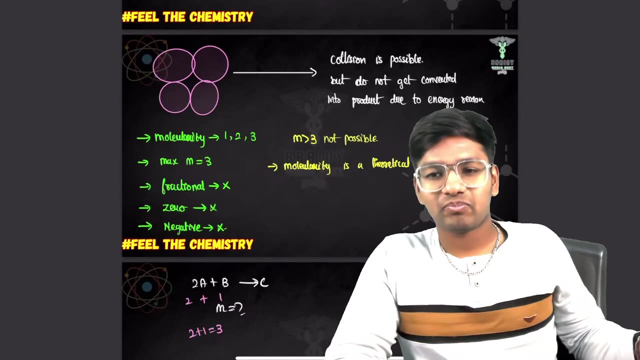 i will tell you you want to come, but i don't know what to do. what to do? ok, don't talk, because son is waiting. don't worry about it, don't care, we will speak later. ok, ok, bye, bye, bye, goodbye, good night, bye, bye, good night. 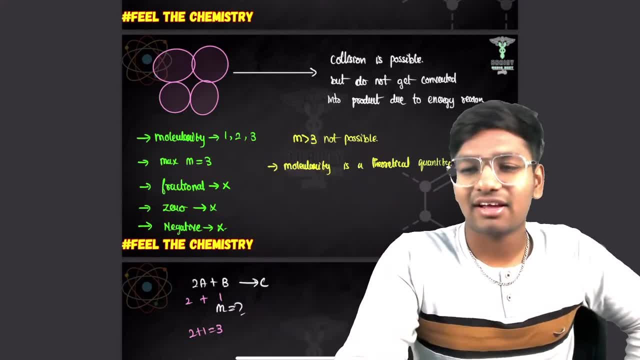 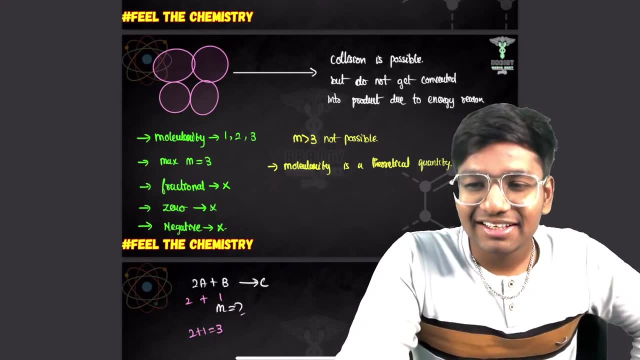 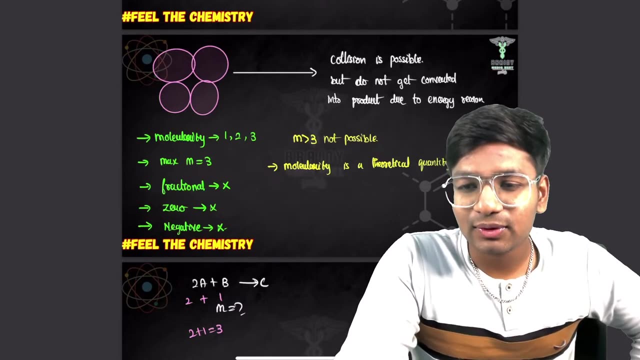 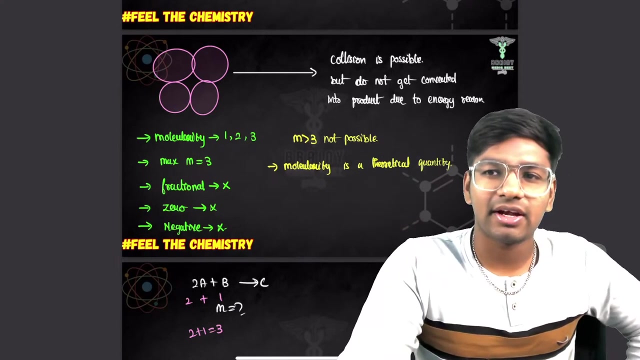